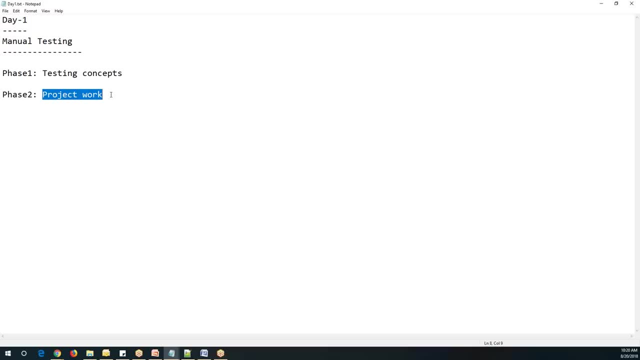 how to write the test cases okay, how to execute the test cases, how to find the defects, how to report the defects. So all these things comes under the project work. So while learning those concepts, parallelly you do also projects. So whatever concept, you learn the concept. 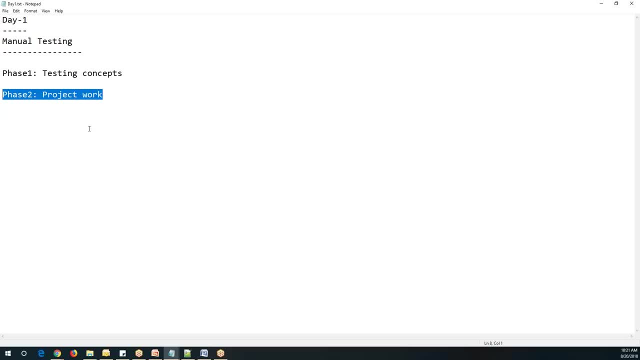 will be applied in the project. So parallelly you will learn both side by side. This is a phase two And the phase three once we have testing, concept learned and project work, and also the phase three. I'm going to introduce a few tools like test management tools and 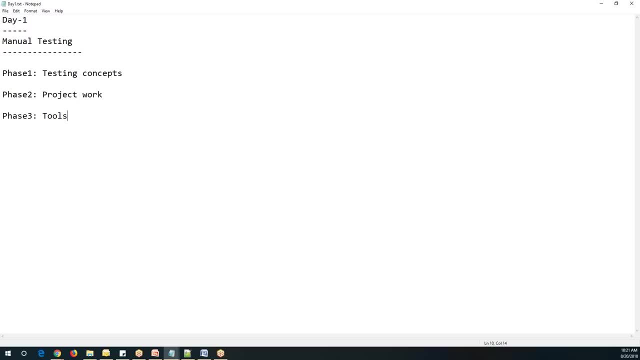 buck tracking tools and also agile process. Like today, agile is a very important process in a real time, So I'm going to use multiple tools. So, especially for agile, we use a JIRA tool. I'll tell you how to create the project, how to update the schedules and how to add your test cases and how to execute them. 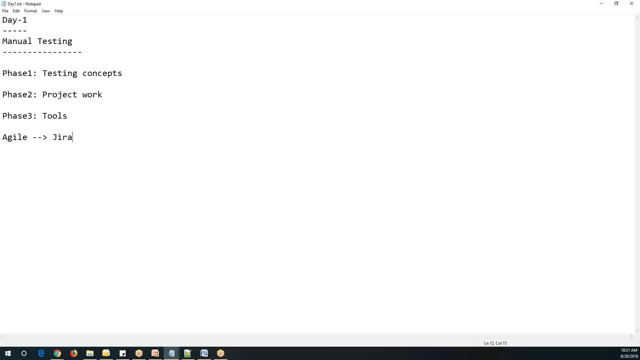 Okay, how to get the reports, Okay, All these things will discuss about the JIRA tool, how to create the bugs, how to create the test cases, and all will be part Of the JIRA. So in the phase 3 we are going to learn about completely agile process and a JIRA tool. 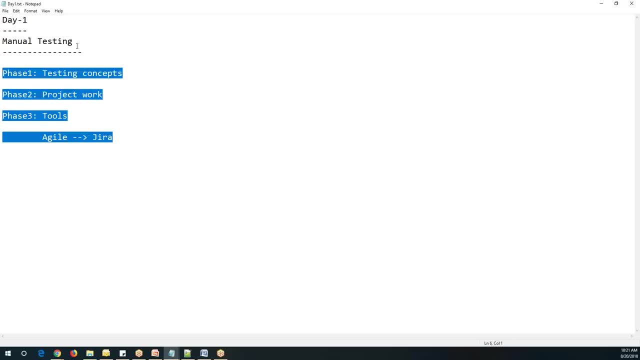 Okay, So these are the things we are going to learn about manual testing. so phase 1, we are going to learn testing concepts, and phase 2, we are going to learn the project work, and Then phase 3, we are going to use a special tools. Okay, Now I'll go through in detail in phase 1, what we are going to learn. 2 & 3. 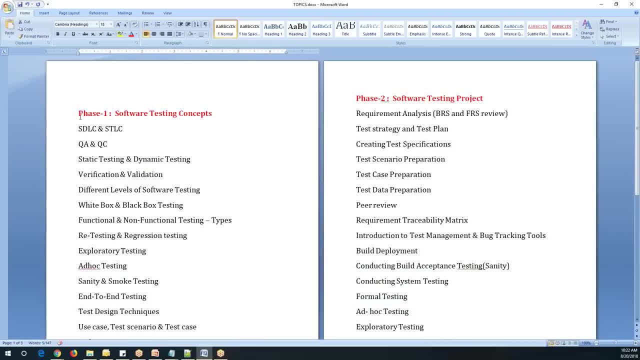 So let me just share small document here. So in the phase 1 we are going to learn about HDLC, and HDLC means software development lifecycle versus software testing lifecycle And many more concept we have. so these concepts will take at least 3 to 4 days of time and 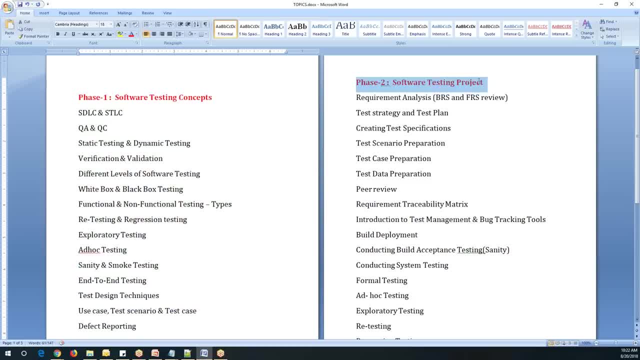 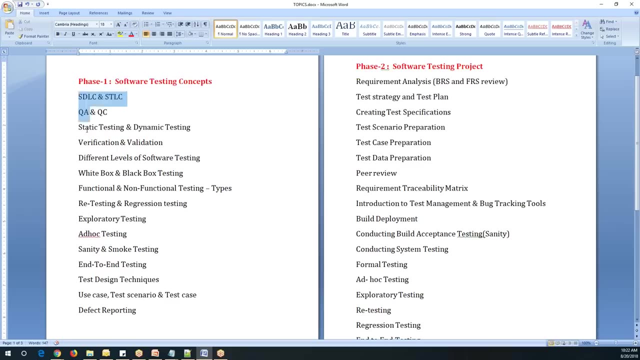 Then we'll discuss about the software testing project. So as part of this, this is our completely practical. So first phase will be completely theoretical, because until unless we know basic concepts, we cannot directly jump into the project. So first we need to know about the. what are the different topics or concepts which we required to enter into the project right? 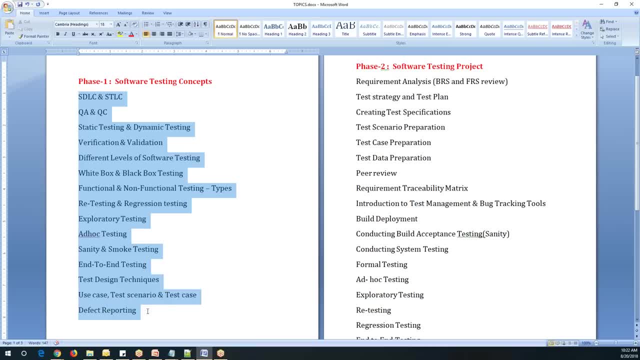 So the phase 1: we are going to learn different concepts and it will take almost 5 days, almost 1 week, and once we get in familiar with the concepts, then we'll jump into the project. and Phase 2, it is completely practical part, Okay, TG plus part. So we will understand the requirement document and then we'll review it, will prepare the test plan. 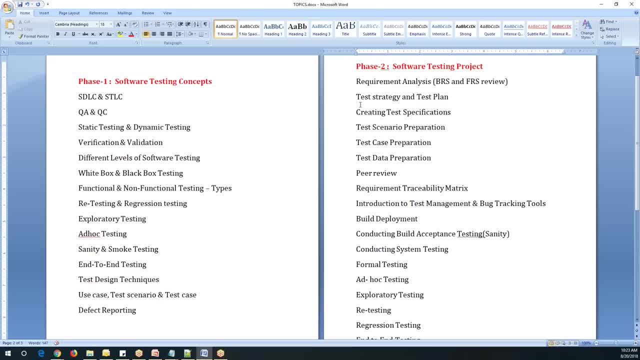 We'll prepare the test cases, will prepare the test scenarios and will execute the test cases, will prepare the test data. so all these kinds of things we do as part of software testing project, and Whatever concept we learn as part of phase 1, the same concept which we are going to implement in project. 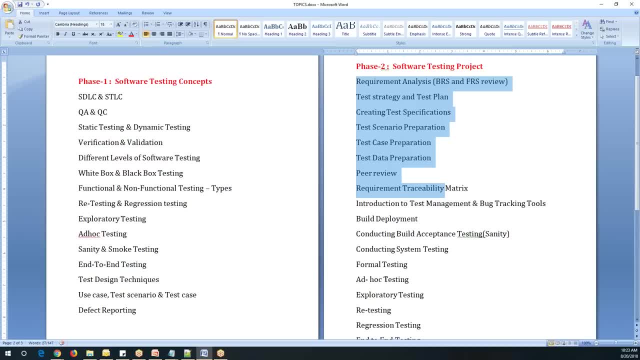 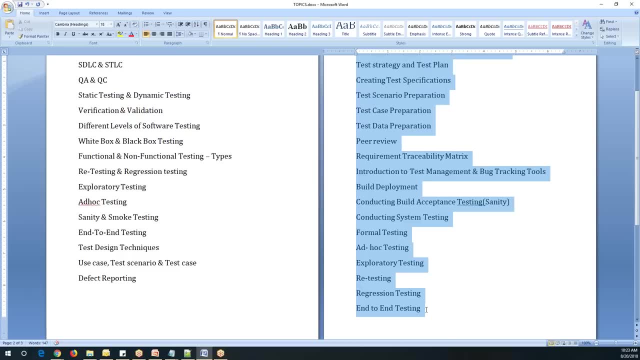 That is phase 2 and there are many more things We are going to learn about phase 2. Okay, and phase 2 itself will take one more week of time, or most of 5- 5 days It will take. this is a second like a phase 2 software testing project. 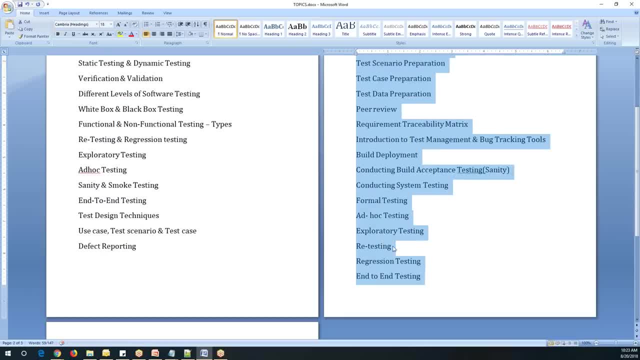 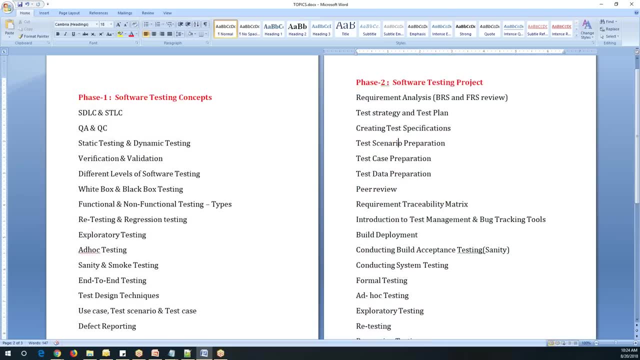 so once we complete this phase 2, you will get the confidence on how we can work on real-time projects. okay, and So here I'm going to show you either e-banking or application or e-commerce or some HRM domain. So there are different type of projects we have. 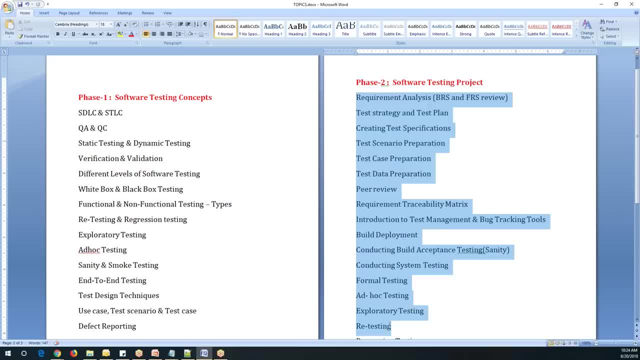 So I'm going to introduce one project and we'll do all kinds of activities on that particular project, Each and every activity we do, just like a real time. OK, I will show you how we can do each and everything And you, side by side, you also will be involved. 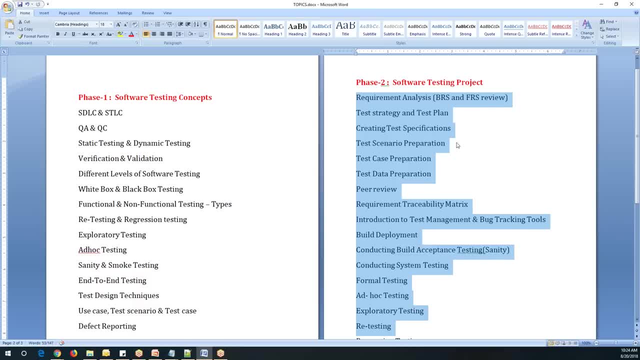 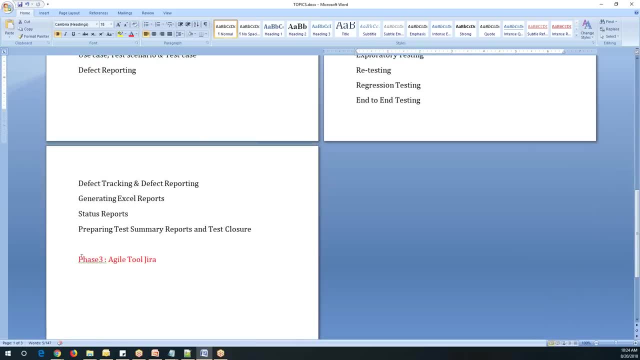 All these actions, are all these activities? OK, there's a phase two, And this is a completely purely practical part. Now, third one is agile tool. The third phase three: we are going to learn a few tools like test management tools. 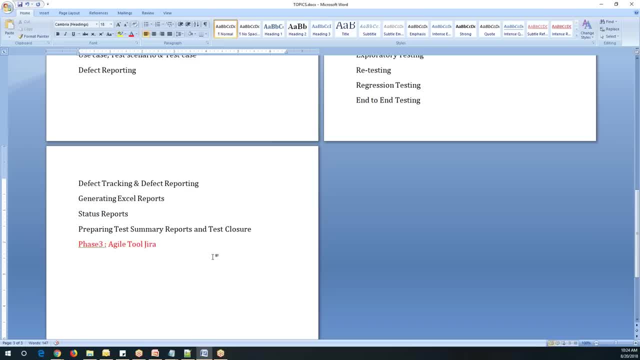 We have bug tracking tools. We have and we also have test management tools and all We have also having agile tools, Right? So all these tools we are going to learn as part of phase three. So this will take Another two to three sessions, not more than that. 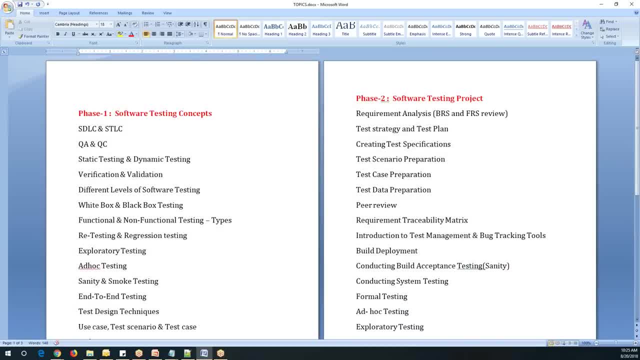 So with this we will complete a manual test. So the overall training is divided into three different phases. Right, So each and every activity is very important, But before directly jumping into the practical session, we need to understand a few basic concepts from software testing. 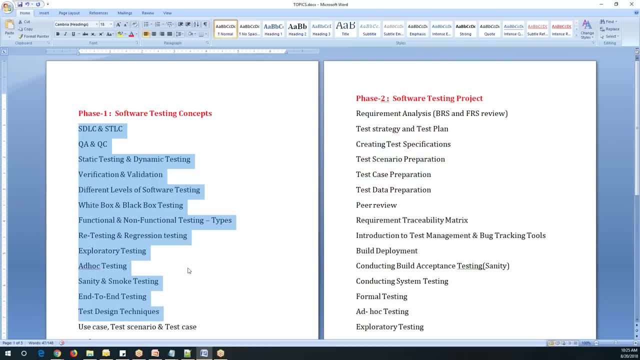 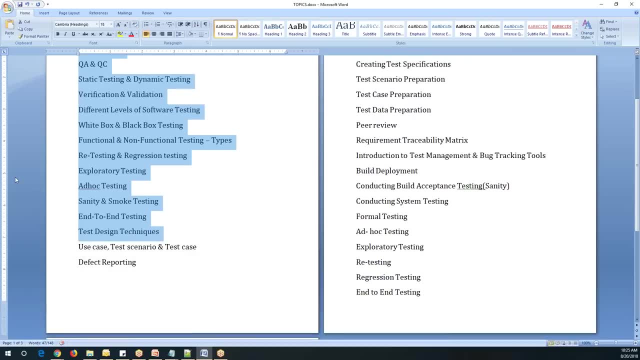 So those concepts we are going to learn in the first week. OK, so are you clear about the curriculum of manual testing? Yes, So please confirm on the chat window, if you're. if I ask something, OK, Fine, So now let's move on. 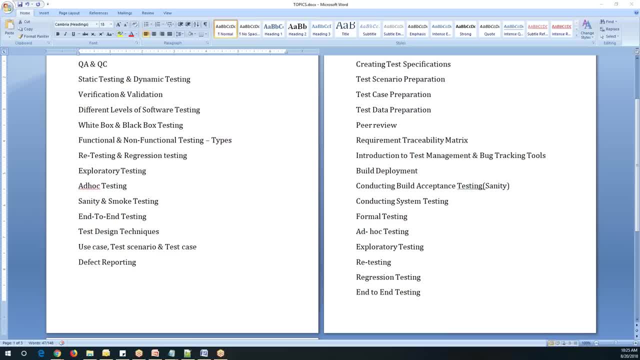 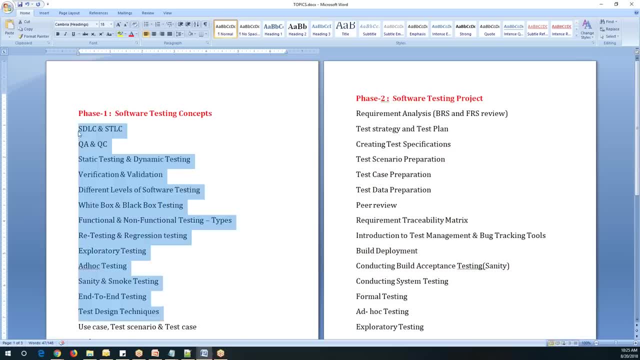 OK, let's move on to the next concept. Let's see. OK, today, as part of today's session, I'm going to discuss about very basic things like SDLC and SDLC and QA and QC. OK, So these are the topics. 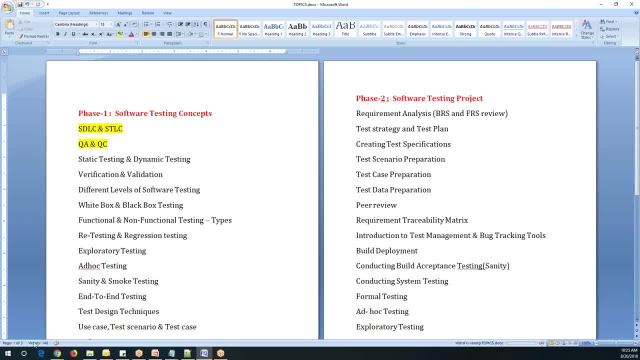 I'm going to discuss today. So let us see. So, in software industry, we need to understand something called what is software, What is software testing, Where the software testing come into the picture, Why do we need to test the software and all these things we need to learn before. 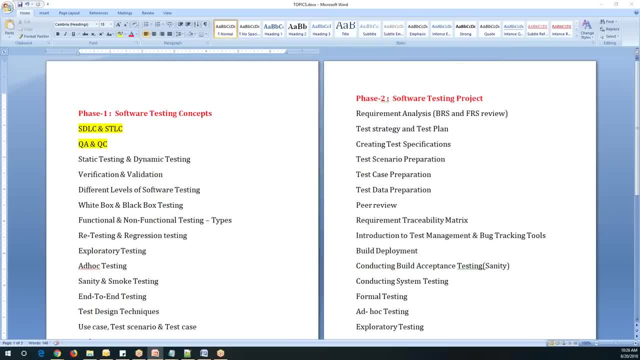 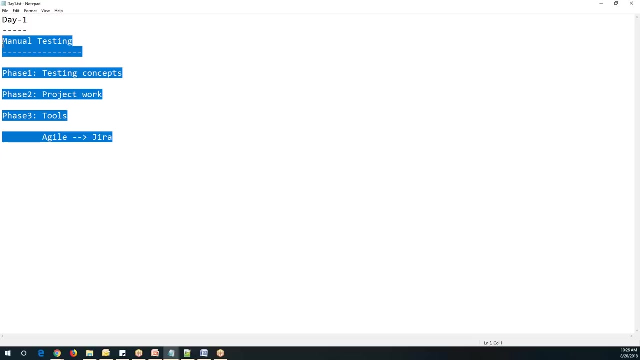 Right. So what I can do is I'll just share a small document here. So let's first understand what is software. Why do we need to test the software? What is QA and QC? all these things we need to understand. so especially software is. so here I will use this notepad as a note sometimes, and sometimes I will present a presentation. I can just show you the PPT. I'll use a multiple to demonstrate different topics. 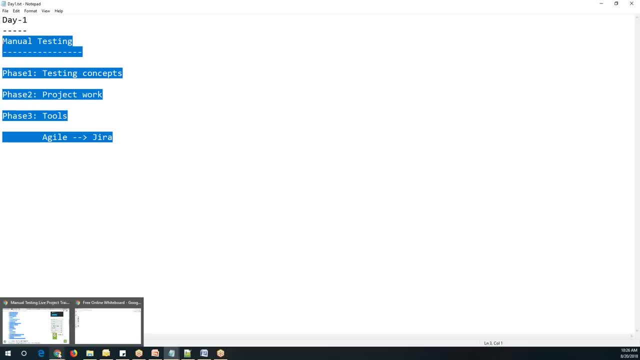 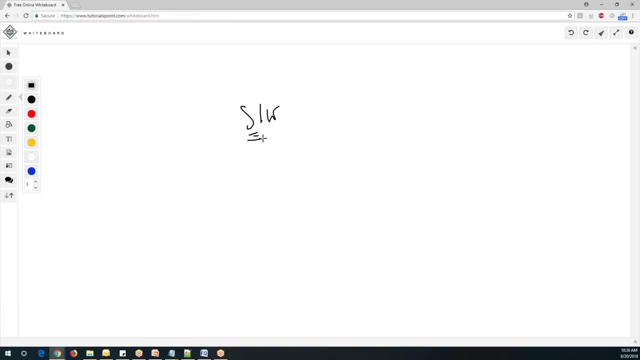 OK, so let's understand what is software and what is software testing. So we are already from IT background. So if you have some IT background you know about. So software is basically a set of programs which will perform certain tasks. right, software is a set of a program or a collection of computer programs. it will perform certain tasks. so this software can be developed by multiple developers or multiple people, based on the customer requirement. 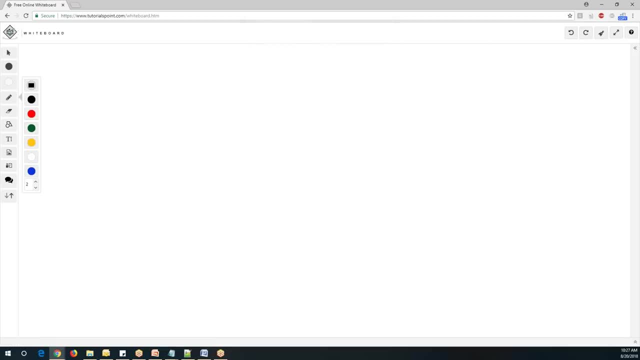 So for whom we develop the software? for the customer. So, for example, let us understand there is a bank, OK, and they are doing A manual transaction in their environment, So they want to automate their system. So what they do is they will approach an IT company and they will ask this IT company to develop the software according to their requirement. 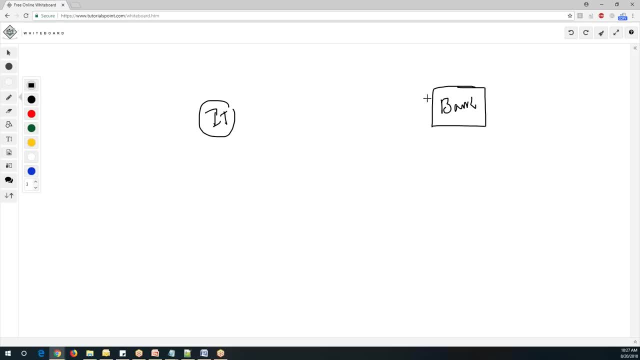 So they will communicate each other. So what the customer? so here the bank is a customer and IT is a vendor. So here the customer will provide all the requirements. So what is the process going on in their environment and what are the transactions they do and everything? whatever required details, they will provide and the vendor or company will analyze those requirements. 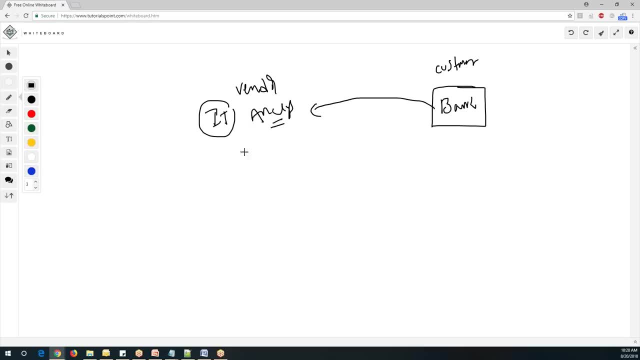 Right. So, based upon their requirements, they will propose some budget, OK, and this much budget will be there and this much time will be taken for this complete to completion of this project and all they will discuss. So first thing is budget and time. 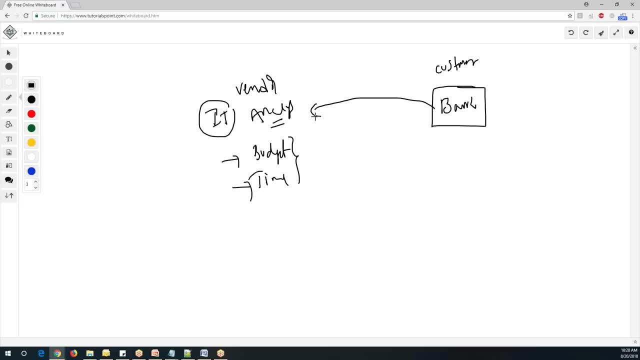 And if the customer is OK with this, then they will do set a proposal or they come to an agreement. OK, so and so budget I will spend and then, within that particular time, I need a software which will perform all kinds of activities in my organization. 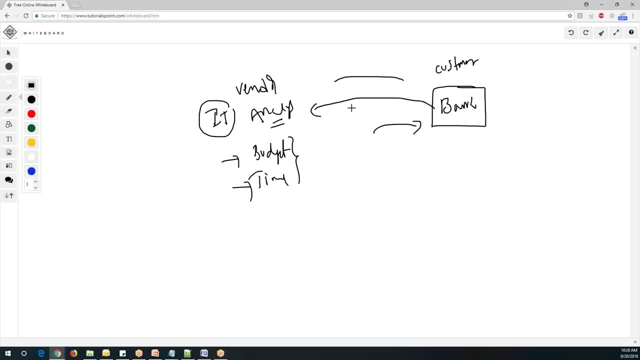 So that kind of proposal they said at the beginning level, this is called as initial, initial level. So once we have agreed then IT company will start developing the project for this project. So once we have agreed then IT company will start developing the project for this project. 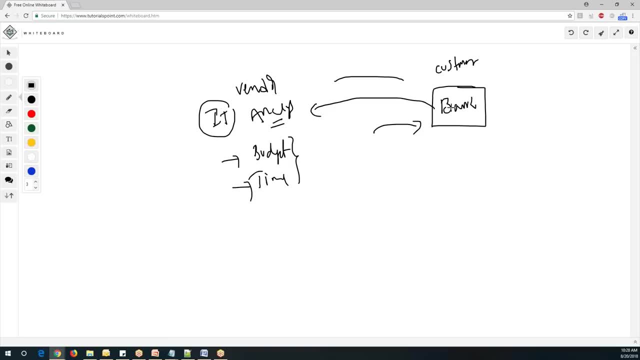 So once we have agreed, then IT company will start developing the project for this project. So once we have agreed, then IT company will start developing the project for this particular customer. OK, so anything. If we want to develop and deliver to the market, we should go through certain process. 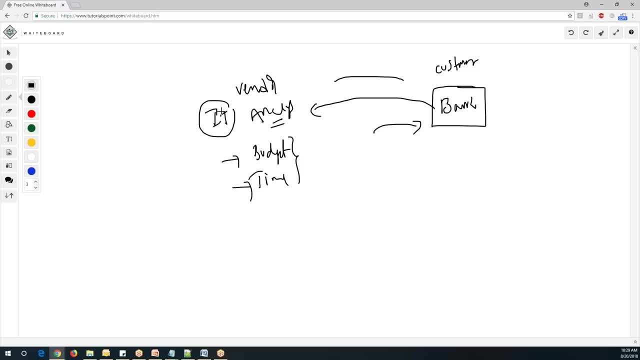 Right Anything if not only IT company. If you go for any other industries, like medical industry or chemical industry or any industry, they will get some raw material or they will do it. It's a process and finally they will deliver something to the market. 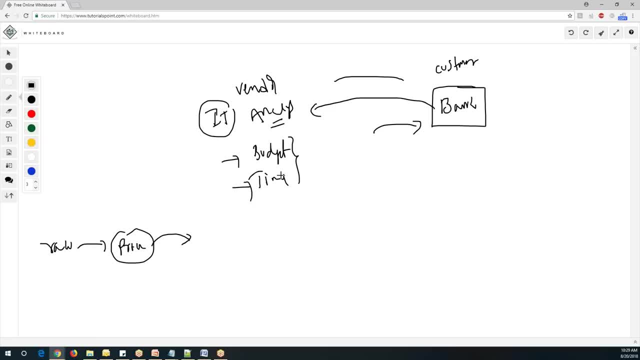 It should go sit and process. I similarly, Software is also will go certain process. There's called HDLC process, software development lifecycle process, the end-to-end process, from where it begins, from where it ends, all The complete step, step-by-step process is called as a HDLC process: software development lifecycle process. 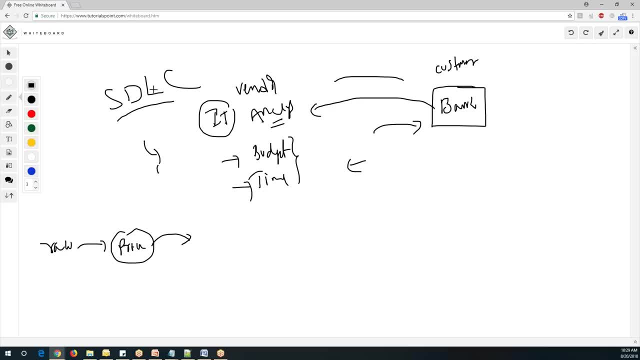 so In this process, in this HDLC process, the software will go through certain stages, like first level, We will understand the customer requirement clearly and then we will design the software and then we'll code the software. Okay means we need to develop the software by using certain programming languages. 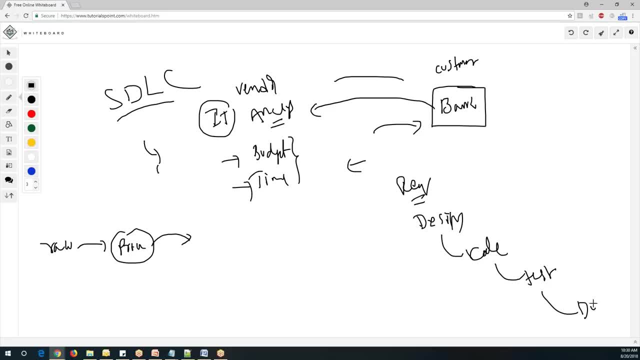 And then we test the software and finally will deploy the software, the customer environment. So software will go through certain stages like requirement, design, Coding, testing and designing, Okay. so here it will start and the final, Finally, customer, will get the outcome. So that's completely called as SDLs: software development lifecycle. 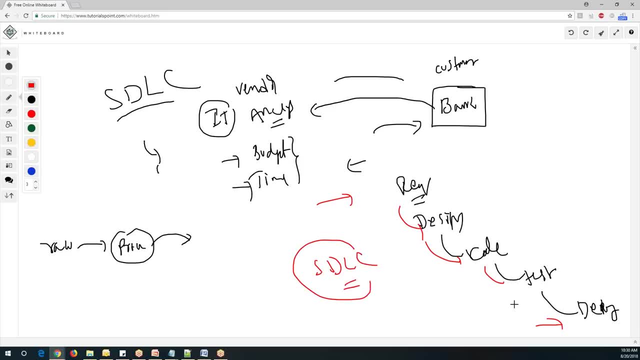 It talks about completes phases, all the phases of software development activities and each and every phase. There are different team involved and different activities They perform, and here the testing is a one of the phase. In entire development process, in complete HDLC process, testing is a one of the phase. This is a main, crucial phase. 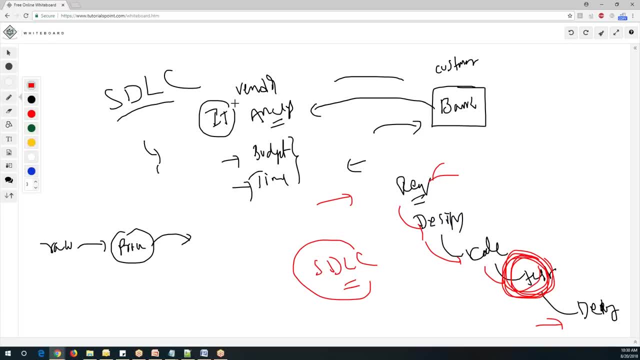 okay, so a software is a collection of programs and if you want to develop a software to the customer we need to go set In process is called as a HDLC process, software development, a lifecycle process. now Let us see Here again. There are two types of softwares We discussed in industry, Normally in IT industry. 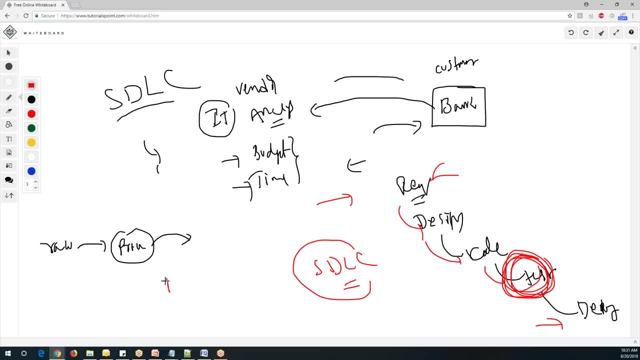 there are only two types of projects. we call them as a. We can call them as a project or product. So because, before entering to the testing of the project, we need to understand all these things: Product and a project. So what is product and what is project? 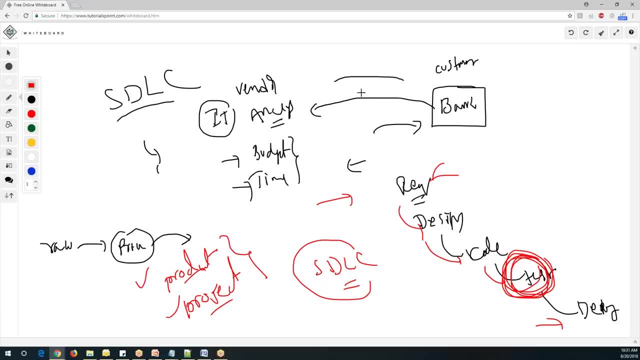 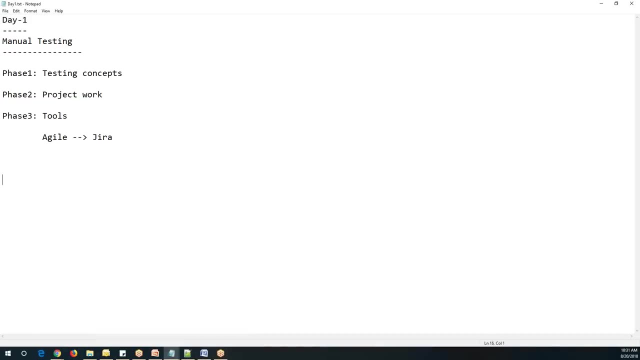 So in IT industry will talk more on this- these two and even companies also. There are two type of companies, like product based companies and service based companies. So I'll tell you what is the differences between these two. Okay, First, let us understand this. Okay, so here, 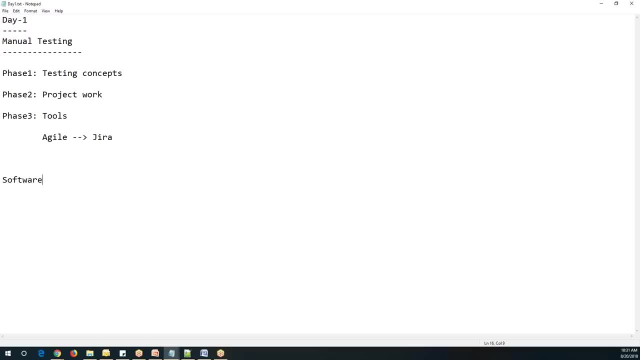 I'm talking about a What is software and HDLC, and now I'm talking about product Versus. the project we'll discuss in detail in the coming session, but here I'm just giving the very high level only. So what is in IT industry if you're entered into the IT industry? 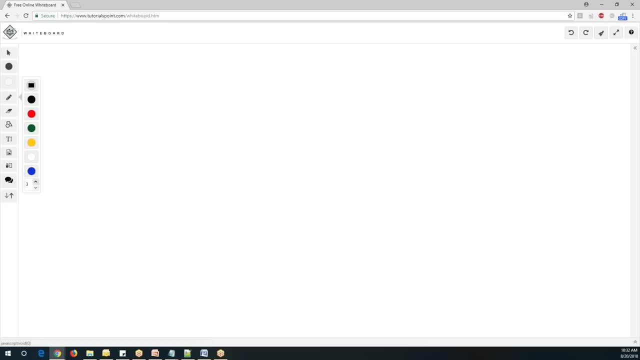 You will hear about two terms: one is project and a product, and similarly, We heard about two different type of companies: IT companies, like service based companies, and product based companies. Now let us understand, or what does it mean? So normally we have a project, Okay, and product. 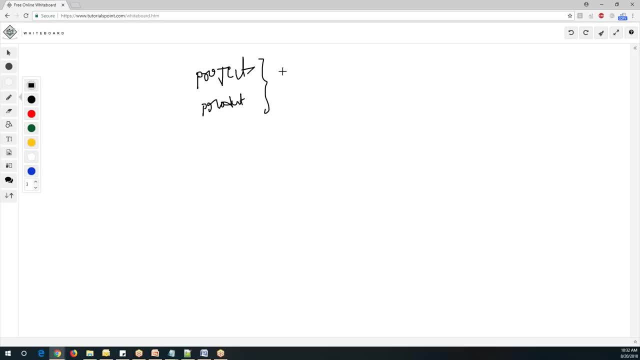 So lumps, we need both our software, something. but we need to understand slight difference. both our software project means we can develop this a specific customer. so, for example, let's say, Achieve a bank and This bank is asking developers of air for the organization. 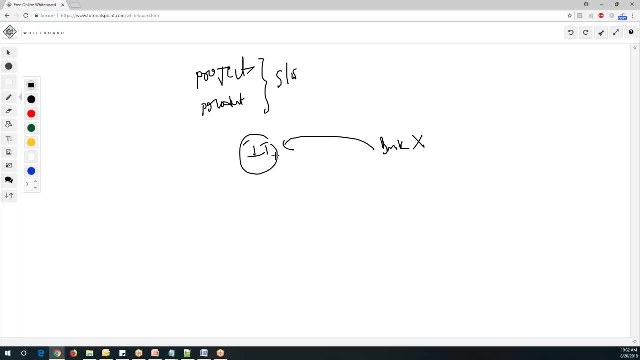 They have requested some IT company, So this company, they have developed the complete software and delivered to this bank X. So this is called as a project. This is called as a project because this is developed Specific to this particular customer, very specific to this customer customer. but this is a project, cannot be used by some other customer. 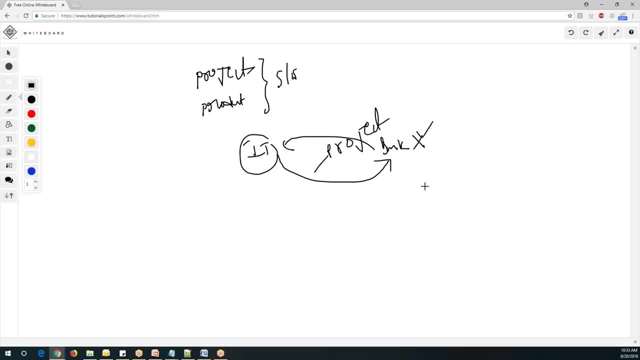 Okay. and if the software is developed for specific customer or specific client, That's called as a project Okay. and sometimes companies will also develop the softwares based on the market requirements, based on the market requirements. So they will analyze the market. So what is the market is? 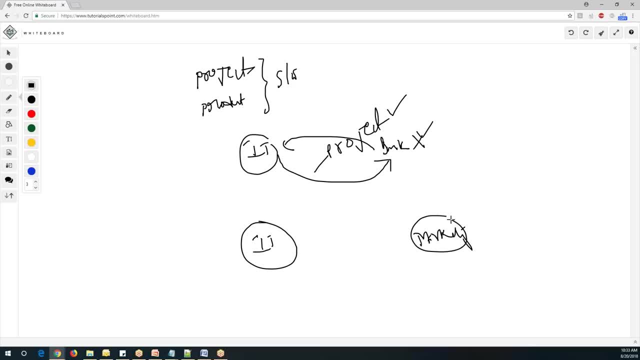 Like what, the kind of software the market like. so what is the requirement of there in the market? They will do certain analysis on the market requirement and they will gather those requirements and then develop a software That's called as a product. That's called as a product. 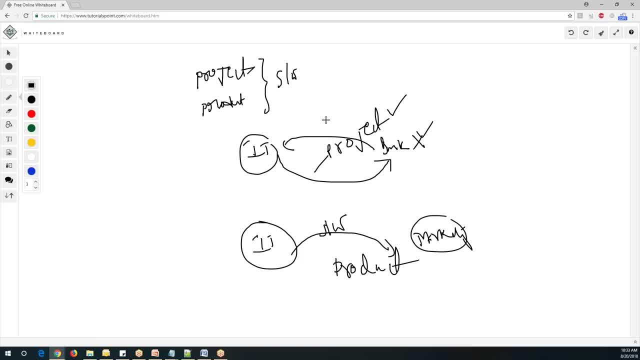 So if we develop a software according to customer requirement or specific to customer is called as a project. And if I develop the software For market requirement- especially for market requirement means multiple users will be there. everyone can be used that particular product. Okay, if you develop a software or based on market requirements, that's called as a product. 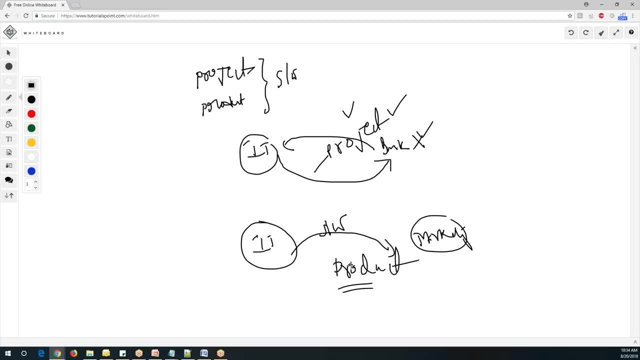 Okay, this is a basic difference between product and product, Project and product. so project will develop a base for specific customer and product can be developed for based on market requirements. here the companies they are Developing, the projects are called, comes under the service based companies like TC is. 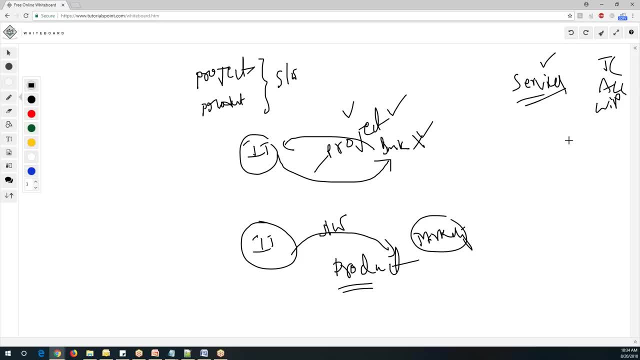 Accenture we pro these are all comes under the service based companies because they were Developing the software for multiple customers. They have n number of claims. these are are service-based companies because they are developing the projects, whereas there are some more companies they will purely product based companies like 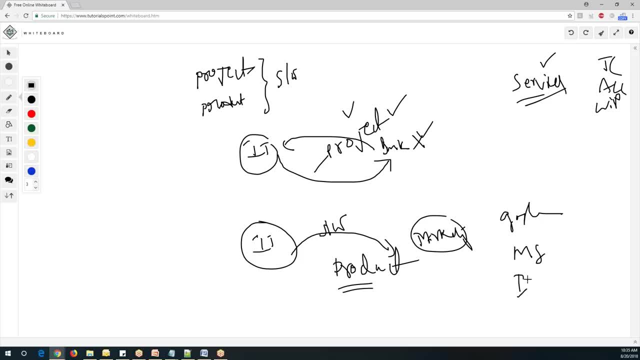 Google, Microsoft, right, IBM, so these are all comes under the product based companies. so they will develop products according to market requirements. so, for example, if I say MS office, like word, Excel, PowerPoint, we will implement at this Microsoft. so this is a one of the product. everybody can use this and 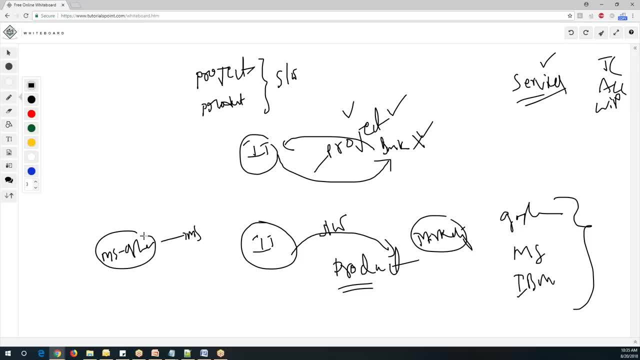 Windows. it is one of the product right. so these are all products based on the market requirements. will get, will develop the software's and everyone make use of it. so that's called as a product. okay, this products is also having. some of them are free or open source and some of them are license based. there are n. 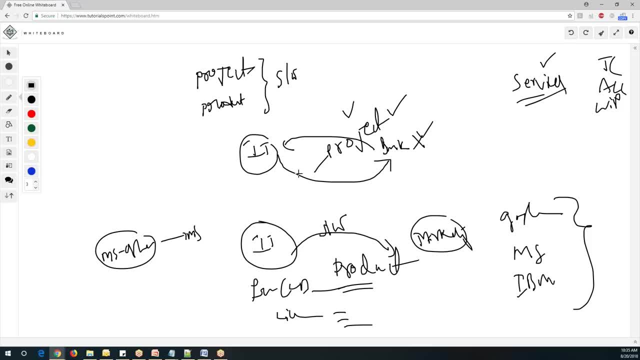 number of products will be there. okay. so in IT industry we can see two type of things like. one is project and product. project is developed for specific customer, whereas product is developed for based on market requirement. very simple, if you understand. this is like a project is nothing but a stitching clothes and 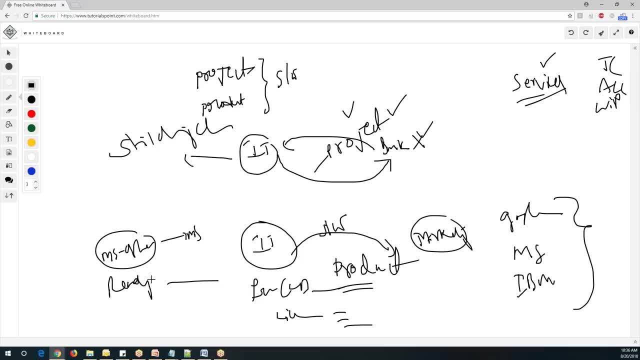 product is nothing but a ready-made clothes. if you understand this one, it is very simple to remember. okay, so project and a product we discussed. so these are the two type of projects we have in the market, and projects will be developed by service based companies and product can be developed by product. 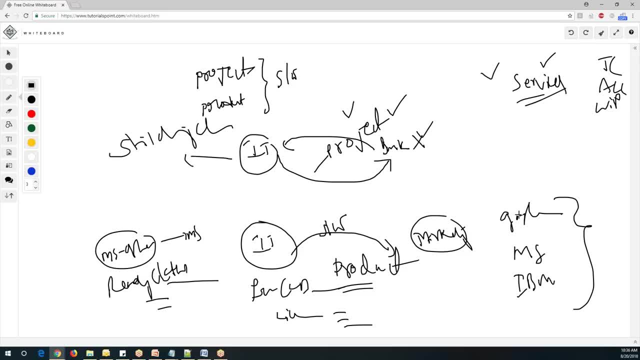 based company, so you can apply that for service based company and product based company jobs. so IT engineers are eligible for all kinds of projects. so now we will discuss about what is testing, why testing is required for this particular software. okay, so far we discussed about what is software, how. 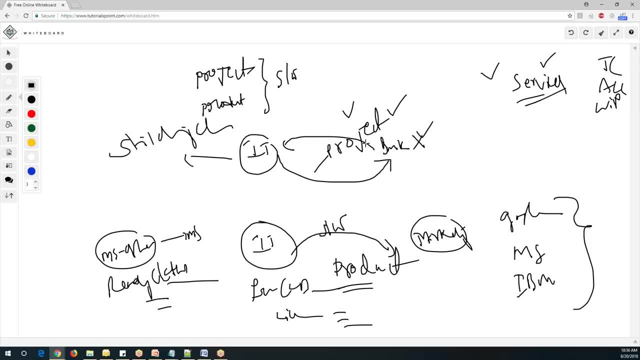 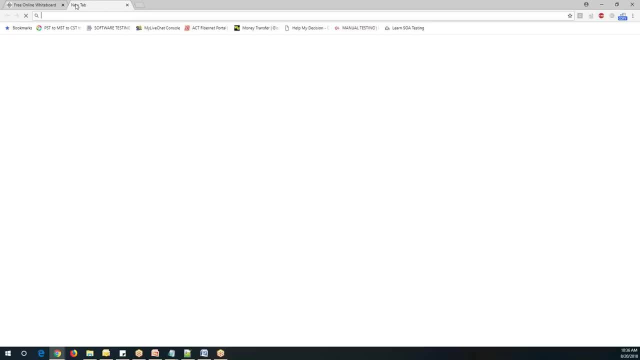 many type of software we have. what is project, what is product? what is service? what is project, what is product? but what is software testing? why do we need to do testing? so I told you in SDLC process. so every software will go through certain process, right? so if we need to start with some more requirement analysis and 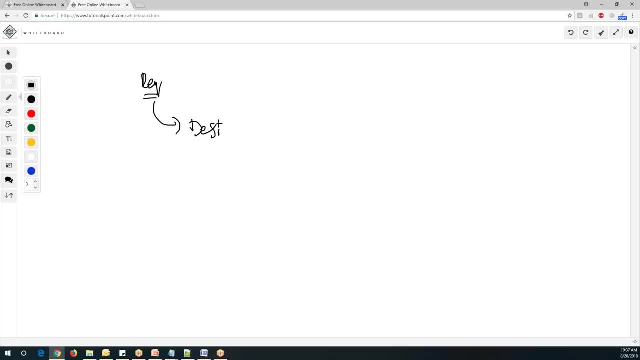 gathering from the customer, then we need to design the software and then we need to develop or coding the software. it means we need to implement the programs and then we need to test the software and then finally, we deploy the software, deployment in the sense we need to hand over the software to the customer. so the 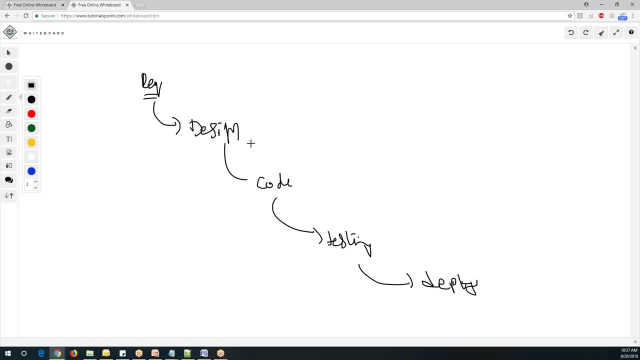 software will go through certain stages. now here, if you observe carefully, testing is a one of the face in entire SDLC process. here we here we call as a HDLC software development lifecycle and this portion is called as a SDLC- software testing lifecycle process. even in testing we need to do lot of. 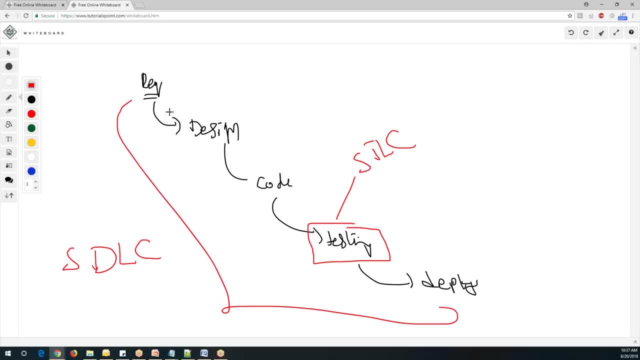 activities. so, like from beginning to end, we do requirement design, coding, testing, deployment, right, this is all comes under the stlc. but inside the test testing phase itself, we do a lot of things, like under stlc. we do test planning and we'll write the test cases. we'll write, we'll execute our test. 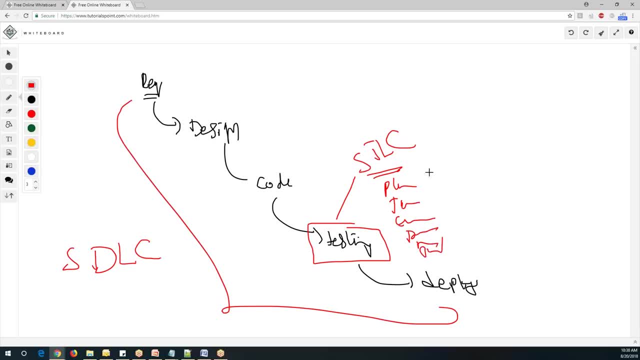 cases we'll find the defects, reporting, test reports- all these things we do as part of testing phase. so these activities all comes under stlc: software testing, life cycle, software testing life cycles. under this we have to do a lot many activities for like test planning, writing test. 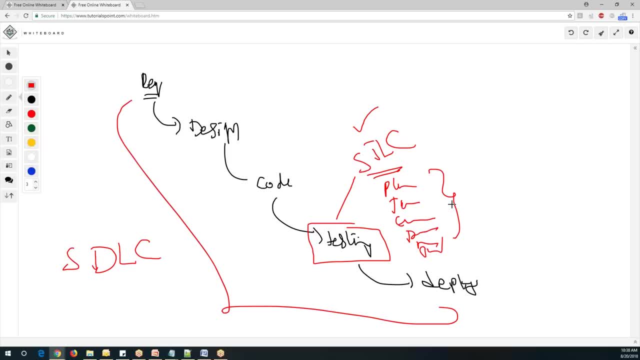 cases: understanding the scenario, writing the test scenarios, executing our test cases, reporting the defects, finding the defects- okay, again retesting the defects, regression testing. all these things we do as part of stlc process software testing life cycle. okay, this is a very crucial phase, but why do we need to do testing on the software? because customer suppose, let's say, a, 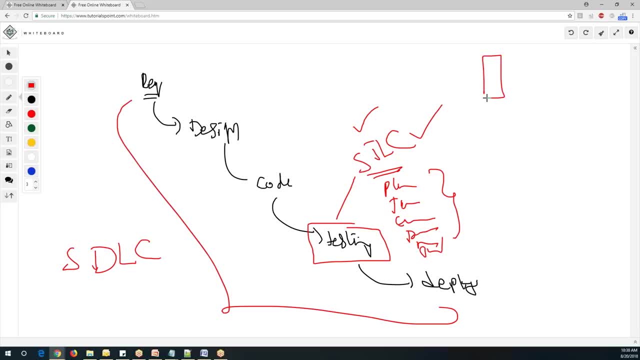 real-time example. for example, i want to purchase a mobile phone, right? so what i will expect: i have certain budget and i i'm expecting some features to be there in my mobile. i have some budget and i want to expect some features to be there in my mobile phone. then what i have done is i have just 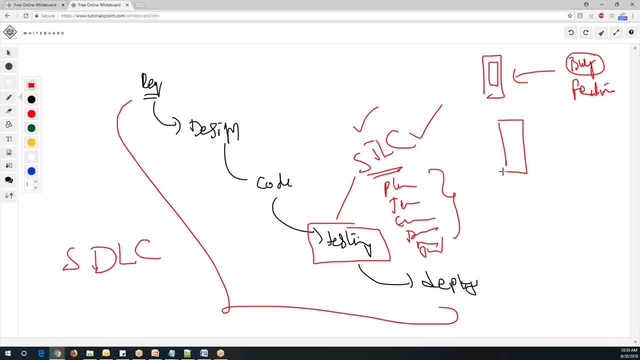 approach a uh the shop, then i have a search for multiple, multiple mobile phones. so which are suitable or which are come in my budget and should have whatever features i have expected. i will just go and search multiple mobile phones and one of them i have purchased. so once i purchased my mobile phone, 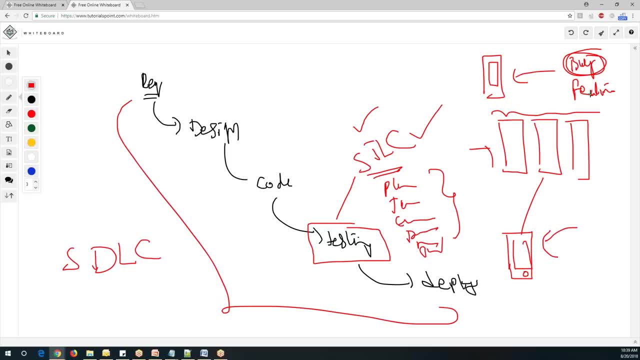 suppose when i start using it. let's say i have some of the features are not working according to my, my expectation. so i spend a lot of money on my mobile phone and i have a lot of features. so i spend a lot of money on my mobile phone and i have a lot of features. 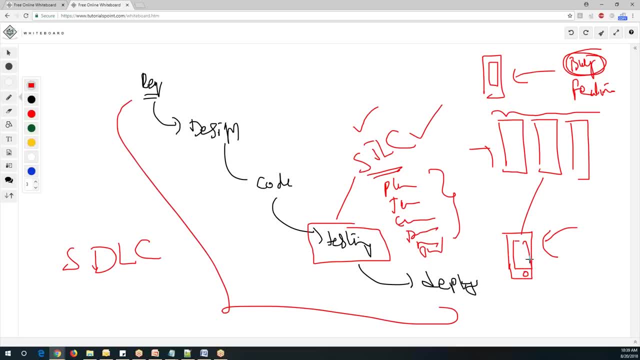 so i spend a lot of money on my mobile phone and i have a lot of features on this. i have expected on this. i have expected on this, i have expected some features to be there and then, once i started, some features to be there. and then, once i started, 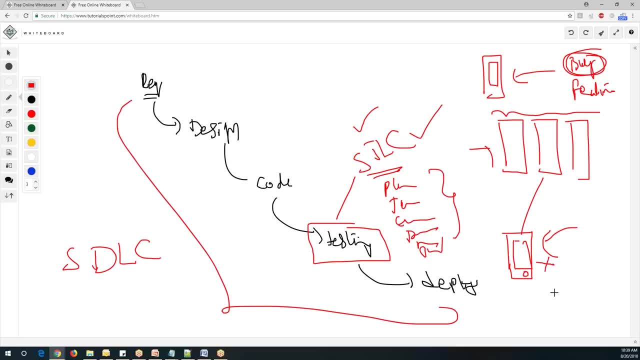 some features to be there and then, once i started using it, certain features are not working here. using it, certain features are not working here using it, certain features are not working here. so, as a customer, i will start frustrating with. so, as a customer, i will start frustrating with. 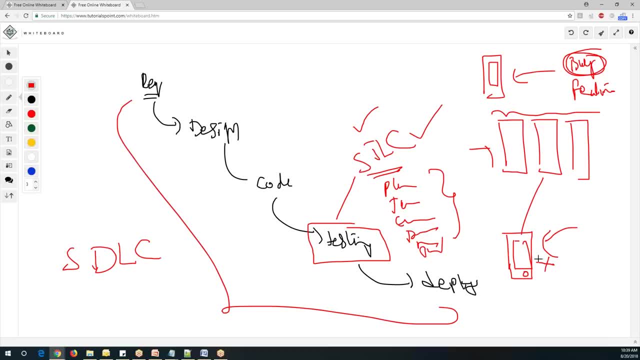 so, as a customer, i will start frustrating with this because i spend a lot of budget, this because i spend a lot of budget, this because i spend a lot of budget- right, so i start frustrating it, right, so i start frustrating it, right so i start frustrating it. so what is the reason for this? is: 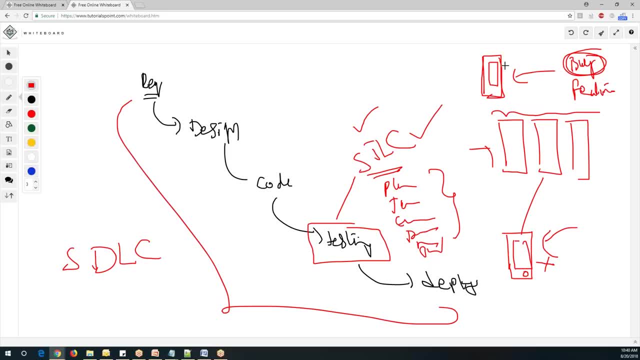 so what is the reason for this? is before, uh, putting this product into the market, they haven't done proper testing right, whether the all features are working properly or not, so that caused this particular issue. later, same thing will happen in the customer also. so when i give the software, when i develop the software for the 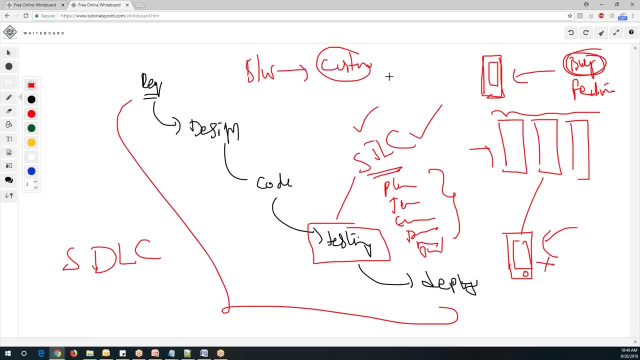 customer. customer will use the software in future, right? suppose he started facing a lot of issues on your software. it is completely buggy product. then he will start frustrating it because they put a lot of time and effort, budget. so many things right. but when i start using it, suppose if you find any defects or bugs or any issues, 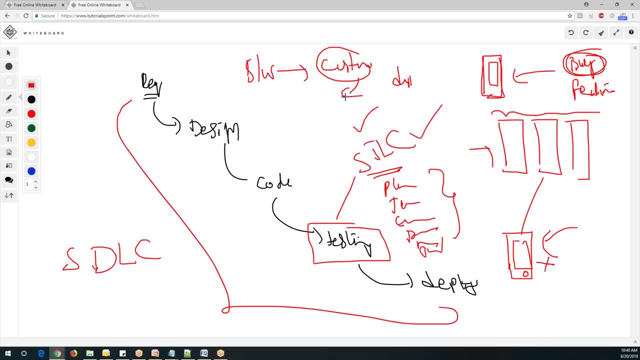 you will start frustrating it, and that is also very sensitive because all customers are like real time, so production environment. suppose, if we take a bank while they are using some banking application, if they get some issues, it will be very complicated thing for them, right? so we need to make sure always we need to deliver the software to the 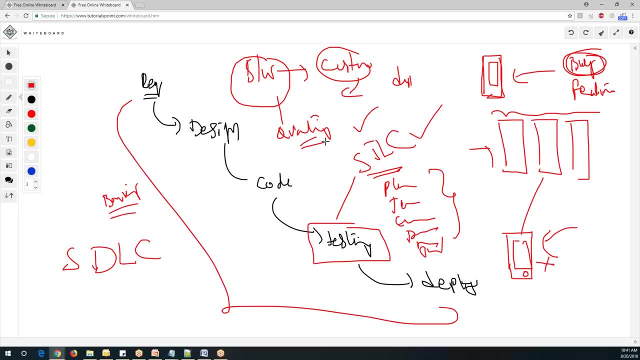 customer very quality product, so we should always deliver the quality product to the customer. so if you want to develop or if you want to deliver a quality product to the customer, we need to perform a testing. so we need to do certain testing on the application or software and then 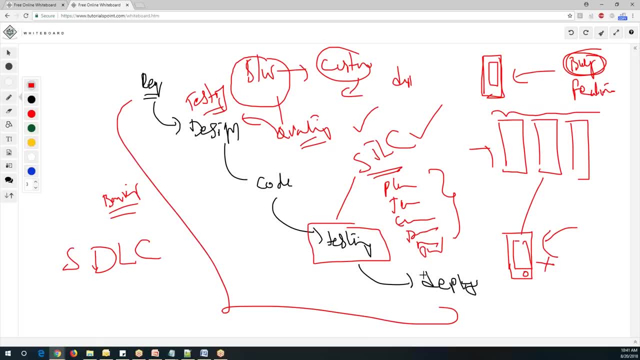 we need to deliver the software to the customer. so before deploying or before delivering to the software to the customer, we need to perform a lot of testings here. there are n number of testings we do so we'll discuss all those things later and testing should be required here. why do we require testing? 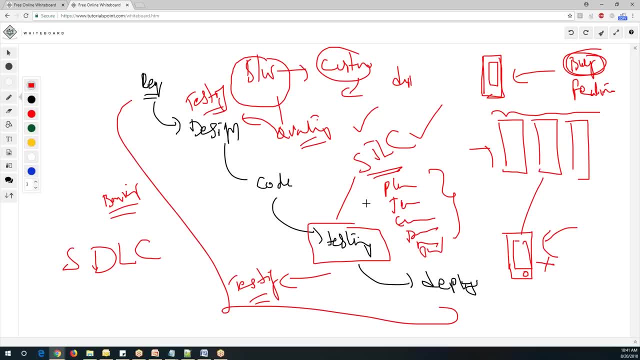 because, finally, we need to deliver quality product to the customer. quality application to the customer- that's the main intention of testing. that is the main objective of testing. the main objective of testing is to deliver the quality product. but what is an activity will do here. we try to find as many as 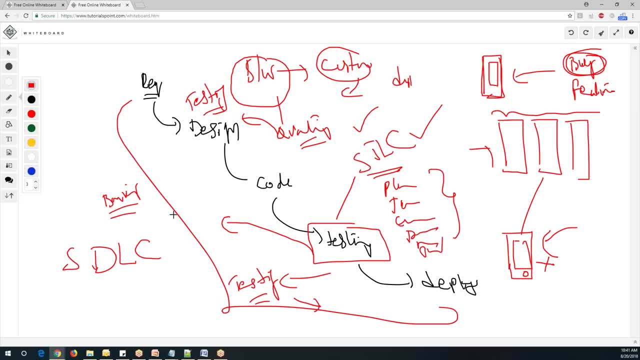 bugs we formed okay. so here we need to find a lot of bugs or defects you can call as a defects or bugs. this is the main important role of the test engineer. so as a tester, the main, my objective is: I need to deliver the quality product to the customer and if you want to deliver the quality project, 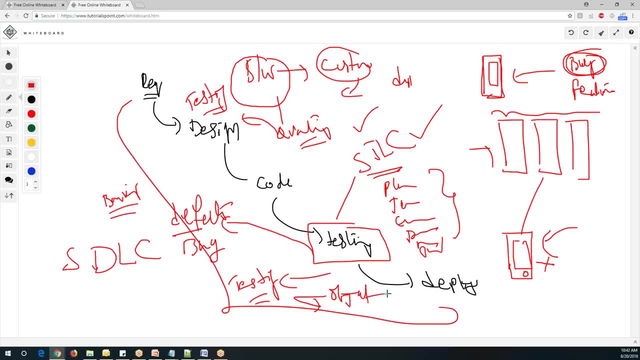 there's a main object of testing. but if you want to deliver the quality product, we need to do certain testing. so we need to find as many as bugs possible and we need to report them to the developer again. developer fix those defects. again we need to test. 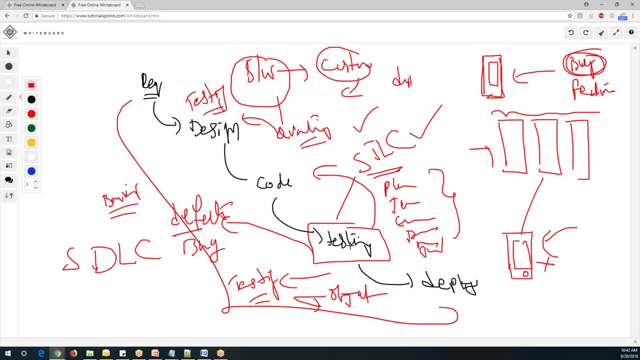 it. so this cycle will go on like this till we get the quality product. okay. so here defect and bug is nothing. but if there is any functionality is not working according to customer requirement or not working as per our expectation, that's called as a defect or a bug. okay, in those cases we will. 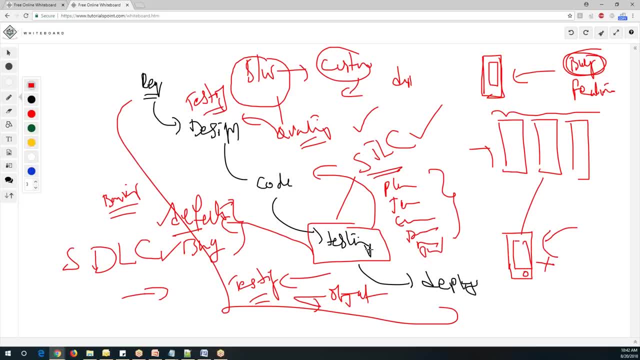 report to the developer. okay, so and so functionality is not working, it's not as expected. so then developer will fix that issue, and again they will provide you one more, one more software, and again we will retest it. so this cycle will go on multiple times and multiple phases, and ultimate goal is we. 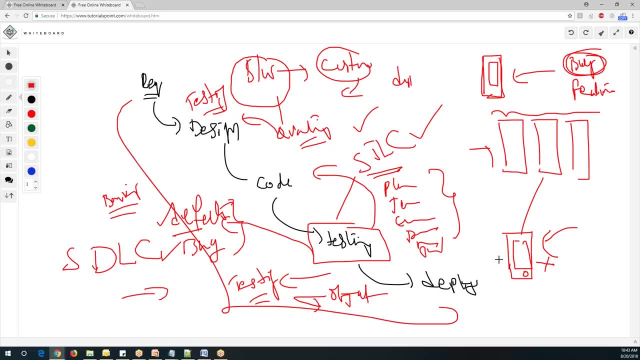 need to deliver the quality product to the customer. that's the main intention of testing. so two things we need to remember: why do we do? but why we need to perform? testing means we need to deliver quality product to the customer. there's a first thing. second thing is: what is an activity we do as? 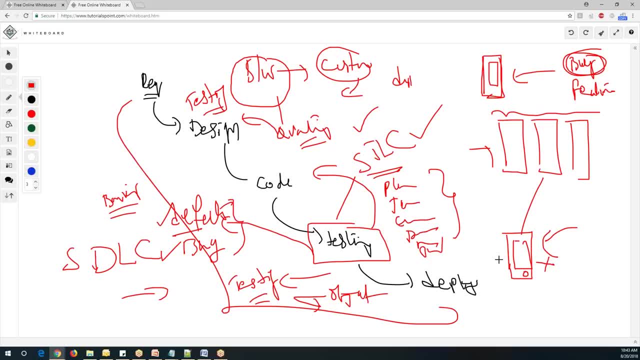 part of testing is we need to find out the defects in the software according to customer requirements. is it working or not- that we need to main focusing on. that's all about the testing. very simple, okay. so testing is an activity to detect and identify the serious acted fault or the sub actions present earlier verses and also. 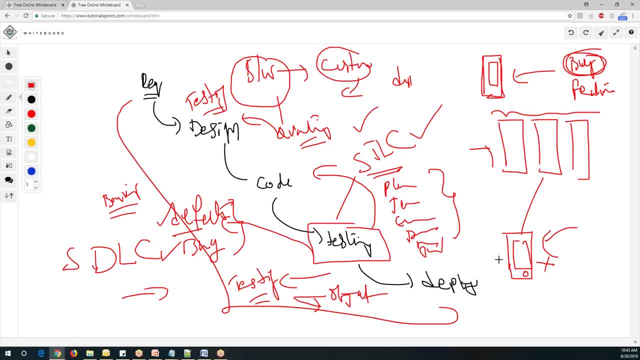 understand the requirements of the tool as well as the use of the device based on the installation present in the software. so several programs is required potentially andpeople defects in the software and the main objective of testing is to deliver the quality product to the customers. quality product to the customer, so that's the main intention of the testing. so sdlc. 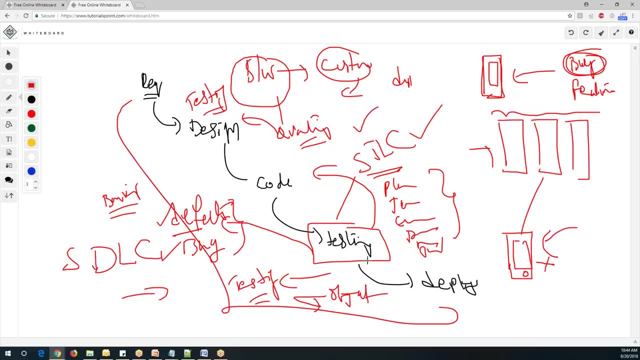 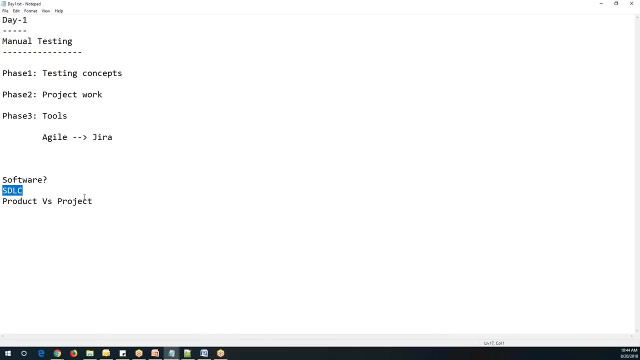 is talking about overall process of software development and testing is talking about stlc, software testing lifecycle process. this is one of the phase in entire software development process. okay, that's a very important thing. okay, so is it clear so far? so we talked about software sdlc. 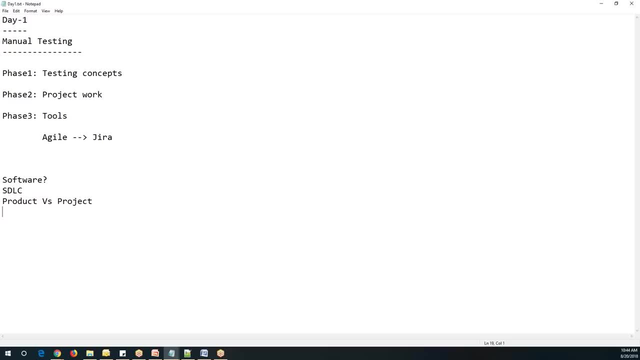 product and project, and then also have a little bit, uh, talked about this one, software testing. what is the testing and why do we require the testing? okay, why testing required, okay, why testing are required. so fine, so here i will just give you very high level understanding of what kind of testing we do. 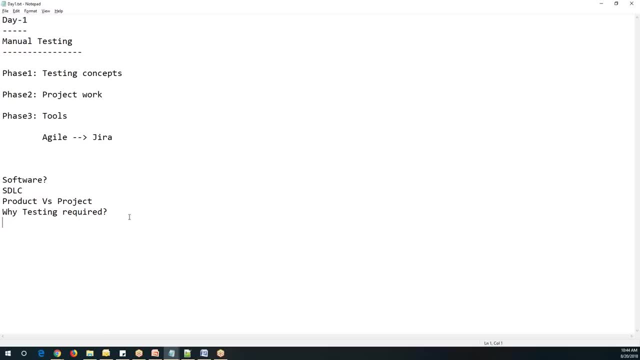 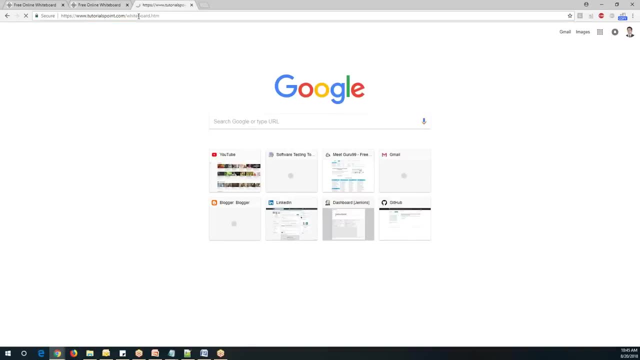 why testers are not don't need to have a programming skills, so let me just give you very high level picture here. okay, so there are different type of testings we need to do as part of sdlc. so, for example, here, uh, in a real-time environment, right, so there are two teams majorly involved in the software. 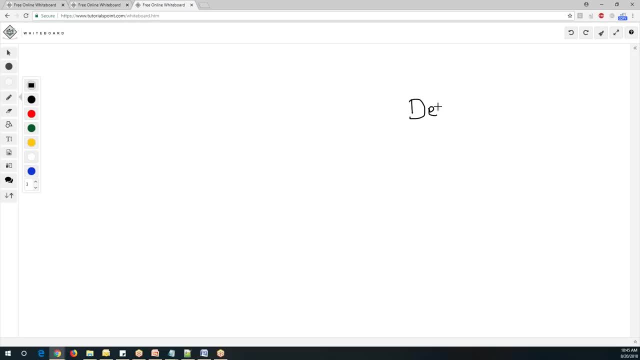 development process. one is developers, or we can call them as a programmers. developers or programmers: these are the people and the other side we have a testers. testers, or we can call them as a qa people- quality assurance people. these are the two teams majorly involved during software development. 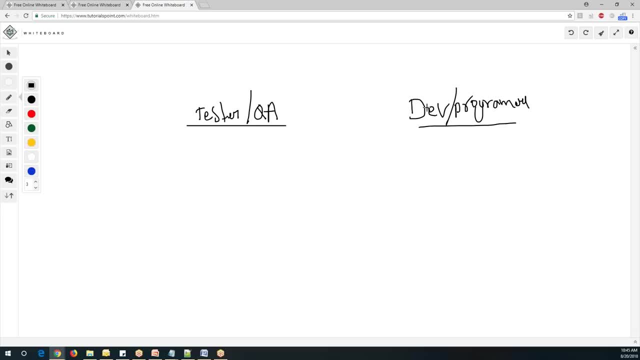 process. okay, so what are the main role of developer and programmer is? they will develop the software, means they will write the different programs. they will write different programs for this requirement from the customer requirement. they will implement number of programs and they don't test this one. so they do certain level of testing but we have to test a lot. so qa or tester team is a different. 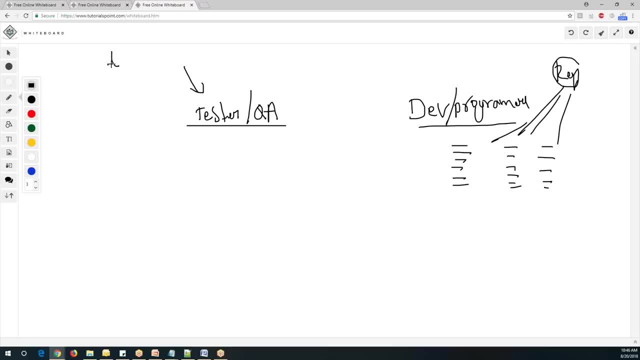 team or separate team, they are completely responsible for testing the software. developer or programmer will develop the software, but testers they test the software. but here, if you understand what is the developer task, they will write a small program and they will also do certain testing here, like whether the program is working or not. they will give some input and they are expecting some. 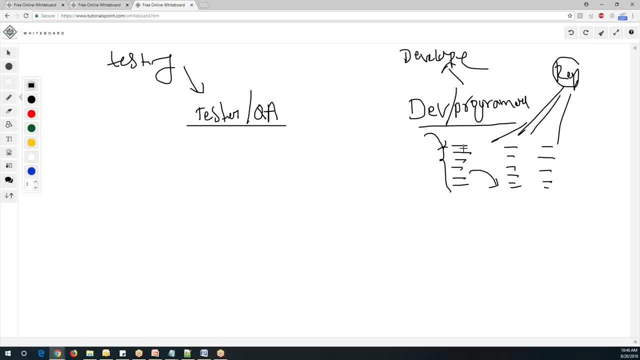 output to be there right. so this is also kind of a testing and what level they do. testing is called as a unit testing. is called as a unit testing means they test their programs but internal logic of the programs, like they will, they will create some kind of a conditional statements and looping. 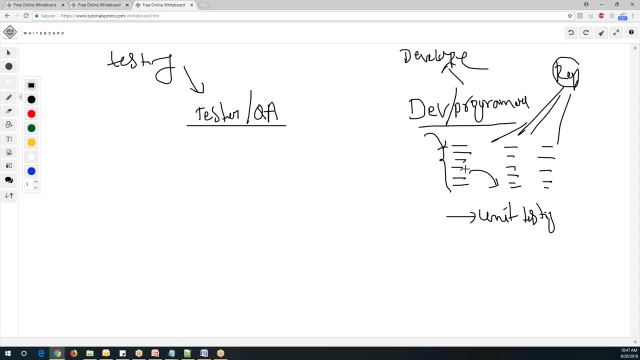 statements and everything right. so they need to make sure all the lines of the code properties are properly executing or not. when i providing different kinds of inputs to this program, are we getting the correct output or not? so they will test internal program, internal logic of the program. 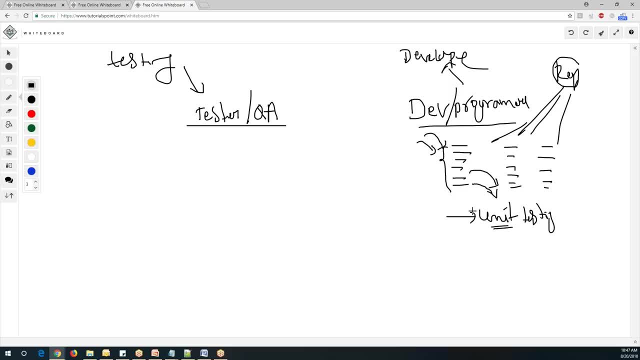 right, that's called as a unit testing and this is basically done by the developers at the developer point of view, because they know the program, how they have written the program, they know himself because they have the developed these programs. now, below this video, i would like to go a little bit deeper into what the facelift platform are. 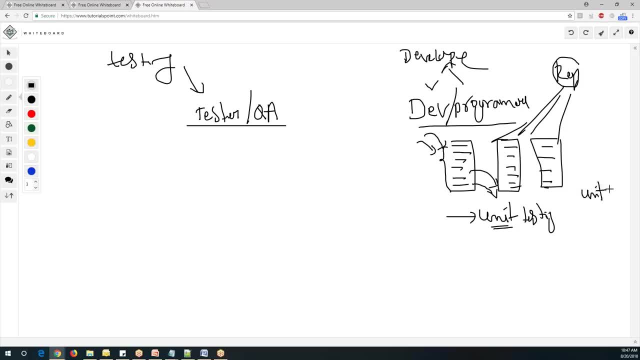 the creation of this program and which variants it represents, like what various community jaket jags. let me give you something very similar. so generally, if you have multiple programs, let's say: this is one program, this is another modular program, this is another component of program. we can say: 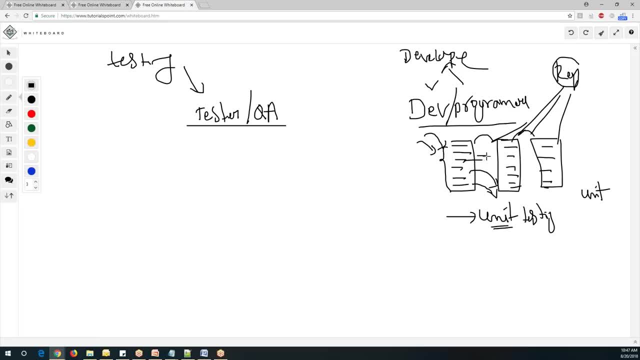 like a unit. unit is a nothing but a single program, or it is a single component, or it can be single module, anything. so sometimes you have multiple programs like this. they have to communicate each other, doesn't it? different works like which one? how do you connect a different computer like this: 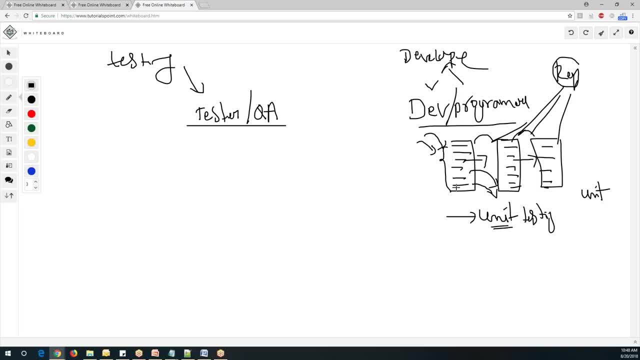 need to test the communication between these modules or these programs. that's called as an integration testing. that's called as an integration testing. so these two testings if you want to conduct, we need to know the programming skill, we need to know the logic, what they have written internally. so that is. 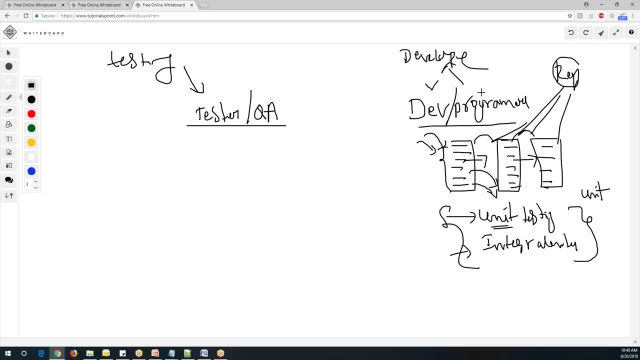 the reason. these two testings are done by the developer itself. okay, in their environment. okay, this is a homosexual level testing, but they don't do the complete testing. they don't do complete software testing. so once they have written this particular code, they will perform unit testing and integration. 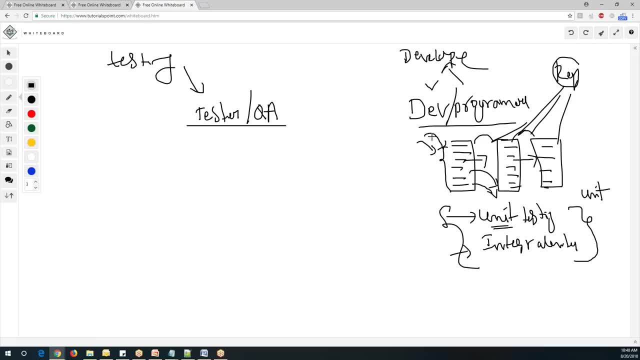 testing. once they have done these two testings, finally, what they do is they will integrate these programs as a build. we call this as a build or package or executable format. so why it is executed format? because we don't see the code. we can't see any code. what they have. 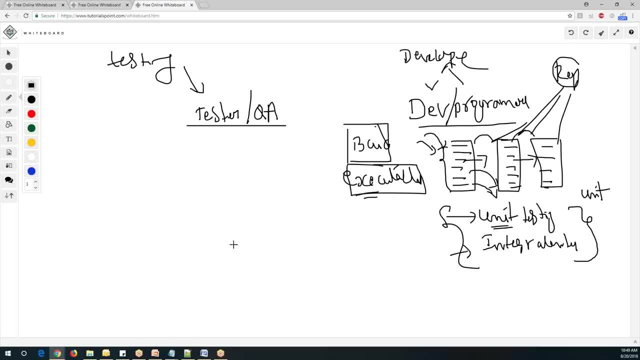 written internally. this just gives one executable file so that we can deploy and install in your QA environment, just like softwares. suppose. if you want to install any software, we download them right and we'll install it. but can we see the code? what they have written internally, we can't right. similarly, 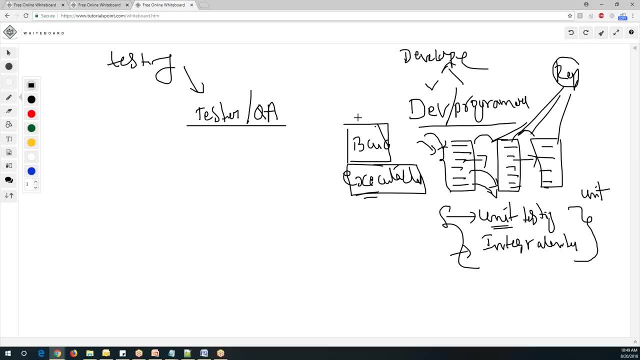 developer don't provide their programs to test, so they will provide the executable files in the form of bills and then we will deploy or install that building QA environment or a testing environment and then we do testing. but here what kind of testing we do already unit testing, integration testing is done. 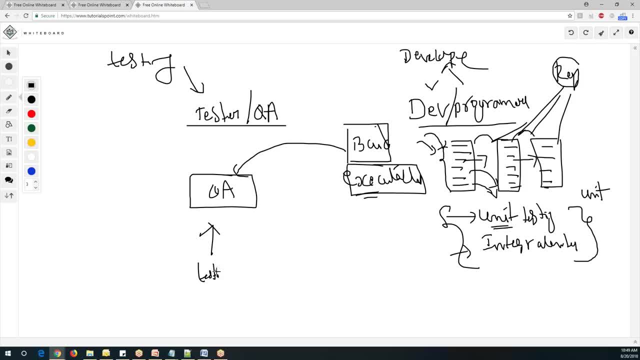 by the developer, but here we also do a testing, but this testing is completely done by the testers, not the developers. complete testers are responsible for performing this testing. so this is called as a system testing. you here we call as a system. system is the complete software, the complete end-to-end. 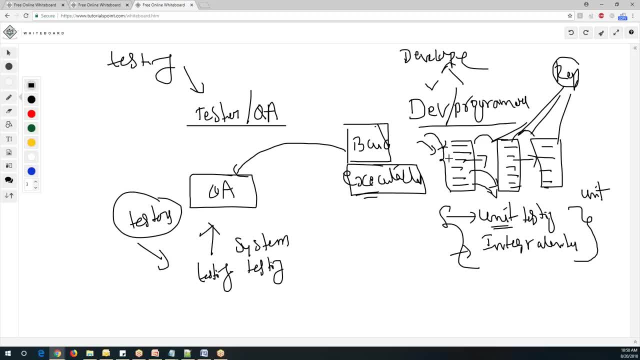 testing we have to perform. but here what is an input? here developer is written the programs, because they know internal logic. they are able to test it in the form of unit testing and integration testing. but when you come to this testing system testing phase, how the testers will know the functionality of? 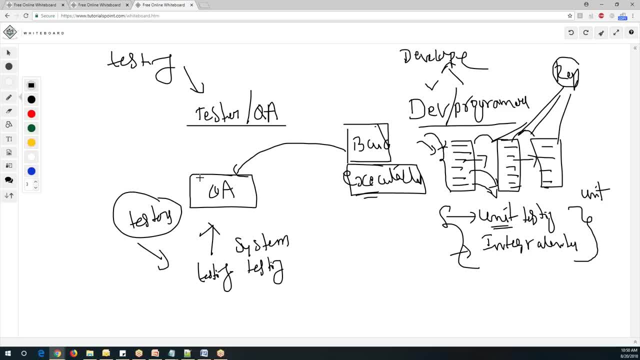 application. so, before getting the build from the developers, the tester has to do certain job. so set an amount of time for the testers to do certain job. so set an amount of work they have to do. what the task they will do is, before getting the builds from the developers, they will also understand the requirements from the 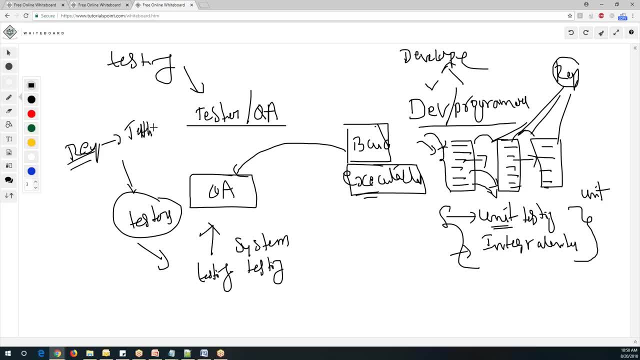 customer and they will prepare some test plans and they will have some test cases, test cases. so all these things they have to complete and get ready and test the build. okay, so, before getting the build from the development team, they- testers- will do these activities. they will understand the customer requirement. 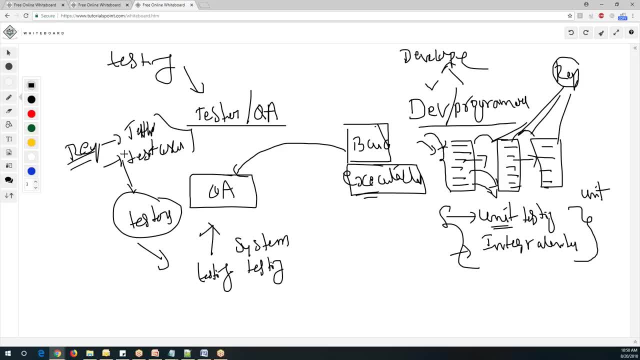 and use case, then they will create some test plans and then create the test case. test case is some in the nothing, but it's step by step steps which will execute on the application- those called a test case. so we'll discuss more on this in the coming sessions. a test case is just for now, understand. 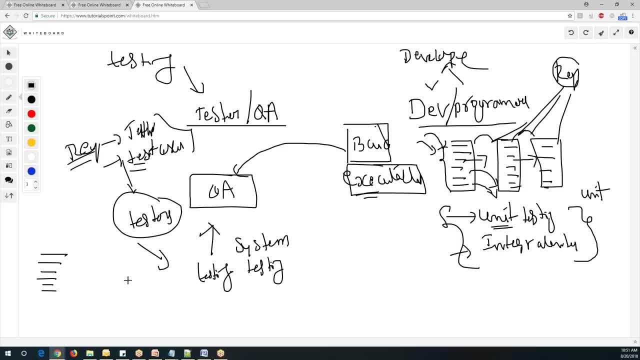 step by step actions which we need to perform on the application. so, for example, if i want to test me login screen, so what is the test case will be: step one, what we need to do- open application, okay. and step two is enter username. and step three is enter password. step four is click on. 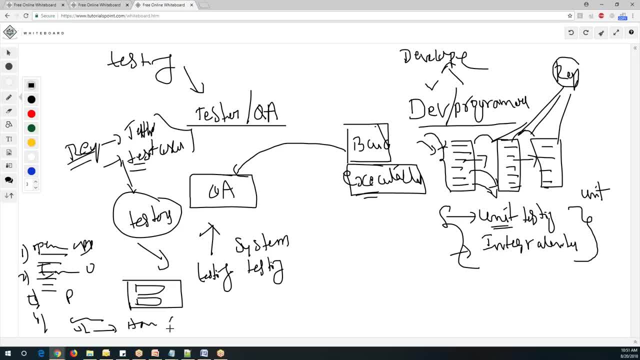 the submit. step five is it should go to home page. that's our expected right. so this itself is called a test case. so test case contains the actions which we need to perform and corresponding result, what we are expecting result. so these things will be there in the test case. so once we get, 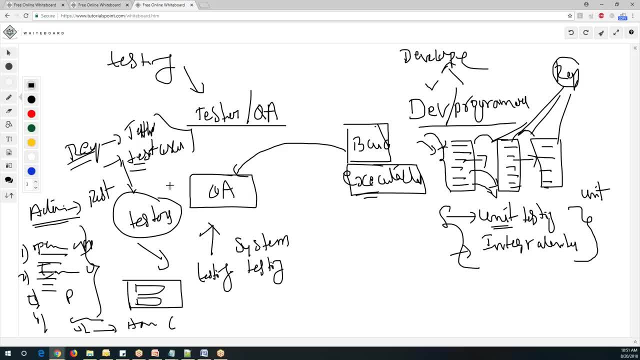 understand these requirements, we can create test cases. and if you're ready with the test cases, then we can easily test our software, which is provided by the developers. this is the main role of the testers. day-to-day role of the testers: he has to understand the requirement. he 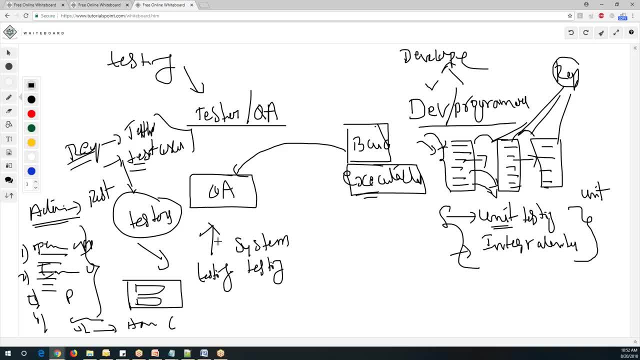 will create the test plans and test cases and once the bill is ready then he will execute the test cases against the bill. if you found any defects, he will report to the developer. okay, again, developer, fix that issue. again. they will create one more executable file again, one more build again will. 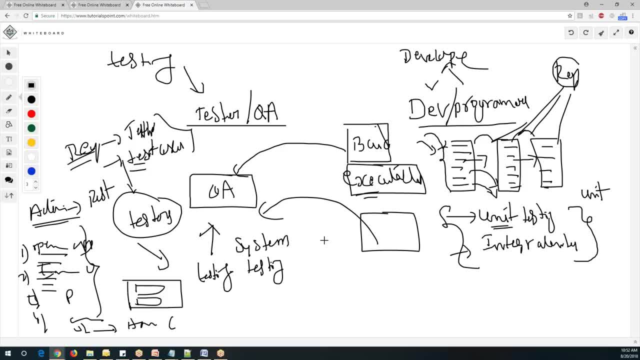 give you, the testing and testing team will again retest the same thing. so this cycle will go on like this till end of the cycle. okay, so here i talked about different type of testing. unit testing and integration testing is done by the developers at the program level, whereas system testing is done by the tester. 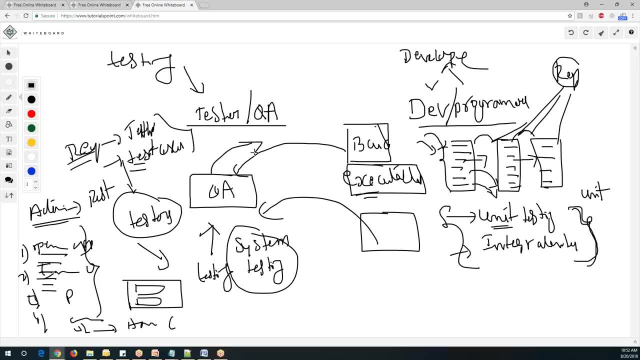 whether this application is working according to customer requirement or not. that's the main intention of system testing. so here we don't know the code, what developer is written, but we should know the functionality, how the application is working, how the screens are flowing, each and every operation or transaction. is it working according? 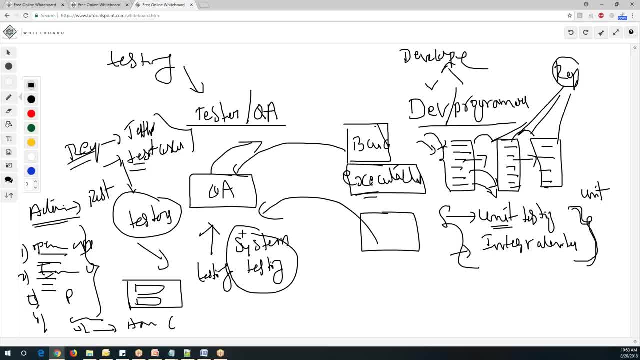 customer requirement or not, so that we need to verify. that's called as a system testing. system testing means we don't test internal logic of the program, but we need to test the software according to customer requirement. according to customer requirement. so that's the reason this is called a system testing. 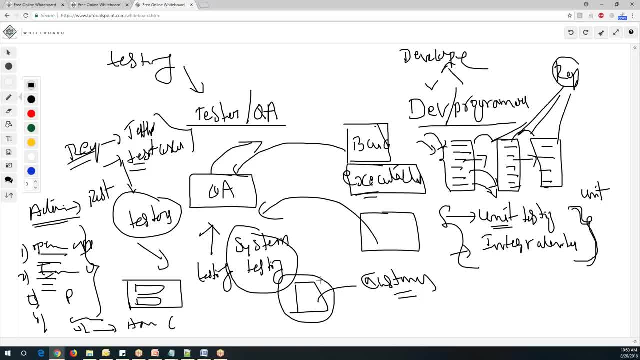 but if we want to do this kind of testing, we don't need to know about the programming skill here, because we are not dealing with any program here. we are just testing the software whether it is working according to customer requirement or not. but the main important here- the task is here- is: 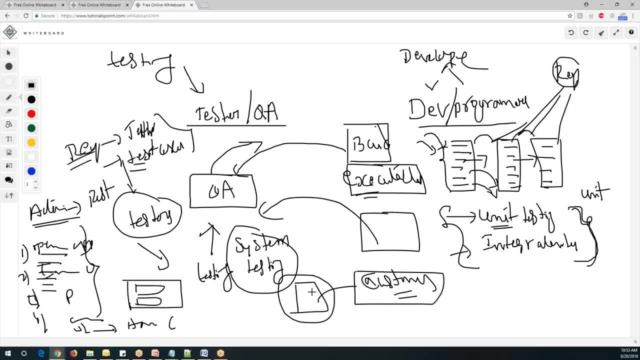 understanding the requirement, so that again, the testing quality is depends on how well you have understand the requirements from the customer. that's the main important task, okay, so understanding the customer requirement and functional flows in the application is very, very important, and then we can jump into the testing, the software. so that's how it will go on. so unit testing and 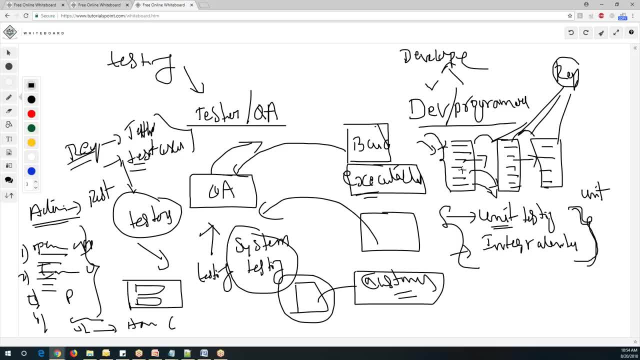 integration testing done by the developers, and they do testing internal logic of the program so that we call them as a white box testing techniques. these two comes under the white box testing because they know what they have written internally right when you come to the system testing here we don't. 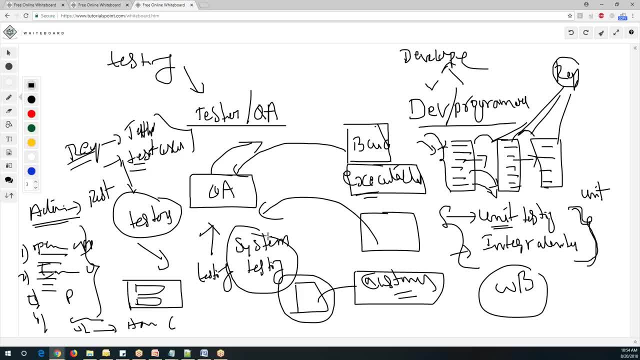 know what it is there internally, but still we are testing the software according to customer requirement. so it is called as a black box testing technique. black box means internally we don't know what it is there, completely black. but here white box means we can see what internally they have. 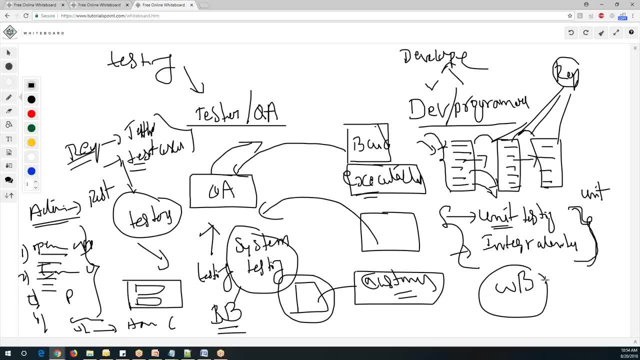 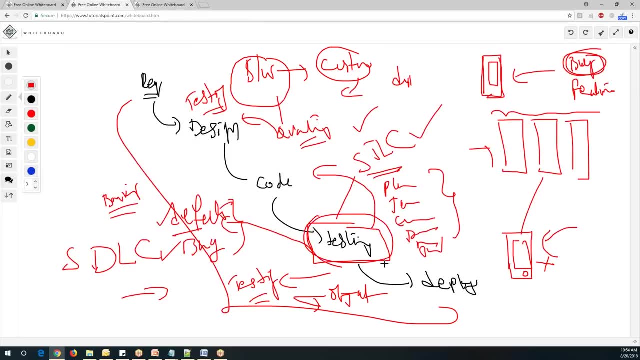 written. so that's a unit testing and integration testing comes under white box testing and system testing comes under the black box testing. all the testing team or test engineers all comes under system testing phase. all our comes under testing testing phase. so this is a phase we are ignoring. 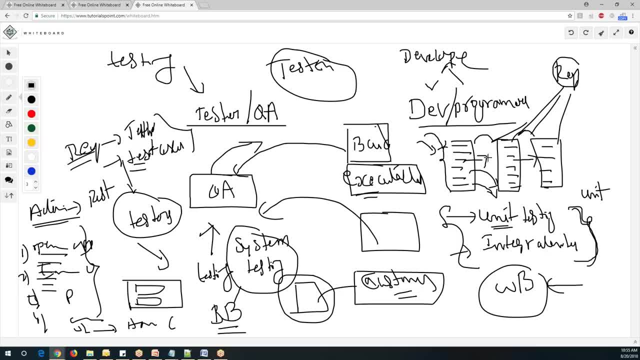 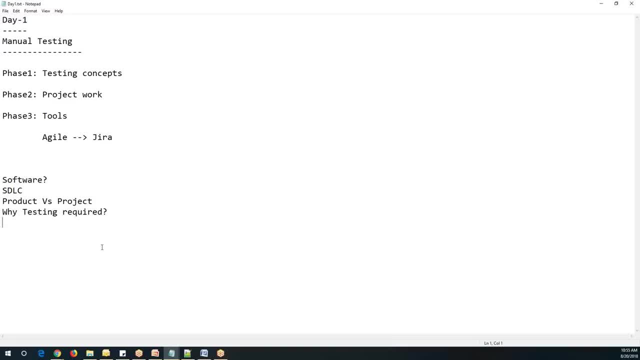 and rest of the testing- unit testing, integration testing- is done by the developers himself. okay, so this is all about different type of testings. i just talked about unit testing and integration testing, and then system testing and we have one more testing called as a uit testing user. 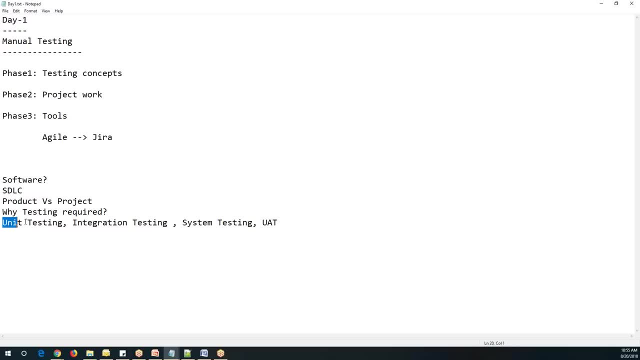 acceptance testing: okay and uh- yeah. so unit testing and integration testing comes under white box and system testing, uat testing- comes under the black box. so these two comes under white box testing and uh and other one, system testing and ut testing, comes under the black box testing technique. so what is uat testing means, once we have done our testing team is completed day testing. 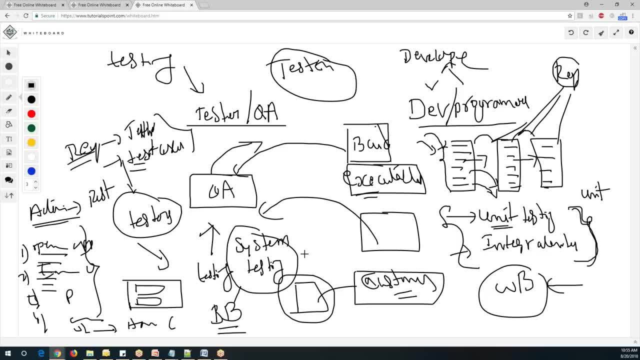 will hand over this project or they will hand over the software to the customer. so customer directly. don't use that in production system live. okay, they do also certain kind of testing because they just ask they have provided the requirements, so once they get it they should know right. 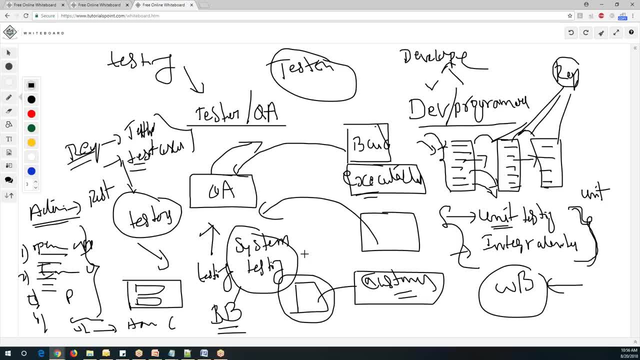 how they are working. they should get familiar with that application first. they should get familiar with the software. they have to learn how to use it. so they will take certain time, certain amount of time, and they will execute their own test cases. they use cases on the software. that's called uat testing, suppose, sometimes in uat phase also. 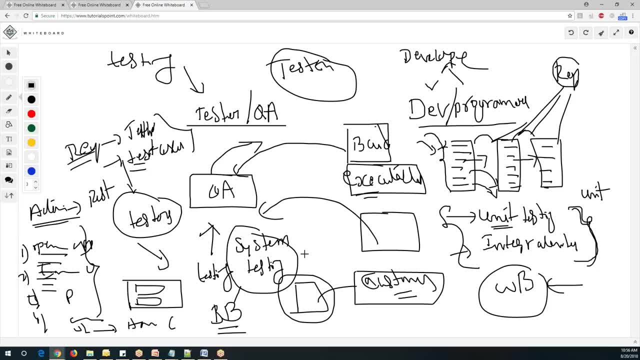 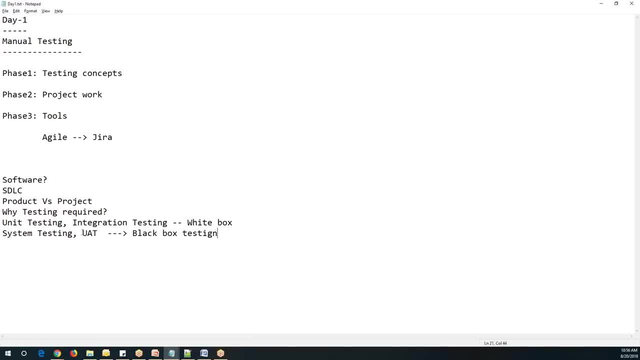 they can identify some defects. so those defects also we can should able to find out. that's called as a uat testing, user acceptance testing. once the uat is successful, then only customer deploy the software in the production environment, in the live environment until, unless they don't directly. 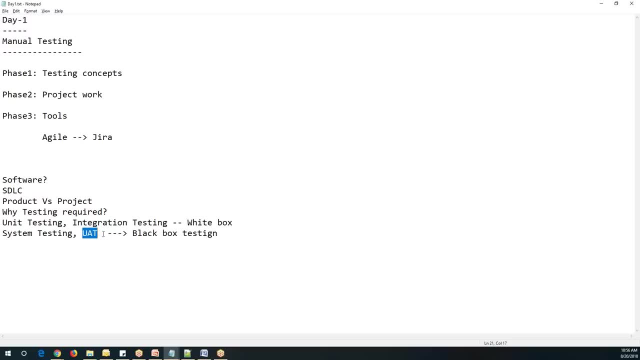 proceed with the live environment. okay, first they will do certain analysis, they do certain functionality, is it? they will execute their use cases on the software and then they will move that into production environment. that is called as a uat- user acceptance testing- which is almost done by. 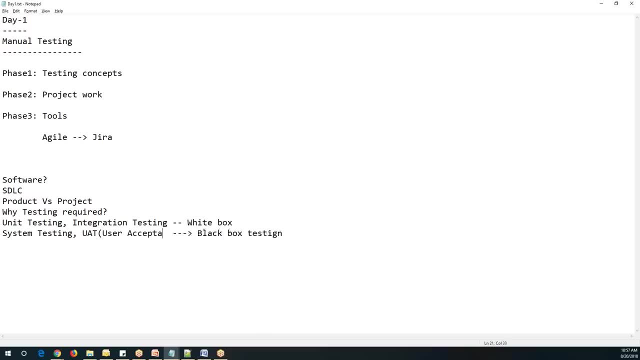 the customers or users: user acceptance, user acceptance test, user acceptance testing. okay, so these are the different type of testings. we do unit testing, integration testing- purely it is white box testing done by the developers, and system testing is a main important phase where all the testing team will be involved manual. 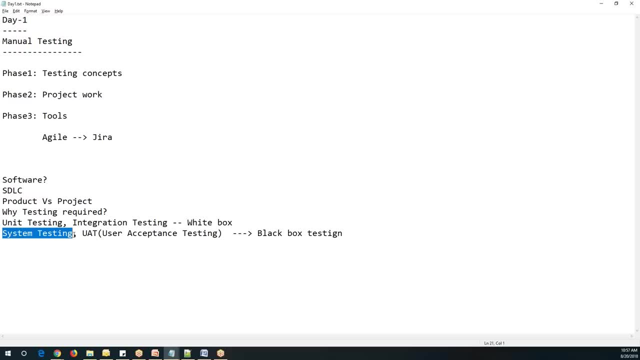 testers, automation testers- everybody is involved in the system testing, because here we need to know the complete requirement of the customer, we need to test the software completely and we need to perform so many types of testings here: different type of testing, functional testings, non-functional, ad hoc retesting, regression testing, sanity, smoke testing. so there are n number of testings we have. 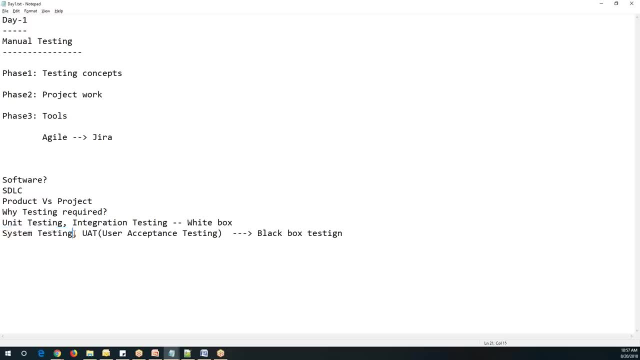 to conduct during system testing phase. so once we have a completed system testing, then we will hand over the project or software to the users and they will perform the uat testing. and once the uat testing is successful, then our application or software will move to the production environment. so this is how the software development testing will happen. 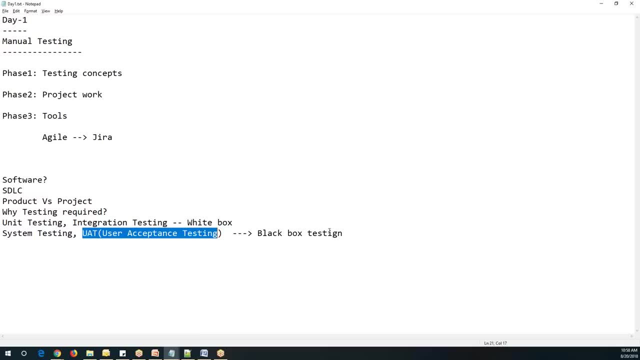 in the real time. okay, so i'll just stop it here for today. just very, i discuss very basic things and, uh, from tomorrow we'll continue the rest of the things, okay, so that's all for today. if you have any questions now we can ask. right, so let's see what we have. 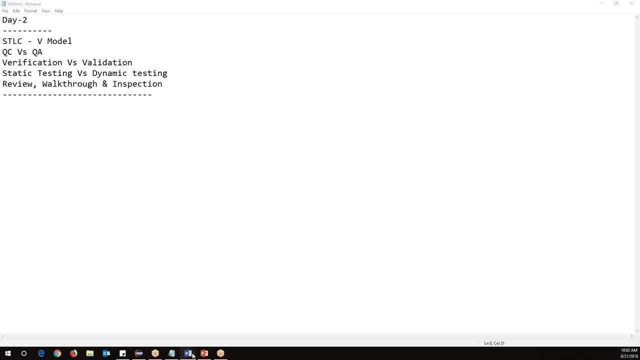 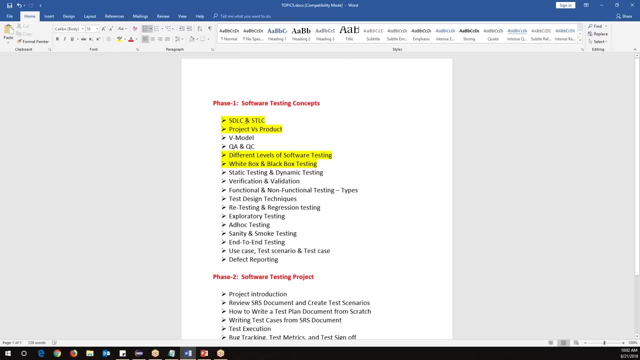 discussed in the previous session and then we'll continue further. in the previous session we have discussed about htlc and htlc, and htlc will talk about overall process of software development and htlc is one of the part of sdlc. so sdlc more focus on testing activities and we have also seen 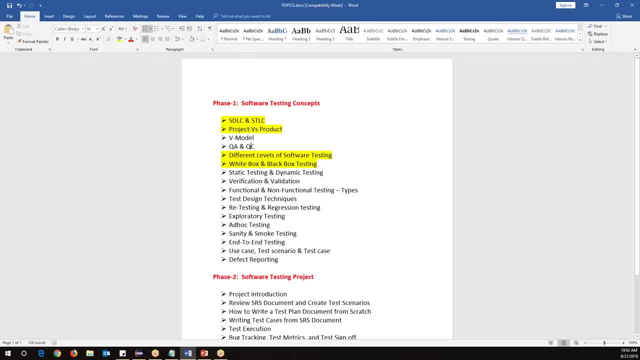 what is project and what is product like project is developed only for specific customer and product is for market requirements for multiple customers. and also yesterday we have seen different levels of software testing, like first level is unit testing, then second level is integration testing and those two testings are done by the developers. 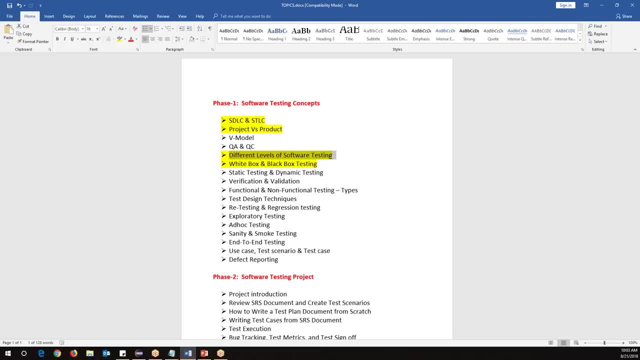 and which all comes under the white box testing, and also we have discussed about system testing and uat testing. so they are all comes under the black box testing techniques. also we discussed about white box testing and black box testing. so in the white box testing we need to test the internal logic of the program and in black box testing we test the application. 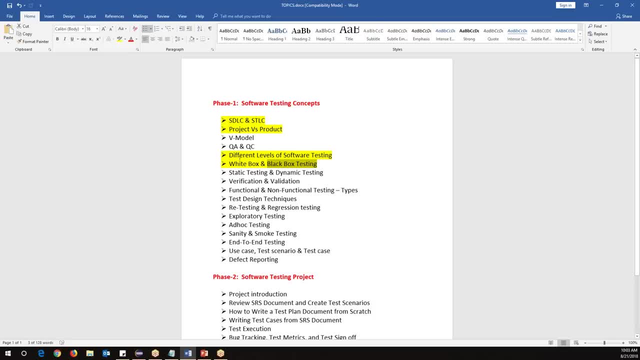 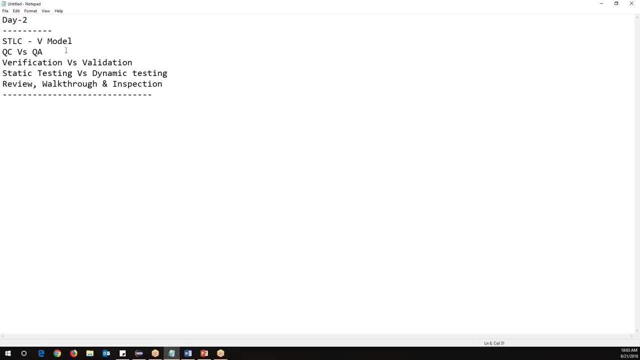 with respect to customer requirements or satisfying or not. so today we will discuss a few more concepts like v, model qa and qc, static testing and dynamic testing, and then we'll discuss about verification and validation. so these are the items we'll discuss in today's session now. 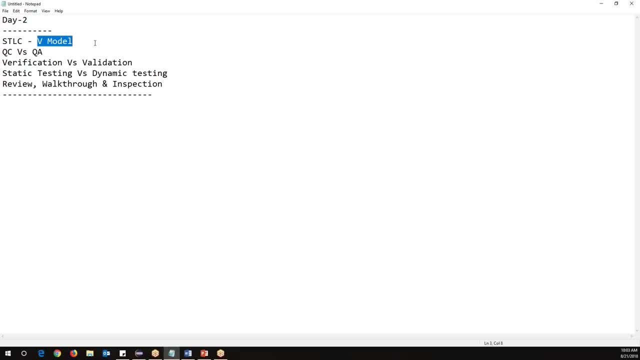 this is our agenda, so first we'll discuss about v model- this is comes under the stlc and the qc versus qa and verification versus validation, and static testing and dynamic testing, and also we discuss about a few techniques like review, walk through and inspection. okay, now let us start with the stlc. yesterday we talked about a few things. 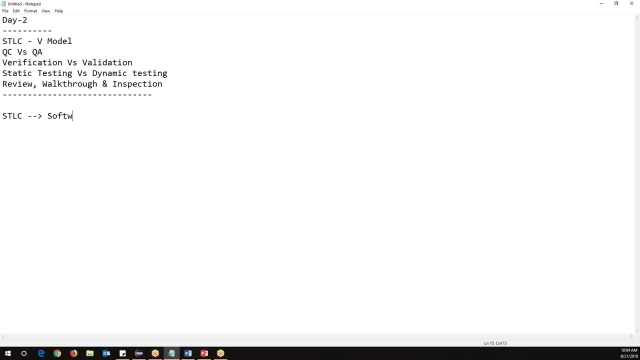 about stlc. stlc means the software testing life cycle, software testing life cycle, so this is a również step for urban software development process- and stlc more focusing on testing activities like understanding requirement, writing test cases, writing test plans, executing our test cases and defect reporting. all this comes under stlc part. now, before discussing the rest of the 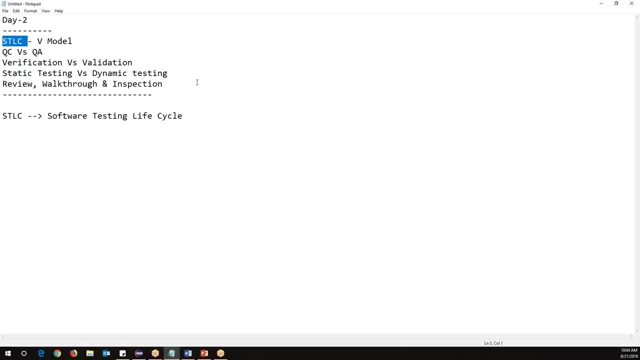 things. let's understand the v model. so in stlc itself we have a different model like a v model or fish model and agile model. so there are multiple software development models. we have STLC more become famous In V model. Okay so, but nowadays people are not using this, but it is started in V model. 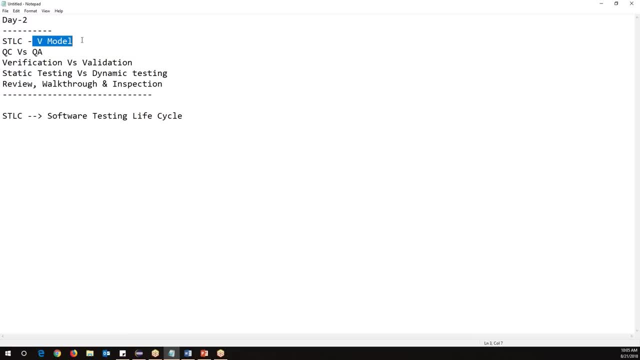 So nowadays all the companies are using agile process, So we'll discuss that also in the coming sessions. So first let us talk about the V model, because all the stuff we can know about V model- So QSC, QA, verification, validation and all we can learn by using V model- 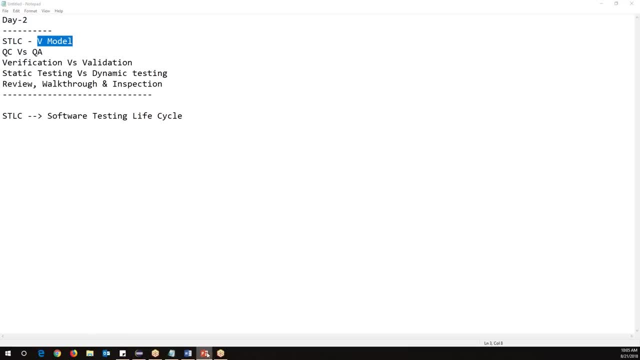 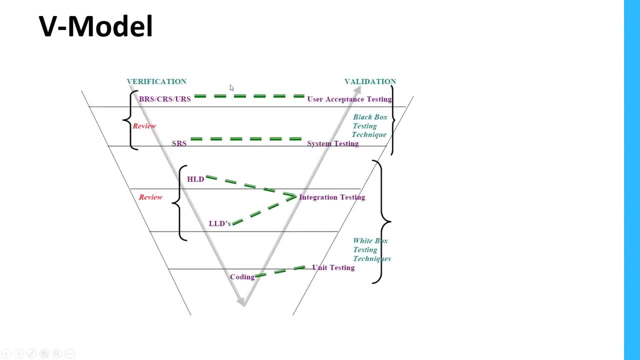 So what is V model means? Let me just share small presentation. Yeah, now, in this model this is called as a V model. So why it is called V model? because it is a shape of V, right? So let's understand this model very clearly. So here, one side is a verification part and the other side is a validation part. 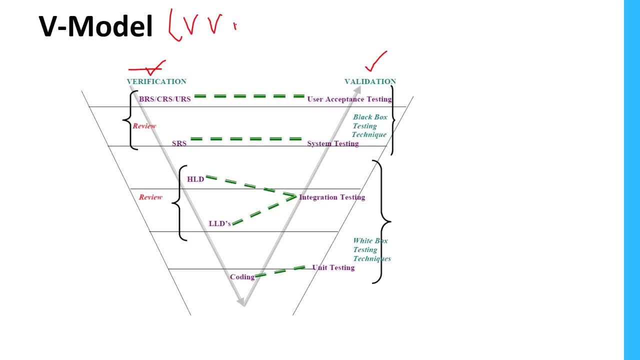 Okay, verification and the validation. These are all Also called as a V V model, verification and validation. So in this model, okay, all development and testing activities go parallel. Okay, So if you see this, one side is called verification, This part is completely Verification part. the development activities will happen here, and this side is completely, the testing activities will happen. 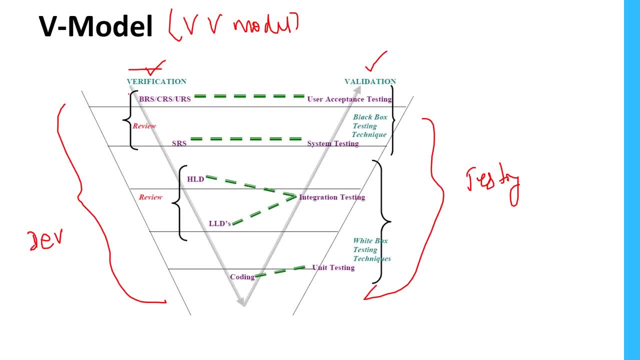 Okay, Now, if you observe this side by side, so it's of- the SDLC process will start from requirement understanding night. So here these are. first is BRS, CRS and URS means business requirement specification or customer requirement specification or user requirement specification, So all are same, basically. 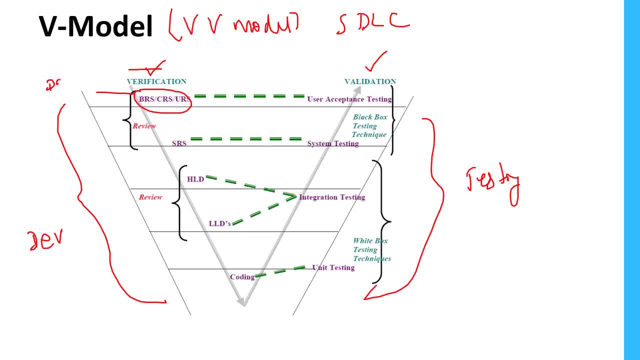 These are a document which is provided by the customer, which contains the customer requirements. Okay, this is very important for us, but this is general format, So it is not in the technical format. So, again, Business analyst will prepare some document called as a SRS document- software requirement specification document- based upon the BRS document. 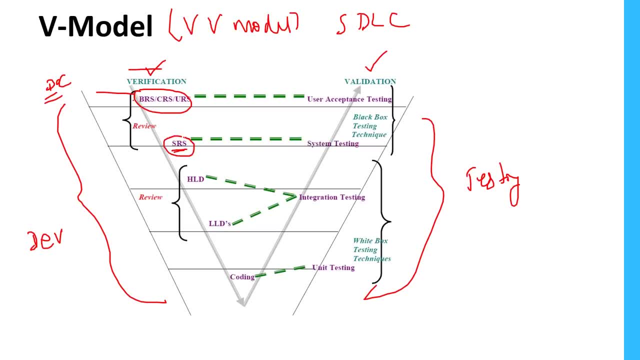 And it is more technical format. So even developers, testers, everybody in the team, can understand this SRS document, which contains data, flow diagrams, ER diagrams, use cases and Everything will be there in the SRS document. and also what are the variations we need to perform, What is the functionality of application, will be there in the SRS document. 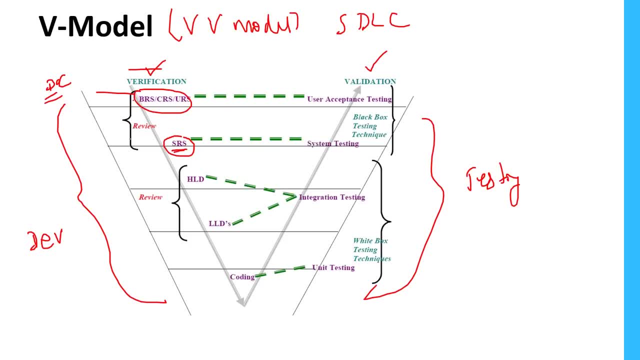 So this will be prepared based on the BRS document. So these are the two initial level documents. when software development is started, Okay, and then based on this, and then these are all comes under the requirement phase, is DLC. This is the first phase, requirement phase, and then HLD and LLD. 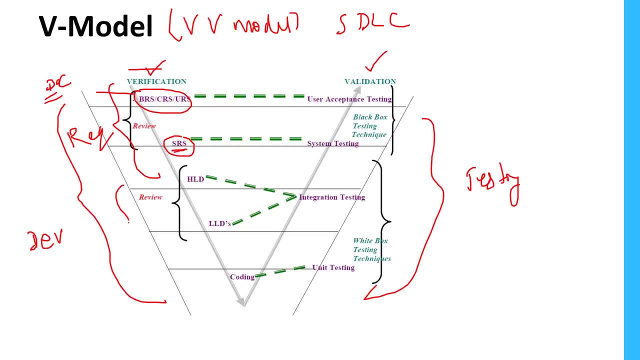 So, based upon the document we've prepared, the next phase is the design phase, right? So in the design phase we have a documents called HLD, and LLD means a high level design Document and the low level design document. so high level design document contains a very high level. 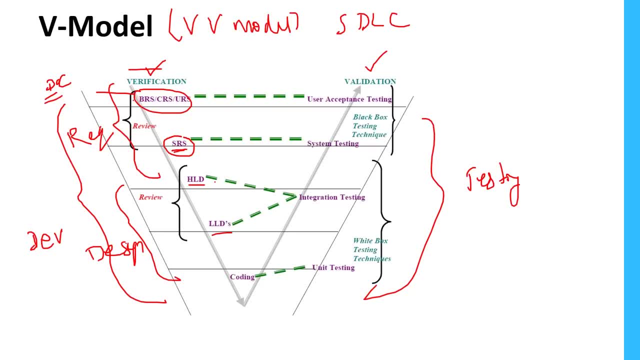 picture of your software contains some data flow diagrams and ER diagrams and everything is a diagrammetical picture or diagrammetical Presentation. we have in HLD very high level modules will define here and when you come to the low level design document, It is a very detailed document again. all the normally the full project will be divided into. 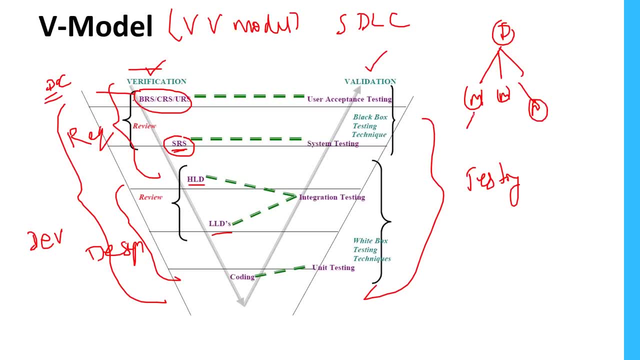 modules, main modules, Right. So again these main modules divided into sub modules. So high level HLD contains a main module- information, and low level design contains a very lowest level modules. Okay, detail information will be there. So HLD and LLD preparation is done by the designers and in the designing phase. 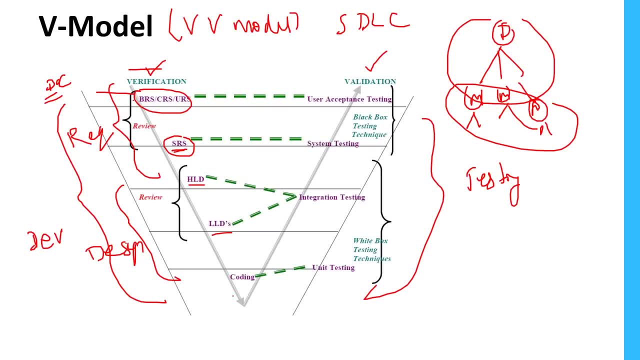 Okay, and once the design is completed, then testers are. then developer will start coding based on the low level design document. So whatever modules They have assigned to them, they start doing coding here. So if you see this part, these are all verification part, because here we don't have software ready. 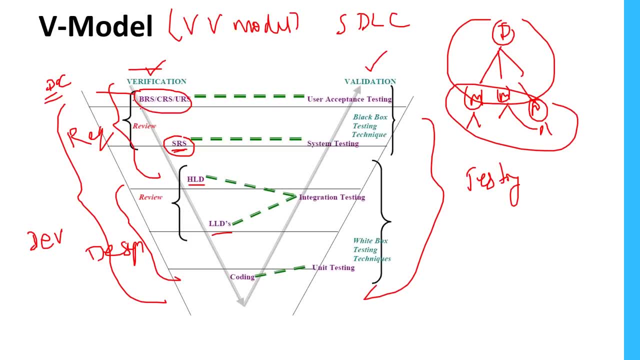 So we do only testing on the documents. So if you observe here we need to review this document again, review the SRS document, review HLD reveal and if these document perfectly correct, And then whatever software we are developing will be the correct, because the software development is based upon these documents. 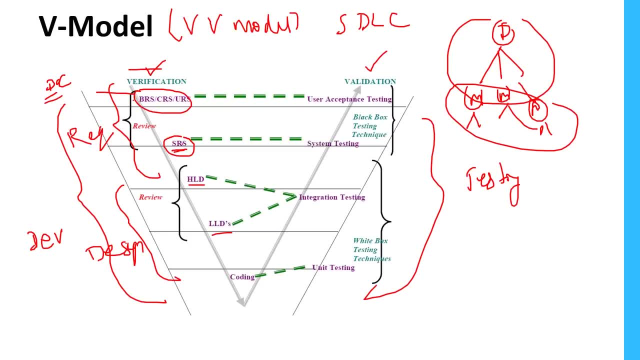 So these are documents which are inputs for Developing the software right. so here There are so many reviews will happen Because to ensure that our documents are correct or right, correct or not, if it is correct, the information is completed or not. So that kind of review we need to do as part of this documentation, if you observe here 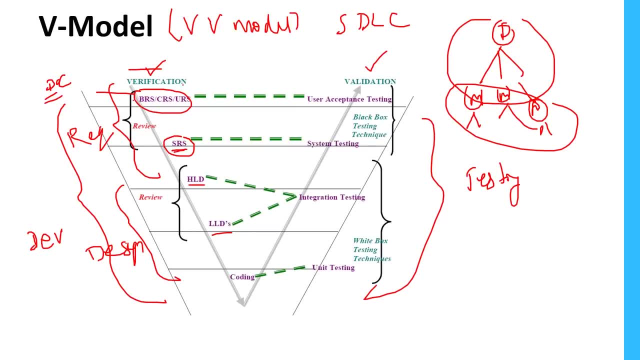 This is a verification area, So we need to verify this dog. What is verification here? verification meant: are we following the process correctly or not? so, in each and every step, if I do something, have you done this correctly or not? so that is a re-verification verification process. verification means whatever we did, which. 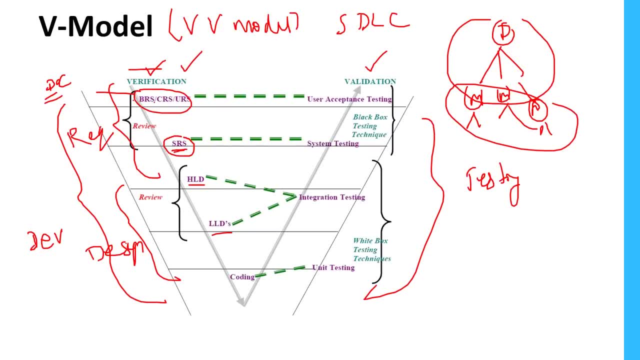 is correct or not, that's called as verification. so to ensure correctness and completeness of the document- if simply say to ensure the correctness and completeness of the document is called as a verification, so we do step by step verification process here. okay, this is all one area verification involves. 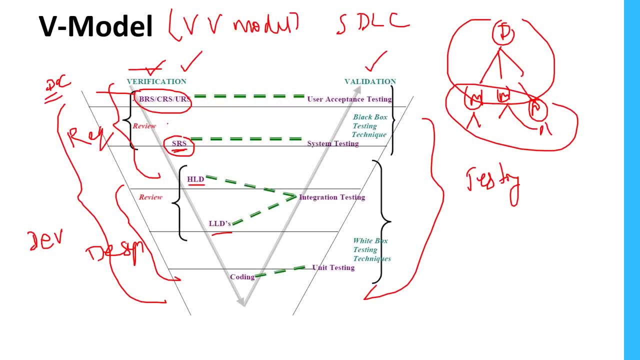 reviewing the document, not only review. sometimes we do walkthroughs, inspections, so we'll talk about those techniques in next slides. but here verification means reviewing the main documentation part. okay, and once the coding is done here, then software will be ready here. okay, once the coding is ready, then software. 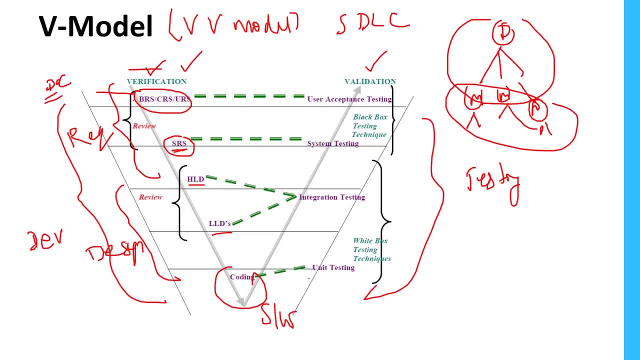 is ready here, and once the software is ready then validation part will start. so before software is ready we do only verification, and after software is ready then we do validation. so as part of validation, unit testing, we do integration testing, system testing, user access testing. so all levels of testing comes under validation part. so what is validation means here? 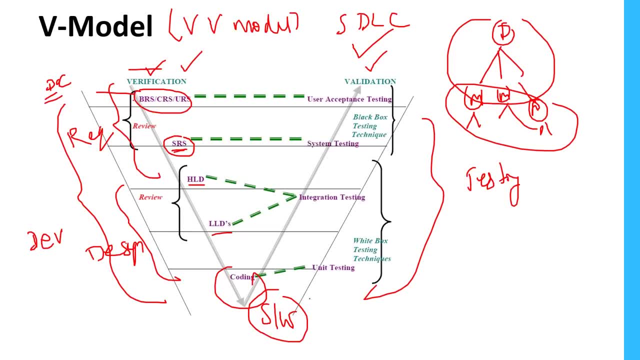 validation means checking our product whether it is working according to customer requirement or not. so whatever requirement is customers provided it should work according to the customer requirement. so that is a kind of validation. so a few things we need to understand here is: verification will happen before software is developed. okay, once the software is developed, then validation. 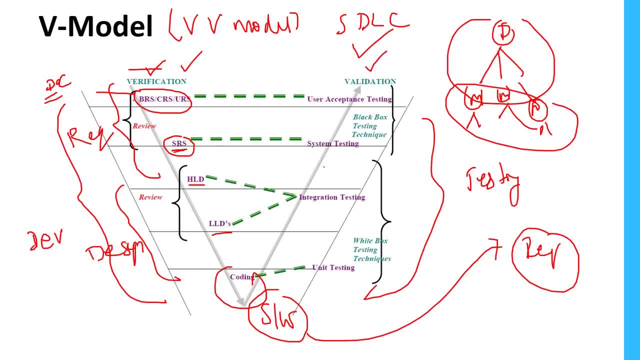 will start here, in the form of unit testing, integration testing, system testing and user acceptance. these are all validation techniques. okay, all levels of testing comes under the validation. the first level of testing is unit testing. we need to do our coding and this is white box testing technique again. 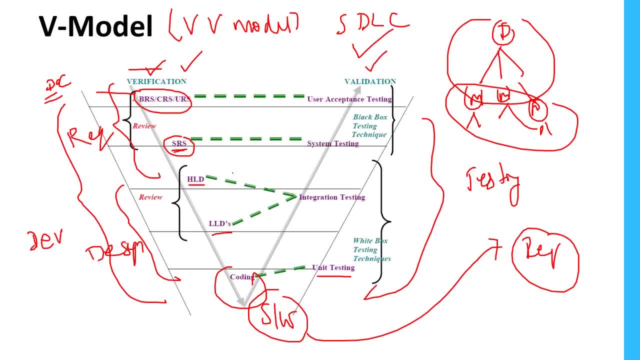 and Integration testing. we do a based upon HLD and LLE document because HLD and LLE documents Discuss more on modules and sub modules, right? So integration testing if you want to perform, we need to refer these two documents, HLDs and LLE. 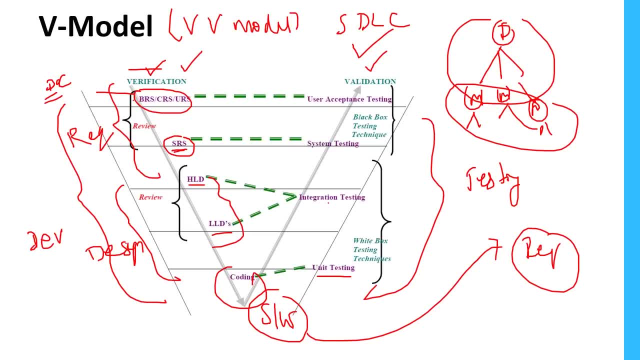 This is also done by the developers. This also comes under white box testing technique and Then system testing. This is the main area where all our testers are involved. So in the system testing we need to refer the SRS document, which contains the all the functionalities provided by the customer. 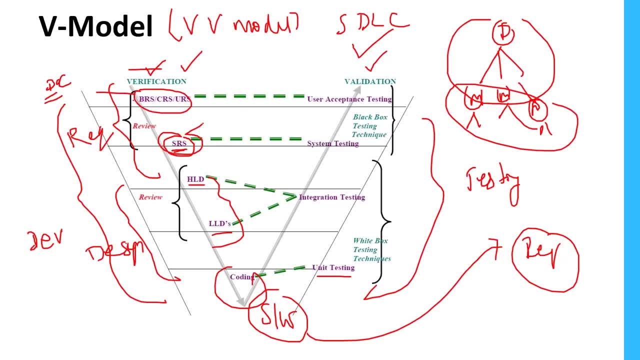 So we need to thoroughly understand each and every requirement, and then we test the complete software Whether it is working according to customer requirement or not. So that is all about system testing here. We don't test the code, we test the overall functionality of the application with respect to customer requirement. 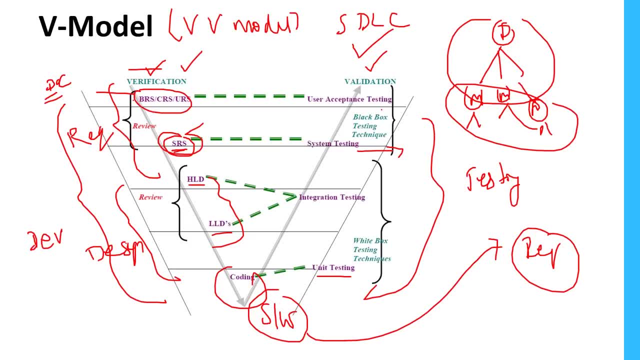 That is called as a system testing and this is comes under black box testing technique, As we discussed earlier. right and what is the input document here? SRS document is our input document and Then user actor acceptance testing is done by the users and based on their document. 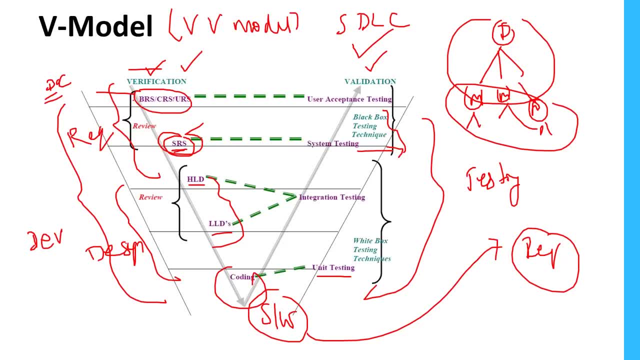 So BRS, CRS, URS is the document which is created by a customer. So customer again, we check your software whether it is working according to their requirement or not. That is also comes under black box testing. here Also they don't test the code. 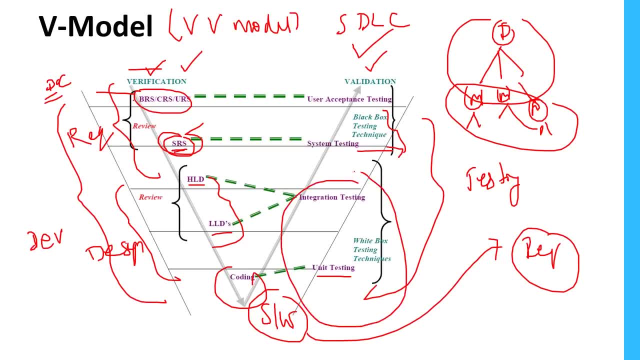 so here, integration and unit testing comes under white box because we need to test the code and Developers will do it, and the next level is system testing and user accept. testing is done on The actual software and these are comes under the black box testing technique. Okay, so one side is verification, The other side is validation, two things We need to remember. 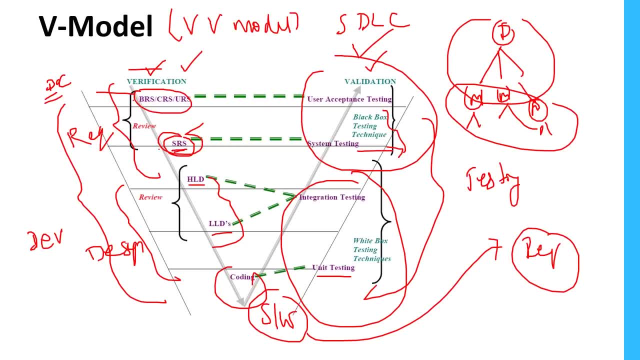 Verification should perform before software is ready. That means we need to verify the only documentation part here. So whatever documents are saying about software, the documents are ready or not completed Or not correct or not. we do a lot of reviews on this. that is called as a verification. 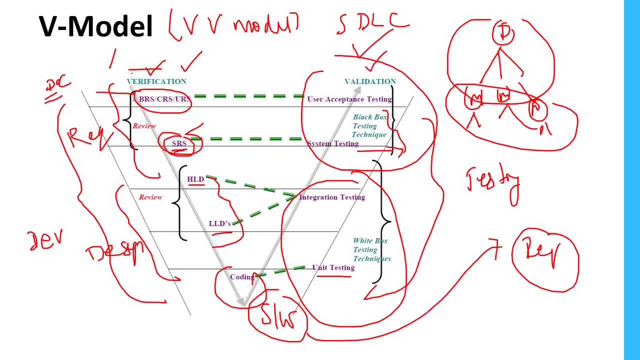 Okay, are we following the correct process or not? So that is the main intention of verification, and validation means whatever we already done, Which is correctly working according to requirement or not. That is about validation. But when you do unit testing, by that time you already done something, you already developed some software. 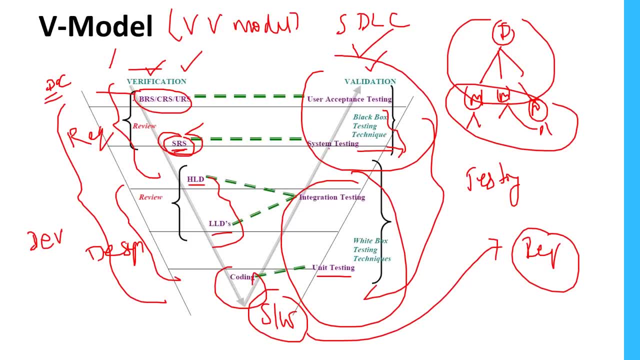 So on top of the software you do testing and integration testing system test, unit testing. so all validation Testings can be can be done on top of software, after completion of your software. That is a validation. Okay, so verification and validation. Just a moment, One second. 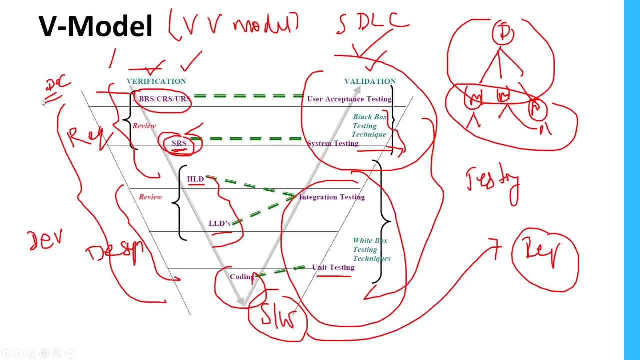 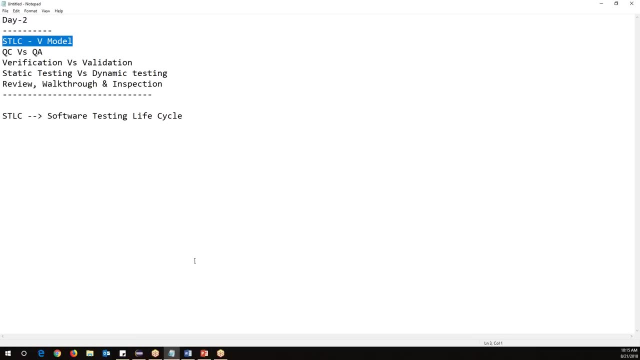 okay, I'm just a moment. Okay, so now we discussed about V model, stlc, V model. so in the V model we discussed about the verification and the validation and one more time. Let me just discuss a few more times. So, verification and the validation. so verification has to be done on the 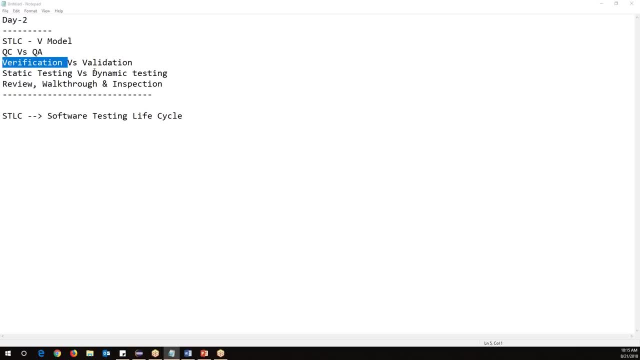 documents before software is ready and validation should be done after completion of the software. So unit testing, integration testing, system testing and UAT testing comes under the validation under verification, reviews and walkthroughs inspections. So I have listed a few techniques here which are comes under the verification part. 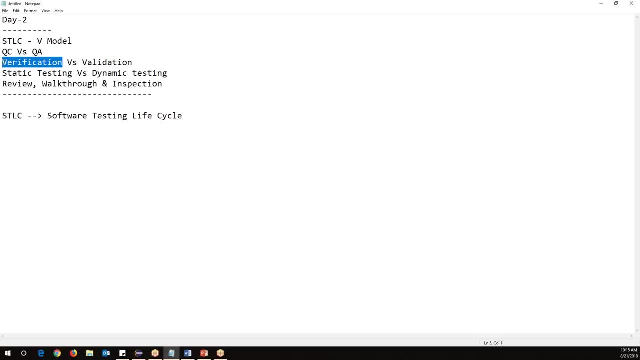 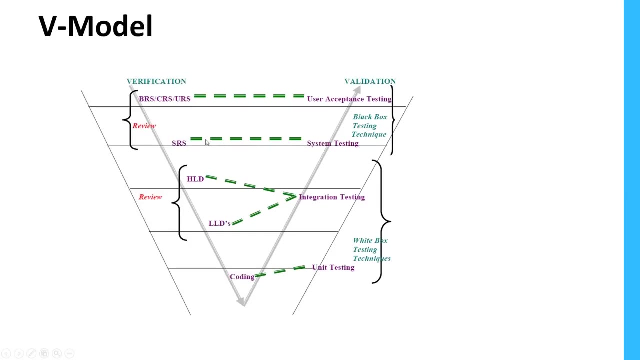 So, because the main focus here is on documentation part, We need to test the documents are correct or not. That is a verification point, verification and validation. Now, here it is also involved static testing and dynamic testing. So, for example, here here we are testing the documents here, right, 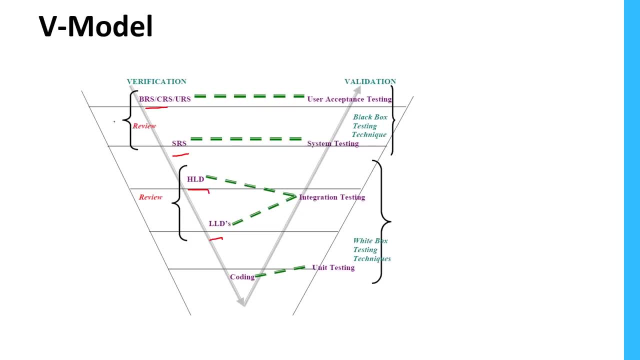 So the software is not it ready. We are only testing the documentation. So documents are always static, So this is called as a static testing. static testing means verifying the documentation part. We haven't test any software. verifying the documentation is called as a static testing. 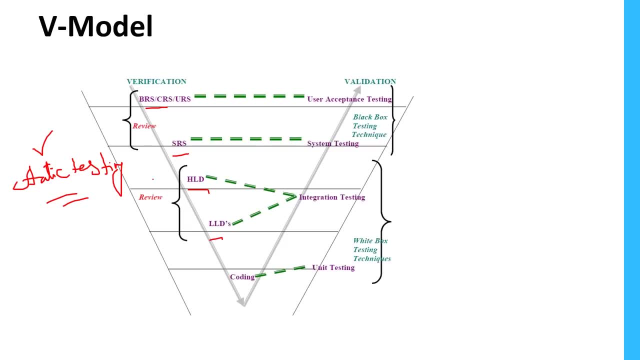 So ultimately we are testing the documents whether they are correct or not. that is called as a statics testing and there is another kind of testing called as a dynamic test. So dynamic testing means once the software is ready. once the software is ready, here We will test this dynamically because while passing multiple inputs and getting the outputs, 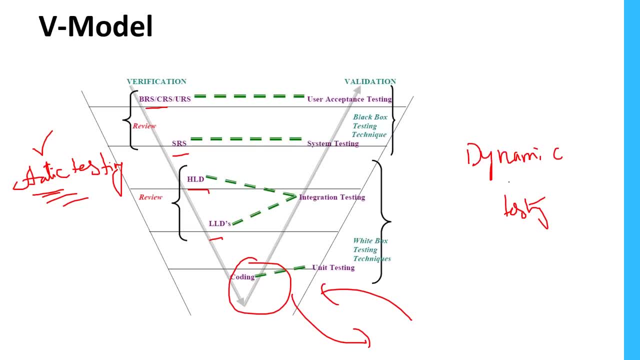 are correct or not. We will validate in each and every step. So this is called as a dynamic testing. So you need testing integration testing system testing all comes under dynamic testing techniques. So the technology is different, almost same. so verification, verification and statics testing. 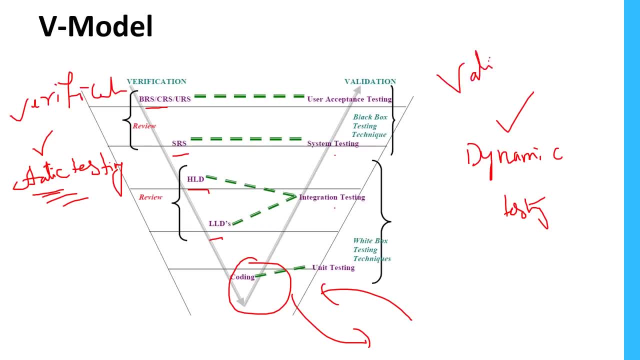 comes under one category, and validation and dynamic testing comes under another category. So verification means testing the documentation. that itself is called as a static testing, because we are testing the static documents here, but in other side we are testing the software once the software is ready. 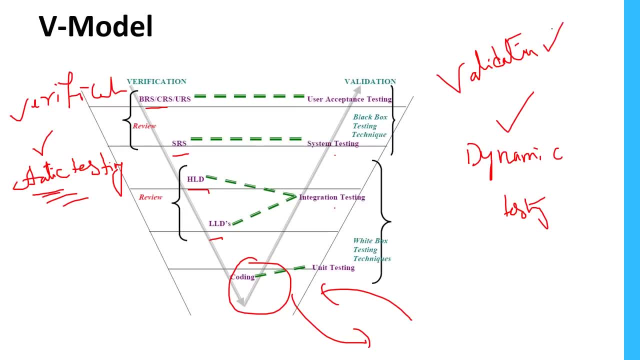 We are testing it according to customer requirements, So it is called as a validation and here we are actually testing the software. So it is a dynamic testing: static testing and dynamic test. now under verification, We use techniques called as a reviews and we have a walkthrough. 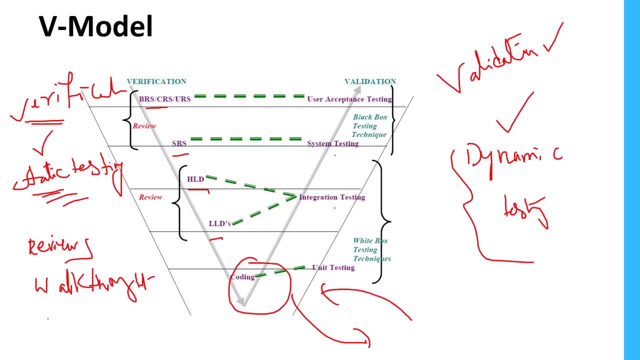 So these are different techniques of use at the time of our documentation and then inspections, reviews, walkthroughs and inspections. So these are the techniques we use During verification process, when, whenever we review this documentation, and here at the validation and dynamic part, we use unit testing, integration testing, system, testing and accept. 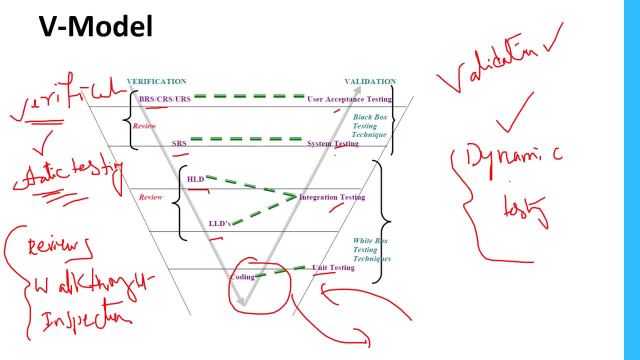 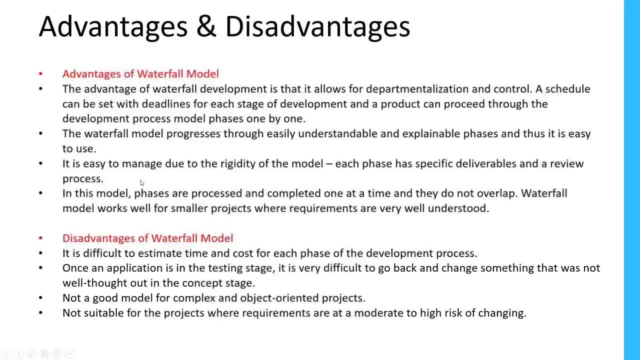 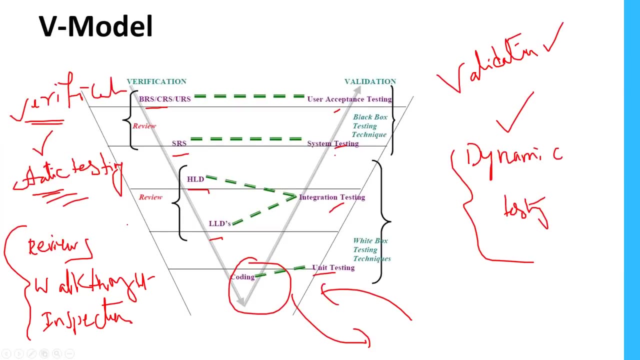 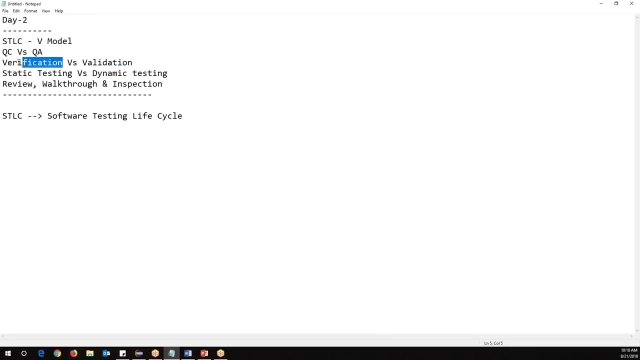 test it. These are all examples for validation and dynamic testing. Okay now, okay, Let's see rest of them. This is about V model. okay, fine, So let me just conclude. Yeah, so verification and validation. we discuss a verification is mainly focusing on the documentation. 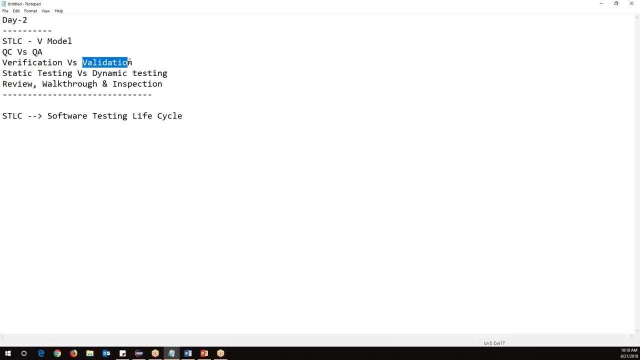 part and a validation is mainly focusing on the software to be tested according to the customer requirement and also static testing is a example for verification and dynamic testing is example for the validation. during static testing with test the documents. during dynamic testing, We test the application or a software. now here review, walkthrough and inspections are. 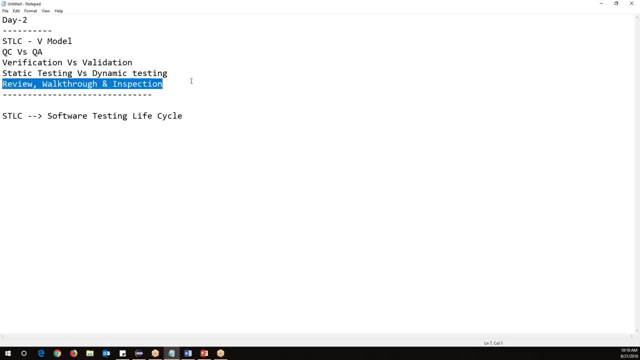 a techniques which we need to use as part of verification. So let us see what is review, walkthrough and inspection: review, walkthrough and inspection. So review means reviews are conducting on the documentation. Suppose, if you have any document we do set in kind of a review. okay, whether the, whether. 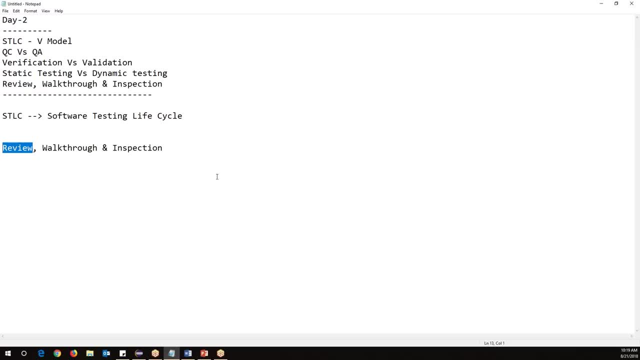 the document is completed or not. if it is complete, it is correct or not. we will verify. that is a part of the review. Okay, So this can be done individually. So in a team we have five to six people, each individual can review their documentation. 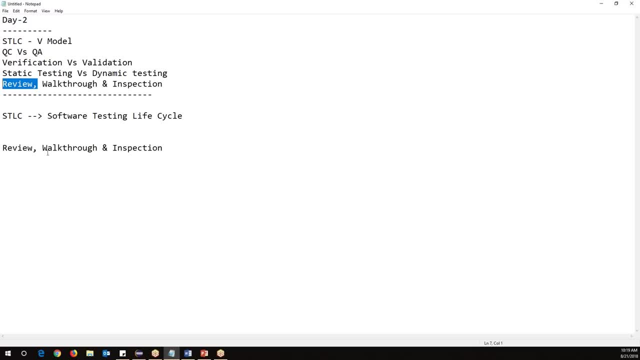 Okay. so whether the document is correct or not, complete or not, so the main intention. So, for example, what is few examples of reviews are, let's say, requirements reviews: once we have get the requirement document, we do requirement review. and similarly, if you have some design document, you do design review. and also sometimes developer will do the code review. 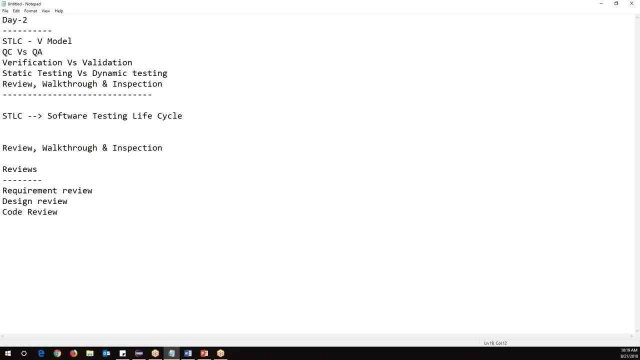 This is not part of testing, but code. once you have done, the developer is written the code. that code will be reviewed by somebody else. that's called code review. and once you have prepared your test plan- So we have a test plan- reviews, test plan reviews. and also once you have created some document. 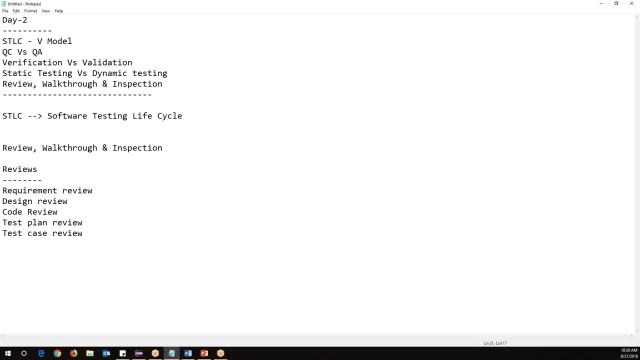 on test cases, you need to do test case review. So for each and every document you created during testing activities, you have to review with yourself or some with that something, okay, other team. So these are all reviews. So review is mainly focusing on whether the document is correct or not and the information. 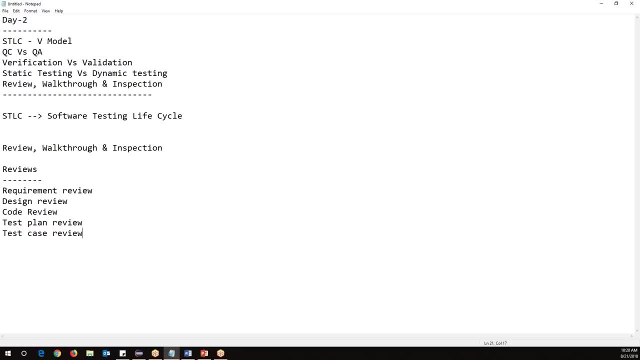 which is provided in the document are complete or not. So that's the main intention of doing the review of the documentation part. Okay, and there is another technique we have all through that is also comes under the verification part. So what is that walkthrough? 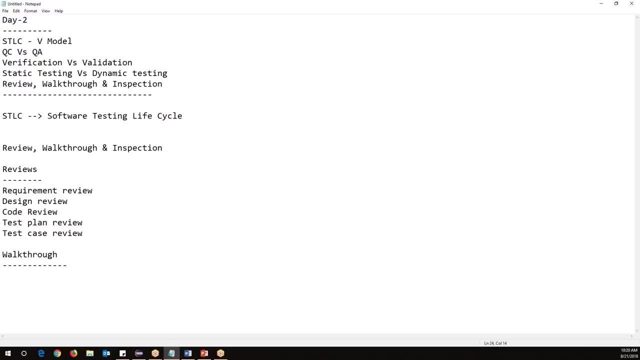 So during walkthrough. so there are people are involved, not only one guy. it is not individual review, Okay, It is a formal review. We can just discuss the issue at the peer level. So for example, in your team, let's say, five people are sitting together. 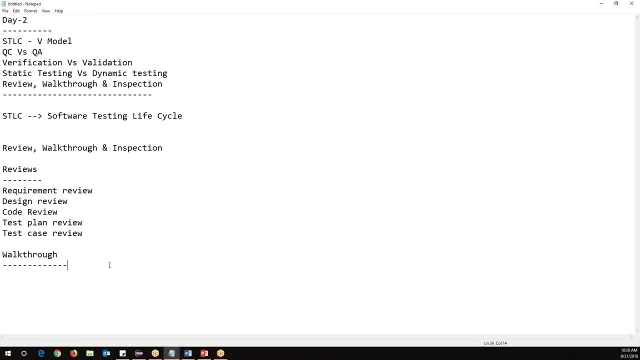 So what you guys can do is just going, enter into the room and one guy will read the document and the rest of them will just see the document and, if they have any clarifications and doubts, and discuss within themselves. there's a kind of a walkthrough. 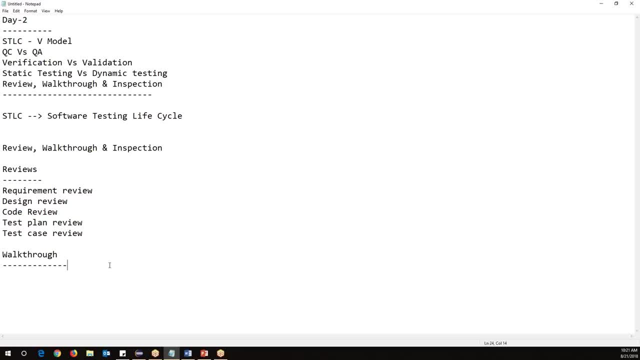 So walkthrough means it is a formal review And it will be done. It will be done between multiple people, Okay, and this is a more formal because we need to go to a room and invite the people and do the review and this walkthrough should be done within the team. 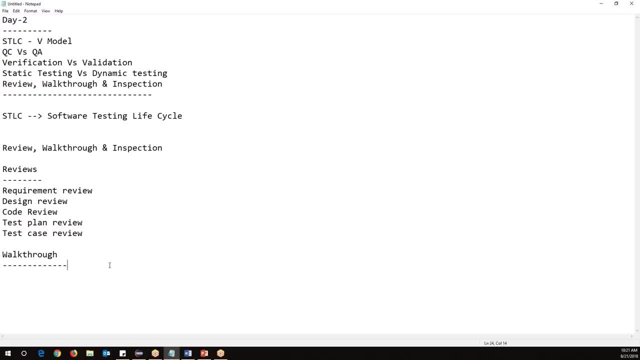 Suppose, if you are working on five testing years, between those five testing years the walkthrough should happen. Okay, and this is a walkthrough, So walkthrough is also done on the same documentation Here. we need to remember a few points here. So walkthrough is a formal review and we can discuss and raise the issue at the peer level. 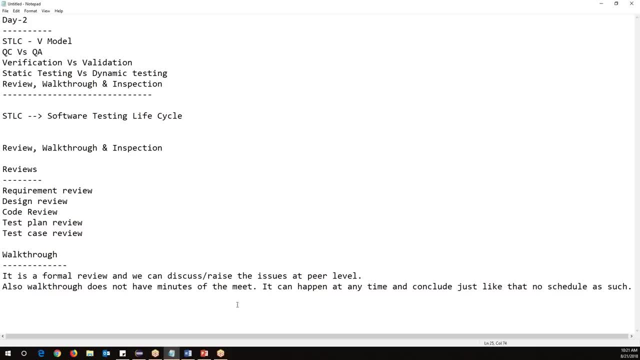 Peer level means within the team, and also walkthrough does not have any meetings of minutes. Suppose if it is an official meeting and then if you have all the team members, then we may prepare some kind of minutes of meeting, what we discussed during that meeting. But here walkthrough is whenever we want. we can just go and walk through the document. 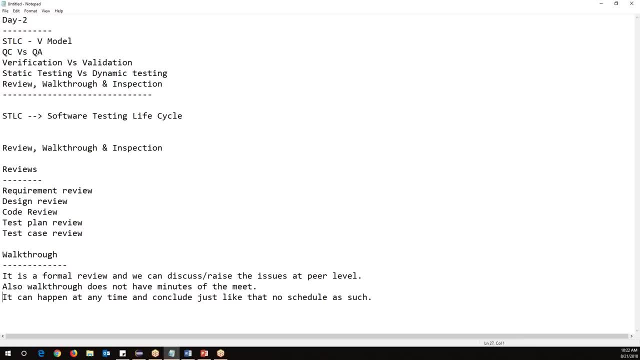 with the team, internal team. So we don't need any minutes of minutes for this. So it can happen at any time. Okay, And conclude just like that. So no schedule assets. So for this we don't need to have any schedule. 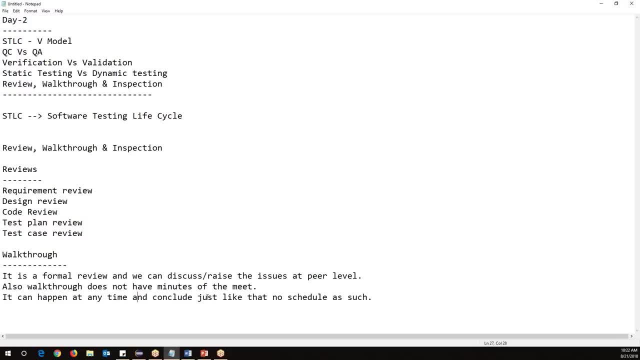 So whenever we are having some free time, just call the team members and just go and walk through the document to understand more about it. Okay, There's a formal review called as a walkthrough is another kind of type of review, but only the differences in the review. it will do individual and when you come to the walkthrough it will. 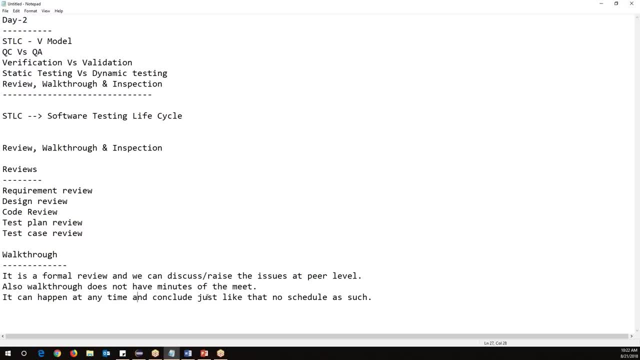 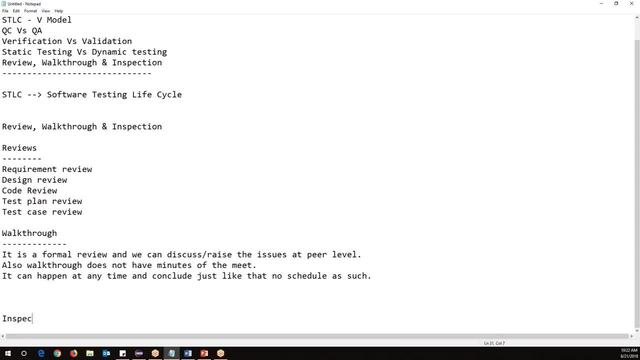 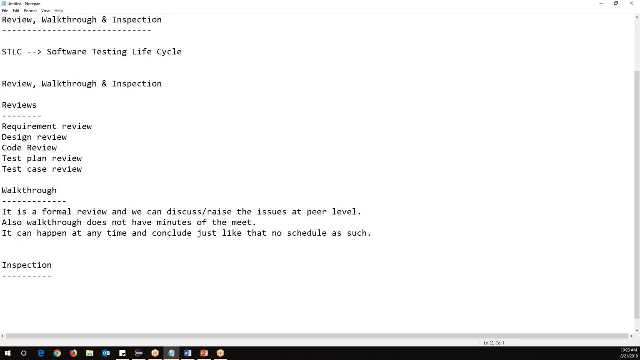 do within the team. Okay, This is another technique we use during verification and there is another technical, as an inspection inspection. So inspection in the sense it here. this is again a different kind of meeting and this is also formal, very formal. So here we need to invite all the team, like testing, development, production management. 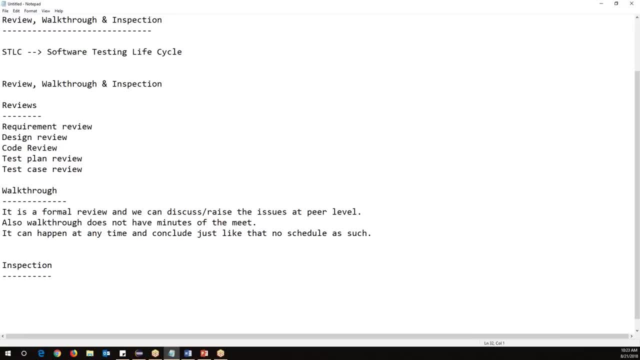 So whoever is a part of your project, You need to invite everybody, and here all the team members will be involved during this kind of inspection, But the mainly three people will be there. may not three roles will be there, So one is other, So other means war is created. the document. he is the author. 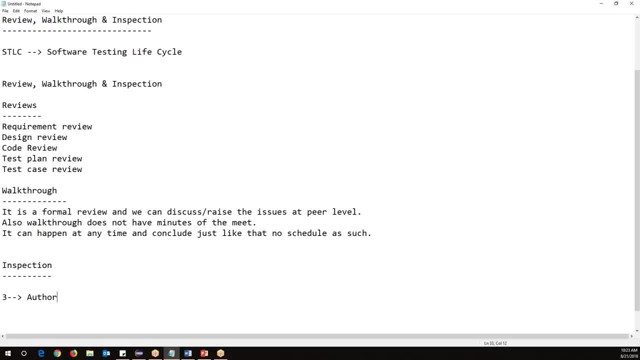 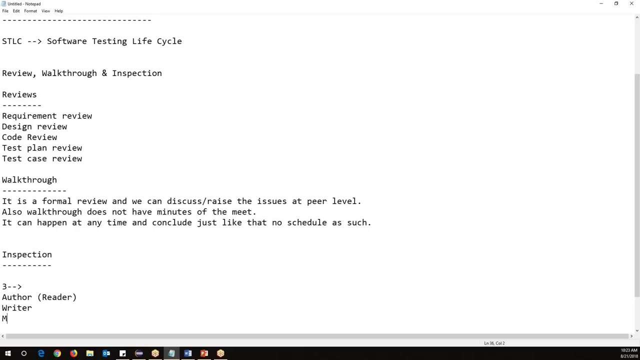 So he will explain the document. and there is one more guy, other and second. one is called reader, Okay, And then other it's called as a reader. other himself is called as a reader, and then whether one is a writer and a moderator, Okay. 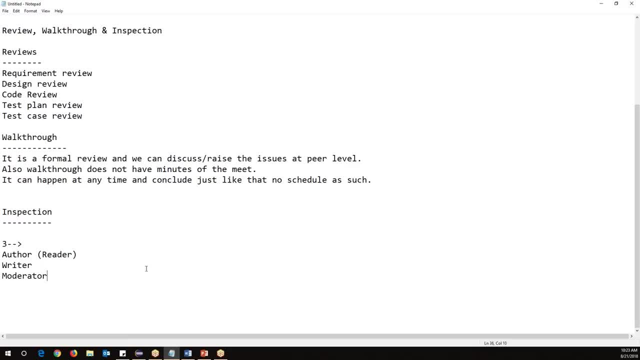 These are the different roles we have during inspections. other is a reader. He will read the document, what they have created or what they have mentioned in the document. and one more guy will play writer role, So what he will do is So the other people are. team members will rise and questions on the document. 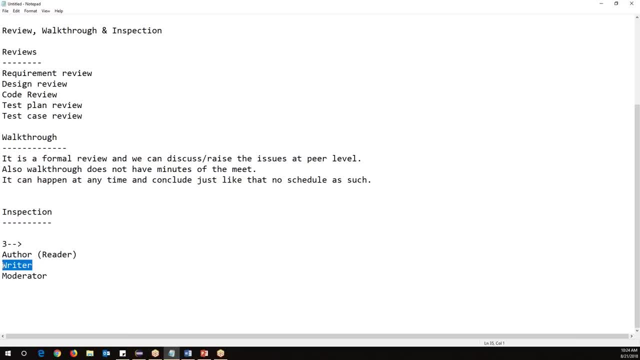 So he will note down those questions and comments. So writer is responsible for writing all the comments which are provided by the team. There's a writer, There is another role called as a moderator, So he will mainly moderate these people and along with the other team members. 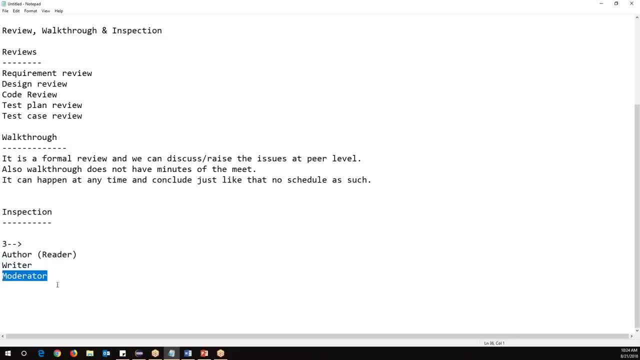 Okay, He's just play an anchor role. Okay, So these are the people, main people involved during inspection, Other than this. So a team member. So this is a team member plus a leader team. It means a QA, means a testing team, developer and project management, project management. 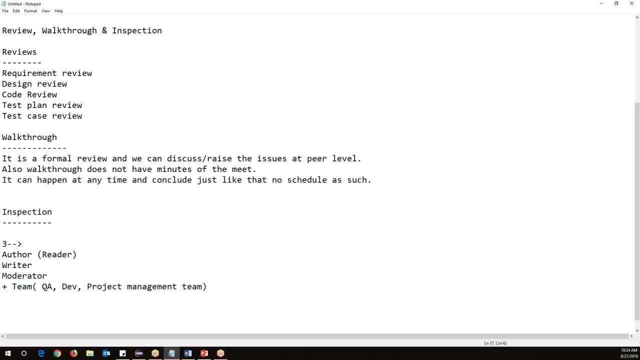 So everybody we know involved in the inspection. so that's the reason it is more formal. So we need to send an email, Schedule a meeting on that particular time and invite all and do certain inspection. So these are all called a review technique, Verification techniques, reviews, walkthroughs and inspections. reviews, walkthroughs and inspections. 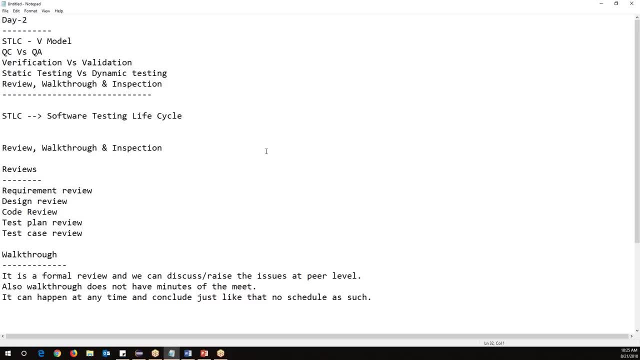 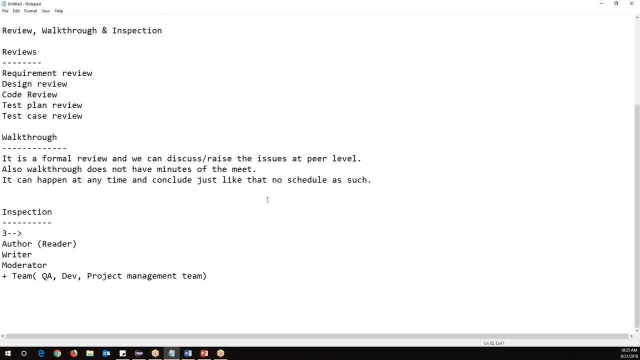 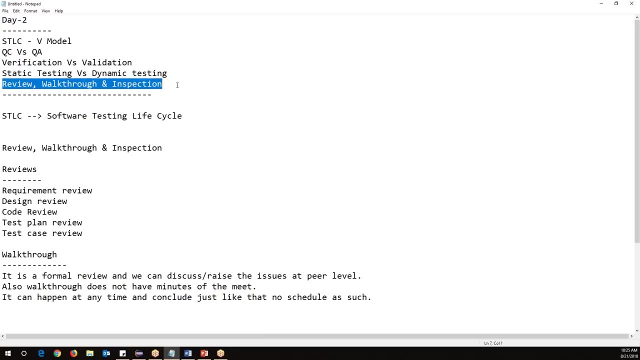 which are comes under the verification part. okay, so in we model the firm side, left side, comes under the verification right. so reviews, walkthroughs, inspections, always conducts on the documentation part, right. so in the next one is: and these are also comes under the static setting. we can say simply static testing techniques. these are all interrelated, so verification. 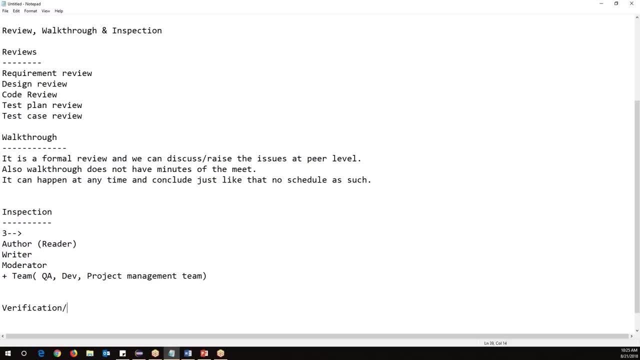 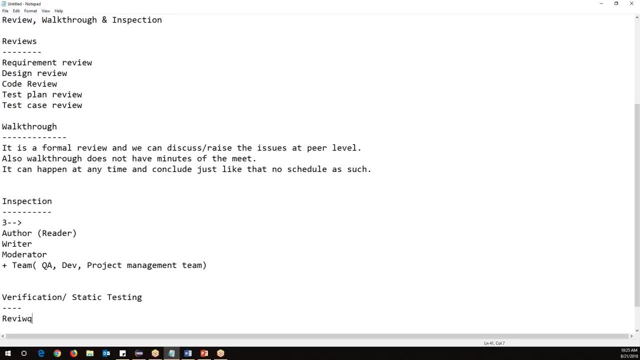 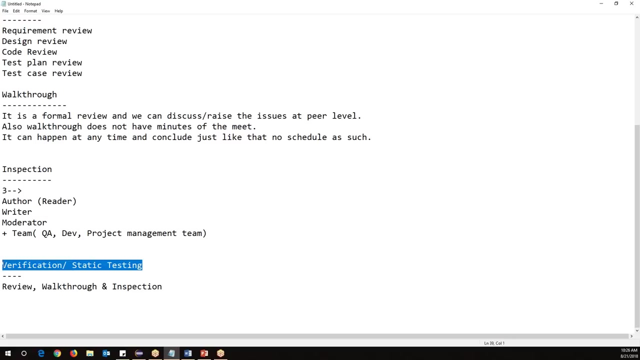 okay, and static testing okay. under this- this review, walkthrough and inspection- so these three comes under one category: verification, static testing. so these are the techniques. these are just games- okay, if you want to do sense of verification and static testing. so we follow these techniques. these are all called as a techniques. 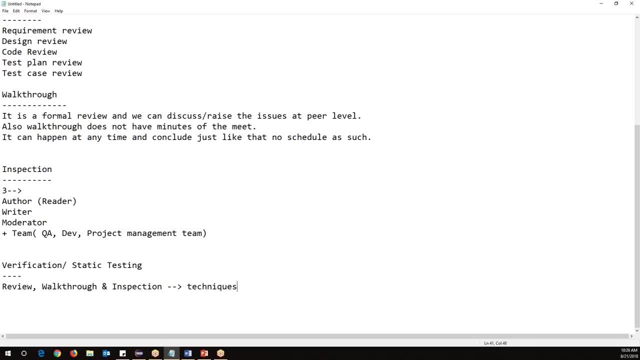 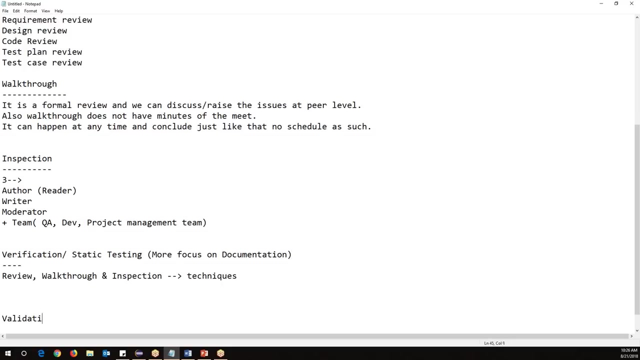 okay, so more here we more talk, concentrate on documentation or focusing on more, focus on a documentation part, because the software is not yet ready. okay, so once this is done, then validation will start. so validation means validation and this is also called as dynamic testing. dynamic testing- okay. 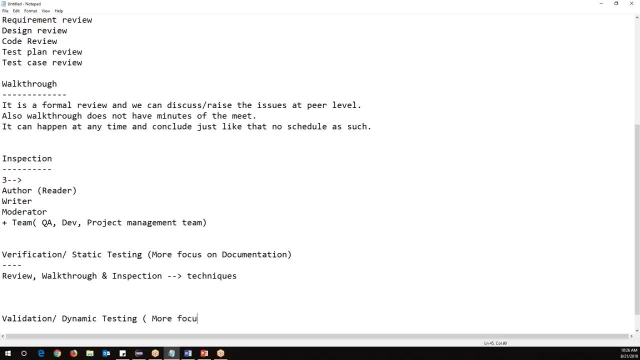 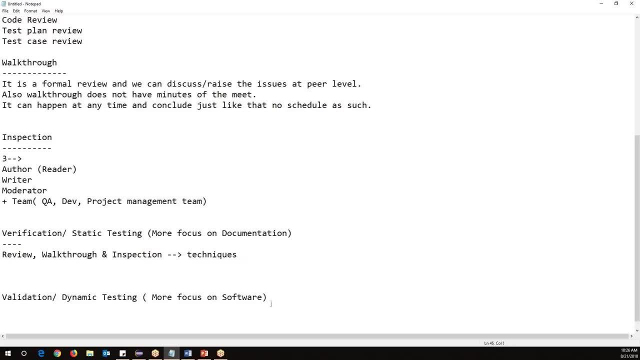 So here, the more focus on the building or more focus on software, more focus on software. and what are the techniques we use here? we use unit testing, right, and then integration testing, integration testing and then system testing, system testing and then UIT testing, UIT testing. so these are the examples of verification and validation. okay, so these are the examples. 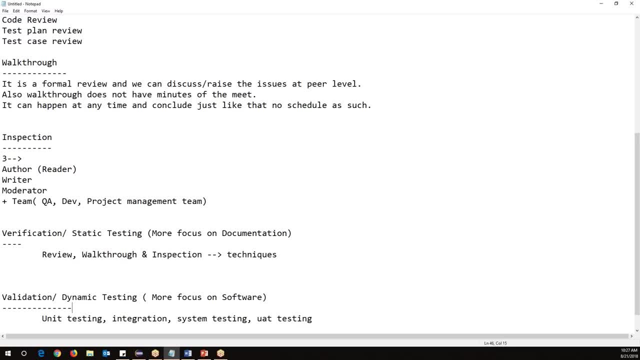 of verification and validation. Okay, So is it clear so far. now please confirm on the chat window. if you are clear, then I'll proceed further, okay, Okay, so we have discussed about verification, start testing and this will be more focusing on documentation part And review. walkthrough inspections are a technique which we have used during verification part. 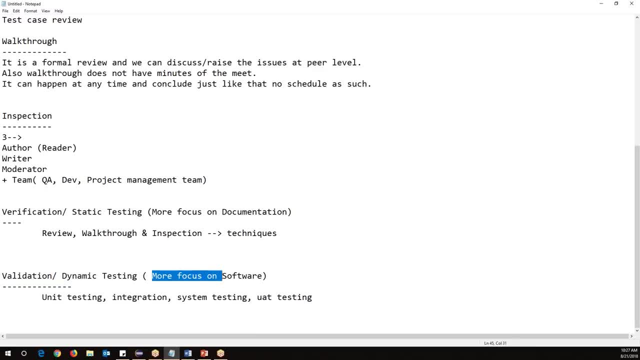 and when you come to the validation, these are dynamic testing and here more focusing on software, which is already done, and here are the main techniques, or unit testing, integration testing, system testing and UIT testing. these are also comes under the levels of testing. okay, so just a second. let me save this. 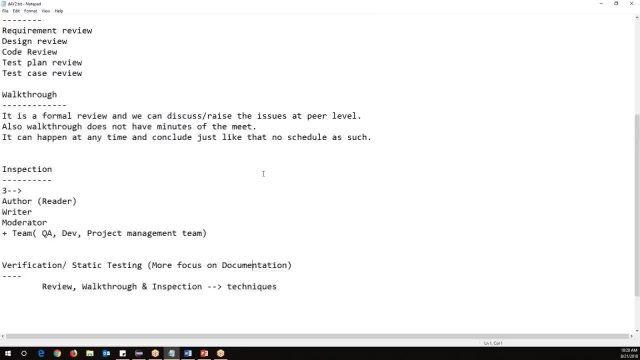 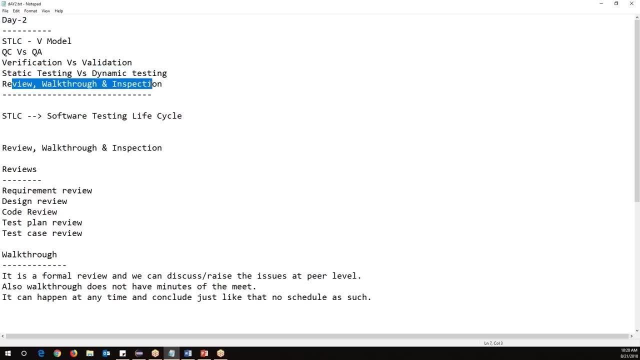 Fine, Okay, Okay, Okay. So now we have discussed about the verification, validation, static testing and dynamic testing, and review, walkthrough and inspection, and then we'll see about QA versus QA, QA and QC, and also we have a QA- QC, and also we have a QE versus QE- quality engineering. so let 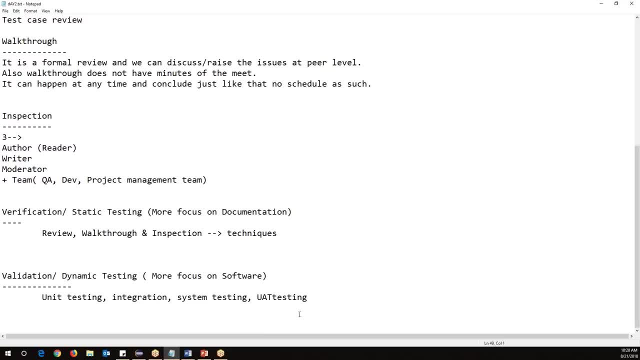 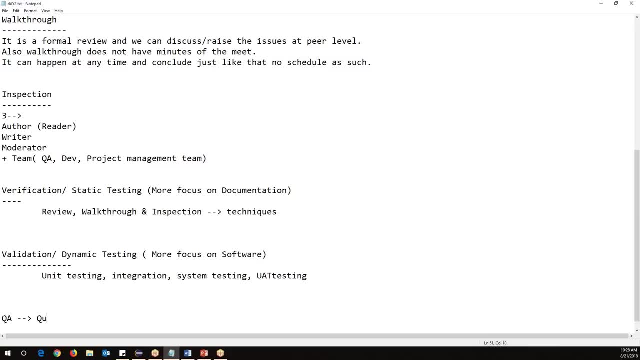 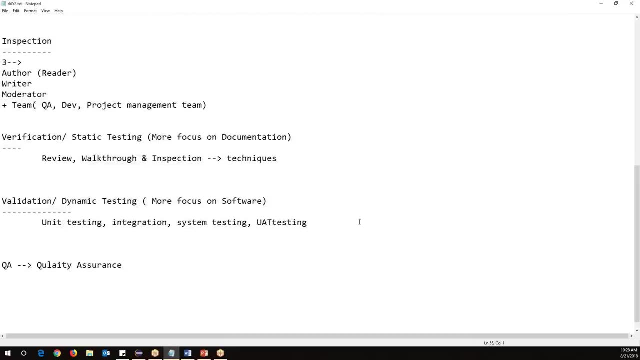 me just talk about these two. So normally testing team called as a QA team, in real time we call as a QA team. QA means quality assurance, quality assurance, quality assurance team and QA QC means quality control team. quality control and there is one more like: QE means quality engineering and QE means 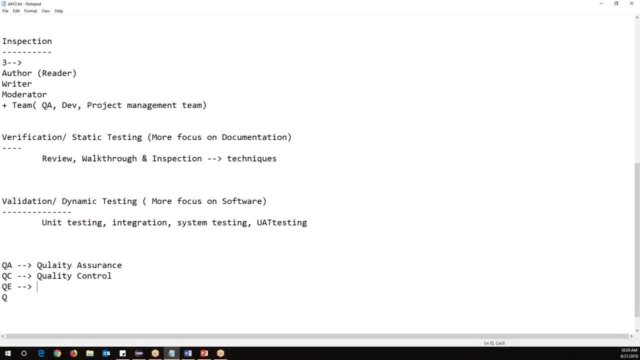 quality control, Okay, Quality engineering. So these are the three different words we commonly used when you're working in real time. QA means quality assurance, quality control, quality engineering. So let us understand these three words: quality assurance, quality control and QE. Okay, so here, first, let us talk about QA, quality assurance. 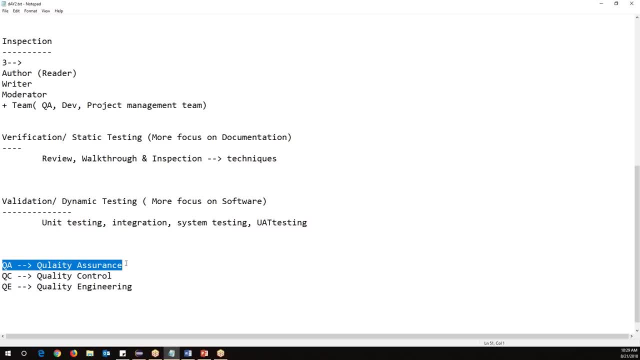 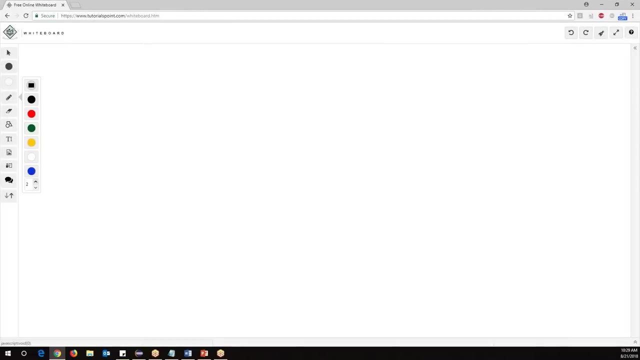 So quality assurance, So in short, QA, quality assurance basically is a process. Okay, so let me just give you an example just a moment. Okay, just yeah. so we have three things right: QC, QA and QE. QC is QA and QE- Okay. 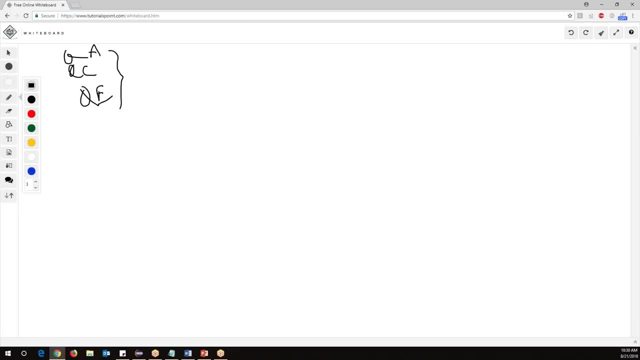 QA and QA quality assurance, a quality control and the quality engineering. so here, if you develop some software, we need all the steps like requirement analysis and design, and then we need to code the software and then testing and then our deployment or maintenance the software. these are the steps we 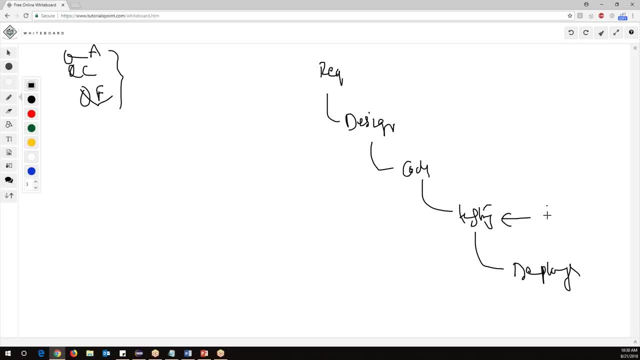 discussed. so this is your testing case. okay, this is your testing face. so now here in V model, we discussed review. don't write here. we model, if you observe here this time, is this part is verification and this part is validation we talked about. so both are testing. only right, verification is also. 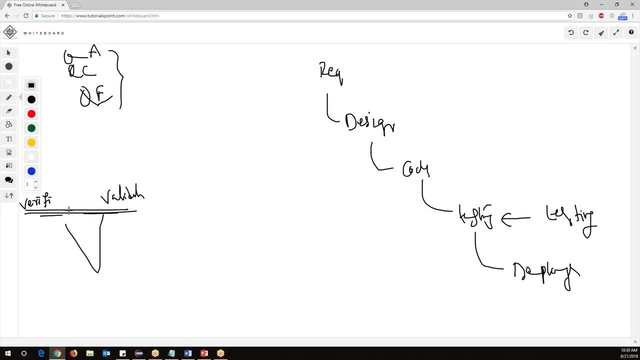 testing. meridian is also testing so, but the difference is verification is done on the documentation whereas the validation he's done on the software, that's the 漕 Lead from GBA output. only difference. but overall, this verification and validation or a testing techniques on right. so here, each and every phase, this is a normal SDLC process model in. 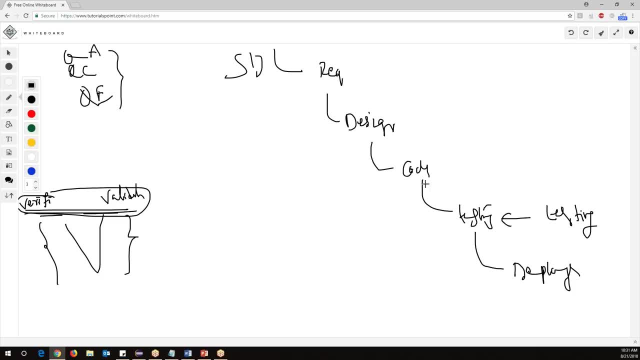 SDLC. once the requirement- design, coding- is completed, then testing will start and then deployment. so testing people should wait till all the previous phases are completed. so that's the main issue with the SDLC process models. okay, but in the V model what happens is in each and every way there is a kind of testing. 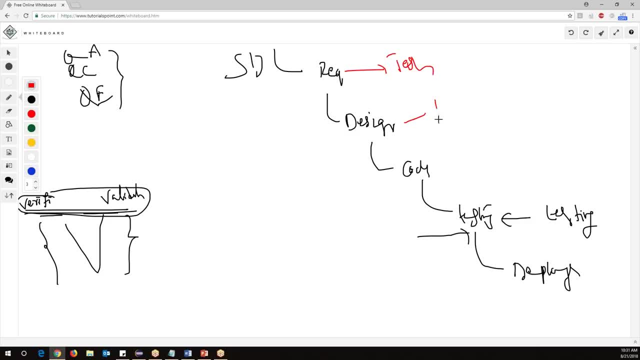 so industry, in the requirement we have a testing. the design phase we have a testing. the coding phase, we have a testing testing phase. we have a testing. in the deployment phase also we have a test. so this is a latest. we modal and agile model. every phase we do set a kind of testing. so for example here: 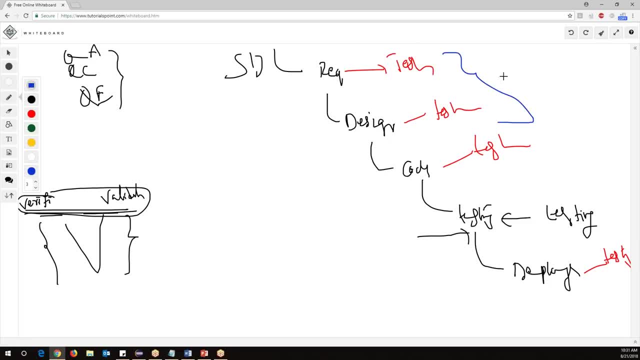 requirement, face and design phase. we do testing. what is the kind of testing? V to verification, we are doing right. so reviewing the documentation, that is also a testing. and in the coding to lay on��서, we are doing testing and we ומodernization will come as a modification of the testing in order to 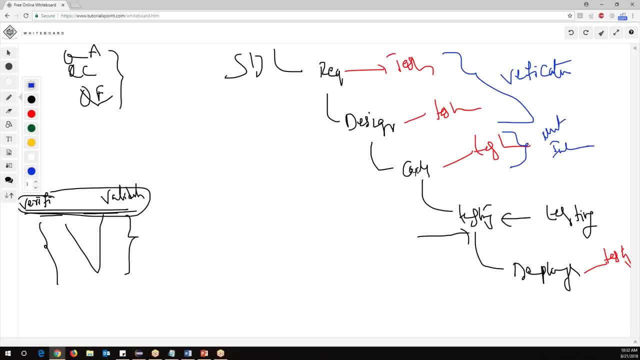 so in the coding our layout should be also done by design testing. so the we do unit testing and integration testing also. we are doing during coding part and then testing phase. we do system testing and deployment stage. they do uat testing. so in the new models every. 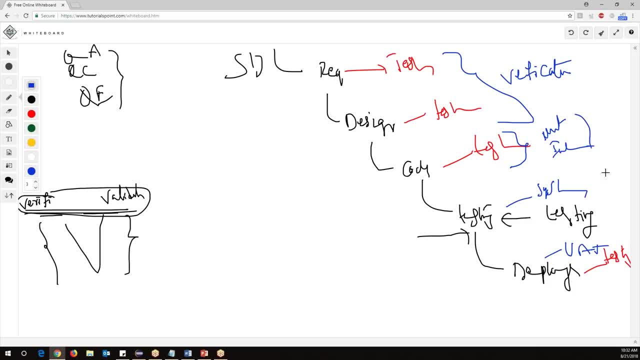 phase, every phase, we do testing. so unit testing, integration, these are all comes under the validation again. okay, so in each and every phase we are doing certain level of testing. so what is an advantage of this? if you are done already, testing in the previous phases, there is less. 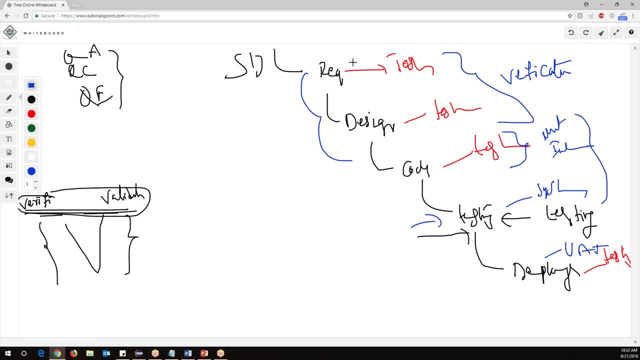 chances to get an issues in the testing phase. suppose, if you don't do any testing in the previous phases. if you found any defects in the testing phase, again we need to go back and change the code accordingly. design: we need to change according to requirement: we need to again. 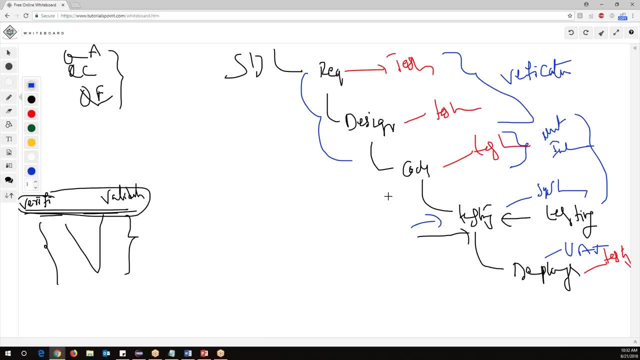 re-verify. so this is again repeated process. so to reduce that, every phase we have certain kind of testing. so that is a mainly htlc process. okay, so here quality assurance means this is talking about the complete process, complete software development process. qa is a process oriented or process related. 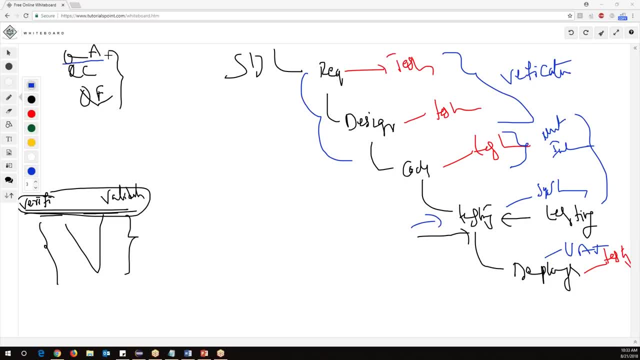 okay, and qc is a actual testing of the software. so qa will involve entire thing and each and every phase we do certain testing. that's all comes on the qa and qc mainly focusing on testing part. it is validating the software by providing different kinds of inputs and capturing the outputs whether it is working according to customer. 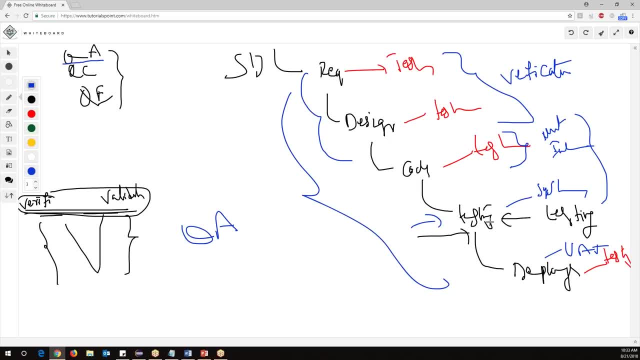 requirements or not. so that will be taken care by the qc quality control. so qa is a process related, qc is a testing part, actual testing of the software. so qc is purely related to the testing, whereas qa is related to the complete process. okay, there is a one difference now. 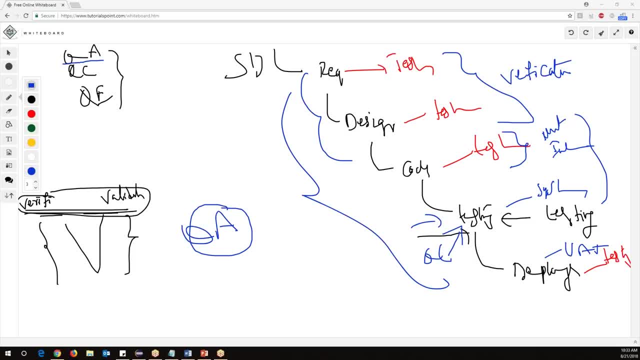 qa is for building the quality. so why qa is required? because to build the quality. so they will define the process, will define the process and the QC will implement the process. so QA will define the process. okay, you have to do like. this process means this one: designing. 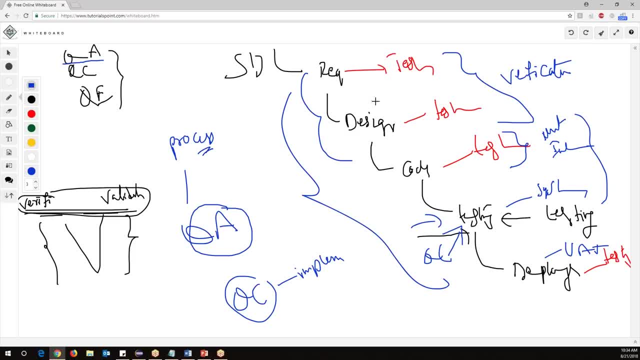 requirement design, coding, testing. this is a process and each and every step. what are the different activities we have to do so that all comes under the process? so, like during requirement phase, what are the activities we do? we get the requirements from the customer, creating the SRS document, reviewing the SRS. 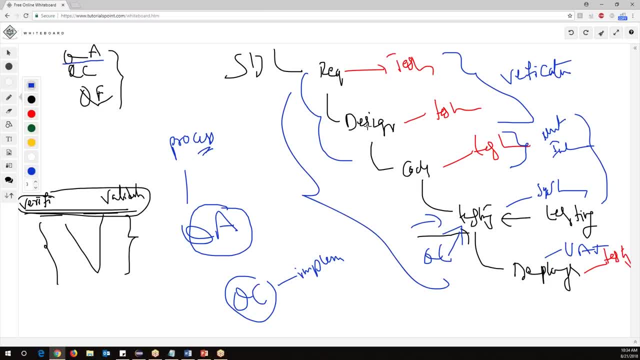 document, which are all comes under the requirement part. so what are the activities we do in the design part? we understand the requirements, will create the LED documents, create the HLD document. these are all activities done during design phase. in the coding phase they have to write the code. they perform. 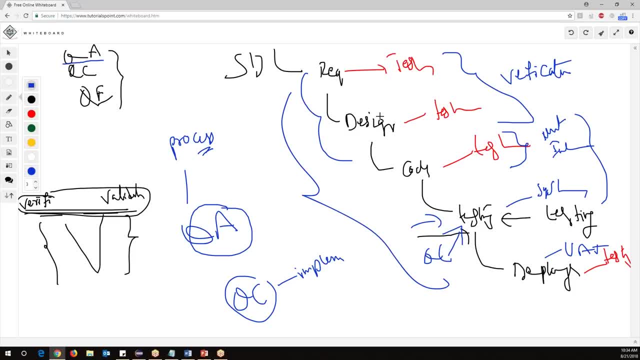 unit testing. right, they all comes under coding phase, like that, each and every phase, what are all different activities we have to perform? so that is comes under the process. so the QA will define the process like what is the process, and the process will define the process like what are the. 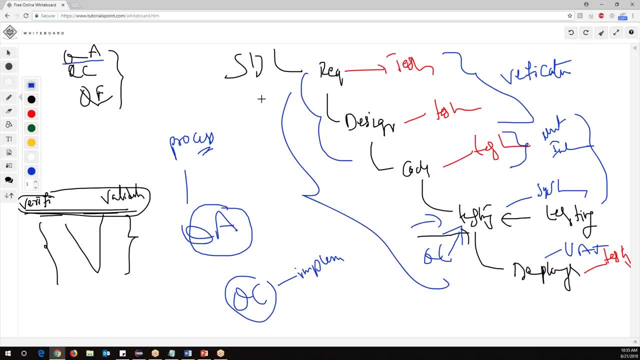 what is the process we have to follow? okay, so if you want to develop the quality product to the customer, what is the process, what is the strategy we should follow? so that is defined by the qa team, quality assurance team, but who will pro? who will follow that process? qc will follow the process. 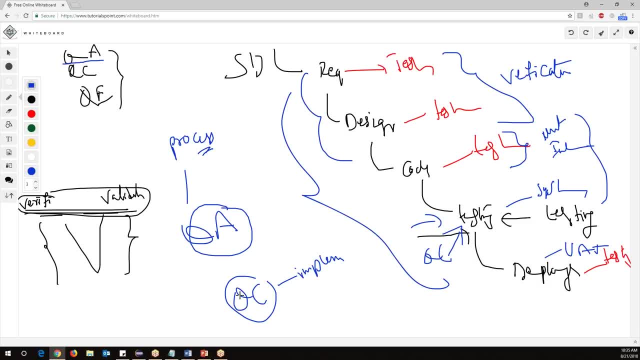 quality control is the team who are responsible: follow the process. okay, so one is a qa is define the process, whereas qc is a pro: implement the process. they will follow the process. so qa is focused on, completely on process. whether qc is follow the process most more lead uh focusing on. 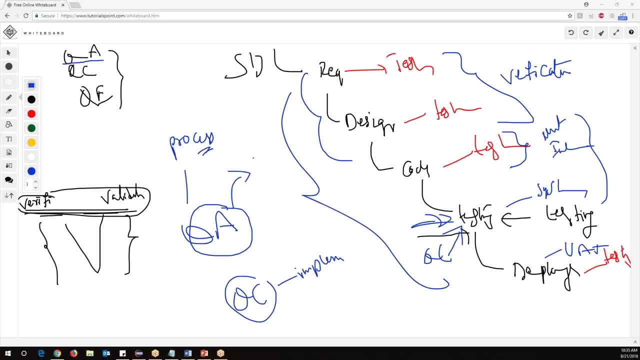 testing part, that is, the qc, and qa is for preventing the defects. why qa is there? because prevention of defects. in future, if you don't want to get any defects, we need to carefully test each and every phase. so who will take care of this qa? so qe is? 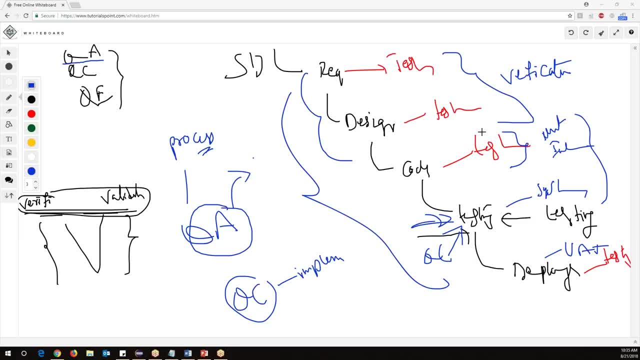 a prevention activity. we say qa is a prevention activity. in future i am not going to get any error. so that kind of assurance the qa will give you prevention activity. but whereas qc is a detection activity. detection means identifying the defects but already build or software is already having some defects and we are trying to finding those defects. so qa is prevention activity. 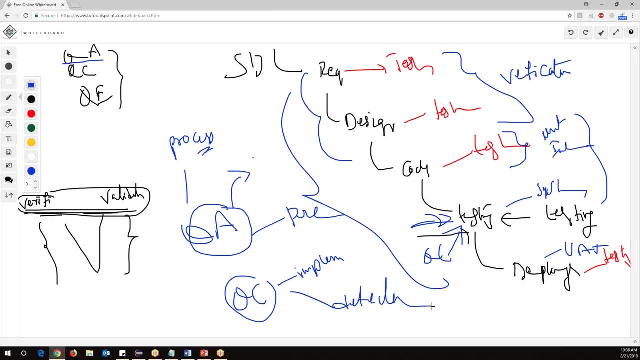 whereas qc is a detection activity. detection means we need to find the defects. there is a lot of difference, okay, so qa is process oriented, qc is the testing activity. qa will define the process, qc will implement the process. qe is for qa is for prevention activity, qc is for detection of defects. 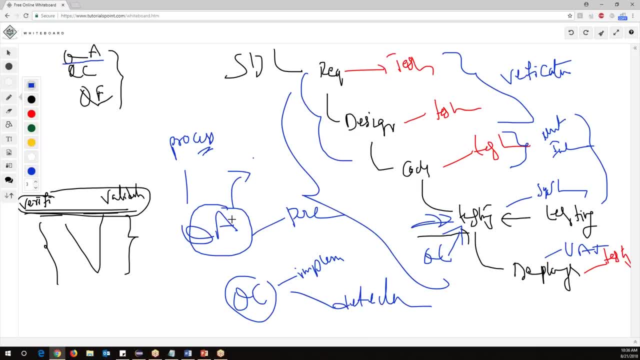 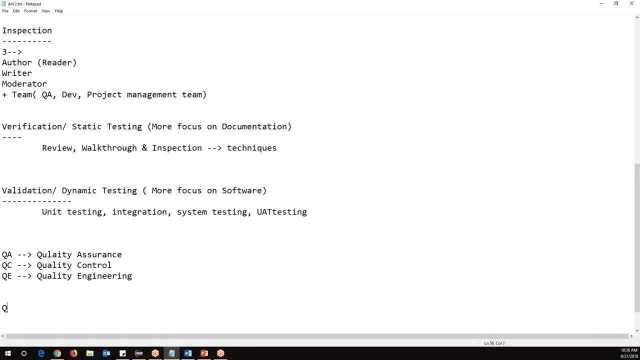 but qa is prevention of defects- okay, and qa involved throughout the development process, but qac involved only during the testing process. so that's the difference between qa and qc. so let me just write a few things here. qa is a process oriented- okay, and whereas qc. qc is a actual testing software, okay. there's one difference: the 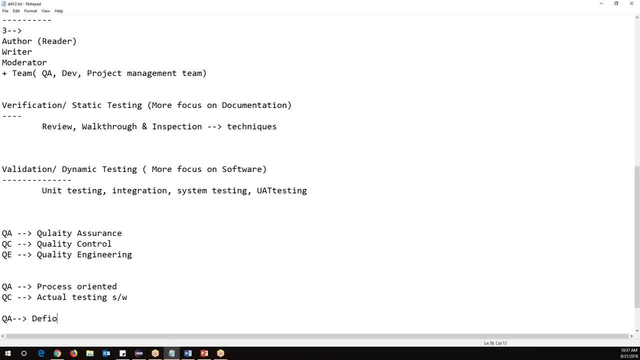 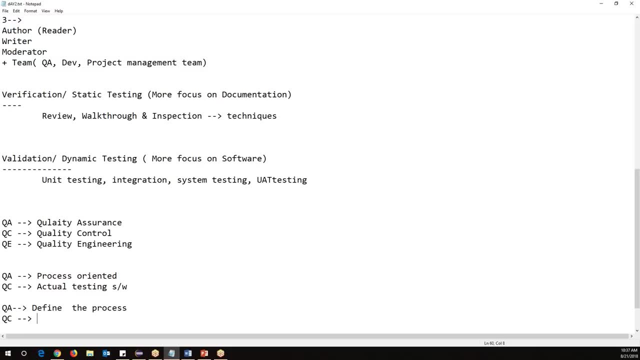 other difference is: qa will define the process, define the process, but the qc will follow or implement the process because they are the actual, actual activation. will do so: follow the process, follow the process or implement the process. somebody should be there to implement the process, only the definition. define the process itself doesn't work right, so they will just do the. 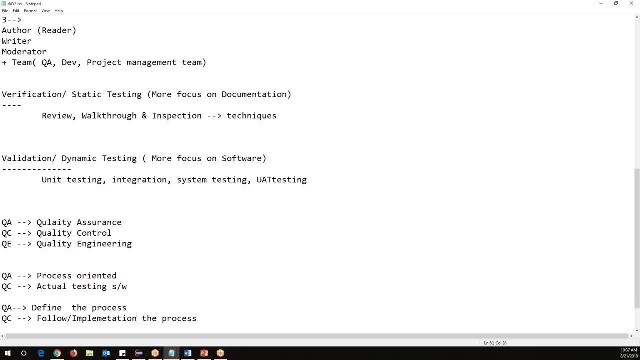 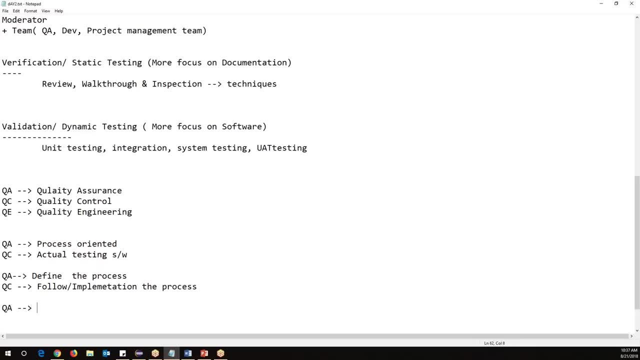 planning activity. so whatever people are responsible for implement that plan comes into the queues follow or implementation of the process and the other defect qc. qa is why they have defined this process, because in future we should not get any defects. that's the kind of prevention activity, so qa. 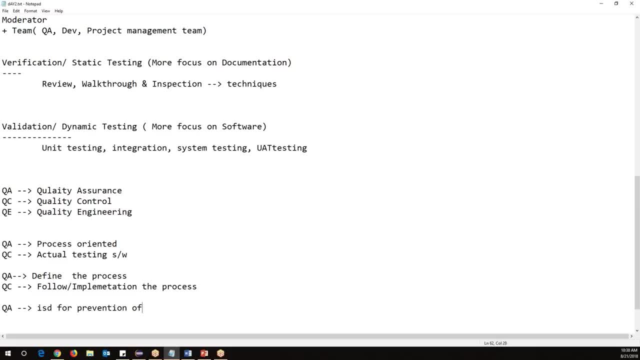 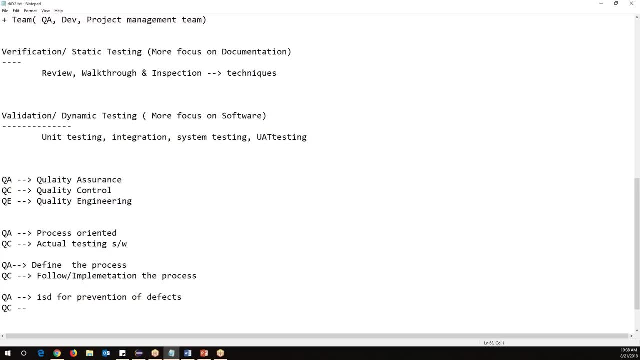 is for prevention- prevention of defects. but even if you do certain kind of prevention, still there is a chance to get an error. so we will identify those issues. qc is a for detection activity. detection activity, this is the prevention of defect. this is called prevent prevention activity, whereas qc is detection activity. okay, so this is about the major differences between qa and qc. qa is 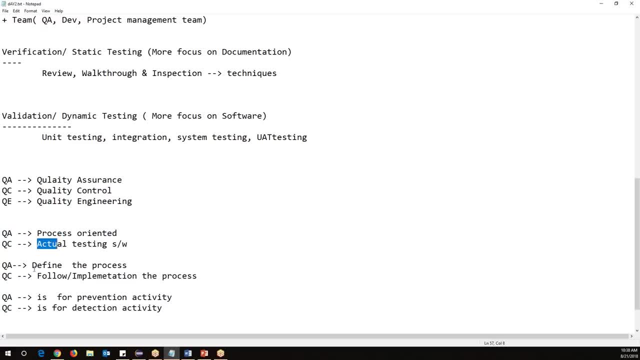 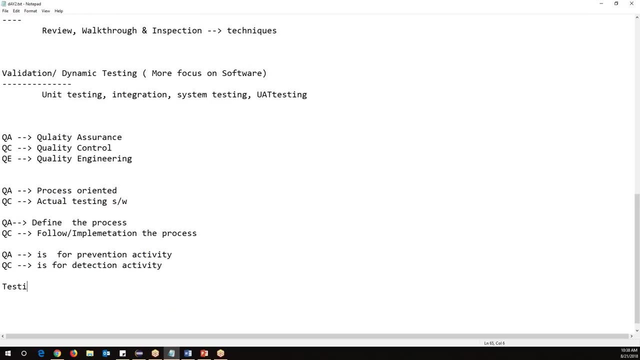 process oriented. qc is actual testing. the software. qa is defining the process. qc will follow or implement the process. qa is for prevention activity and qa is for detection activity. okay, now you can tell whatever testers, team, testers, teams- comes under which category. now all the testers comes under which category, qa or qc. so these are all comes under the qc. 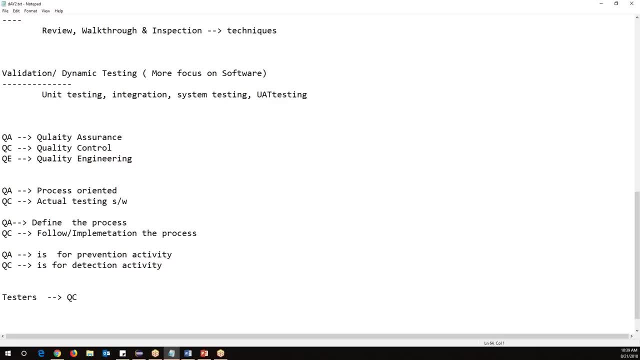 qc means quality control qc team, but other management team like test manager, product managers. they will define the process, they will manage the process, but they don't do actual testing. right, so they are comes under the QA. so all the test managers, right, like project managers, okay, and then product managers, product managers or leaves, so over is. 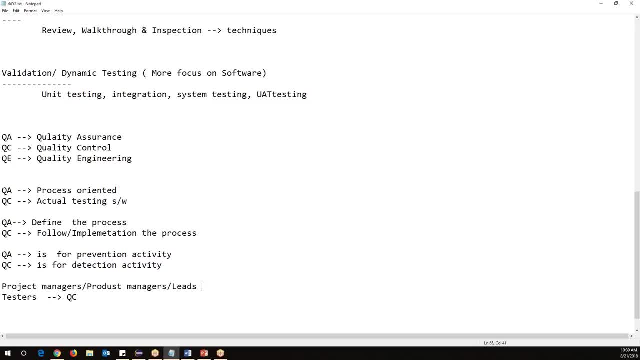 not participating during testing. they are all comes under the which kind of what's category? QC team, because they are driving the teams, but they don't involve during the testing. so what is involved during testing? we're doing the actual testing- manual or automation- and all will comes under the testers. so 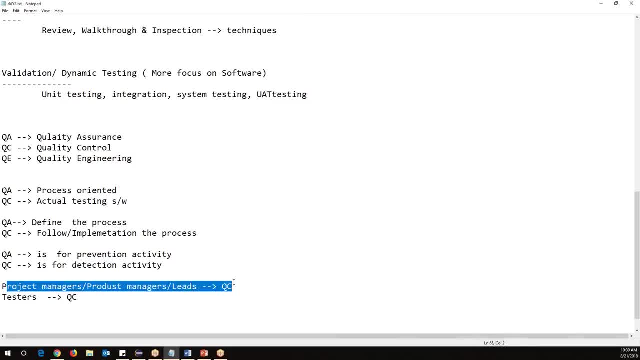 actual testers are comes from the quality control and rest of them comes under the QC quality control. okay, so is it clear so far. what is the differences between QA and QC? so, but normally in the companies, people are called as a combined with a QA team or QC team. okay now. so once we understand QA and QC. 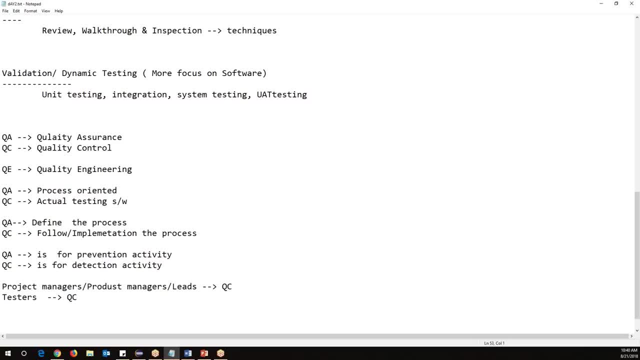 there is another one called as a QE- quality engineering. so this world recently become a very popular because in you, while you are searching for jobs in, out there or some other websites also, people are asking: like QE's quality engineers, okay, so even project manager also, all managers comes under here, all project managers- product. 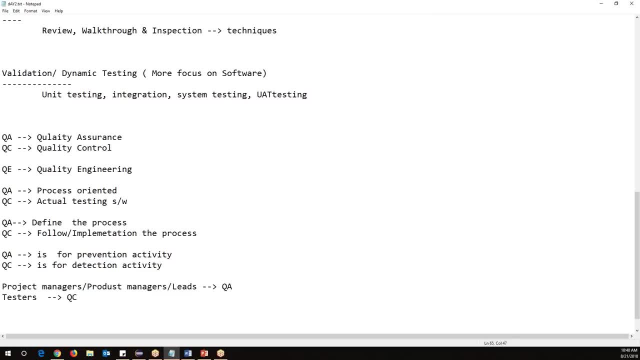 everybody comes and sorry, this is QA. okay. project managers like a product manager: yes. whoever is not participating in testing, okay, they are. comes under the QA parks because they are the driving, the teams. they will define the process, they do the planning. so all people. or comes another QA quality assurance team: okay. 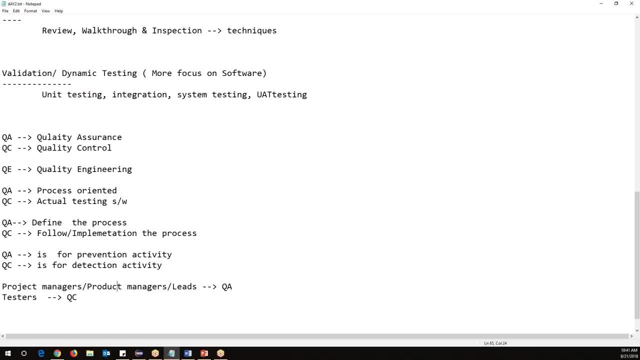 and testers are actual tester. so they will implement the process. they do testing, they will write test cases, they will execute test cases, they will report the defects. so actual implementation is done by the testers. but how we need to get the software from the developer, how we need to write there. 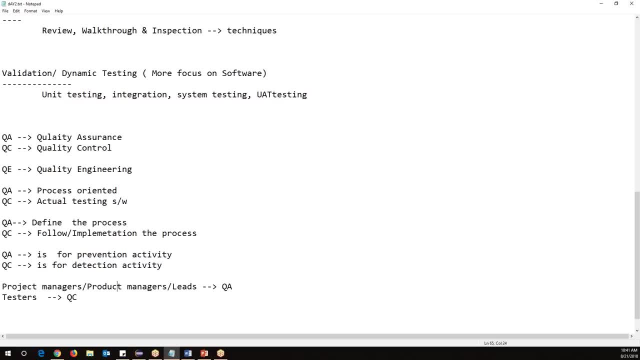 How we need to, how many cycles we have to run the test cases. okay, So, and when we need to perform some testing, when we need to perform sanity, when we need to perform function testing, Timelines, schedules, who will define all these things by the QA team managers will define this. 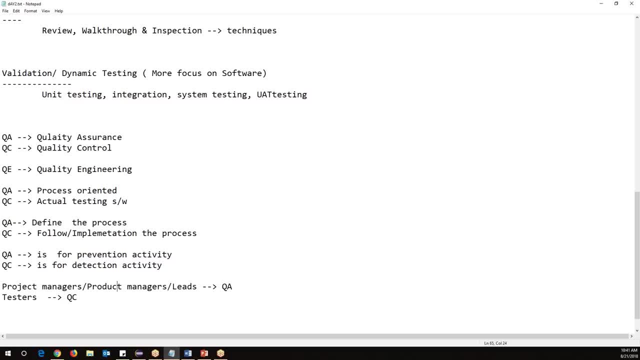 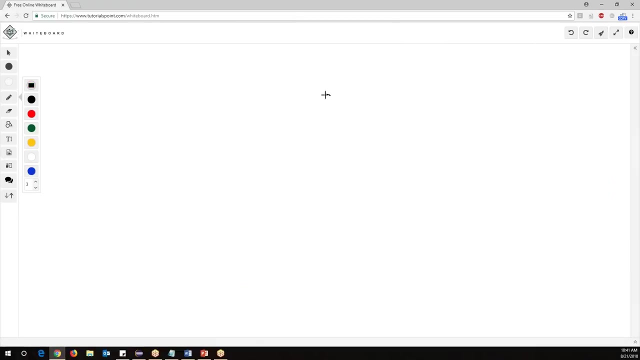 Right, So they are all comes under the QA and QCT. Now let's discuss about QE, quality assurance, So quality engineering team. so this become this. QE is become very popular whenever, whenever the automation Came into the market. So now here, observe this carefully. So what is the main job of developer is to develop the software, right? So let's say: this is our software. 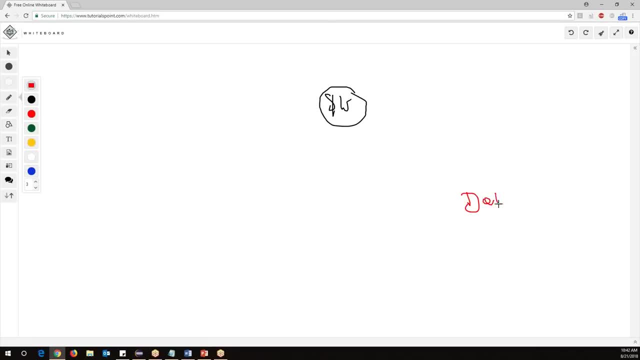 so Develop. what is a developer role? to develop the software is he will write Different type of programs to develop the software. So he will. the main activity of the developer is he will develop the software and to develop the software He will write the code. He will write code by using some programming. 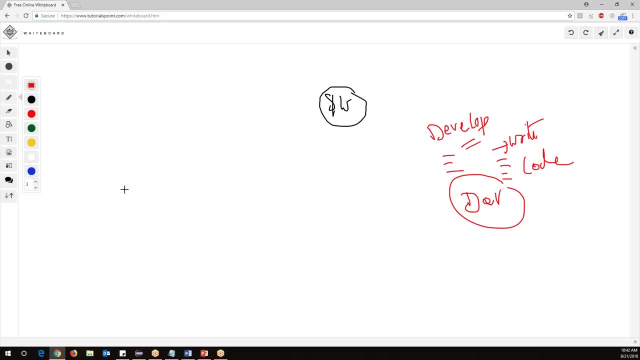 Either java, she shot, dot and whatever. okay, and here, what is the tester role? What the tester will do is, Even if it is a manual tester, he will write a test cases manually, will execute your test cases and reporting the defect. So these are all activities done by the testers. again, in testers There are two type of testers. one is a manual testers and 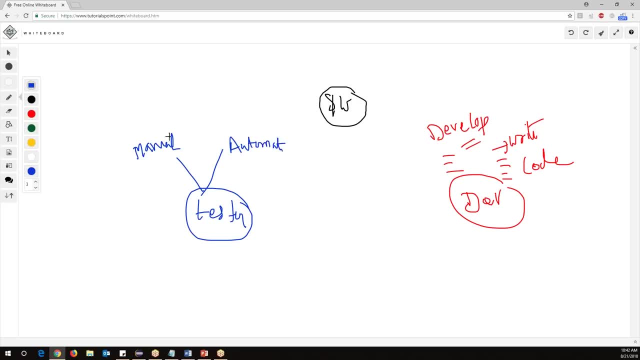 their automation testers. So manual testers job is: they will understand the requirements, They will write the test cases, test plans and they will execute test cases manually and reporting defects- all activities done by the manual testers, complete manual execution. Okay, they don't use any automation tools and they don't require any programming language. 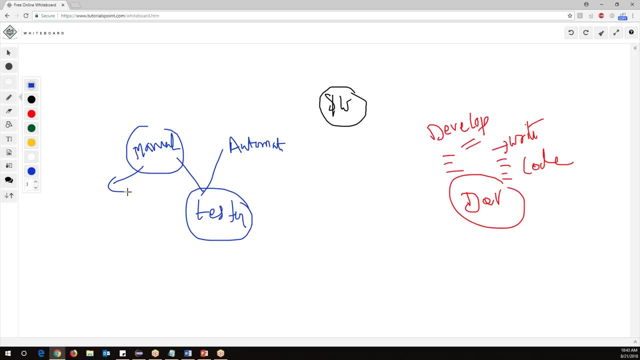 They don't need of any line, any knowledge on programming language. if, as a manual tester, Now come to the automation path- So there are automation testers also this: what the automation testers will do is whatever test cases they have written already, They will write an automation code for those test cases. 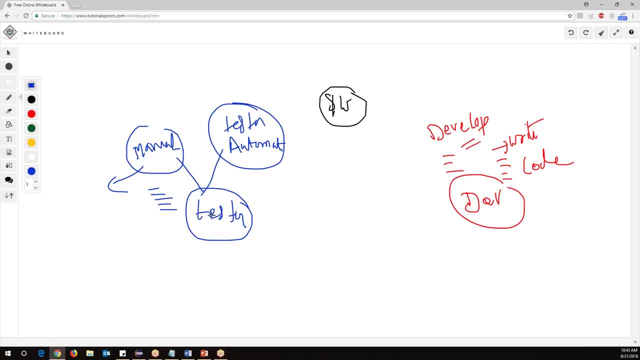 So they will automate these test cases. automation means they don't do anything manually, So everything will do by the script. So they will write some Java code and she sharp or Python code, automation code. We call, when I run, this particular automation code automatically just like a Java program. 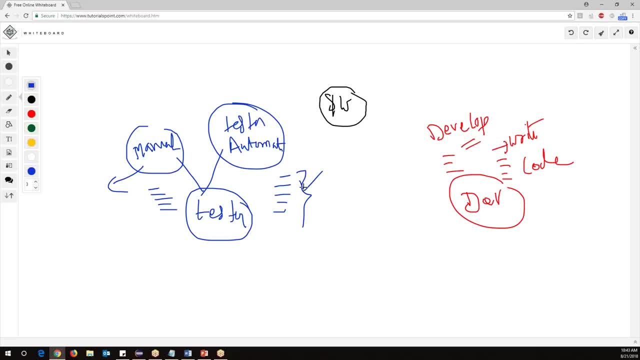 Okay, if I run the Java program, what happens? it will give you some output, It will take some input, It will give you some output. same thing: If you run your automation code, it will perform the same actions. Whatever actions we perform manually, the same actions are done by this particular automation tool on the application or software. 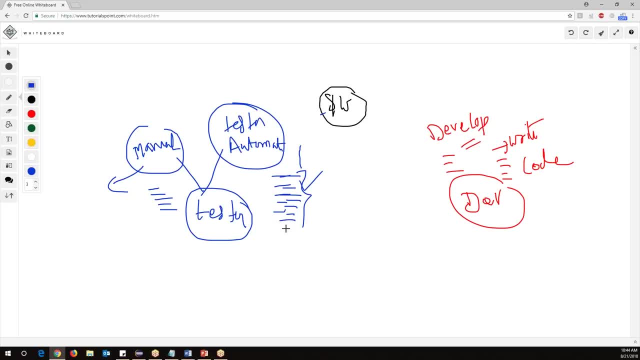 And this is also code. Okay, This is also script. We will write this code Automation tester. you have to implement. Okay, this is also kind of development, right, But while you are developing this particular code, to test the software. so the main activity here is testing. 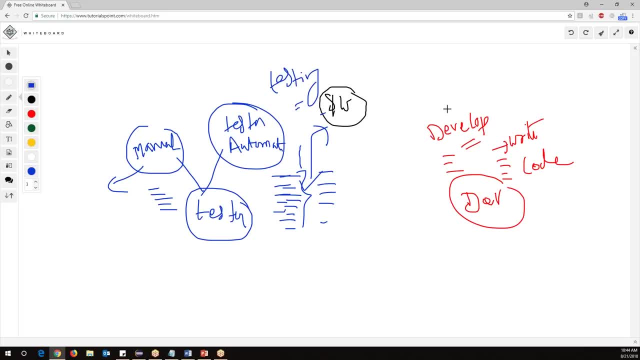 Testing the software. so developer is also writing the code to develop the software, But tester is also writing the code to test the software. So both are almost writing the code on it. almost Both are comes together. Okay, so that's the reason developers we call as a programmers or software engineers. So what is software engineer? 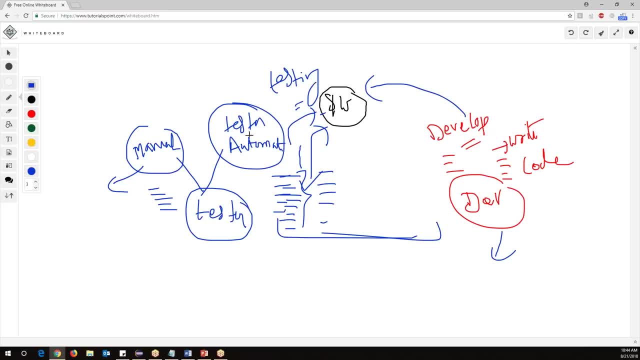 They are engineering the software Is, they are developing the software. So what is here? tester is also developing the software, developing the code to test the software. So here we call as a quality engineers. So quality engineer, so Q is terms come like that, So QE means quality engineers. all automation testers comes under the QE team. 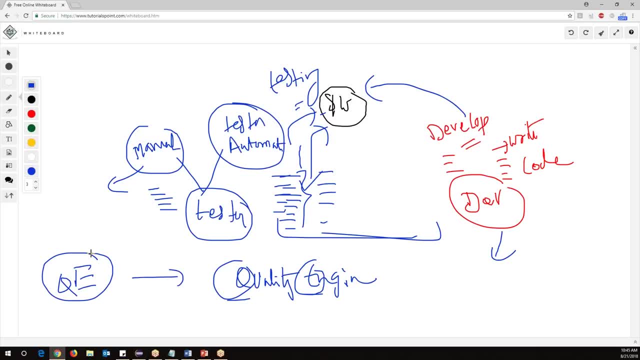 They do automation testing. they do automation testing. So here developers are writing the programs, developing the programs or Writing the program to develop the software, but whereas the automation testers also writing the code to test the software. So activity same, but the aspect is different. One is for development, The other one is testing. but writing the code is same. 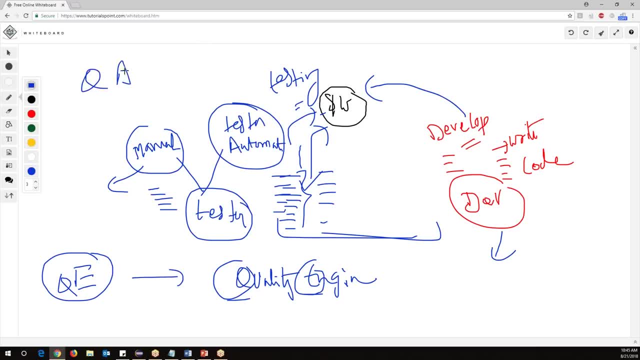 Okay, So now we have understood about QA, QC and the QE. so QA is related to the management related activity and QC is actually testing activity and QE is for automation- automation activity. Okay, so now it is clear What is QA, QC and QB. So these are the terms very popularly used on day-to-day basis in the companies. 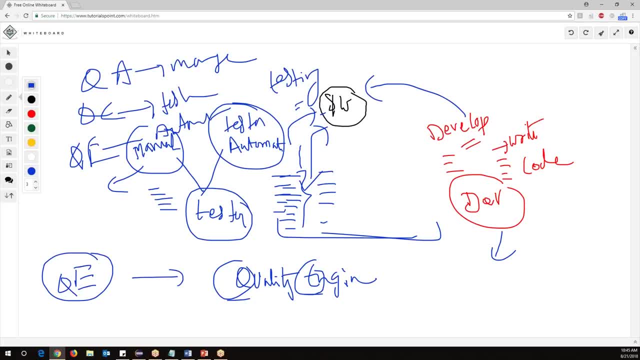 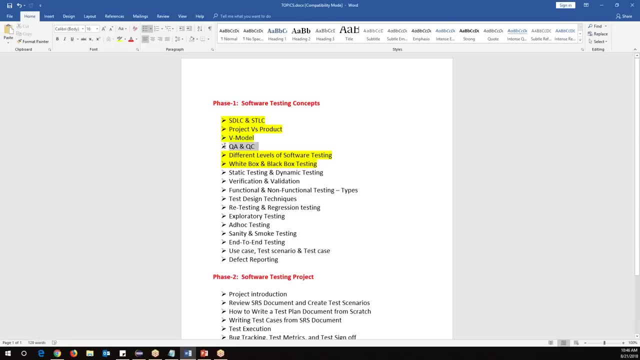 Okay. so before jumping into the testing, we need to understand these words clearly. Okay, so this is all about QA, QC and this one. So we have discussed about V model and then QA, QC and also QE, quality engineering and White box testing and black box and different levels of software testing. We already discussed unit testing. 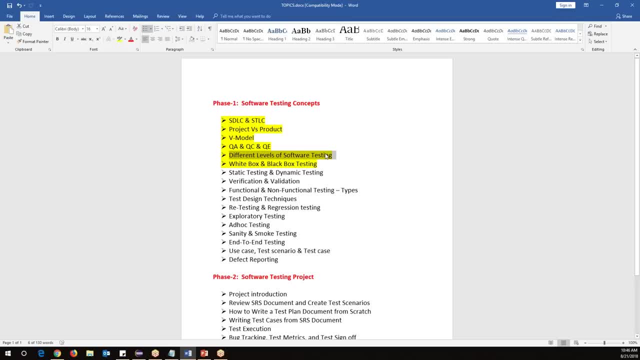 done on the program level and will do that. unit testing. developers will do the unit testing on the code and Integration testing and system testing and everything right now. Static testing and dynamic testing is also. we have discussed verification, validation is also discussed, And now let us Focus more on this one black box testing, because all testing team is comes under the black box, not on the white box. 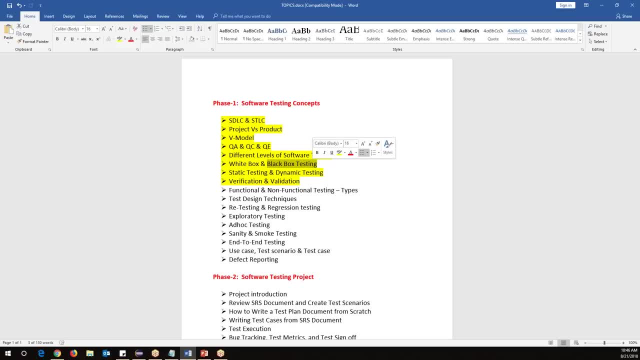 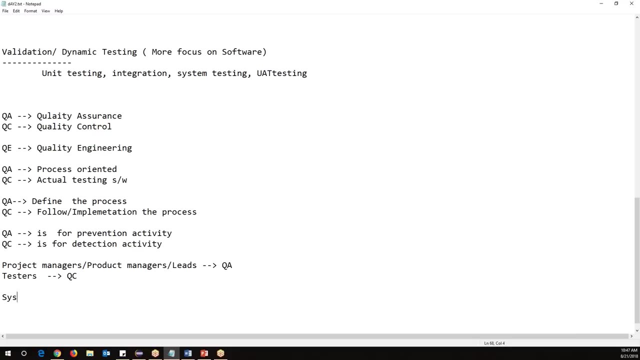 Okay, so it all comes under the black box, or manual testers, automation test engineers- Everybody will comes under the black box testers, not on the white box. Okay, so Let's focus on black box testing. This is also called a system testing. There's a main phase, right where we have been system testing. 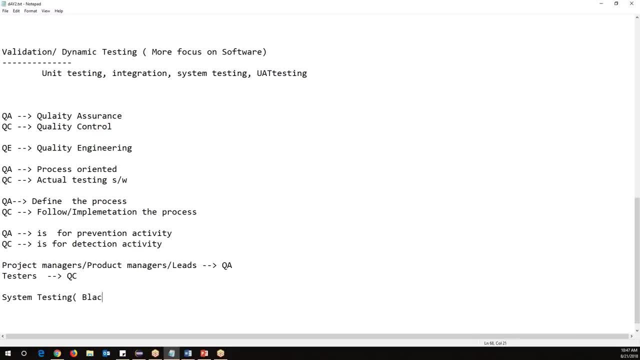 And what is system testing? This is a black box testing take Because we don't know what is the code the developer has written. So we call as a black box test, This time testing as a black box testing. Now. here actual tester will be involved. 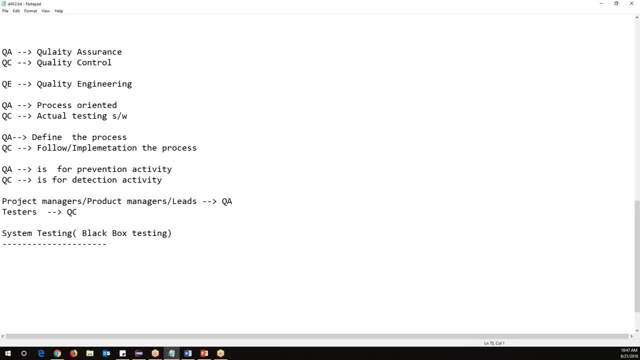 Action tester will be involved. So again here, some people will do manual testing, Some people will do automation testing, according to their skill set. Okay, so in that system, testing normally what manual tester will do is manual tester responsibilities are. They will understand the requirements first. 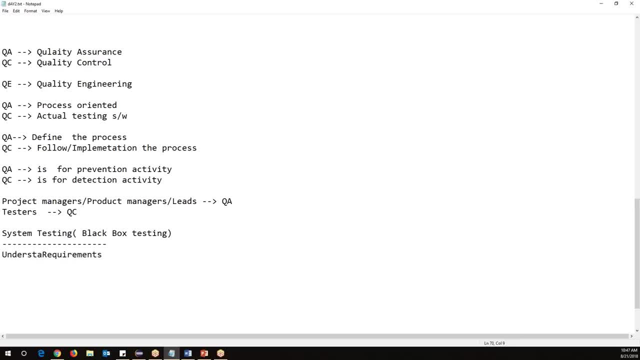 Understand the requirements clearly. that is first important activity. Okay, so how well we have understood the requirement is depends on the quality of your test cases. okay, so if you've well understood the requirement clearly, then you can create a good test cases and those test cases will able to find more number of. 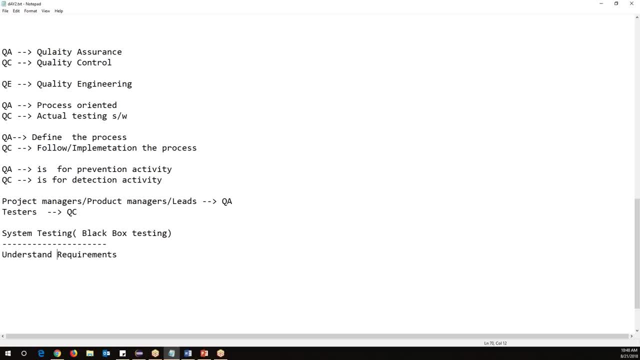 Defects. so that's the main job of testing here. We need to find more and more defects. So the base is we need to understand clearly requirements and then, once we have understand requirement, We need to write our test cases. So test case in the means, the test step by step action. 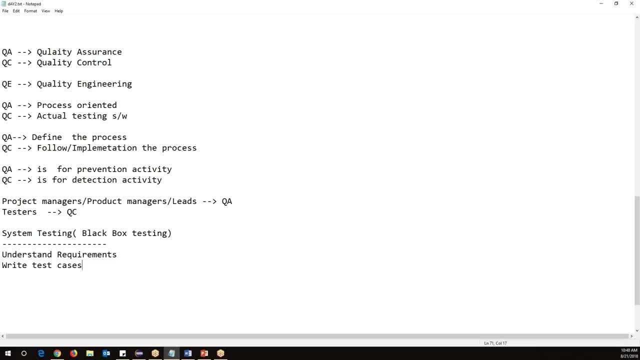 We need to perform on the application and you need to also verify what is expected output and what is the actual. The behavior of the application we need to verify according to the customer requirement. So we'll write a writing test cases and then we will Execute those test cases and we need to find the defects. 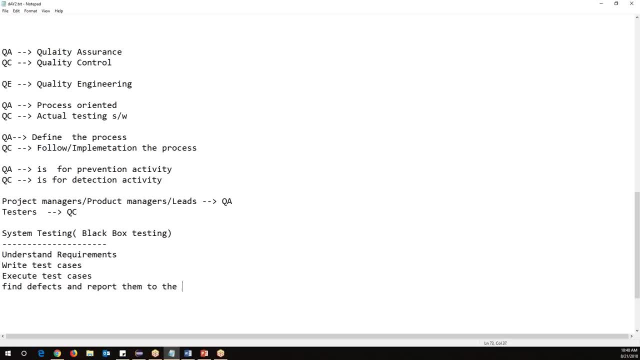 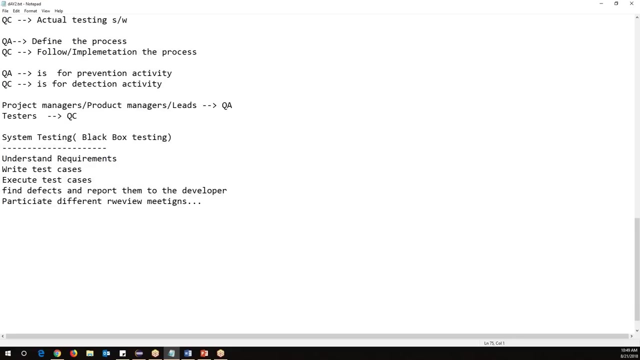 Find defects and report them. Record them to the developer. Okay, we put them to the developer. Okay. and again, we need to participate. Different review meetings, Review meetings and also these are other different activities- will be done by the test engineer. So if your automation tester, You need to also additionally do certain activities called writing automation code or automation scripts. 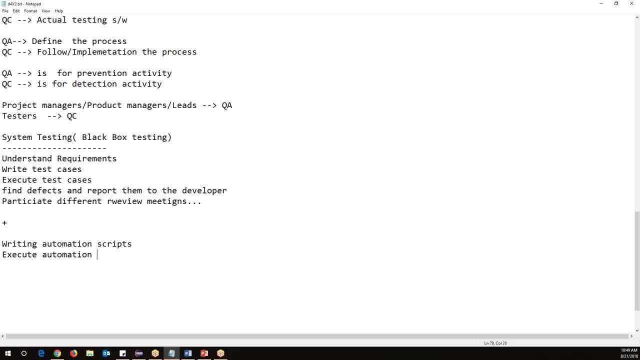 Okay, and then execute our automation scripts. Execute our automation scripts and then you need to also generate the reports. generate reports, Okay, and also need to prepare some status reports and then Send to management. So these are the different activities will be involved during system testing. 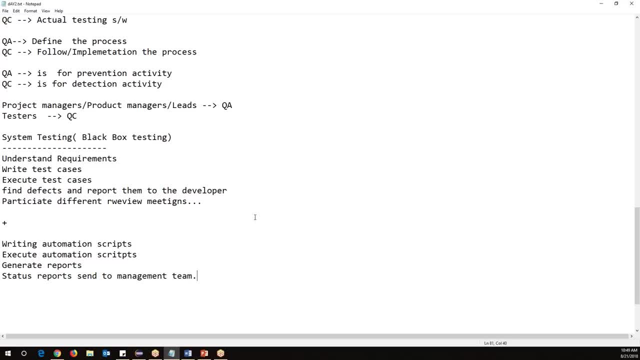 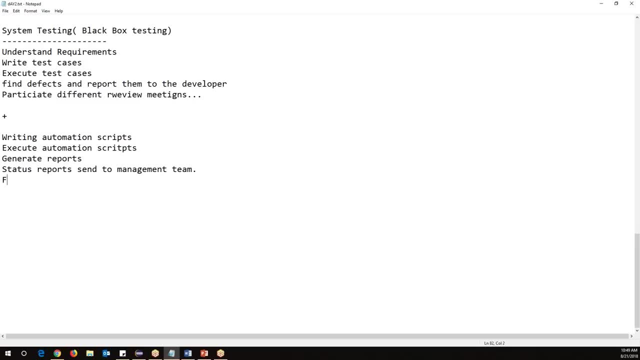 And as a test engineer, we do a lot of testings here, So different type of testings. So those testings will be again divided into two categories, like functional testings and non-functional testing, Functional testing and a non-functional testing. Functional testing and non-functional testing. 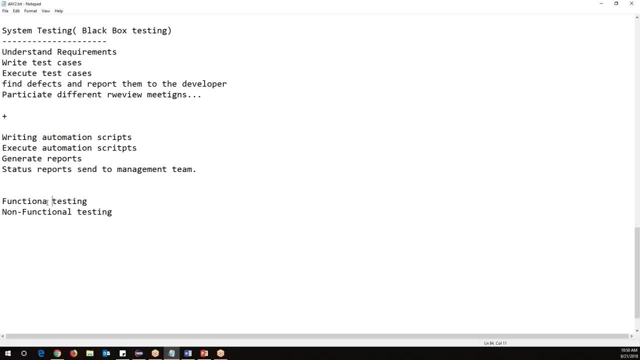 So system testing is divided into multiple categories. again, We need to perform a lot of testings like object properties testing, error handling, input domain cookies testing, links testing, Data based testing. these are all comes under the functional part and also non-functional, like performance testing, stress testing, load testing. 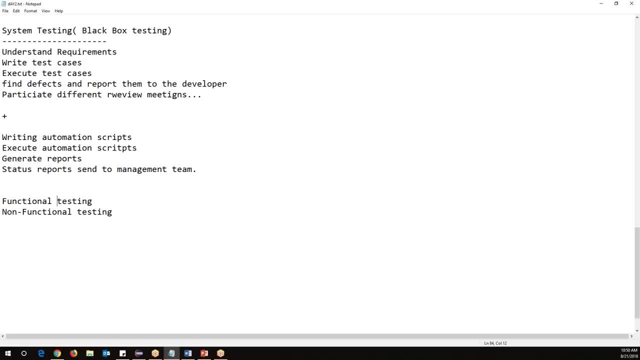 The recovery testing, security testing, all these comes under the non functional test. Okay, so, as a system testing, as a system tester, as a black box tester, We have to perform a lot of testings. Okay, it will take a lot of time to perform all those things. and before going to do these kinds of testing, 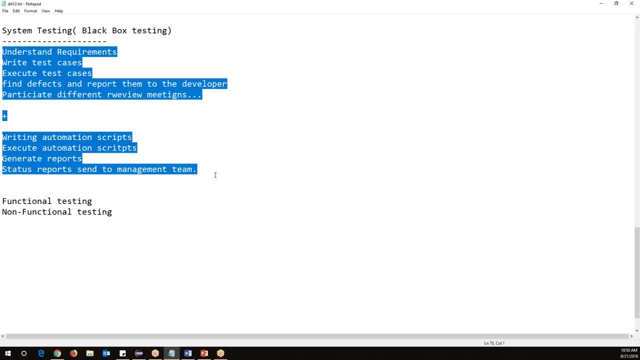 We should have proper documentation. So these are the different activities, activities we do before directly jump into the testing part. Okay, so we need to understand the requirement, We need to write our test cases, We need to execute those test cases. The main activity of the tester is to find the defects in the software. 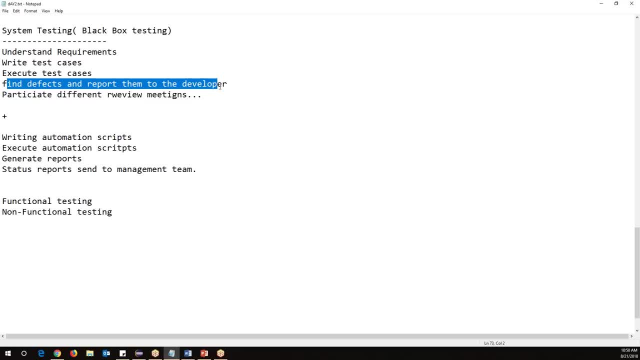 As soon as we found the defects, we need to report the developer and developer fix them And again we need to re-verify And if it is working fine, then we need to close the defects. So that's the main activity of the tester. 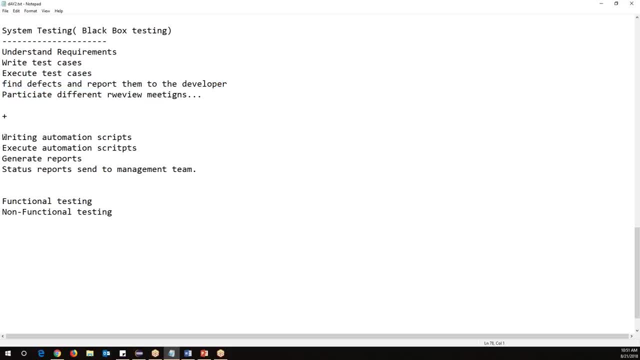 And if you're an automation tester, then only the job is: we need to write our automation script for manual test cases. You need to choose the test cases from manual test cases and then automate those test cases. Once we have automated those test cases, 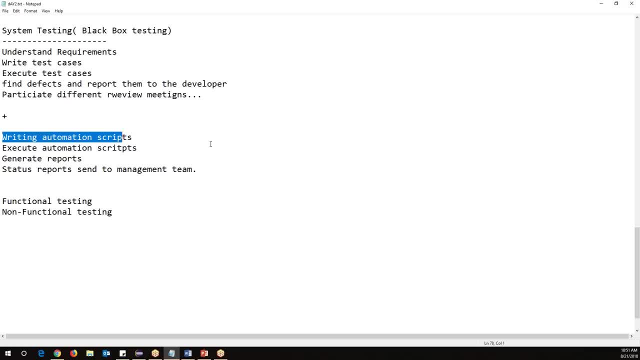 you can just execute the same test case again and again, multiple times or multiple builds. So that is all about automation activities. Now in the next session, I'm going to discuss in detail about functional and non-functional. So there are so many types of testings we do as part of functional and non-functional. 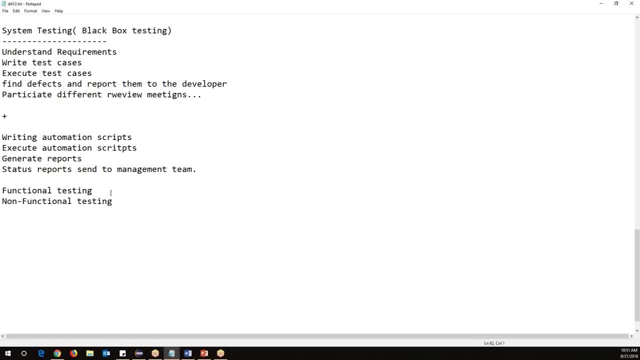 because why we need to know all these things? Because before directly jumping into the testing, what kind of testings I have to perform- you need to have some idea right. Suppose, if we give some application, okay, test it. How to test it. 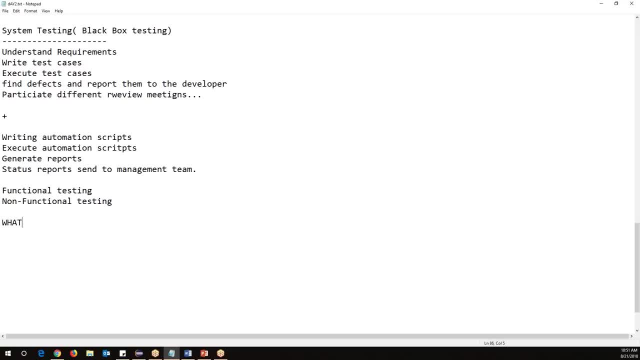 First, we need to know what to test. Okay. these are the two things we need to more focus on. First thing is: what to test? Okay. so if anybody gives an application, ask you to test that. So the two questions will be there in your mind. 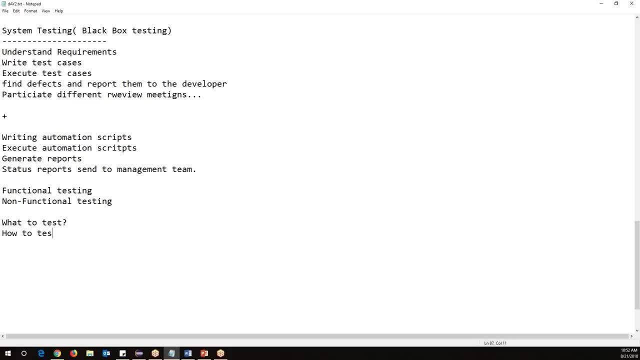 The first one is: what to test and then how to test. Okay, what to test, how to test. So what to test means we will discuss this in these two concepts: functional testing and non-functional testing. What are the different type of testings we do as part of functional? 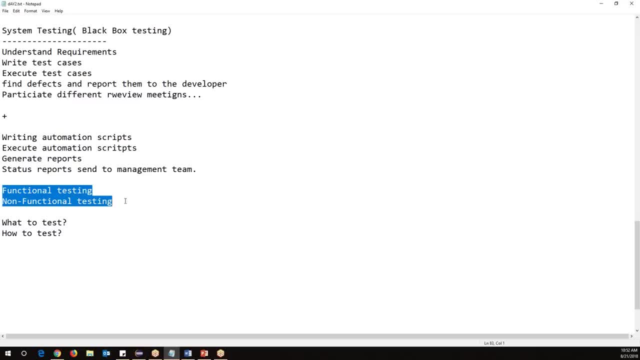 and what are the different type of testings we do as part of non-functional. So those testing types we will discuss in the next session. So they are comes under the what to test. So once we have clear on what to test, then we will discuss how to test. 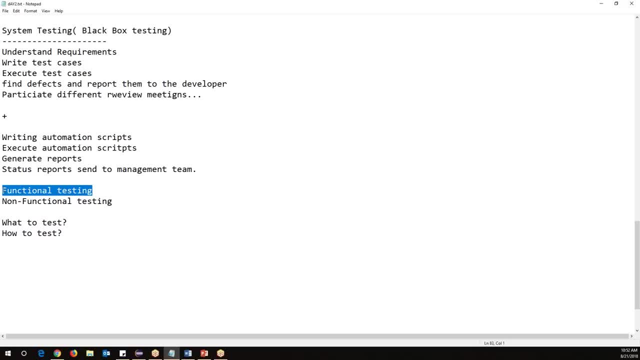 And hopefully we can transition them. Suppose there is a function testing called as an input domain testing, So one of the type of testing. So once we know about the testing, the next step is: how do we need to do that test, How we need to perform the input domain testing. 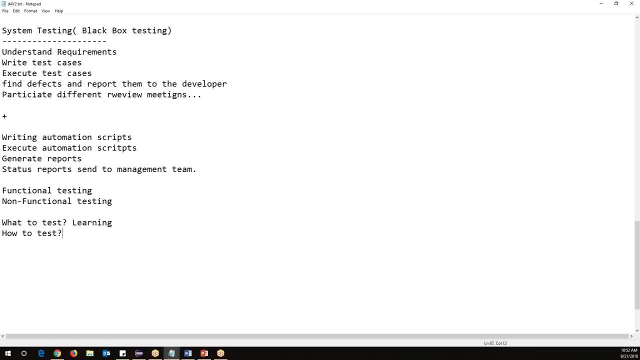 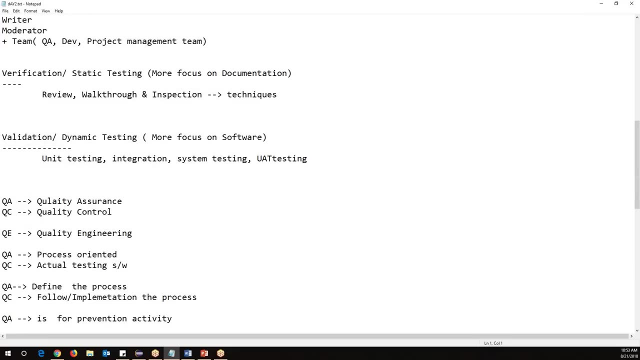 That's the next activity. So first, this is a theoretical learning purpose and once we learn what to test and then how to test, We need to do So. the next session we will discuss that one on functional testing and non-functional testing. so for today, just understand these concepts, okay. 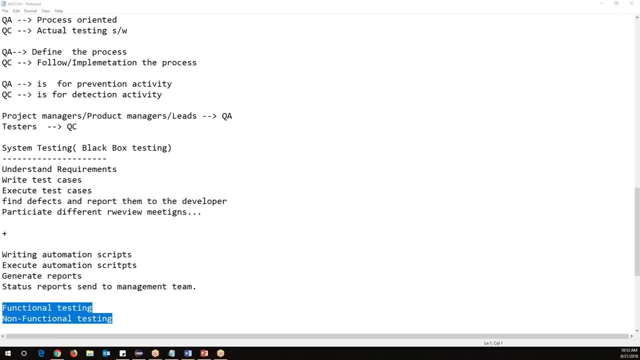 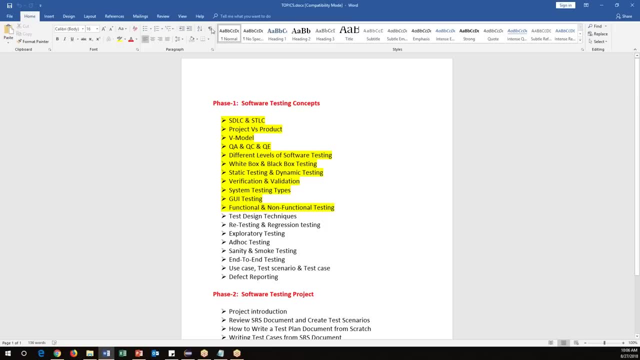 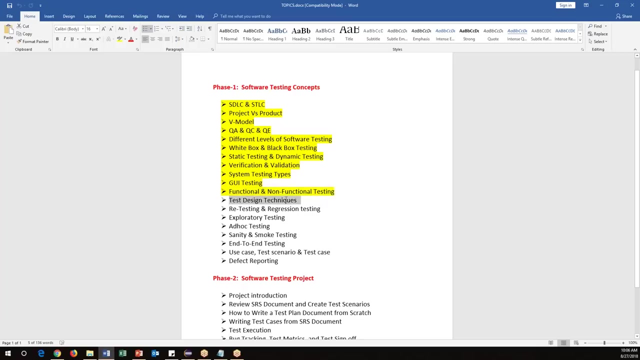 so i'll just stop today here and rest of the concept we'll discuss in the next section. right? so let's start today's session. so far we have discussed about a few items from the manual testing, so functional testing and non-functional testing- types we discussed, and today we will discuss about tested design techniques. so what are the different techniques? 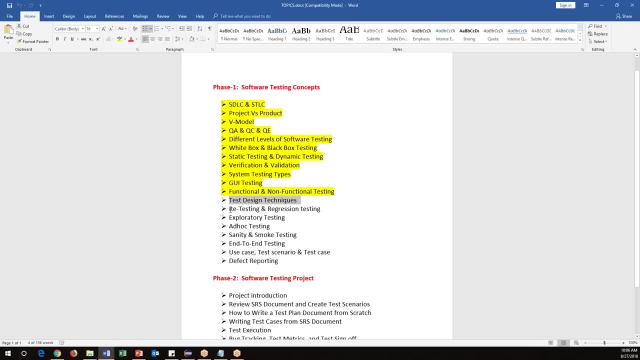 we use at the time of test designing and also we discuss about retesting, regression testing and exploratory testing, ad hoc testing, because these are the common technologies we use a day to day basis on the working environment. so before going to test an application, we need to understand. 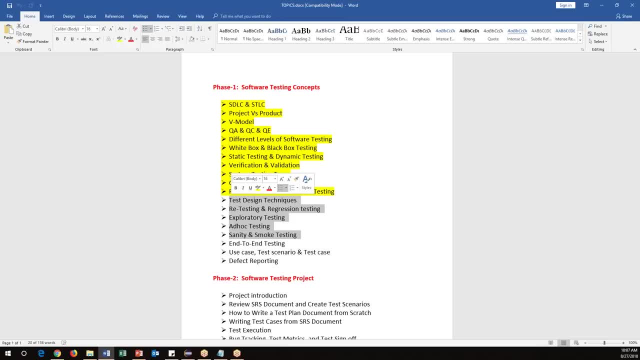 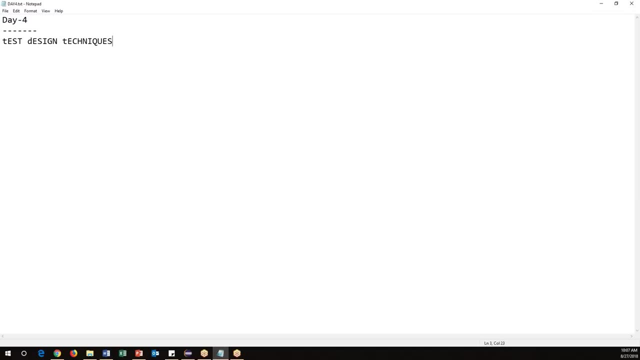 what are the different types of testings we have to conduct? so we need to aware of those type of testings. okay, so let us start with the test design techniques- very important concept. let me start writing some notes here: test design techniques. so in interview point of view also, these are very important. what are the test design techniques? you? 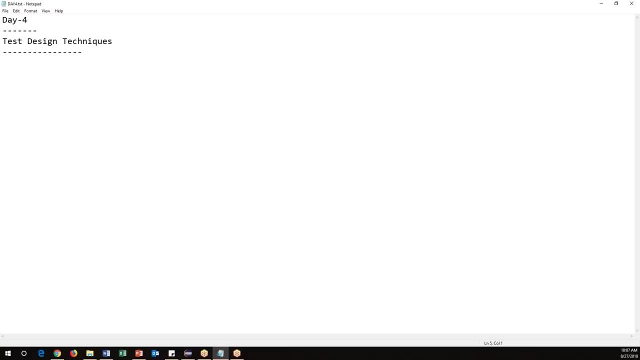 used at the time of writing your test cases. the main important role of test engineer is writing your test cases. so test case in the sense the step by step actions which we need to perform on the application. so, for example, if you want to test a login, so how? 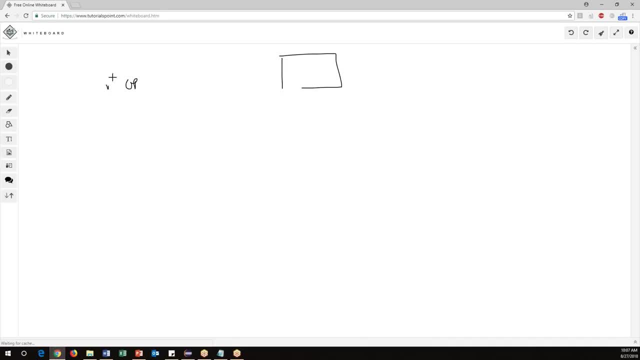 to write a test case for the login means. so we need to open the url, first step, and second step, enter username. third step, enter password. fourth step, click on submit and fifth step, and check whether home page is working or not. so these are the steps, the sequential manner we need to write. 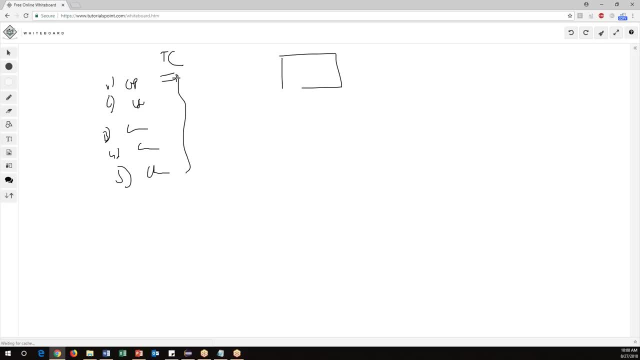 so this called as a test case. so the main job of test engineer is to writing the test cases. but at the time of writing the test cases- and a few scenarios and few areas- we need to use certain techniques to design the test data okay. so let me give you a small example here. so when we need to use these kind of techniques, 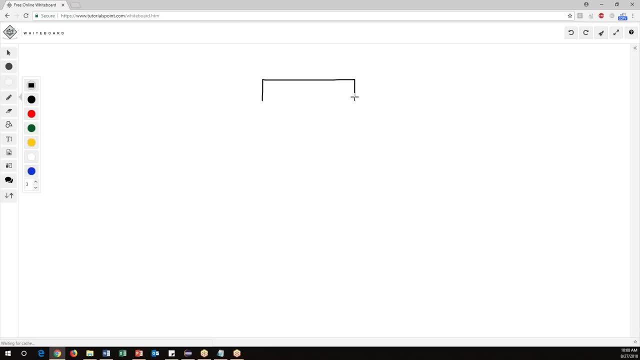 so, for example, i have a text field like this in the text field: okay, so i want to check whether this this text field, we need to enter the username. so, as per my requirement, i need to enter this username between minimum four characters and maxon eight characters. that's my requirement, and i can enter here only the lowercase letters. and from a. 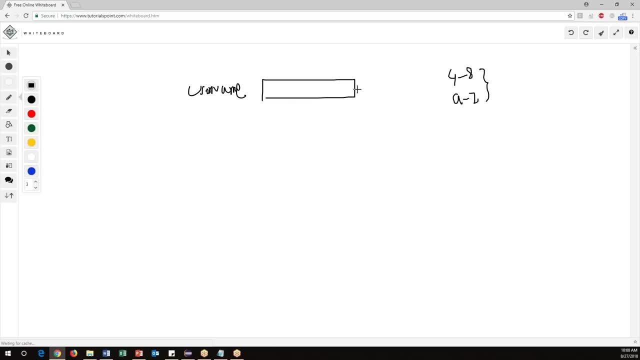 to z, so this is my requirement. so in this username text box i can add minimum four characters and maximum eight characters. this is called as a range and it accepts only a to z, so all are lowercase letters. okay, this is called as a value and, based on this requirement, i need to prepare the test data. 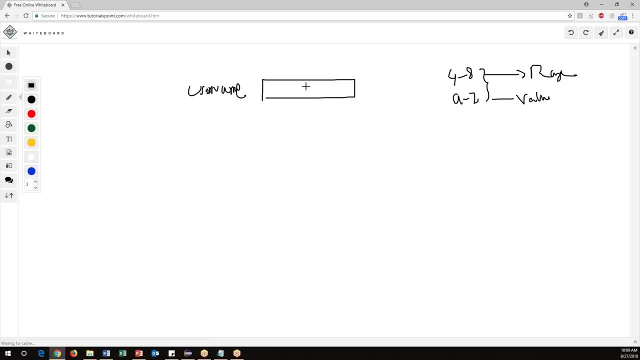 so, for example, i want to test this, so i want to test this kind of scenario. now, if you want to test this, how many kinds of inputs we require? normally means, suppose let's take a range here. range is four to eight, right? so if i test four, our test should pass, and if i test with eight characters, our test. 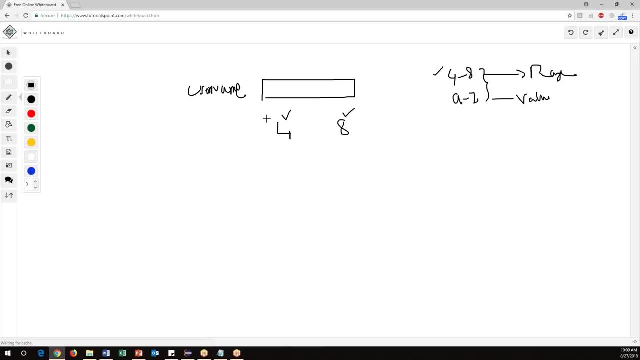 should pass and we need to also check invalid scenarios. suppose if i give a uh before uh, four, for example, when i give like this before four, one and so on. it will go on like this. and suppose, after eight, if i give like this, nine, ten and this: 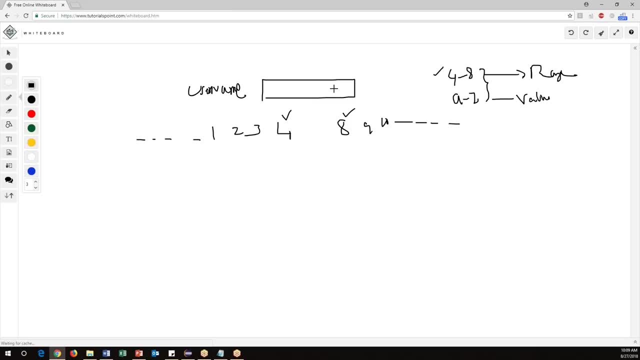 is infinite, right. so if you want to test this completely, we need to test with all kinds of inputs here and here and suppose if it is small, it is fine, suppose if it is a very lengthy. so we cannot test all kinds of input like this. but if i don't test all these things, our test cannot be. 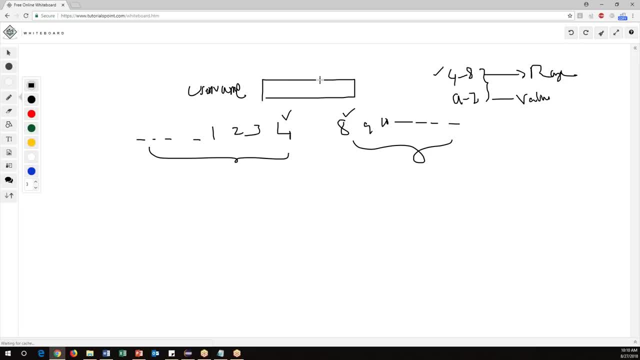 completed. okay, so what we need to do here is we need to reduce our test data. so we need to use minimal test data which will cover the complete test scenario- okay, complete application scenario. so in, that's how we need to prepare the test data, so to prepare that kind of test data. 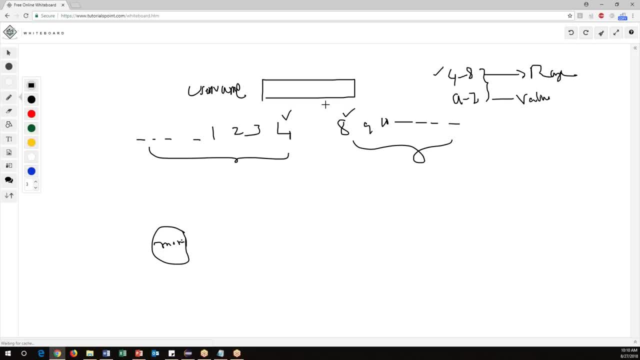 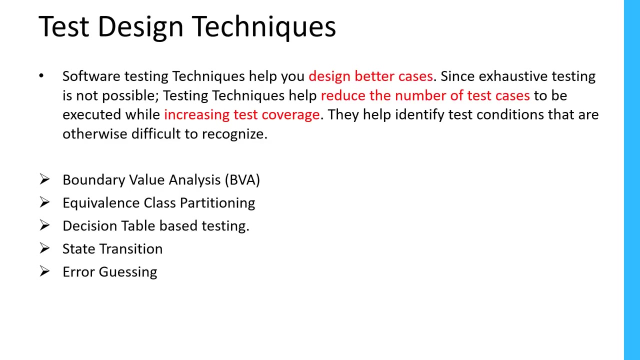 we need to follow certain techniques in testing. okay, now let us see what are the techniques we use during testing. let me just share a small presentation, okay, fine, so okay now let us discuss a few test design techniques. so why test design techniques are useful to reduce the test data, which will cover maximum coverage or maximum kind of testing. 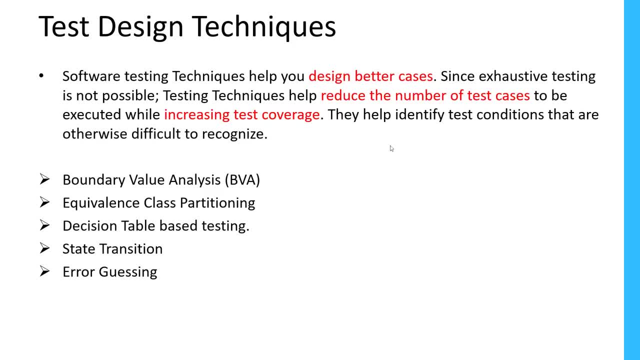 so the main intention of applying this testing Design techniques is we need to test completely. in should cover all the kind of scenarios with the minimal data. We cannot test with the huge data sets. It's a lengthy process and it's take a lot of time, So to reduce the data and it should cover each and everything, positive as well as negative aspect. 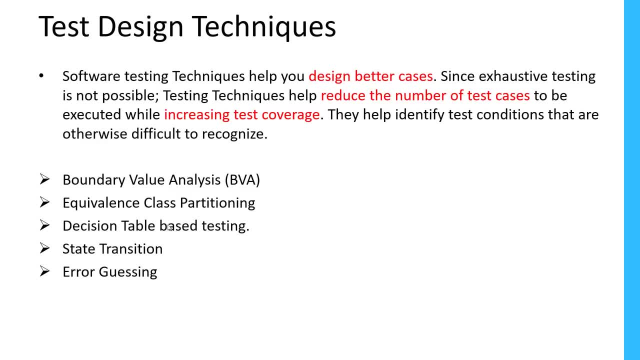 So that is the reason we need to apply test design techniques. now Let us see What are the different test design techniques we have. So here I have listed out a few techniques here: boundary value analysis, called as BVA, and Equivalence, class partitioning. and decision based- the table testing. 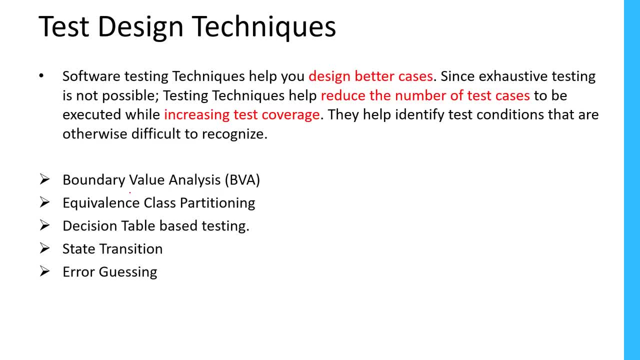 State transition and error guessing. So these are the few techniques we have and if you go for any Certification course, if you want to go for any examination, these are. you will get a lot of questions on these techniques, Okay, and I will give you so many examples here. by seeing those example, You will be easily understand. 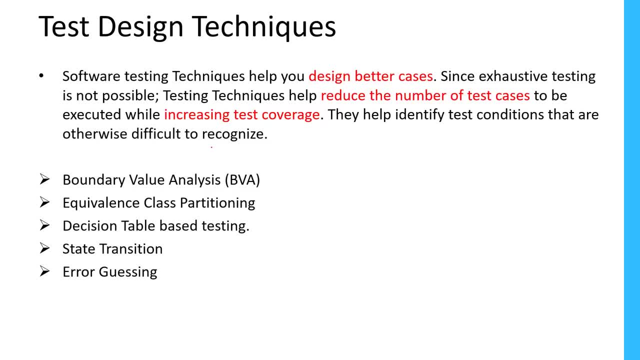 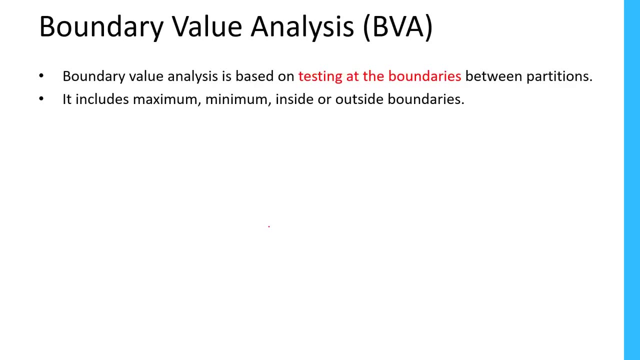 So how we can apply these techniques? Okay so, boundary value analysis, equivalent class partitioning, Decision table testing, state transition and error guessing. So these are the few techniques we have to design out test data. Now let us see one by one. So first one is boundary value analysis. 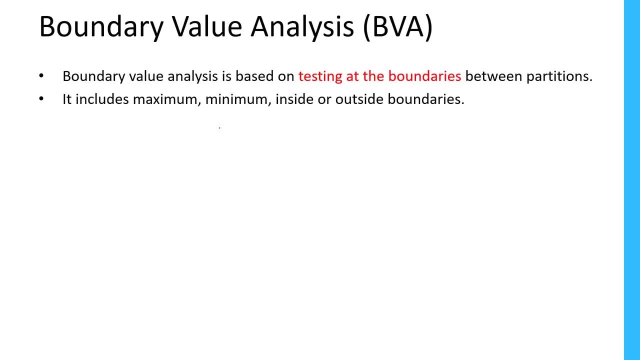 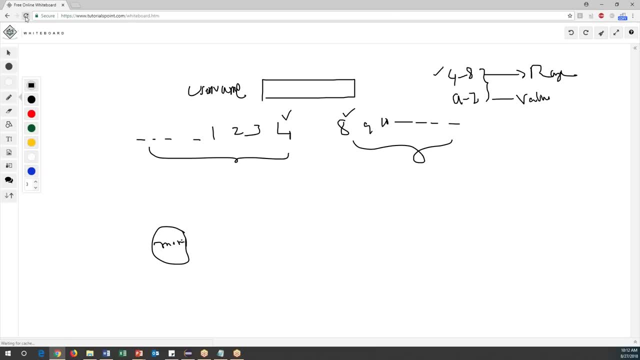 What is this boundary value analysis? So boundary value analysis is a based on testing at the boundaries, So very important here. I just show you one example right here. in the same example, again two important things: equivalence, class partitioning, boundary analyze. these are the combination actually bva. i'll explain together bva and ecb: boundary value analysis, equivalence. 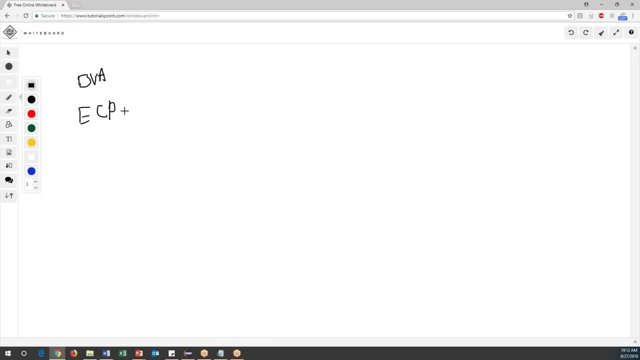 class partitioning, boundary value analysis, equivalence, class partition. so i'll tell you both the techniques very simple. now let us say a simple a username text box. a same requirement i'm telling again this is, let's say, username. okay, how to prepare the test data for this? and by using 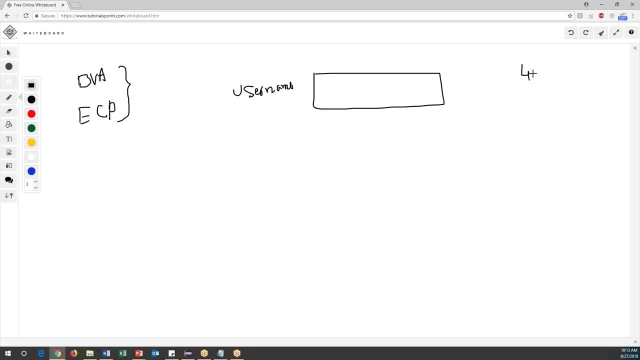 these two techniques. so let's say, this username will accept four minimum eight as maximum characters and it accepts only lowercase letters, a to z, any characters we can use. this is my requirement. now, what is bva means boundary value analysis is talking about the range. this is called. 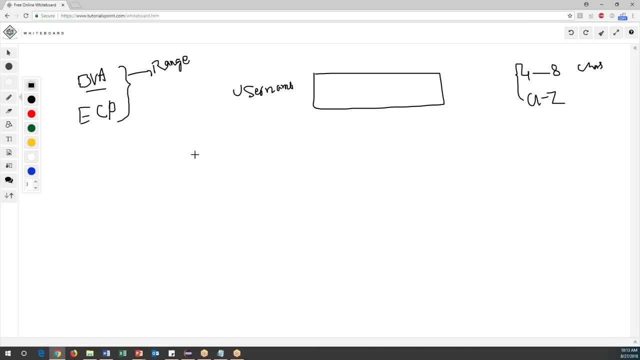 as a range verification. range of the data means what is the minimum and what's the maximum, and equivalence partition is talking about the value. so it is range check and this is called value check. what exactly it is allowing the values. that is talking by the ecp equivalence class partitioning. now let's see an example here. 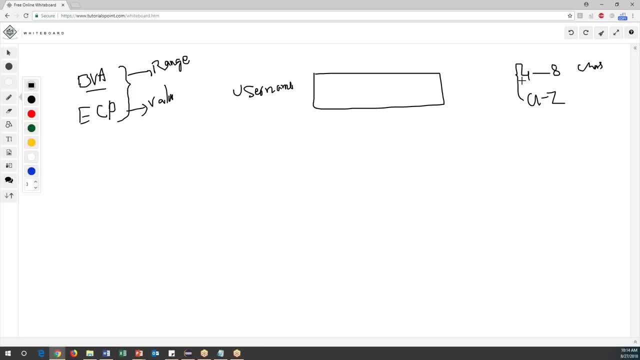 boundary value analysis. so, as per my requirement, it is saying four to eight characters are eligible. okay, so boundary value analysis techniques? uh, basically divide the boundaries, like, for example, let us say a small boundary like this: so what is the minimum? four is a minimum. what is the maximum? eight is the maximum right. 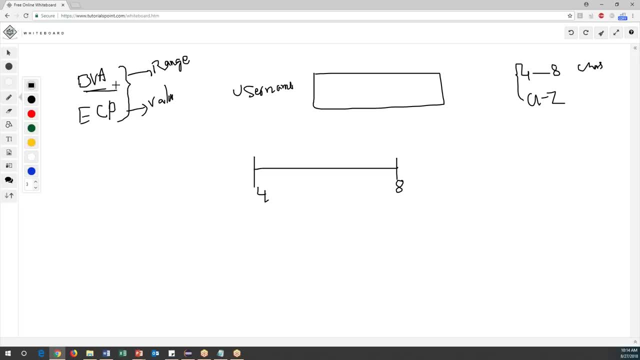 so in the boundary value analysis we will take, uh, seven parameters, totally six parameters. so if we cover these six parameters, the whole testing is completed. we no need to test with other inputs. okay, i'll tell you why. suppose, if you want to test this completely for positive. 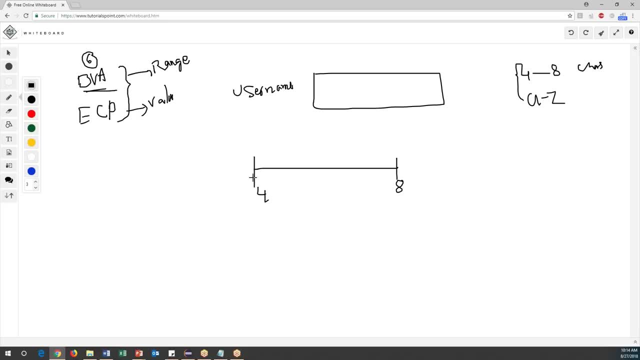 of testing what. what are the inputs we need to give here? four characters, five characters, six, seven, eight. so these are all valid characters. four is also valid. five, six, seven, eight is also valid. so, other than this, four to eight, rest of all characters invalid, but there are n number of. 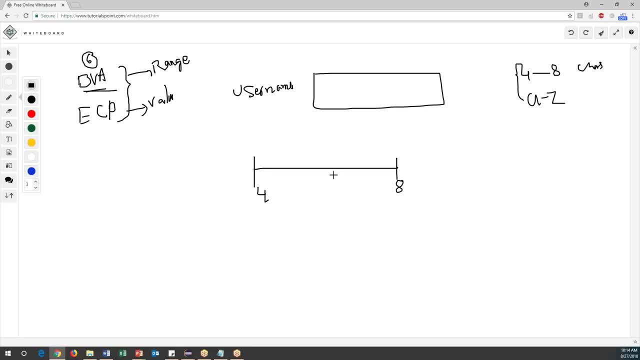 characters we have other than the 48, so we cannot test all of them. right, so we cannot test. after eight. there are infinite numbers. we cannot test all the inputs with this box. and similarly, before four we cannot test with uh, two or three, three, two, zero, one minus one minus two minus three. 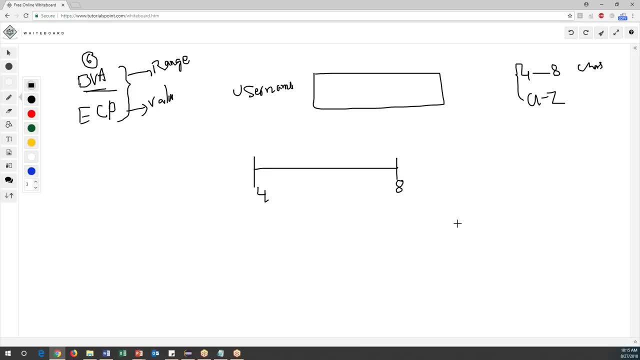 so, instead of covering all the numbers, all the inputs, we need to cover all the values of these numbers, the sets of data. what we can do is we can just reduce the data only. we test the boundaries. so, for example, this is a minimum total, this is your minimum and this is your maximum, okay, so if you 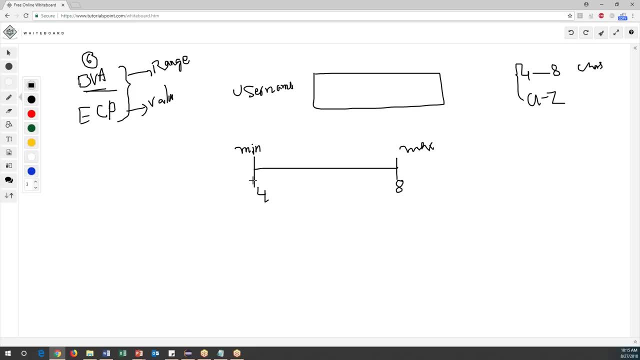 want to cover this range boundary value analysis. we need to take six parameters. one is minimum. if i say minimum, this should be pass. that is our expectation. and if i enter the maximum number of character, this is also pass. now, here, at the boundary level, we take two more parameters. let's 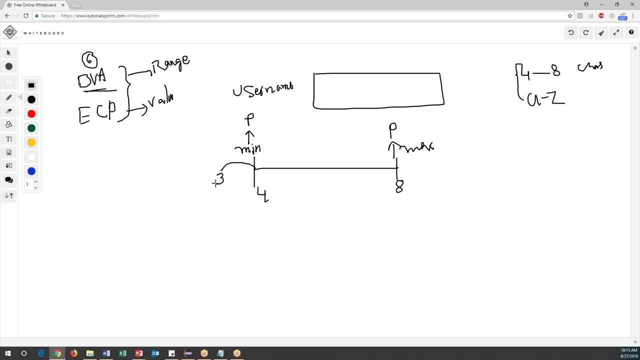 say four minus one, let us say three. so this is called minimum minus one, right, minimum minus one. if i say three, what is an expected should fail, and here minimum plus one, minimum plus one, we'll add one more one. so what is that five? five means it should pass. so if we cover these three parameters, 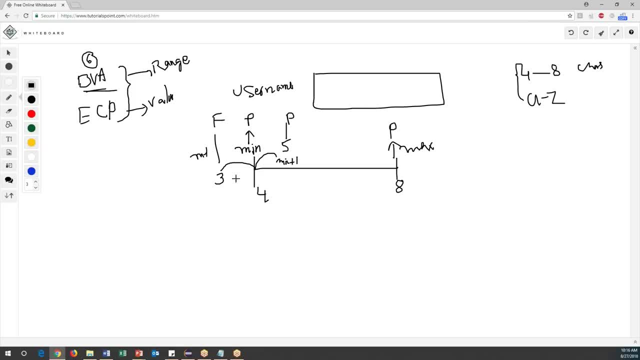 that is enough here. so if i have three is failed, what does it mean? is obviously two, one zero one. everything will be paid. if three is failed, right, because they are lower than minimum mark. and similarly, if a five is passed- for example, minimum is four- will pass four plus one. five is passed. that means 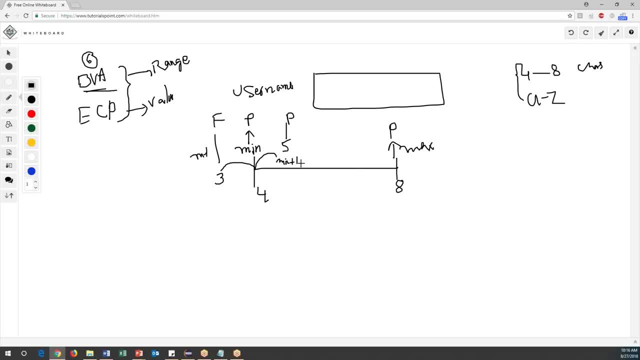 six, seven, eight will also pass. so that's kind of that gives a guarantee. so here eight. so this is the maximum movement. so if i say maximum plus one, so that is nine. so if the nine should fail, or obviously ten, eleven, twelve, everything will fail. and similarly we need to test minimum boundary, so eight minus one, maximum minus one, so we need to. 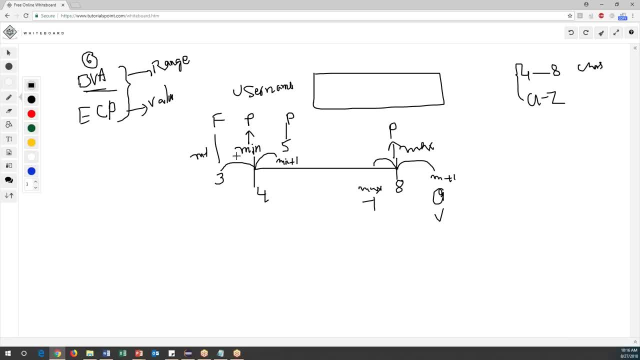 cover the only the boundaries. so minimum, minimum minus one, minimum plus one. there are, see three parameters here. here maximum maximum plus one, maximum minus one. so here three more parameters. only six inputs are enough to test complete structure. So other than this we don't need to go for any other. 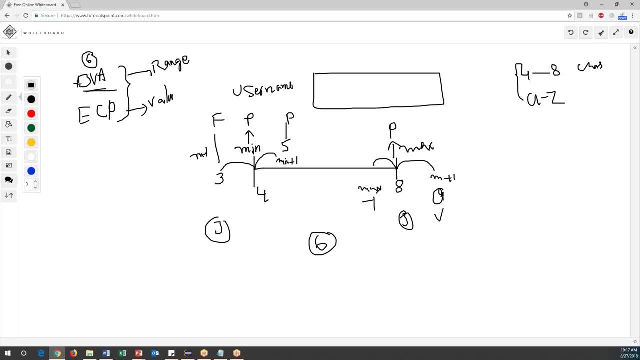 Okay, so this is called as a boundary value analysis, also called as a range range check. What is a boundary? So we need to go. we don't need to cover everything here. Okay, Similarly, suppose there is a number field. Let's say: 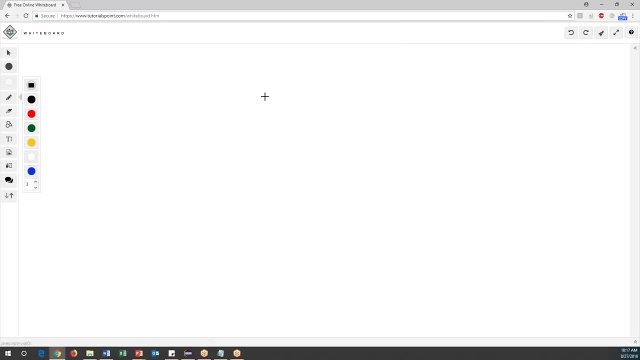 Let me take one more example. So here I have a number field, so I need to enter this number. Let's say this field accepts one to one thousand numbers- Okay, one to minimum one mark. or let's say minimum hundred, Okay, minimum hundred. my exam: one thousand numbers, It will allow us. so how to test this now? 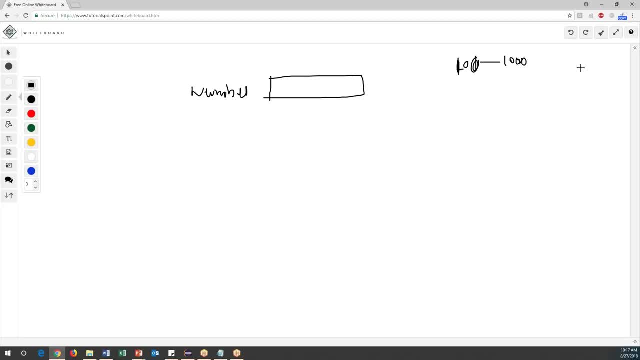 So we cannot test one, two hundred plus one thousand plus number, So it will be infinite. So we cannot test all the numbers right, even hundred to one thousand. There are n number of numbers, So we cannot cover everything. So in this time we need to go for boundary value analysis. 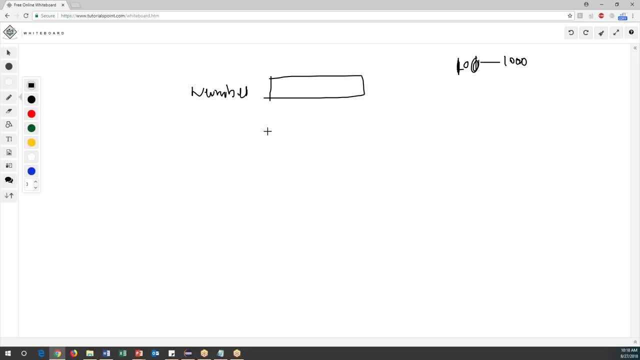 So in the boundary value Analysis, how we need to categorize the data range. So minimum is Need to make a boundary. So this is: hundred is a minimum, 1000 is a maximum boundary. So here we need to test 99. that should fail and 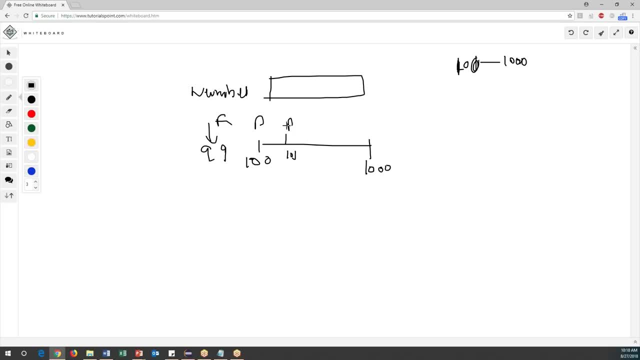 100 should pass and 101 should also pass. these are three parameters here and other side maximum boundary 1000 should pass and 1000 plus 1 should fail and 1000 minus 1, 999 should pass. so totally here 63 parameters if. 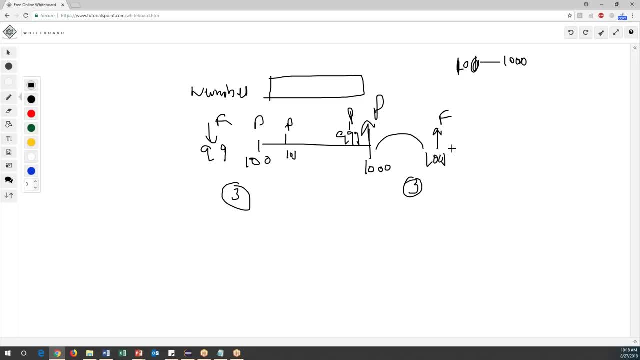 1001 is failed. That means after 1000, whatever number comes, everything will fail. and similarly, if I is, 99 is failed, whatever comes below 100, everything will fail. so that kind of Flexibility we have in boundary value analysis, This is called as a boundary value analysis technique. 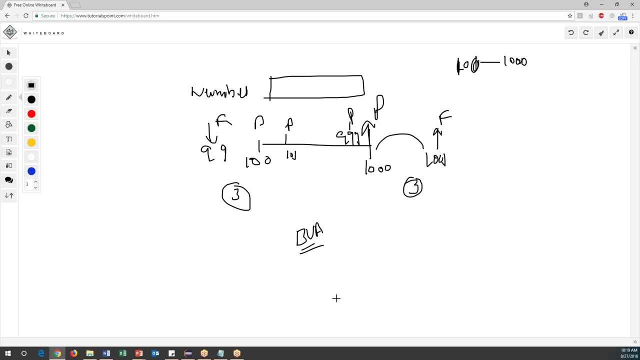 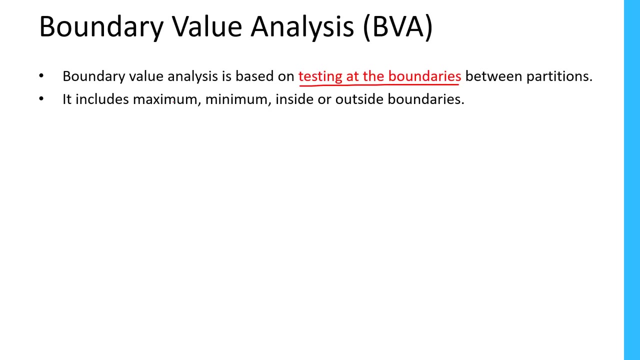 So by using boundary value analysis technique, We can just create some test data which is valid and invalid. Okay, so there's a first thing: boundary value analysis. Now here, boundary value analysis based on testing at the boundaries between partitions, So it includes maximum minimum inside our outside boundaries. 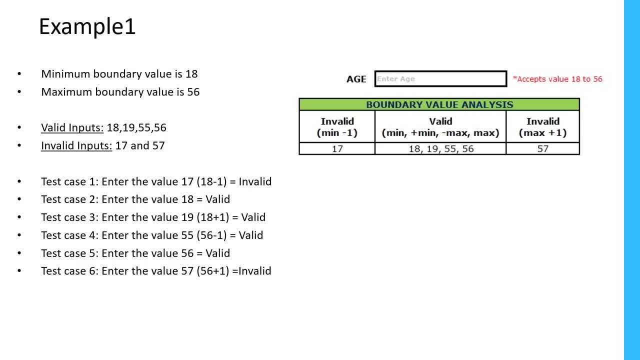 Now, same example here I have. this is one more example. Let's see. So this is the text box We need to enter: age between 18 to 56. This is my requirement. now for this requirement, or how we can differentiate the boundaries: minimum minus 1 is 17. 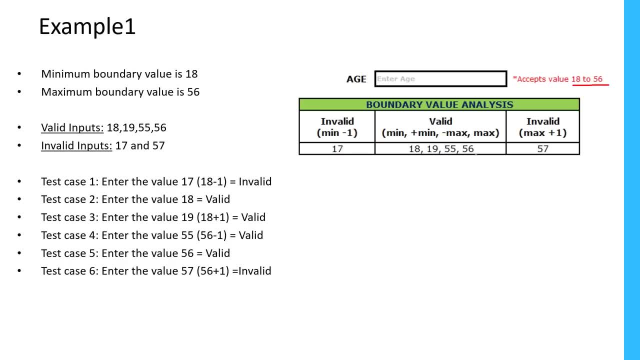 minimum minimum plus 1 maximum maximum plus. Okay, this is invalid criteria, valid criteria and again invalid. So if you observe here 18, 19, 55, 56 are valid, in this again need to follow the boundary. So 18 is a minimum, 56 is a maximum. 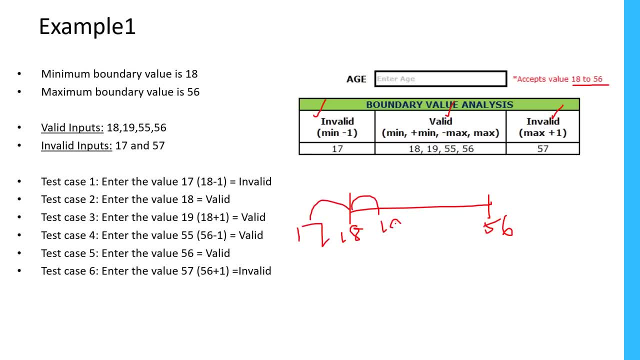 So 18 minus 1 is 17, 18, 18 plus 1 is 90 and 56 minus 1 is 55, 56 plus 1 is 57.. So how many are valid? how many are invalid here? This is invalid and this is invalid. 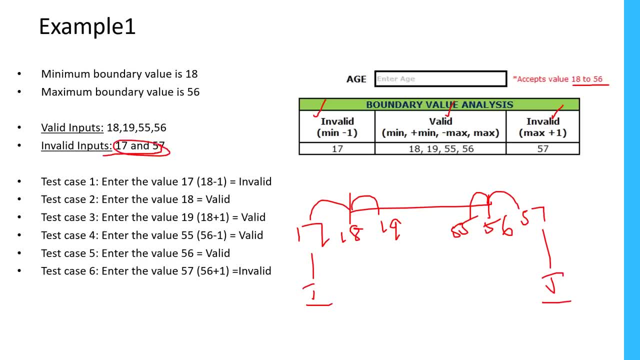 Right, 17 and 15, 7 are invalid. These are the invalid and rest of them are valid thing. So how many test cases we can write with the data six, number of test cases we can write. Okay, so this is how we can just prepare the input: the boundary value analysis technique. 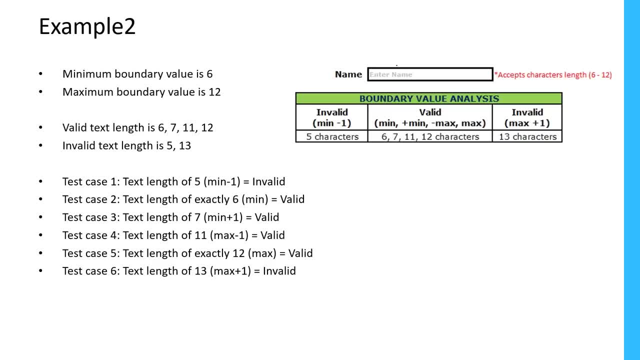 Now one more example, same again I told you before. so this is the text box which can accept, Let's say, 6 to 12 characters. so 6 to 12 characters, I'm saying it, 6 is a minimum boundary and 12 is a maximum. 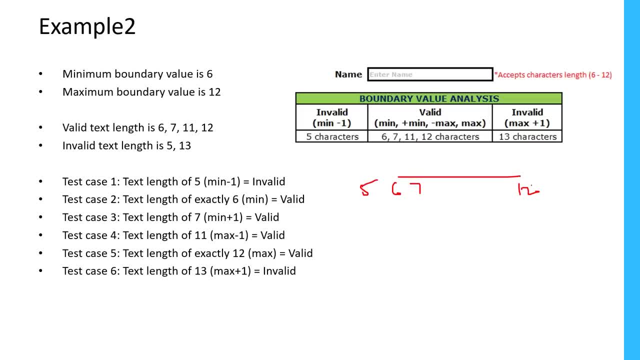 again: minimum minus 1, 5. minimum plus 1, 7. Magnum minus 1: 11 back 1 plus 1 is 13.. So again 5 is invalid here, 13 is invalid and rest of them are valid. So 5 that in are invalid. and then: 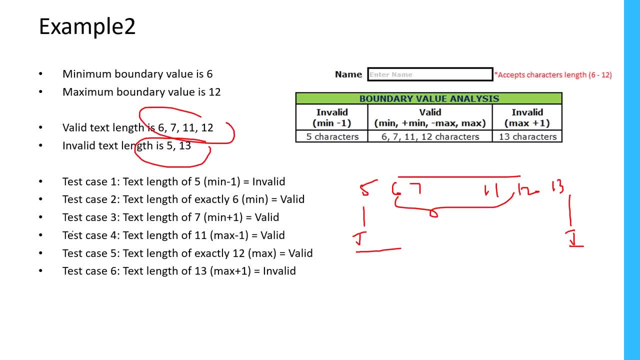 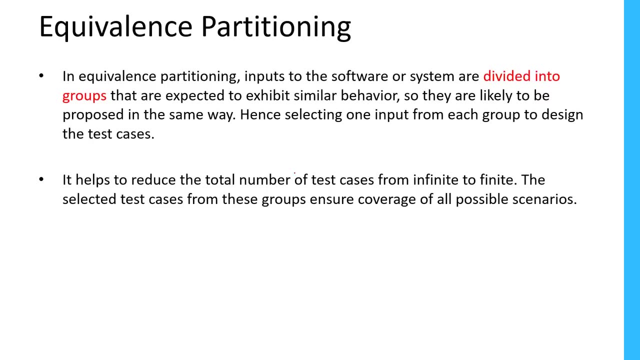 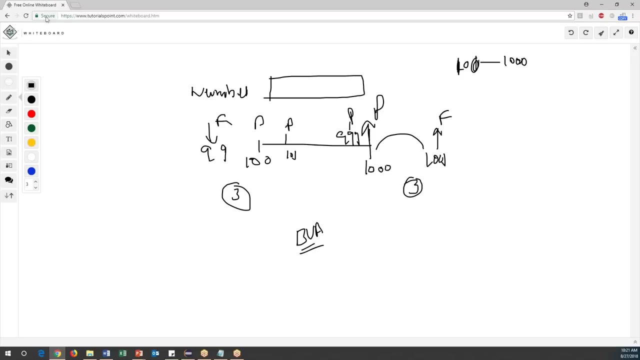 Best of them are in one. so total again 6 test cases we can take. this is also comes under the boundary value analysis, So boundary value analysis is basically focusing on range or boundaries. Okay, So let me see equal and Equal as the foundation. So this is also almost similar to boundary value analysis, but your difference is there. Let me just give you the difference. 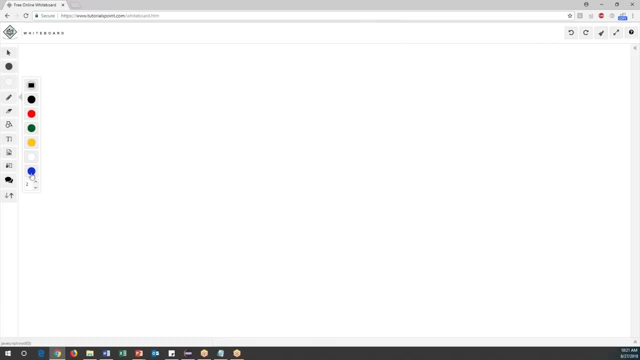 so boundary value analysis, mainly focusing on boundaries of data. okay, BVA and ECP. So boundary value analysis is mainly focusing on range of data or boundaries of data, But equal as class partitioning will verify actual value of the data. Okay, I'll tell you difference. the same input box again. Let's say this is again. use a name. 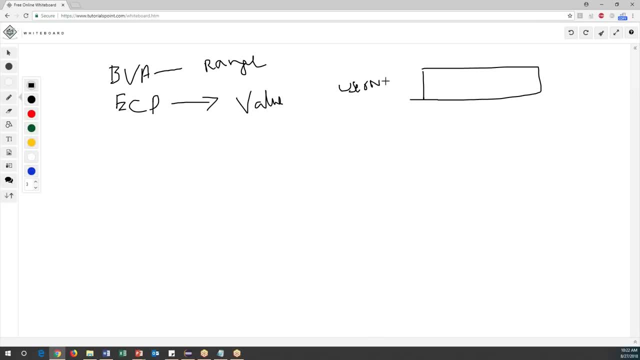 I'll tell you what is the difference between both. Okay, this is a user name field. So here my requirement. again, I say four to eight characters, it will allow, and it will allow only small case letters. So for the same thing, I need to prepare the test data based on by using these two techniques: boundary value analysis and equal as class partitioning. 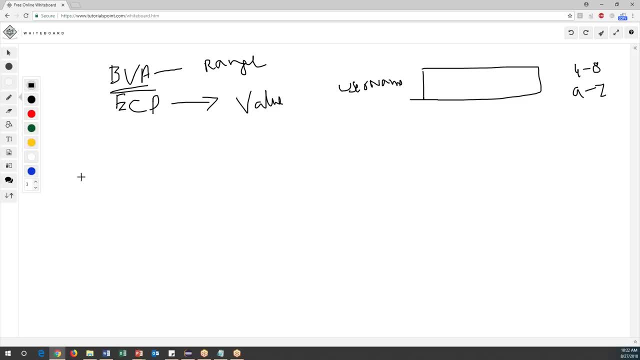 Now let's see boundary value analysis. What what we have seen is we have created six parameters, right? So minimum minimum minus one, minimum plus one, and then maximum Maximum minus one and the maximum plus one. So these are the parameters we created. These are not basically talking about the boundaries, but when you come to the equal as partition. 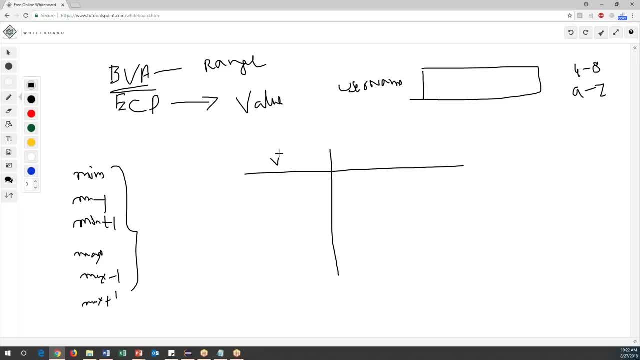 We need to divide the data like this: valid criteria and invalid criteria. So, as per my requirement, this is how we need to focus on value. We have to focus on So the valid- what is the valid data here? as per my requirement, a to J. 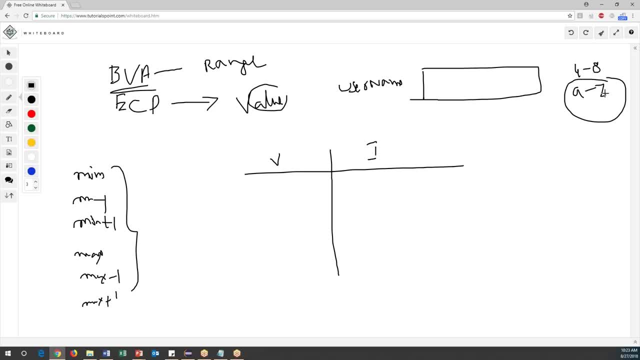 That will lower case. letters are valid other than this. Everything is invalid. So we need to prepare a small table like this. So let's say, only a to J are valid, and what are the rest of them? We have uppercase filters not valid, numbers not valid. 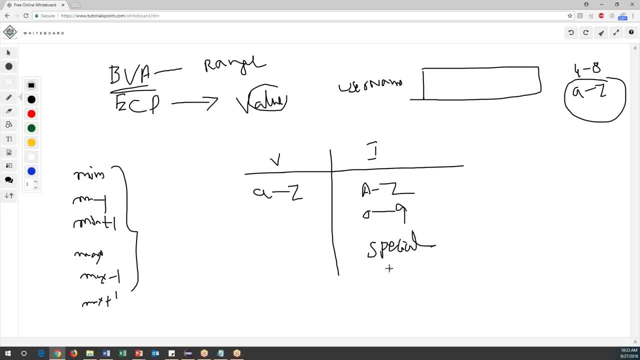 Special symbols or special characters not valid and spaces not valid. So all comes under the invalid case. So when you prepare your test data, we need to consider only this part. We should not consider consider these characters. This is a kind of categorization: What is valid and what is invalid. 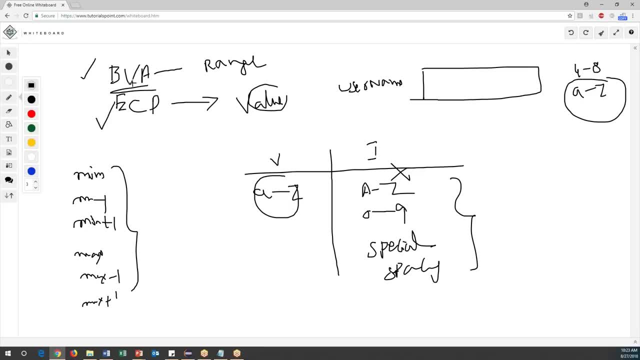 Irrespective of boundary value analysis and equal as class partition. So, in the boundary value analysis, the more focusing on the range- Okay, and six parameters we will take here- and in ECP, the more focusing on the value which we are entering into this text box. 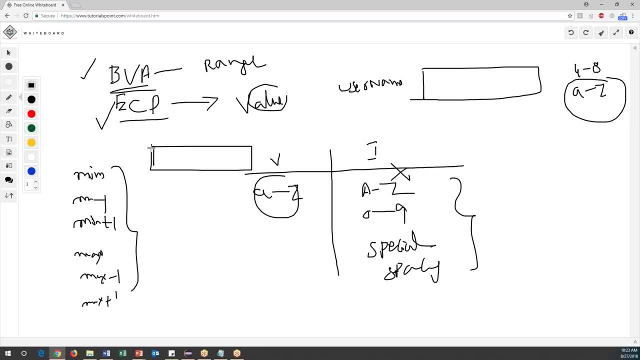 And whenever you see the text box validations, you must apply boundary value analysis and equal as class partition- Very important techniques. Okay, so these are only a to J is valid and best of them are invalid. so this is how this is called: equivalence, class partitioning, or. 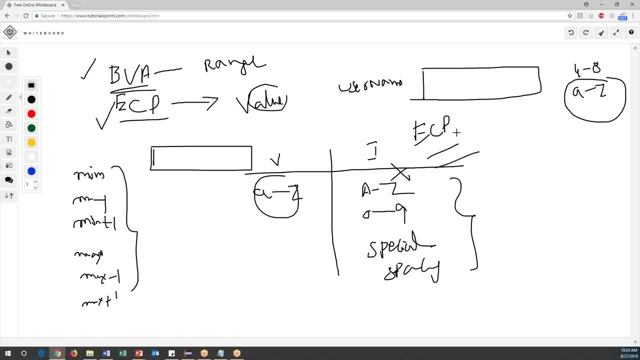 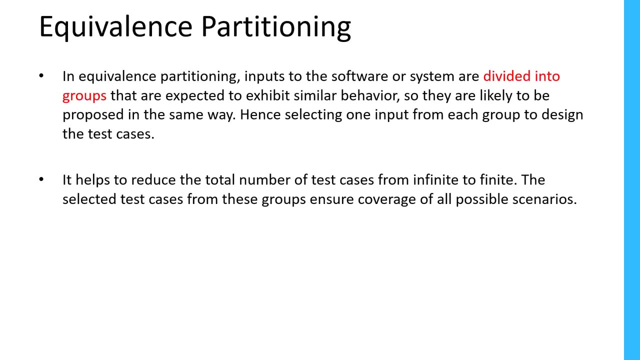 Equivalence partition. people also called equivalence partition or equivalent class partition. Anything is fine. So in border value analysis we have six parameters, But in the equal as partition we have valid and invalid to categorization. Okay now, so this is all about Equal. and so in equal as fast partitioning inputs to the software system or divided into groups. 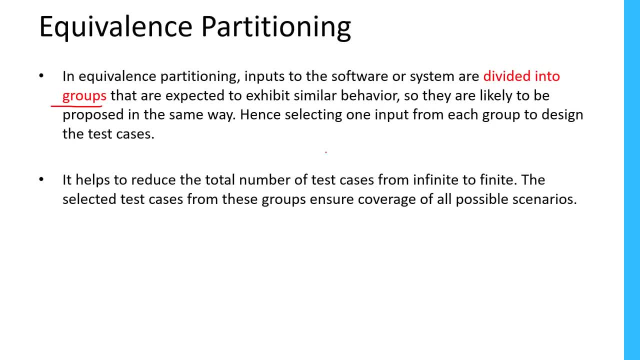 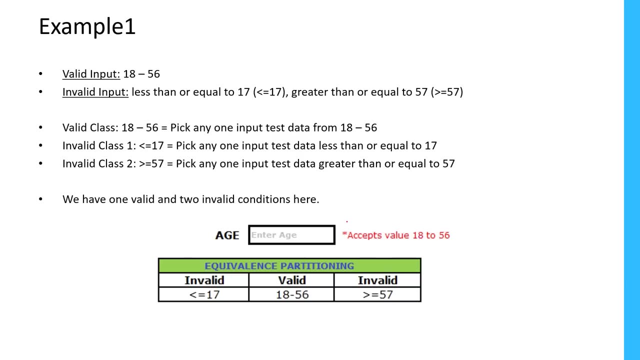 That means it valid, group and invalid, So very important. so it helps to reduce the total number of test cases from infinite to finite. So the selected test cases from these groups ensure coverage of all possible scenarios. That is the main intention of using these techniques and here also have given few examples. 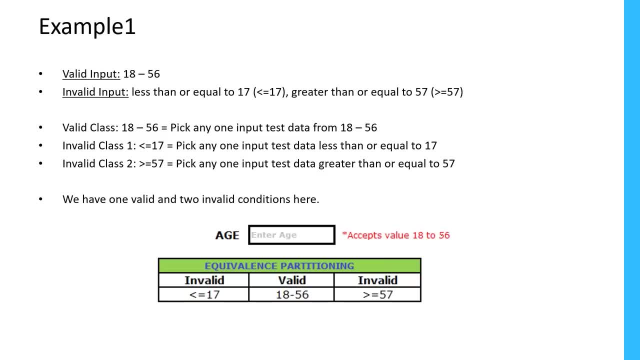 You can see here- and this is the H field, again, 18 to 15, the here 18 and 15, 6 is actually boundary, Okay, and we can consider this as a boundary and also we can answer as a value also, because 18 to 56. 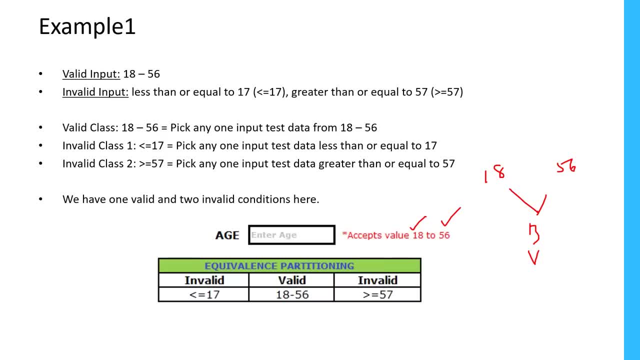 Numbers only it will allow. so how we can prepare equal and start. partition means invalid, so less than 17 if I give something that is invalid. and Again, greater than or equal to 57 if I give anything here, that is also in. So what is a valid here? only 18 to 56 is a valid. 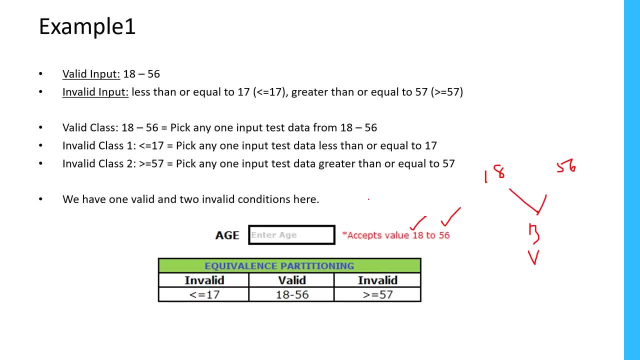 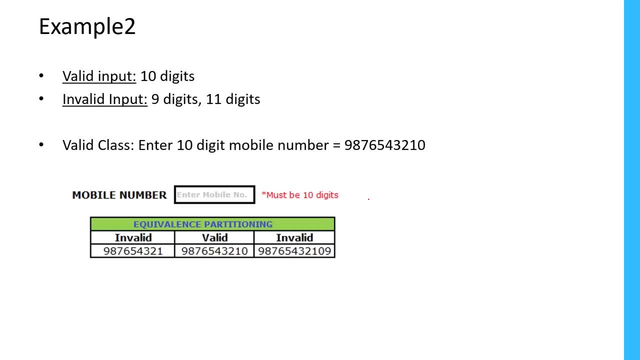 Okay, so this is called equal as fast class partition. We just draw some stable and create some, Categorize some data, valid case and invalid case. and here one more example. So this text box entered, or 10 digits, Let us say, for number. Okay, so 10 digits of 4 number. So 10 digits means are here. What is the equal as that partition is invalid is here. 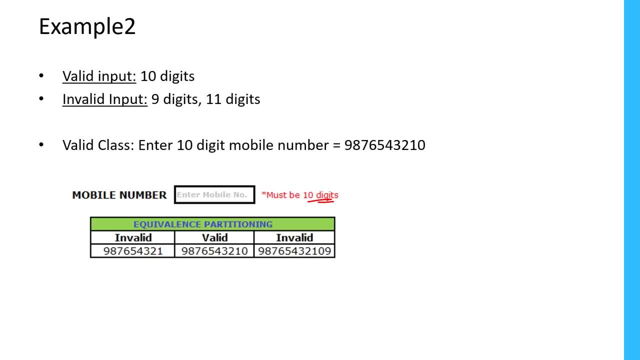 How many characters we have here: 1, 2, 3, 4, 5, 6, 7, 8, 9, 9 numbers We have. this is invalid because, as per my requirement, he tell us 10 digits And again, this is also invalid. I think this is 11 characters I have and this is 10 characters. 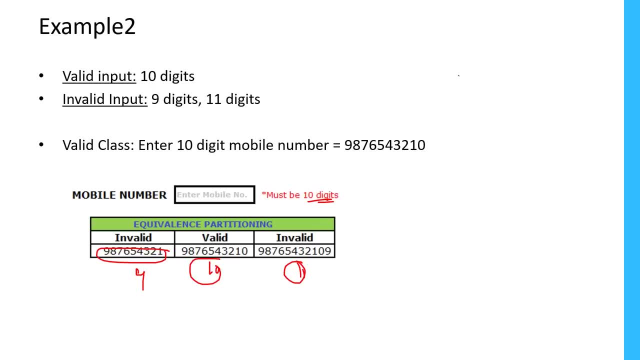 I have. so this is again valid and you need to Remember the difference between these two. so boundary value analysis, mostly focusing on the range- Okay, and ECP is focusing on the value, so range check and a value check- Okay. so remember these examples very Now. this is called equal as class partition. 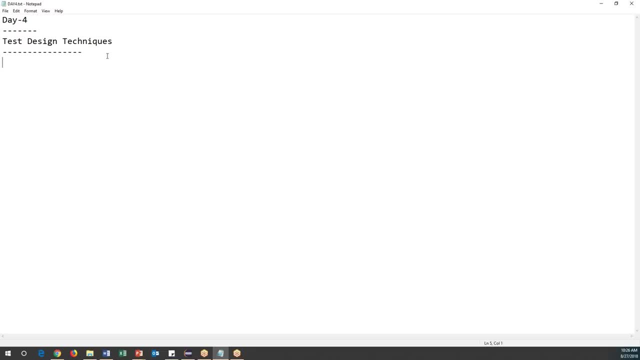 So we discussed about two things. one is a BVA Boundary value Analysis and then equivalence- Okay, and then we'll discuss one more Decision table. so these techniques are like: wherever we need to lose, you can just go and use it. Okay, so there is no rule like the only. this is the place We have to use this technique. 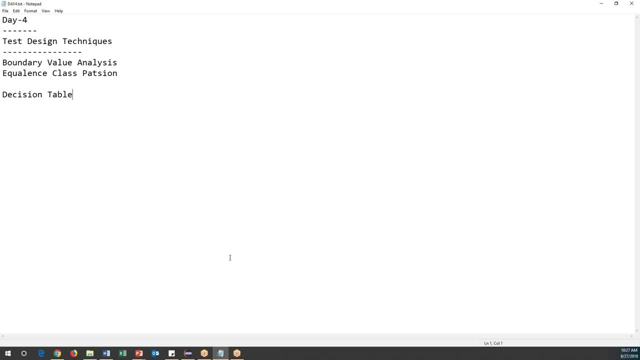 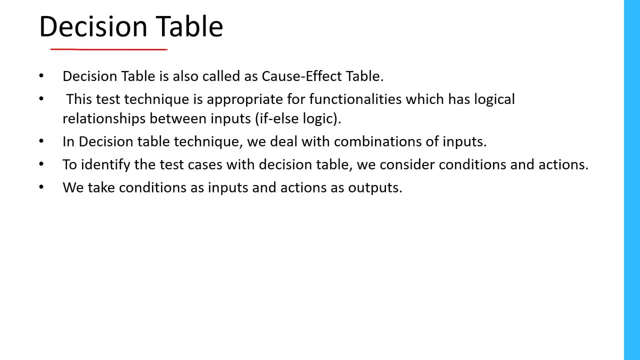 No, not like that. So we can use these techniques or wherever it is appropriate. now Let us discuss about the decision table technique. Okay, and when we need to go for decision table techniques? if you have more number of conditions, Okay, if I'm so, so and suppose so and so is true, and apply certain action. if something is is true, then I've been different action. 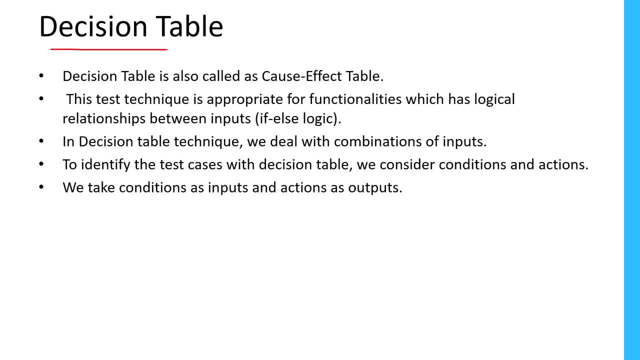 So if you want to add up, if you check more conditions, Okay, so then you need to go for the decision table. So this is also called as a cause-effect table. There are multiple names we have, so just remember this somewhere. if you see, this term name is different. 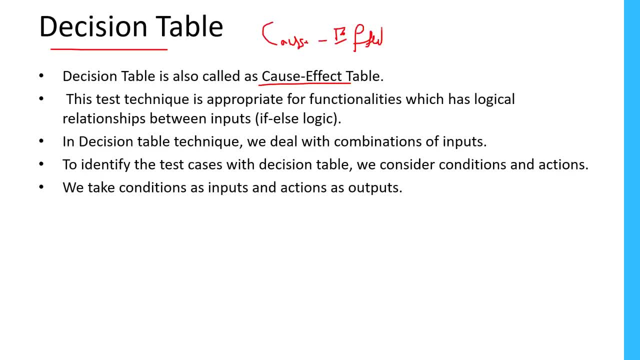 You don't need to confuse a cause-effect table. It's called cause-effect table, reason, cause and effect means What is the decision, what is an action. so the decision table, mainly two important things. one is What is the condition and what is the corresponding action to be done. So these are the main focusing on decision table. 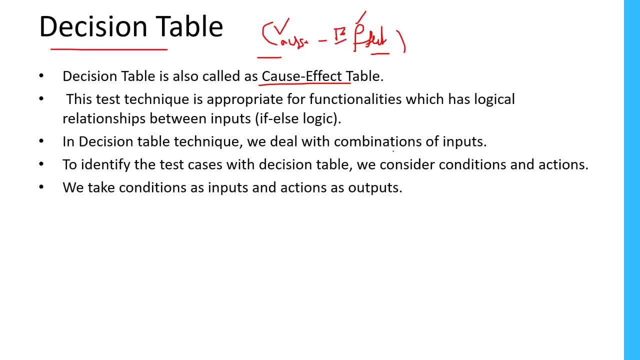 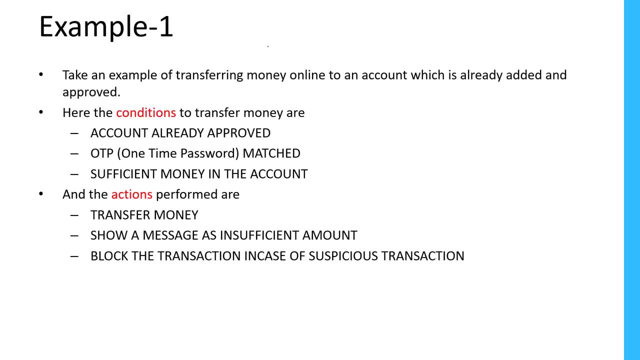 Now let us see an example: How to create the decision table technique, how to use the decision table technique. Now let's see this example here. So an example: transferring money online to an account which is already added and up. See this very correctly, Very important example. Most of the times, interviews also people will give you this example. 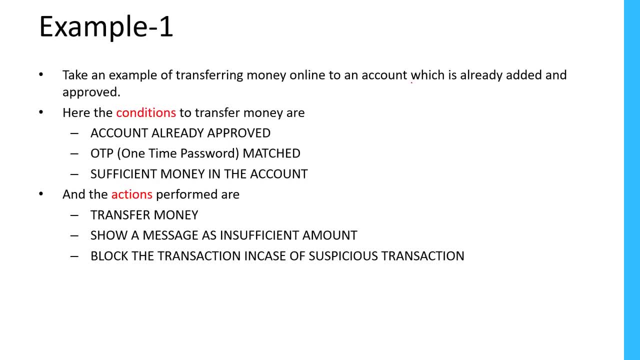 here: Transferring of money online to an account which is already added and approved. So what is a precondition here? if the account is already added and upload, then we can transfer the money online. Okay, So here, what is the condition? What is an action? so already added and approve, so this is a condition. 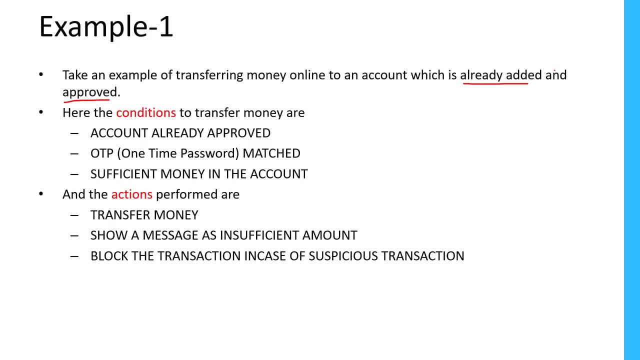 if the account is already added, also approved, there are two conditions and if these conditions are matched, then we can send money online. that is an action. so just transferring money online is an action here. and what are the conditions? we have account added is one condition, one and upward is condition. so if you want to test this particular scenario, we need to follow certain 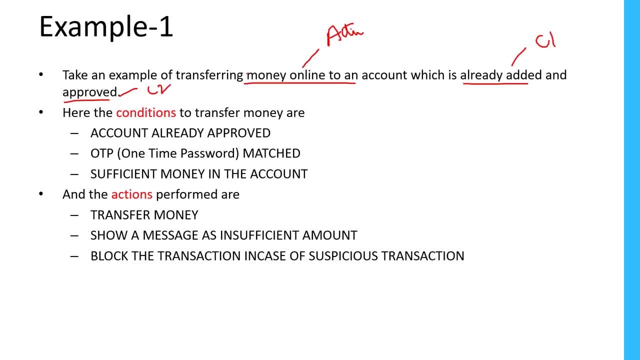 different aspects. so let us see what are those, as first we need to understand what are the conditions, what are the actions? okay, so in this scenario, what are the conditions? first let us say condition, so account is already approved. that is one kind of one condition and suppose even though 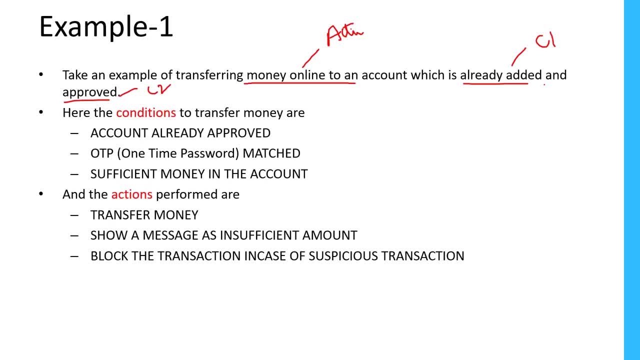 if you approved or an account is added at the time of money sending, it will send you otp right that otp is also should match and then only you can send your money. so that is the condition, also a kind of condition. so under conditions i have three things. one is account already approved. 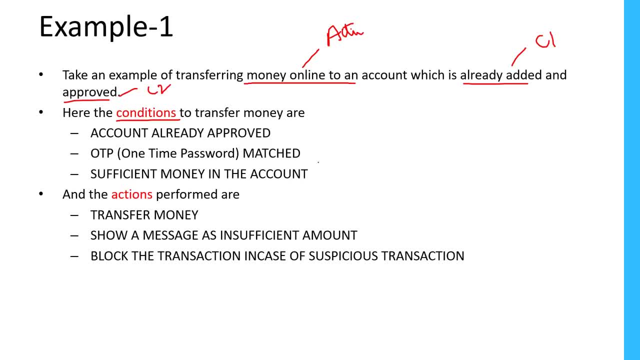 otp matched and sufficient money in the account. so if the account doesn't have the sufficient money, we cannot send money right. so these are the conditions, but all the conditions not given in the example, but we need to assume few things here. but in the requirement what they have given is: 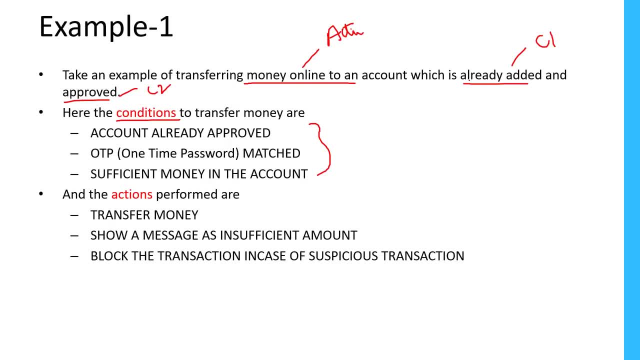 only account is added and approved, but other things i have not mentioned. but we need to assume those things because already added and approved, fine, but money is not there in the account, we cannot transfer and otp is not matched. we cannot transfer. right those things. they cannot mention everything, but we need to. 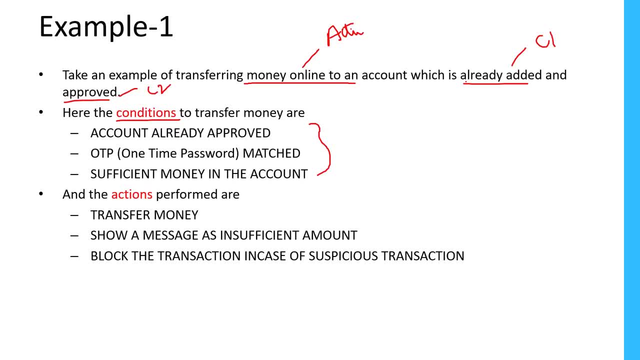 assume few things here. so overall we have three conditions here. one is: account is already approved and o2p should, otp should also should match and it should also have sufficient money in the account. in these three cases, if these conditions matched, only we can pass, we can send the money online. so now let us see actions part. so 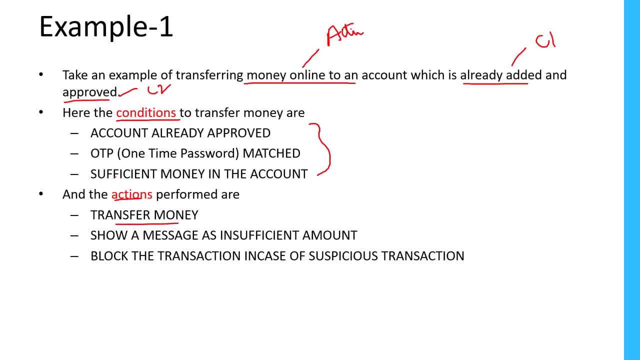 we get in the actions, we can transfer money if all conditions are becomes true and sometimes show a message in: and you know, suppose, suppose money is not there in the account, there is no sufficient money, then what is the message? I will expect you should show message like insufficient amount and 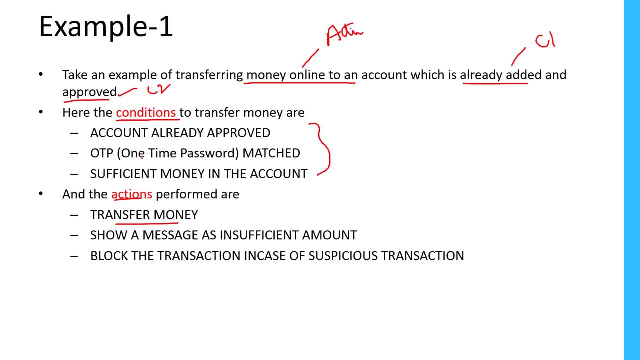 suppose OTP is not matched. so what I should accept expect: block the transaction in case of suspicious transaction. if OTP is not matched, that will be considered as a suspicious transaction. so there are three possible conditions and there are three possible actions here. suppose account is not approved, they can say: block the transaction in case of suspicious. 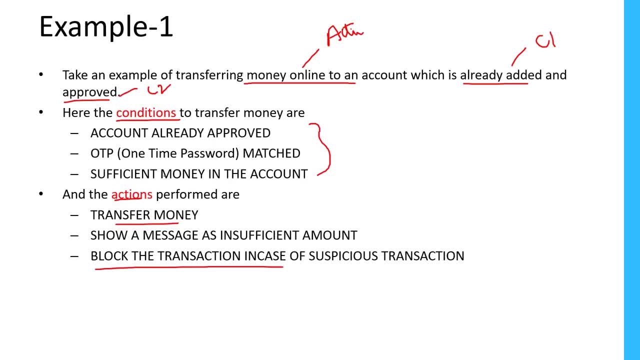 transaction or OTP is not matched. also same message: money is not enough in the account in that case. so we should show a message called insufficient amount. if all conditions are matched, then we can send the money. there's a first condition. so if you observe, here there are three. 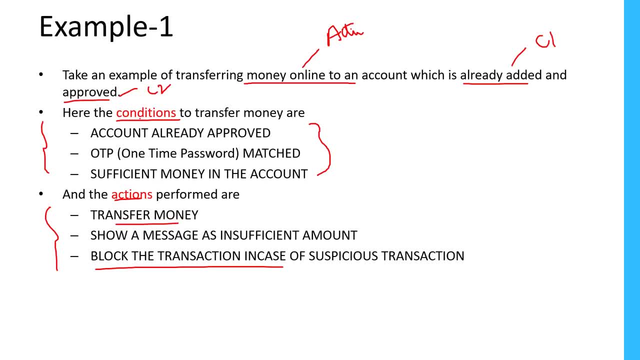 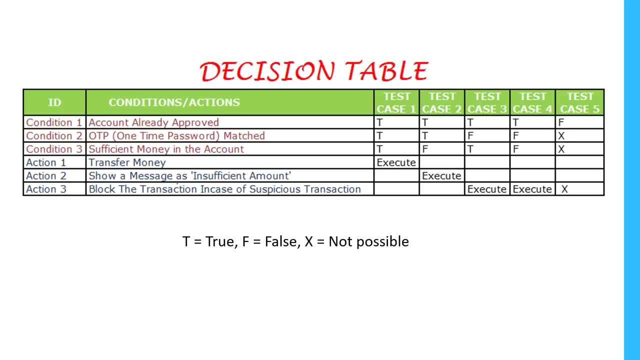 conditions and three actions: everything we need to cover. all the conditions and actions also we need to cover at the time of testing. so if you prepare a smaller decision table, that will be very simple to categorize this. so let me just show you decision table now. so this is our decision table. so, based upon our 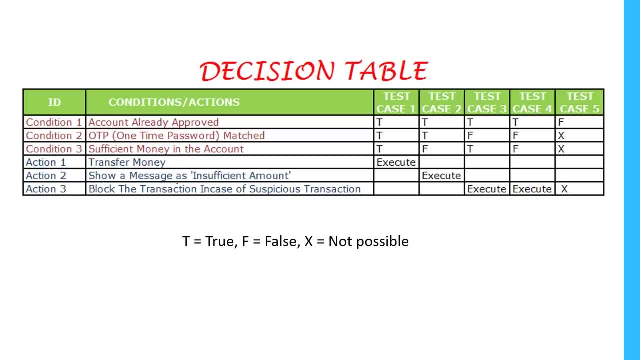 conditions, actions are prepared, some table here. so the decision table is always having common columns, like here. let's say an ID column is one, can the ID column? I'll specify all the conditions first and then actions. okay, I already three conditions. so I mentioned on three conditions and three actions. one, two. 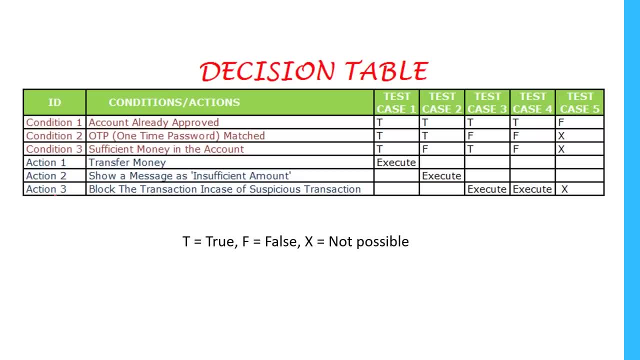 three, four like this. any number of conditions you can have. any number of actions also we can have. and then I also mentioned what are the conditions and actions. so condition one is account already-up буде approved. condition two is one time password should be matched. and condition three is sufficient money. 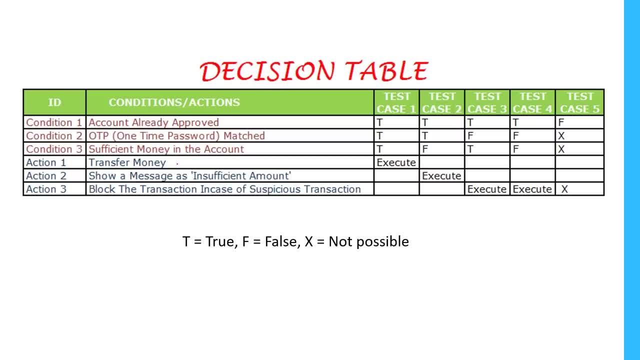 in the account. next, what are the actions here? action one is transfer money. action two is show a message as insufficient amount. this is also a kind of action. and action three is block the transaction in case of suspicion transaction. now let us put all of the all of them in the list. 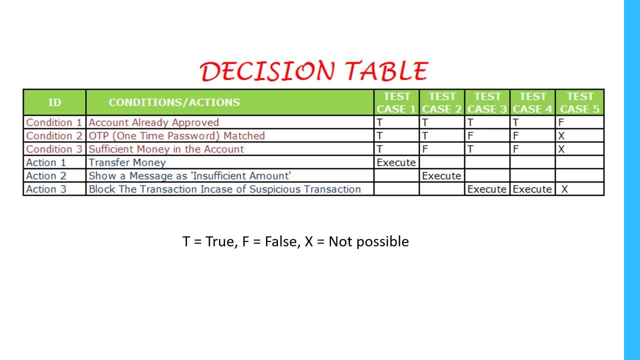 format. so conditions and actions. now let us check the all the combination. this is very important. please focus on this test case one. okay, suppose my account is already approved. condition is true, then what i should do now i need to verify the otp matched or not. so even otp is also matched. 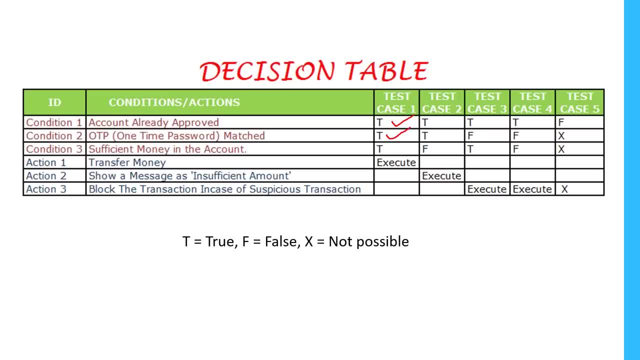 and then what i should do. you need to check whether sufficient money is there in the account or not. yes, money is also there in the account. so what should i execute now? money transfer. so transfer money should be executed. okay. so action two and action three is not appropriate here. 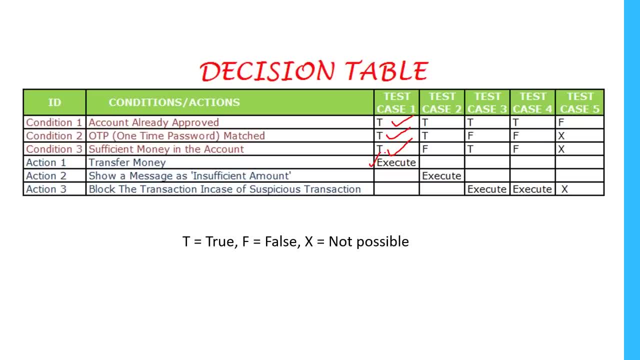 because first three are exactly matched. so the first test case. now the second test case. the second account is already approved, is true? okay, upload is fine, otp is also matched, but sufficient money in the account is known. okay, there is no sufficient money in the account, so what should i need to execute now? so show a message as insufficient amount, so this: 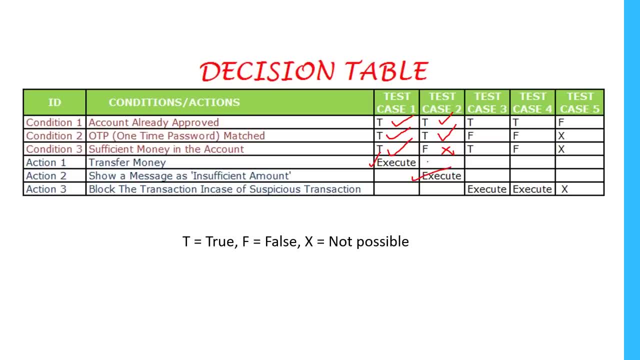 action two should be executed. so here action one and action three is not appropriate. it okay, this is one test, case two. so the coverage is very important. okay, we are. are we covering each and every uh path or every condition and action or not? that's a very important. so the decision. 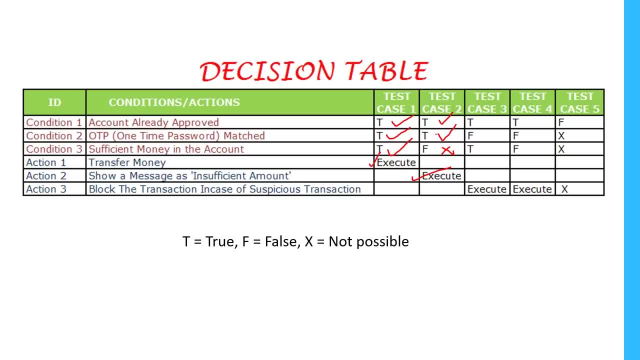 table gives you the clear picture what we have covered, what we haven't covered. okay, so now test case three. so account is already approved, okay, true, but one time password is not matched. but even account is also having the enough money, but otp is not matched. so what is the action you need to perform now? third action, that is, 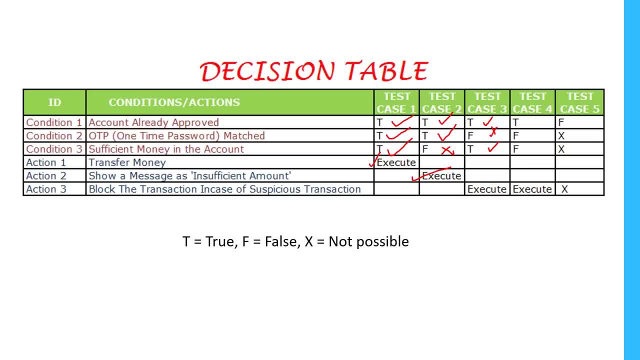 block the transaction in case suspicious transaction, otp is not matched, because we need to execute a third action. this is test case three. now test case four. suppose account is already approved, okay, fine, one time password is not matched and it is also not having sufficient money. but in this case what i should execute? now again, action three should execute: block the. 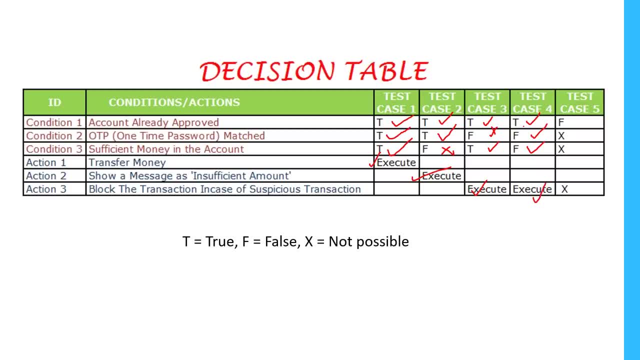 transaction. in case of the, because account is not approved, otp is also not matched with as a suspicious transaction, so we can just execute action three. now finally, test case five: account itself is not. account itself is not approved means we cannot do anything, anything we cannot. so none of the actions are not applicable here, because account itself is. 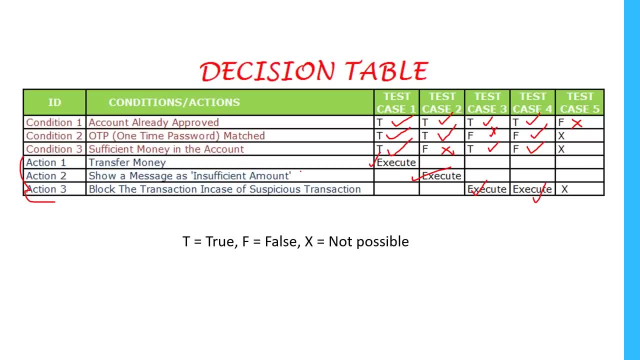 not a promise. none of the actions are, cannot be even money transfer message. okay, okay, so this is completely invalid area. okay, so, not possible at all. so, based on these conditions and actions, we can create five different test cases. so while at the time of testing, we need 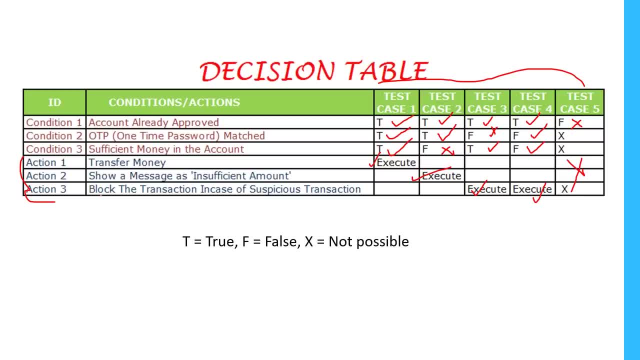 to cover all the conditions. so this will cover everything. so we haven't missed anything here. if you observe clearly, we haven't missed anything here. everything is covered. so the decision table gives you, gives you the clear picture what you, what you have tested and what you haven't tested. 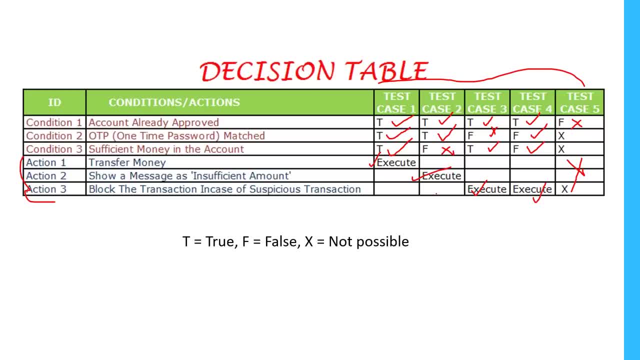 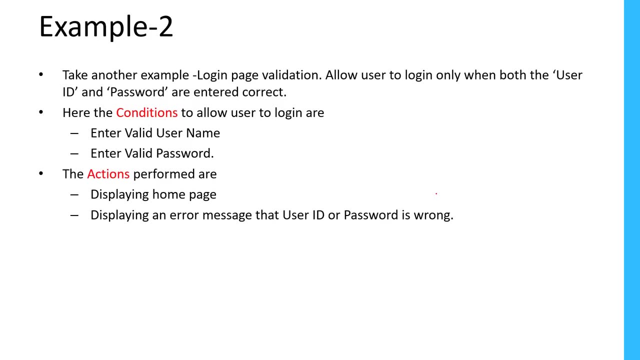 what is covered and what is not, so that kind of clear picture the decision table gives you. okay. so this is also one of the techniques at the time of uh doing testing decision table- very important. now let's see one more example for a decision table. uh, take another example: login page variation. so i have a login page. 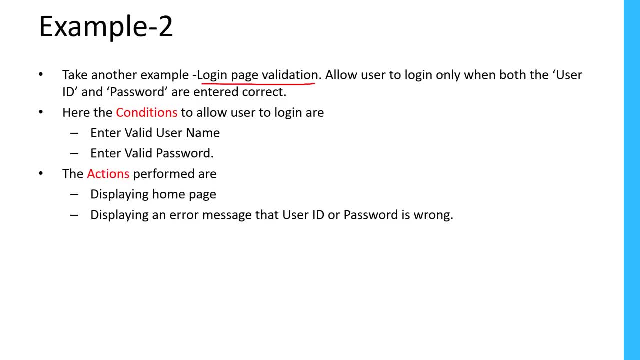 need to valid allow user to log in only when both the user id and password entered. Okay, so let's say: let's create a decision table for a login screen. So I have a login screen. the as per requirement is saying the login screen. I have a username and password. 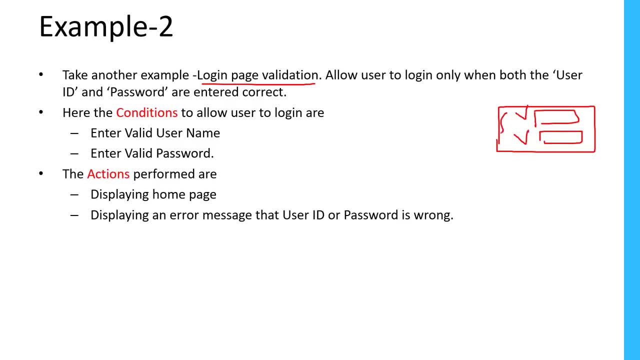 I need to enter valid username and valid password. if both are valid, then only I need to. I should able to log into the home page. Okay, if I enter only valid data, then only my login should successful, and that's my requirement. Now let us understand what are the conditions and what are the actions here again, 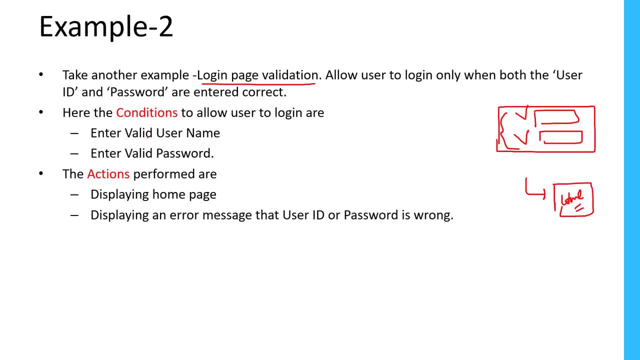 This is the one more example for decision table. Now, what is the conditions and what are the conditions and what are the actions here? now? conditions are: we need to enter username, valid username, valid password. So these are the conditions. what are the actions? we need to open either display home page or. 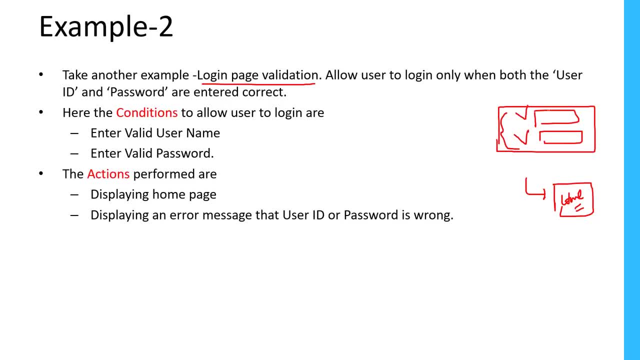 it can display some error page, some somehow, if suppose username or password, any one of them. If it is not valid, then it will display some error page or error message. These are the only possibilities we have. either it should go to home page if login is successful. 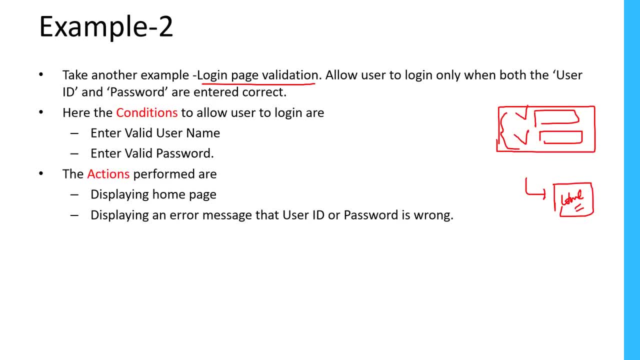 or if the login is failed you, it should throw an error message. This is the only two possibilities we have. so those are comes under the actions and conditions are, if we provide the username and password, providing the username and providing the password. So these are all two conditions. now let's see the decision table for this scenario now. 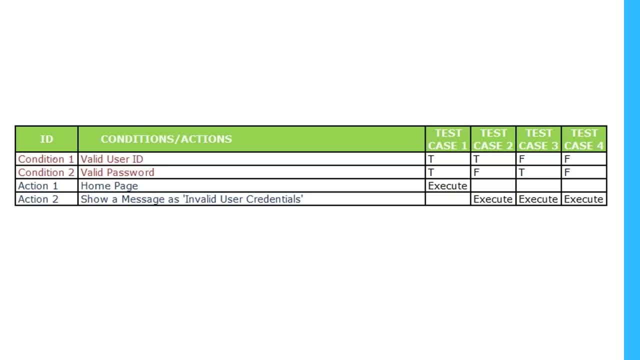 same way. I mentioned first two conditions and then two actions. So what condition? one and condition to: valid user ID, valid password. Okay, These are two conditions. and what is an action? one home page should display and the action to is show a message as invalid user credentials. 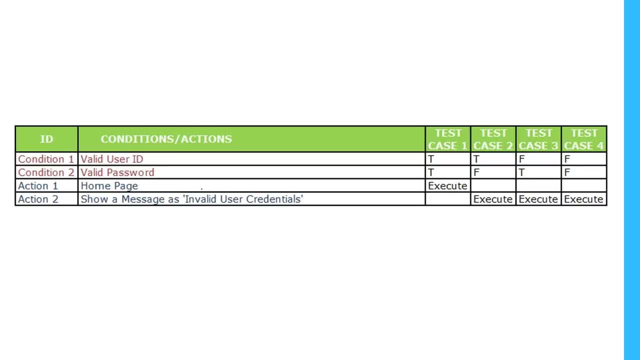 This is another action. Now let us see cover all the scenarios now. So test case one: So valid user ID. have given valid user ID and also have given valid you a password. Then what? what is an action should execute? It should go to home page. 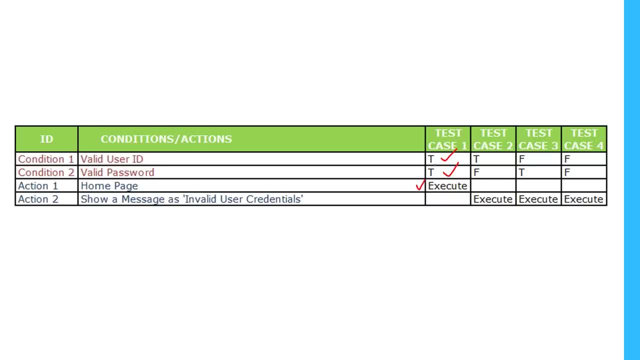 So that means a login is successful. This is test case one. This is a positive test case, Okay. and then test case two. So I have given valid user ID, Yes, but I have given password is wrong. So then, what is an action should execute, action to, should excuse invalid user credentials? 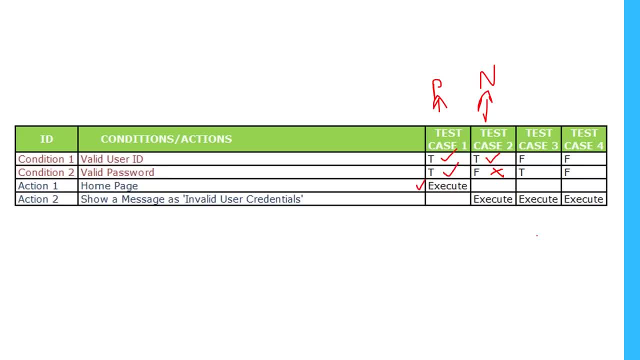 This is again negative test case. If I give invalid, it should fail. now test case three. I have given user IDs false. User ID is invalid, but password is valid. again It should execute. third second action, that is show error message: invalid credential. So test case three also come now test case four. if I give, both are false or invalid user. 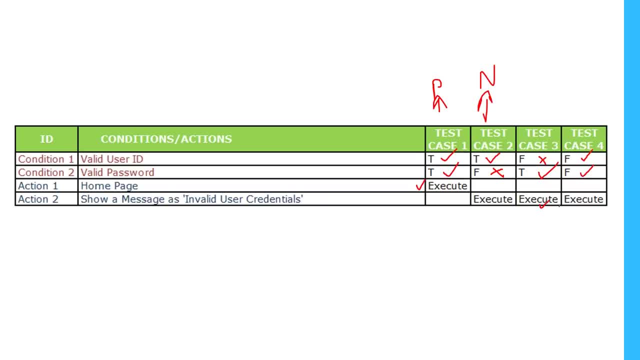 ID and invalid password. both are invalid and then again it will go to action. only the one test case is a positive test case because both are providing the false, both are providing the valid, So it is executed, It's good in only action, and rest of the test cases are invalid, negative test cases. 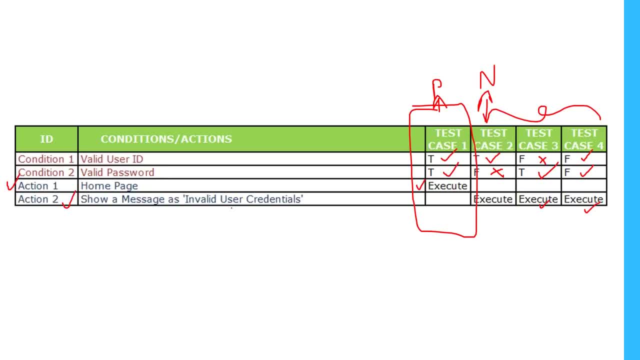 So it always is good, only action. This is another example for decision table for login scenario. Okay, Okay, Sometimes you will have a lot complex kind of conditions and those times the decision table will help you to cover all kinds of test cases now kinds of scenarios and in interview. 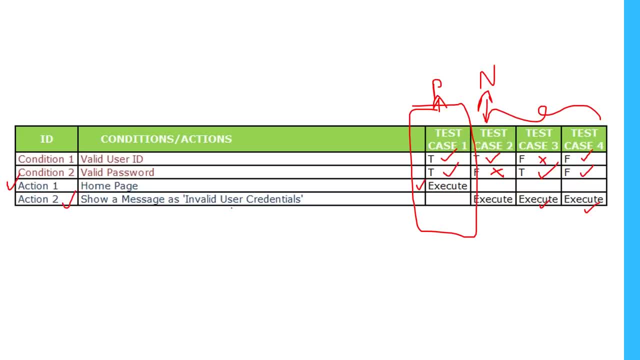 These are very important questions. They will give you a scenario like this: ask you to write small decision table- Okay, like this. or people ask you to create some boundary value analysis or equivalence class partition, something like that. Now, so we discussed about decision table. 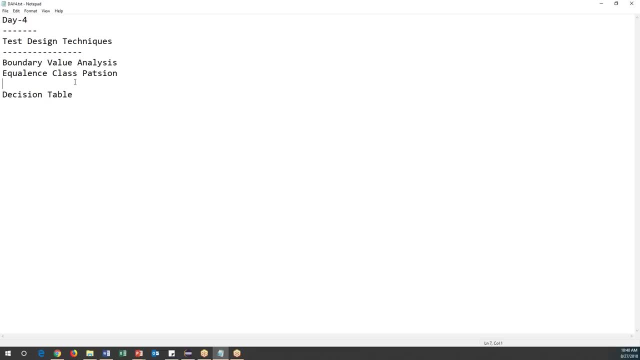 The next one is a state transition. This is another technique, So decision table will be discussed. The next one is state transition Sometime. This is also very important. So state transition diagram: you can just draw a small diagram to check all scenarios. 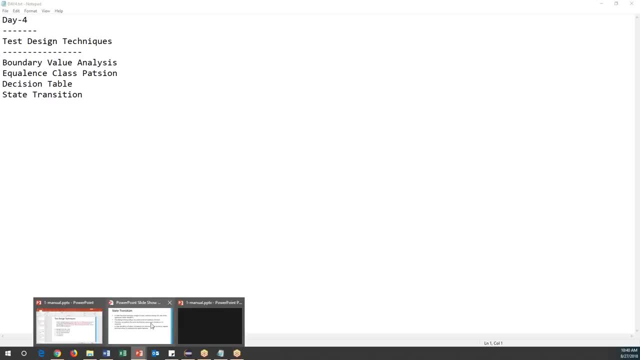 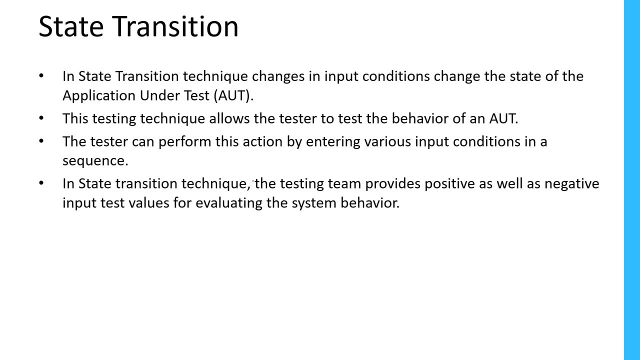 are covered Or not. Now let's see state transition diagram. This is all TV part I have just written here. You can just read it later. Very simple, Okay Now. by seeing example, you will easily understand What is this technique, how to apply this. 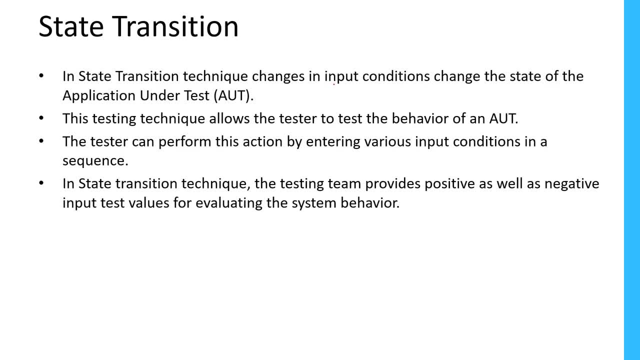 Okay, So in state transition, technique, changes into techniques, changes in input conditions change the state of the application under test. So here input conditions are keep on changing. Okay, Suppose let's say condition one: So, and so action should happen. There's a action one if the condition is to and so, and so action should be done. 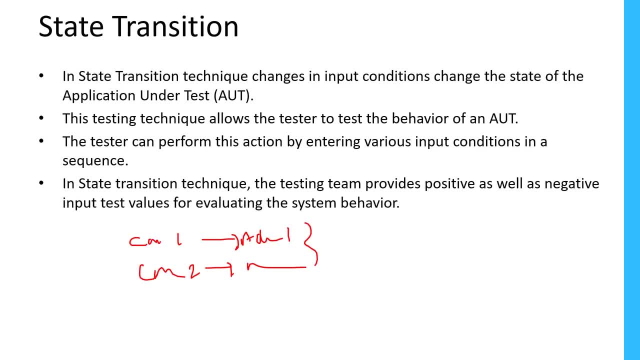 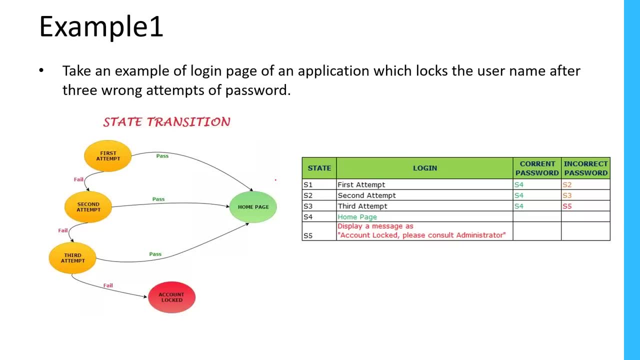 So this is decision table, but here this is not the case. If the condition is changed, the state will be changed. So let me just show you small example. So in this example- okay, so I have taken a login page example- again observe this how. 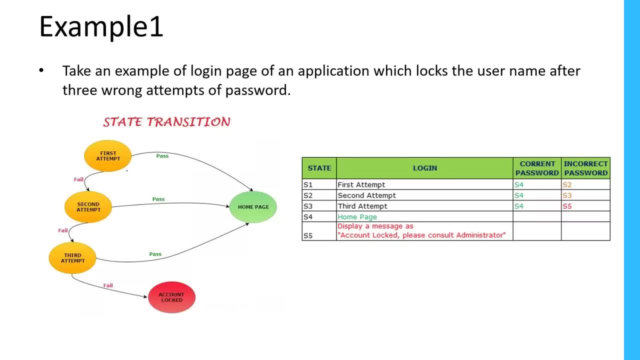 we can create a state transition type. We can see a few more examples also, So in the login page of an application. So So what is the requirement here is the application which logs the user name after three wrong attempts of password. So sometimes we can observe this in ATMs or some applications. If you enter your password three times wrong, it will lock your user. you need to again unlock and winterize the request and so on. right, So it will allow three attempts, but third time also, if you enter something wrong, automatically your account will be locked. 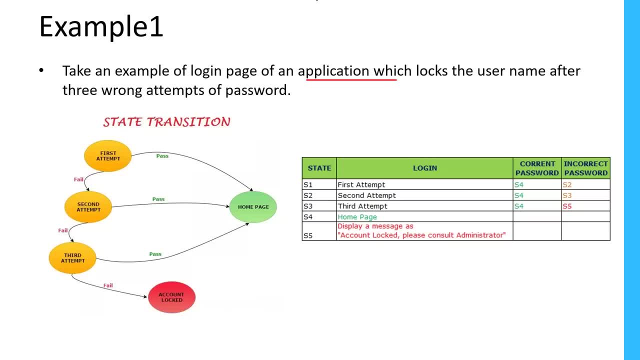 So that's a requirement here. Now let us see For this requirement, how to draw a state transition. So here we need to understand What are the states. Okay, what are the states and what is an action? So two things are very important. 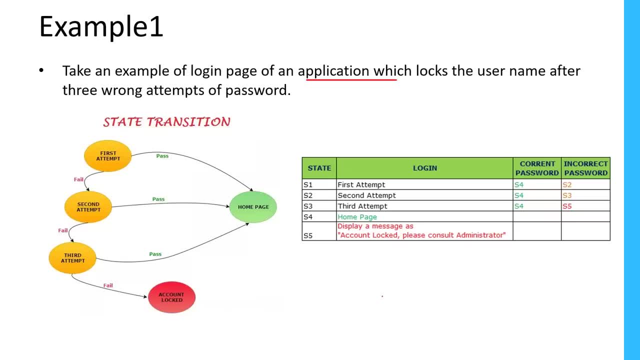 So first attempt, second attempt, third attempt, they are the actions. So first time we will enter the path, username, pin number, Let's say pin number. first time, that is action. second time, also action. third time, also action. So three attempts, we can say three attempts. 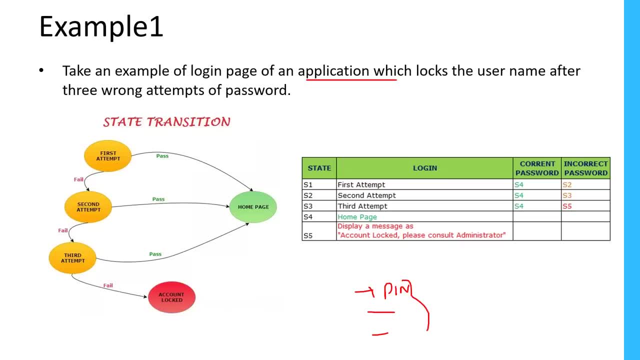 Now let us say we have written three different boxes: first attempt, second attempt and third. Suppose first time attempt itself is passed. and then I should go to home page. Suppose first attempt is failed, for example. Now what I should do now. first attempt is failed, second attempt: 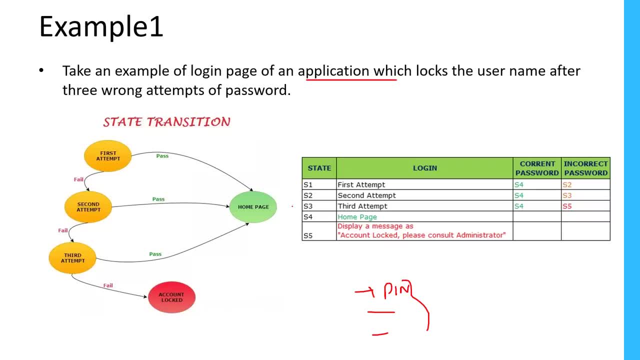 I need to do in the second attempt. If I give right input, then it will go to home page. even in the second attempt. If I give invalid input, it will go to third attempt If it is second attempt is failed. Now in the third attempt, if I give correctly, 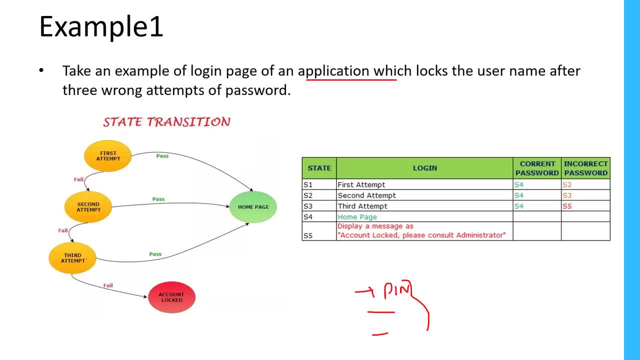 then it will go to home page or even in the third attempt, If I give invalid input, account will be locked. So this is the state transition diagram. Okay, and based on this, we need to write a small table here, We need to draw a small, small table here. 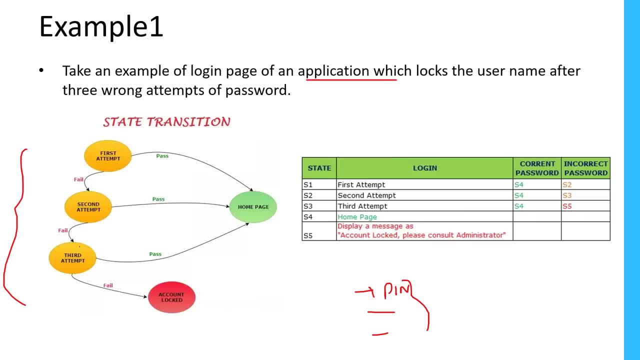 Let's see how we can do that. So this is simple example in three attempts and every time state is changing. Okay, So if it is a pass, first attempt is passed. state is different. If first attempt is failed, another state will go to next stage. 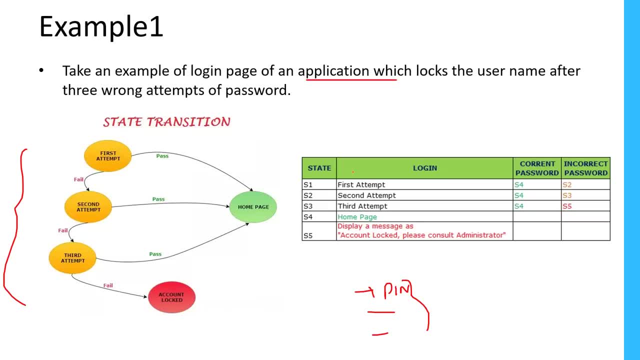 Now see this table. So I have listed out a few columns here. states will be in the one column and logging correct password and correct password. So means invalidate, validator and invalidator. Now let us see What are the states here. I need to list out the first, all the states each. 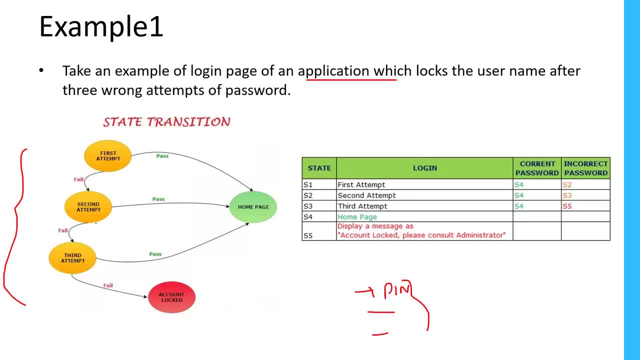 and everything is a state here. Okay, So first attempt, second attempt, third attempt. not only this, even go to home page. account is locked. These are also states. So I have listed all the states here based on the trans state transition diagram. So s1, s2, I name it as a. this is called. 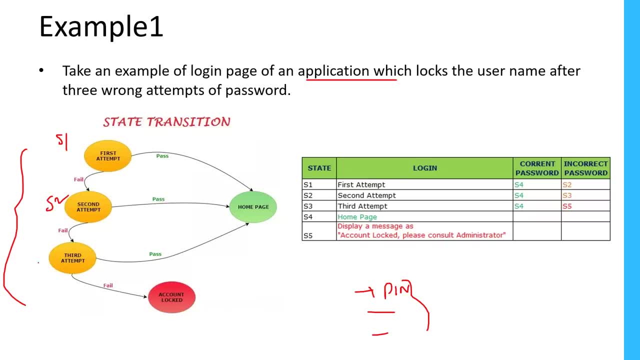 I name it as s1 and this is, I name it as s2, and this is s3. and let's say: this is s4 and this is s5.. Okay, five different states now, Yes, one. What is that? s1, first attempt. 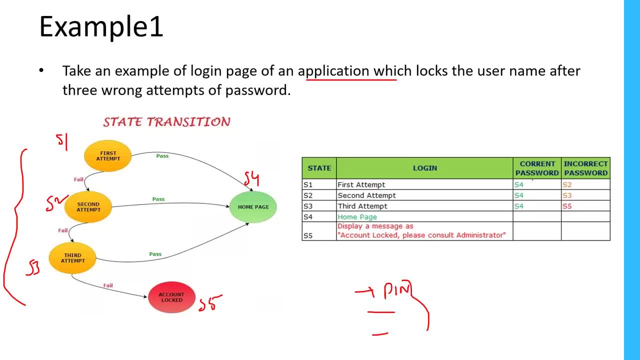 So when I do the first attempt, okay, if I give the correct password, what is the next state? It should go Yes. for what is an s4 home page? It should go to s4 home page. It should go so from here to here. 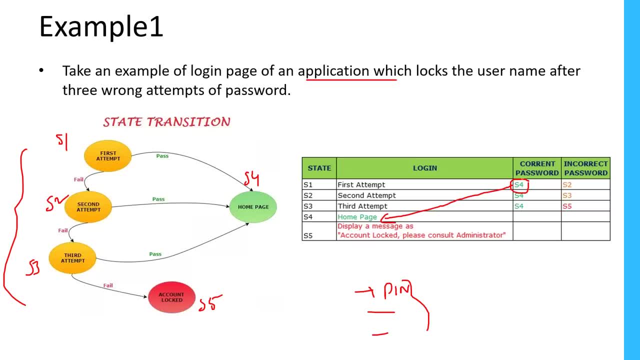 It should come in the first attempt. If you give the correct password, what is the state? It should change home page. that is s4.. It should go suppose the first attempt. if I give invalid password, then what is the state? You should go s2. s2 represents 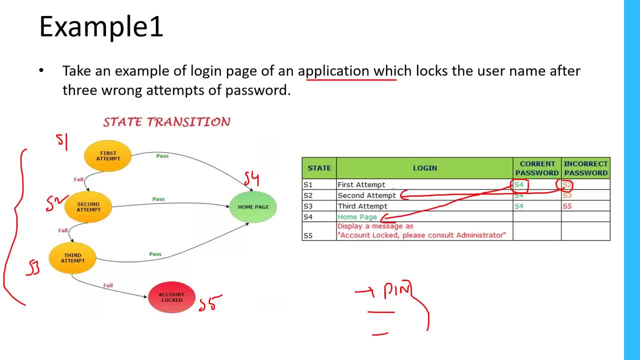 Second letter: Okay, in the first attempt if I give right password, then directly it will go to s4 state. and if the first attempt, if I give incorrect password, it should go. the second attempt, that's called s2 state. Okay, one coverage then come to the s2 now. 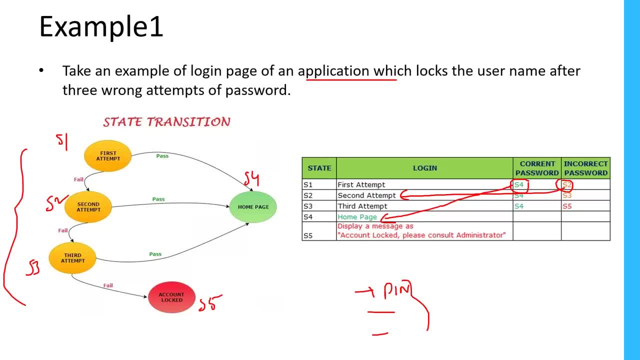 So in the second attempt, if I give right password it will directly go to s4 home page. fine, Suppose, if I give invalid, again it will go to s3 state. Okay, third attempt, the second attempt: if I give invalid input, it will go to third state. 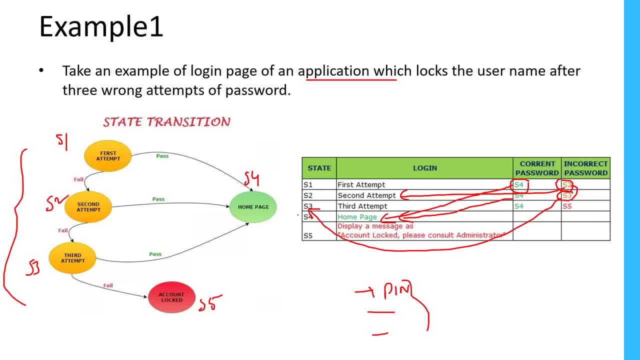 So here these are all states. it will representing the states. Now s3, third attempt. in the third attempt, If I give right input it will go to s4 home page And if I give invalid input it will go to s5.. 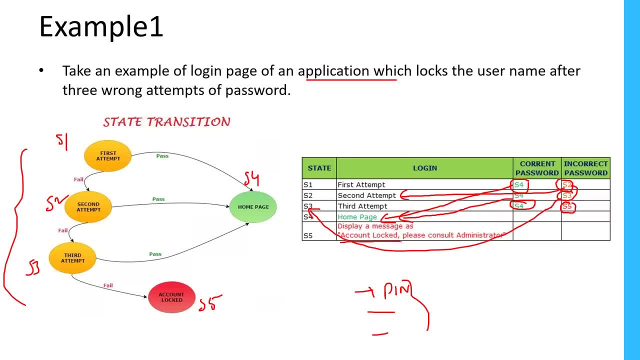 What is an s5 here? Display message called account is locked. So that is the final status. Okay, So there's a final state. So we have only five states based on the state, automatically based upon the action We perform, based upon the data. 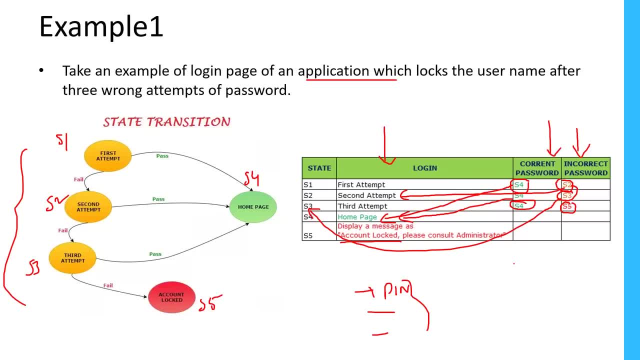 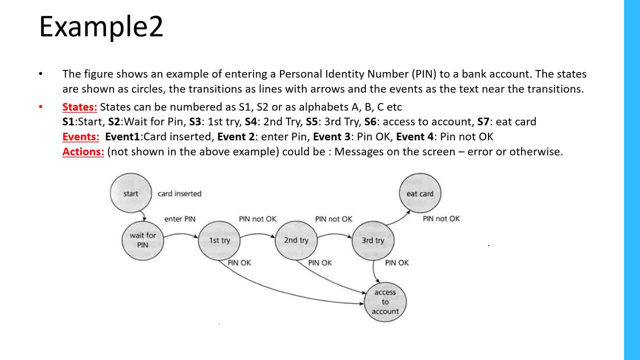 We provided here, The state will change accordingly. Okay, So, if I remember this diagram, you can just easily design this particular table. We'll see one more. So this is a ATM example. So in this example, this diagram clearly demonstrate our ATM process. 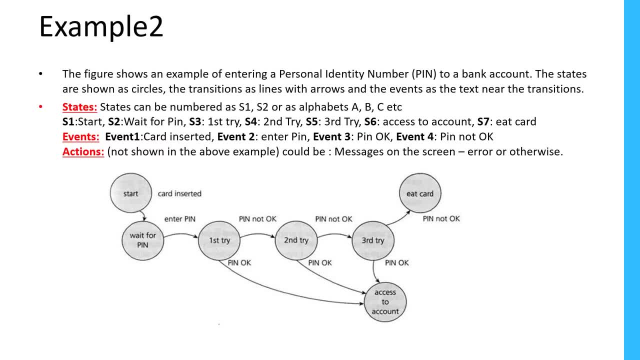 So normally when you go to an ATM machine, first we will insert the card. that is one state So immediately what happens. it will ask you a pin number, So it will wait for pin number. So the first time when it enter the pin pin is okay. 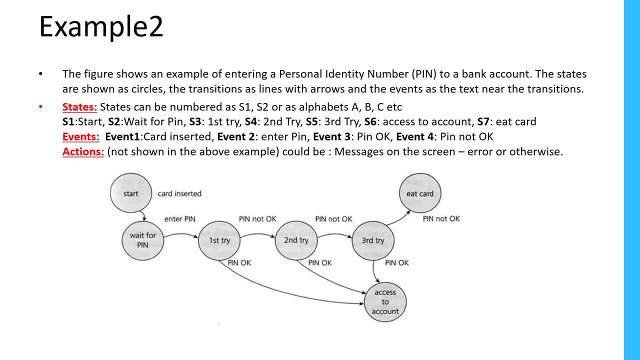 then we can access the account. if pin is not okay, Again it will go to next state. second right will ask, and the second time. pin is okay, Then go to access. a pin is not okay, Then go to third right And the third time is okay. 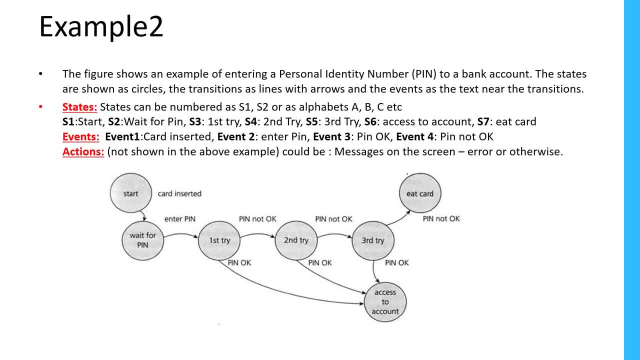 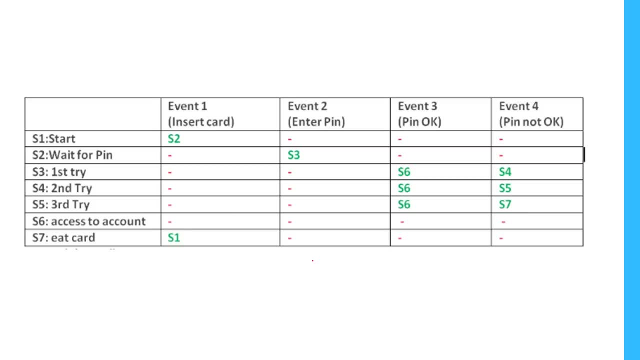 Then access to account. If we third time is also fail, then your card will be gone. So this is the state transition diagram. So now, based on this, we can prepare the table. Now let us see So here, what are the states we have here? starting waiting? 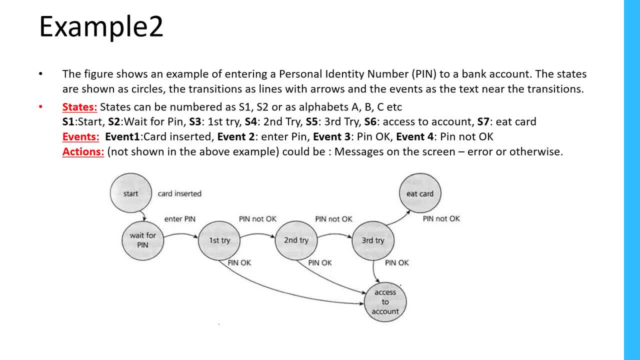 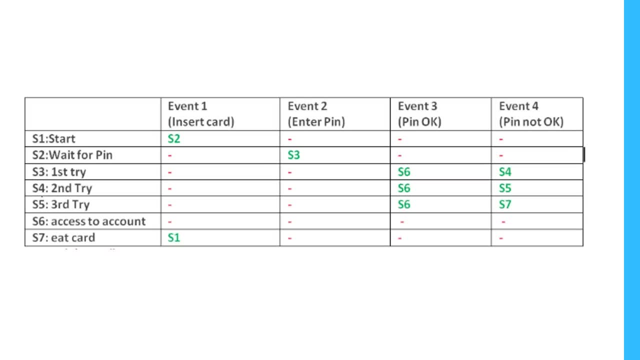 for the pin. first try, second try, third try, eating card access account. everything is the state, everything is the state. So here I mentioned all the state, like s1, s2, s3, s4, s4, everything. So s1 is start, s2, wait for pin, s3, first try, s4, second try, s5, third try, s6 and s7. 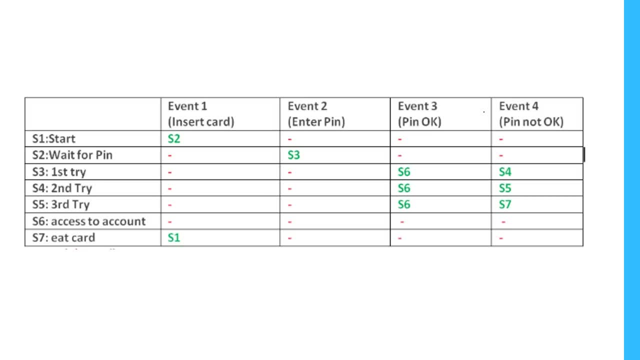 So each and every state I mentioned. now I have created a few more columns for event. Now let's see, when I start here. s1 state What it will ask you. it will just need to insert a card. So once we have inserted a card, 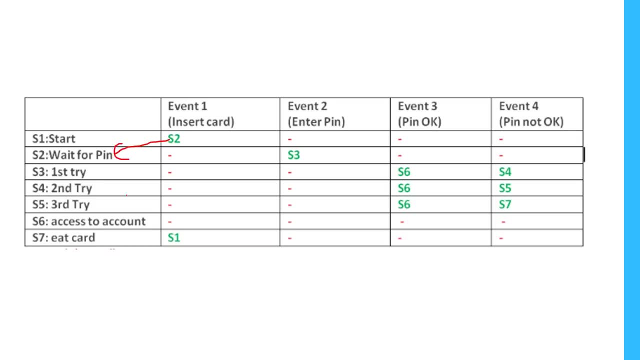 what is the next action? it go Yes to. it will wait for the pin. So here, okay, We don't need to do insert the card. So what is the next action? We do enter the pin. when I enter the pin here? 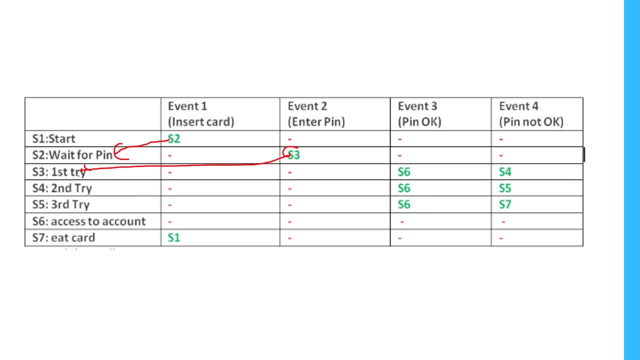 what happens? it will go to s3 state. So first try in the first try. if pin is okay, even three, then it will go to s6 access account. Suppose pin is not okay, Okay s4, it will go to second try Valid as invalid case here. 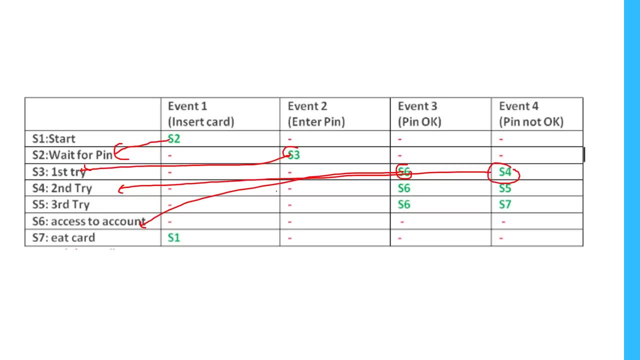 It is covered. and in the second try come to second try. So here all events Are there. in second try: if I provide pin is okay, we go to s6. as we pin is not Okay, it will go to s5 again. third try: again in the third try. 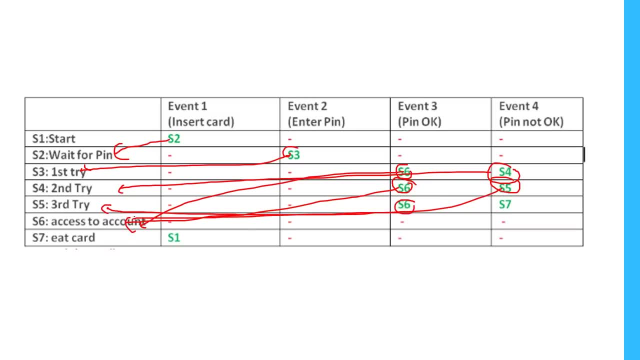 If a pin is okay and then it will go to s6 access, the account pin is not Okay, then it will go to finally last. Here is the card. Okay, So this is again state transition diagram. So everything is representing the states. 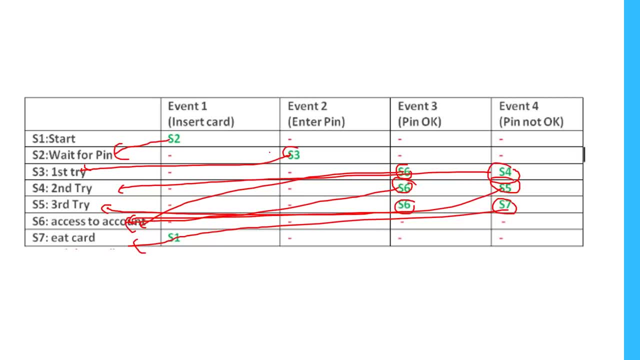 So there is a lot of difference between decision table and decision tables, The main focusing on the conditions and actions, but here, the main focusing on the states, how the states are changed. state and event, what in which state and what is the event we need to do? 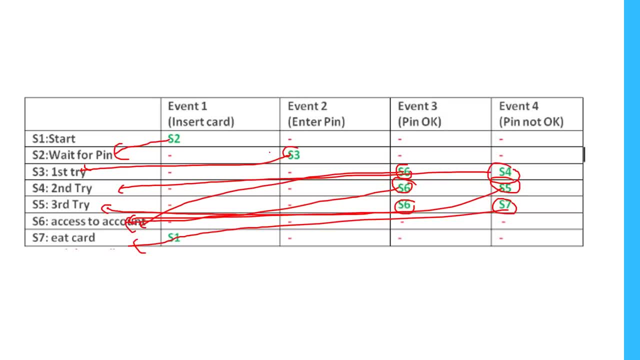 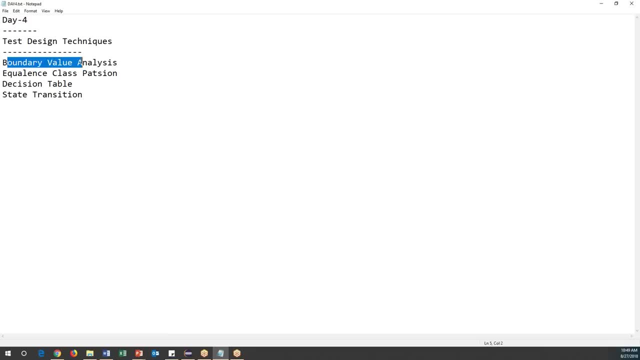 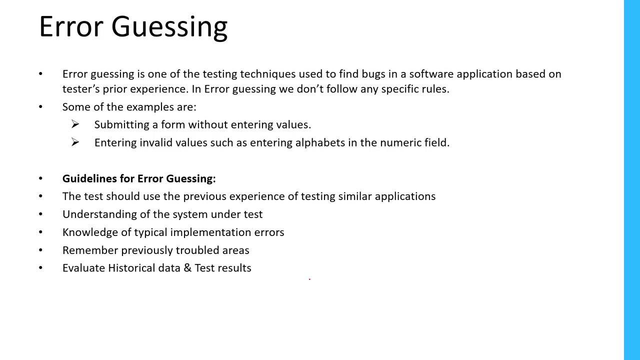 So that's the main, focusing on state transition diagram. So this is also very important technique. So boundary value analysis, equivalence, class partitioning, decision table and then state transition diagram. Now let's see one more technique: Error-guessing. so error-guessing is mostly unit testing technique. developers will use this. 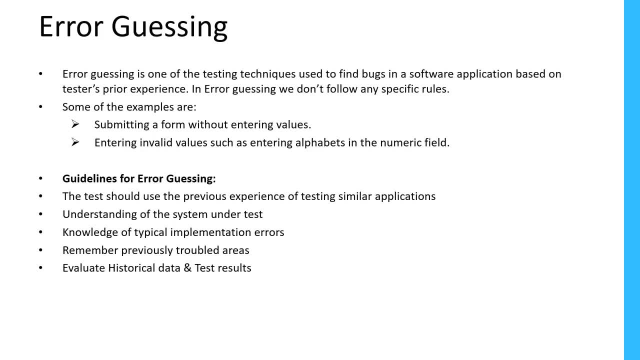 This is not exactly a small kind of technique. We can just say error-guessing is based upon our experience, previous experience and before itself. we will get something, suppose, if I do something so and so and maybe this error may come. so that kind of expectation. 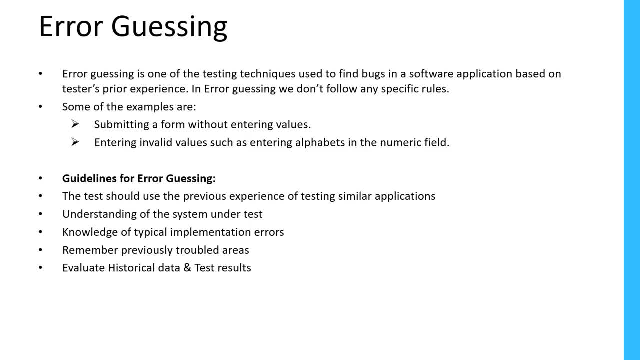 We should have. based on our previous experience, We will guess the errors. Okay, but as per the requirement, we don't do anything here. Just if you do something. okay, if I do some certain kind of action, there may be some error will come. 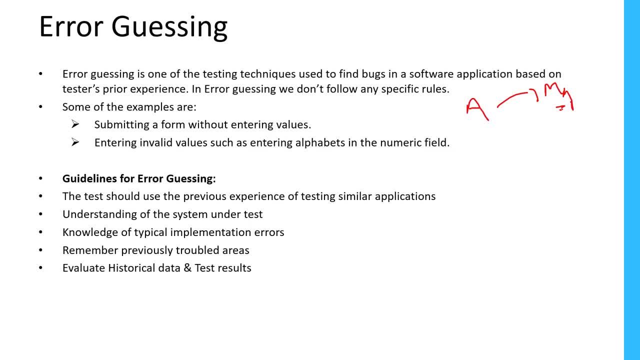 So let's test this scenario So like that, we can assume ourselves: Okay, that's called error-guessing. So error-guessing is a one of the testing technique used to find the boxiness software application based on Testers priors experience. 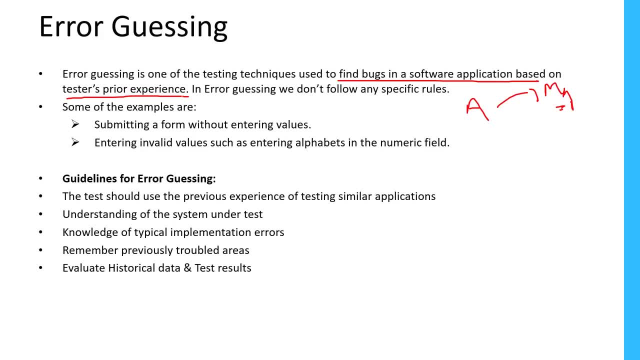 So if you are already working on some applications, you will get have some, some experience. Suppose, if you are working work on some banking applications. so suppose tomorrow if you are testing a banking application, some other new bank application, you have a some kind of thought process. 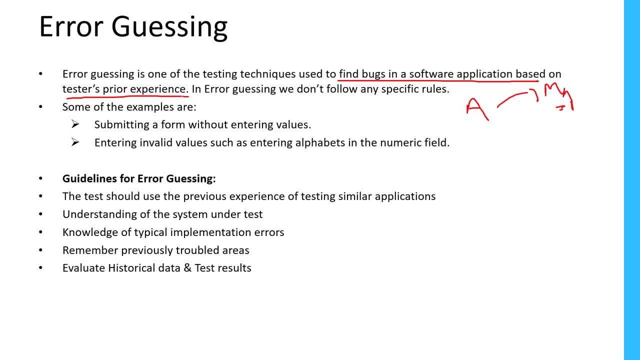 Like if I do some action it should come like this. So if I do something like this, there are messages should come up. I do something like this transaction successful. So these kind of thought process you will have if you have certain experience on the same kind of projects. 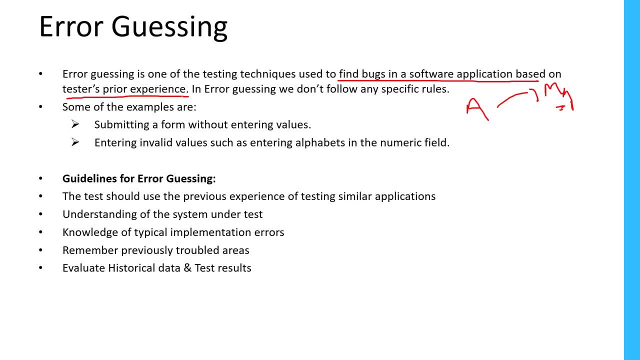 So, based on that experience, you will test the application. that itself is an error-guessing technique. So here, this is not a written or oral format. here We don't have any diagrammatic on tablet format. This is just your thought process. 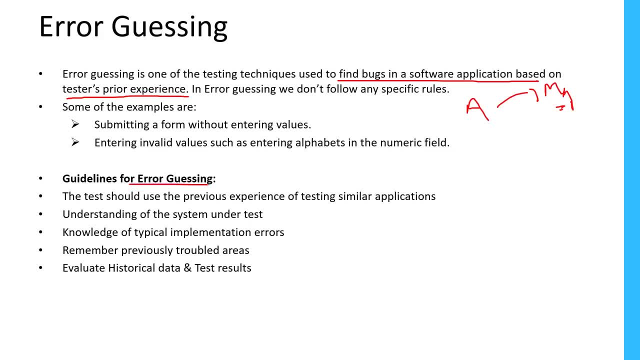 Okay, So here the what are the main guidelines. in error-guessing means, the tester should use the previous experience of testing similar applications and understanding of system test knowledge of typical implementation errors. Remember previously troubled areas, Suppose if you are working on previous projects. 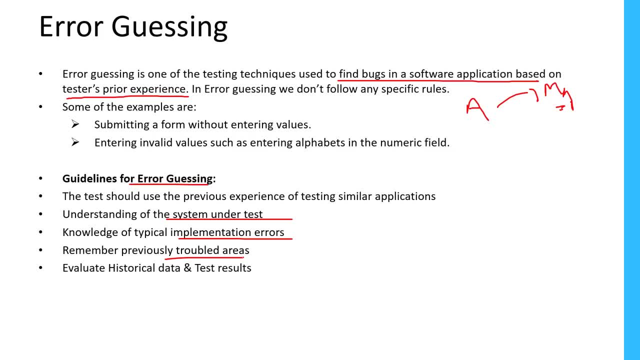 so you will face some kind of challenges and issues and troubles and, based on that experience, in the new application you will utilize that experience And you value to historical data and test. So these are the few guidelines we need to follow while you are applying error-guessing. 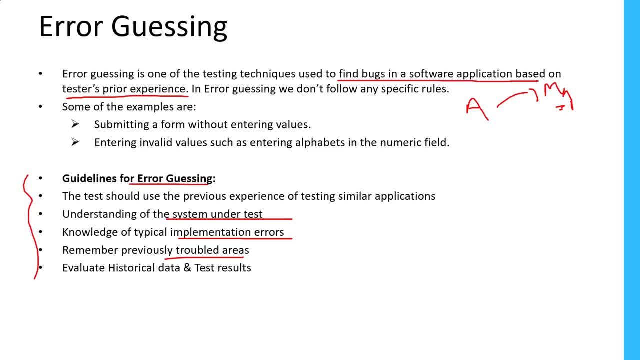 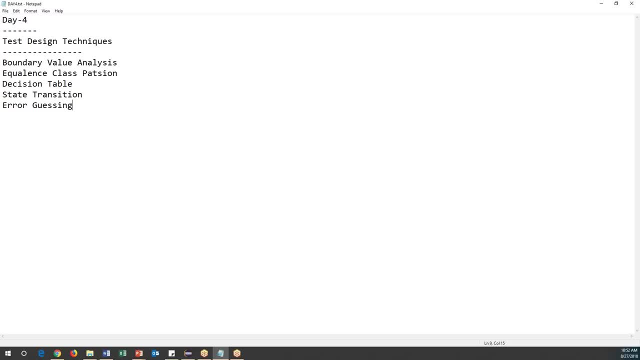 So this is also one of the techniques. So how many techniques we discussed? here is Five techniques, So boundary value analysis, equivalence, class partitioning, decision table, state transition and error-guessing. These are the five test design techniques at the time of for preparation of test data. 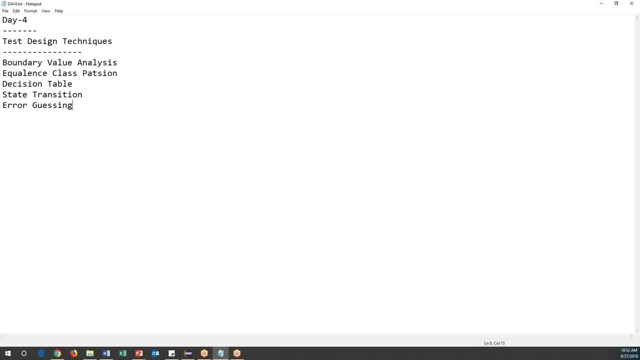 or testing. we use these test design techniques. So what is the main usage of test design techniques? to reduce our effort and with minimum data coverage will be more. Okay, that is the main Objective of our test design techniques. Okay, so is it clear. 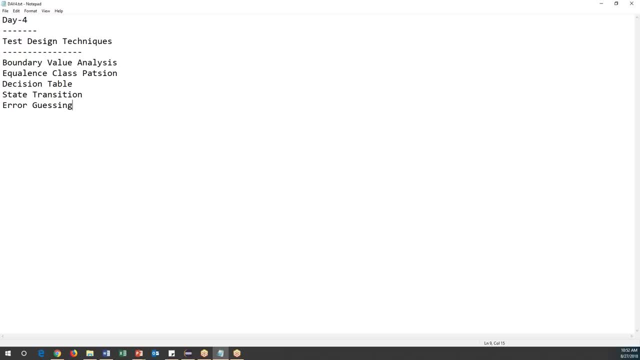 Tulsi. Yeah, yes, It's not clear, sir. I'm in the window, sir, Fine, So hello. So please confirm in the chat window, Sir, my voice is not being heard, Hello. Okay, Now let us discuss about few things. 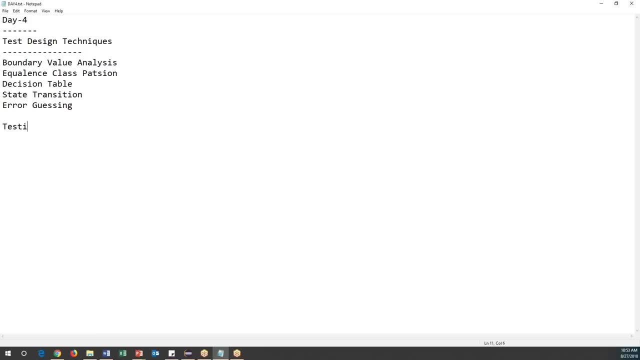 Different testing terminologies. Okay, So different testing terminologies. We already discussed about functional testing, non-functional testing. So under function testing we have so many types of testing and a non-functional. We have also discussed so many types of testings here. 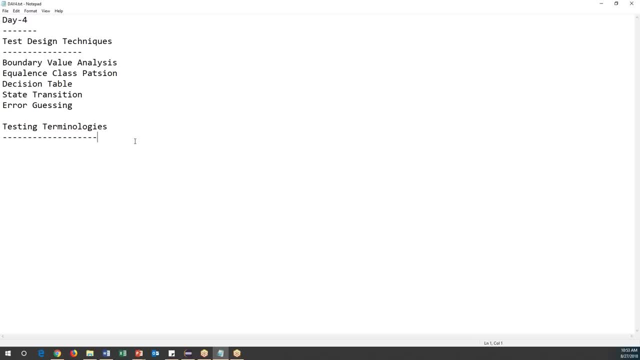 I am talking about terminology, because in the day-to-day life we use these terms very frequently in the real-time environment. Okay, so, for example, e-testing, regression testing, ad-hoc testing, mock testing, exploratory testing. So these are the terms. 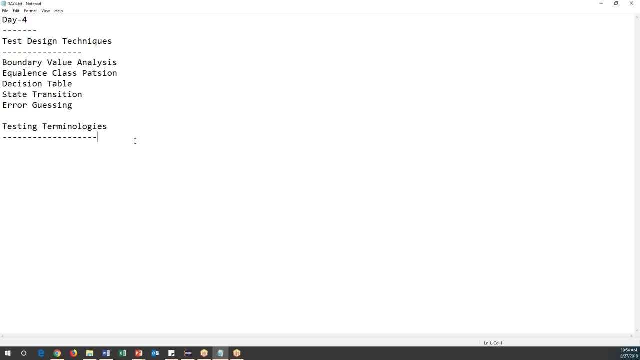 So we commonly hear very frequent. So when you hear those words we need to understand. suppose somebody asked you to do ad-hoc testing, So you need to know what is ad-hoc testing, how to perform ad-hoc testing right. 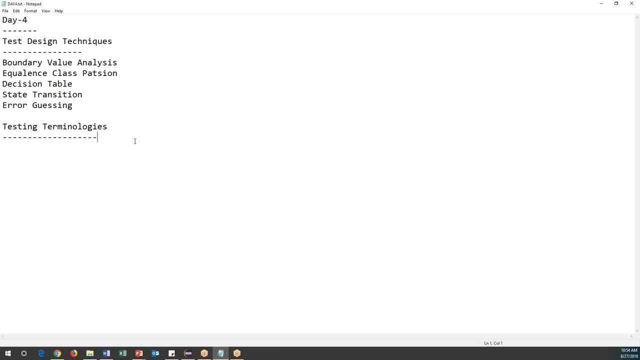 So similarly, if I somebody asked you so- to regression testing, and then you should know about what is regression testing and what is retesting, What is exploratory testing. So these things you need to have an idea. So now let us discuss about testing terminologies one by one. 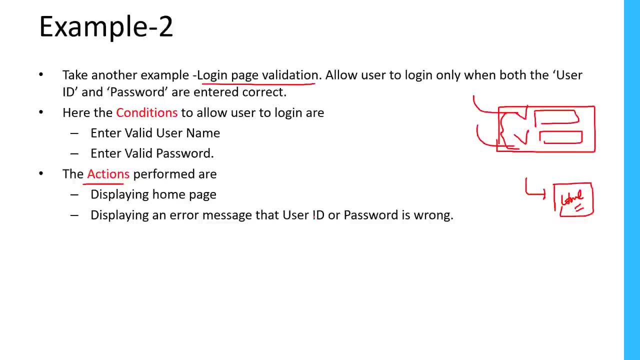 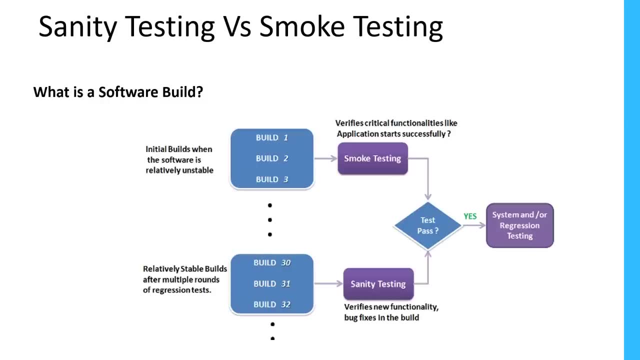 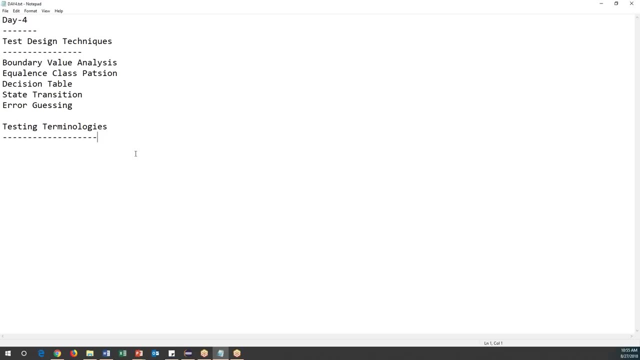 Let me share a presentation now, Just a minute. So now let us discuss about testing terminologies. Let's start with the sanity testing and smoke testing. first one Very important in interview perspective or in examination perspective to go for any Certification course: ISTQB. 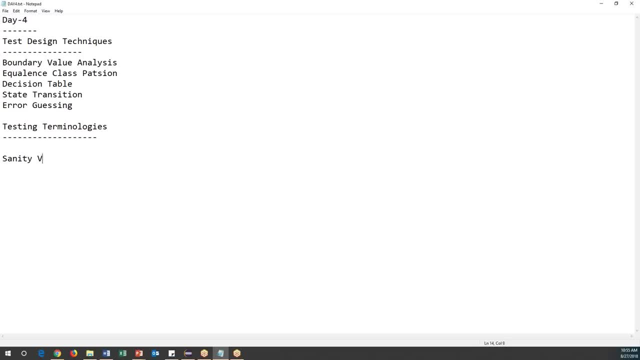 These are the very important questions. Sanity versus smoke testing is the first one, Sanity and smoke testing. So why I am collecting these two? because almost everything is same. It's a small minor difference, but almost people will feel very same. So sanity and smoke testing. 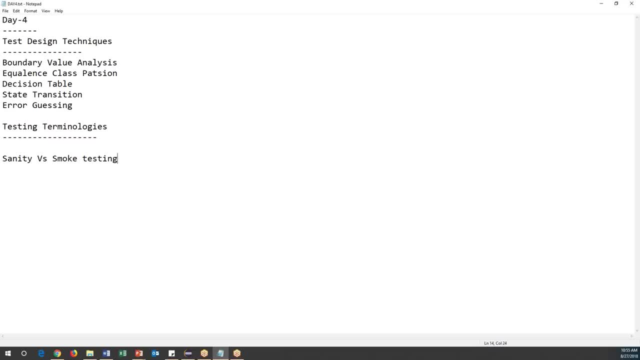 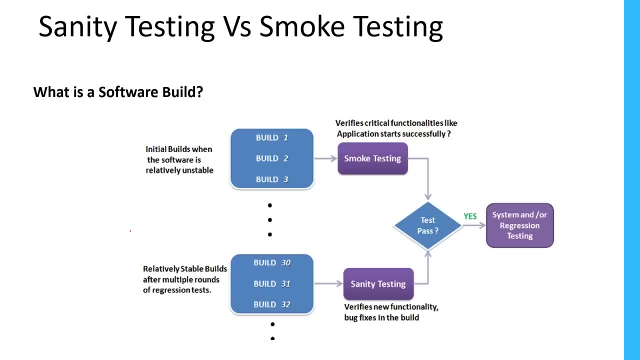 So let us see what is sanity testing, What is smoke testing. So, in this small, small presentation: So what is sanity testing and smoke testing? Let's see. So, before understanding sanity testing and smoke testing, we need to understand what is the build software build. 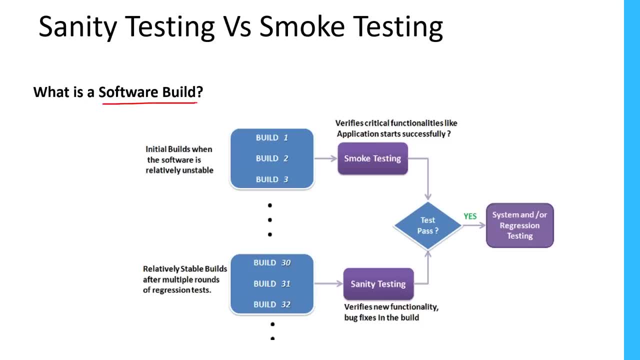 So the software build is nothing but a developer will create a number of programs, right? So the why they will create a programs to develop the software and but they don't provide the programs to the devour to a team testing team. So testing team don't test the programs. 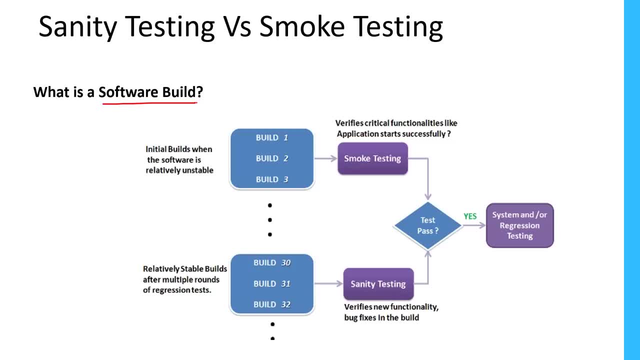 So they test the software completely. So they need a build. So the build is nothing but an integrated product, integrated program. All the programs will be integrated and make a package format and executable format. So that is called as a build, software build. So tester is always gets software build for testing. 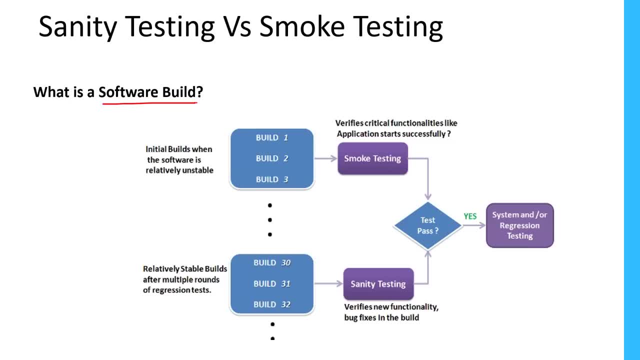 Okay, Now let us understand what is sanity testing, What is smoke testing? Very simple, Let's understand. So developer will provide you multiple bills, not only one, two, three, four. So there are n number of bills, because every bill having certain number of issues. 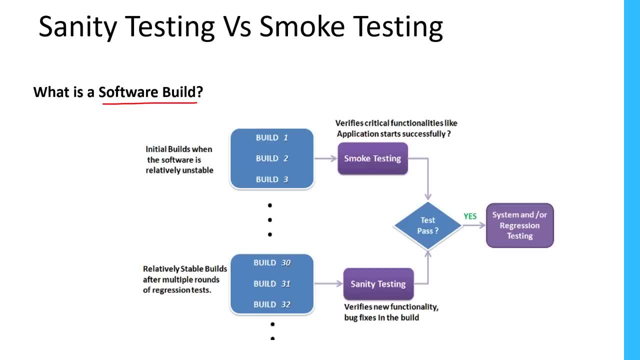 We will report them to the developer, and developer will fix those issues and they will again deliver the new build. So this is a common process. entire life cycle: This is a common process. So we will get day-to-day every time new bills whenever we reported any issues. 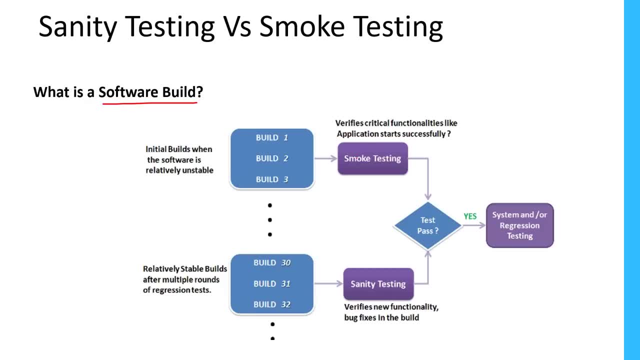 and sometimes they will Add a new functionalities also in the same build. along with the issues, along with the fixes, They will also add some more new functionality in the build and they will provide us the bills. Now when sanity and smoke testing come into the picture, 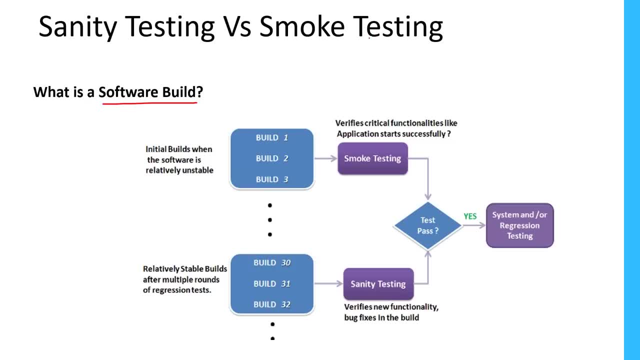 let's understand this very clearly. So sanity- smoke testing is the first entry point and sanity is the next point. So smoke testing verifies critical functionalities like applications start successfully. So here smoke testing will done the early stages. So, for example, whenever the developer start giving the bills, like build one, two, three, first a few number of bills will not be stable. 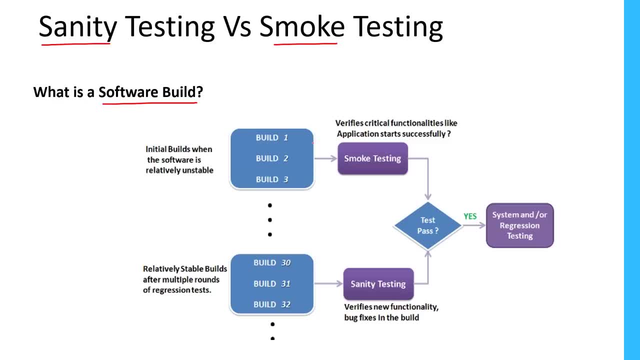 Okay, so that is common thing in every environment or every company. So first a few bills will not be stable. So even sometimes we cannot install those bills, So the both the bills will be broken. So in those cases we need to first verify the critical. 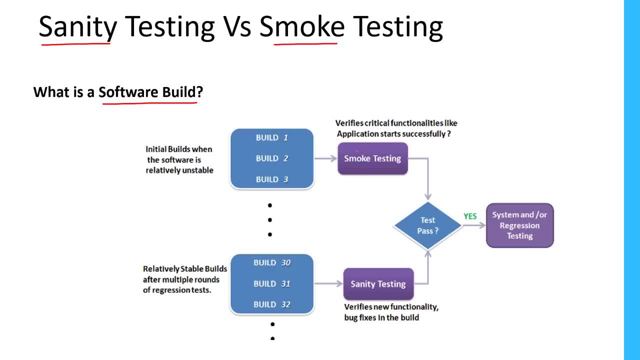 critical functionalities. So, like our application or build is properly installed or not, or if it is installed, it's giving the pages properly or not, All pages are web page. If it is a web based application, all pages are home screens and everything is comes or not. 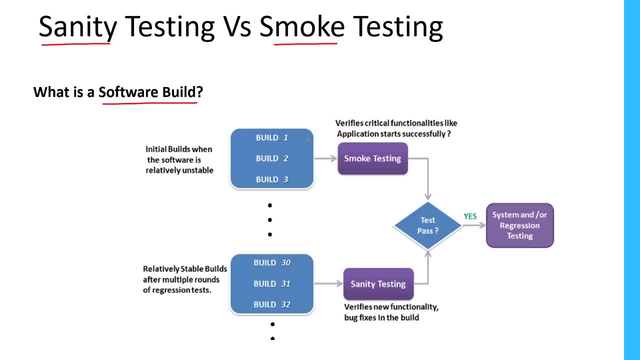 So they are very critical. So before starting the testing at the initial level, we do testing called as a smoke testing. So during this testing, what testing we do? what we do is we will just install the build In our environment and verify where the basic 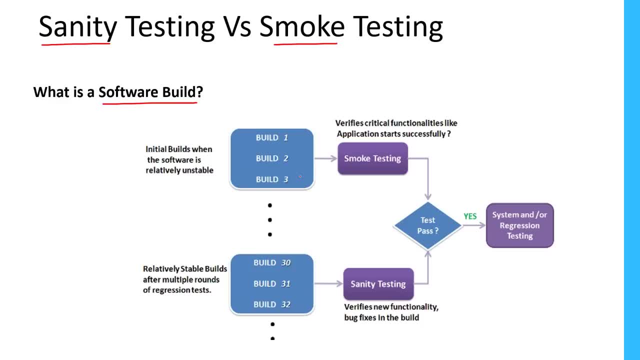 or very critical functionalities are working fine or not. That is called as a smoke testing. We do this in early stages, like initial bills, when the software is relatively unstable. So whenever the developers start giving the bills at the initial level, we perform smoke testing. 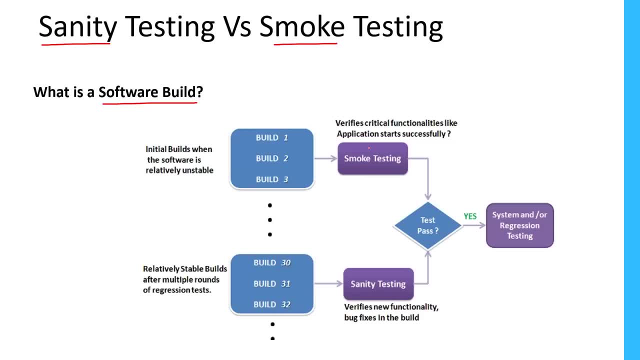 So it focus more on critical functionalities are working or not. So after some time, or after so many bills, slowly the bill becomes a stable. Okay, slowly the bill becomes a stable, So you are able to install your bill and the critical functionality also works fine. 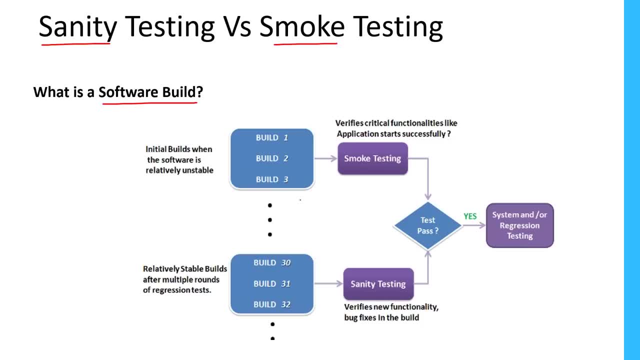 Okay, everything goes well. and after some time, you, whenever you receive the bill, again. this is also. these two testings will be done as soon as you receive the bill. Okay, very important thing: smoke testing. What is the similarity between these two? is smoke testing. 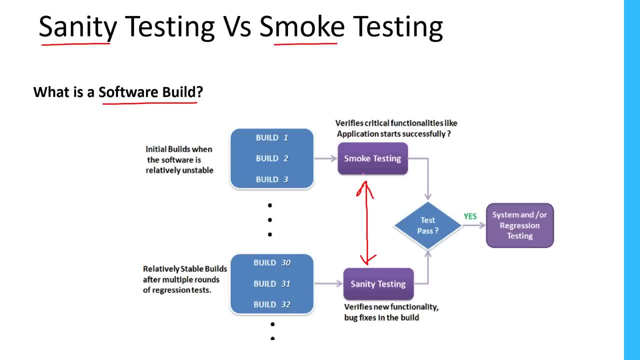 You will conduct smoke testing and sanity testing at the same time whenever you receive the bill from the developers. but the small difference is smoke testing will do at the initial level on critical functionalities working or not, and Sanity testing will be done later stages. The main functionalities are working or not. along with this set, a number of bug fixes are also available. 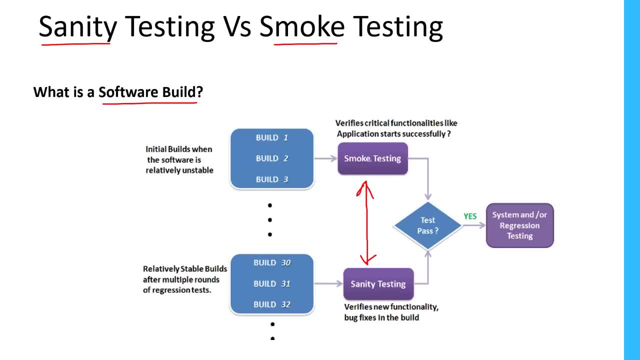 or not. that also We need to make sure. that is Sanity testing. So smoke testing is only focusing on critical functionalities like build is installed or not properly, or the main screens are working or not. That is a scope of smoke testing. When you come to the Sanity testing, 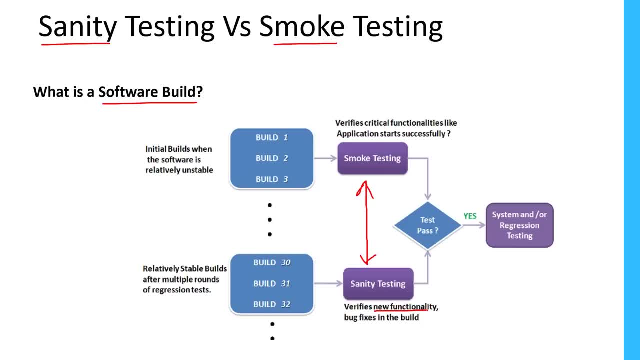 we will mainly focusing on verifying the new functionality along with the bug fixes. Sometimes we are getting the multiple bills right to why we are getting these many bills? because every bill is having set a number of fixes- Bug fixes along with the new functionality. So to me to verify them in each and every bill. 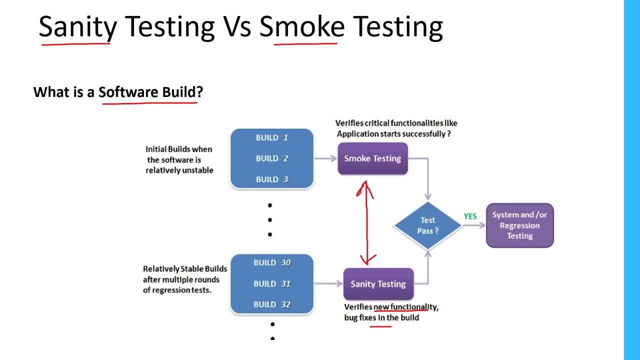 So that comes in the sanity testing. So smoke testing, sanity testing, both are conducted at the time of receiving the bill from the developer and smoke testing will be there in the initial level, initial stages. We need to focus on more critical functionalities, but sanity testing is more focusing on new functional testing. 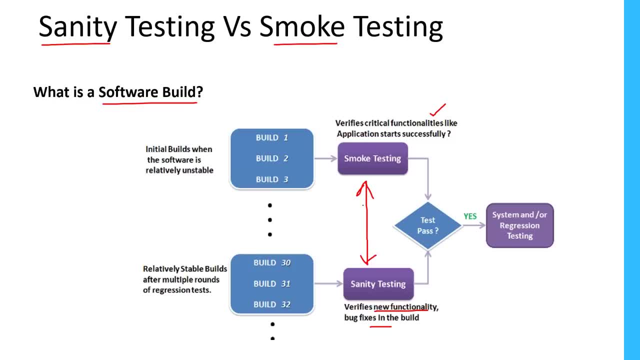 and bug fixes, Whatever they provided in the bill. So if one of them is fail at the smoke testing is fail or sanity testing is fail, We will reject the bill. So we don't accept the field bill for further testing. So the developer need to provide at the new bill to us. 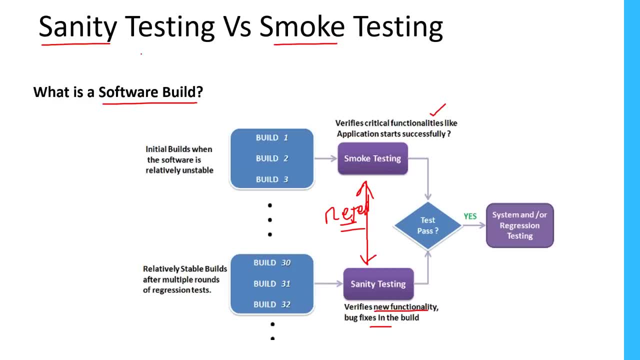 Okay, so that is called sanity testing and smoke testing. So both are basic functionality testing is. there are multiple names. We have build verification test or tester acceptance test, PAP or build verification test. This is also called as a initial testing or we can sometimes we call shakedown testing. 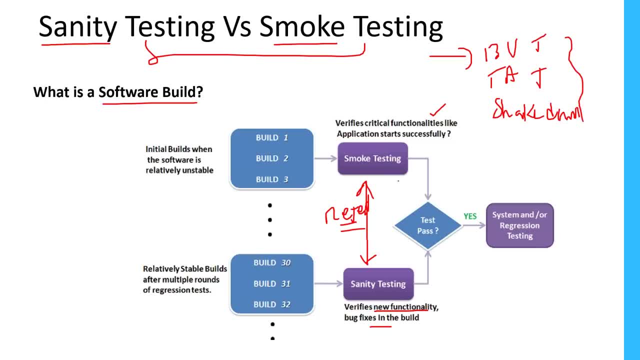 Okay, so multiple names we have. so smoke testing and scientists. smoke testing will be conducted at the initial level and sanity testing will be conducted at the later stages. smoke testing is focused on critical functionality. Sanity testing is focused on the new functionality, along with the bug fixes. 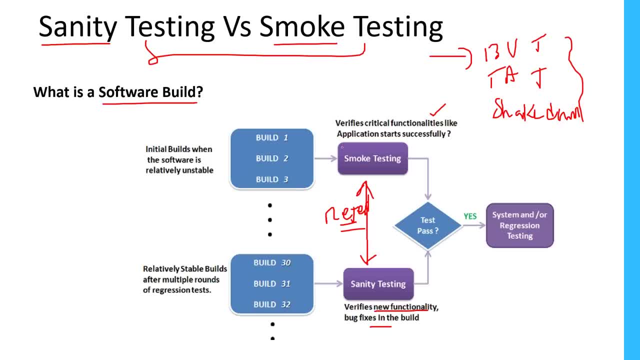 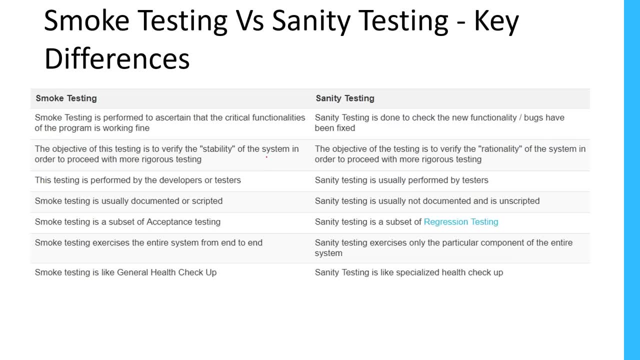 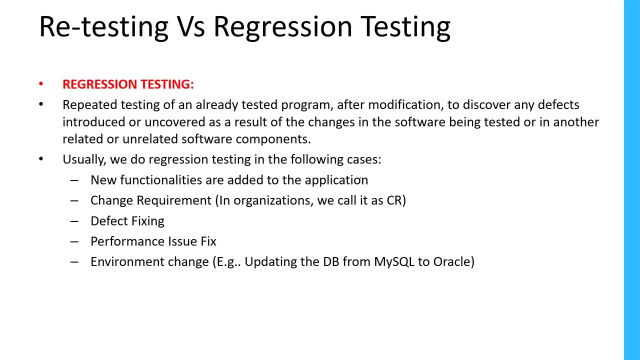 Okay, so this is a Main clarity on smoke testing and sanity testing. Now I have a list of few differences here. same thing. Whatever I have explained, you can just read this presentation. I'll send you this later. Now. so retesting and regression testing. 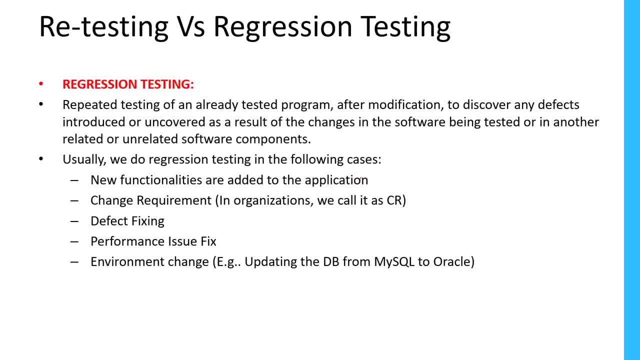 So these are the two also very important. So what is the retesting and what is the regression testing? Basically, automation is also came because of challenges we face during retesting and regression testing. So let us see what is retesting and regression testing. 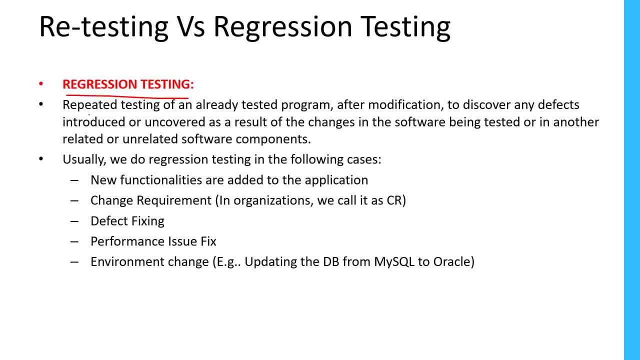 So first to talk about regression testing: repeated testing of an already tested program After modification to discover any defects introduced or uncovered as a result of the changes in the software being tested or in any other related or unrelated software components. So what does it mean is repeated testing of an already tested program after modification. 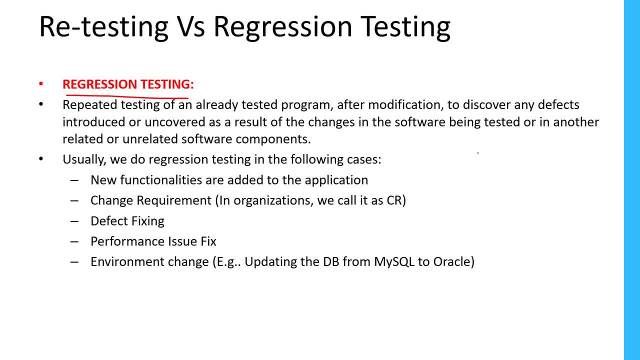 So let me give you one example. So we are testing a bill, Let's say bill number one. We are testing it, We found some issues in this and we reported to the developer. Okay, So what the developer will do is: developer will provide you one more field. 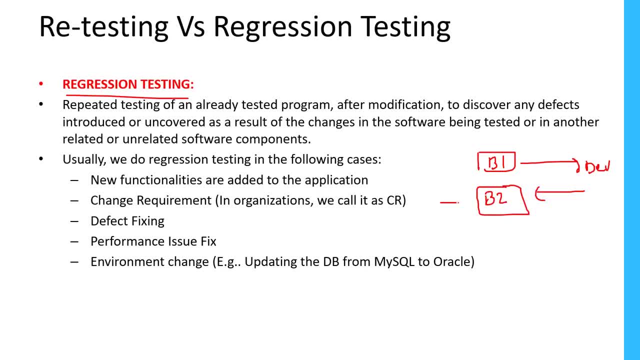 So let's say bill number two. So in the bill number two what we will need to verify now, whatever we already tested in the build one, Okay, the same thing again. need to test it here, because in the build one we found an issue in that. 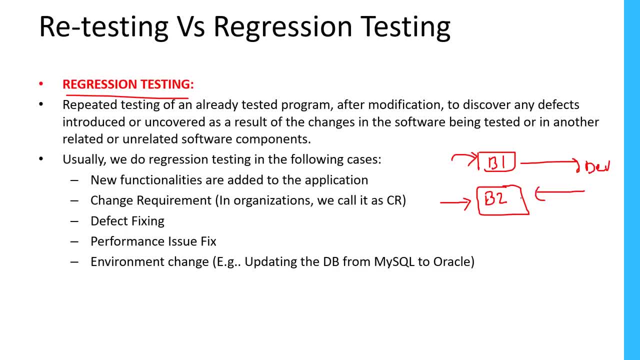 so we reported that issue to the developer. but in the build two we get the fix for that. So what we need to do, we need to again repeat the same test case. So that's the same here: repeated testing of an already tested program. That means already tested functionality in the build one again. 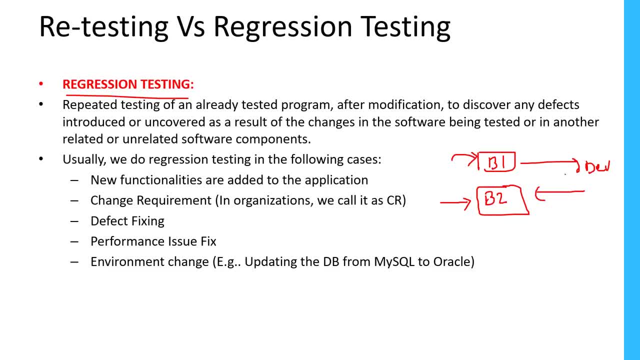 We need to test it again after modification means after applying some changes, after fixing the defect, So discover and any. the main intention is to discover any defects introduced or uncovered as a result. So the main intention of regression testing here is testing the same thing again. 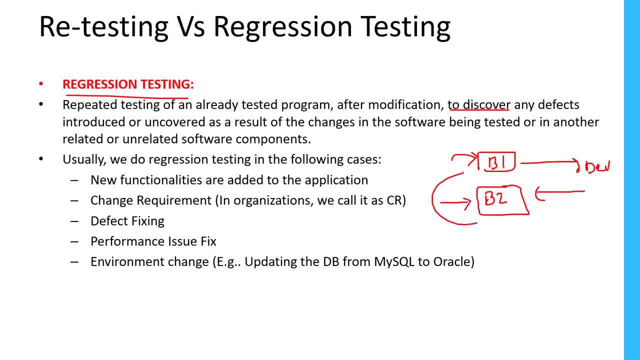 because of this change, there should not be effect on other functions. That is a main objective of regression testing. There is small thin line difference. is the retesting and regression testing. Okay, please focus on this: regression testing, mainly focusing on side effects, suppose. 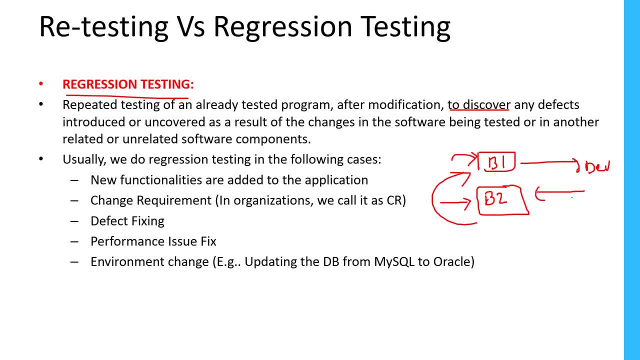 Okay, we have reported one issue to the developer. developer fix that issue. We have tested it again: right, that is called retesting. We have tested it again: right, second time, that is called retesting. but because of this, because of this change there may be, some other functionality will be broken. 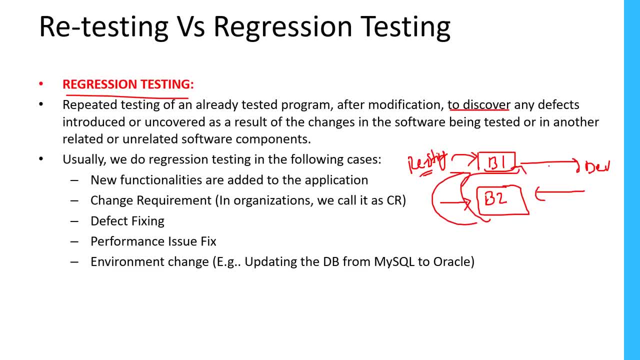 Okay. so if you test all of them- other functionalities also- that comes on the regression test. Okay. so retesting means testing only that particular change. whatever defect we raised, Okay, they have fixed it and we verified it. retested. that's called retesting. 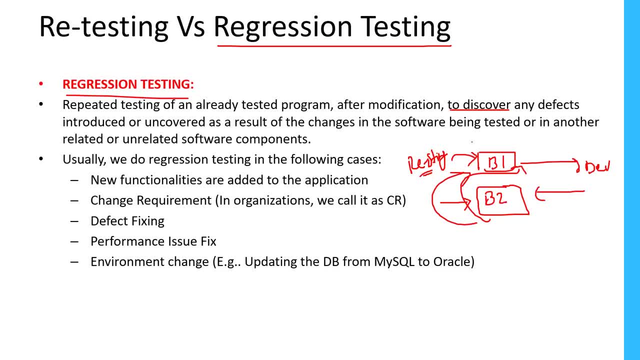 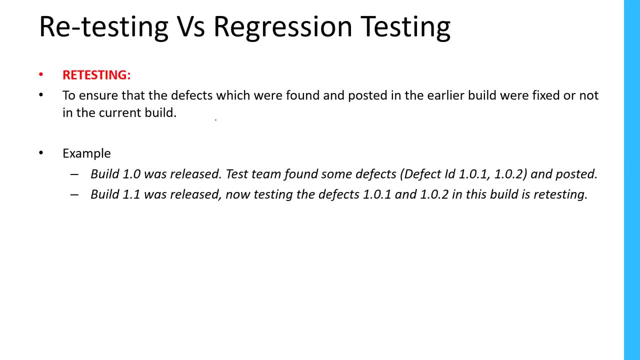 and because of that change, if there is any other dependent functionalities, if you test all of them also, that comes on the regression test. So coverage is very important. Okay, So let me just give you a small example: retesting is also retesting. 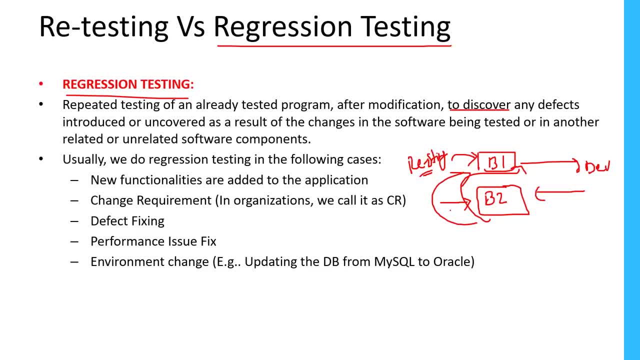 I already told you here itself, regression testing and retesting. retesting means testing the same thing multiple times. is called a testing after changes are affected and because of the changes, if there is any other functionalities impacted or not. If I also test those functionalities, comes on the regression test. small difference between retesting regression. 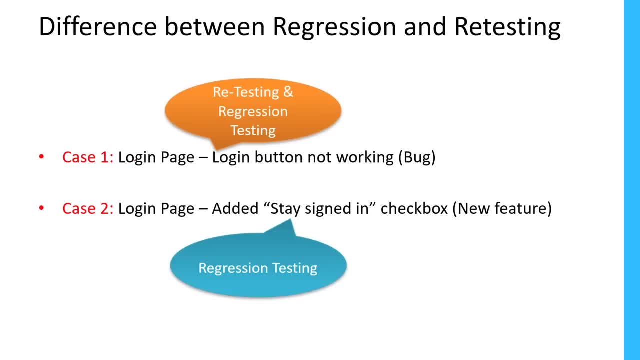 Let's see the difference here. Okay, So here it is very. it will give you the clear picture. What is the retesting and regression test? See now case one. So have a login page. login button is not working. Let's say in the login page: a login button is not working. 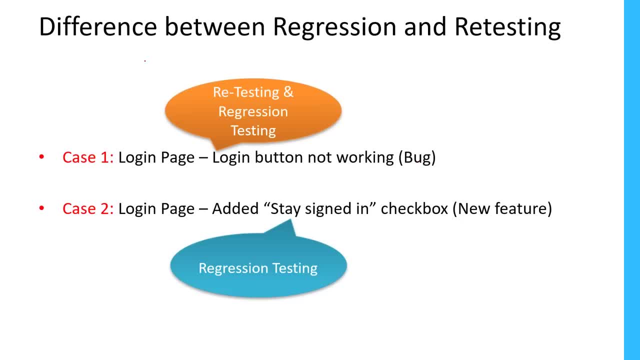 So obviously that is a bug. Okay, So in this suppose let's say this is fixed, So login button is not working, means this is fixed, So we do the retesting on this, because once it is fixed we do the retesting, suppose, along with this login screen. 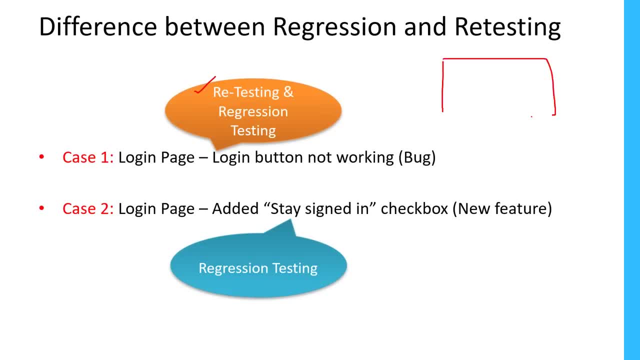 Let's say they have added one more functionality. Let's say: this is the login page. observe this carefully. This is the login page. So in the login page, this is a login button. This is not working. Okay, so we have reported this issue. 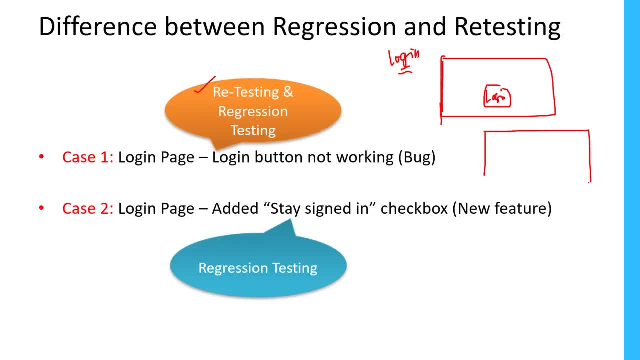 and they have given the new build. So in the new build, what they have given is, along with this login button, They have introduced one more checkbox here. Let's say they added: stay in, signed in. So this is a checkbox they have given. 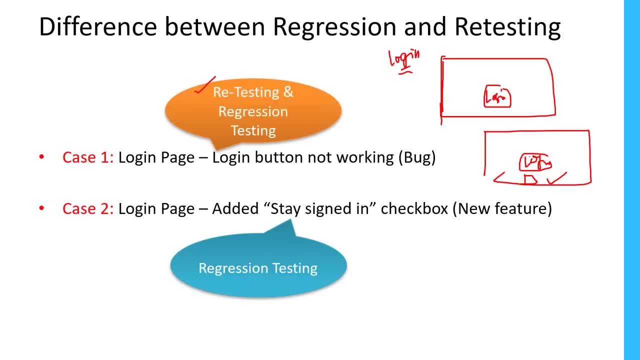 So if I test this only login part, whether this is working or not, that comes on the retesting. So along with this in the same login page. if there are any other items we have, if I test them also, because this is again depends on other other items. 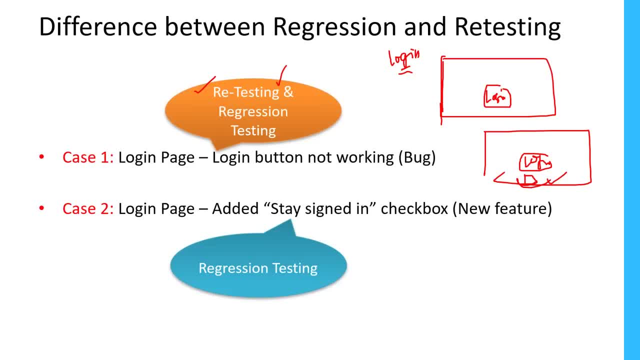 If I do the testing, these also, that comes under the regression testing. So dependent functionalities: if I test only that fix, that is retesting. If I test other functionalities which are depending on that particular fix comes under the regression testing. There's a simple difference between retesting and regression testing. 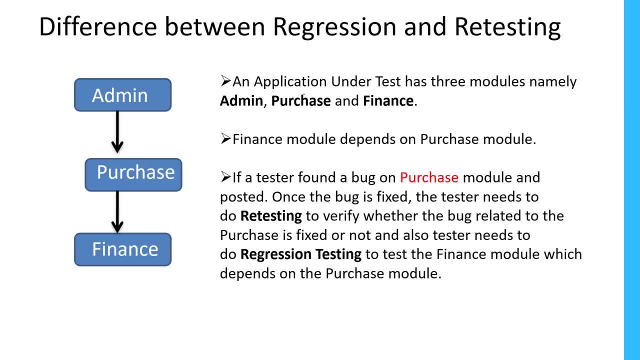 So I'll show you one more example. Let us say I have three different modules: admin module, purchase model, Finance module. in my project I have a three different functionalities in one application. I have three different functionalities: admin, purchase and finance. So admin, purchase and finance. 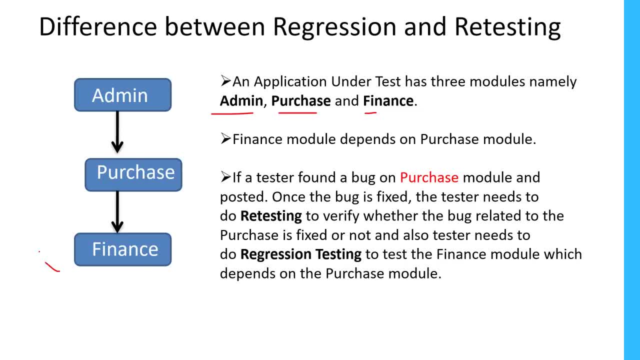 So finance module is depends on purchase module. So finances depends on purchase modules. Let us assume finance module is completely depends on purchase module. Okay Now in this scenario, if tester found a bug in purchase module, So a tester found a bug in purchase module here. 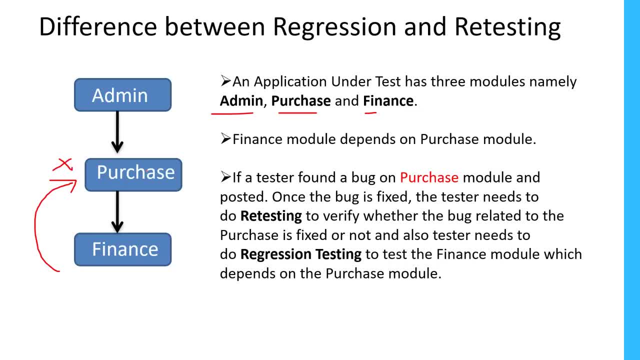 Yeah, there is a bug. now he posted that bug to the developer. So once the bug is fixed the tester needs to do retesting to verify where the bug is related to the purchase is fixed or not. So we found issue in the purchase. 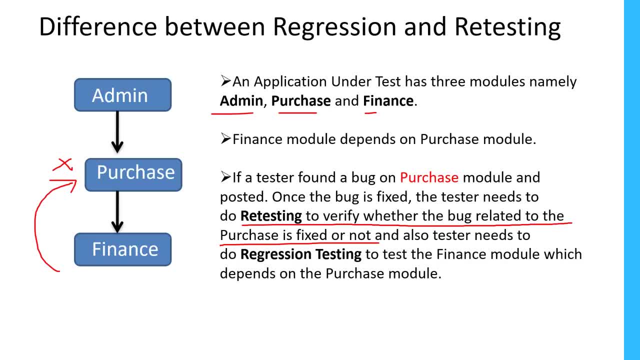 We reported that issue to the developer, fix it and we test that. only that part, only that bug on the purchase module, If I do, only that testing is called as a retesting. But finance module also depend on purchase right. So along with this bug, if you also test this finance module completely, 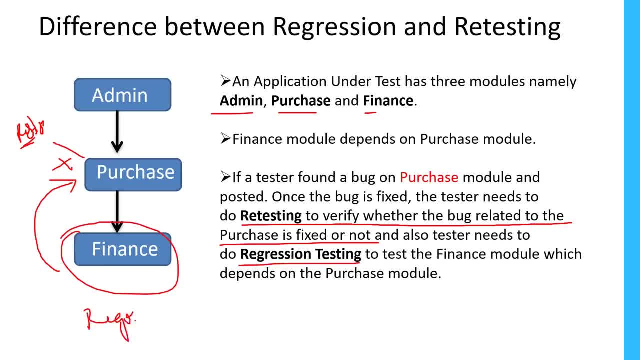 that comes on the regression test. This is a simple difference between retesting and regression testing. So retesting means same thing- We test again and again, repetitively- and regression testing means not only that change. if there is any other dependencies, We need to also test those dependencies. 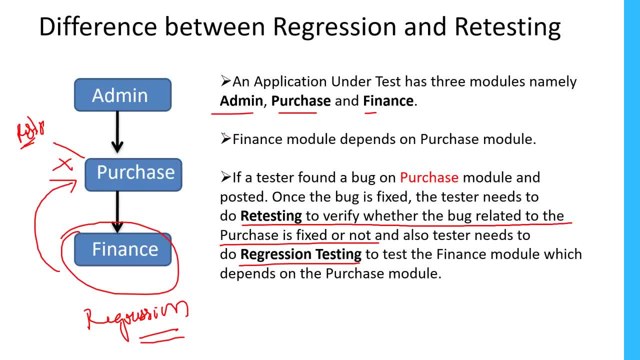 because because of this change or defect or fix there may be, some other functionality may affect right. So we need to also make sure because of the stage There should not be any effect on other functionality. that is called as a regression test. So retesting and regression test. 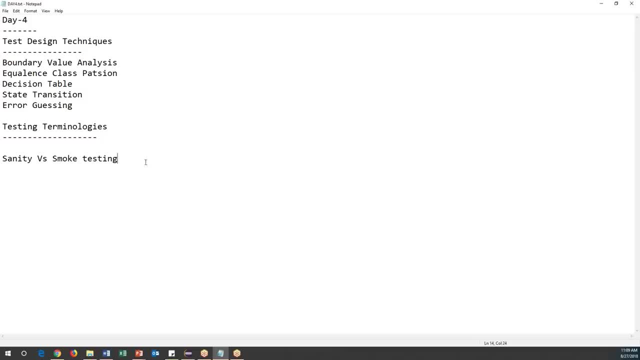 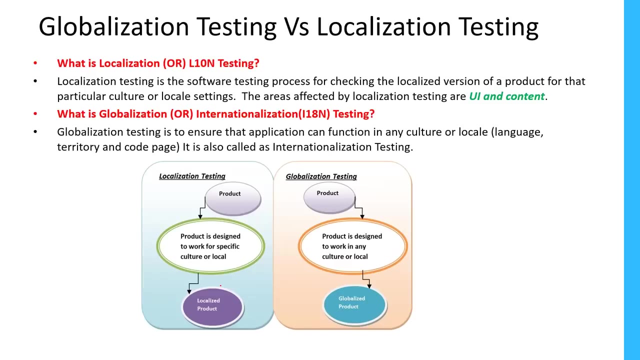 Okay, very important. So sanity and smoke testing we have done, and then retesting versus regression testing, Because in interview people will asking these combinations, Retesting and regression test. Now let us move on to the next one: Globalization testing and localization testing. 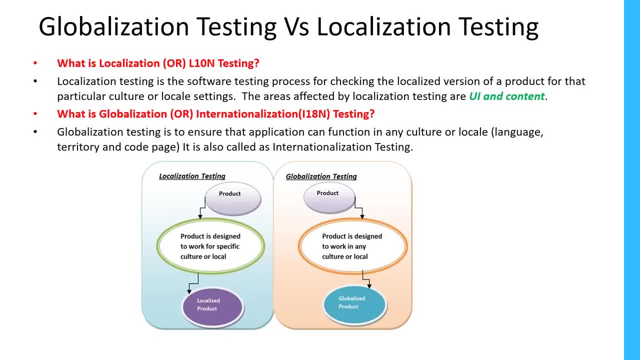 Globalization testing is also called as a internationalization testing. International, which is very simply say localization testing, is also called internationalization testing. I 18 and means an internalization in this particular keyword. First letter is I, last record is N, So in between all the letters will be exactly 18 characters. 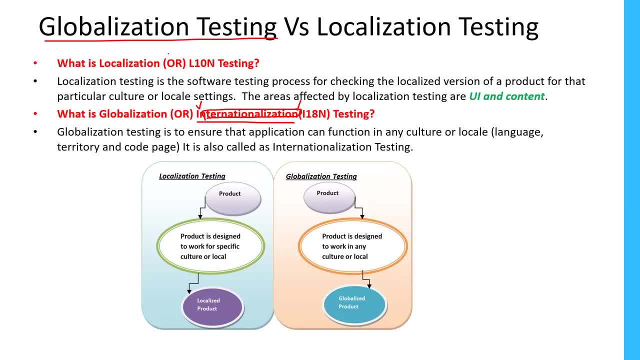 Okay, so it's called I, 18 and test. now localization testing is also called L, 10 and testing. So first letter is L, last letter is N. in between, exactly, We have 10 characters. So let's see what is this. So localization testing is a soft, is the software testing process. 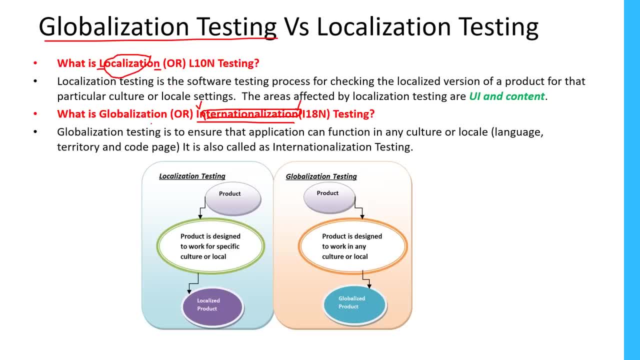 for checking the localized version of a product for that particular culture or locate settings. So the areas affected by the localization testing is our UI or content. So sometimes there are some websites will be supported multiple languages. So for example, let's say PayPal is a website. 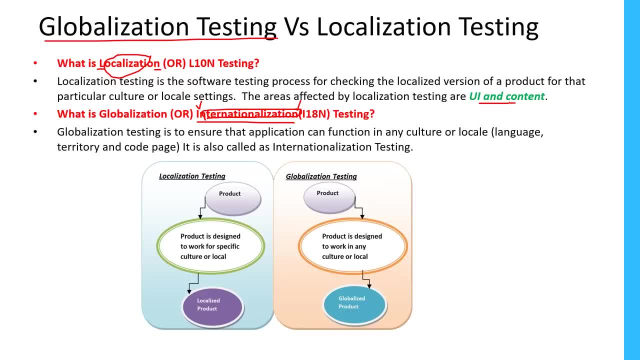 So if I open that website in this country, specific country, the web page will appear in specific language, Okay, and in UK or US, and it supports multiple languages. So in the localization globalization simply say: in the localization testing, our application is supporting, the local languages are not. 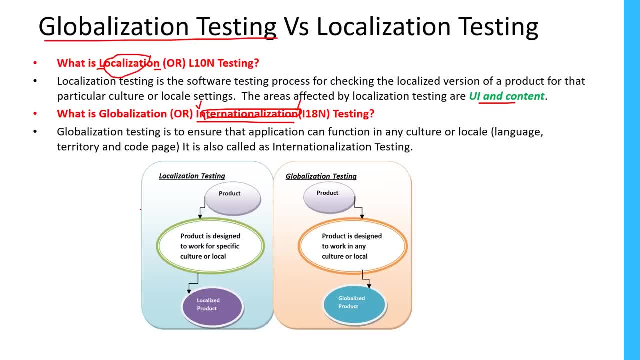 Okay, and in the globalization testing with testing application, whether it is supporting the global languages are not a global support or not. So simply one example: in application There is a date field. Let us say there is a date field Here. I need to enter the date. 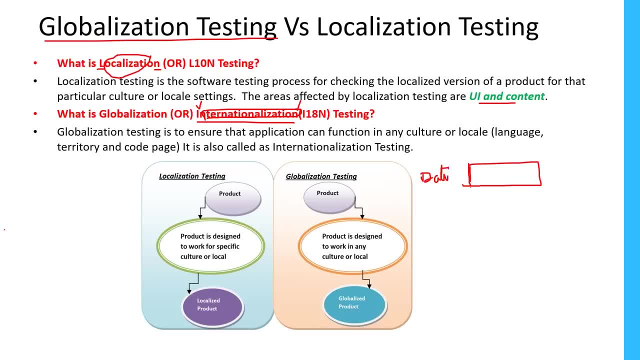 So normally this date format will be different from one country to another country. Okay, So here, suppose in this application It is allowing DD and then YY format. It is allowing only this particular format. that is a localization, So it supports only within. 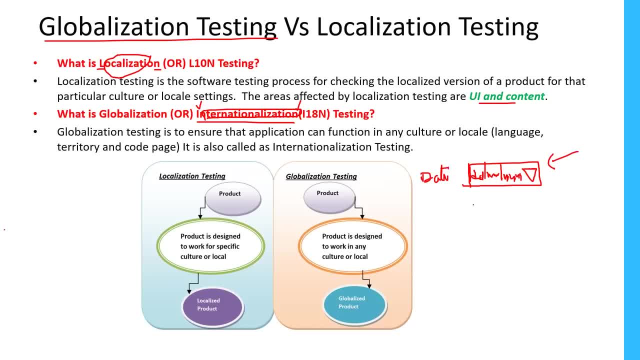 In India, So only within India. We can just this format will part and if I is, this application is open in some other country, Suppose in that particular country. If this application gives the flexibility to give any format, let's say first MWAM and YY and then day, 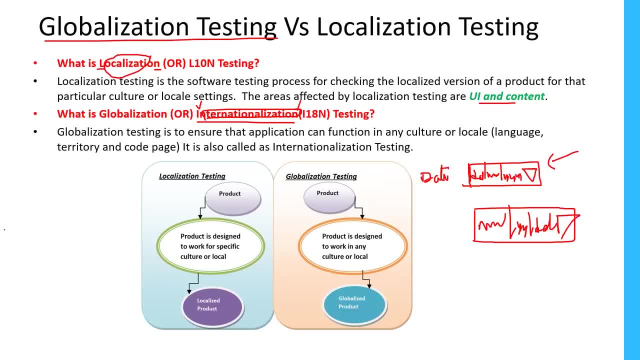 So this kind of flexibility, if it is provided, that is, comes under the globalization or international support. So this is just simple example. So like this, There are so many Examples will be there. So there are some applications in some countries will be. appearance is different. 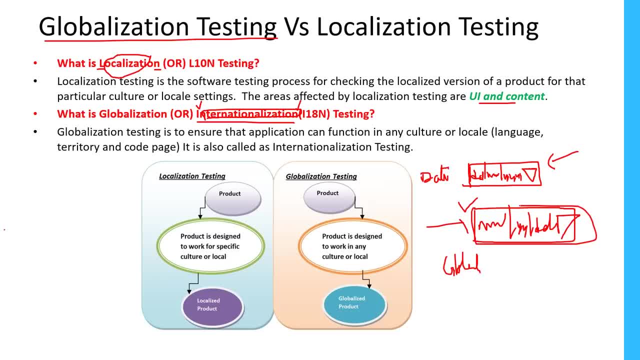 and some other countries. appearance is different. Okay, and the logo. so some companies, or some international companies, they will put logo in the right side and some companies, they will put a logo here in this side. Okay, that's again based upon their culture and their tradition. 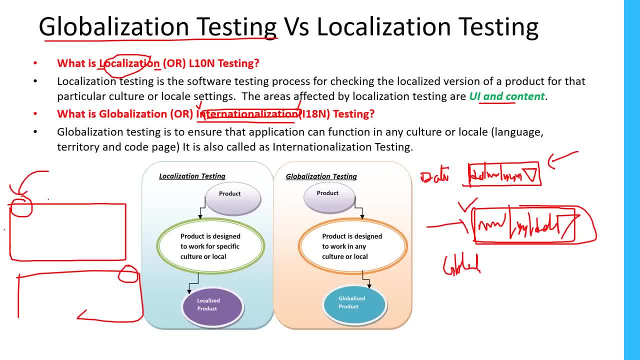 So our application is supporting according to their culture or the tradition of their requirement or not, So that we need to verify as part of globalization and localization. So simply say so here: product is designed to work for specific culture or local, that is a localization. and if product is designed to work in any culture, 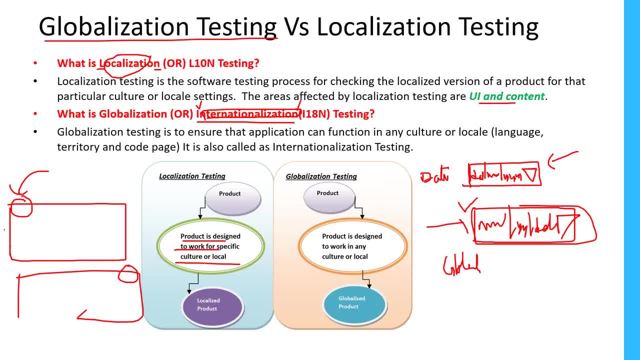 or local. it support local or any other culture, but here local along with the other specific culture. This is very specific to culture but this is not very specific to culture. it covered Kinds of cultures. that's a globalization testing and localization test. very rarely. 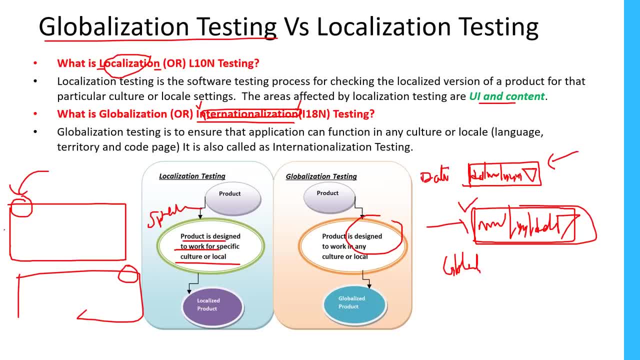 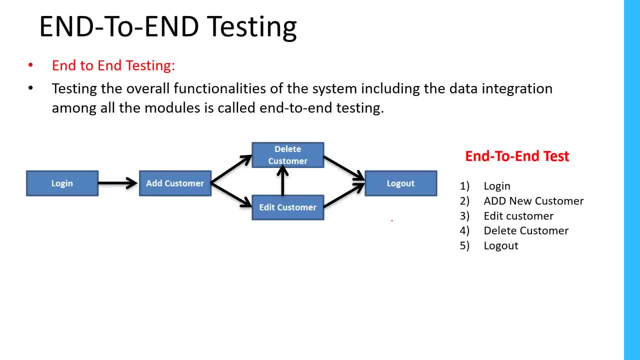 We do this kind of testing, especially for international websites. Okay, So now let's move on to the end-to-end testing. So this term we commonly hear in the real time end-to-end testing. Somebody will ask you to end-to-end testing. 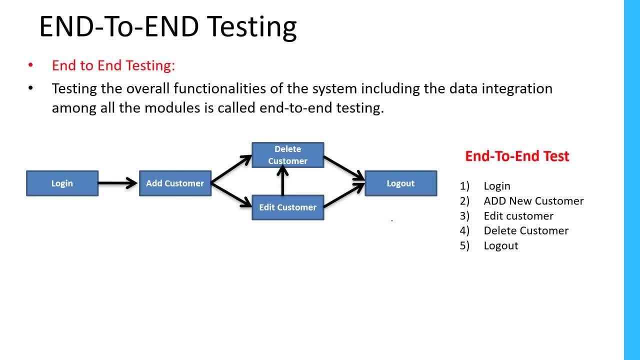 So we need to understand what is end-to-end testing. So end-to-end testing means testing Overall functionalities of the system, Including the data. integration among all the modules is called end-to-end testing. So suppose somebody give you an application? Okay, you have, let's say, 10 test cases. 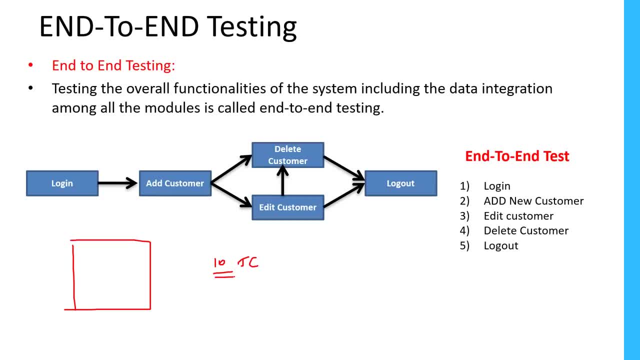 You have written for this application. You have 10 test cases in your hand, So each and in each and every test case is individual, So every test case will representing a certain functionality. Okay, let's say the first test case is login. 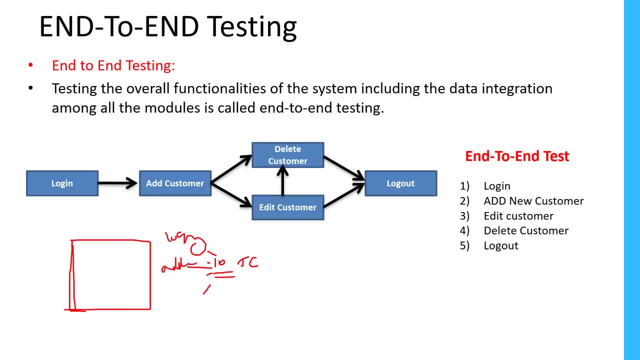 And second test case is adding a new customer into the application and the next test case is deleting the customer and another test case is editing the existing customer. The other test case is logout process. So for every functionality you will write a different kinds of test cases. 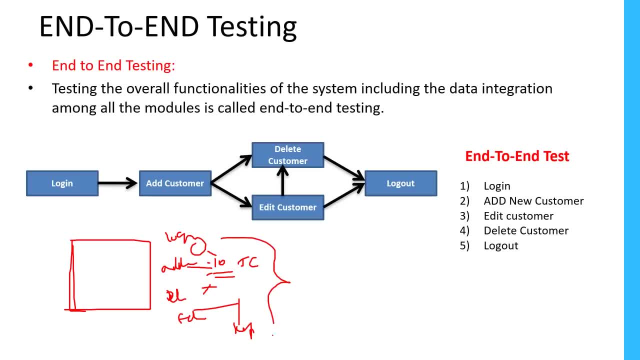 All are independent test cases, So you will test all the test cases differently, one after another, but at some point of time we need to perform end-to-end testing. So you will have one test case which will cover entire functionality, end-to-end functionality, the complete flow of your application. 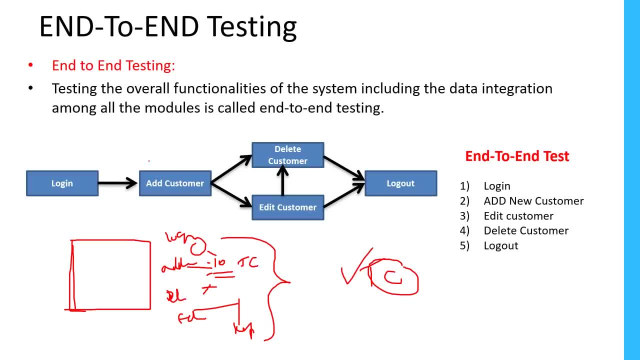 So if we execute this test case, this will touch each and every functionality in the application, So that is called as an end-to-end testing. So here an example. So here I can write multiple test cases for these functionalities. right, So I can execute these test cases. 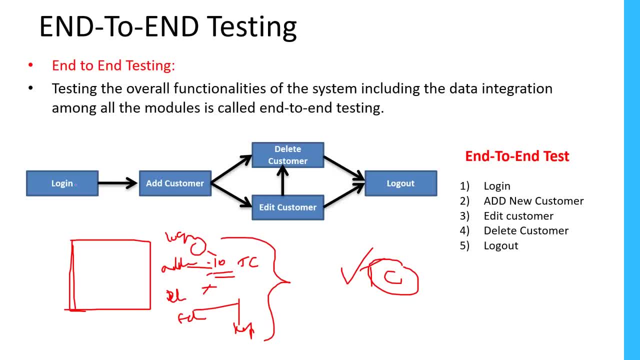 and also I can write one test case which cover every functionality or which will test every functionality. So let us see here: first login, followed by add customer, and the next step is delete customer, edit customer. Let's say this is a step one, This is step 2, step 3, 4 and 5.. 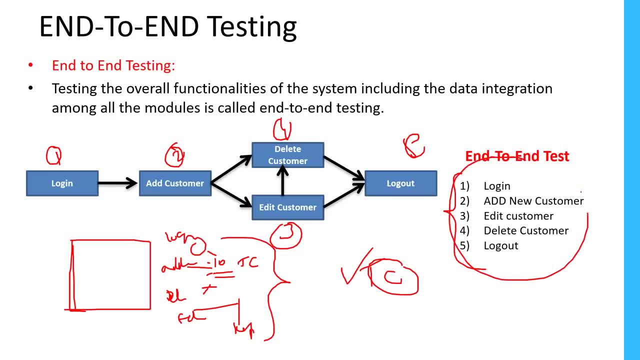 So if you write test case like this, so this test case is covered, all the functionalities, or you can also write individual test case for every step here. So edit: customer is one test case, delete: customer is one test case, logout is one test case. But if I write one test case, 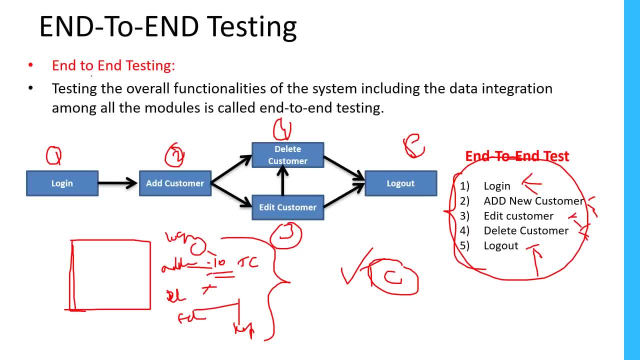 which will cover each and every functionality in your application. that's called as an end-to-end test case, also called as end-to-end testing. end-to-end testing So means there are set of test cases which will cover each and every functionality of your application. 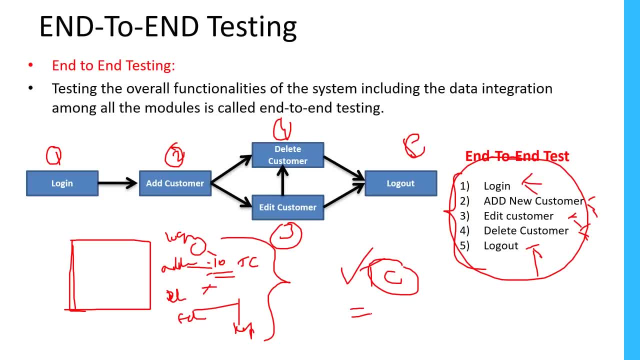 Okay, if I execute only those test cases, you will have certain assurance. Okay, I have done everything, almost Okay, so that kind of assurance They will give you. that's called end-to-end testing, So testing the overall functionalities of the system. 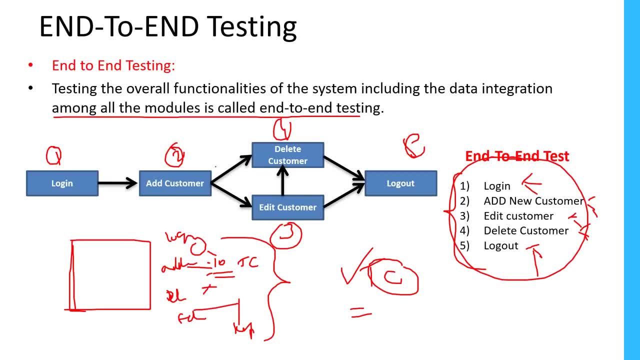 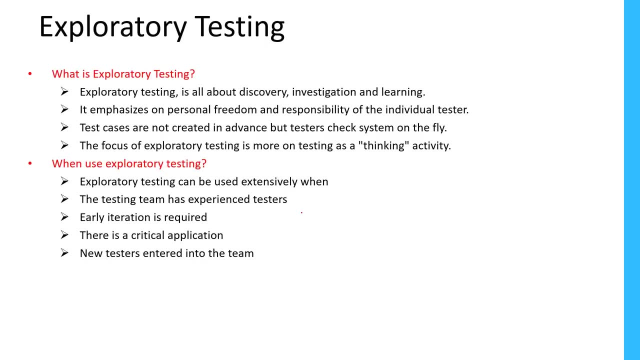 including the data integration among the all the modules is called end-to-end testing. Okay, next, exploratory testing. So exploratory testing is basically all about Discovery, investigation and learning. So I'll give you a smaller example here. Suppose if you join in a company. 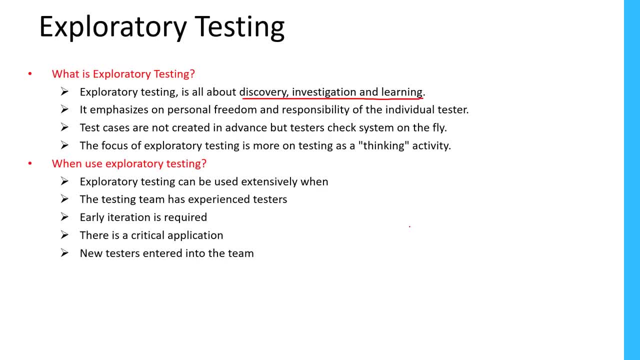 you don't have any skill or any knowledge on the project currently is going on. So what they will ask you is just they will give you an access that application and just play with it for a few more days, because you need to get familiar with this application. 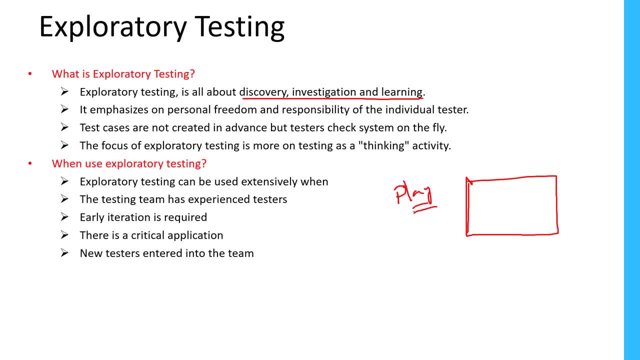 Right, but you don't have any documentation, So you don't have any test cases, You don't have any requirement, You don't have anything else, You, you have only this application. So what you will do now, you will just. 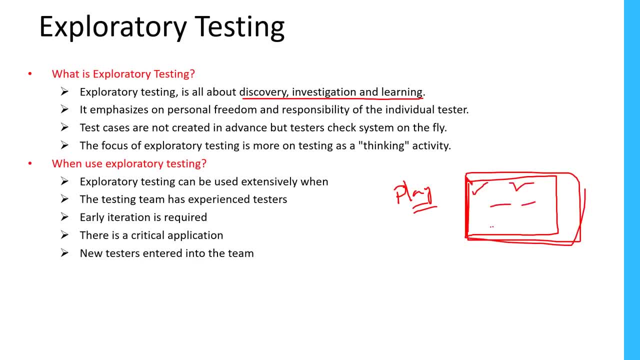 just click on something, you will do something, or set an action or some transaction. you will do So slowly. what happens is you will get to know what is working, What is not working, how it is working. You will get some knowledge on this right, without any documentation, without any dependency. 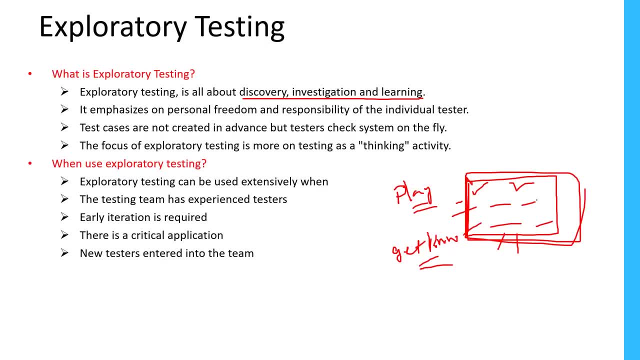 You will get certain knowledge on this slowly Once you start and using this application. that itself is called as exploratory testing. So exploring your skill on that particular project without depending on any documentation is called us Explore it. while exploring the application, You will test it. 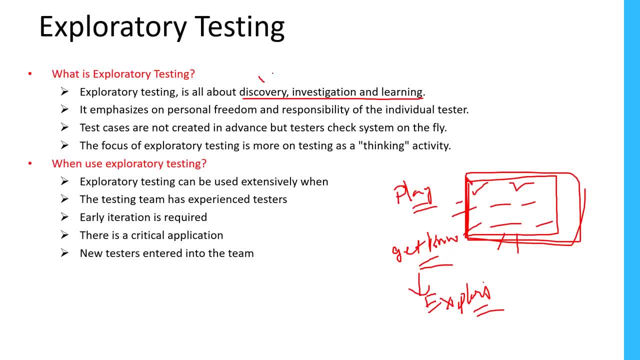 Okay, so exploratory testing is all about discovery, investigation and learning. all things will be included. So it emphases on personal freedom and responsibility of the individual tester. So that is again up to you. Nobody will ask you to do exploratory testing. 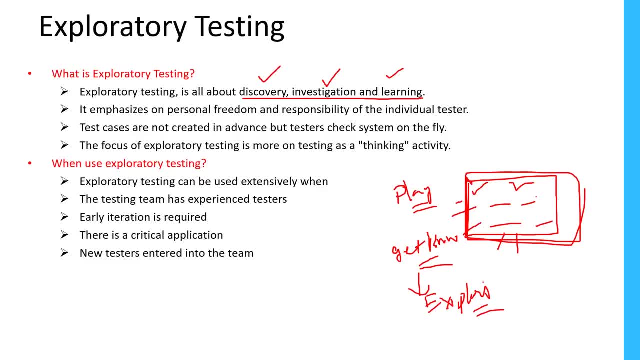 But whenever you found some time, whenever you find some time, you can perform this kind of testing. So there is no specific schedule or there is no specific cycle or plans will not be there for exploratory testing. You can just directly do and explore the functionalities more. 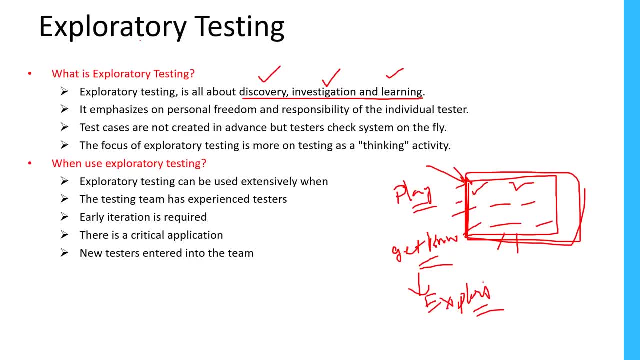 and more and you will get to familiar with this application That's called as exploratory testing. Okay, so exploratory testing can be used extensively. when the testing team has experienced a tester- suppose that they have the previous background or experience- you can test it. 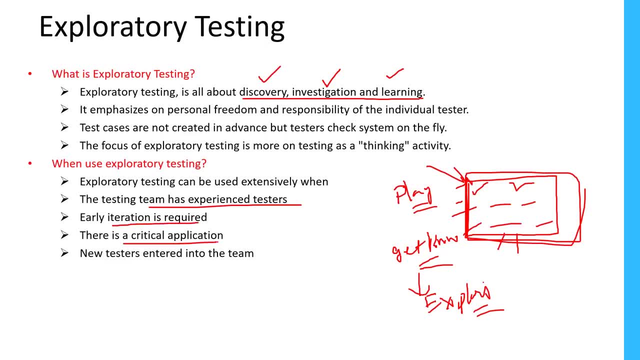 Early iteration is required. There is a critical application or new testers enter into the team. This is a very important point. Whenever the new testers enter into the team, they do exploratory testing because they don't have any knowledge on the application. So all the time they will do exploratory testings here. 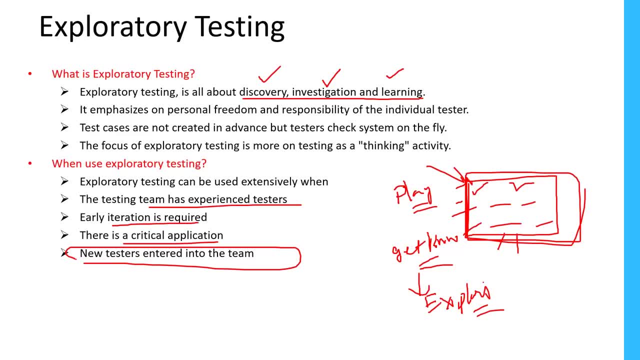 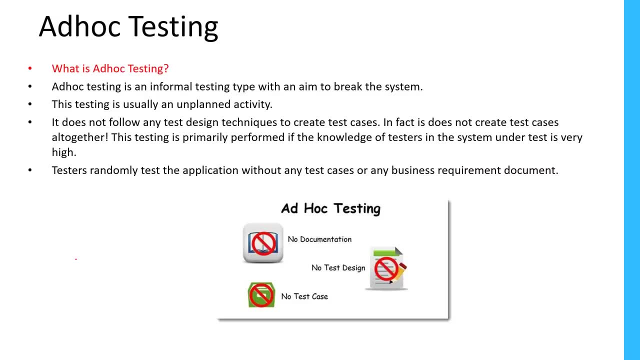 We just exploring the functionality of the application and learning it. the learning is a main, important focus here. Okay, exploratory test, now ad hoc test. So exploratory, ad hoc and monkey, These are three types of testings. seems very similar, but I'll tell you what are the differences here. 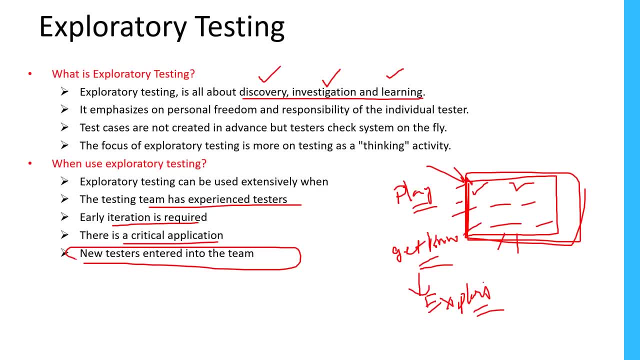 So, exploratory testing, remember few points. exploratory testing is mainly focusing on learning. We are, we don't have any knowledge on the application. We start with the zero knowledge. We are exploring application. We are learning, we don't have any documentation. Okay, These are the key, important points which we need to remember. now come to the ad hoc testing. 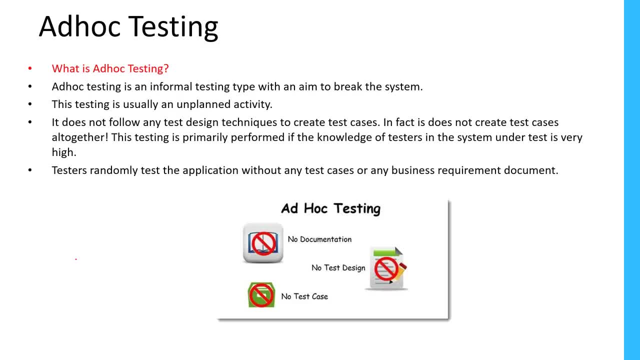 In ad hoc testing is just like a ad hoc means a randomly tested. There is no proper plan, There is no proper flow or proper structure strategy, Nothing. just we do the testing random and this is informal testing time. informal means it is not properly. 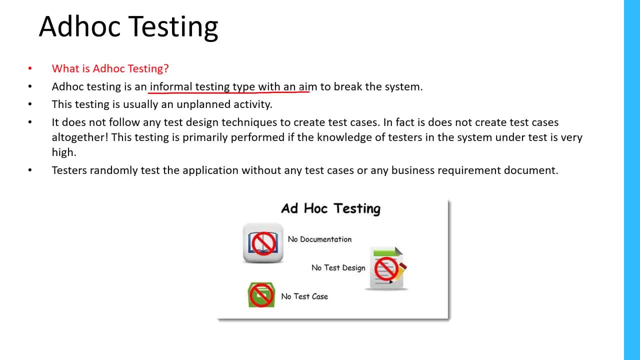 So whenever we find some time we can do at all testing. but here we know little bit about the applications. So we know certain functionality of that application, but here we don't even have Documentation but we know the functionality of the applications. So what are the different functionalities are available, how to test them? 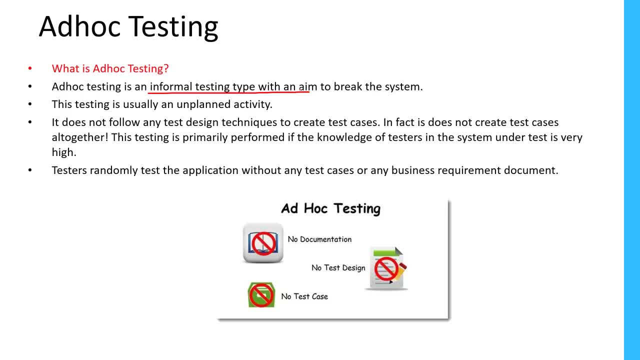 What is an output we will get. so this kind of skills we should have. Okay, ad hoc testing means randomly test that application functionality Whether it is working or not. The main intention of this testing is to break the system. So the main intention of the tester is to find as many as bugs possible. 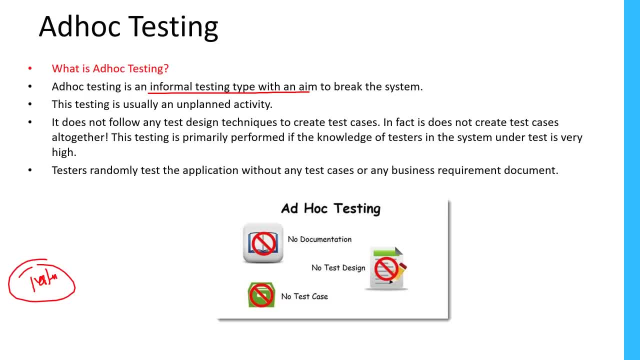 There's a main job of test. So this is ad hoc testing, is informal testing. So the main intention of this testing is to break the system. So somehow somewhere there are corner cases. The test cases also cannot be covered, those corner cases. So those cases we can test through ad hoc testing only. 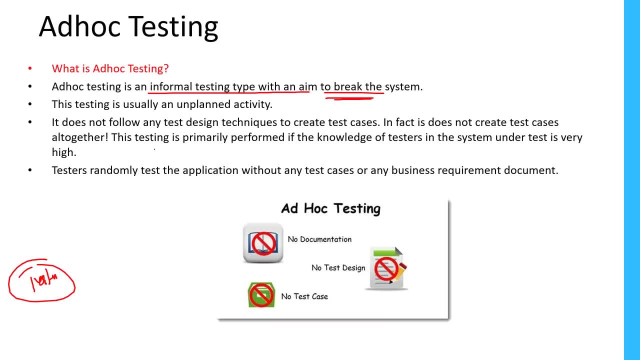 So even we cannot write test cases, those scenarios. So in those cases ad hoc testing will be very useful to find out the corner defects or corner issues. So this is completely unplanned. We don't plan any time for this. So whenever you find some time, whenever you have some still time, 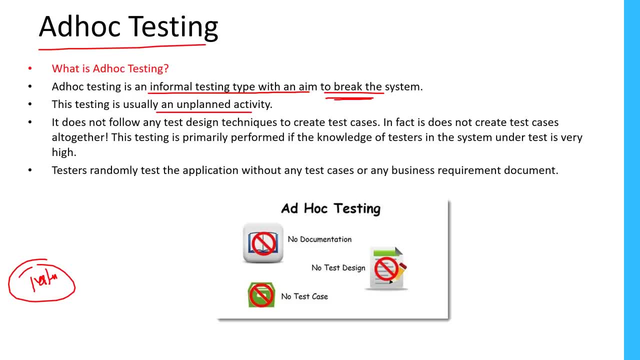 or last time you can do an artist, just test the application randomly. So go through all the functionalities and flows and test whether everything is working fine or not. all these things we can do it, and here we don't know, don't have any documentation, No design, no test case. 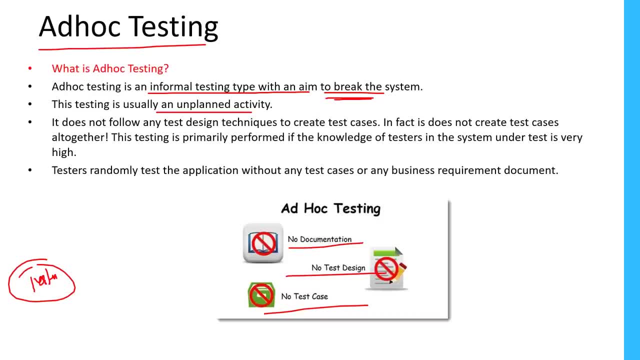 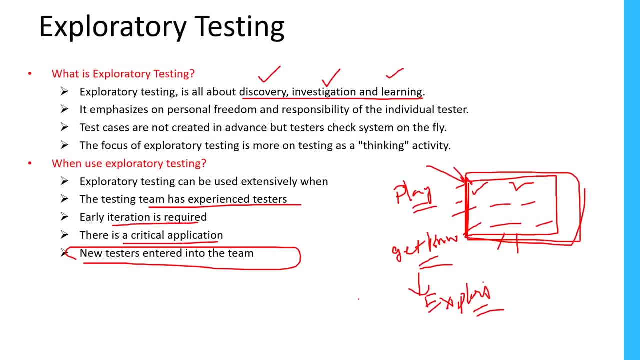 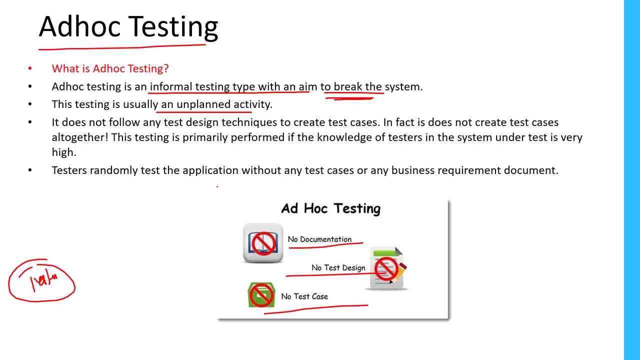 Okay, we don't have anything. but what is the difference between exploratory and ad hoc? in exploratory, We don't know anything about the application. We are just learning that application. But here we know little bit about application. We are testing it based upon our knowledge. 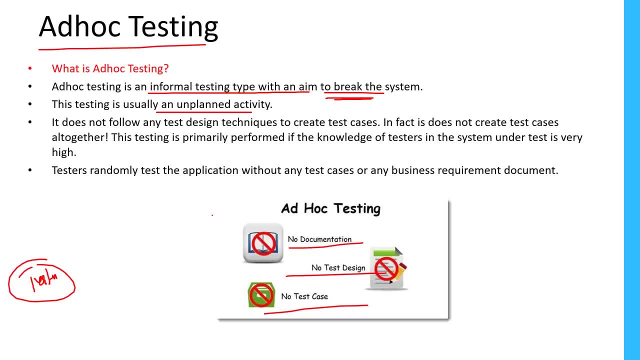 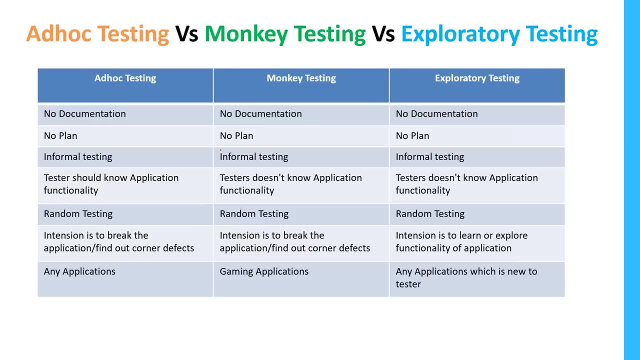 and this is a random testing. Okay, that is ad hoc testing. Now let's compare ad hoc testing. There is also one: monkey testing. I will talk about here ad hoc testing, monkey testing and exploratory test. So these are the very important. 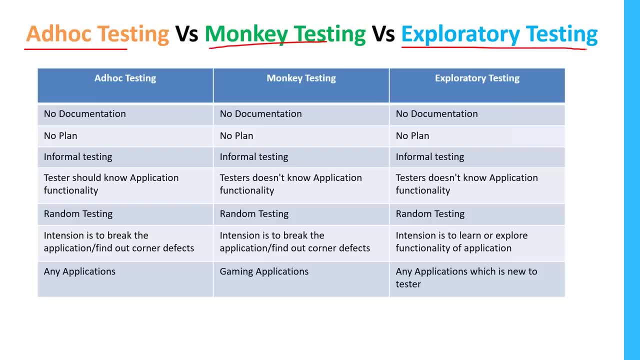 The three people will ask you differentiate this because almost very similar, except the only one or two differences. almost very similar. Now let us just compare this: ad hoc testing, monkey testing, exploratory test. So in ad hoc testing, as I said before, there is no documentation. in monkey testing 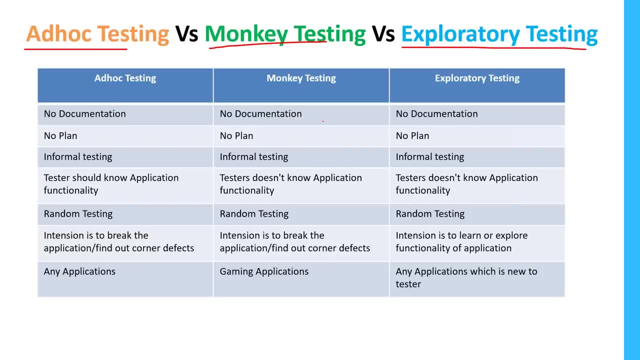 Also, there is no documentation. documentation means requirement document, test cases document, Test plan. These are all called documentations. Okay, so we don't have any documentation during this kind of testing. So I don't testing monkey, testing expert and all these testing. we don't have any documentation. 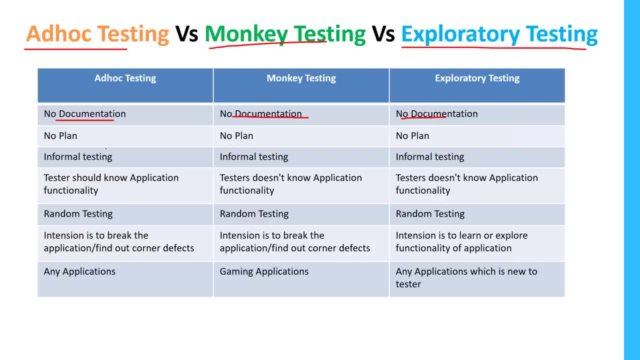 without documentation. We do these type of testings and we don't have any plan. So there is no specific cycle for this, but we have a cycle for retesting, regression testing and all but here these are just ad hoc testings, are randomly. Whenever we find some time, we do kind of testing that is up to your wish. 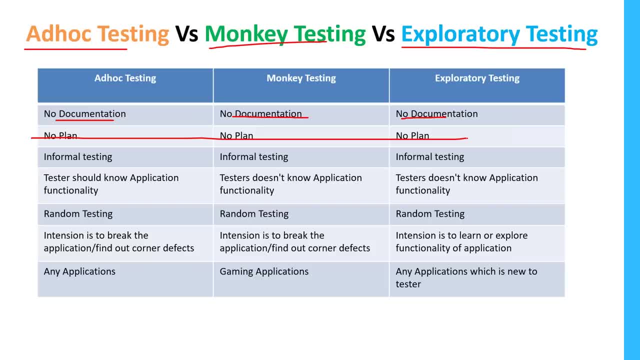 Nobody will ask you to do these kind of testings. This is up to you. complete your wish. if you have fun sometime, if you find some more corner defects, you will do these kind of testings. So there is no plan at all because these are completely informal testings. 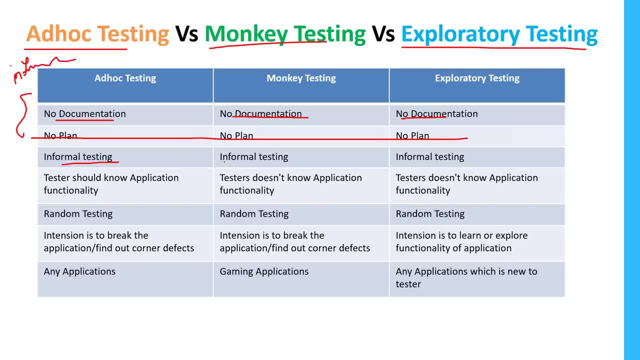 There is no formality for this. Okay, everything is informal. now tester should know application functionality. So, as I said, in ad hoc testing we should know the functionality, but in monkey testing and exploratory testing We don't know the functionality. Okay, monkey testing, but everything is random testing. 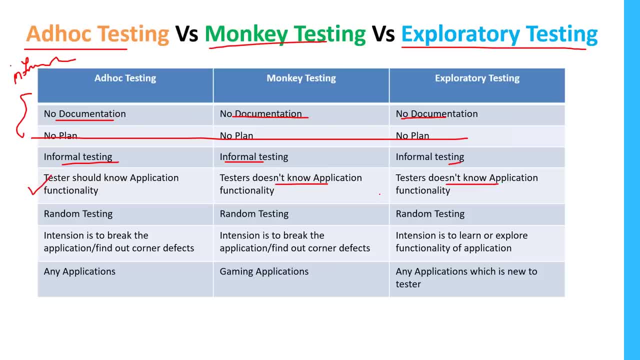 Okay, randomly test. There is no proper plan or proper strategy. But in ad hoc testing we know the application functionality. but in monkey testing and exploratory testing We don't know any functionality and everything is a random testing. So randomly means there is no proper order. 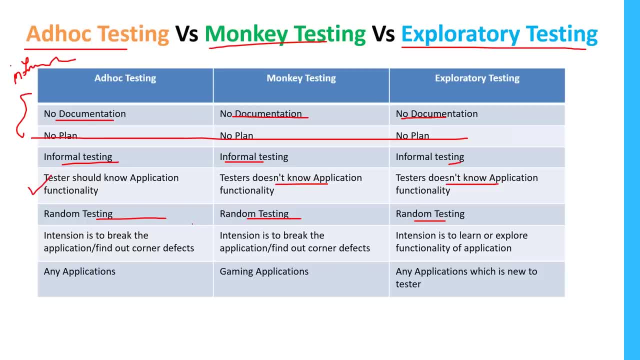 So that is up to you. So how many ways we can test application? you can just go blindly. So there is no proper plan, There is no proper documentation, There is no proper schedule, Nothing, just you go as you wish. that is random test. 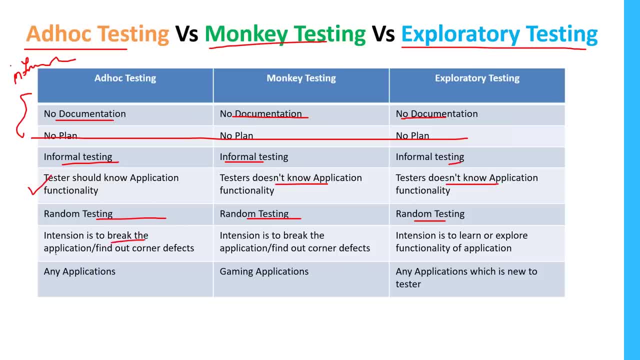 and the main intention is ad hoc testing is to break the application and find out corner defects. The main intention of every testing is same, So to find the, to break the application and finding the corner. but here the exploratory testing is. the main intention is learning the product. 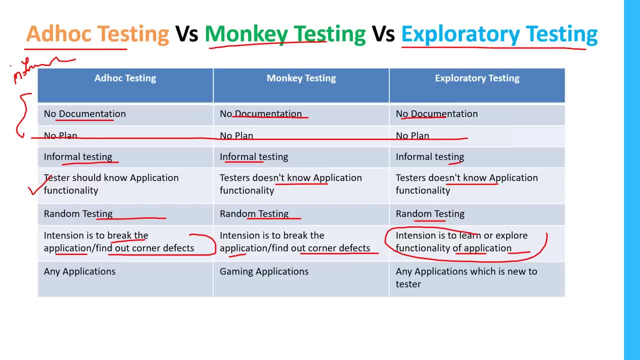 or learning or explore the function. Okay and ad hoc testing can be done for any kind of application, all kinds of applications like base applications, desktop applications, gaming applications, anything- and monkey testing, especially for suitable for gaming applications. So when games will be played- games normal is, the children will play the games. 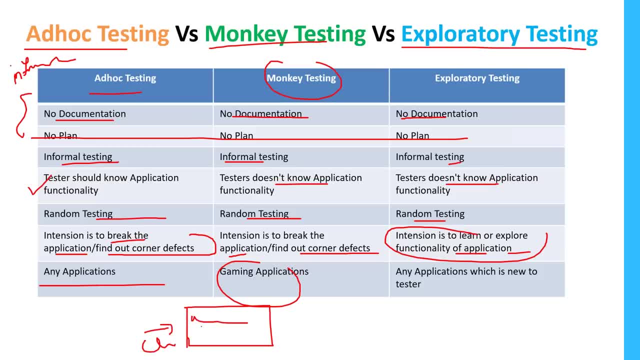 so they don't know how to what happens when they click on something, right, So they do randomly clicks, randomly, They do some clicks and the some effect will be happen. We don't know exactly what is happening. So in the monkey testing we test the application randomly. 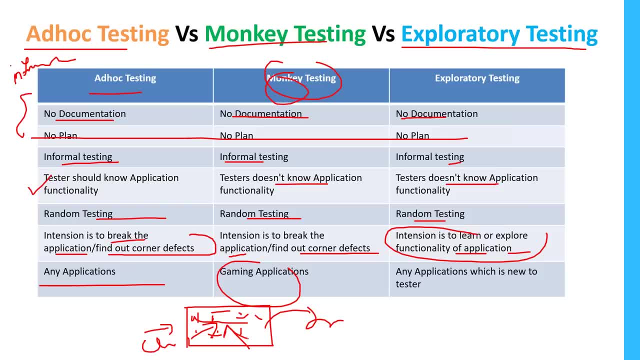 without proper planning, without proper strategy, and then we will check whether it's somewhere in the leakage or not, or somewhere it is broken or not, will verify. that's called as a monkey test. So mainly this is suitable for gaming application And exploratory testing also can be done. 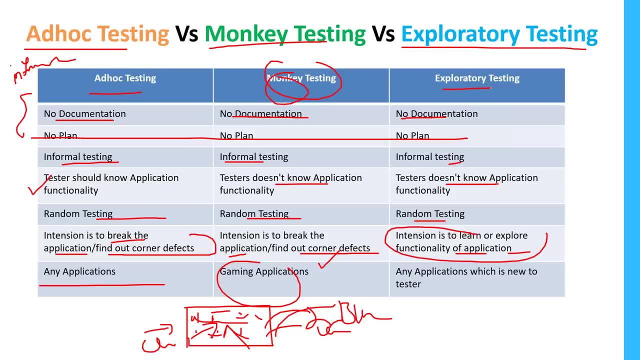 for any applications, but especially this testing done by the new new testers, or tester will join in the team newly. They can do this testing. This is at all testing, monkey testing versus exploratory testing. Okay, So is it clear? Yes, sir, internet, internet. 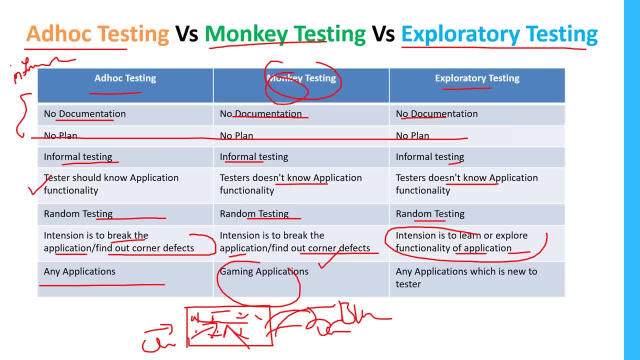 Sir, now I speak in person. The Hello, just stop it here today So we can use. tomorrow We have one or two classes and then we'll do practical classes. Okay, Okay, sir, Now I speak in picture later. Right, so far. 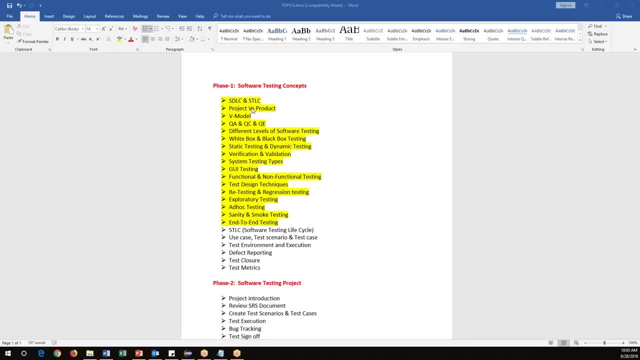 We have discussed about these things like HDLC and project versus project product. We model different levels of testing: White box, black bus testing and various types of testings. We have these cases so far and now we'll enter into the testing process. So in the actual, in the real time, how the testing process will be going on. 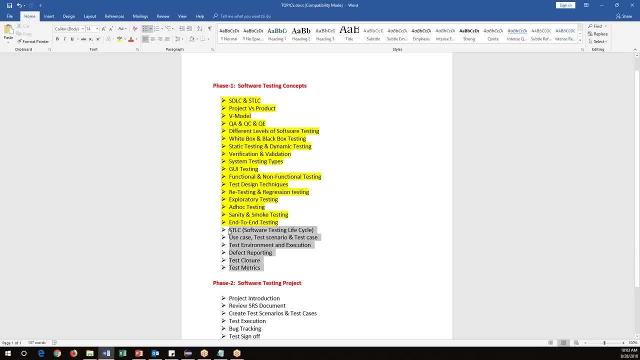 So we'll make my main focus on these items and then we'll go to the project. before going to the project, We need to understand what are the different activities We have to perform as part of the project and day-to-day life. Okay. 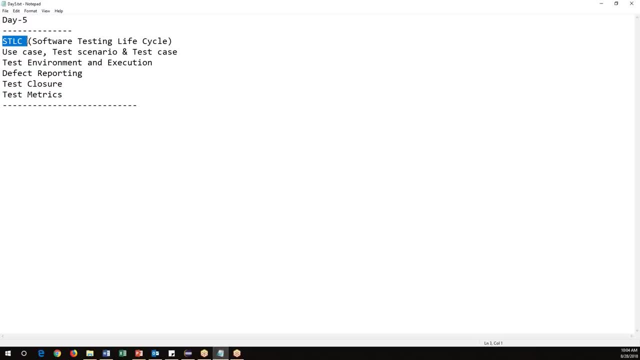 So today session I'm going to cover HDLC software testing life-cycle in detail and what are the different activities we perform in the step-by-step, and we'll understand what is use case test scenario, What is test case and how to write the test cases and all. 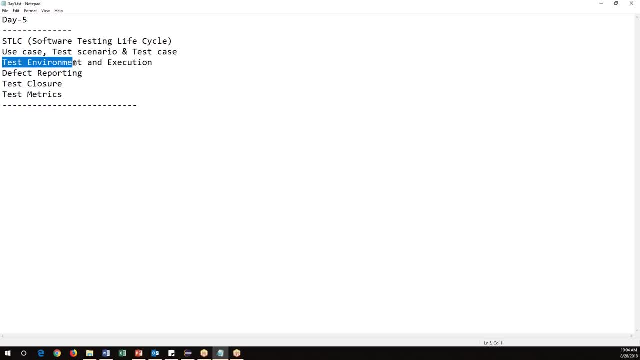 and also we'll see about what is test environment, how to execute our test cases, and then we'll talk about more on defects. This is a very important data. So what is the defect or what are the different details We need to send to the developer as part of default reporting? 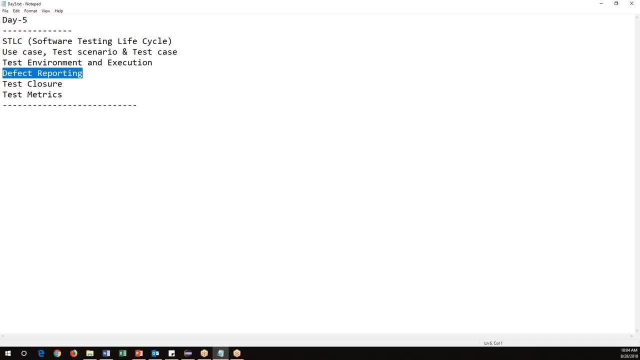 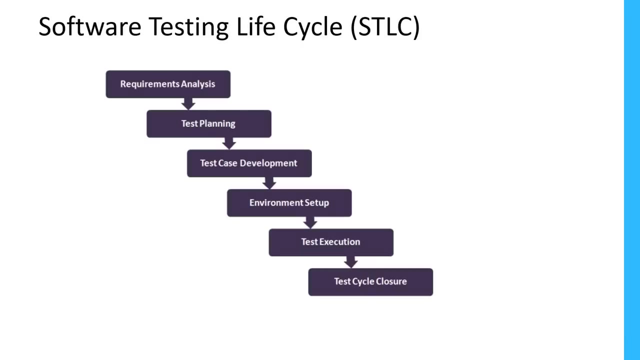 What are the activities we do, And we'll discuss that and then disclosure, and also will discuss about a few test metrics. Okay, So these are the topics which we are going to discuss today. Now let me just share small presentation. So, as I said before, SDLC is a part of overall SDLC process. 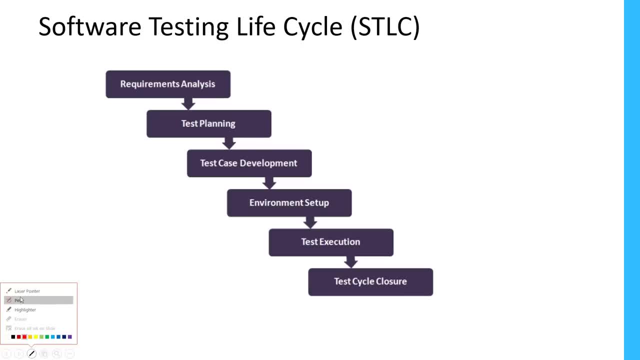 SDLC will talk about the complete development process, right? So means we have to start with analysis, development, analysis and design, and then coding and testing and then a maintenance. So this is comes under the SDLC. SDLC talk about the complete software development process. 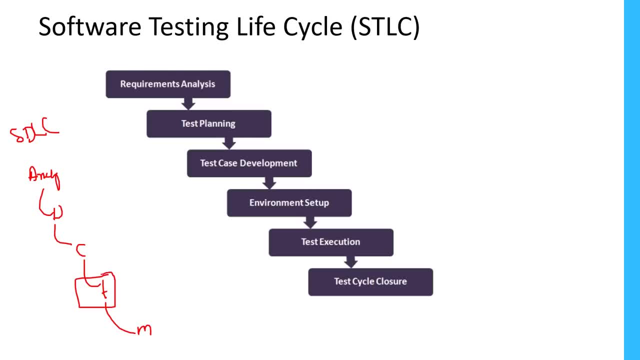 So here the testing is one of the activity which we need to perform as part of SDLC. So this is a SDLC here in the testing environment and the testing phase We follow. the SDLC software test life cycle is a one of the part in the overall SDLC. 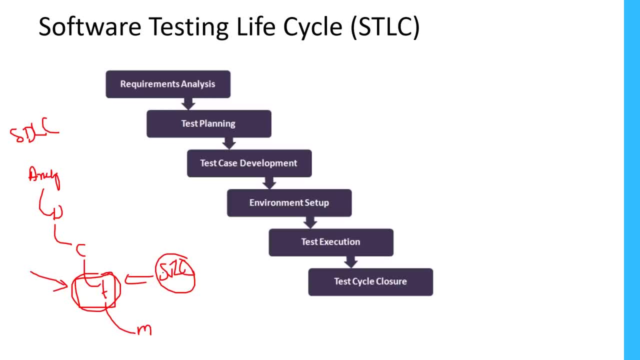 So we are working under the testing part, So we need to more concentrate on SDLC software testing life cycle. So what is software testing life cycle means it is talk about each and every stage or step-by-step activity which we need to perform as part of our testing. 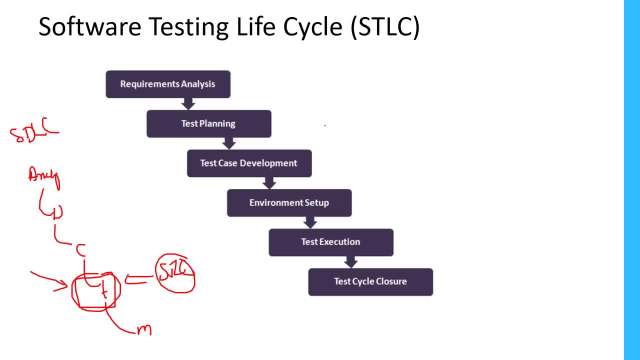 So let us see in detail each and every stage: What are the different people will involved in the stages and what are the different activities we do and what are the different documents we use. So we need to be have a very clarity on this. So, SDLC, start with the requirement analysis. 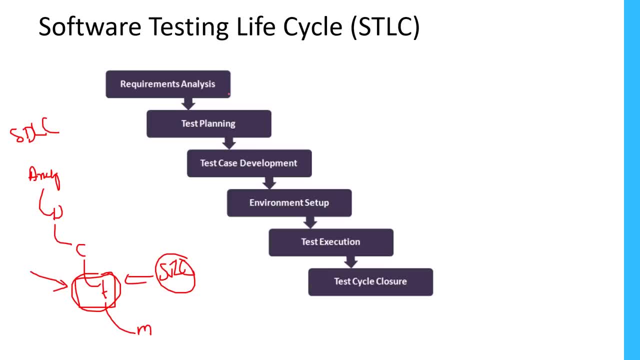 This and understanding the requirements, customer requirements- and we do test planning and test case development. Then we need to set up our environment, testing environment- And then we do test execution. That means test cases execution and then we can close our test cycles. So this is a step-by-step process. 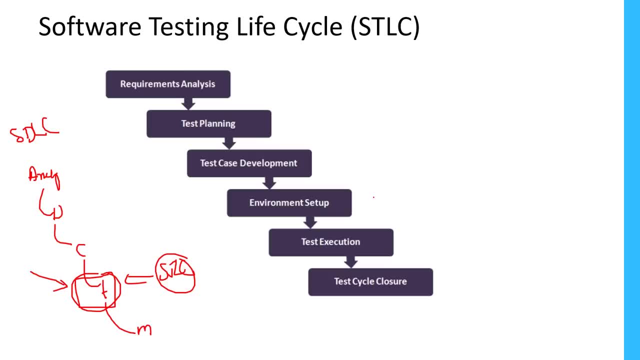 We need to follow. So this is all part of SDLC software testing life cycle. We talk about the testing process, complete Testing process from the scratch. So starting from understanding requirements till we close or we can stop testing in some point of time. 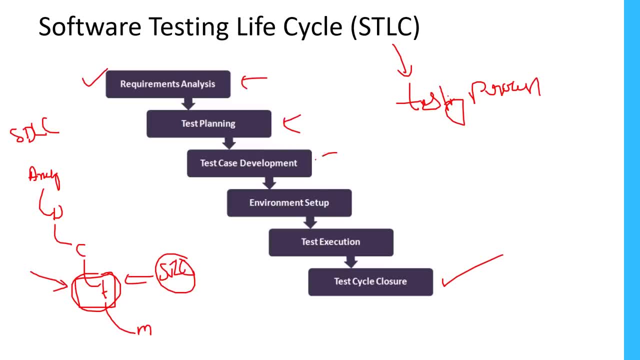 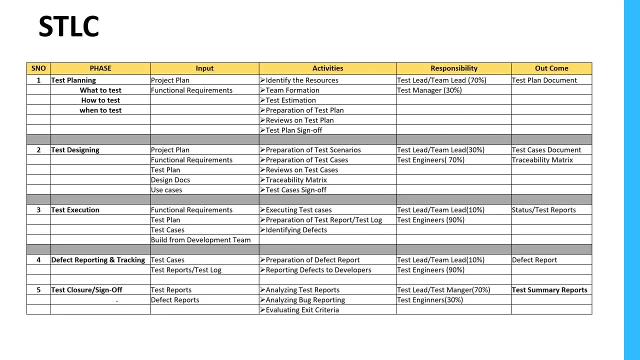 So each and every phase we have different people will involved and different documents We will create and also different activities we perform. Okay, So let us discuss in detail, step-by-step now. here I have make a list of all the phases, like what is the different phases we have in SDLC. 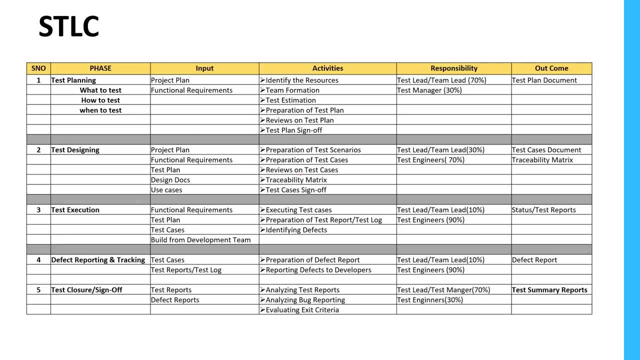 and what are the input documents we require and what are the activities We perform during that particular phase and what are the responsibilities of the people who are involved in the SDLC process. and then what is the outcome of that particular phase motor: The output documents will get once we completed that particular phase. 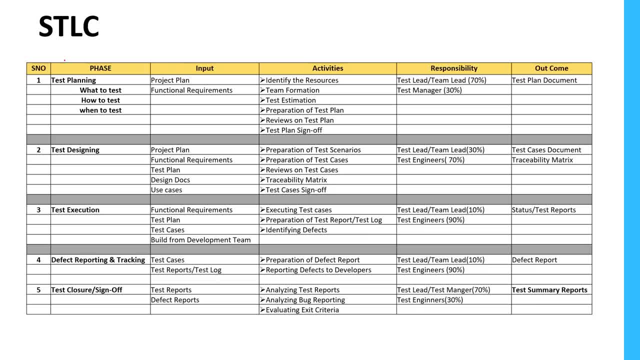 Okay, So let's start with the test plan. So before test planning anyway, we need to understand. the requirement is the basic step. So understanding requirement is a common thing for dev as well as QA, So everybody should able to understand the requirements. 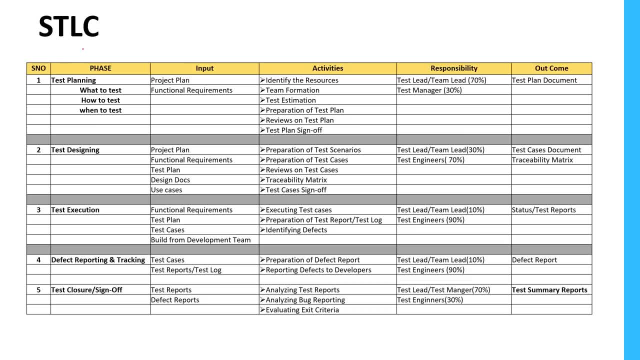 Because until unless we are clear about requirements, even developers can't develop anything and even tester also can't test anything. So understand requirement is the first and very important task of test engineer. So actual activities will start from the test planning. Now what is test planning? 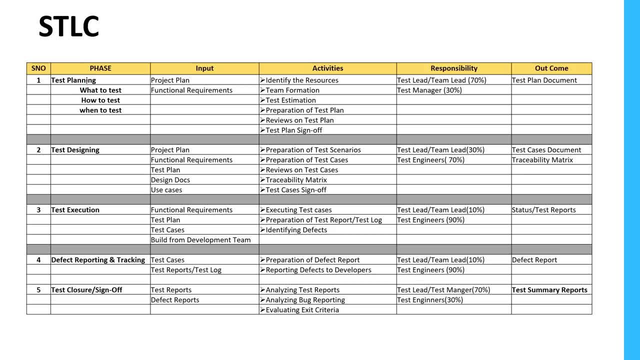 So this is a one of the phase in SDLC. So in this phase the main focus should be on what to test, how to test and when to test. So in our application, what are the areas to be testing? So we need to have a very clear picture on that. 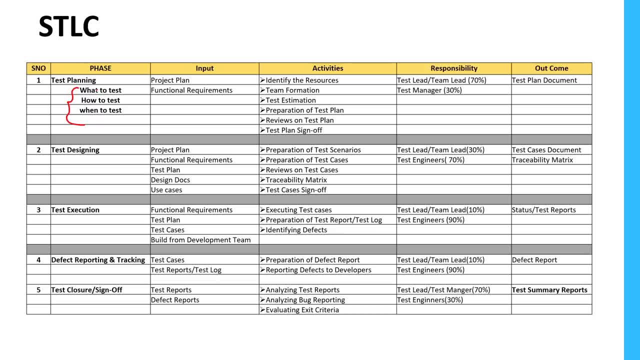 and how to test means what are the tools we have to use and what is the whether we do manual testing or automation testing, and if it is automation, what are the tools we have to use? Okay, and what type of testings we have to do. 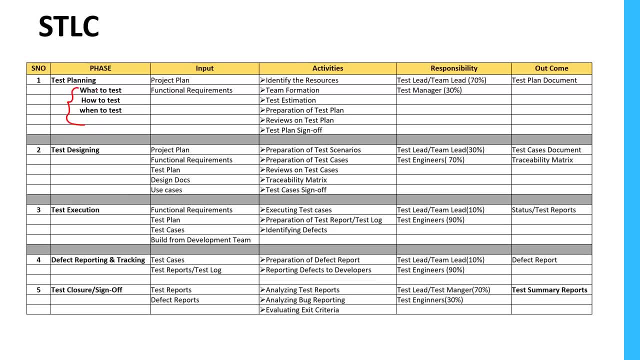 so different type of testing we have discussed earlier. So what kind of our testings we do on the application, so that we need to have a clarity, and when to test means the schedule. So what we will test, We will execute our test cases in different cycles. 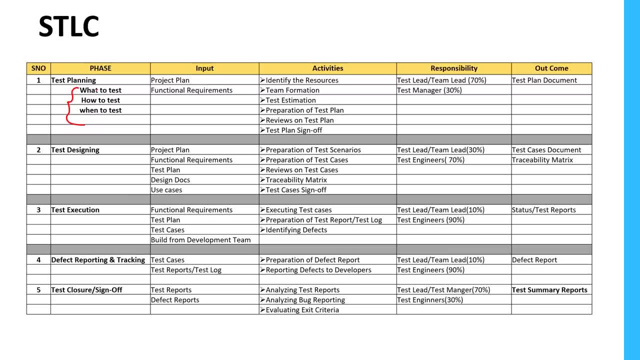 like sanity testing, small testing, function testing, regression testing. So these testings will be conducted in the different timelines. So when to test? so the dates and schedules- we should have a clear picture. So in the planning phase, the main thing is we need to focus. 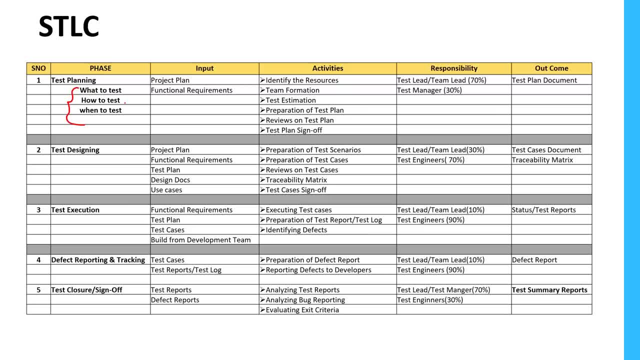 on what are the areas to be tested and how to test those scenarios and when. to test those scenarios means the timelines. So these are main focusing on a test planning phase. So here, what is the input document for us is project plan and functional requirement. 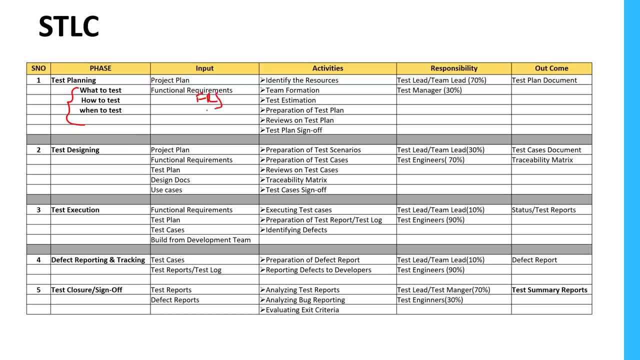 So function requirement in the sense again, if I was document, functional requirement specification. this is a very important document for us to understand requirements, customer requirements. Okay, and here the input document is project plan. So this project plan will be prepared by the higher level management team. 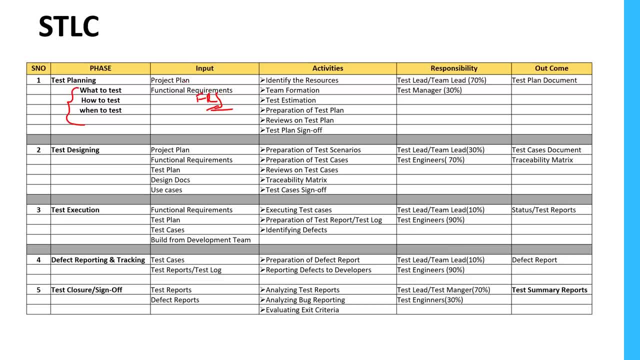 because this contains a lot of information, very high level, very project high level, like time range schedules. everything will be part of project Plan. So in the project plan they will mention the complete SDLC process like a understanding requirement. How much time will take design? 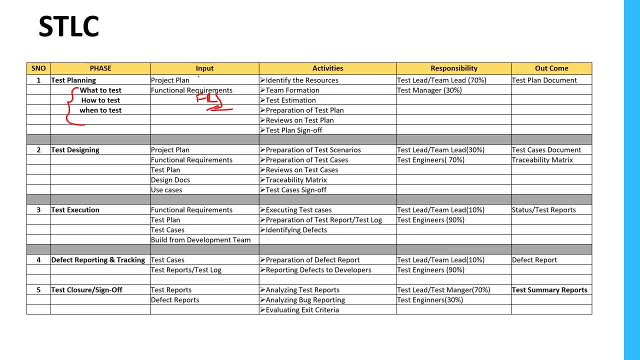 How much time will take and testing your coding How much time will take testing How much time will take. so each and every phase there will be separate timelines will be there So that information is available in the project plan. So why do we need to refer this project plan? 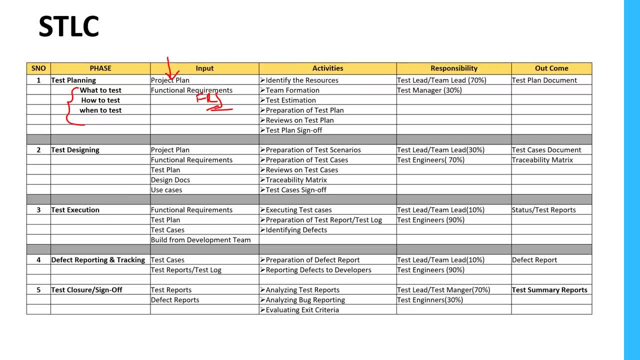 Because it contains the timelines and function requirements We need to refer because we need to know the requirements. So until unless we know the requirements, we cannot test the application. So this is a very important document for us to understand the requirements from the customer. functional requirements. 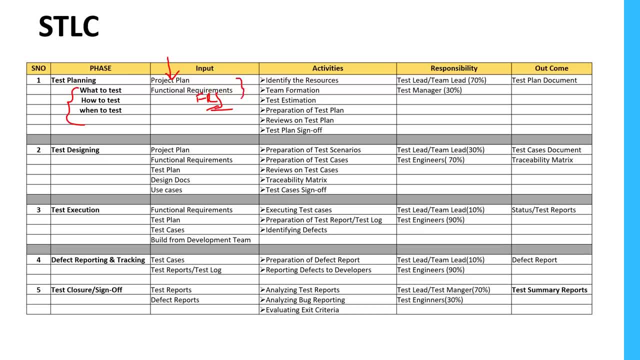 So these two input documents we require. until unless we have these two, we cannot plan anything. Okay, so project plan and a functional requirement. So project plan describes the timelines and schedules and the function requirements, specify the customer requirements and, based on these input documents, by referring these input documents, 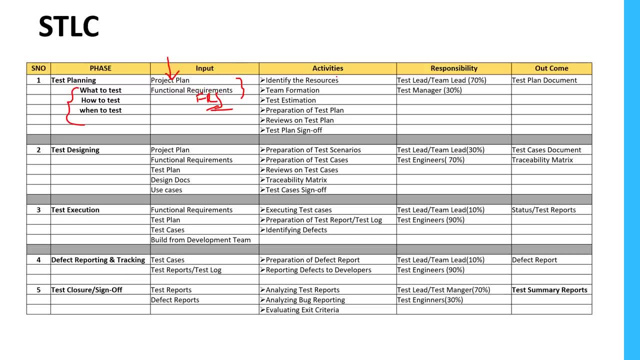 We do set in activities during test planning Phase. Okay, this is the initial level, first stage. So what are the activities we do here is identifying the resources means there are two types of resources, like human resources and hardware and software resources. human resources in the sense. 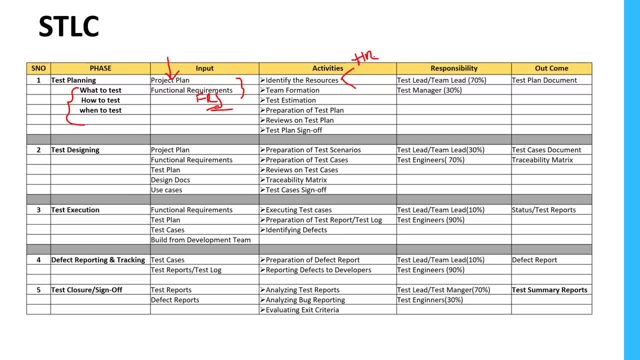 of the testing years on, the team who are is having the skills. We need to select them to your project for testing. and then hardware and software resources Suppose, if you want to conduct some testing. so we need certain hardware and certain software should be installed in our system. 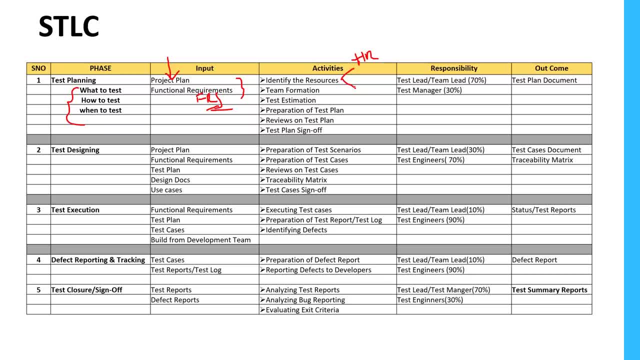 Say so. these are all comes under the identifying the resources. So if you want to conduct all the testings, what kind of software we required, what kind of hardware environment we required and what skills to the people should have, so we will select only those people but testing 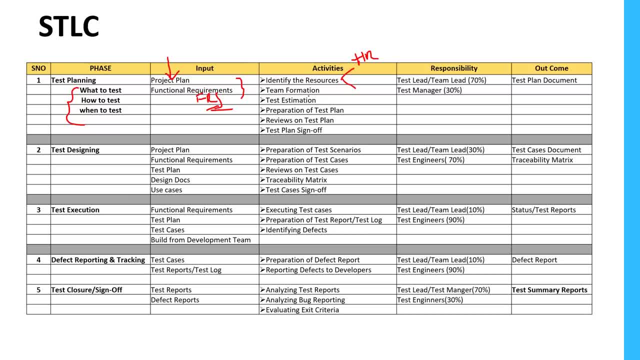 So this is a first stage. So here, team formation. So suppose the testing should happen in the three months of time. How many people should do work on this testing part and how many are manual testers, how many are automation testers will be decided during this phase. that is, test team formation. 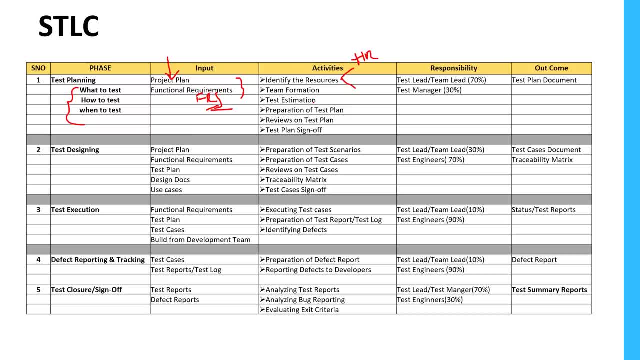 and test estimation also will be done here. test estimation means how many people we have, how much work we have, how much time will take and how much budget we need to spend. So this is all about estimation. So these activities normally done by the management team. 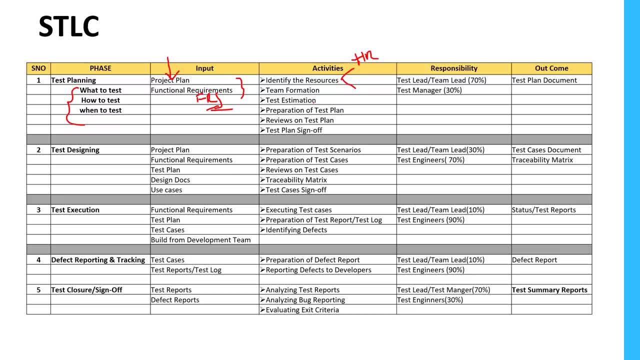 Okay, this is not the job of testing year or test leads. Normally these are the tasks done by the management team and the test estimation and preparation of test plan. And here the main document we need to prepare is a test plan document. This is also a document. 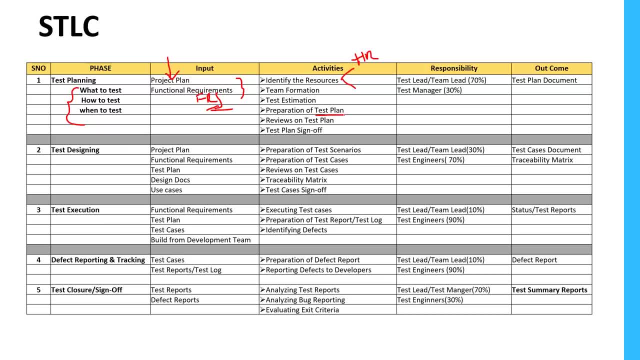 So this document can be. normally it will be in the word format, So I will also show you this one. So while doing our project, we will come across all these documents. So test plan is a document which contains all the information about what are the different areas to be tested in our application. 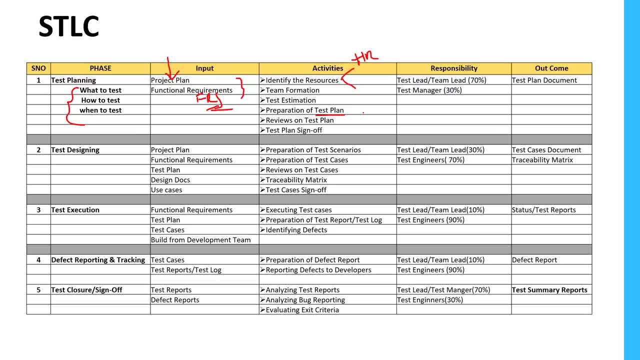 and what are the different type of testings we conduct on this application. and then what are the timelines and what is the what are the team members are involved in during testing. all these things will be part of test plan document. So test plan is very gives the clear picture like what to test, how to test. 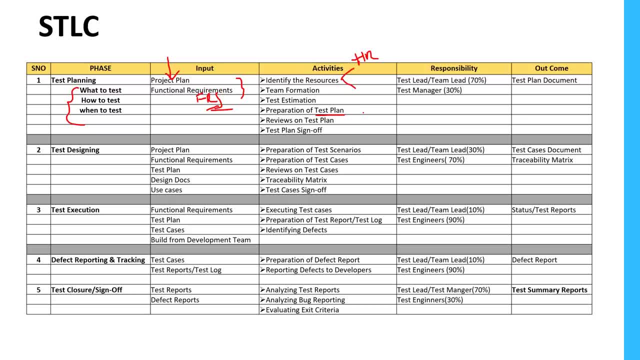 and when to test. so, as per the plan, we need to follow further. So that is our main activity during test planning phase. So the main activity of the test planning is creation of test plan document. and once create the test plan document, also some reviews will happen in the test plan. 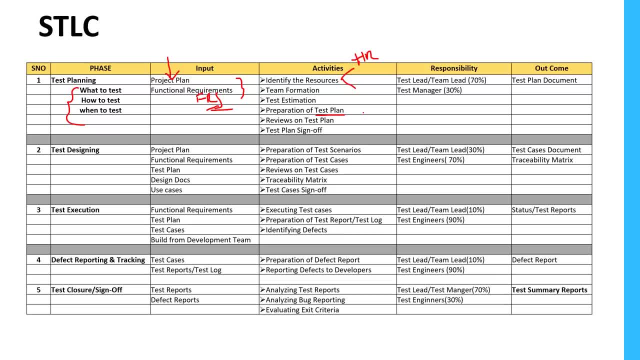 So not only test plan document, any kind of document. If you put there there should be some review happen, Okay, without review you cannot get an approval on this. So once the prepared test plan document is ready- So I hear document higher management will approve the document. 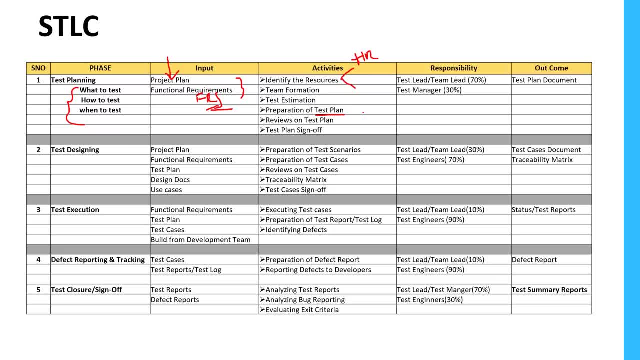 and then we'll proceed further, because you will mention everything in the test plan What you are going to do in the next few days or few months as part of testings. that information will be part of test plan. So test plan will give you the clear picture. 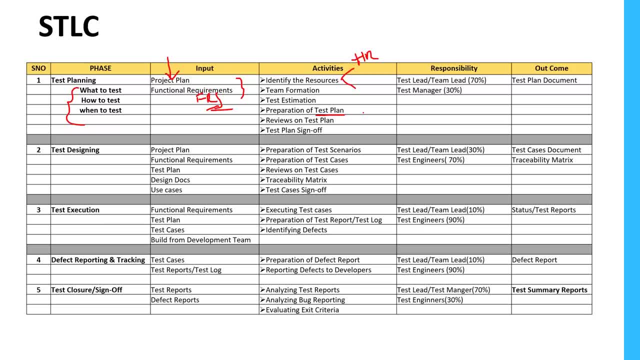 of the management, what you are going to do in future. Okay, and so they will also review your test plan, how we have prepared, what content you have mentioned in the test plan and whatever content you specified is correctly written or not. So those things, so they will review and finally they will give you the sign. 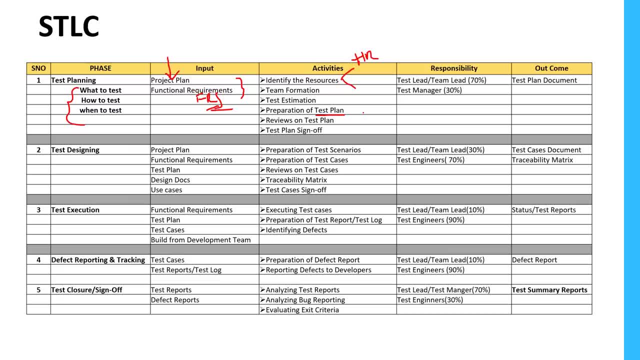 up on document or they will approve your document. So these are the main activities we do as part of test planning phase, the. but here the main responsibilities are test lead or team lead, or test manager. So, as I said before, so the major role will be. 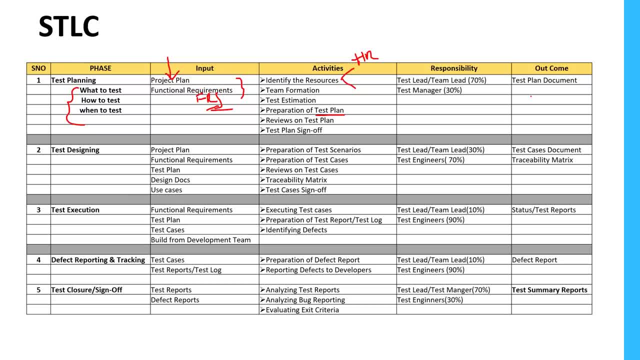 a management management role. So normal test engineers are not involved during this phase most of the times. very less percentage. but 70% of the role will be test lead or team lead because he has to prepare the test plan, and test manager role will be 30% because he has to review all the test plan documents. 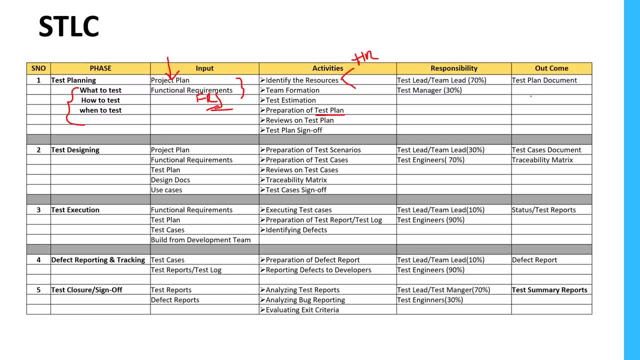 and he will provide the comments and he will ask you to update something in the test plan documents and he has to finally review and approve the document. So his role is almost 30%, and 70% role will be team lead or test lead, because they are the management level people. 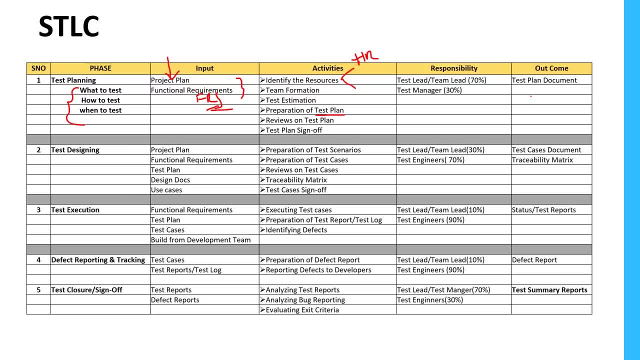 So they will prepare the test plan document and they do these activities. Okay, so there's a first plan, test planning phase and once we have done this phase, what is an outcome we will get is test plan document. test plan document is a output or output document, once we completed this phase. 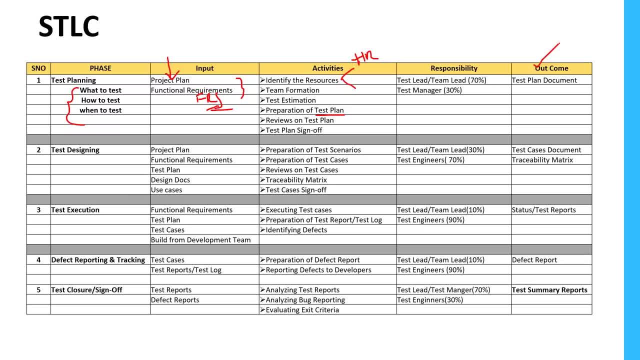 So when you do project also, we follow the same steps. first We do the planning and we do the test designing. then we start execution of test cases, then we will identify and reporting the defects. Finally we close our testing. So these are the same sequence of steps. 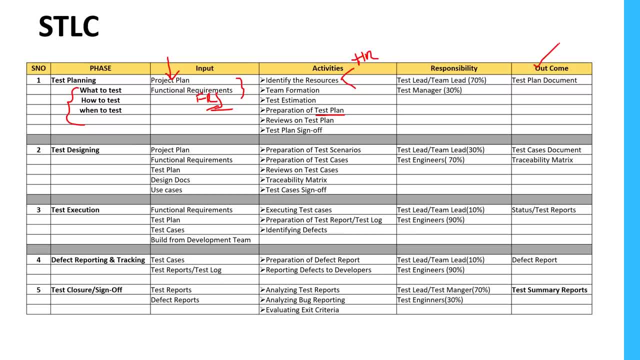 We follow while we are working on project also. So first stage is test planning. So we will get test plan document as a output and, once the test plan is completed, and review and approve and then we will move on to the next phase, that is, test design phase here, actual testing. 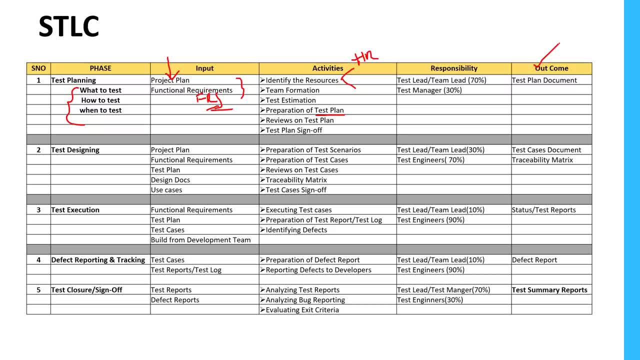 In your role will be there, very important role. So test designing and execution, defect reporting. So first and fifth phase one and five, mostly management team will be involved- Okay, senior people- but two, second, three, second, third and fourth, these three, four, three stages, the major role will be the testing. in here 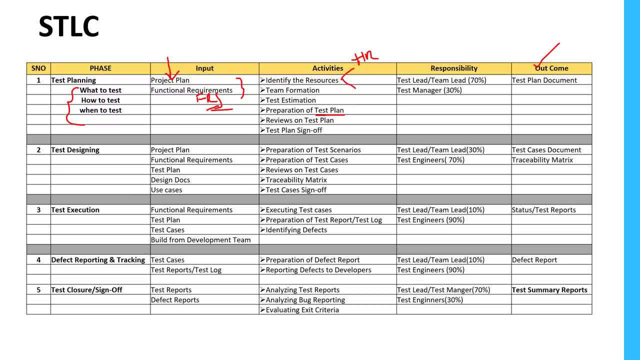 Okay, so test designing is the second phase and during this phase, what is the input documents we require? is project plan, Functional requirements test plan document, because this is already done in the first phase test plan document and sometimes we need design documents. So, based on the functional requirement document to sometimes we cannot understand the complete functionality. 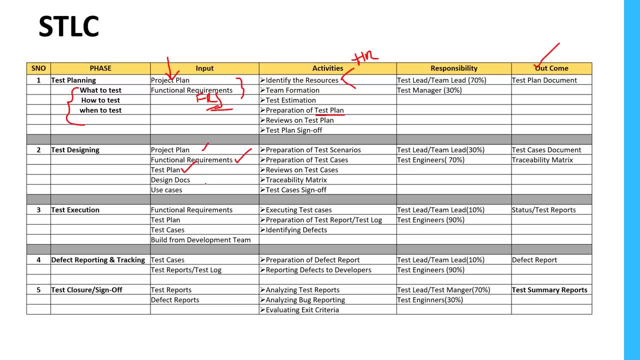 because sometimes functional requirement doesn't have the complete information. They will give the all the requirements in the form of text. So sometimes they don't provide any pictures or screenshots of application dummy screens and all. but if you have those things we will get the complete picture how the application will be, how application behavior. 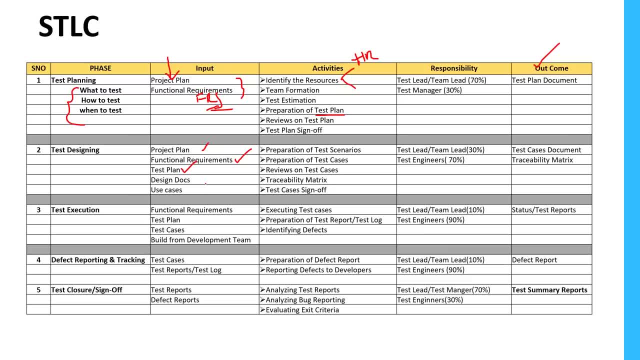 how it works and what kind of features to be tested, So we will get clear picture while writing your test cases. So until unless you know the functionality and all the flows, he cannot write your test cases. So that's the reason we need to refer these document very clearly. 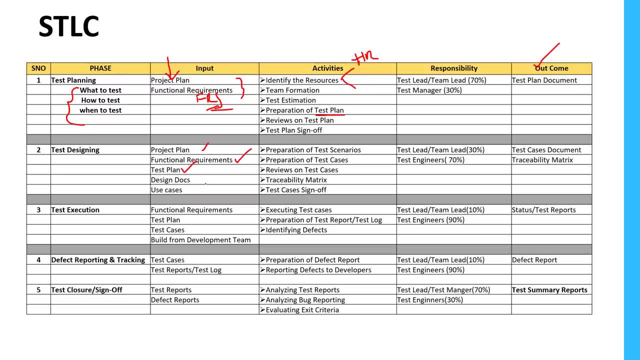 and once we get confidence and then we'll start writing your test plan test cases. Okay, So these are all input documents We need to refer during test design phase. So test plan, Project plan, functional requirement, test plan document- because test plan contains what are the areas to be tested. 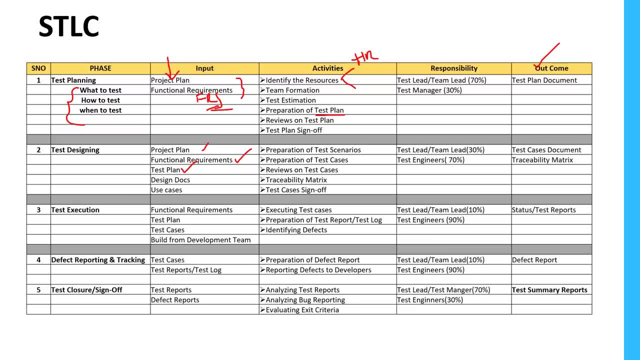 and design documents. design document in the sense: sometimes they will provide some data flow, diagrams, flows, a screenshots, Okay, and all the things will be available under design documents and use cases. use cases also a kind of a document which contains the some picturized format. every requirement will be part of a described. 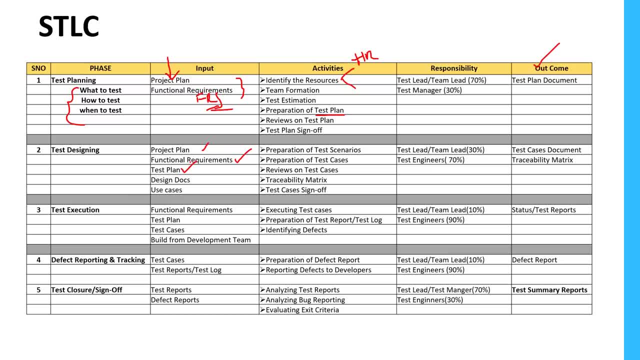 in the form of pictures. So while reading the test, instead of reading the complete test on paragraphs, if you see the pictures, you can easily understand the flows right. So use cases will be part of requirement again. It will give you the detailed description. 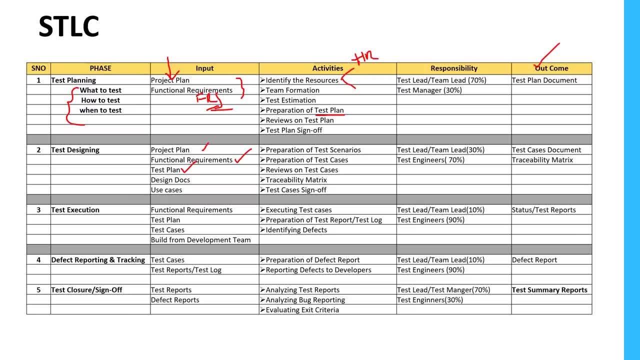 and information about the requirement, That's, the use cases, will be part of functional requirement. So these are the input documents we required at the time of designing phase. So testing in here should refer all these documentation. So why we need to refer this? the main objective of to understand requirements very clearly. 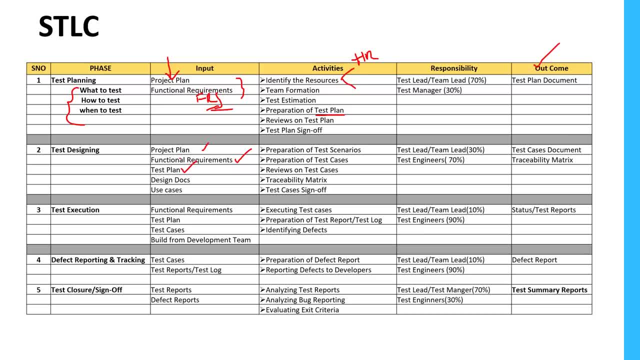 until, unless you know the requirement, you cannot test application through fledgling. Okay, So this is all. these are all input documents and based on this input documents And once we refer this document, we do set an activities especially for the test. engineer role will be 70% here. 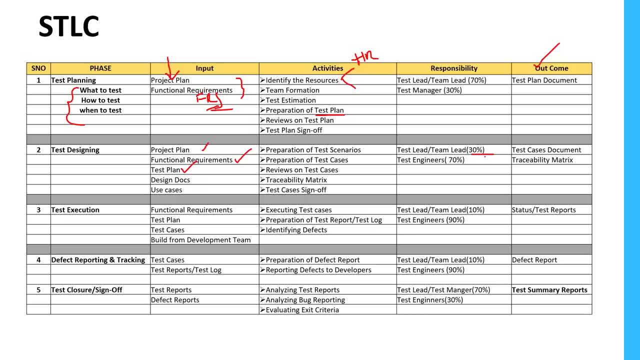 and 30% role will be team lead or testing, So they he will monitor the team and he will just solve All the issues whenever comes and he will assign some tasks to the test engineers and that role is a little bit management level but maximum the major role will be testing here, 70%. 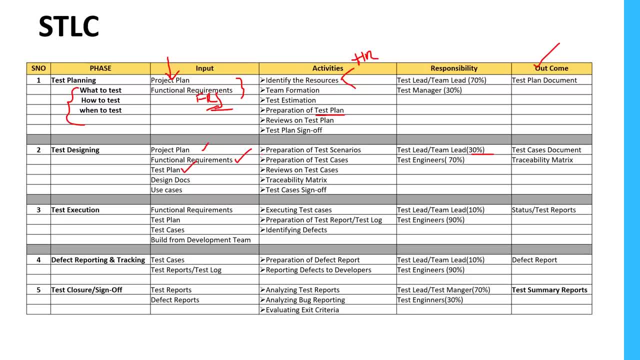 of the role will be: the test engineer has to do all these activities. So preparation of test scenarios. So, based on function requirement, design document, use cases, Once we have understood, we will prepare test scenario. So what is test scenario? test scenario describes what to test. 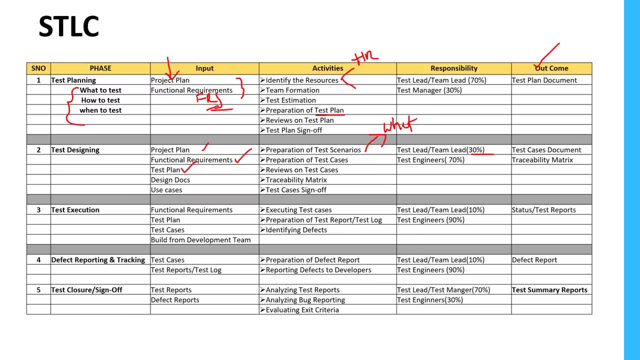 Okay, in the application, What are the different scenarios we need to test? So, for example, if I take a banking application, so login is one scenario. one transfer is one scenario. Okay, check balance is one scenario. creating the statement is one scenario. So these are all different scenarios. 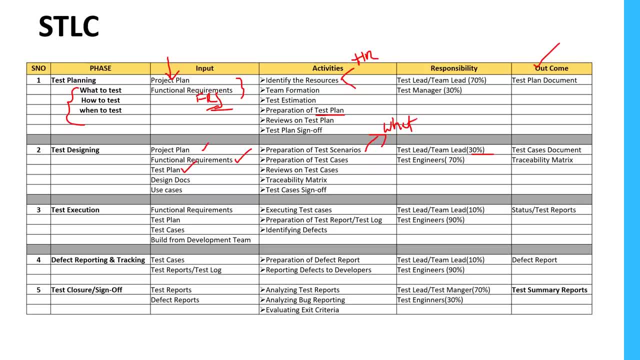 So we need to prepare those test scenario based upon the functional requirement and for those scenario again we need to write in detail steps. Suppose, if you have a login scenario, so how to test this login, We need to write steps called as a test cases. 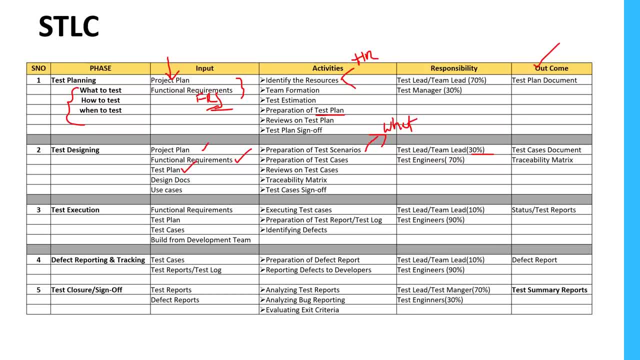 So for every scenario there may be one test case, or sometimes there may be more number of test cases. If the scenario is very larger, then we can create multiple test cases for the single scenario. So we have to also create the test cases. So test case is in the sense: 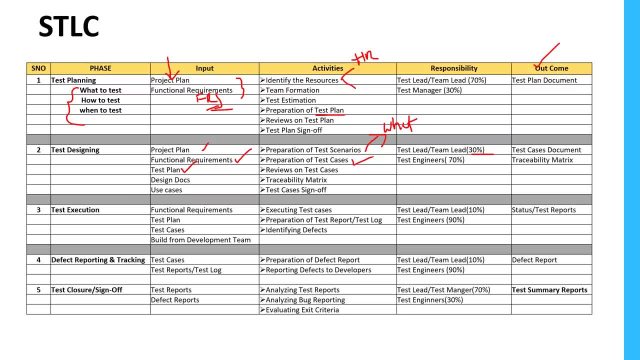 It is step-by-step actions: expected result, What is an actual result? Everything will be there as part of test case document. So we'll discuss that into next two slides and this is again Very important and main activity of the test engineer, So he has to prepare the test scenarios. 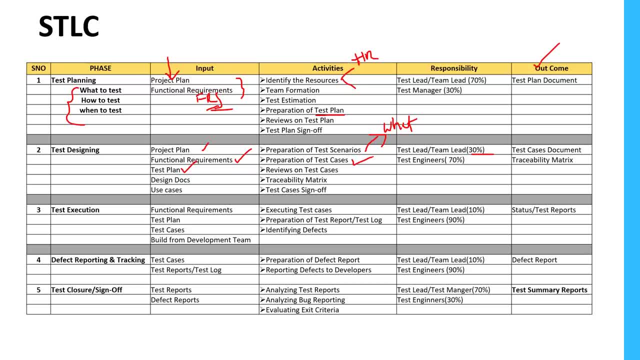 and he has to prepare the test cases and he has to conduct reviews on test cases again. here They need to conduct peer reviews. peer reviews means you need to review that augment with your colleagues in the team And once your team is okay, and then you need to again review with the development. 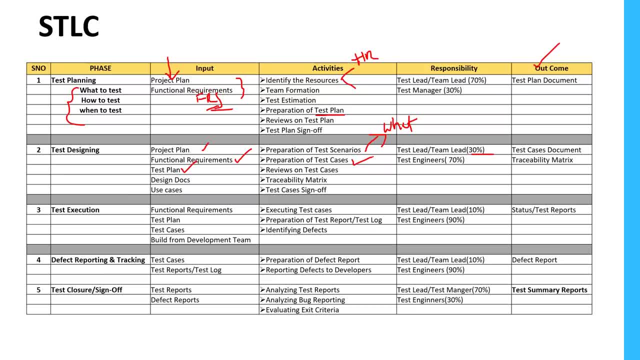 and testing and product management teams And finally, everybody should review it And if you want, if they want to add something else or some other scenario, you should able to add them and again reread it and after multiple reviews, then finally it will be approved by the manager. 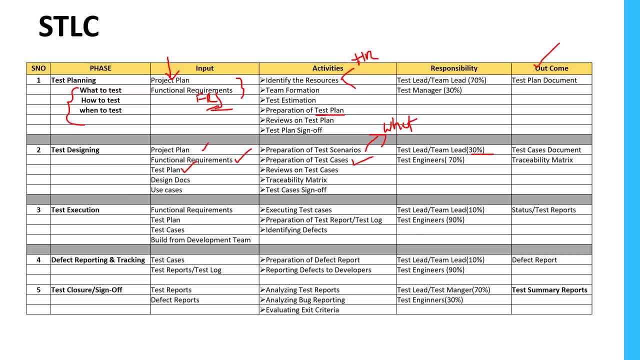 So that is about test cases, reviews about test cases, And we also prepare the traceability matrix here. So traceability matrix is a kind of Excel document, Excel file spreadsheet, and which contains the what are all requirements we have, what are all corresponding test cases we have written for those requirements. 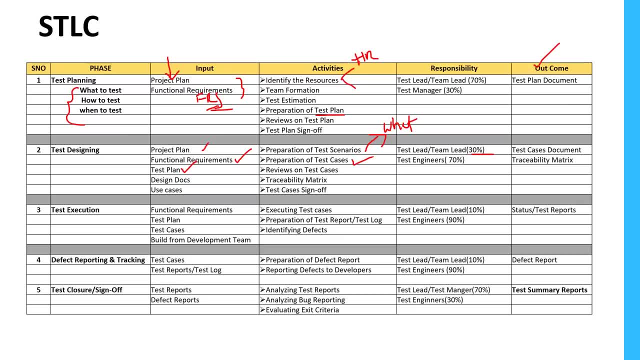 It is basically the mapping of requirement and test cases, So that's called traceability matrix. So we will see all these things in the coming slides- how to prepare and how it will be. traceability matrix preparation is also one of the activity, and then, finally, we need to get the sign off on test cases. 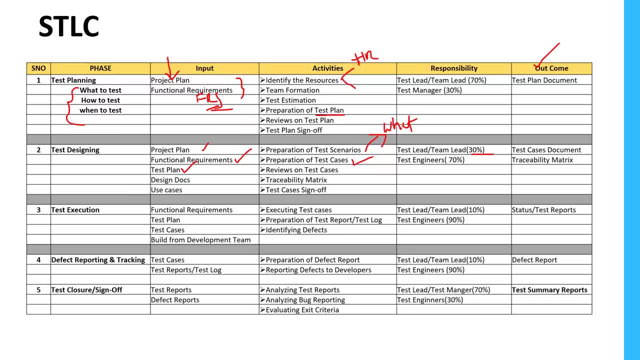 So from everybody, what development product manager management team leads, and everybody should able to sign up the document test cases and then, once they sign off and approved, then we can execute Those test cases. So these are all activity we do as part of test designing phase preparation. 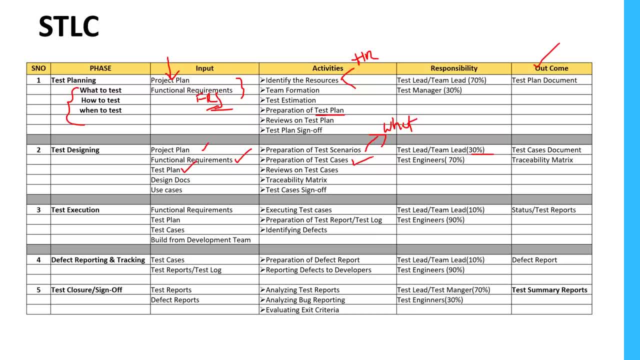 of test scenarios, preparation of test cases and review the test cases along with the team. and we need to also prepare the traceability matrix to check the mapping between requirement test cases, because traceability matrix is very useful which will give you the clear picture. like do we did? we created test cases. 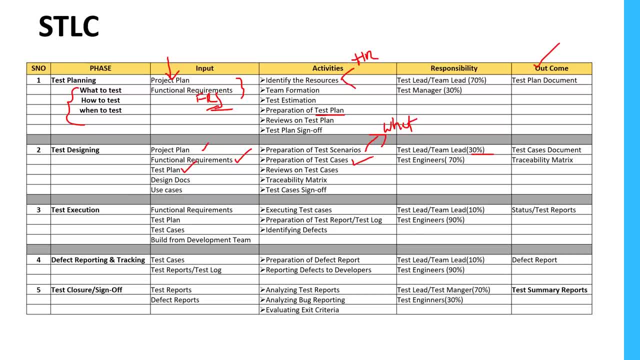 for all requirements or not, or do we miss anything? So that kind of clarity the traceability matrix will give you and finally we will review with the test cases and get the sign up from complete the team and then we are ready for execution. So before going to the execution part, test execution part. 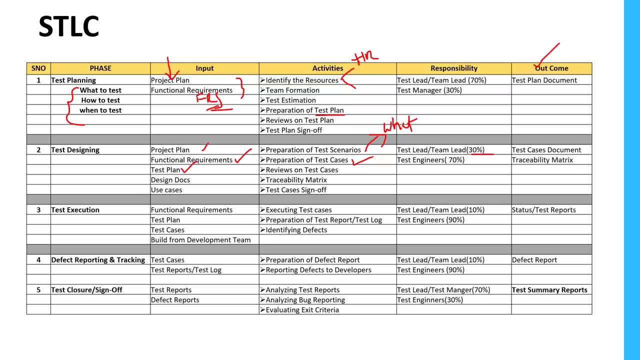 we need to ready with all the documentation part. So test cases, test scenarios, everything should be ready and approved by the team. So that is a test designing phase. So in this phase the team lead and activity will be 30% and he will just participate and monitor the team. 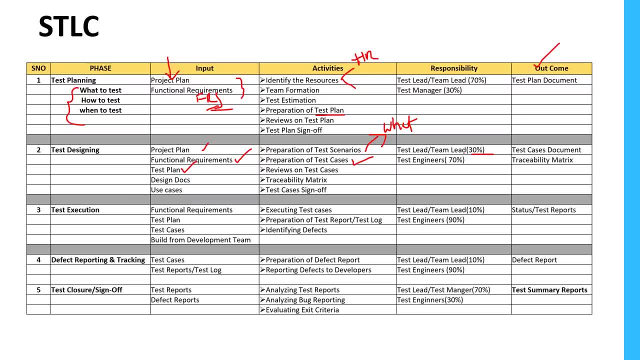 He will assign the tasks and test engineer role will be 70% because he has to create all the stuff. So he has to create test scenarios, He has to create the test cases, reviews and traceability matrix and he has to get the sign up from the management team. 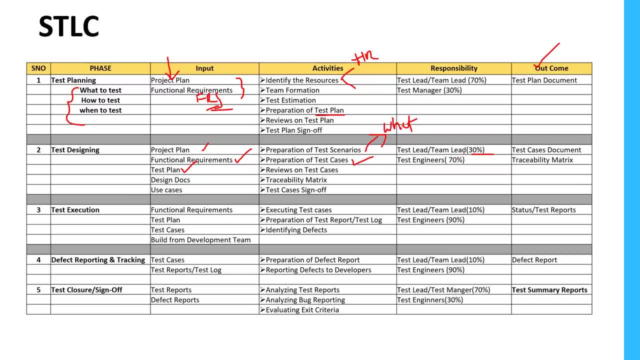 So the test engineer role will be more here, test designing phase as an outcome. what we will get once we exit this particular phase, We will have the test cases by hand and then we'll have also traceability matrix- test cases document and traceability matrix. 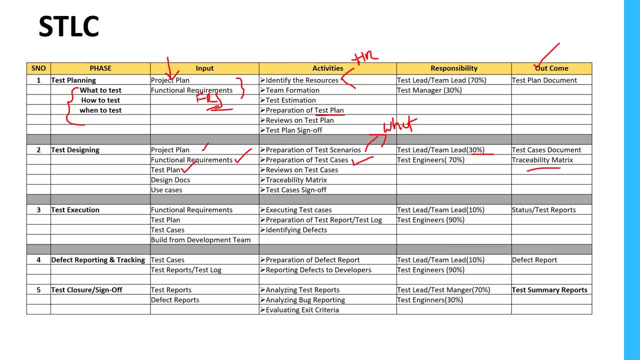 So these are the two documents we should have in by hand before exiting the test design phase. So once we have test cases and traceability matrix and everything, we will start test execution. So by that time we need to also get the bill from the developers. 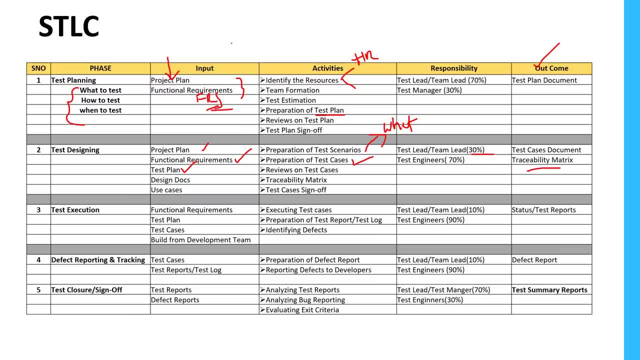 So these are a parallel activities. a developer from they said they will understand requirement They do design the, develop the code, they will create the build. So those tasks are done by the developer side and the parallelly and the tester also will do the these activities test. 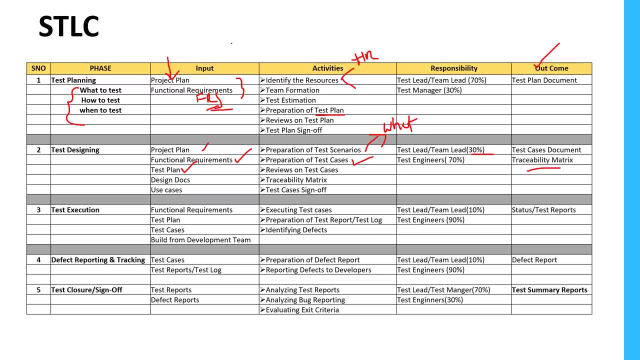 running test designing. by the time we completed test is designing, developer is ready to send a bill to our testing environment. So in that phase test execution will start. So as soon as we get the bill from the development team, once we have these documents, then we can start execution our test cases. 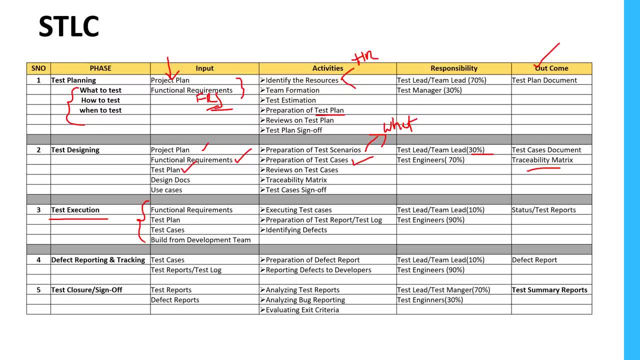 So what are? the input document We should ready with the when, at the time of test execution, is functional. So what are the requirements? test plan document, because test plan document. if you have any doubts about the functional requirement, we can just again re-verify the function requirement document. 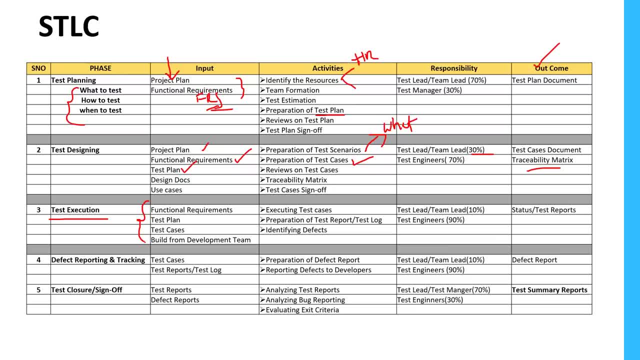 and also the timeline is very important and we test plan contains the timeline, So those time is we have to follow. and test case is also very important because the test case is only will able to find the defects in the software. So test case describes what to test, how to test. 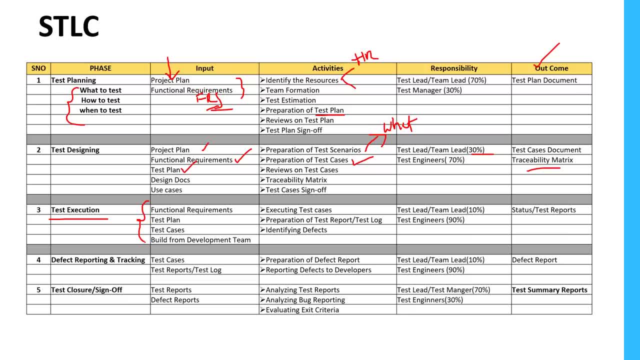 and what is an expected output from the application. So everything will be Available in the test cases, or test case document, is also very important for us and these are all documents. So with this documents we need to, by using these documentation part, by referring those document. 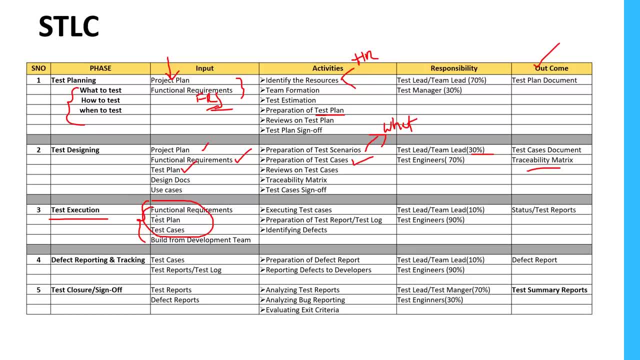 We need to test. the build means build is nothing but the final integrated product from the developer. So we need to also get the bill from the development team. So once we get the bill from the development team, then our activities will start. So our documents are ready. 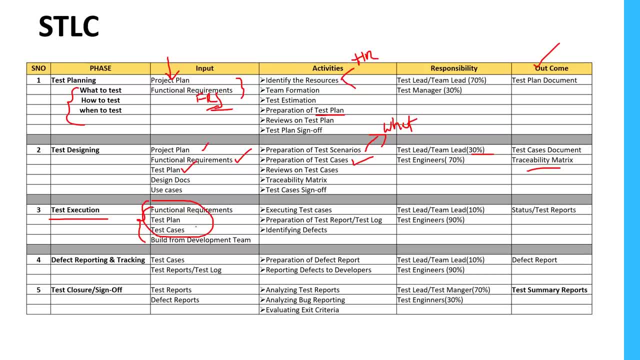 We get the bill from the development. So now we are start execution. So what are the activities we do as part of test execution is we will execute our test cases. So whatever test cases we already done- created, approved in the previous phase, tested, designing phase- 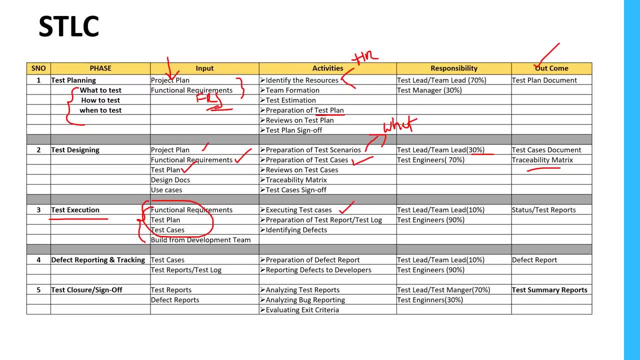 We will execute those test cases and, while executing your test cases, you will prepare the test report, also called as a test log document. So what is this means How many test cases you have executed, How many are passed, How many are failed. 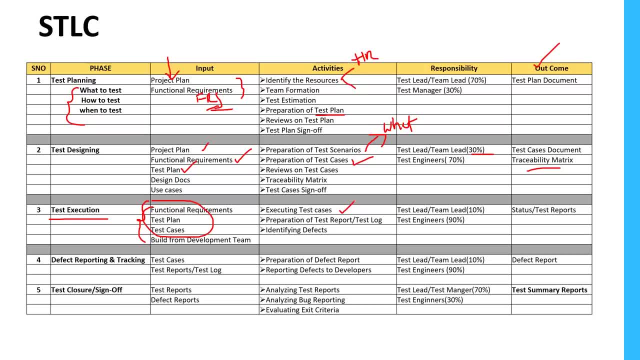 How many are blocked? Okay, so how many defects you have raised So that information need to specify in the test report, because this is a very important document which we need to send to the management test report. on the day-to-day basis, You need to send a status to the team or management. 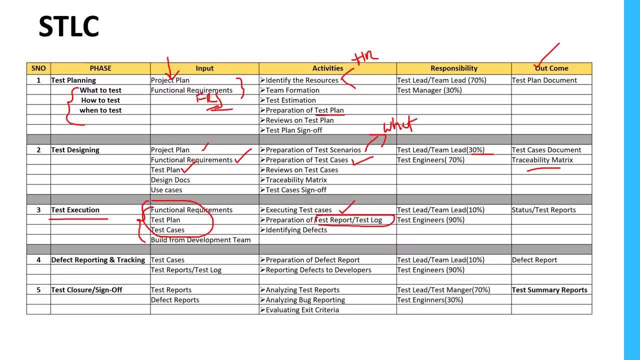 Okay, on the particular day, How many test cases have been executed, How many are failures you identify and how many defects you re-verified. So this kind of information will be part of test report. This is also called as a test log document. 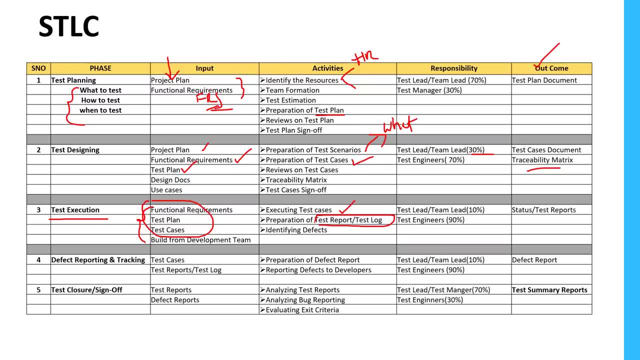 That we need to prepare and the main activity is identifying the defects. So why we are executing test cases? because we need to identify the defects. So if somewhere, if you found some mismatch behavior, suppose we are expecting something, but actually in application, is behavior in some different way. 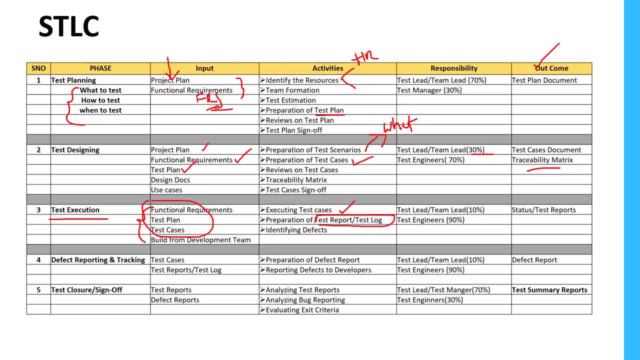 then we will expect, we will observe, the will notice the mismatch behavior and those kind of behavior will consider as a defects and we will report that information to the developer. that is called as a defect reporting process. Okay, so we'll take- we'll talk about default reporting process. 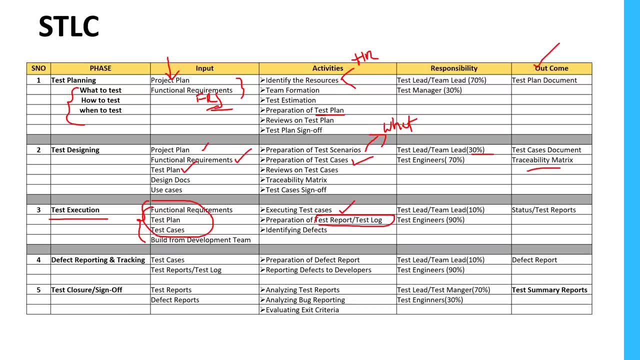 in detail in the coming slides. So these are the main activities we do as part of test execution. So execution of test cases, preparation of test report and test log document and identifying the difference. So these are the very important activities We do as part of test execution. 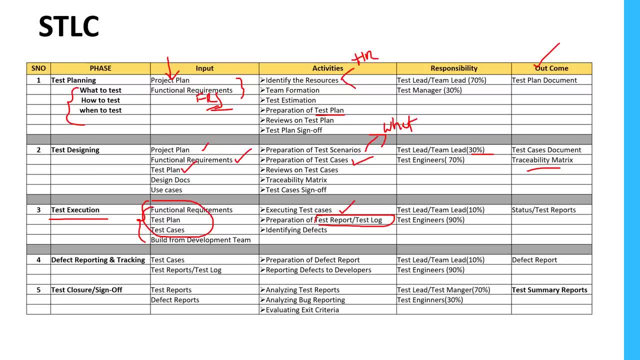 and here also test engineer role will be more. almost 90% of the role will be played by the test engineers, and only lead will just coordinate the team between the testers and developers. He will review what our test cases are. He will review what status report. 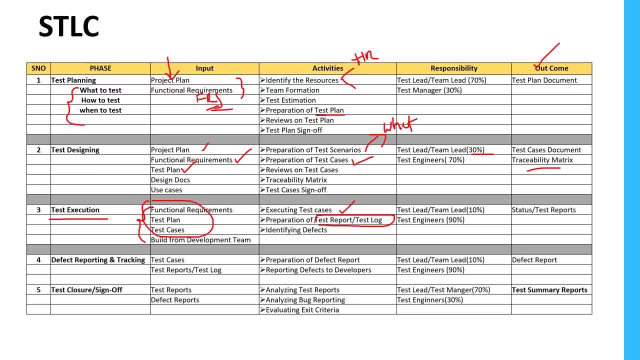 and he will review what defects, what you have found, and also he will review the you will. he will communicate with the development team if there are any issues. Sometimes you will say something is not working, that is an issue and sometimes a developer will say that is not report school. 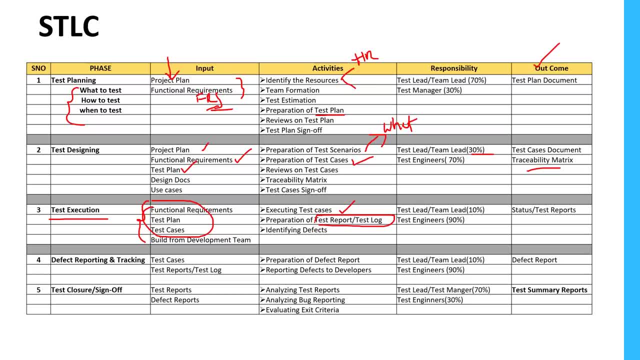 in our environment and that is not a bug or it's not a defect. So like that, the developer will says so, the team need or test. it is a responsible for coordinating the teams, or developer or tester or management in everybody. So there's a role is only 10%. 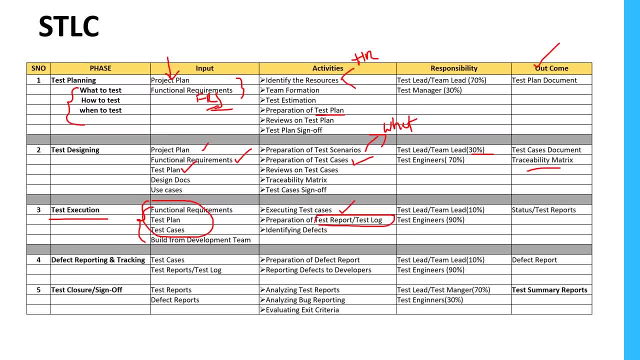 but 90% of the role will be testing, because he has to create the test cases, He has to execute it, He has to prepare the test report, He has to send the test report to the management and he has to identify the all the defects was a major 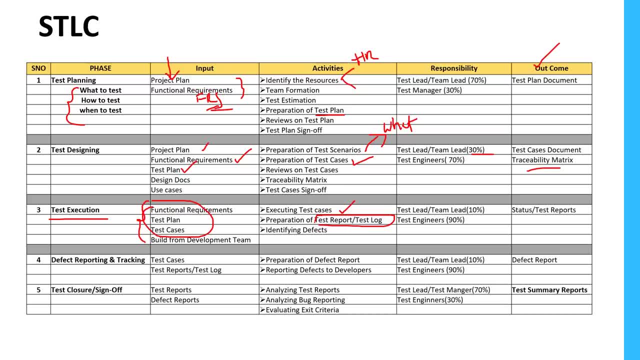 and very important task of test engineer. And finally, what is the outcome will get during this phases: status reports. Okay, so that is our state test execution phase: test planning, designing and execution. So this test execution will happen multiple cycles, because at least two cycles we have to do test execution. 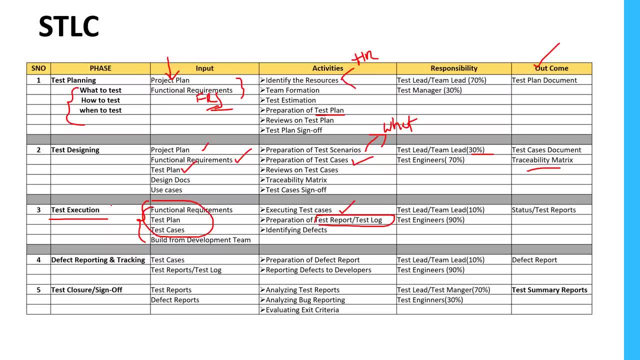 because every time we will get multiple bills from the developer. developer don't provide the company stuff in one build itself. Okay, they will introduce some functionality in first build. in the second build They will introduce some more functionality. in third will they will introduce some other functionality. 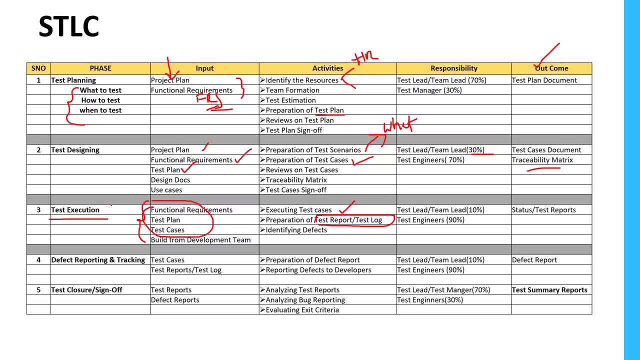 and along with the functionality they will also fix some bugs. So whatever bugs or defect we reported to the developers, they will also resolve those bugs and again they will implement those fixes in the newer bits. So every bill we need to test. So these testings will be done multiple cycles, not only one. 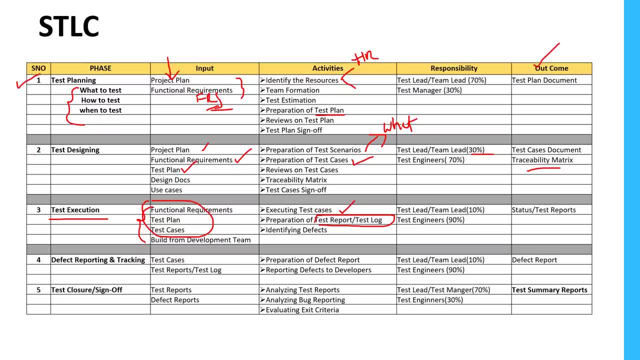 cycle but test planning is one cycle happen test designing only one time activity and test execution, defect reporting. These two are happening Multiple cycles because every time as soon as we get the bill we execute our test cases will find out the defects report to the developer again. developer will fix those defects. 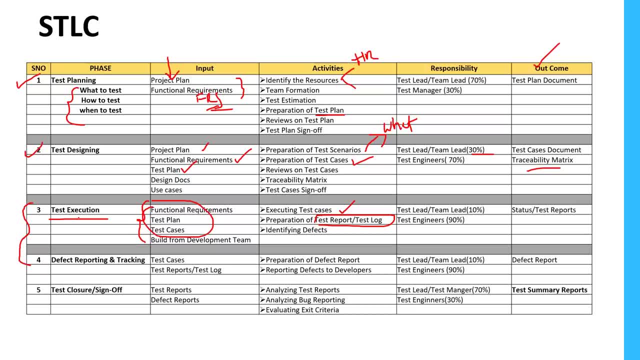 and also they will add a few more new functionality and provide the new pin again. We will retest. So this is a cycle will go on till we reach the end of the test cycle. Okay, at least two cycles are minimum, So after that we'll go as many as possible. 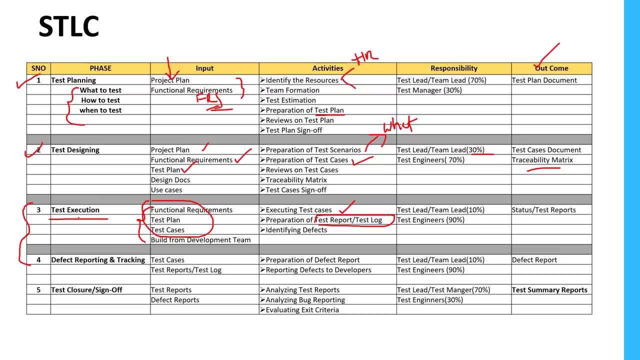 but that is again should be part of the test plan document: How many cycles we need to execute, how many bills we need to get from the developers. So these are all will be part of your test plan documentations. Okay, so that is a test execution phase. 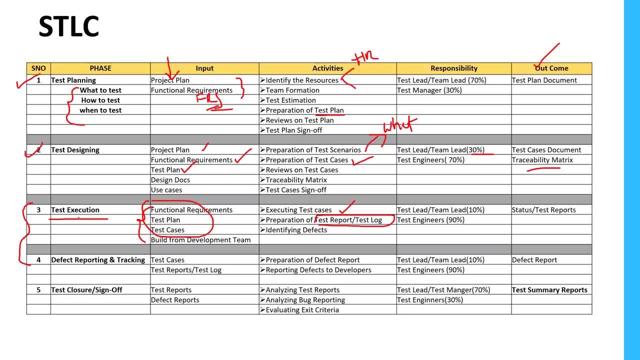 and then defect reporting and tracking is also part of our test execution. It's not a separate phase. Actually, This is the sub part of test execution, because when you will find the defects at the time of test execution, if I execute our test cases, then only will identify whether 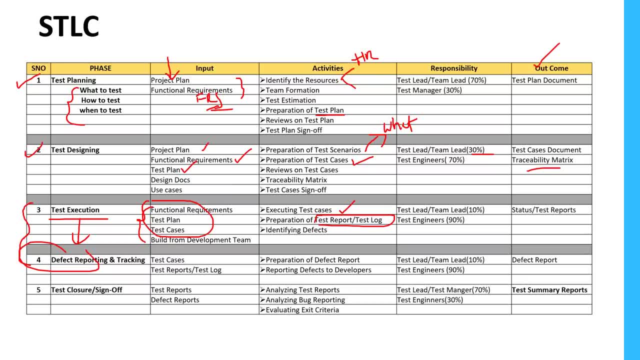 the having defects are not. So as soon as you found some defect, you will report the defect to the developer. and what is tracking? So once you report to the developer, you need to track the defect. So what is the status of the defect or developer is going. 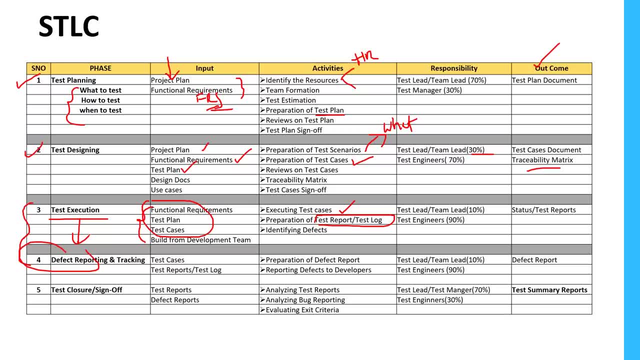 to fix the defect, or it is pending, or developer is not accepted this defect. So what kind of status it is so that we need to track till we rise that from we rise the defect till we close the defect. So each and every step we need to track that particular defect. 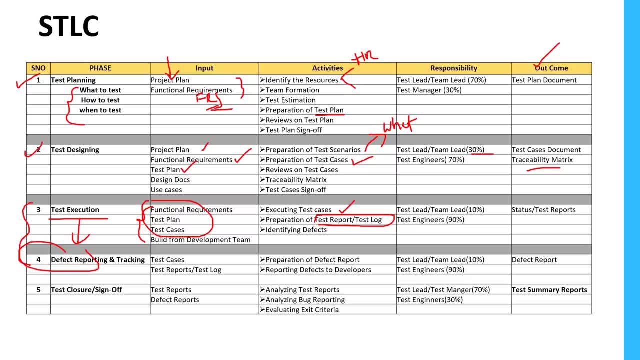 So that is the defect reporting and tracking. This is not a separate part. This is all already part of test execution. So here we will refer the test cases and test reports and preparation of defect report. That is a very important So how we will report the defects to the developer. 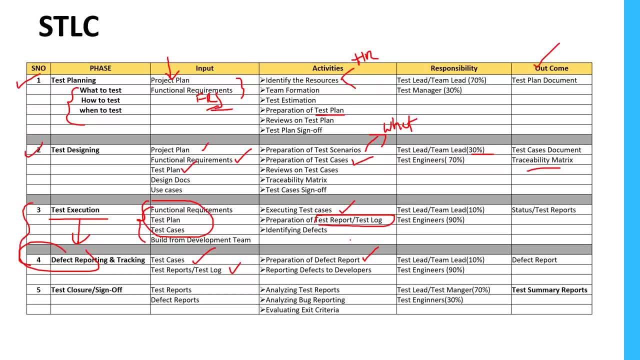 So normally nowadays some people are using tools. Okay, I'll tell you how to report the defects using Jira tool in the next session, but normally we will just list out all the defects In the Excel file, initial level, and at the end of the day. 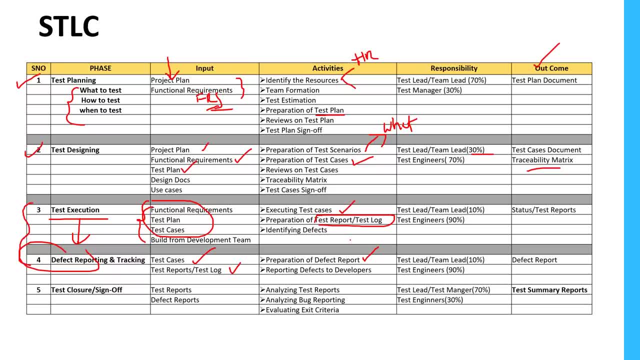 we will just put everything in the bug tracking tools. So when I report this defect to the developer, we need to provide certain content, like a defect ID, defect description, What are the steps we have to perform and if screenshots are required, we need to also send the screenshots and logs. 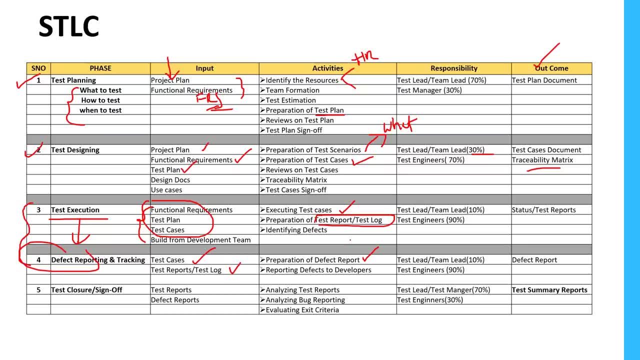 So there is a lot of information We need to send to the developer. So developer will read the all information and then he can understand the what is the defect, how it is happened, where it is happened And once he get clear picture on the defect. 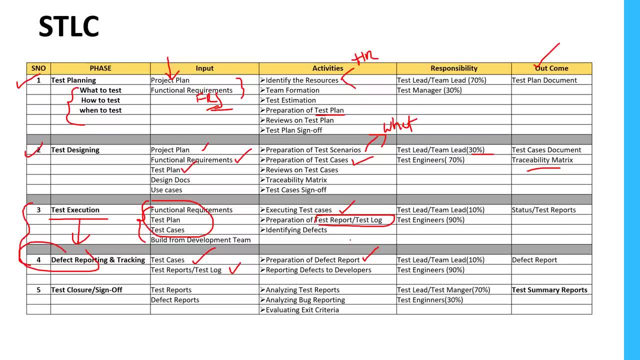 then he can try to fix the defect. So that kind of information we have to provide, and sometimes the developer so says. whatever information we have provided, that is not enough to understand clearly. So in those cases you need to try to some more information. 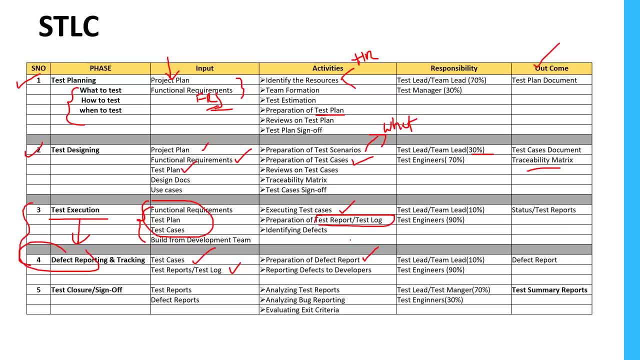 You need to provide some more information regarding the defect. So this is all part of defect reporting and tracking phase. So here the main activities: preparation of a defect report and reporting defects to the developer. So this is the main activity we do as part of defect reporting. 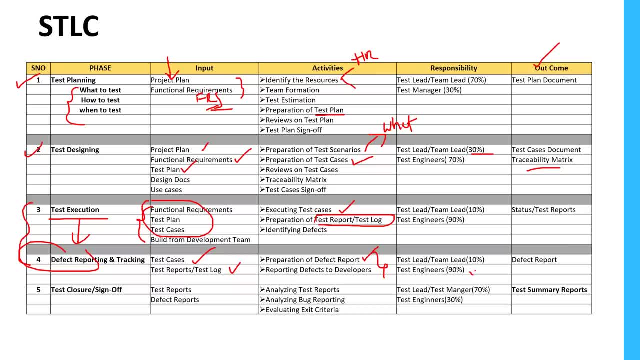 and here test lead role again 10%. testing year role will be very high, So 90% of the involvement will be the testing and the final outcome is a defect report. So defect report is a kind of Excel document which contains what are all defects we raised on particular bills. 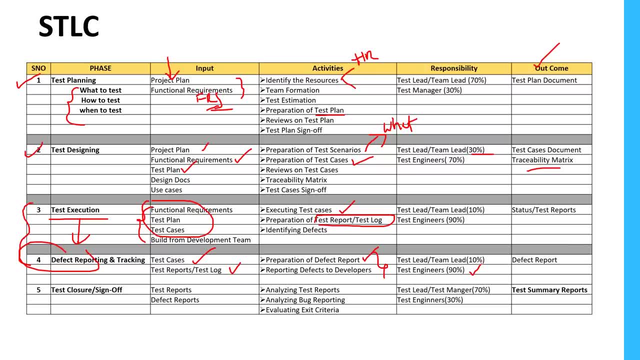 and how many are fixed on. we are still pending. how many are yet to verify. So this kind of information will be there under defect report. So this is your defect reporting and tracking piece and once we tested all the bills and almost every defect is closed, verified and closed. 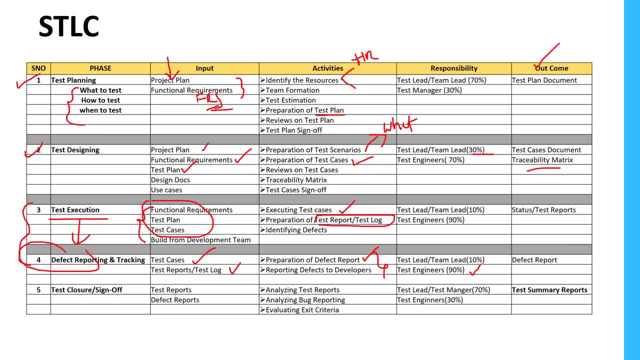 So there are no more bugs in your software. Then finally, we will end up the session, end up the testing. So that is test closure phase or test sign-off phase. So this is again leads and management activity. So once we enter into the fifth, 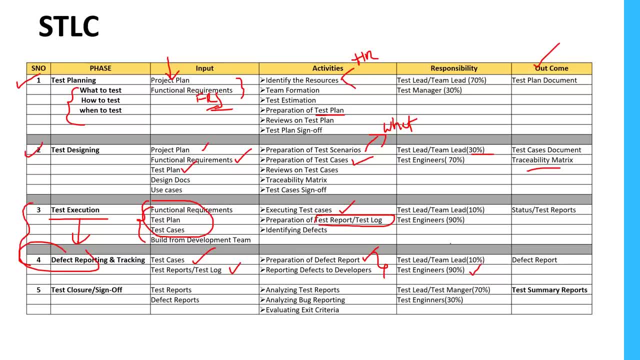 so they will do set an analysis. So, based upon the test reports, we provided defect reports We provided to them. They will analyze these reports. Okay, are we good to go or not? So that final decision will taken by the management. 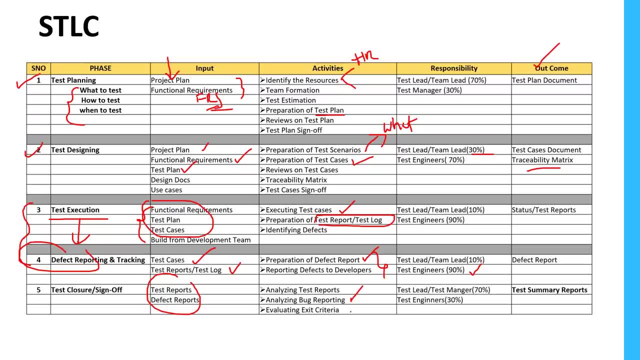 So here they will analyze the test reports, analyzing the bug reporting, They will evaluate the exit and the entry criterias And finally they will take the decision: Do we need to stop our testing or still we need to continue our testing? So that kind of decision they will take. 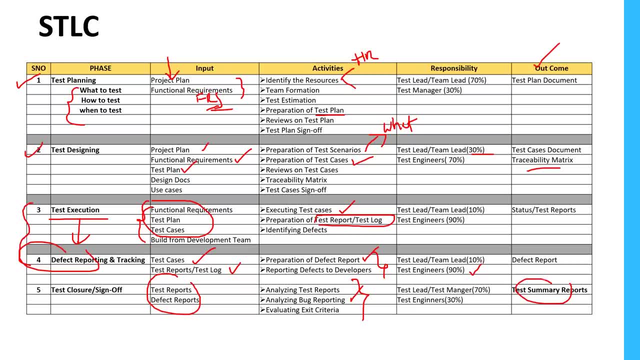 and finally they will send this test summary report Means all the documents, whatever we prepared so far, combined together We call a test summary report and will send to the customer. So here the main activity will be test lead and test manager role will be 70%. 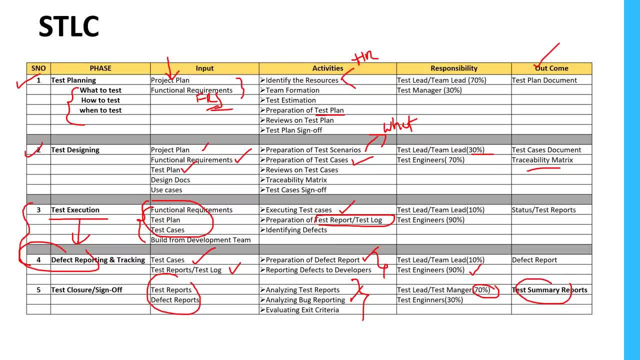 because they are the approvals, So they are the decision maker, So their role will be very high and testing years role is only 30%. Okay, So just they have to demonstrate what are the test reports and defect reports, but the final decision will be taken care. 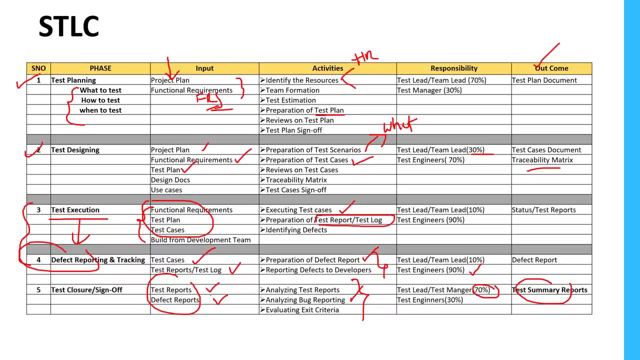 by the test lead and managers. They will review these documents and, based on that, they will take the decision and they will stop our testing. once we completed this, then we will hand over the build- final build, tested build- to the next team that is called you. 80 test loser acceptance testing. 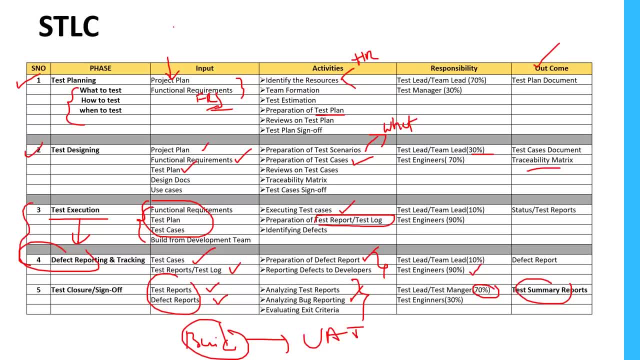 So this is all comes under the system testing I said before. right, So there are four levels of testing: unit testing, integration testing, system testing, UAT test. So system testing is a third level of testing. So in the system testing we do all these activities. 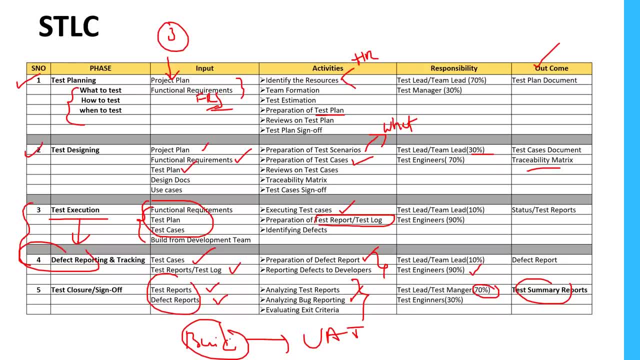 and once our system testing is completed, then we'll hand over the final build certified bill. certified means we have done So. after completion of all these activities, at the end we need to certify that build QA team should certify the bill. Okay, so, and so bill is certified and everything is working fine. 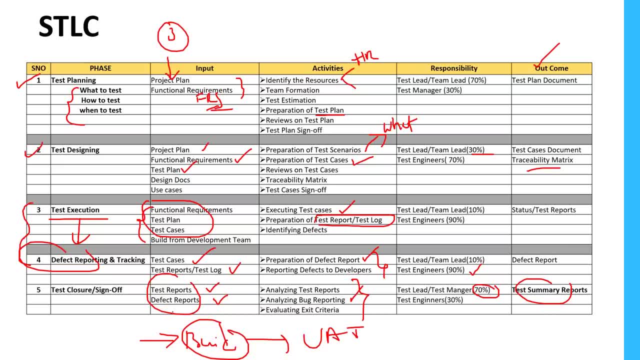 So we have tested so and so things. So these are the report. So, along with all the documentation, we need to approve and sign off our testing and then this bill is handed over to you. 80 user acceptance testing team and then they will process further. 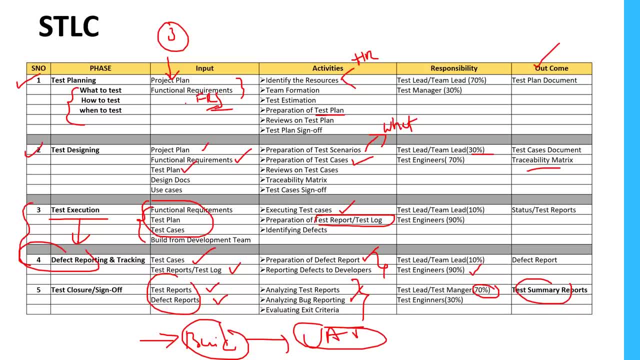 So this is how STLC works. This is a complete testing process in testing environment, in QA environment. as a test engineer should follow all these things: Okay: test planning, test designing, test execution, different reporting and tracking, and then test closure. Fine, So now let us discuss in detail, one by one, test planning, test designing, execution. 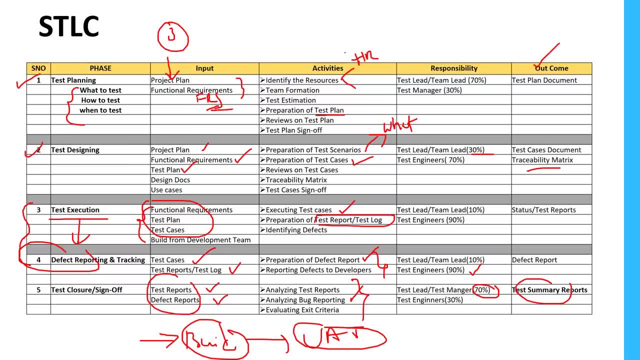 defect reporting and test load. This is very high limit. If you understand this table, it's very much clear about what are the different phases, What are the input documents we require and what are the different activities we perform and what are the different people. 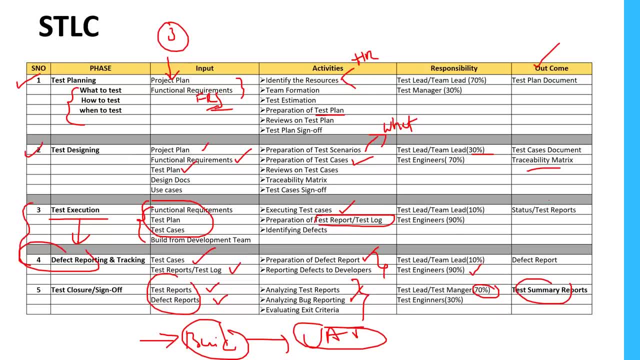 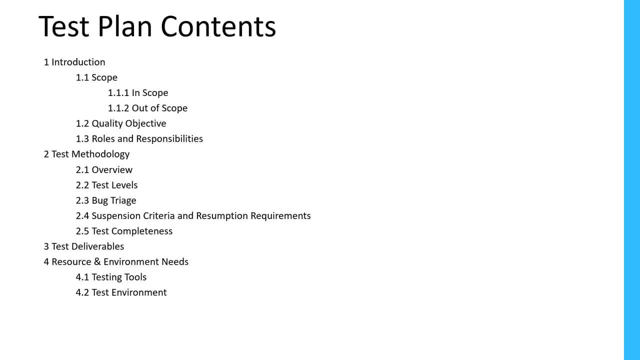 and their responsibilities in each and every phase and what is an outcome we will get once we completed that particular stage. Okay now. so let us move on to the test plan. So the first activity is a test planning. So what is the main activity in the test plan is creation of test. 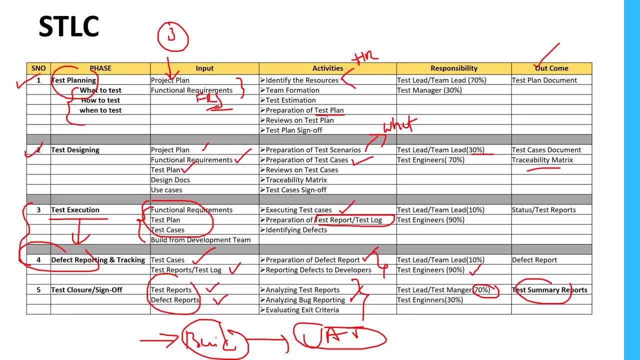 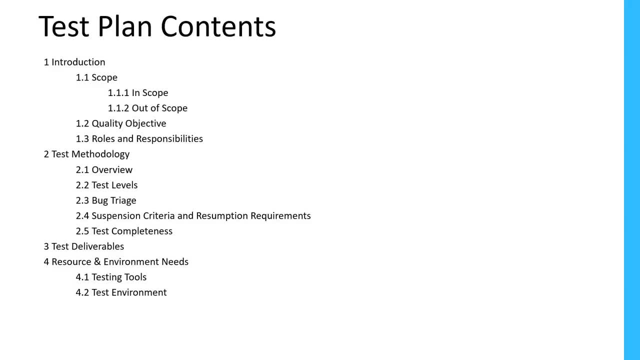 Plan document. creation of test plan document is a very main, important activity, So this is the outcome we need to get from the test plan. So what is the test plan? So test plan is a document which contains the scope of the testing. scope was schedules, timelines of our testing. 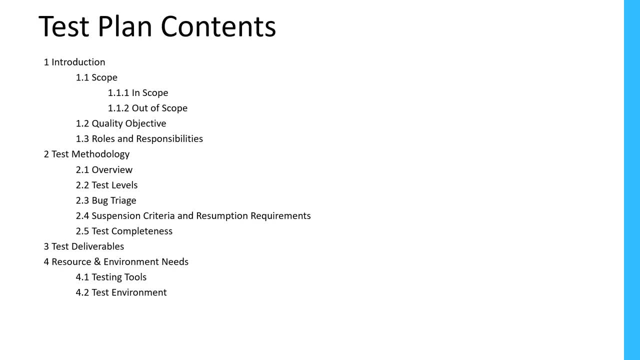 So simply document which will be prepared by the team lead or test. So what it contains normally is a introduction about project. What is the scope like? what to test, what not to test? Okay, out of scope and in scope. What are the different functionalities to be tested? 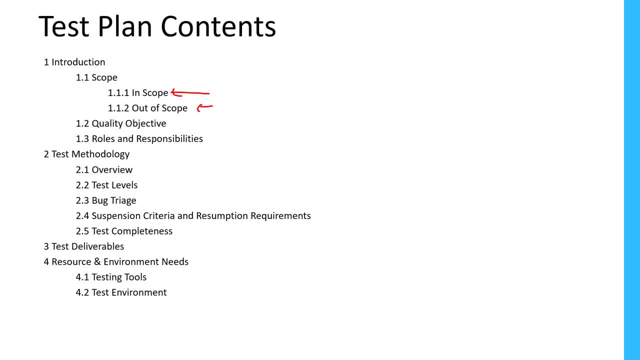 and what are the different functionalities should not be tested and what is an objective. What are the rules and responsibilities of the people and what are the test methodology we follow? What are the different levels of testing We do- bug tracing and suspension, presence and criteria. 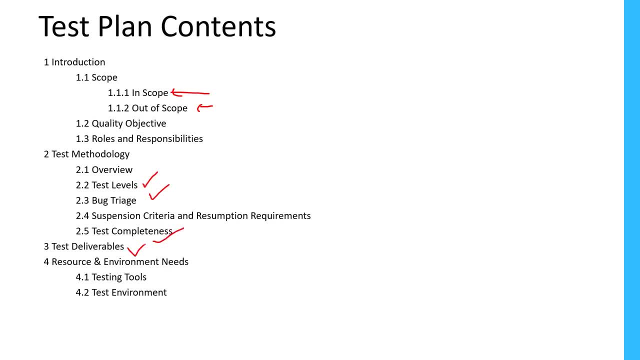 and what is the criteria for test completeness? What are the test deliverables or means in documentation? What are the different documents we create and resources and your environment needs, What are the testing tools we use during testing and what kind of environment We need to set up. 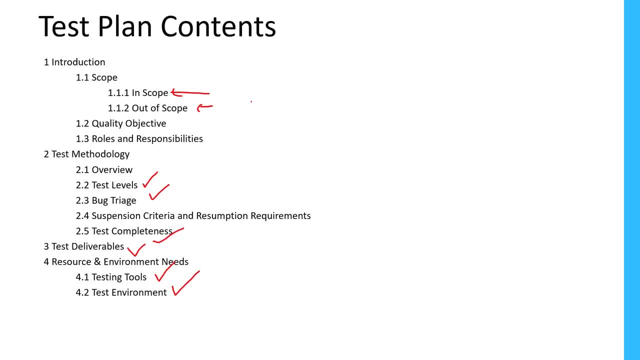 So all these details will be part of test plan document. All the details will be part of test plan document. So this says majorly what to test, what not to test and the timelines, schedule, environment. different type of testing should be kind of what type of testing should be conducted. 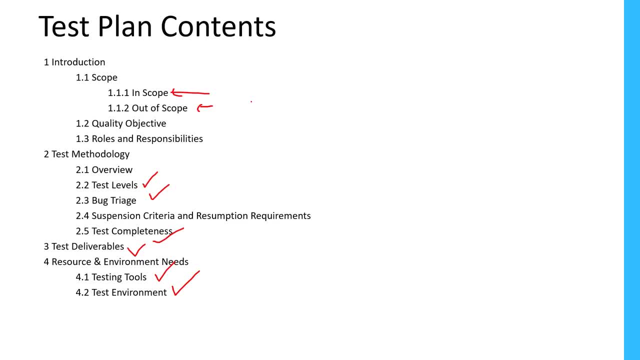 So how many people should be involved? What are their roles and responsibilities? So all the things will be part of test plan document. Okay, so this is. these are the different content We have in the test plan content: test plan document. So, if anybody asked an interview, what is test plan? 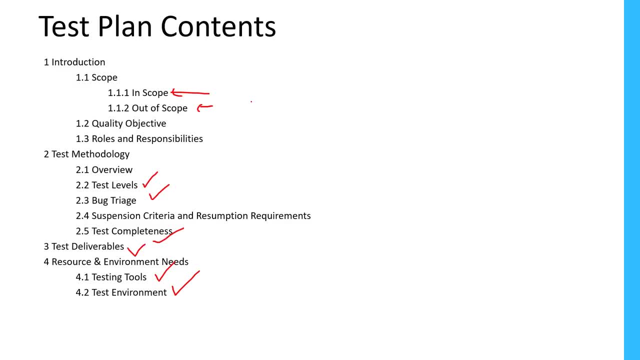 What it contains. you have to say, test plan is a document which will describe the scope of the testing: What, what are the features to be tested, What are the features not to be tested- out of scope or in scope, and schedules, timelines, resources. Okay, so all these things will be part of test plan document. 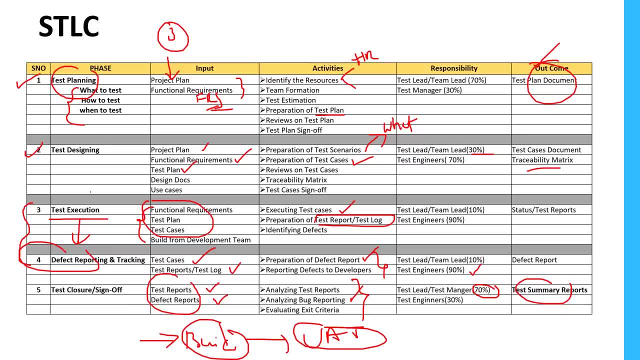 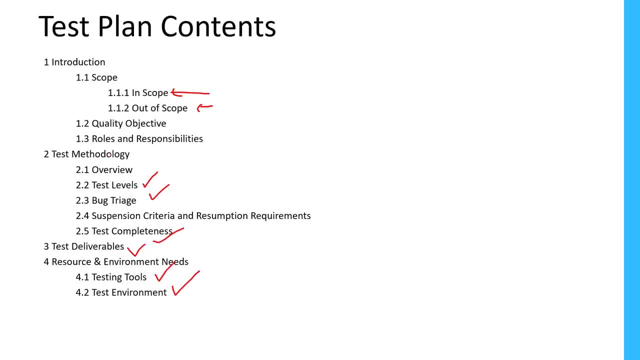 Okay, so there's a main activity in the test planning phase, And now we are entering to the test design. Here We need to understand what is use case, What is test case, What is test scenario. Let us understand this use case, test scenario and test case. 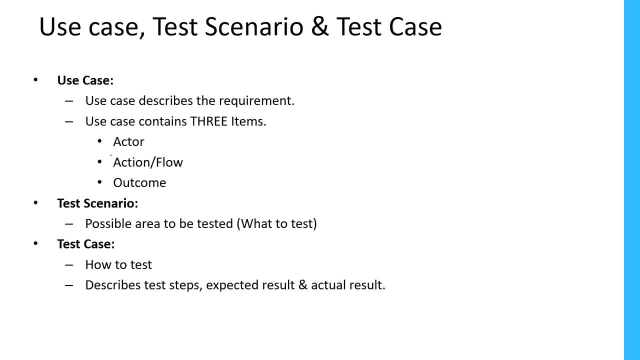 So in interview also, people will ask you: what is use case, What is test scenario, What is test case And what is the difference between use case and test case? Okay, let us see very clearly: use case is a small requirement. use case will be part of functional requirement. 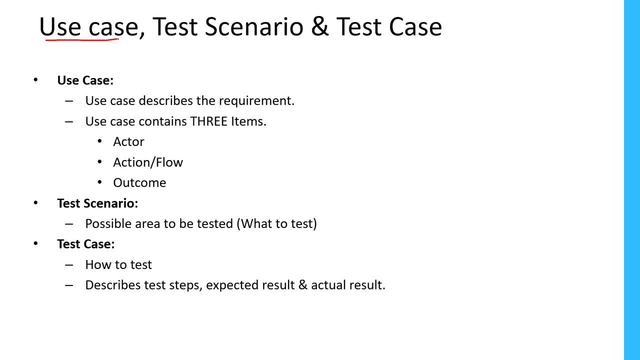 So suppose in the functional requirement you will see small documentation and some paragraphs. So by reading the text you can't understand 100% context. So sometimes you need some pictures and diagrams and write some drawings you need. So by seeing them you can clearly understand the flows. 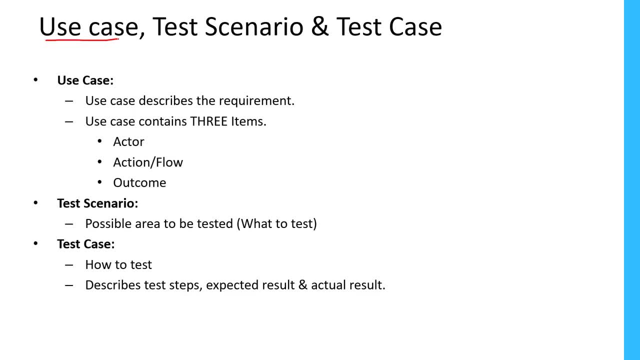 So those things will be part of use case. So use case describes the requirement. use case will give you more about more information about your requirement. That's the reason use case is a part of your requirement. Okay, so it contains some actor flow and outcome is very simply say: 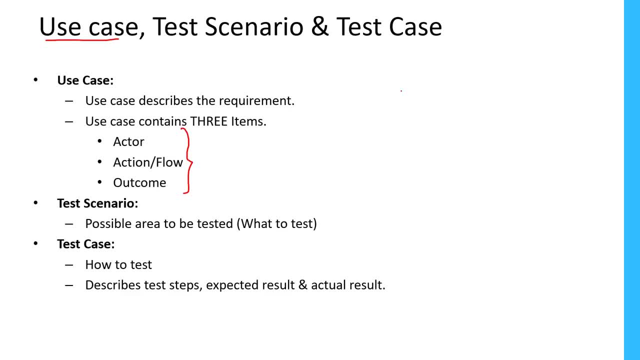 so, for example, for the login screen, how the use case will be. So let's say the person Okay. so let's say some login and he will get some home page. So this is kind of a use case. So this is your login process and this is a home page and he is a user. 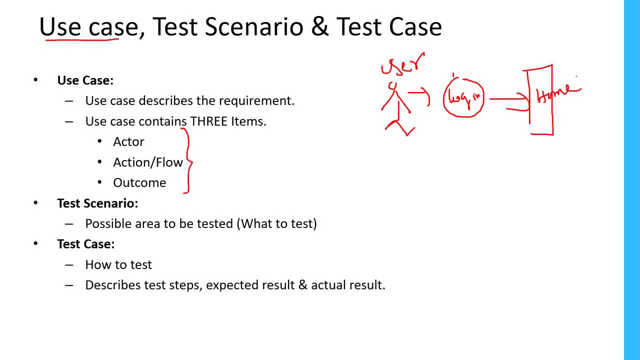 So if I see this diagram, you will be very clear about the okay. This is a login process. user is able to log in and then he will. if it is a valid, he will go to home page, If it is a invalid, he will go to the error page. 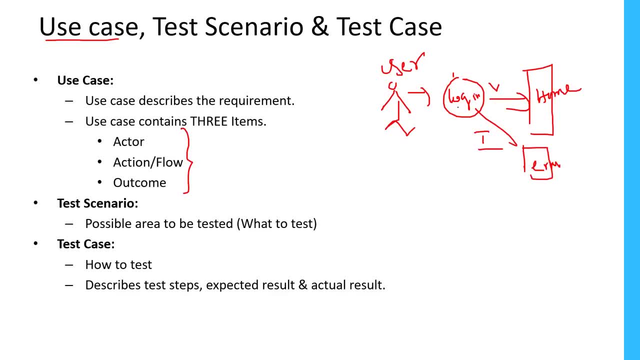 So this is clearly saying the picture, your requirement, but the same thing if you write in the text format, it is little difficult to understand if it is a complex functional piece, right. So the use case will give you the clear picture. So use case contains three parts. one is actor. actor means a user. 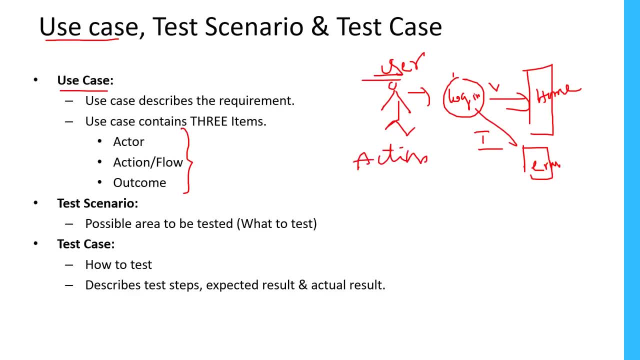 He's an actor. whoever perform the action is called as an actor, and here action is the login. What is an action here? Login is an action, So we will do this action. actor will perform the action. What is an outcome here? getting. the home page is out. 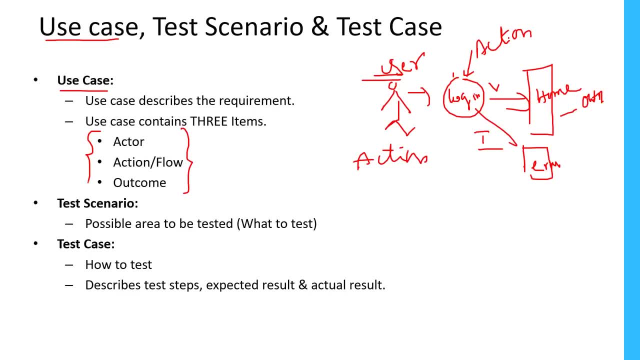 So use case contains the parts after action or flow and outcomes. Okay, so use case is a part of requirement. It describes more about requirement. What is test scenario now? So test scenario and test case- these two will be prepared by the test engineer. 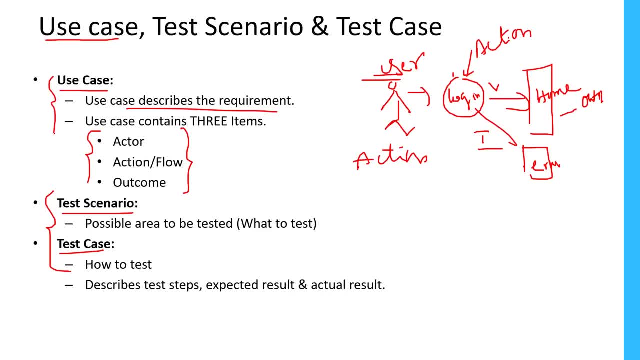 but use case will be prepared by the business analyst, which is again part of requirement. So over is designed the requirements, So those people are responsible for creating the use cases, whereas test scenario and test cases have been prepared by the test engineers. So test scenario is a possible area to be tested. 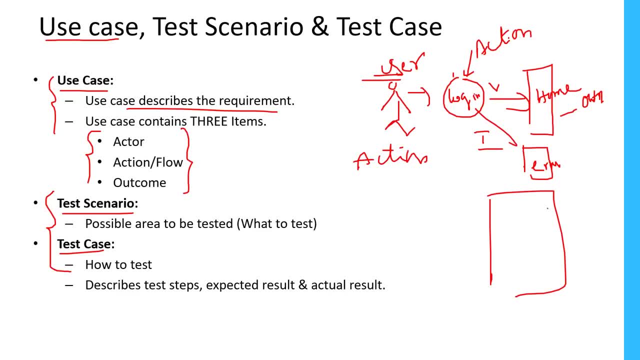 So what to test? So in our application there are n number of functionalities we have. So what are the different areas we need to test? So what to test? that is tested scenario. So test scenario is, basically, is a possible area to be test. 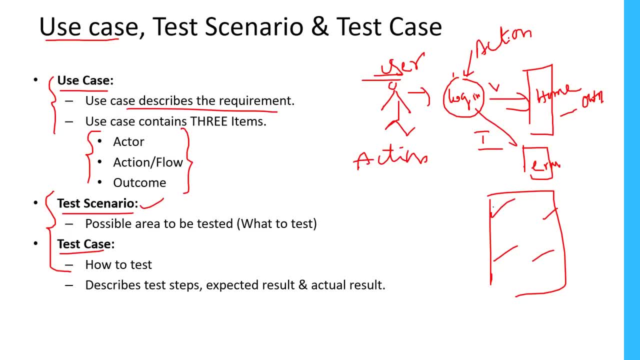 What are the different areas we need to test. So that is comes under the testing app. So it more than more describes on what to test and test case is describing how to test. So, okay, we have identified a few areas to be tested. 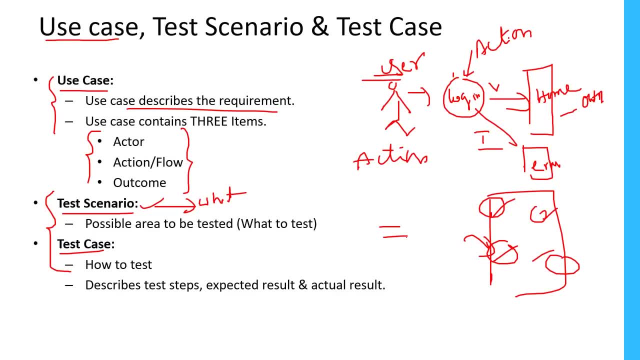 But if you want to test this particular functionality or area, what are the steps we need to follow? Okay, so that comes under the test case. So test scenario describes the what to test and test case will describe the how to test. Okay, it describes the detailed steps. expected result: 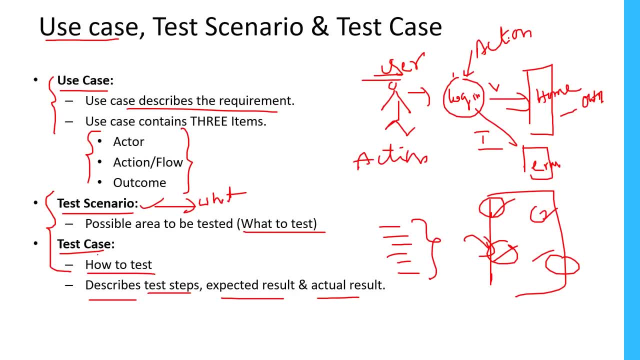 and actual result and ability. So this test case is very in detail. So test scenario can again divided into multiple test cases. So based upon the use case will prepare the test scenarios. So for those test scenarios we will prepare the test. So at the time of getting the bill from the developer. 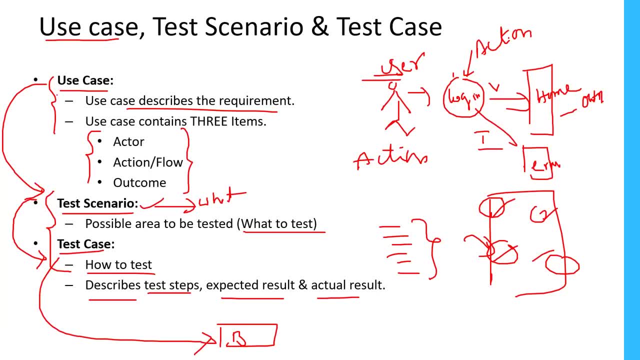 we will execute this. test cases: Okay, this is a link between use case, test scenario and test case, So use case will be part of requirement test scenario and test case will be prepared by the test engineer by referring use cases. Okay, so this is about use case, test scenario and test case. 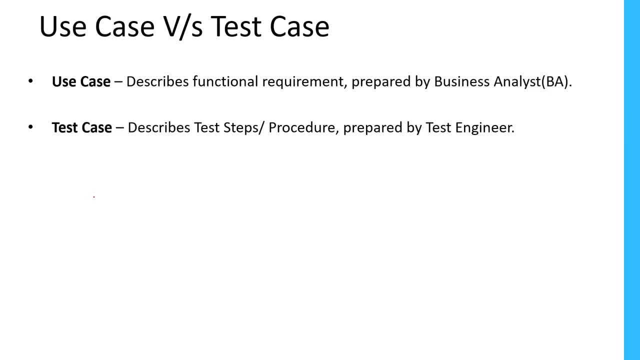 We will see all these things practically in the coming session. So now use case versus test scenario, Test cases. So people will ask you an interview like: what is the difference between use case and test case? use case describes the functional requirement prepared by the business analyst, as we said earlier, 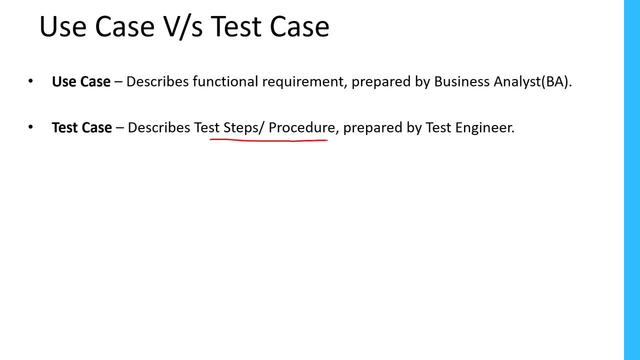 So test case describe the test steps procedure and which is prepared by the testing. Okay, there is a lot of difference between these two. use case will be part of functional requirement and prepared by the business analyst and, based on the use case, We will prepare the test case. 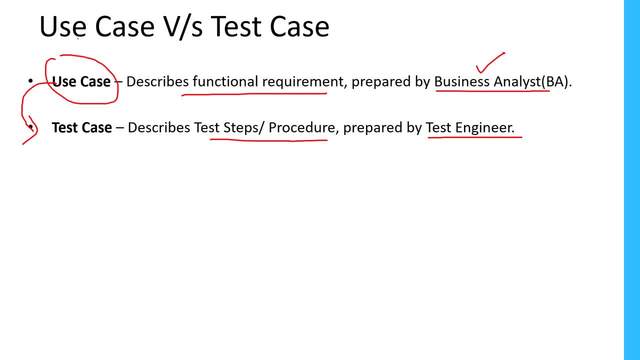 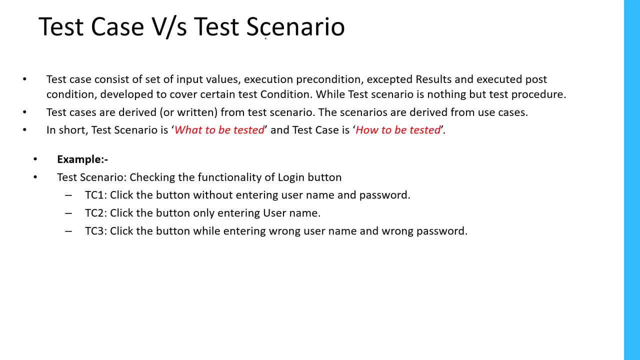 So, before creating A test case, we need to understand this use case- very key- and test case describe the steps procedure which is prepared by the testing. that is use case versus test case. Now, so test case versus test scenario. So simply, test case, test scenario is focus on what to test. 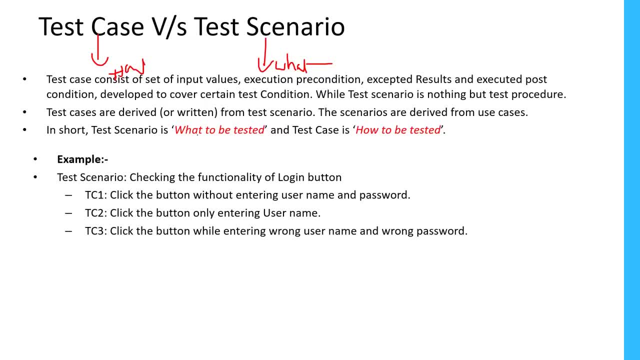 and test case is focus on how to test. So what to be tested and how to be tested. So test scenario is what to be tested and test case is how to be tested In detail scenario. So here I have given some example. So test scenario is checking the functionality of login button. 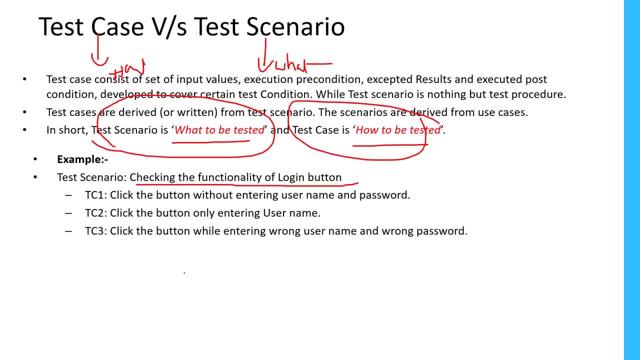 Okay, checking the functionality of login. So this is a scenario area to be tested. So how many test cases we can write for this scenario? So test case one is: click the button without entering username and password. So this is one test case, and click the button only entering the username. 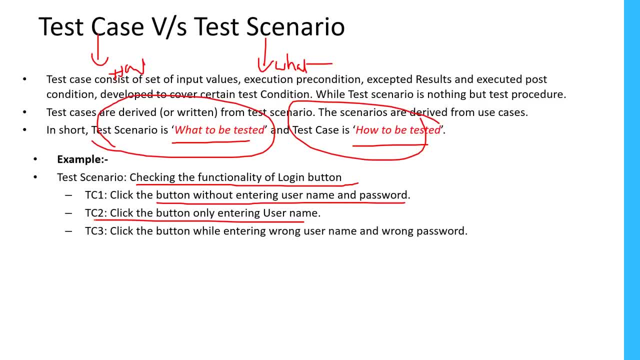 Then we'll see what is the output. This is test case 2 and what is the test case 3? click the button. I'll entering the wrong username and the wrong password. This is again one more. this So for one test scenario. we can create any number of test cases. 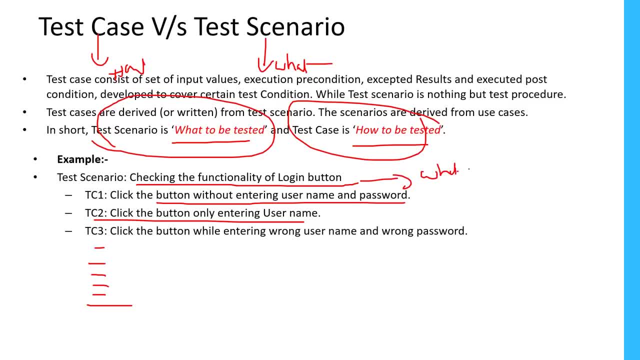 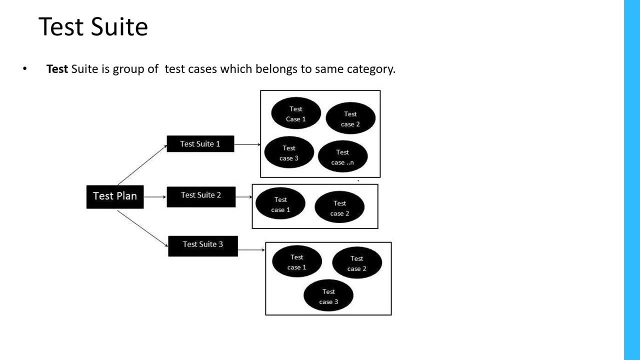 So test scenario is describe what to test and test cases are describes how to test. That's the difference between test case and test scenario. Fine, So now test suit. What is that test suit? So test suit, That is a group of test cases. 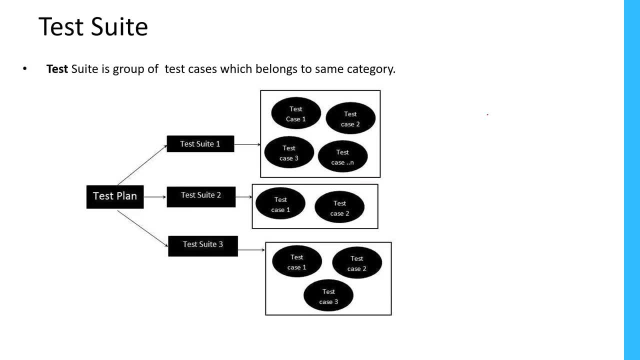 So, for example, in the previous session I talked about various kinds of testing like retesting right and regression testing and then functional testing, a smoke testing, sanity testing, right, So all these kinds of testings. there will be separate test cases, So some test cases are fall under really a retesting. 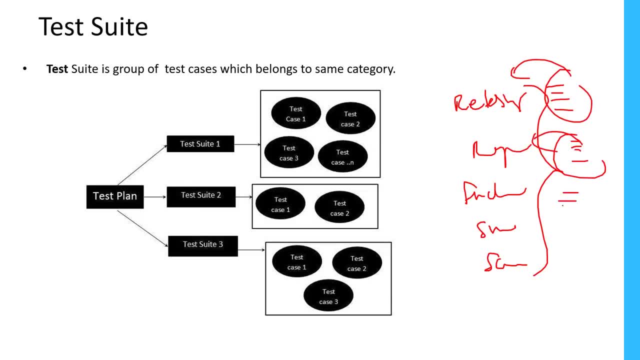 and some test cases are fall under regression testing. some test cases fall under functional test cases. on some test cases comes under the sanity test So we need to group this test cases into multiple categories So that itself is called as a test suit. So sanity test suit, regression test suit, functional test suit, smoke test suit, sanity test suit. 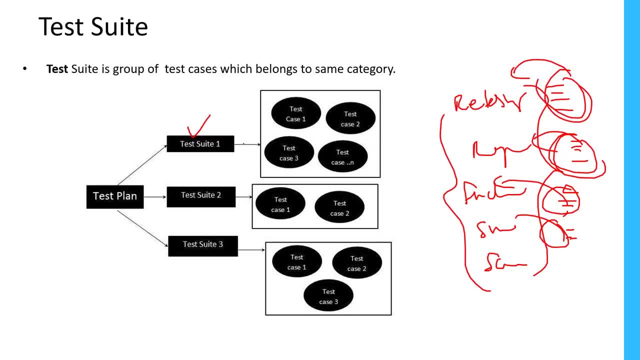 We can call all the test cases grouping like this using test suit. Okay, So these test suit contains number of test cases, again, contains number of test case. Suppose somebody asked you execute regression test suit. What does it mean? is we need to execute? 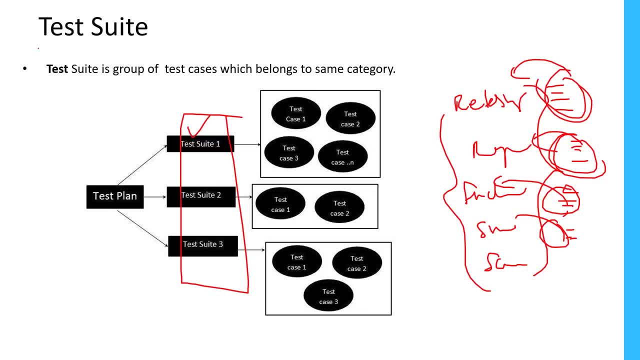 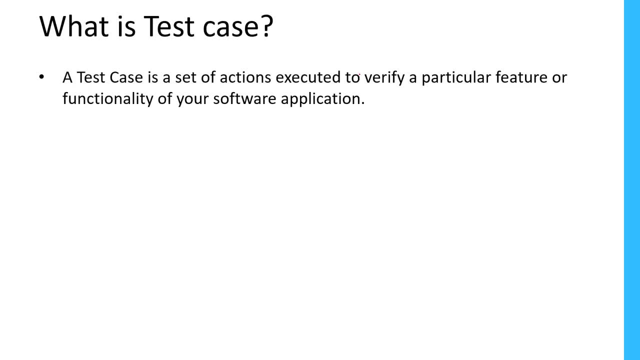 All your regression test cases. that is a test suit. So test suit is a group of test cases which belongs to the same category. Now, what is test case? as we discussed, a test case is a set of actions executed to verify particular feature or functionality of your software application. 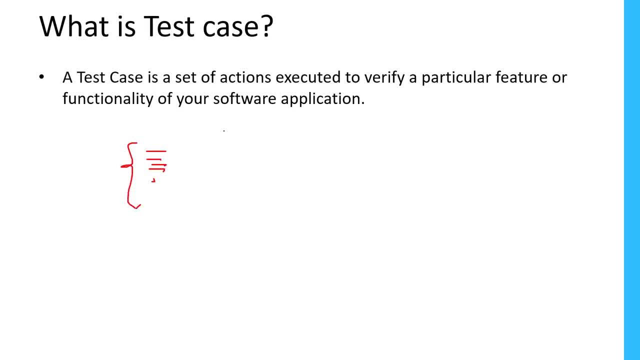 So, step-by-step, we need to write what are the actions we need to perform, What is an ever expected output, What is an actual output in the application. So, whether actual and expected, both are same, then my test is passed. Now both are not same, my test is failed. 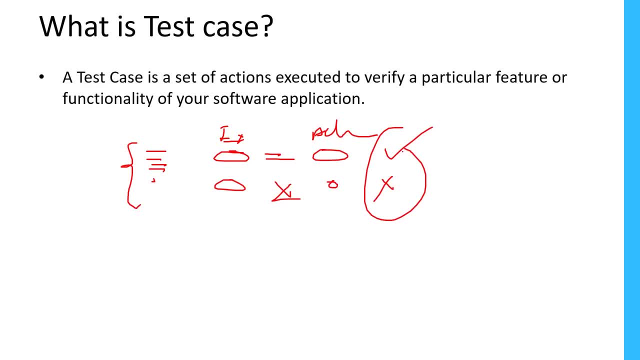 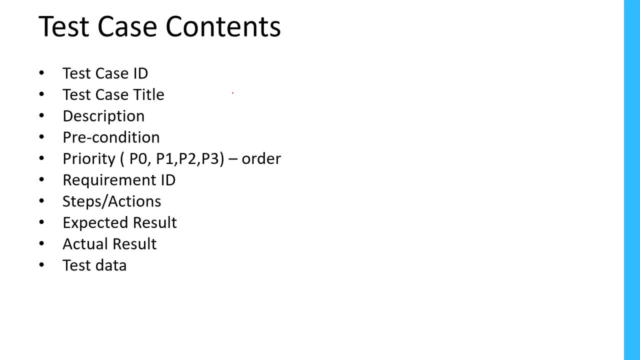 So who will decide? test case test: who will decide? the function is passed or failed? our test case will decide. Okay, so test case is very important for testing now. So how? what are the different contents we need to add in the test case? Suppose somebody asked you to write a test cases. 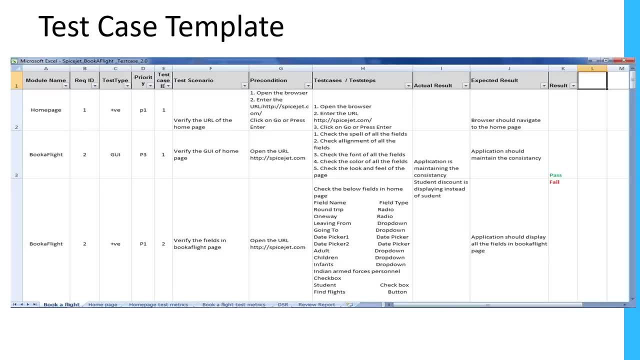 What are the fields. So test case is a kind of document. It will be. It seems like this test case template, So normally we'll write all the test cases in Excel file, So, which contains a number of columns like: what is module name? 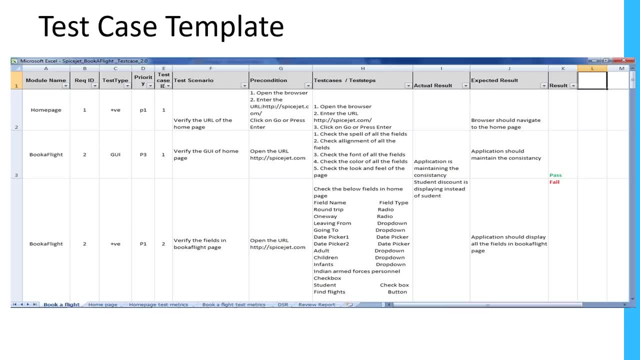 What is the requirement ID, What are the testing type, priority test case ID, test scenario. What are the P conditions we required and what the test steps we need to execute- actual result, expected result and everything. So this is called test case template, So the same kind of template we follow while writing your test cases. 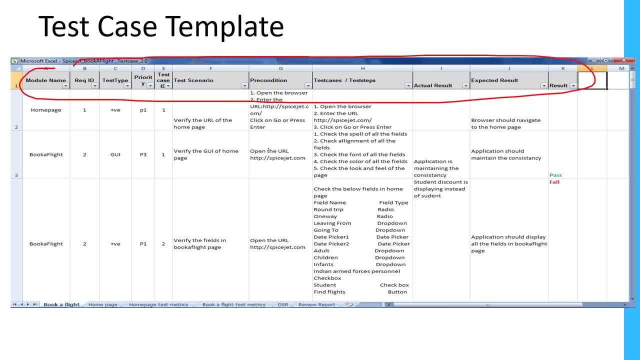 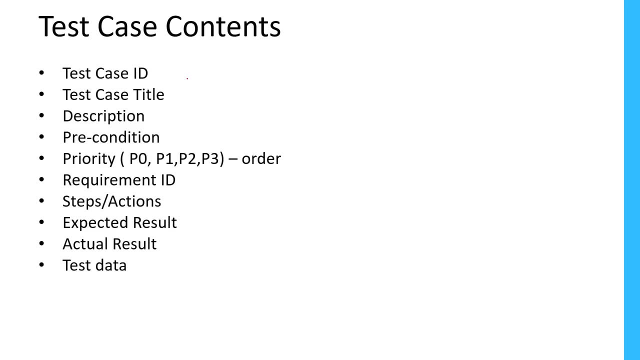 but these are all the different We need to provide at the time of writing your test cases. So let us discuss what are the fields? test case ID. So every test case should have a unique ID. Okay, every test case should have a unique ID. 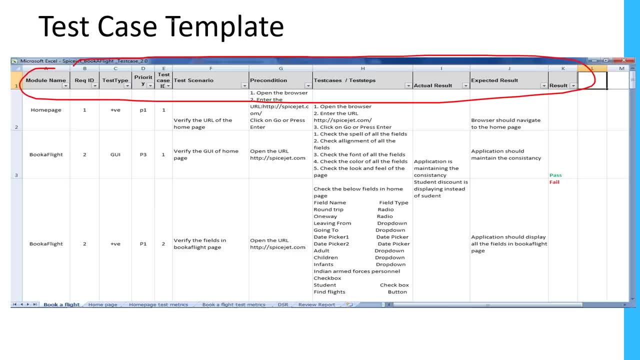 So by referring the test case ID will refer the test case. If you observe this template, Here you can see the test case ID. So here only one is given. this is completely wrong. So every test case is having a unique ID and the ID is also should not give like one. 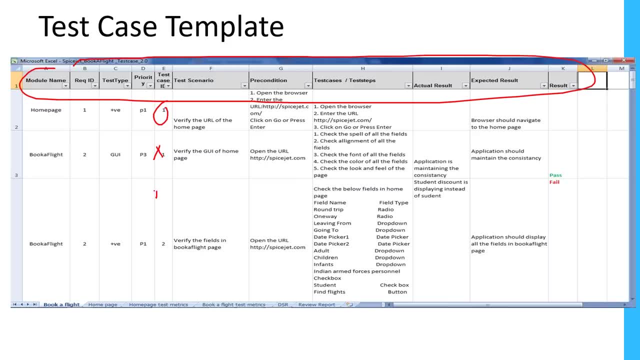 Two, three, four, not like that. We need to give certain format. Let's say, some project name underscores a module name, underscore TC, underscore some zero, zero one. So like this, the test case ID format will be. so every test case is having a unique ID. 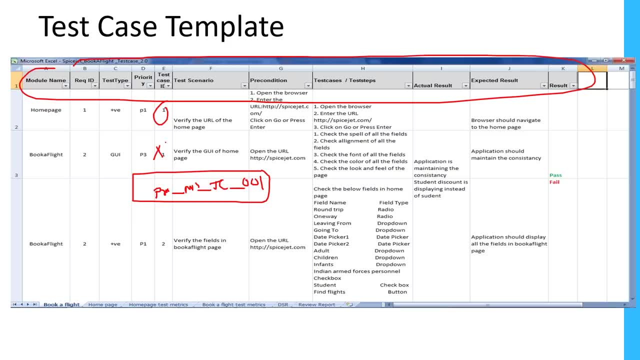 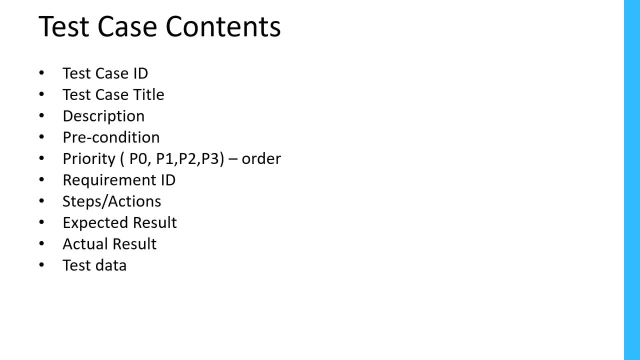 So based upon that ID we can identify the test case very easy. hundred test cases You have. for each and every test case You have a specific ID and unique ID. That is the first one, and title also should be. So by reading the title everybody should able to understand. 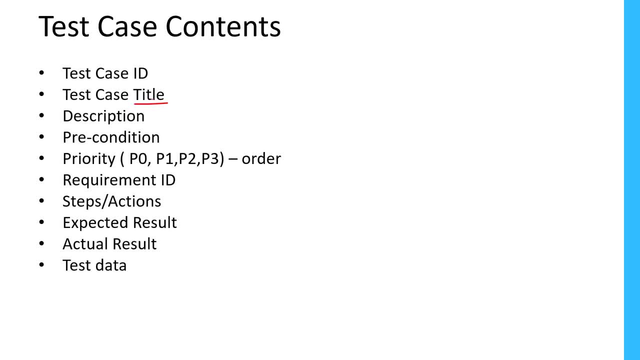 and what is the functionality that is case is going to test his case. title is also required and description. So by reading the title sometimes because title is very small, only one line statement now to give, sometimes by reading the title if you cannot understand the functionality. 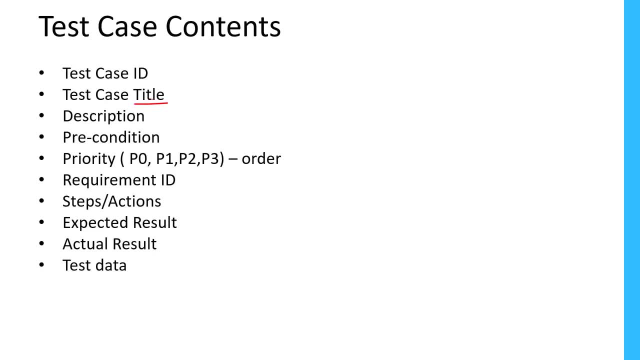 we can just write the video description about the test case and then precondition: If you want to exclude our test cases, what is the precondition? So, for example, if you want to test the login, what is the precondition? or URL should open in the browser. 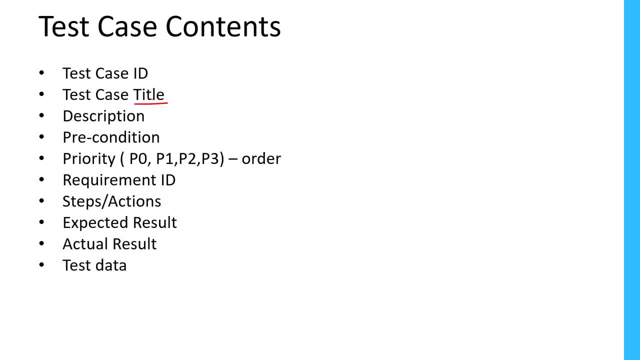 and the home page to display, and then only we can test the login right. So that's the precondition and pray at. so priority means a order of execution. So for example, I have written 1 to 10 test cases and 1 to 10 test cases. 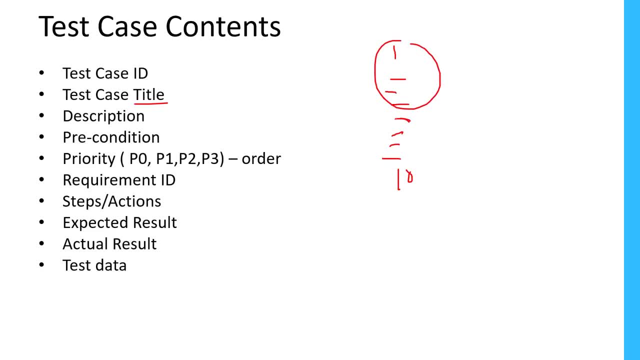 What are the test cases I need to exclude first and what the test cases I need to exclude the next? So in which order I need to execute What will be decided by the priority? So, for every test case, we need to give a priority for every test case. 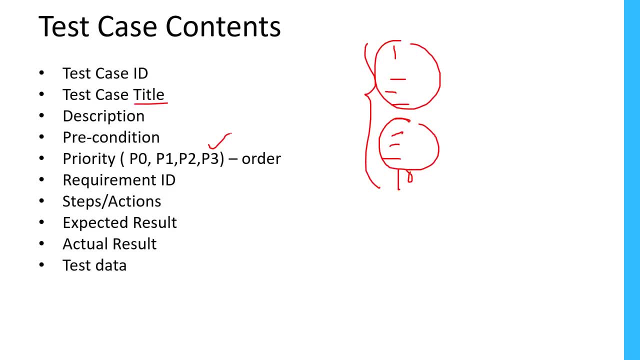 We need to give a priority. A priority will decide when we need to execute the test case, in which order we need to execute the test cases. For example, if I say sanity test cases or sanity or smoke test cases, we have so sanity or smoke test cases. always. priority will be p0. p0 means these test cases must be executed at: 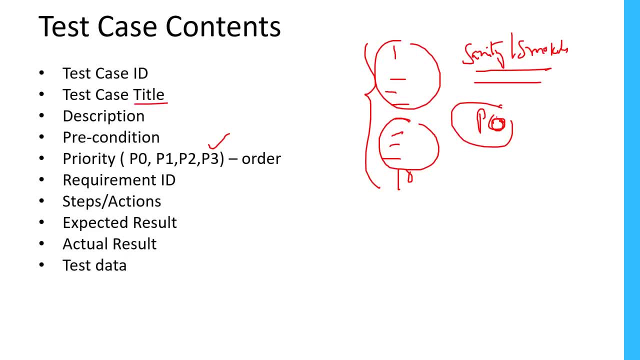 At the beginning: Okay, high priority, because if sanity or smoke test is failed, we can simply reset our bill. The basic functionalities itself is not working like. application itself is not able to install and even if we install, you are not getting the home page. 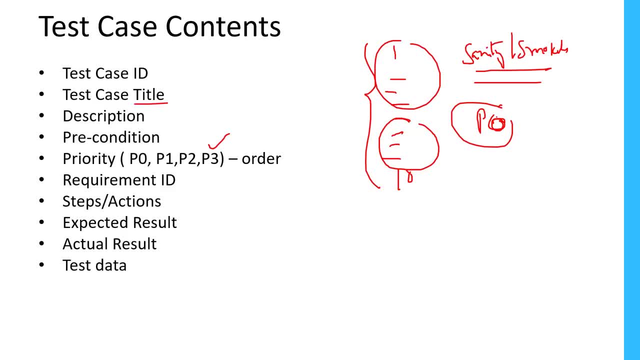 So in those cases you cannot test and go for the right. So in those cases we can just report as a bloggers So we will get the new build from the developers. So those test cases will fall under sanity or smoke category. So those test cases 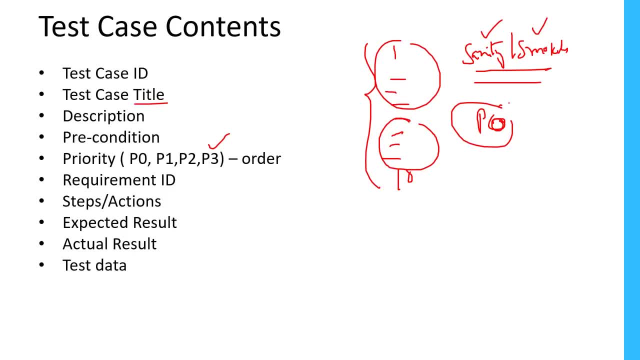 We always give p0 as a priority And rest of the test cases according to your requirement and your timelines. You can just give p1, p2, p3, that all UI related stuff. We will give p2 or p3, UI related test cases. 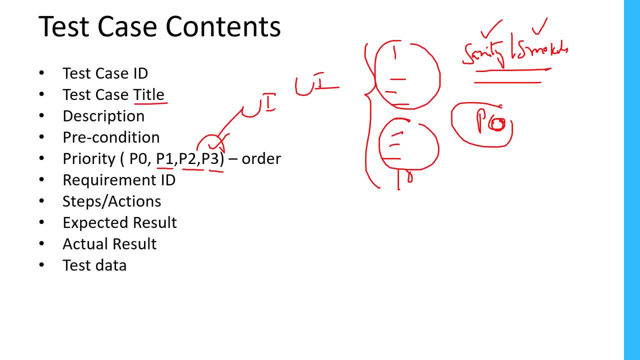 like button is not aligned, spelling mistake colors of font. So these type of testings, test cases, We will give p2 or p3. Okay, we can exclude them later, But p0 and p1 are very high priority. So first we need to exclude. 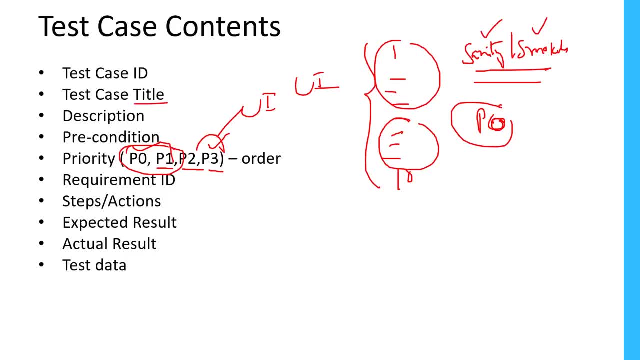 These two test cases. these categories and the rest of them we can exclude later. So what is priority? priority mainly describes the order of executions, in which order our need to execute our test cases. that will be decided by the priority. So at the time of writing your test cases, 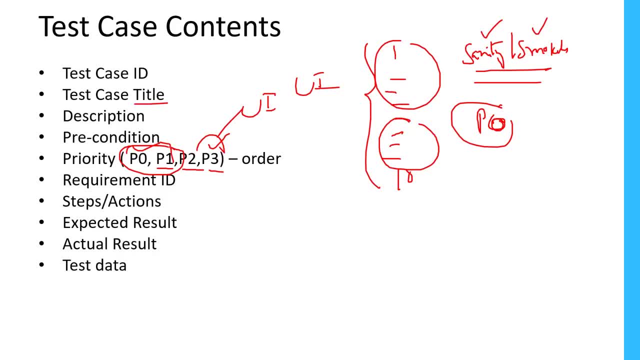 you should also give the priority to that particular test case because at the time of execution you will refer this priority. So you will choose only p0 priorities first executed. if it is passed, you will choose a p1 priority test cases, then execute. if it is passed, then go to p2 and p3, so on. 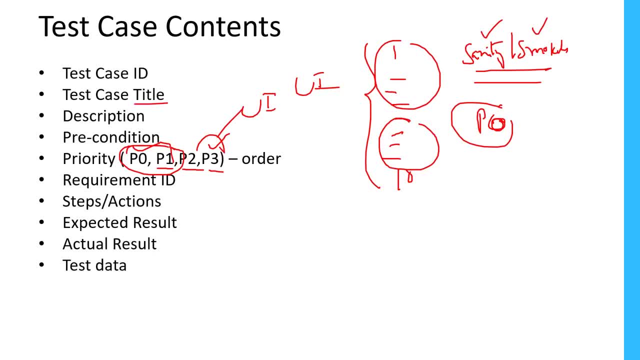 So that's about priority next to every test case. So we need to also specify the requirement ID. So in the requirement document you will have a requirement IDs, So it will clearly give you an idea like which requirement you have written this test case. 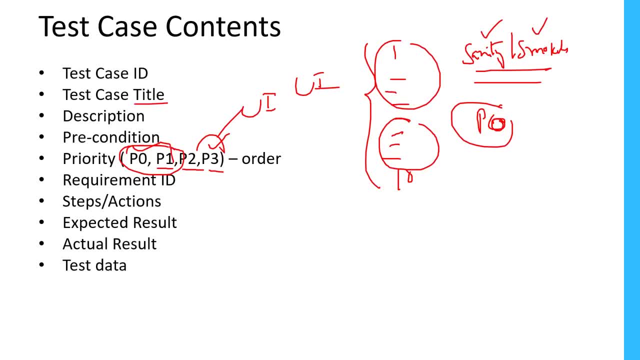 So that's the reason we need to also mention requirement ID and steps or actions. So, step-by-step action: What is an action we need to perform To test? that is also part of test case: expected result and actual result. finally, test data. some test cases: 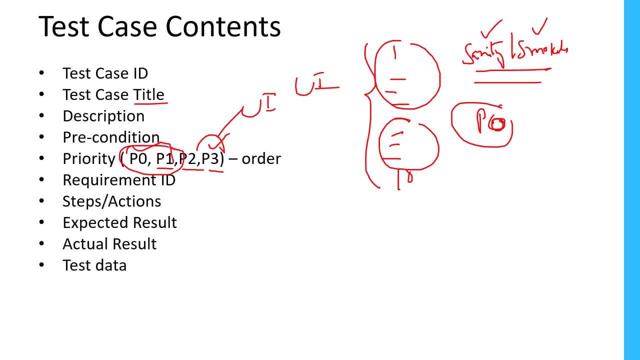 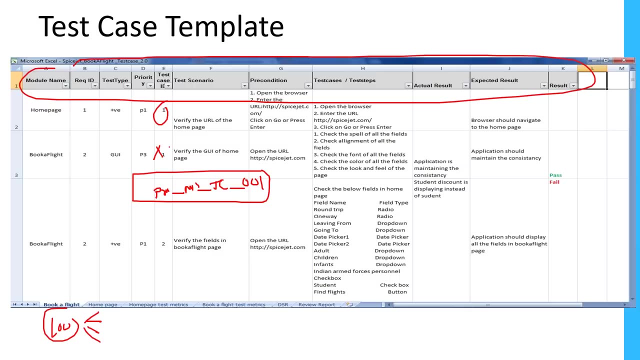 We require some test data So that test data is also part of your test case. So these are all different fields We need to add, we need to use at the time of writing your test cases. This is a test case document, So we are going to write test cases like this in the project. 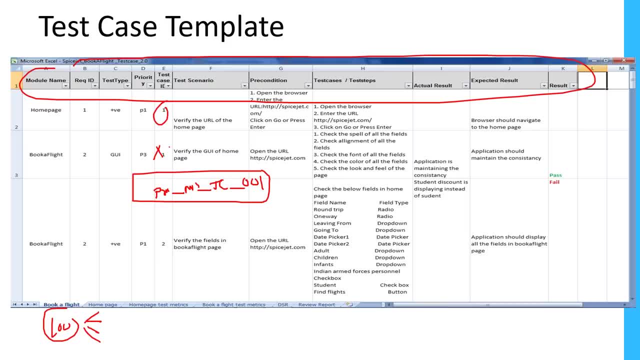 Okay, So this is just for understanding purpose how the test case template will be, how we need to write the test Cases and what are the different documents We need to refer to write the test cases. but till now we don't know the application. 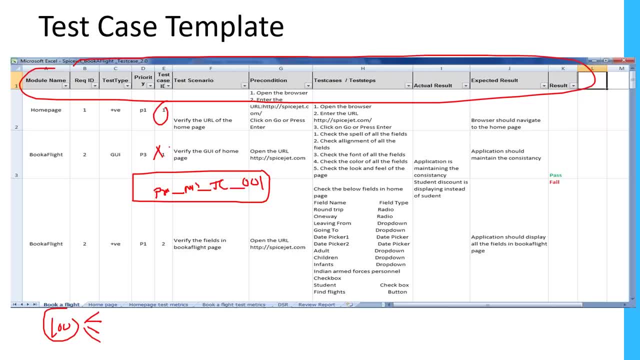 Okay, at the design planning phase of designing phase, We don't know how application will be only based on the documents. We will assume the functionality will understand the functionality, then we prepare the test cases, But while seeing the application, somehow, if you find any differentiation. 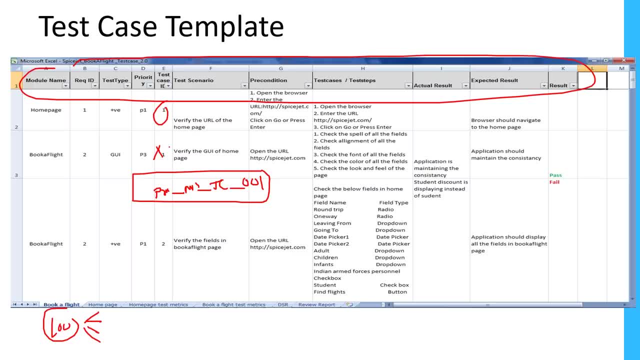 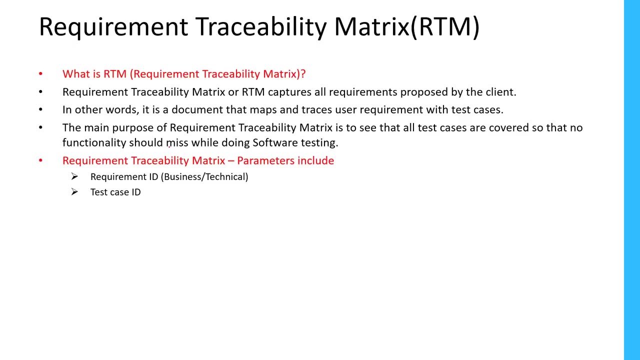 you can just modify the test case. that is fine, but we should not modify majority of the test case. If we, if you need any small model applications, you can just do that. Okay, So this is your test case template. Now let's move on to the another requirement: traceability matrix. 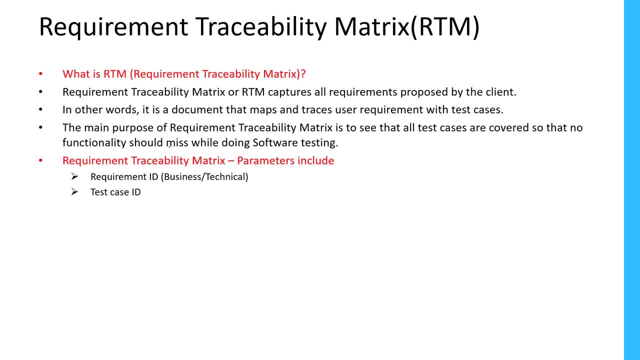 the test designing phase. along with the test cases, We need to also prepare the RTM. RTM is a requirement, traceability matrix, and this is very important. again, in interview people will ask you: Suppose you have a requirement, you have written hundred test cases for your requirement. 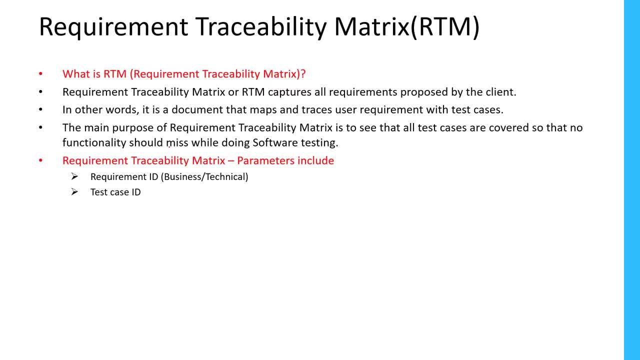 So how do you make sure your test case is covered? all the requirements which are mentioned in the requirement document. So we need to prepare a specific document called as a RTM requirement traceability matrix. So this document will contains a requirement ID corresponding test case ID. 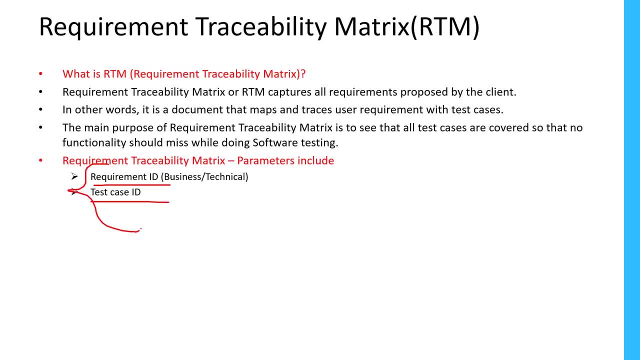 So this will give you the clear picture. So what are the requirements we have and what are the different test cases you created for those requirements? It is a mapping between requirements And test case, so this will give you the clear picture whether you covered all the requirement. 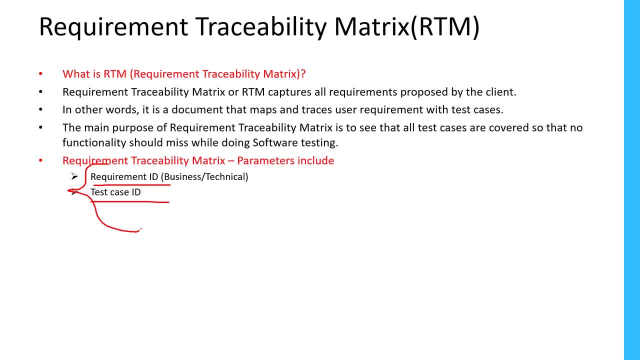 whether you write in the test cases for all the requirements or something you missed out. So that kind of information will give you, because the traceability matrix, which is also very important document. It will be like this: Okay, This is your test case document. 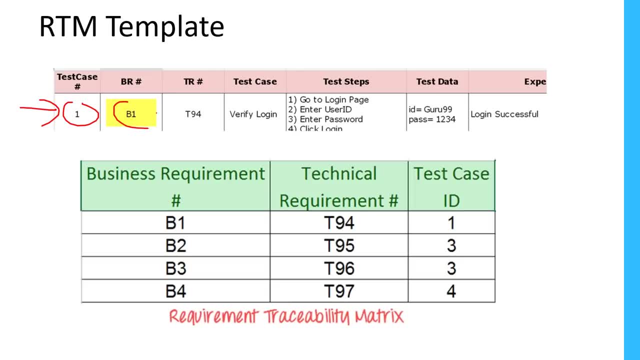 Actually, this is your test case. as a test case one, your business requirement ID- technical requirement ID Is a test case. These are the steps, This is the test data and this is your expected result. So this is your test case and for this test case, 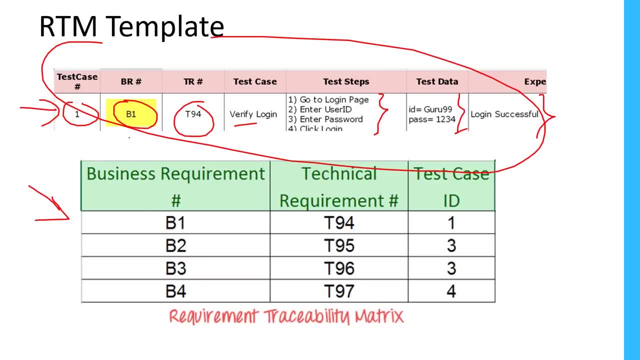 you have to prepare the RTM like this: here the business requirement and technical requirement, and then test case ID will be part of for this business requirement, for this technical requirement, What is the test case you created? So let's say this is one, This is test case ID. 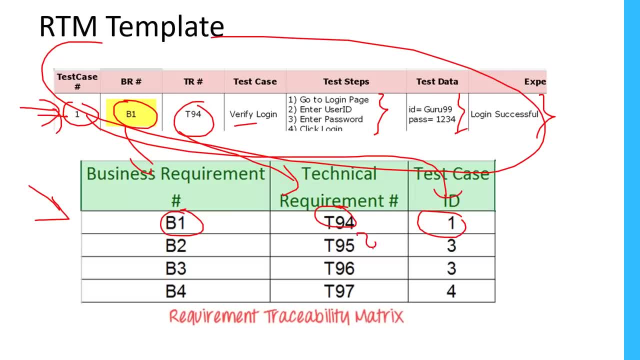 Okay, So one is a test case we created. So for these two requirements we have created Three test cases of three test cases, and this for this requirement we have created business case. So basically, the requirement traceability matrix is a mapping between the requirement IDs and test case. 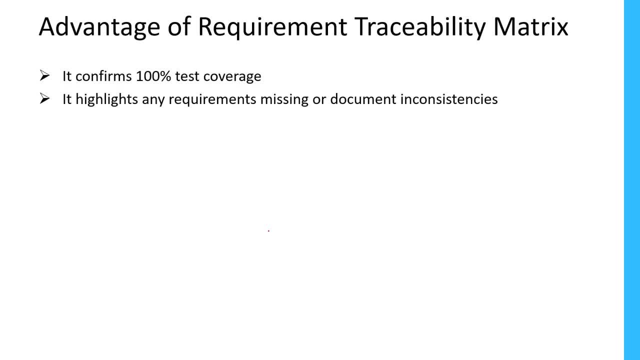 So this will give you the clear picture. So what is the use of it? It confirms hundred percent test coverage, means we haven't missed anything, and it highlights any requirement is missing or document inconsistencies. Okay, So if there is any mismatch you found over requirement document. 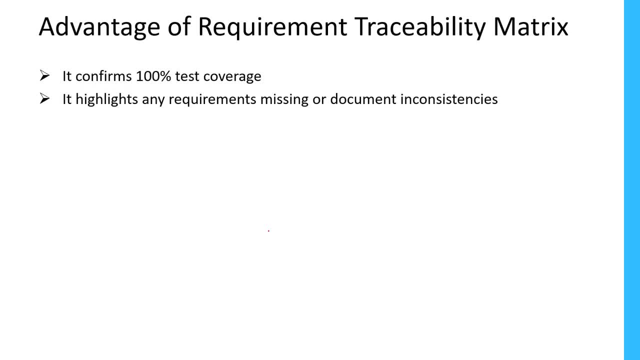 and test cases document. you will easily find out. So that is the main advantage of requirement traceability matrix, called as RTM. So this is also part of designing phase. So test engineer has to create requirement traceability matrix along with the test test case document. 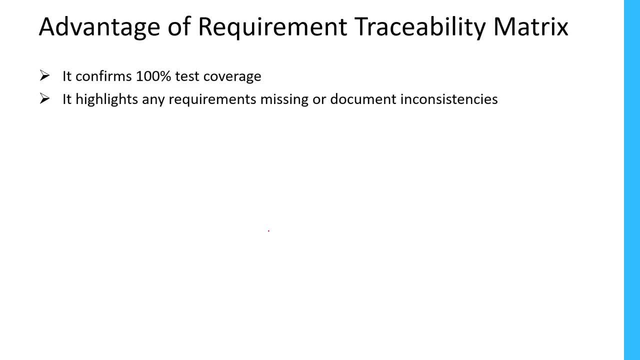 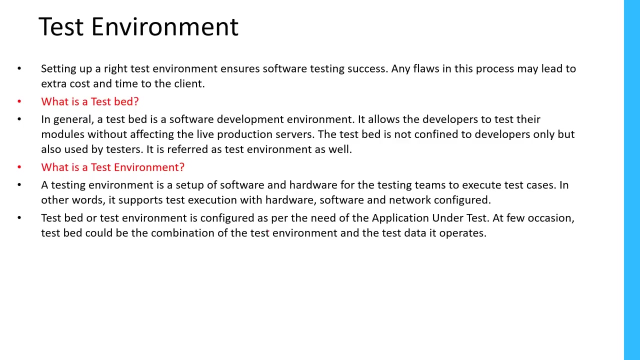 Okay, So these are all documents. So that's the reason test engineer should have the documentation skills. You should know very well How we do use word document, Excel, document presentation and these skills very much required. Okay, document skills are very important. Now, once we have done the design phase, it, once we have test cases, traceability matrix is ready. 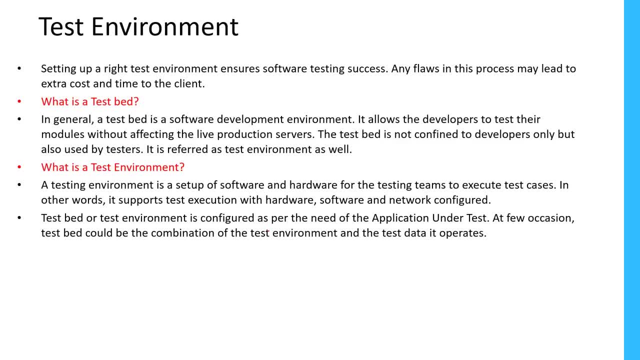 Everything is ready, We'll enter into the test environment. So we need to set up an environment because by the time developer giving the bill, we need an environment where we need to install the bit. So here there are two types of applications. Suppose if it is a desktop application. 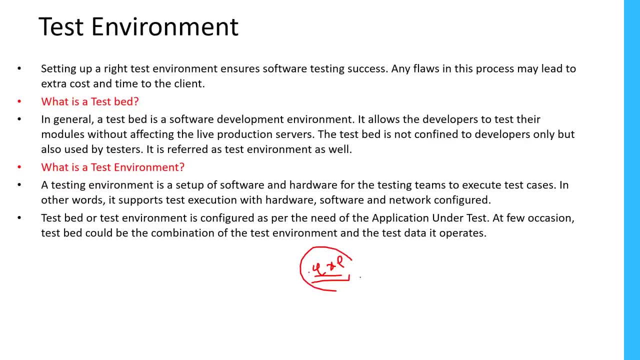 so the developer will just give you one exe file like executable file. So let's say: this is your testing environment and multiple people are working on the testing environment, So each individual is having it their own systems like this. This is testing environment. So if it is a desktop application, 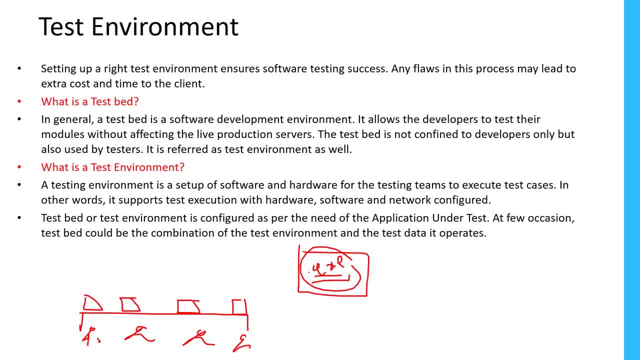 so every individual can download this from the repository server where the developer keep this build, and they can just download here, each individual installing their system. second, They can test it. This is one way of setting up test environment and the other way is if it is a web-based application. 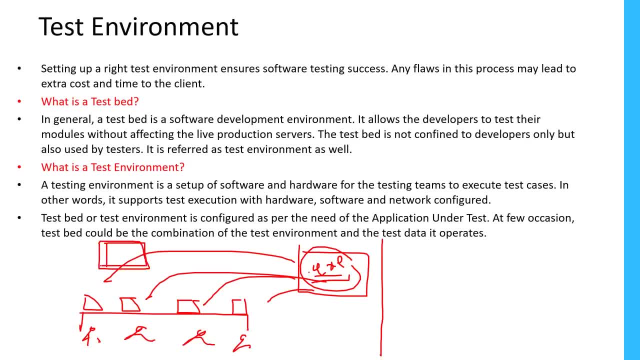 there will be common server in the testing. This is called as a testing server. This is a common mission and here actual application will be installed, because this is a web-based application. If it is a web-based application, there will be a lot of things will be there. 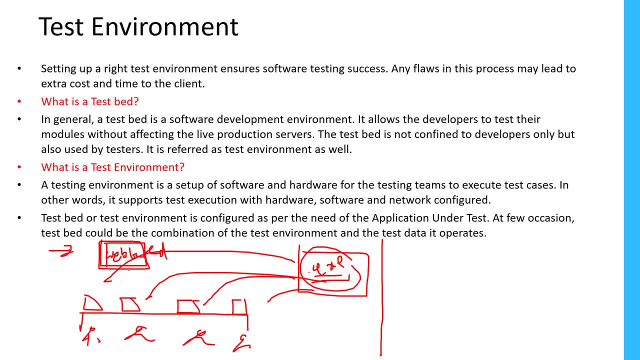 It is not easy to install. Okay, A lot of things. we need to follow the time of installing web-based application. So, once installation is done, everybody will access this application by using URL, because web-based application means we can access through URL only music browser. 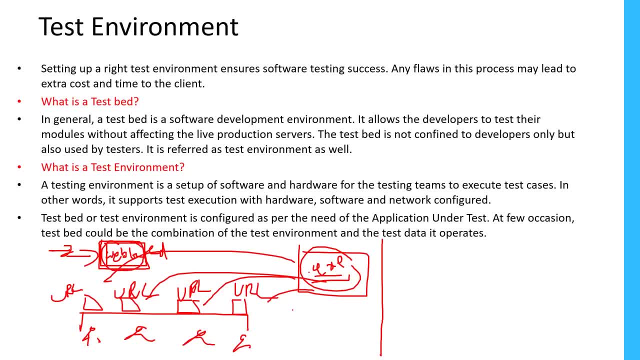 So everybody will access the same application by using URLs. So this is called as a test environment. So before getting the bill from the development team, we need to set up the testing server: individual machines And if there is any hardware, we need to request that hardware. 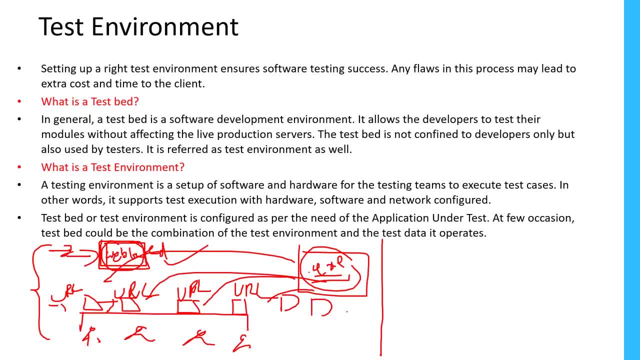 And if you need many more machines, we need also refer. We need to also get those machines and get the riser ID tickets and get those missions and everything. get ready with the everything. Once we get the bill from the developer, we can install that and we can start testing it. 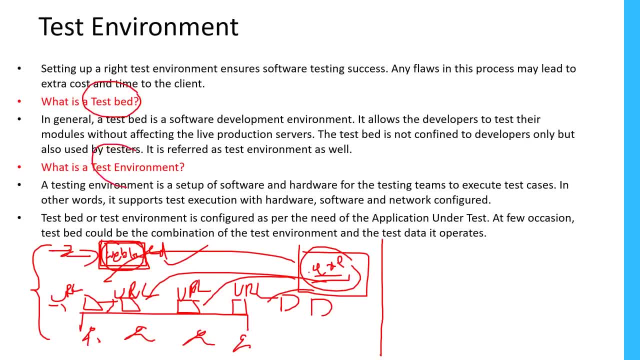 So that's about testing, and test bed is another form of testing. Test environment is also called as technically test bed. So test bed is a an environment where environment required for software testing is called as a test bed Environment: software and hardware- both software. 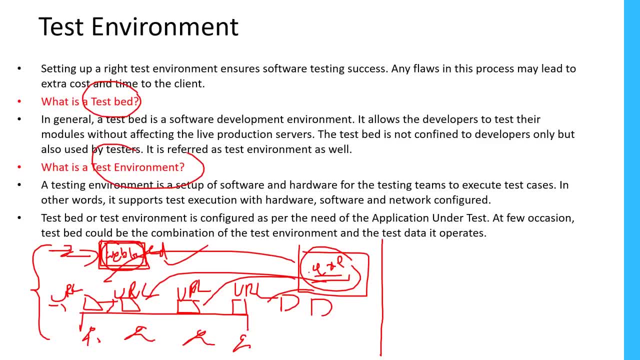 and hardware environment required for software testing is called as a test bed. Okay, So this is our environment part- Test environment. So far we have designed test plan, test cases, traceability matrix and we are entering into the execution phase. So test environment is set up is done. 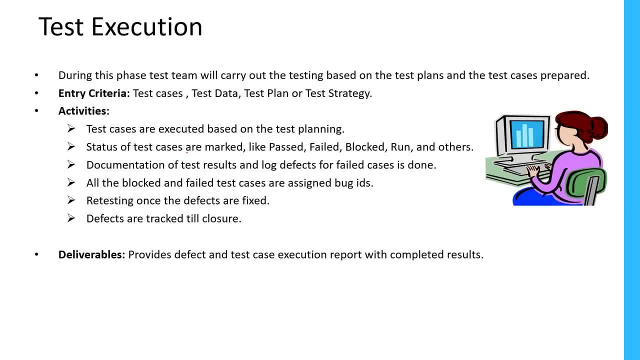 We'll receive the bill from the developer and we install it. then we start execution. So at the time of execution, what we should have in the by hand: we should have a test cases, test data should be ready, Test plan should have and test strategy. 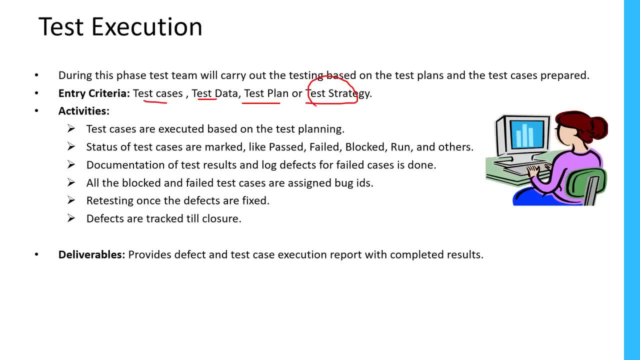 So basically, test strategy is talk about what kind of testings we have to perform and what are the tools we have to use, so that kind of information we should have. So this is entry criteria. So during this test, testing team will carry out the testing based. 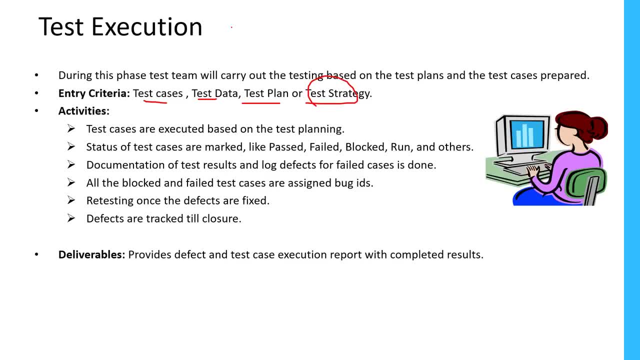 on the test plans and test cases prepared. So once we what are the main activities we do as part of execution is test cases are executed based upon the test planning and we need to prepare the status of test cases, Like we need to mark as a past or failed, or blocked. 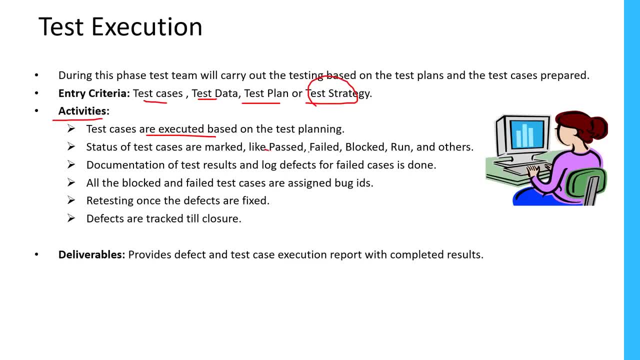 or still in progress running. So you need to mark the test cases, whichever we already written in Excel files and then we need to document the defense. So whenever you found some defects you will report to the developer right. So those defects will be part of the. again on Excel file. 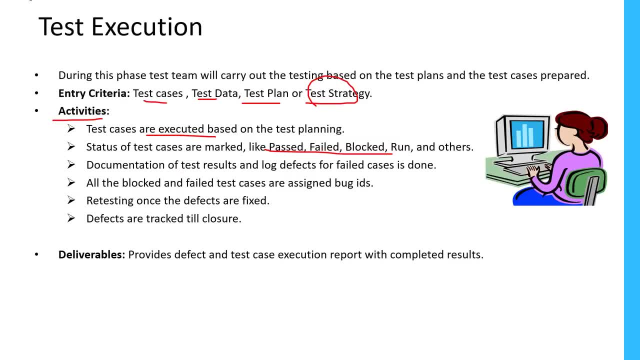 and also you can raise those defect by using tools. and every failure or every defect you have identified, You need to give a proper IDs to them. Even defect is also having set an ID. So every test case is having a unique ID. Similarly, every defect is also having a unique ID. 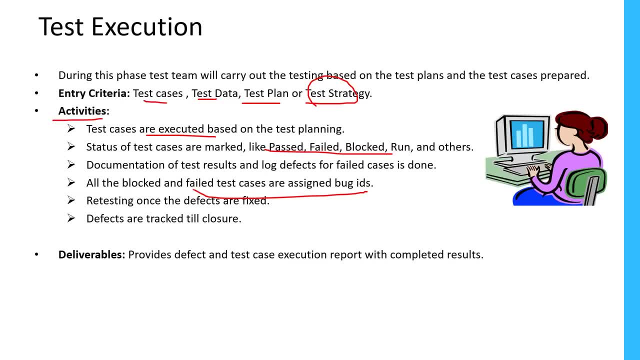 So every defect is identical, identified by using a unique ID number. Okay, retesting once the defect or fix, sometimes You will get number of bills from the developer, So an every bill. So what is supposed to? let's say, build one. we are testing it. 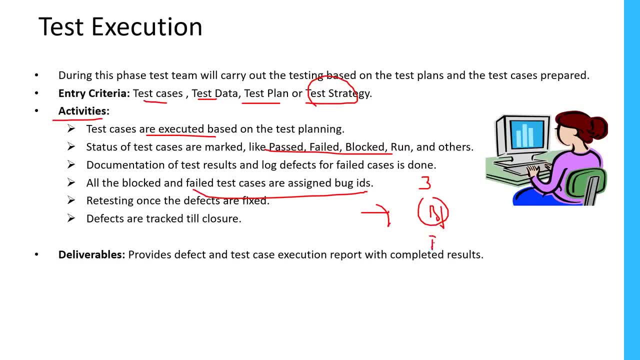 We found our three issues. We reported them to the developer. again We will get the bill number two. So in the bill number two again we need to retest these three defects, whether they have fixed or not. So retesting the bugs once we get the new build. 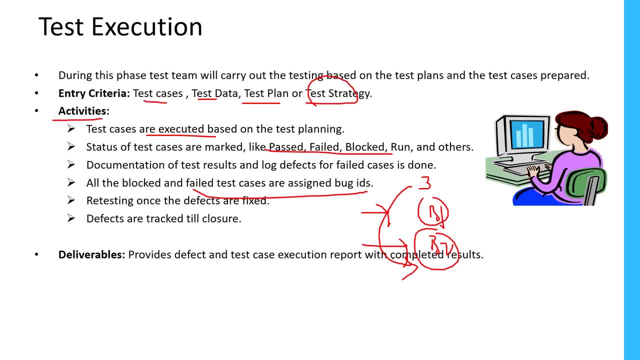 and we need to track this- defects till we close those defects. So when we need to close the defects, So once the developer is fixed and if everything is working fine, then we need to close the defect. Okay, So these are the different activities we do as part of test execution. 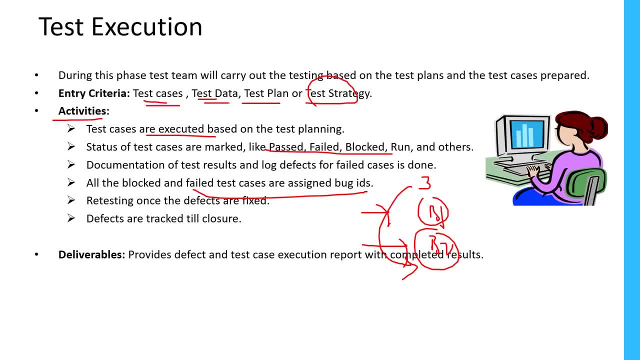 So, test cases: we will execute test data. We have to use test planning. as per the test plan, We need to execute our test cases and, parallelly, will identify the defects as, and then and report the defects to the developer. So what is the deliverables here is defects. 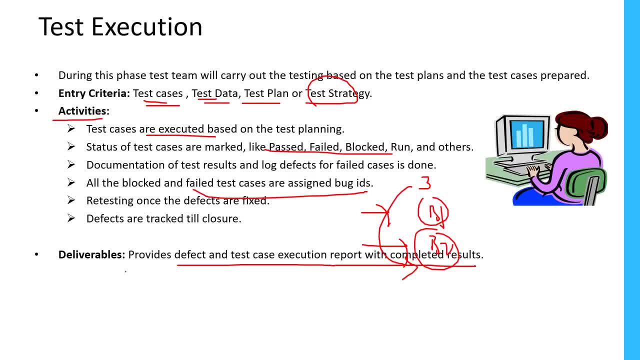 and test case execution report with the completed result will be sent to the management. Okay, that is all about test execution phase Now. during test execution, The main activity is not only excluding our test cases. You need to also more focusing on identifying the defects. 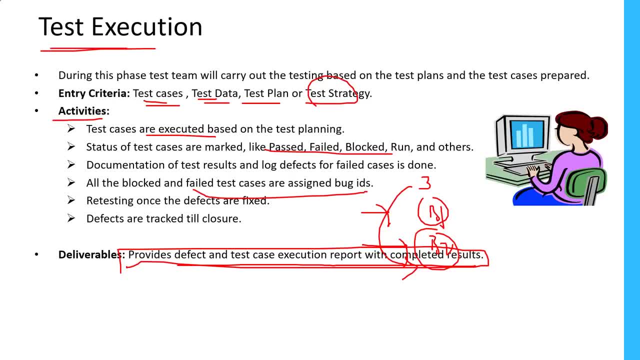 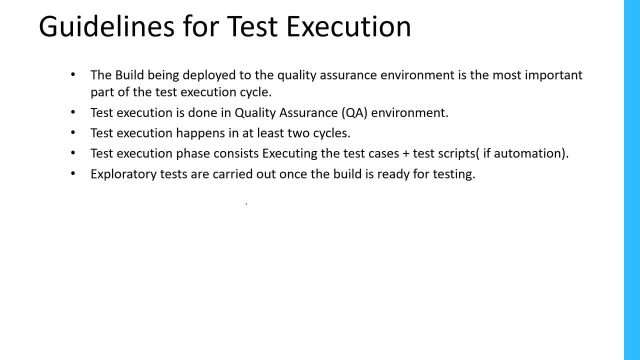 That's a very important. Now let us see the next phase. So once we have execution is done, the next phase is so guidance for testing. So here I have given enough some information about the bill being deployed to the quality assurance environment in the most important part of physics. 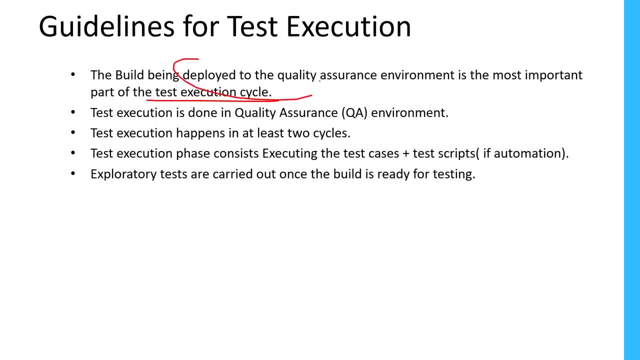 So, as I said earlier, if you want to do the test execution, the bill should be deployed. deployment means installation and test execution is done in quality assurance environment. So testing is always be done in the QA environment. We should not use any other environment. 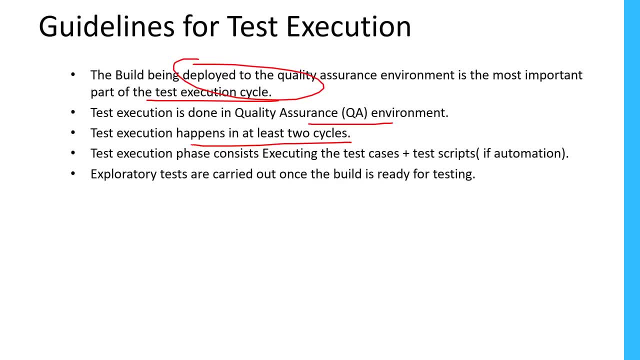 and test execution happens at least two cycles and test execution phase consists executing the test cases plus test scripts. So if your test cases are passed, as soon as your test cases are passed, immediately try to automate them. because once you automate your test cases, in the next build 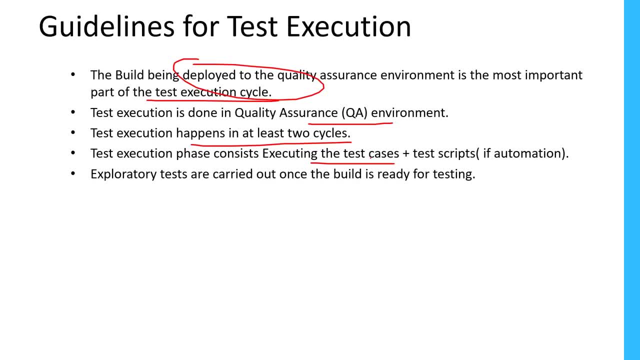 or from the next cycle you can. you no need to verify the same test cases manually. You can just run your automation So that will take care of test cases. So exploratory test also we need to do certain times if you don't know any functionality. 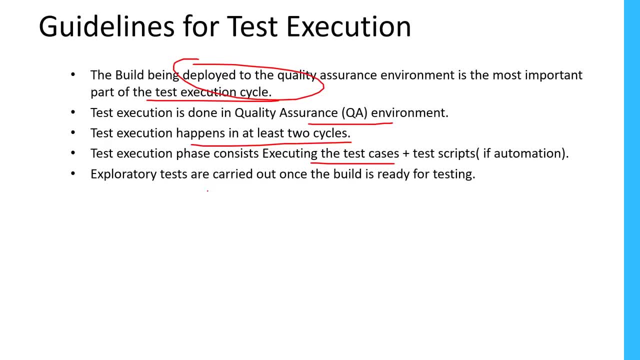 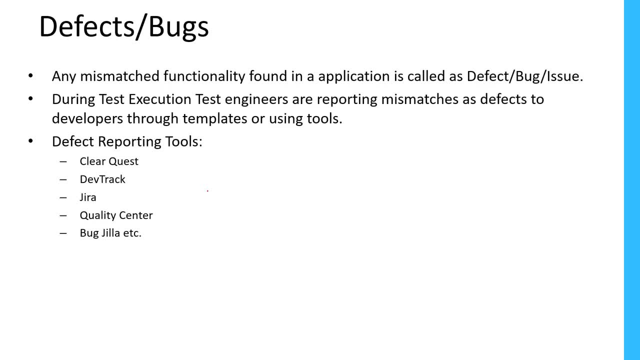 and if you don't know any documentation for that. So these are the few guidelines we need to follow. test execution: Back to the defects or bugs. So in the test execution, test cases that we need to mainly execute our test cases. So, but not only that, ask the main intention of executing. 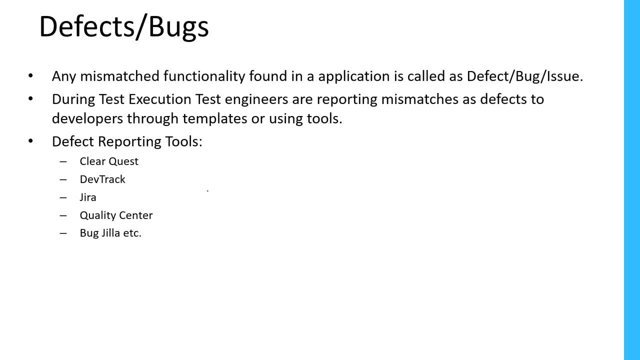 what test case is to identify the defect. So we should write your test cases such a way that it should able to find some defect. Okay, So whenever we are writing test cases, our main intention should be that SK should able to find the defect in the software. 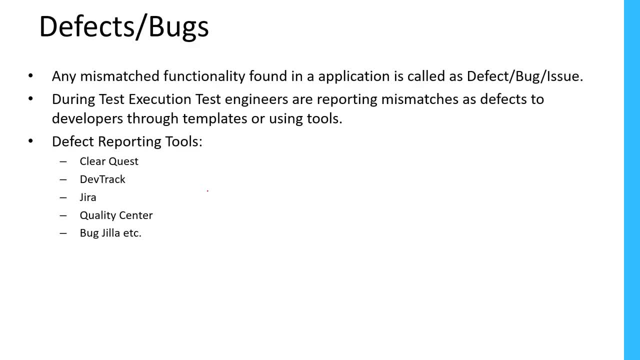 So the main intention. So now, what is the defects of bugs? Any mismatch of functionality found in application is called as it. so some companies or some people will call as a defect or bug or issue. So names are different, but everything is same. Okay, defect, bug and issues. but error is different. 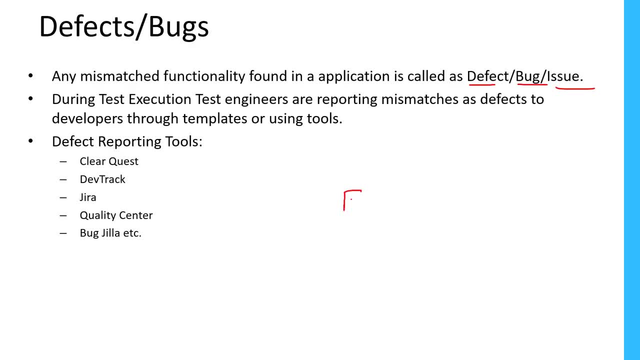 Okay. so error? we should not consider there are something, a theater. Now this one is error and the other one is defect. Error is a bug or issue, and there is one more technology called as a mistake. So there are not mistake, This is a failure. 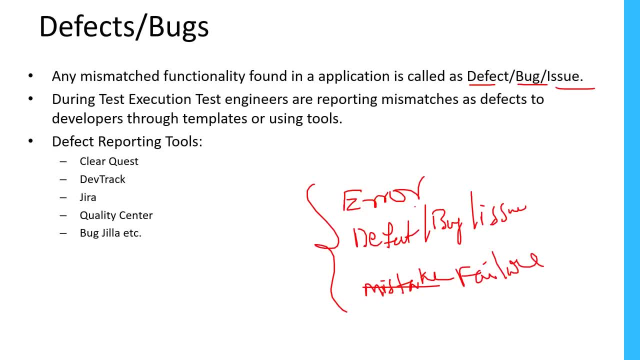 So multiple terms are there we need to understand. So all terms are similar, seems very similar, but a small difference is there. So error is different, error is a programming prospecting. So when developer writing the program, suppose if you do some miss, if you, if the developer is done some mistake, that will cause an error. 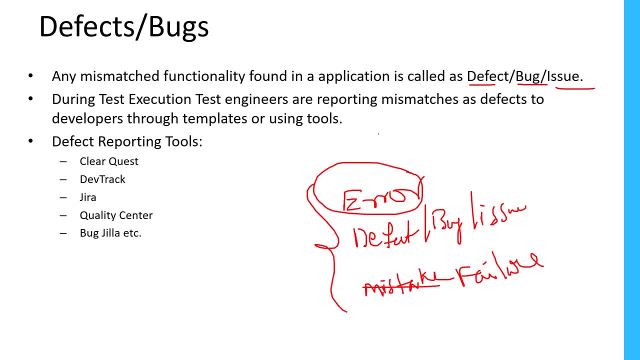 So like syntactical error, logical errors, So those errors will come in the programming, programming level. So there we call as a errors: Okay, so this is purely related to programming, but defect, bug and issue is different. So this is related to functionality. if application in application 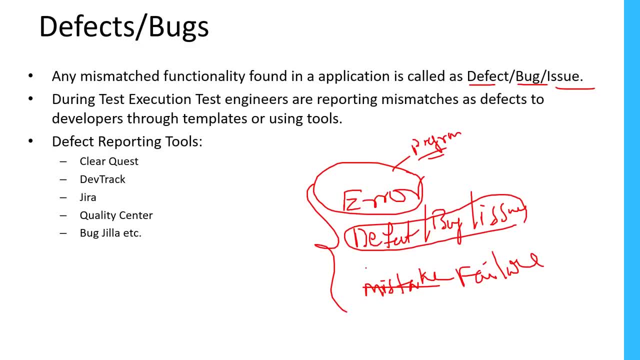 if any functionality is not working according to customer requirement, we will consider that as a defect, bug or issue And the failure means so once we deliver this offer to the customer in the customer environment, customer is working on the software. suppose this customer found something is not work here in the production environment. 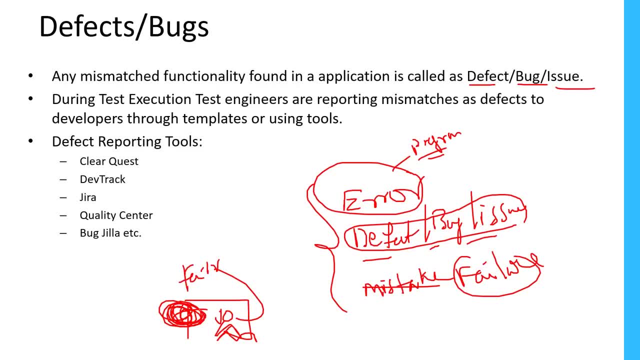 He will say simply failure. So something is failed in my environment. So in the customer point of view, they call as a failure, and testing point of view, We call them as a defect, bugger issue and developer point of view, They call as a error. 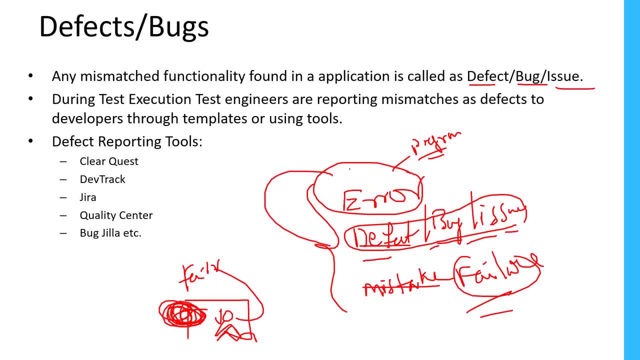 So errors will leads to defects. If the program is having some errors, either syntactical or logical, that will leads to defects and these defects, if they're not found in testing phase, that will leads to failures in the production environment. So this is a connection between error, defect and fail. 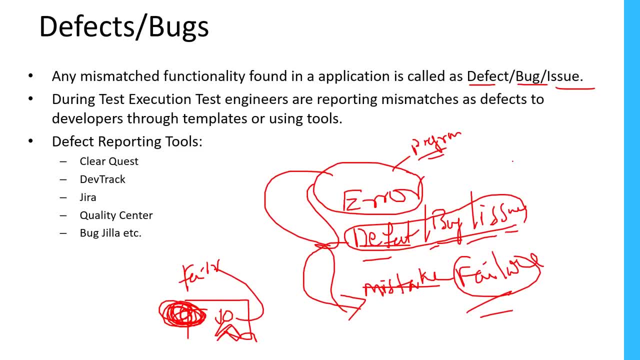 So error is related to the programming, developer, defect, bug issues related to the testing functionality, and failure is related to the customer point of view. Okay, So remember these terms, very important in perspective. these all theoretical understanding, So, but practically no use, but theoretically, the time of interview. you need to know all these things. 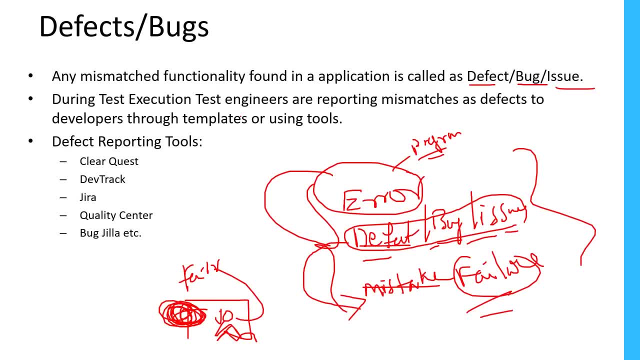 Okay. So when we need to call the defect or bug, if you identify any mismatch between our expected and actual result, that comes on the defect or bug. So whenever you found that mismatch functionality, then you need to report that defect to the developer by using some tools. 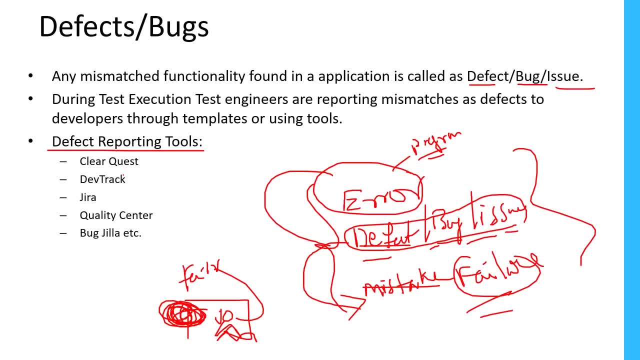 like a defect reporting tools We have point. So these are also some softwares. So clear, quest, dev track, Zira, quality center, bugzilla, These are all the different tools available in the market to report the defects to the developer. Okay, so I'll just cover this, this Jira part, how we can. Jira is not only for defect reporting. 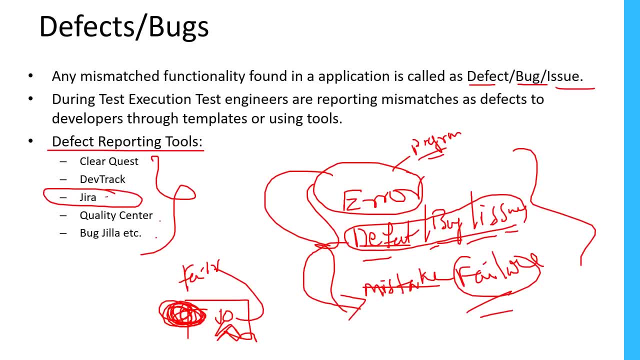 We can do a lot of things in Jira, Okay, so complete the testing activities We do as part of Jira, even in quality center also. So this is not only to our defect tracking tool. It can do a lot of things, all testing activities. 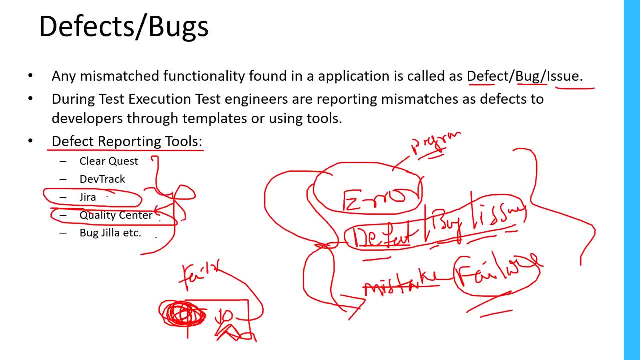 We can automate, so we can write your requirements. We can write your test cases. We can execute. our test cases will update the status. bug reporting- everything will part of this, So we use some tools to report the defects to the developer. Okay now. 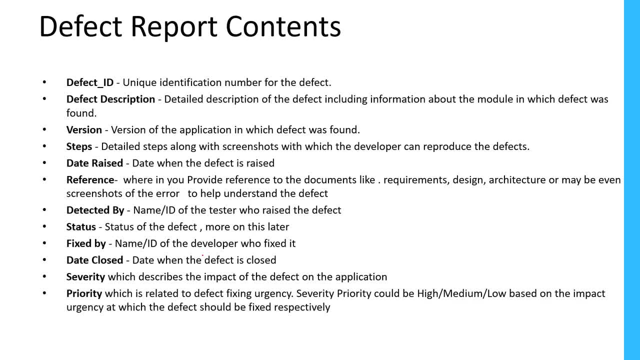 So what is the defect report? So we don't tell developer like simply say if you find a defect, we need to give a lot of information to the developer regarding the defect. So every defect we need to add some unique Defect ID, defect description and which version of the application you found the defect. 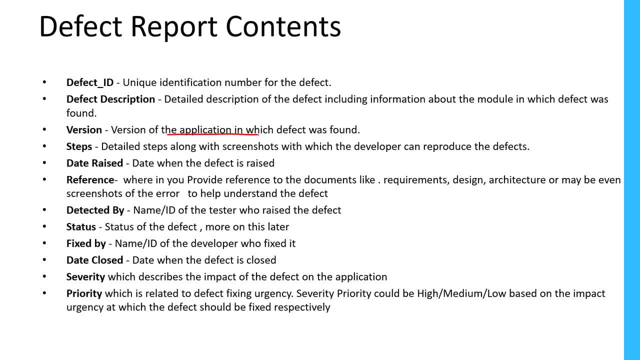 So there are multiple bills or multiple versions of the bills You will. you are going to test it- on which bill you found that effect. The bill number is also very important. Okay, and steps. So what are the steps you have executed While reproducing the defect? so that is also very important. 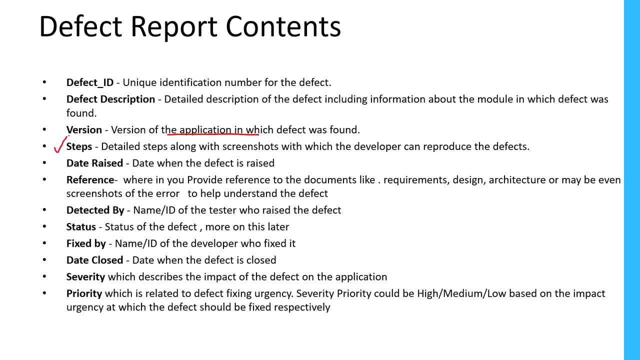 We need to send these steps to the developer and when you have rise in the defect date and what is the reference document you followed. So what basis you are saying that is a defect? is a part of a, the requirement, or is it part of use case so that you need to tell reference document? 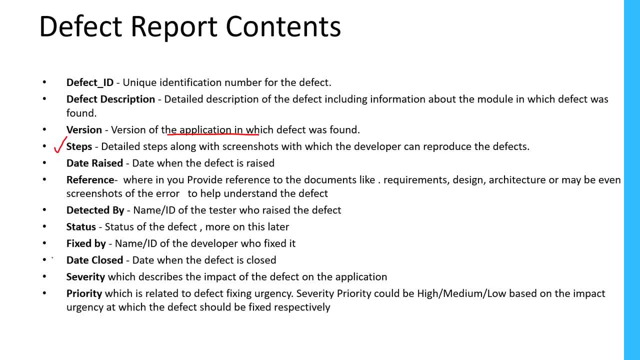 and detected by this is normally test engineer name, and what is the status of the difference? So this status will change according to status. So I suppose when you raise a new defect, the status will be the new and once the developer is started working it is in open state. 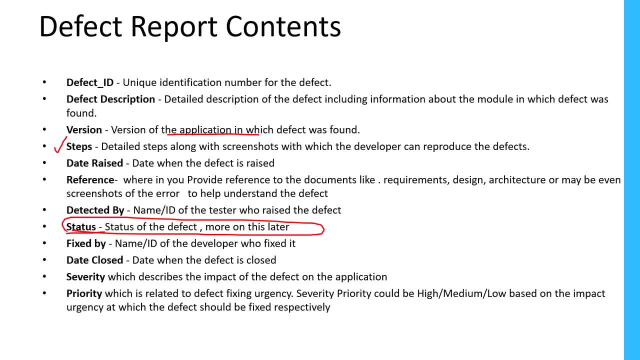 and suppose the developer still in progressing. he is in the middle of fixing the defect. that is in progress and once the developer is resolved the defect, the status will be resolved state and once we verify the defect and it is verified state. So once we close the defect, that will be closed state. 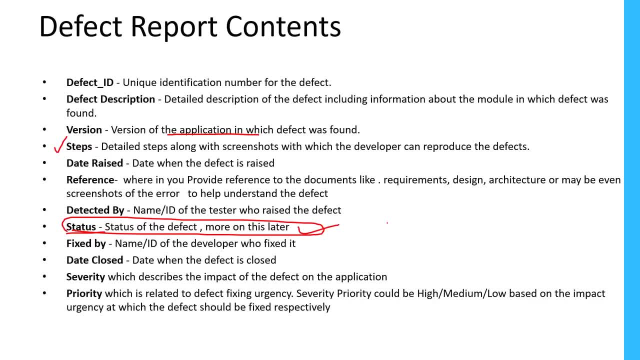 So this status will be changed according to the movement right when you raise the defect till it closes the defect. So it will go to status stages. So in each and every stage the status of the defect will be changed And then fix it by. so who is the developer is responsible to fix the defect? 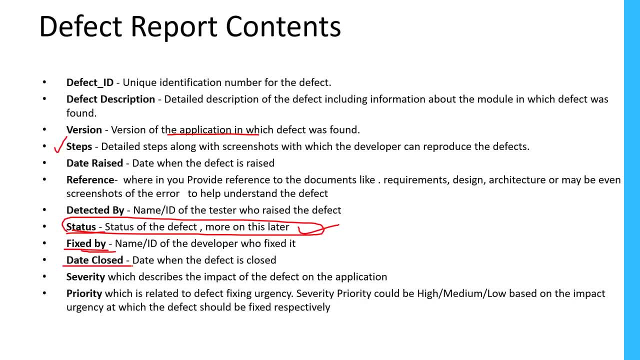 and date close, on what date you verify it and close with the defect and CVRT and priority. CVRT priority is very important topic in the defect reporting especially. you will also get a lot of questions on this, So let's get clarity on this in test case. 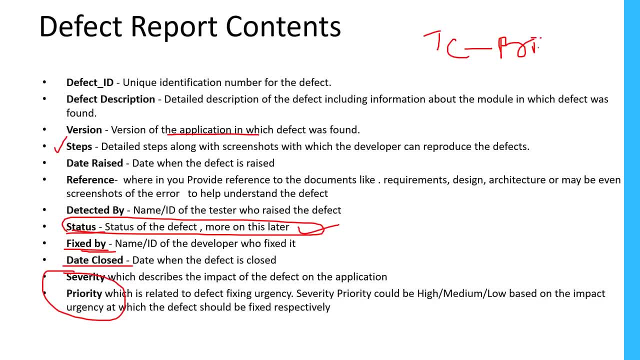 We talk about priority. So in the test case point of view, the priority means order of execution, in which order we have to execute Our test cases and which test case. what are the test cases We need to exclude? first level, second level, third level. 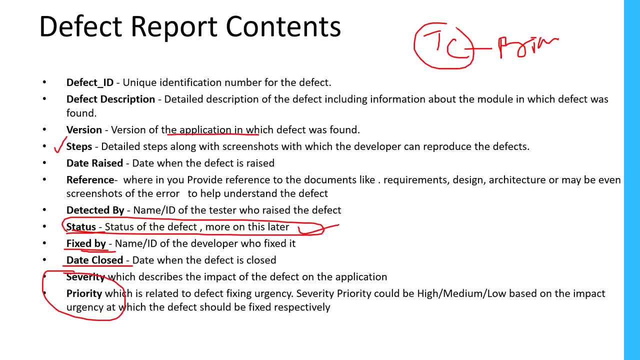 So that is decided by the priority in case of test case but in the defect also is having priority and also CVRT. So defect is also having priority along with the CVRT. So priority describes the timeline. So priority is basically described. the timeline means suppose if I give P1 as a priority, developer immediately has. 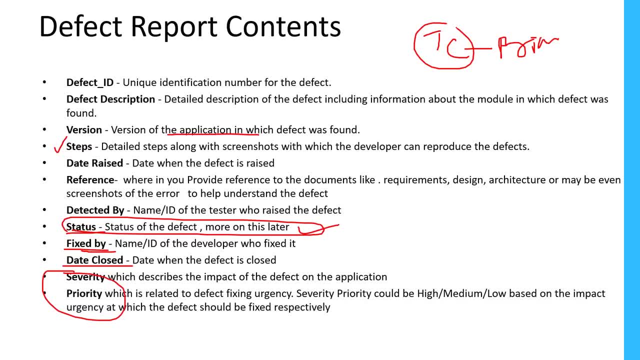 to fix that issue because high priority. So if I give P2 or P3 developer will take some time to fix that. So that is again based on the timeline we have to give the priority. Suppose let us say I have a 15 days of time to test that application from the day one. 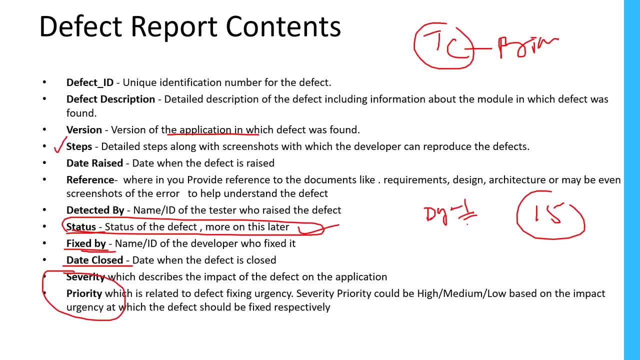 I got some issue. Okay, that is not a blocker because of that issue. We are still able to proceed. but I got issued in the day one. So in this time we don't need to give the P's zero as a priority, even as a priority, because this is not urgent to fix by the developer. 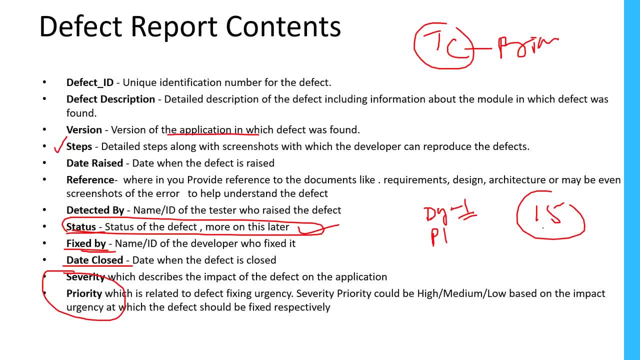 So this because this is a very minor issue and still we have more time, So developer can fix it later, So we don't need to give P1 for this, So we can just give P2 or P3, like same different. But for example, let us see this scenario: 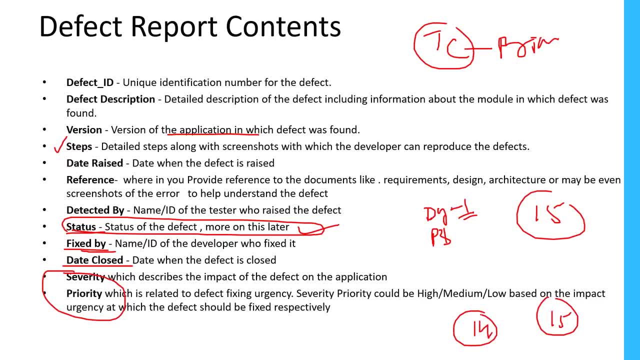 We have 15 days time. We are almost we reach 14th day here. We got the same issue. Whatever I should have found, even this issue came in the fourth day. 14th, 14th day- We found this issue. 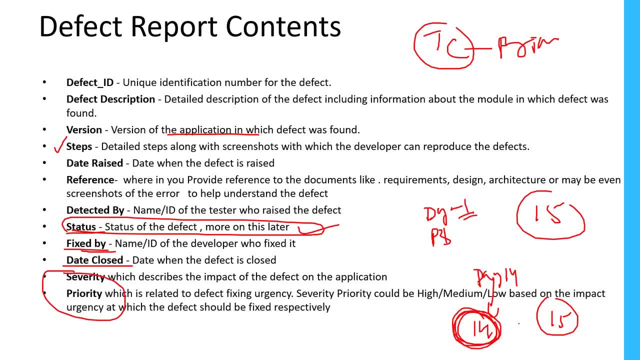 Now it is a minor issue only but as per the timeline, we have to fix immediately. So the same issue, that priority will be very high. Okay, So based on the timeline we have to decide the priority of the defects, How early that developer should fix that issue. 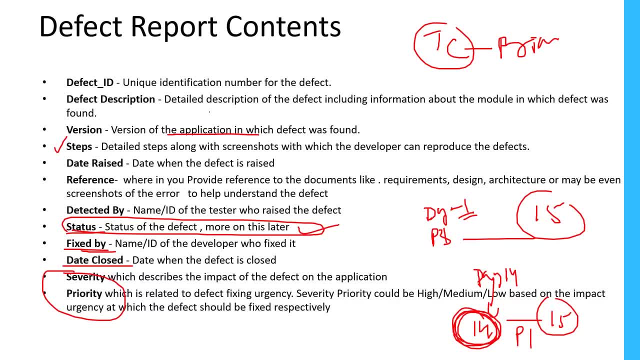 Okay, that's the talk about the priority. It's very important. So priority and severity. So priority will be changed based upon the timeline And severe severity means describe the seriousness of the seriousness of defect means. how impact, how well the defect is impacted that application. suppose application is not installed. 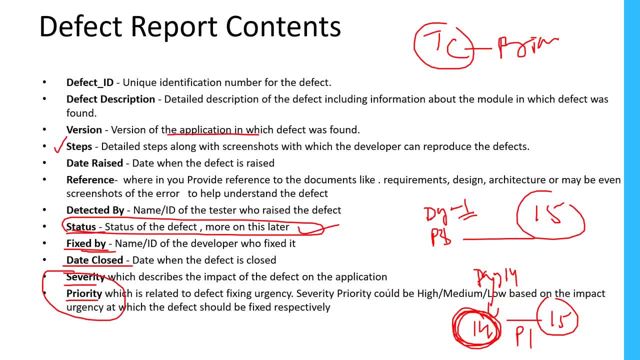 For example, while at the time of installation the installation itself is paid. That is a defect, That's a blocker, first of all, right. So because of that we cannot proceed further testing. So for those we have to give high severity, like s1, s2, s3.. 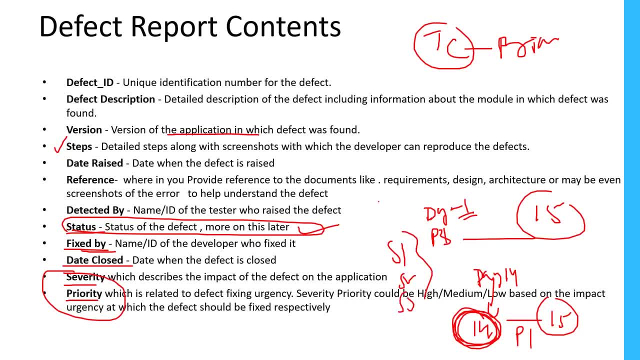 We can give some code for this. So, blockers, we need to always consider very high severity, So that will completely stop your execution. Okay, so, CVRC, talk about seriousness of defect, how well it is impacted your testing, but priority: describe the timeline. based on the timeline. 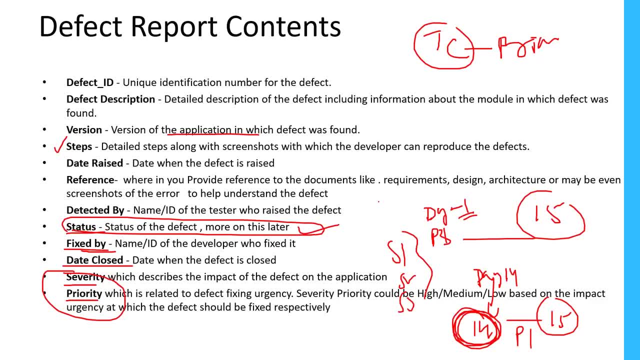 Okay, how much, How many? the developer should fix the priority. So that will talk about priority and severe and interview The people are so many questions on this. What is severity, What is the priority, What is the difference between priority and severity, and who will provide the severity of priority to the defect? 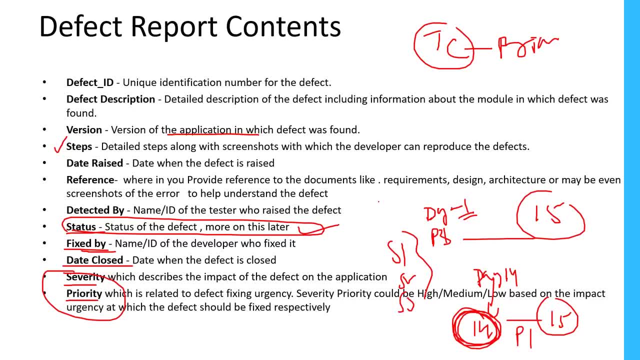 So normally, when you rise your defect according to your opinion, you will give you severity and priority. Okay, you will give you test. engineer should give you severity and priority According to your knowledge, but severity- completely newer control because you know how well the defect is impacted your system. 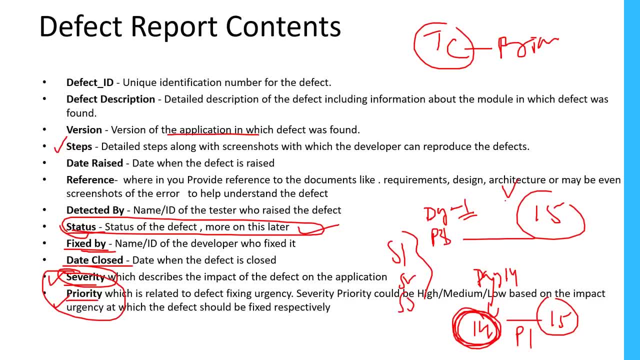 because you are the tester. if you find some defect, because of this, because of that effect, you completely blocked your testing, or somehow you are able to proceed, or okay, even though if you have some particular defects till you are continuing, or able to test all other functionality. 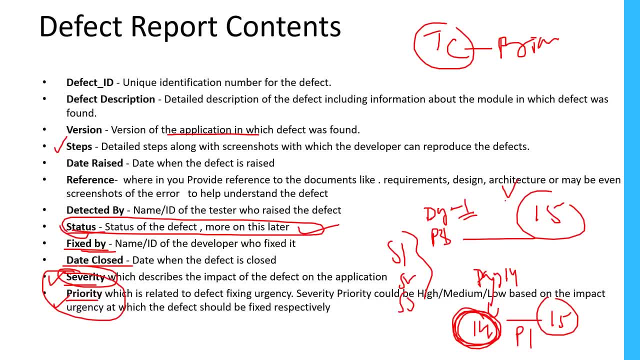 So that status? Because you know right. So developer doesn't know business analyst management leaves, They don't know about it How the defect is impacted your system. So severity is always given by the tester or me, So this should not change by anybody else. 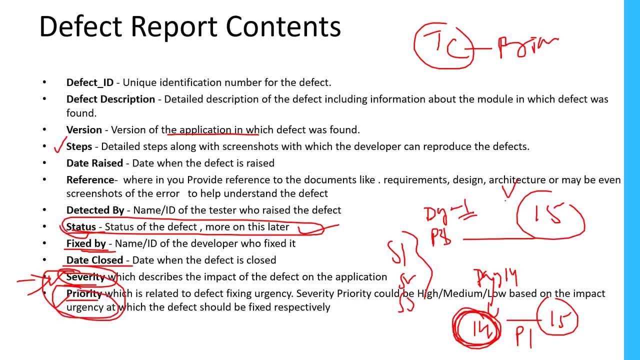 But the priority can be changed later by developer or business analyst or leads. That's not in our control. But at the initial level we have to give severity and priority. But Priority- suppose you think that effect is higher priority You have to fix today itself. 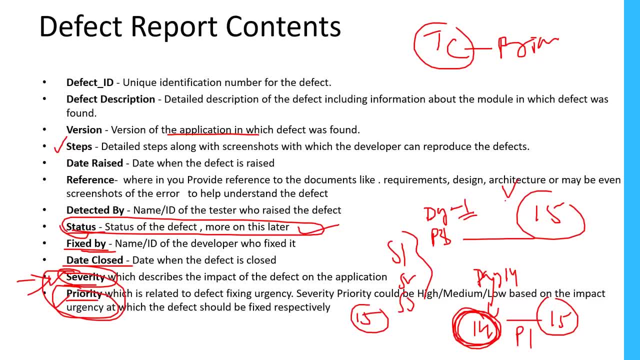 For example, let us say you have 15 days duration, You are there in the fifth days. Let's say you are testing in fifth day. So here you have found a defect. So, as per your knowledge and as per your opinion, you have given, as a P1, high priority. 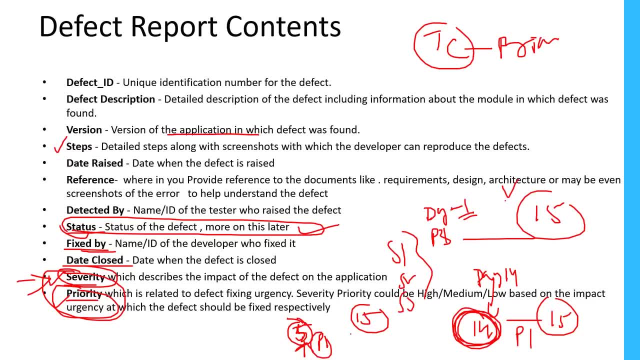 So once the developer is received this defense, so developers think like, okay, still we have 10 more days, I can fix it later. So just reduce this priority. So they can reduce the priority, They can make it as a P2.. Okay, 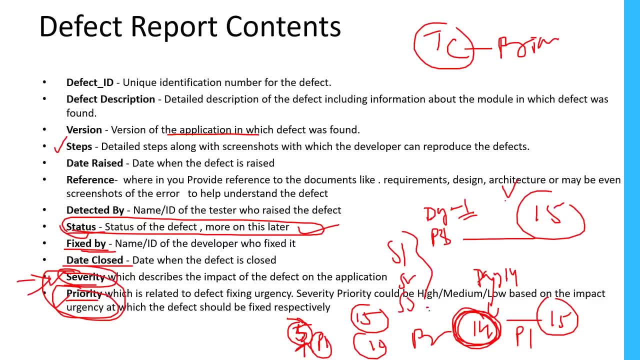 Suppose the timelines are increased, for example, 15 days is extended, 30 days Now again, priority still reduce. P2 is comes to the P3. So priority can be changed by testers or developer or business analyst or stakeholders. that is up to them. But your responsibilities you have to give as per your opinion, severity and priority. 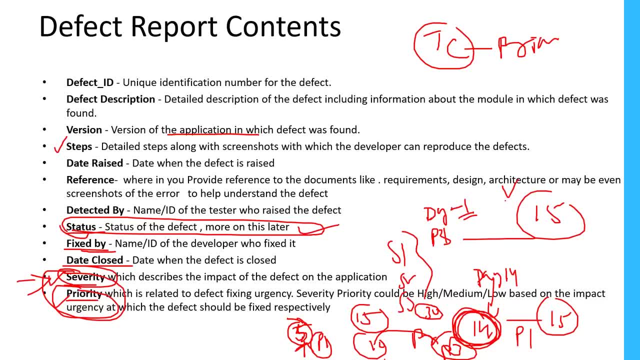 Okay. So see, a severity means how well your application is impacting because of the defect, and priority means order of execute. priority means how early the defense should be fixed by the developer, So that you have to tell a very important question. So we will give the severity. priority means you have to explain all these things. 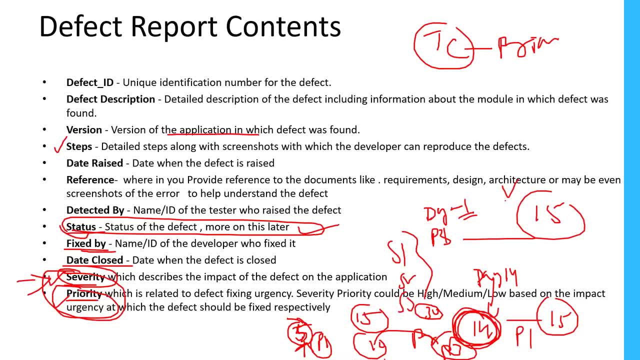 So testing in here will provide the severity and priority. but the priority can be changed by the developer or business analyst according to their opinion later, but severity should not. It will change once the testing here said this is a severity. That's it. 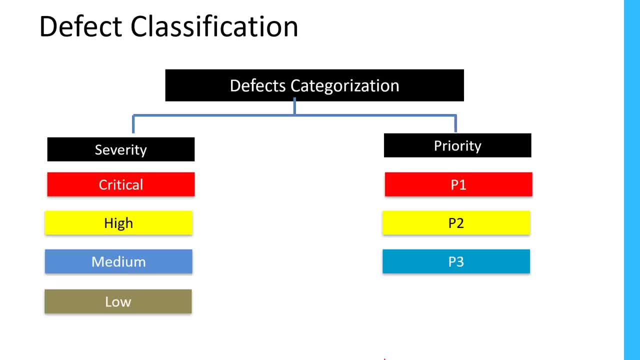 That is fixed. So now let's class categorize the difference. So defects normally comes and let's see severity priority in detail now. So normally severity will be cancel like critical high medium. No, even in the defect reporting tools. Also, they will provide you in the list box. 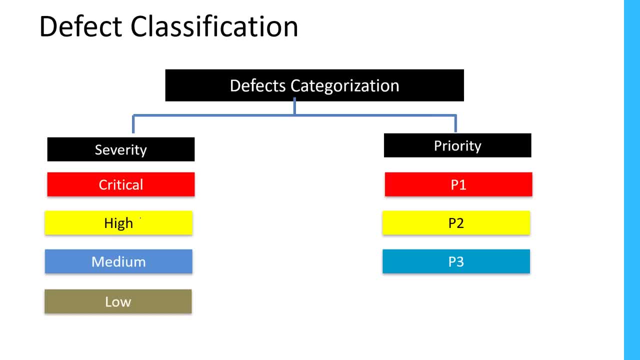 So as soon as you write in all the defect information, they will. they will give you some drop-down box To select these fields. So what is severity level? Whatever defect you rise, that's far under either critical. high, medium or low, or priority also P1, P2, P3 is a priority. 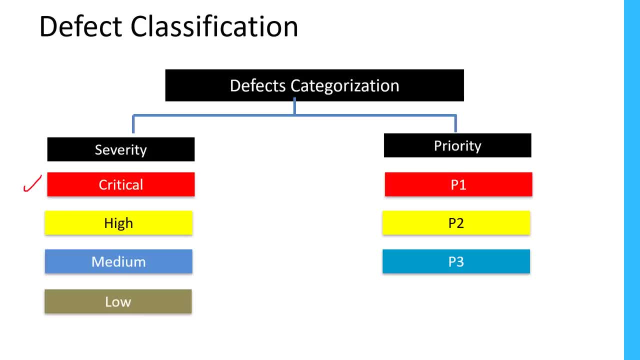 So severity means a critical means a blocker completed, block. You are cannot proceed further testing. in those cases Your defects should be fall under critical. now Sometimes the major functionality is not working Okay. So, for example, application is installing fine, Okay, login is also working fine. 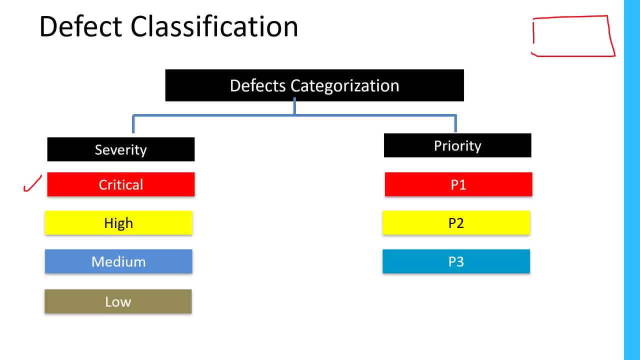 But let's say this scenario: I have a login. Okay, login when you need to login should be successful. when I provide valid data values on a valid password, then only login will be successful. Okay, so my scenario is like that. So I am providing valid input. 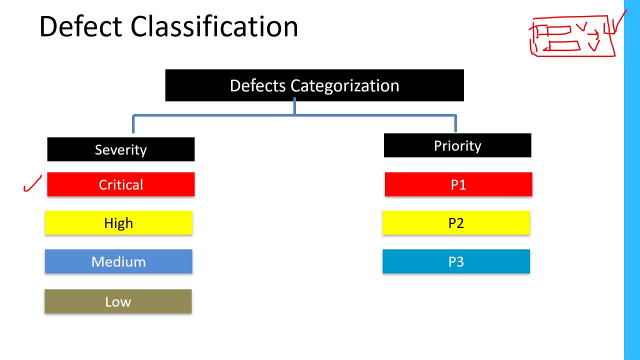 I'm successfully logging. that is fine, But even though when you provide invalid input also, it is able to log in. So this is a bigger defect, right, But here did we block? I'm pre-testing here. No, we haven't blocked here. 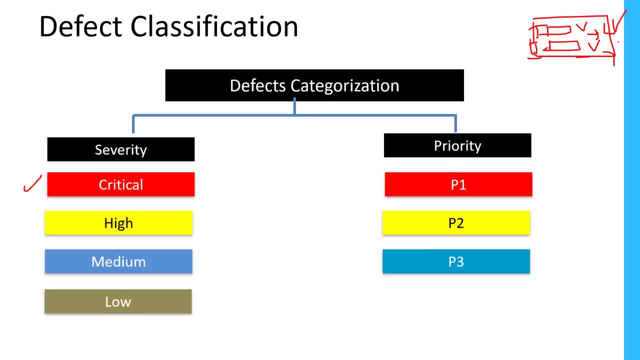 We are still able to log in and we are continue other functionalities, but still this is a high priority because this is a major function. This is not a blocker, but still it is far under high CVR key because login is very important. authentication property. 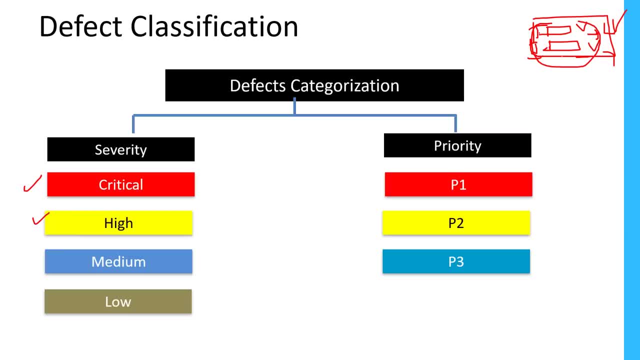 right, very sensitive. only valid rendition should able to log in, but here it is also accepting invalid. So this is a major functionality of the application. If you find these kind of defects, that will be fall under high and then medium. So medium means this is also a functionality. 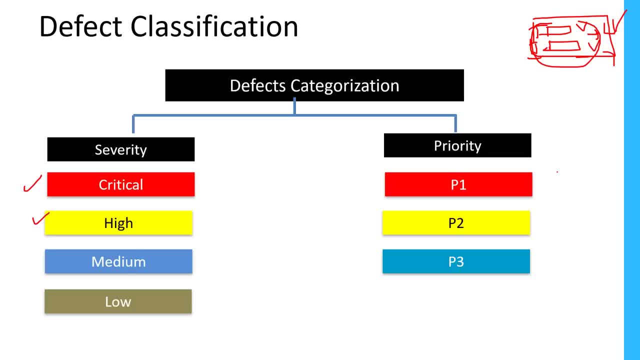 and that functionality sometimes is working and sometimes is not working. So that kind of unstable behavior like, for example, you are expecting some logo should be there in your UI. So, for example, this is your application, The logo should be present here and you are expecting the logo should have a. 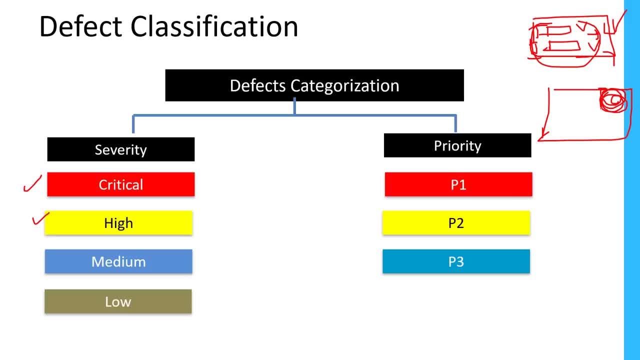 clarity. Okay, so this logo should have some clarity, and then it should display the right and left side. So that's your expectation. But, as per your requirement, this logo is very larger size and it is not aligned properly here, but this is not blocker. 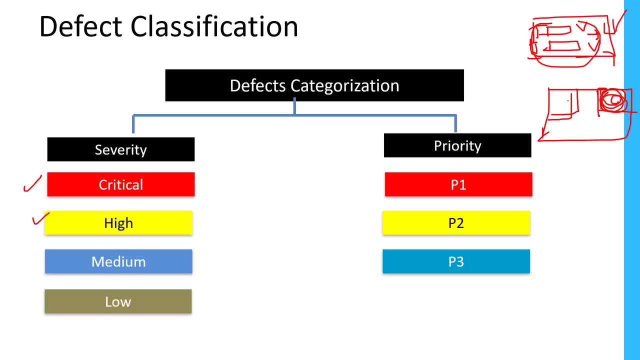 and this is also not major, functional, but customer point of view This is very important. So these kind of defects we can give under medium Okay, And the low priority means, like the spelling mistakes are, colors alignment. So these kind of issues will fall under low priority. 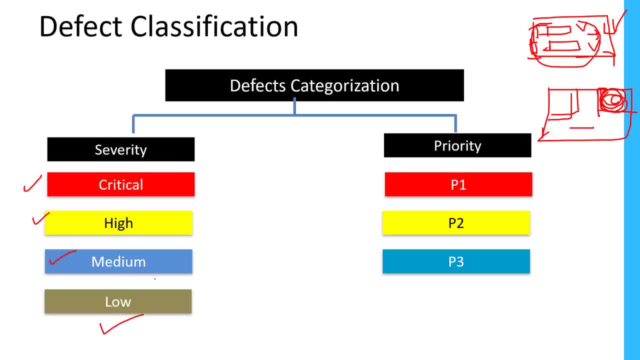 low severity So that will not mostly affect the functionality. Okay, that is again based upon your knowledge and based upon your experience. You have to give the severity to the defense. Okay, that's very important. So all the defects, we have to give it a critical. 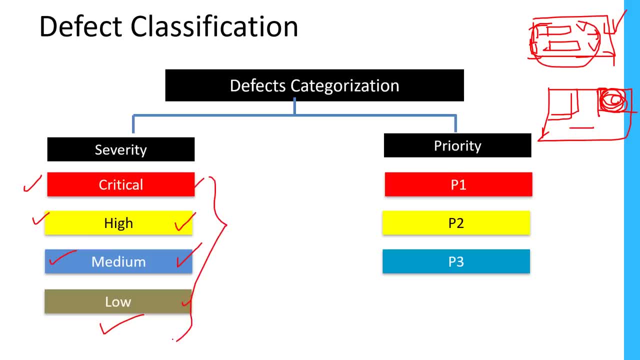 or high, medium or low. So based on the severity, the developer will decide whether we need to Fix that immediately or later. So if it is a critical within three to four hours, they have to fix the difference because you are completed block. If it is a high, within one day. 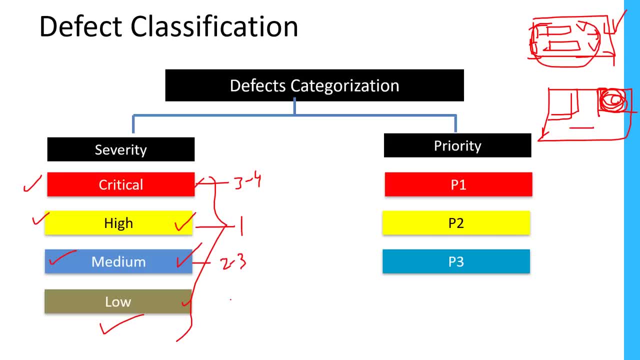 they have to fix. if it is a medium to take two through two to three days, three days of time. if it is a low, it will take more than one week of time. So they will try to fix those defects based on the severity which you have provided to the defect. 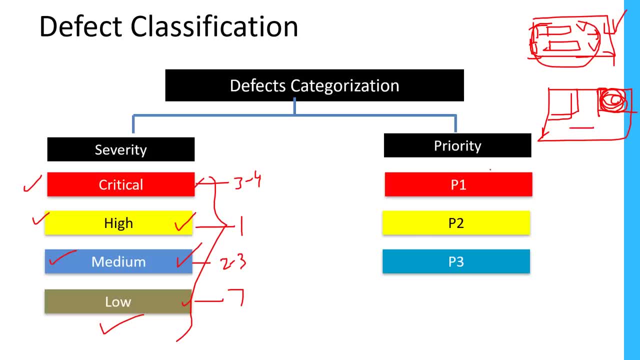 Okay, So this is about severity. now come to the priority. So priority is your opinion. However, you have to fix the difference. So if I give a p1,, so that means you are asking developer to fix immediately. So if I give p2,. 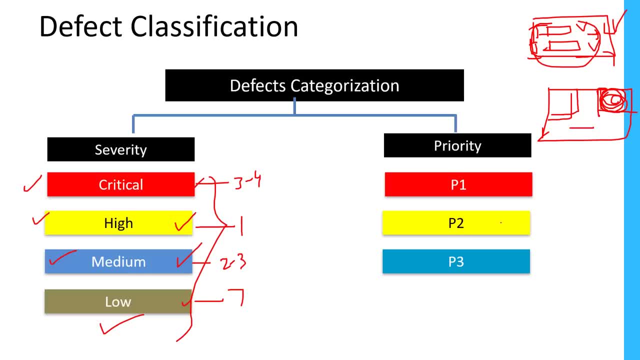 so you are asking developer to fix this in one or two days, or if you three means this is not high priority, You can just fix later in the coming builds, Not an issue. So that's priority. Also, We have to give to the deep. 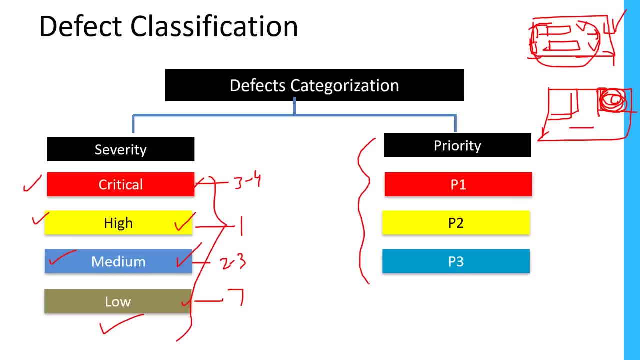 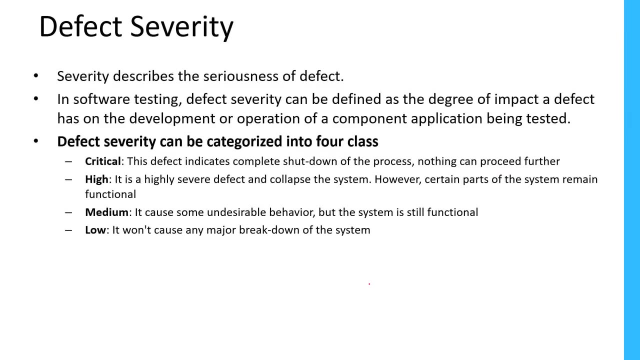 This is a DVR CBR 10 priority concept and the overall defect reporting concept. This is very, very important concept in input perspective and while you are working on in real-time environment. severity and the priority: Okay, and then sometimes I just talk about defect severity, right. 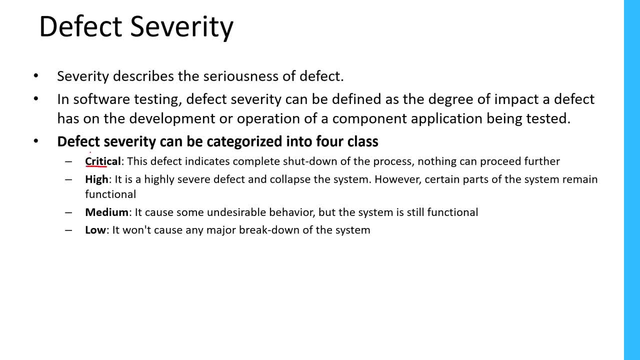 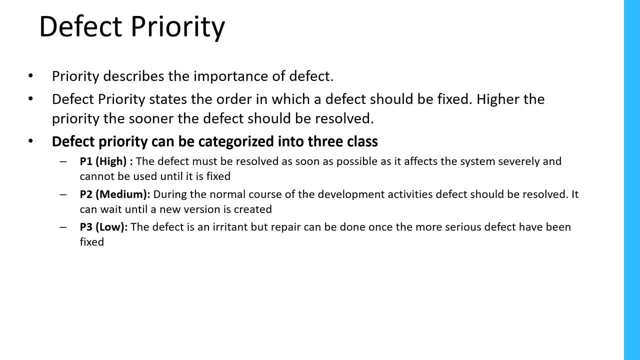 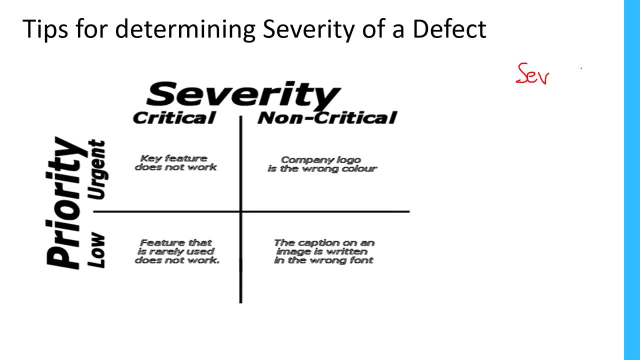 and what time when we need to give critical high, medium and low. I have given same example here. You can just read this later. Now This is your again defector priority now. So sometimes we have talked about severity and priority right. So if I divide this zone into four section, sometimes priority will be low. 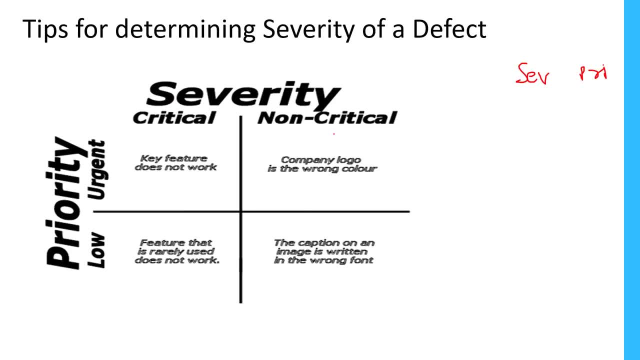 and high urgent and severity will be critical and non-critical sometimes. So there are some defect. Suppose if you have one difference, that defect can fall under either in four coordinates: in the first quadrant, second, third or fourth. Sometimes your defect will be very critical and also urgent to fix. 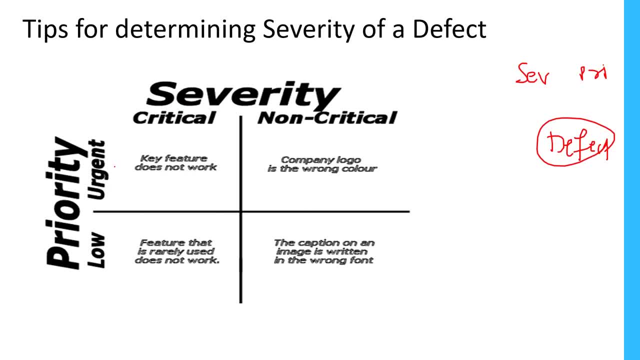 That means very high severity and high priority and sometimes you are defect fall under the second coordinate. That means it is not critical but very urgent to fix it. And sometimes your defect is fall under third section. It is very critical but it is a low priority. 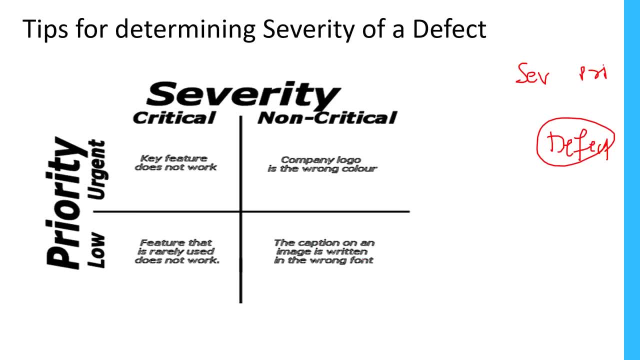 and sometimes your defect fall under the fourth coordinate, So it is non-critical, but it is low, not critical, and also it is low priority. So that will be decided by the testing. So here are given some examples. Suppose the major functionality is not working. 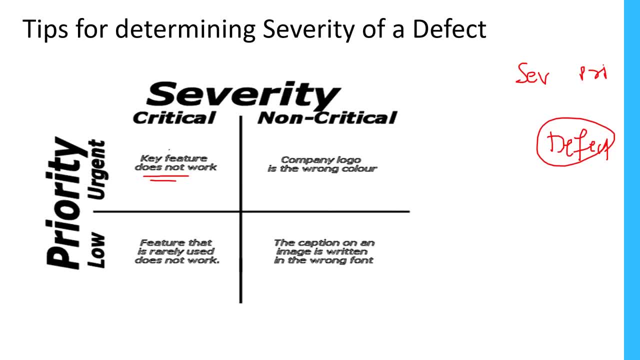 Suppose installation error, installation itself is failed. That is critical right because we completely blocked. and also it should urgently fix because unless until it is fixed We cannot proceed further. what testing activities will be completely blocked? So that will be impact the again timeline and deadlines. 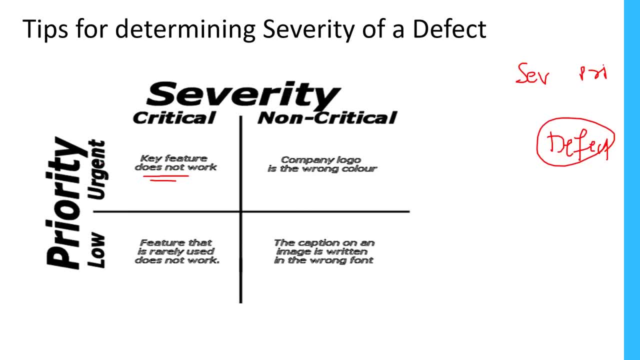 So that will comes under critical as well as urgent. And here company logo is wrong color So we are expecting some color should be there. company logo: It is not in the color. This is not much critical because this is not affect the functionality. 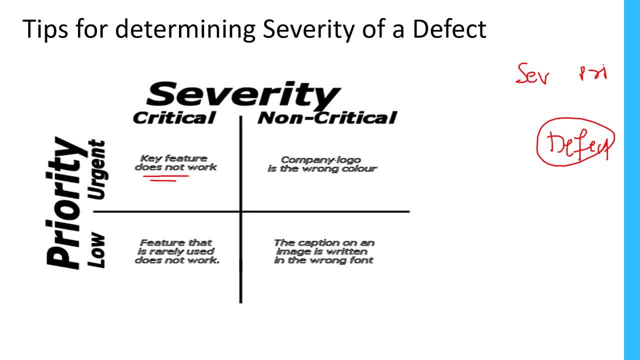 We are still able to proceed further, and excluding all our test cases is not critical, But sometimes the same issue will be the urgent. So when it will become urgent? the deadline is tomorrow. So customer first will see the logo itself right, So whether his company logo is properly aligned color or not, 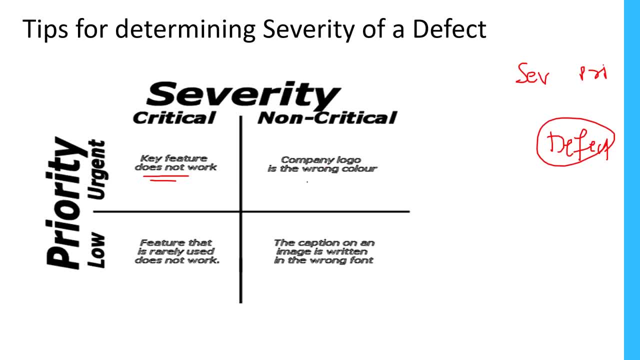 So the customer point of view, that is very important. So if tomorrow is a delivery need to deliver the application to the customer tomorrow. So if still logo color is not there, So even though that is not critical, but this is a very urgent customer point of view. 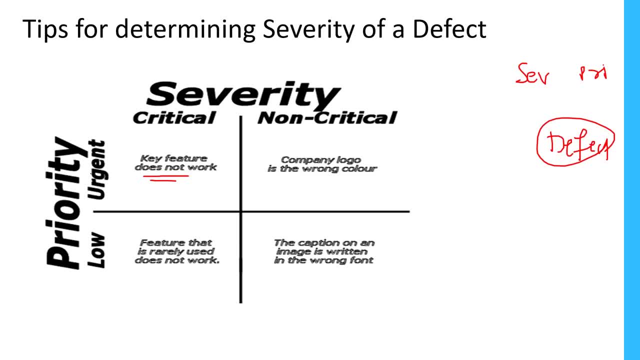 So those defects come fall under non-critical and urgent. and one more so feature that is rarely used does not work. So there is some feature available in application that feature normally working fine, But sometimes It's very corner, Suppose, if I do the same function at hundred times somewhere or once or twice. 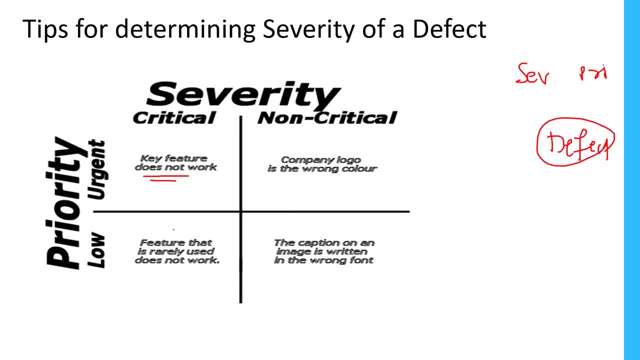 It is not working Okay. So those functions are critical only, but low priority. So why it is critical? So customer using hundred times somewhere He got an issue, but still customer point of view that is a failure. So it is a critical only major functionality. 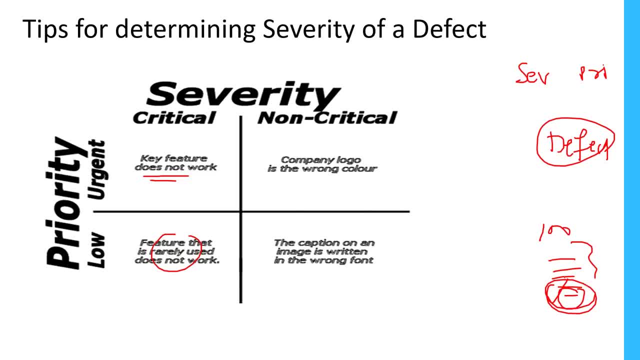 But we don't know, we don't expect, we can't expect in which time This error is coming. but if comes, that will impact more on this application, more business. So that is very critical, but testing point of view still, we have a time deadline to deliver the customer. 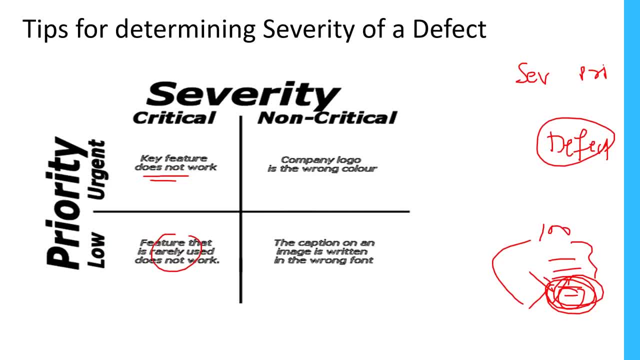 So we can just give a lawyer- It is critical, but it is a lawyer- And one more so the caption on an image is written in the wrong font, So this is a font actually. So suppose, as per the customer, the website, they want to use a bird bird as a font instead of that. 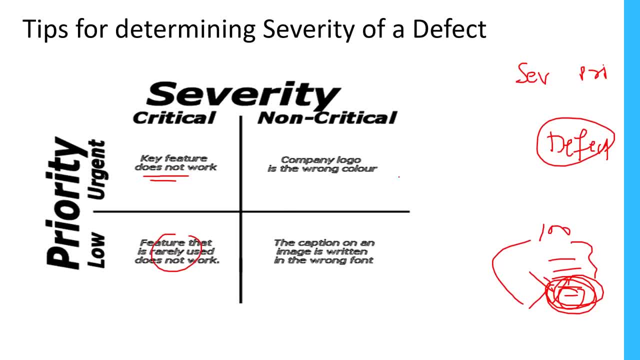 They have to some other different font and those are non-critical and also low priority. Okay, So, based upon the criteria, you have to decide what severity and what is the priority of the deeper. This is a very critical job of the testing. 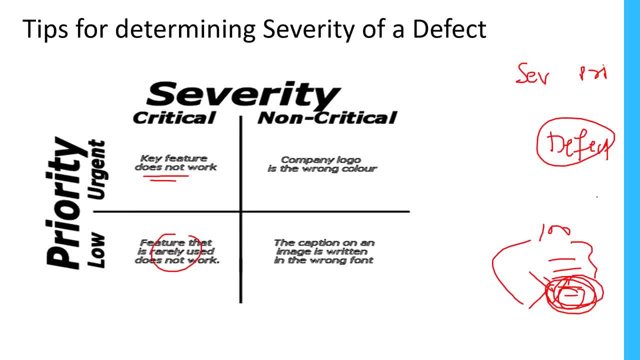 This is a main scale. Okay, so you will get a lot of things into the questions on this. They will give you a lot of scenarios like this and ask you to: okay, This is the scenario. What is the priority? This is my situation. 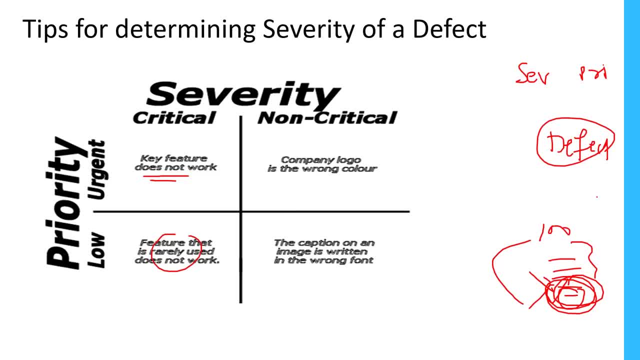 This is my scenario. So what is the severity and priority you will give as a testing? So people will ask you questions like that. So it will come through experience slowly. So by seeing some examples like this, we will not come to know which severity and which priority you have to give based upon the time. 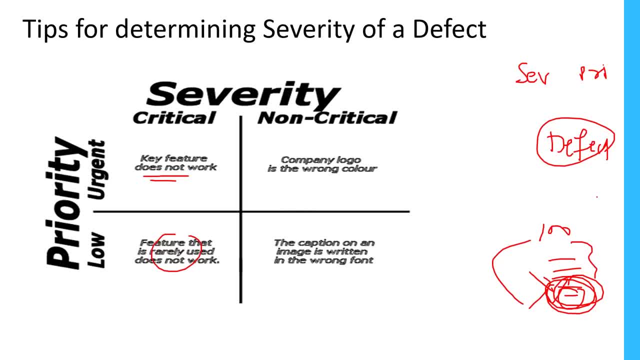 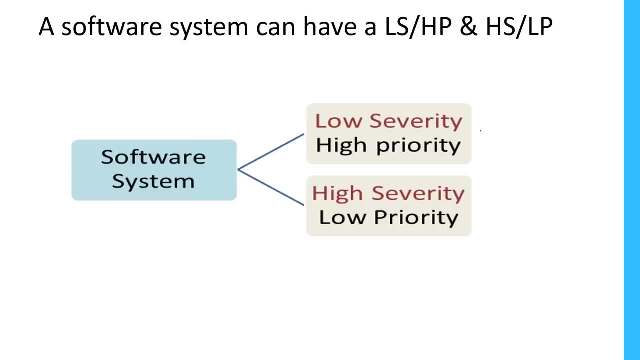 You need to always remember priority is always based on the timeline Okay, and severity is always talking about the seriousness, how well the defect is impacted Your system. that is very important. Next here, sometimes some defects comes under low severity and high priority. high severity and the low priority. 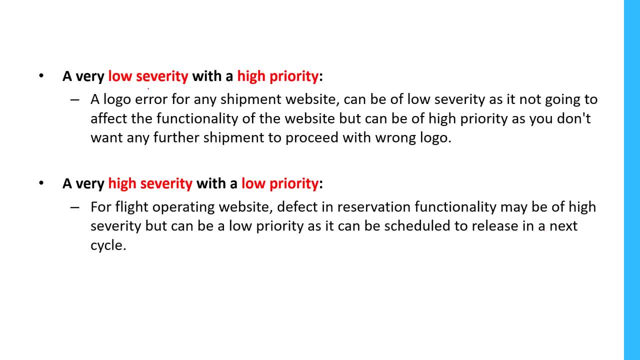 So just now I talked about the same thing and here I have given few examples: low severity, high priority and high severity and the low priority. Okay, So see the example: low severity and high priority. A logo error of any shipment website can be low severity. 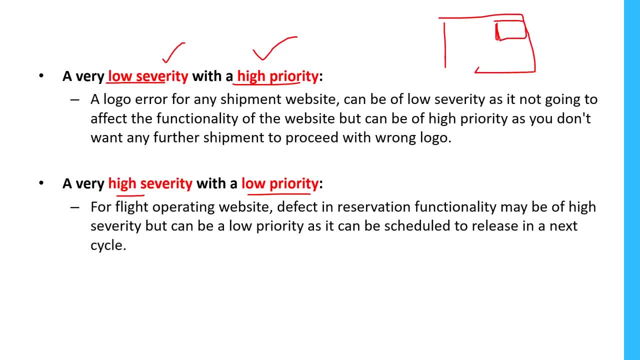 So a website we have a logo should have that our website contains a logo. Okay, So this logo is not properly aligned, a logo error. So this comes under low severity because that is not impacting other functionalities. not a blocker, low severity. but customer point of view, this logo is very high priority. 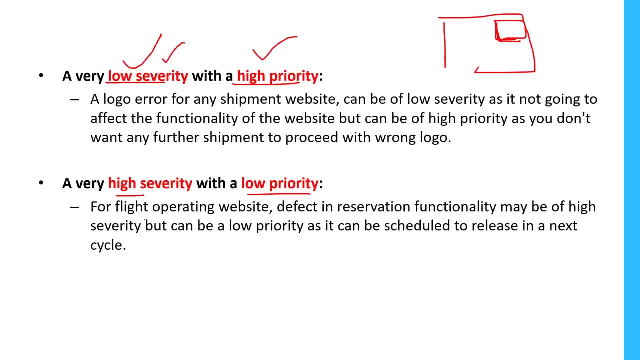 right. Similarly high severity, low priority. Suppose there is a flight operating website, So we need to book a flight. So in this functionality, while booking your flight, there is a functional error. Okay, there is an error of there is some defect in the while booking your flight. 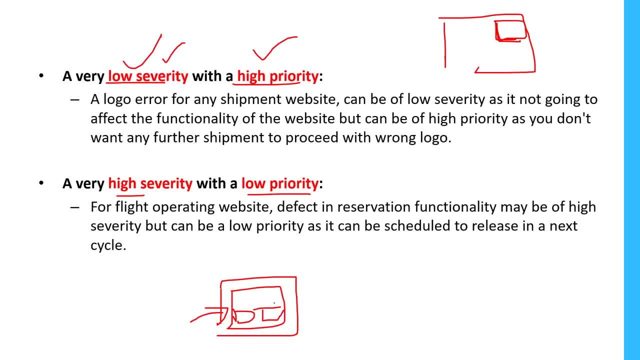 So this is high severity because this is a main critical functionality. booking flight is a very critical functionality, but still you have some timeline right. Suppose if you have long duration to complete this project, still it is in testing cycles- then you can just give the low priority because in the next two bills 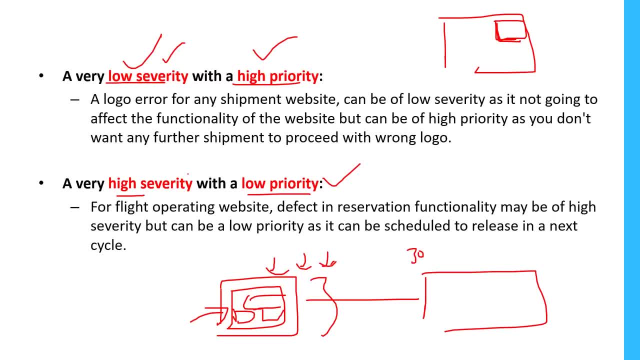 the developer may fix that issue. So in interview also, people will ask you like this: So can you give one example for low severity, high priority, or can you give some example for high severity in the low priority? So you should, you should remember few examples like this. 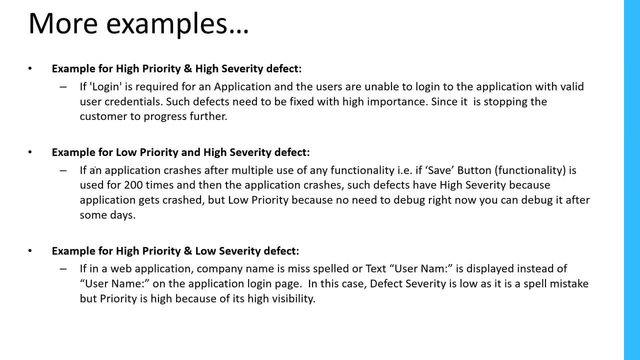 I have given more example in the slides. You can just go through this later one by one. You will understand, at least if you remember one or two examples. you can easily answer these questions in internet, Okay, So here I have given more examples, different combinations. 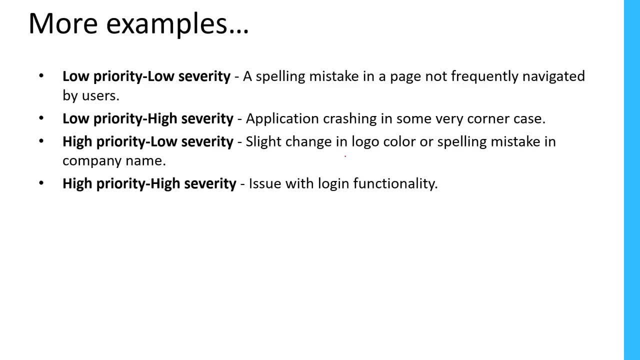 So you can just go through this very simple and no need to remember all of them, just one or two is enough. So to answer the interview questions. So this is all about defect related stuff, and the one more important field in the defect report is defect resolution. 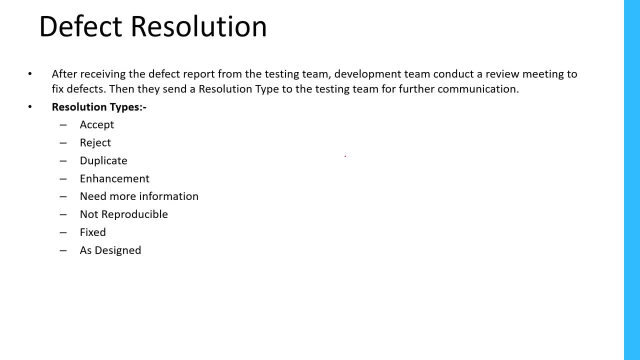 So people will ask you: what is the defect resolution? the normally when you rise your defect, So developer will have some opinion on the defect. Okay. So what is that opinion means? Sometimes developer will accept that our defect, Okay. he says okay, whatever you have report is genuine defect. 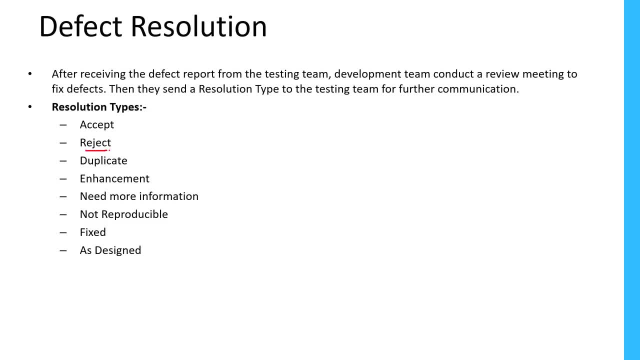 or sometimes he may reject your defect. It doesn't feel that is a not a mismatch behavior. So developer is having different opinion. So in those case he can reject the defect also and sometimes he will give resolution as a duplicate. Sometimes you already rise defect earlier, the same kind of defect again. 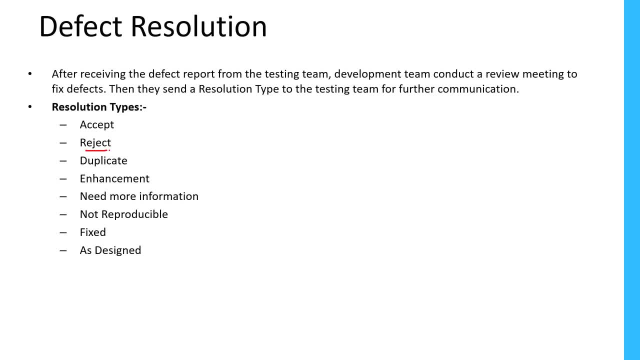 You rise again. So the developer will say: okay, this is a duplicate effect which is already raised earlier, So we already have the issue, or I only have the defect ID for that. So this is again. you rise to second time. This is a duplicate. 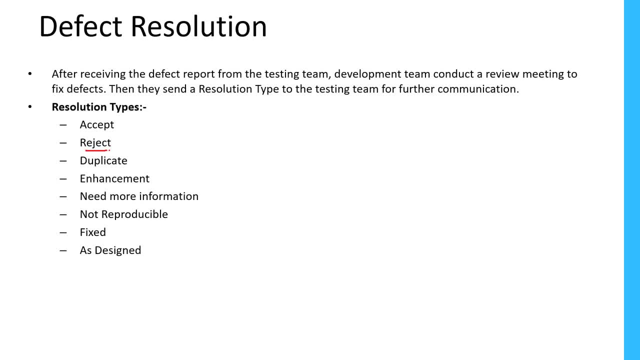 So please close it. So developer will ask you like that if it is a duplicate and sometimes developers is enhancement. So sometimes what you will feel is you will feel some function to be. the function is there in application. that will be good, but that is not part of requirement. 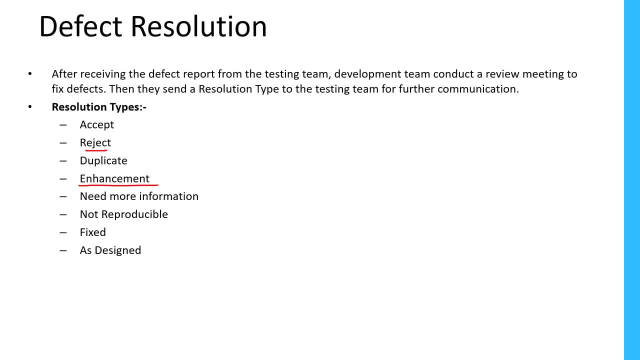 Just that is your feeling. Okay, so you thought something should be there in your application. If it is, add this option, that will be good. So let's say, I need to select. I have a small application like you need to send: select from location and to location. 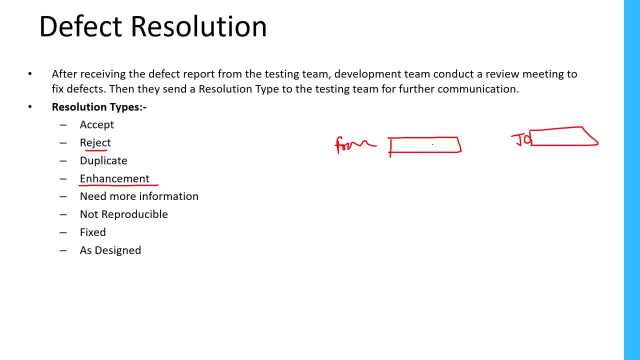 Okay, So then here let us say, you need to write your, you need to type your locations here: city names and Hyderabad, the Delhi, and so on. like this right, You need to type Your locations. so, as per the requirement, it will be like this one: 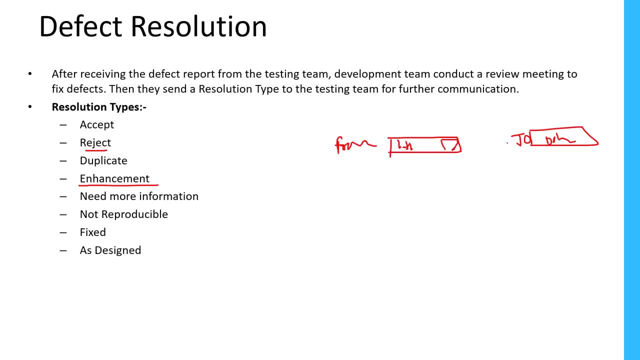 but what you feel is, if they have provided some drop-down boxes like this, if you are able to select the city from this list, that will be good right. So that is your feeling, but that is not part of it. But suppose if you rise defects like this, the developer will say it is enhancement. 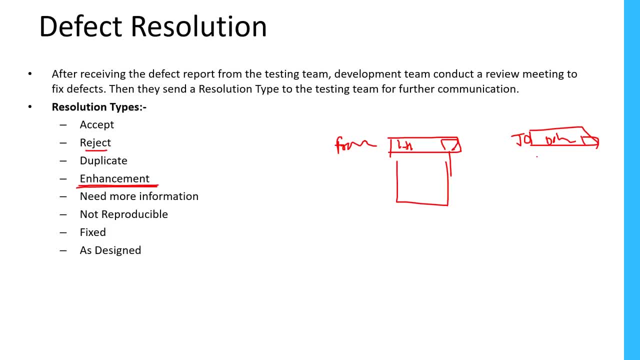 Okay, this is idea is good, But this is comes under the enhancement, not part of requirement, So we can fix it or we can implement This later after having all multiple discussions. Okay, after talking to the business, and we stand on once they approve this design. 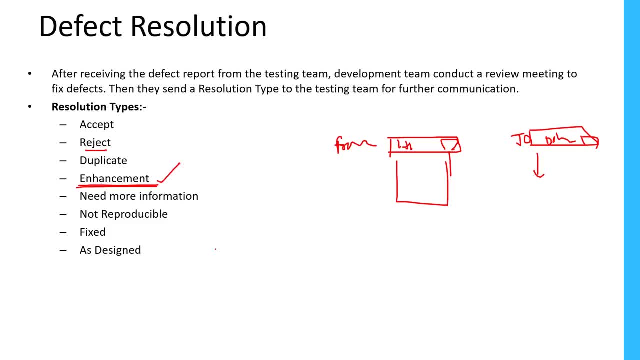 then they can implement this in later builds. that is called as an enhancement And sometimes need more information. So, whatever defect you reported to the developer, that information is not sufficient them to understand the defect. So in those cases they will ask you more information. 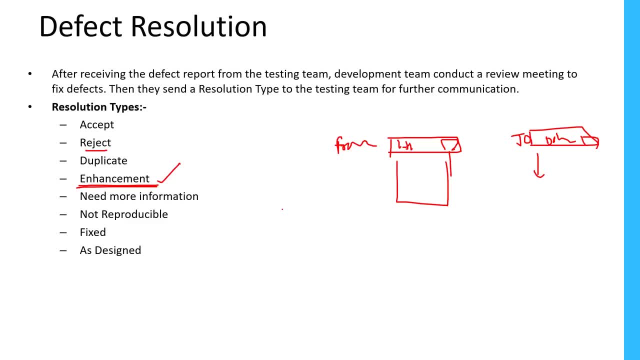 So you need to send screenshots, test case and logs. all these things you have to send to the Developer. that time They will ask: you need more information And sometimes they know they said not reproducible means in the testing environment You are able to reproduce the defect means you are able to see the defect. 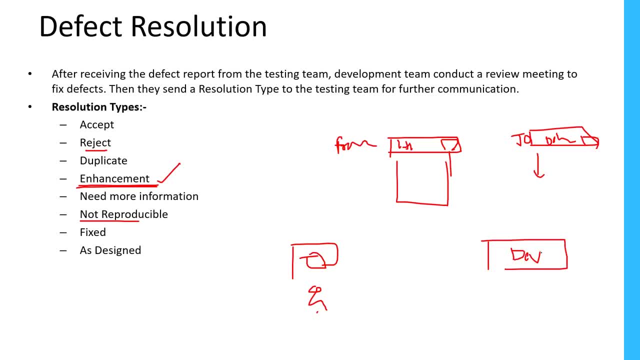 but the same test case, if I exclude, in the development environment. Okay, so the test case will pass. So that means they cannot reproduce the same issue, their environment. So this, those cases also will be there, because the environment completely different. So maybe you're operating. 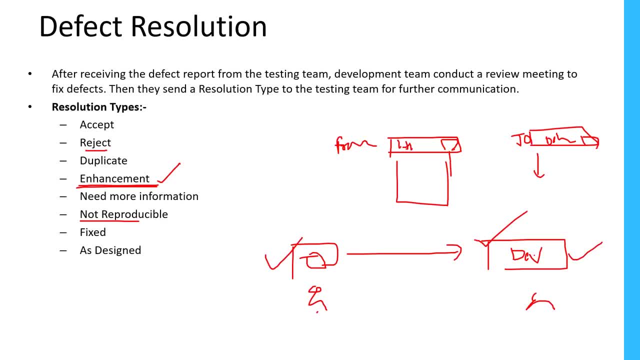 System is different. Their operating system is different. Even the operating systems are same. Your version is different, Their version is different. Your browser is different, His browser is different. So there, we need to do the debugging here. So what is a root cause? 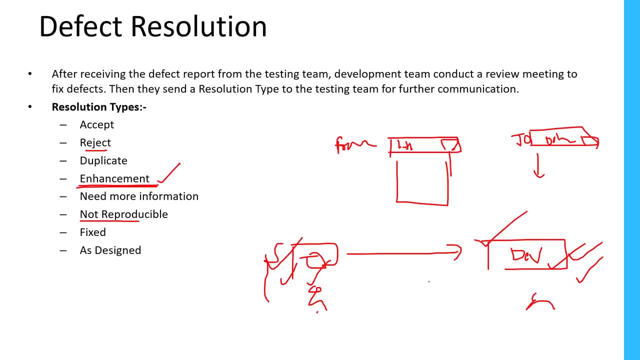 The developer is unable to reproduce the issue in their environment. So we need to dig deep into it and we should also before reporting the defect. We should also exclude the same test case and multiple systems At least minimum three times. So if three times, if you get the age defect every time and multiple systems. 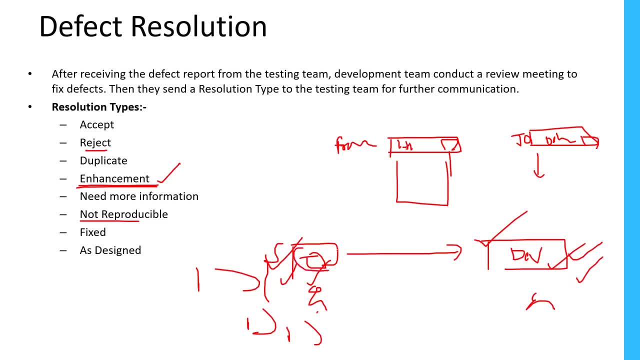 then we have to report that sometimes we may reproduce one system. If I exclude the same test case in another system, it may work properly. Okay, so we should not be in a hurry-burry situation here. So at least we need to try at least three times in at least two to three systems in a team. 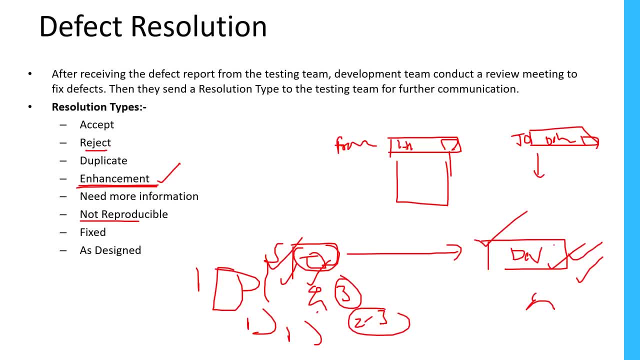 and then we need to finalize: Okay, this is the defect and send to the devil. So if I don't do this, what happens is sometimes you will send the defect and developer is not able to reproduce and he will identify what is the rules cause and we will come back and say: 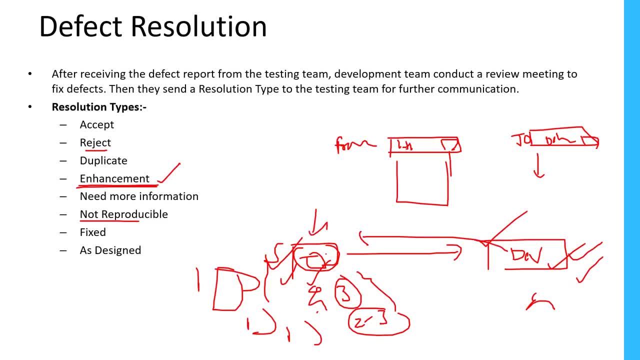 okay, you have some environment error. So that's the reason you are not able to- you are able to reproduce issues in your environment. So that is the environment issue, not application issue. That is your view. That is your problem. You have to set it up environment properly, right? 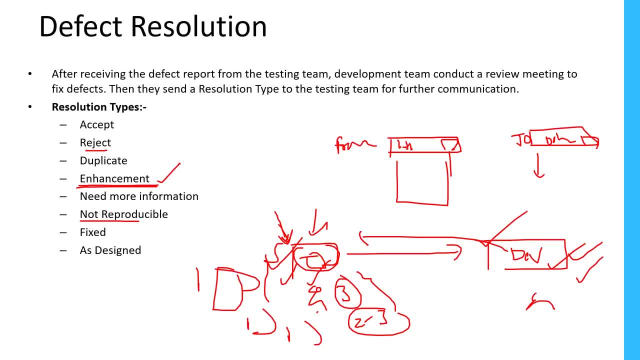 So these kind of things will normally happen in the real world, So not in reproducible developers, and fixed developer will accept it and he will also resolve it and he also fix it sometimes and sometimes he will also say: as designed means, whatever defect you raised, the developer thing. 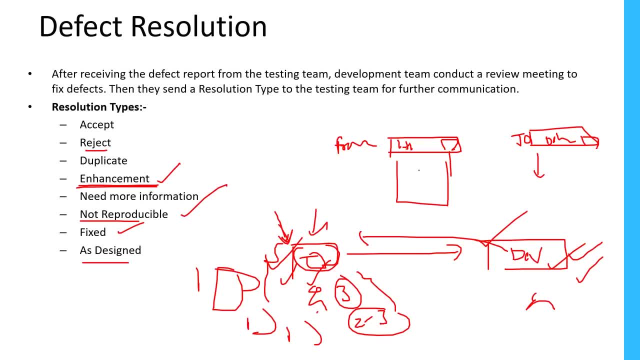 Okay, that is not a defect. that is working according to the requirement. Whatever requirement says, it is exactly working the same way. So it is not a defect. is? it is as per the design. So developers say like that. So that's the reason we need to carefully. 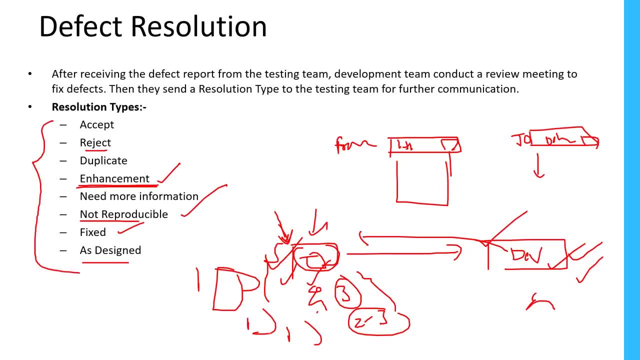 Try this, reproduce the defect once, twice, thrice, in multiple environment And finally we need to check as per the requirement is defect or not, and then finally conclude and then report to the developer team. So this is about defect resolution. different What is a defect resolution means. defect resolution is a opinion about the developer opinion. 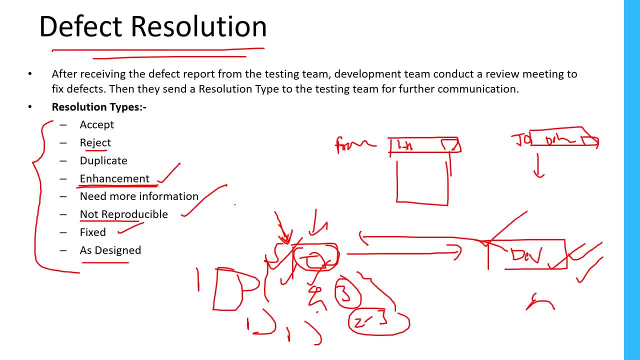 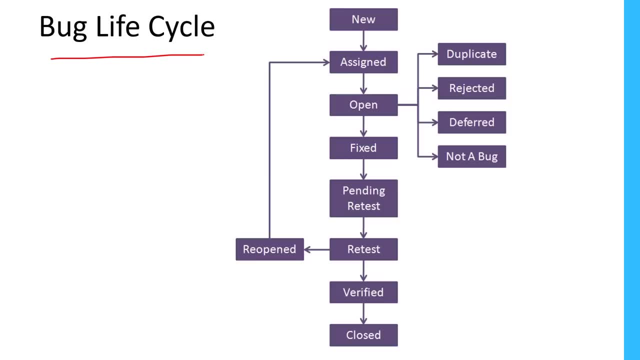 about the developer, about the defect. Okay, So now bug life. This is the last and very important concept in defect reporting. bug defect- Both are same, Okay. so bug life cycle means it will say what are the different statuses, will go on when you start rising a new defect till it closes. 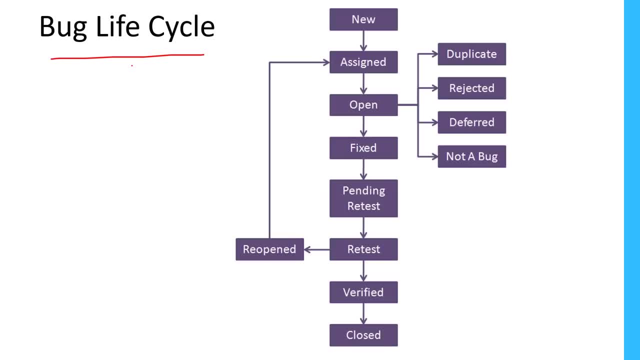 So what are the different stages? is it will go on, So that's called as a bug life cycle or defect life cycle. So in interview people will ask: explain bug life cycle or explain defect life cycle? So you should able to draw this picture and you should able to explain each and everything. 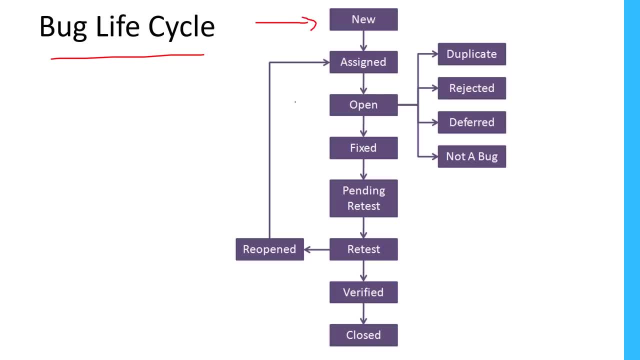 So first, whenever we rise a new defect, that will be in a new state and then it will go to assign state because it will assign to the particular developer and whenever you start working on that it will be in the open state. So once he opened the defect, he has a chance to put a duplicate defect. 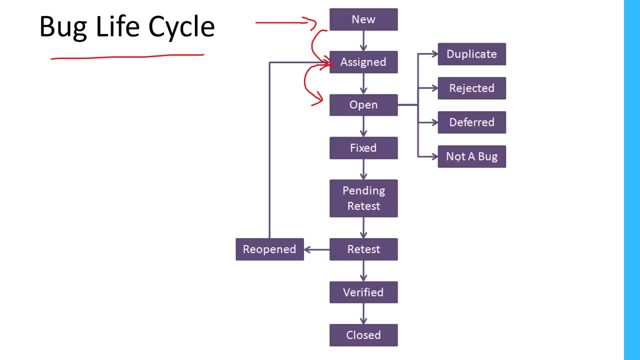 or you can reset the defect, or you can defer, or you can say: not, it bug. What is different here? different means you will accept as a defect, but they wanted to fix it later. That is called as a default. So once the developer is open the defect, they can say either duplicate, 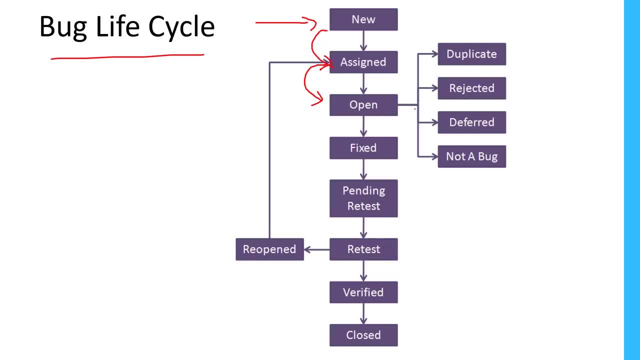 or they can reject, or they can default, or they can say not a bug. Suppose he feels okay, It is a bug, then he will fix it. So once he fixed, the status will be fixed, and once he is fixed again the tester has to retest. 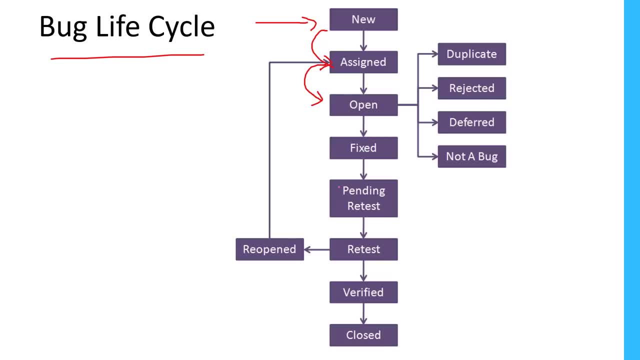 and then confirm whether it is working, or working fine or not. that's called pending retest. So whatever fix the defect, we need to retest the same thing And once we retest is done, suppose if still it is not working again, We reopen the defect again assigned to the demo. 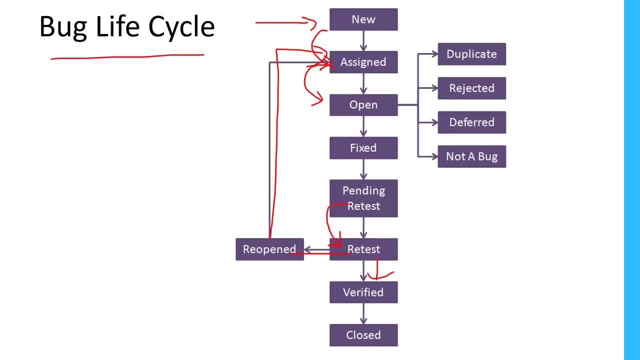 If, while retesting, if it is working fine, so go to verify stairs and then close the state, close the different. So from here to here the defect will go different stages. This is called as a bug life cycle or defect life cycle. So at the time of retesting, if the developer still not working again, 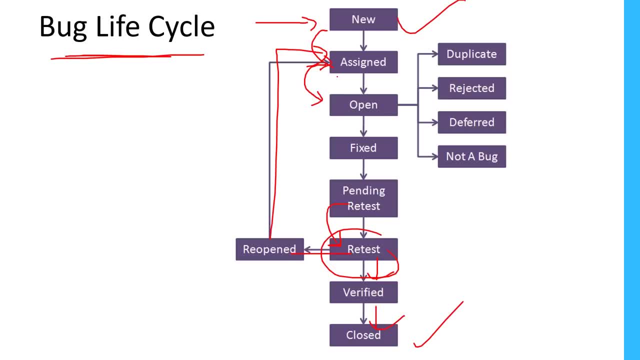 we need to reopen, And again same defect reassigned to the developer. So this cycle will go on till the defect is closed. Okay, so that is defect life cycle or bug life cycle. Okay, So is it clear so far. So bug life cycle will talk about different stages of bugs, different statuses of bugs. 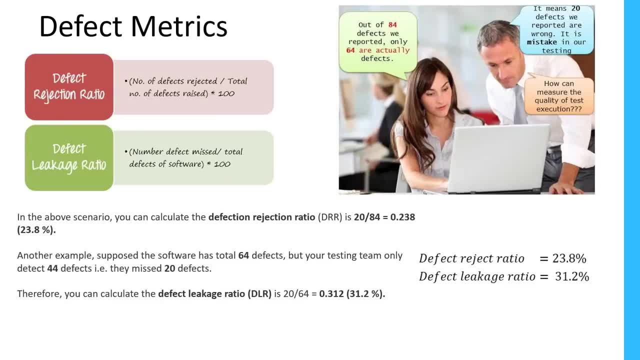 Okay, So finally, defect matrix. So we need to also calculate defect matrix. This is very important activity because this will give us our effectiveness, like how effectively we have done testing, how well we have done. The testing will be represented by the matrix. So matrix gives the clear information right. 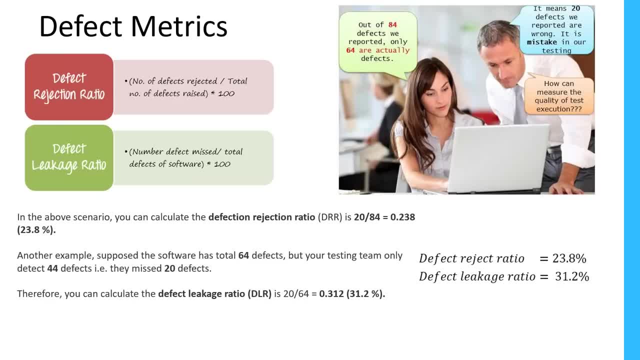 So until unless we have a matrix, we don't know how well we have performed, So we need a matrix. So especially for the defects, we have a two important matrix, that is, defect Rejection ratio, defect leakage ratio, defect rejection ratio, defect leakage ratio. 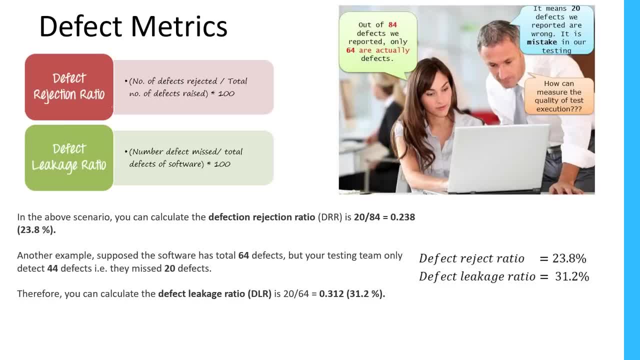 These are very important and these two metrics will tell quality of our testing. So how well we have conduct tested. We have conducted testing very well or we have conduct testing very bad. So that will be decided based on these metrics. So management will always calculate this matrix. 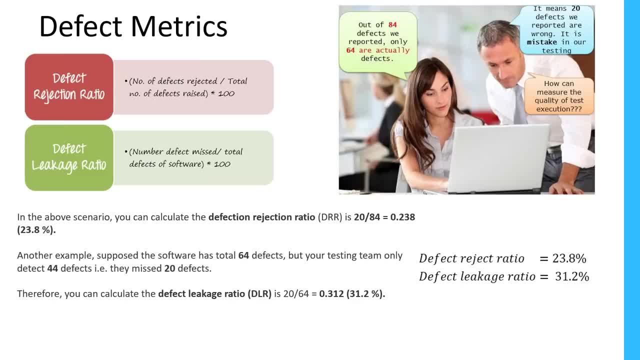 Okay, Let's see What is rejection ratio. So, for example, tester says out: 84 defects be reported. Let's say 84 defects be reported. Among these 84, 64 defects of actual difference means the rest of them are not defects. 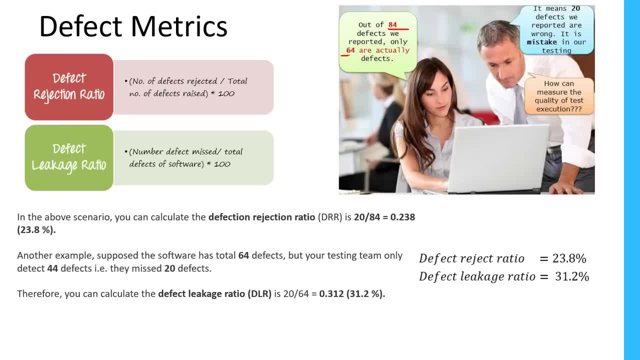 but we thought they are the defects and we raised them against the development. So rest of the defects: the developer is rejected. So developers is not the difference, So that means they are invalid defects. So invalid defects is our poor performance. Okay, So suppose we have raised 50.. 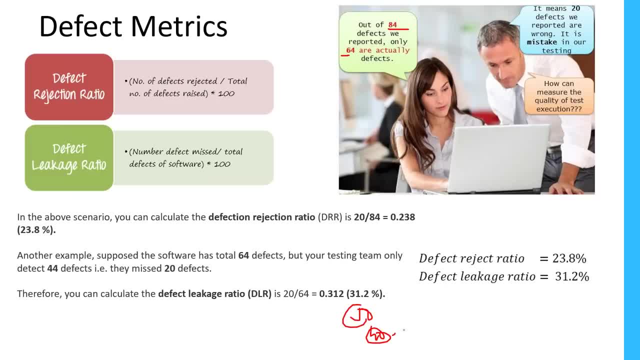 Defects, out of them, 40 or invalid defects. That means it is wasted about tester time and also they have wasted our developer time right. So invalid defects will reduce our performance. So more number of invalid defects should not be there. So we need to make sure as a testing. 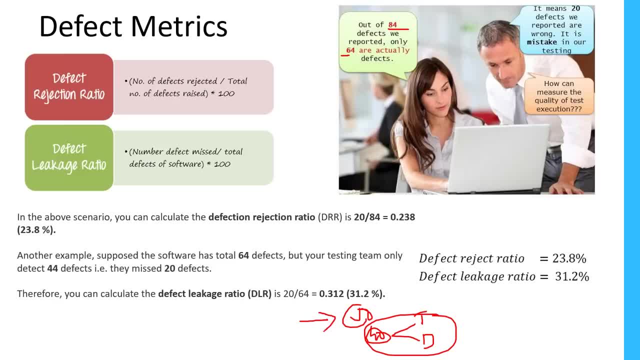 We have. whenever we raise a defect, should every effect should be valid. Different need to make sure out of 50 over one or two is fine, but more percent of difference should not be invalid. Okay, So let's say 84 defects, 64 are actual defects. 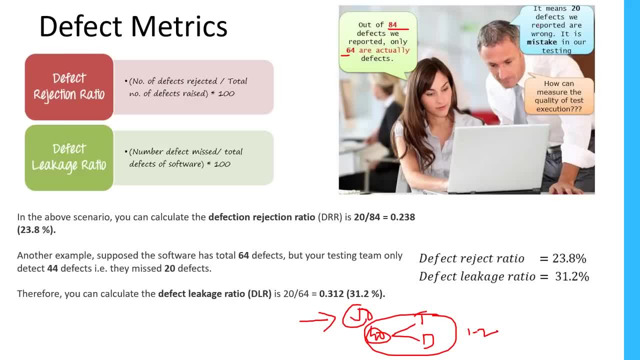 and remaining, or 20 or invalid effects. So that means 20 defects are reported are wrong defects. These are by mistake. We have reported those as a defect. They are. comes out the invite Now how we can measure the quality of test execution. 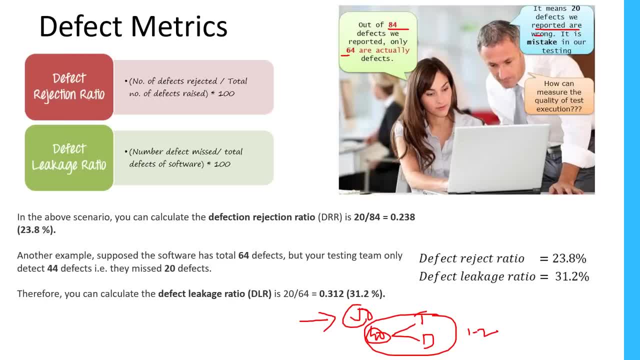 How well we have executed our test. So defect rejection ratio. So the first form is this: one number of defects rejected by the developer divided by total number of defects, We raised into 100.. If we calculate this, this will give you one percentage, that is a defect rejection ratio. 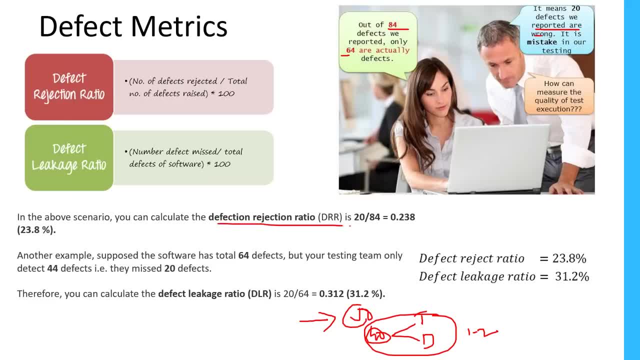 Let us calculate it So: defect rejection ratio- DRR means defect rejection ratio. So in interview people will ask you the questions like this: So what are the matrix you follow in testing? So these are the two important methods: defect rejection ratio, DRR. 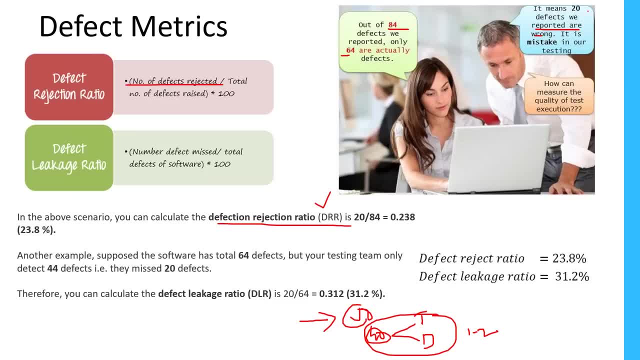 So here, number of defects rejected. So how many number of defects rejected? 20, so 20 by total number of defects, 84 be raised. So 20 by 84 is equal to this one We will get, and if you do, divided by 10,. 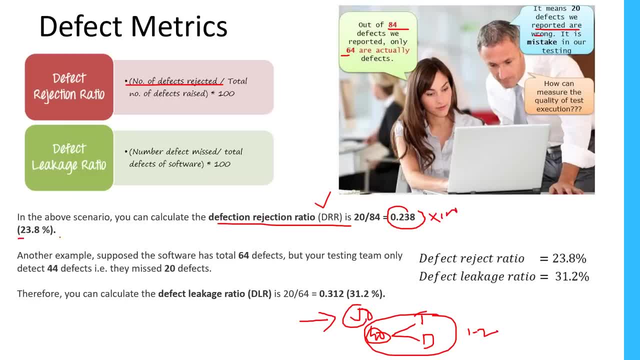 if I do, divided by if we do 100 into 100, will give you this much. So 23 for 8% of these are defect rejection ratio. So 823.8% is a defect rejection ratio. Similarly, we can also get defect leakage ratio. 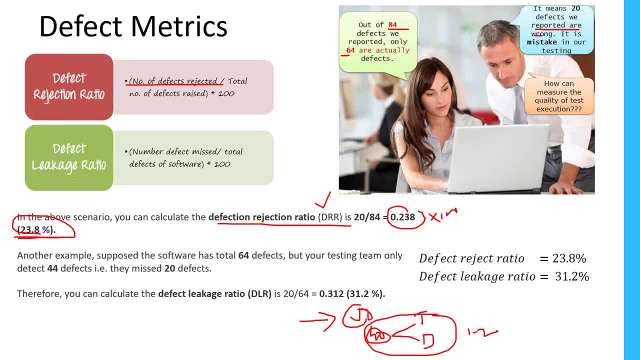 So what is defect Leakage? defect leakage means how many defects we leaked. We have not able to identify those two. application is having some defect, But as a test engineer we missed those defects. So whatever the defects we could not identify, the customer will find out in their environment. 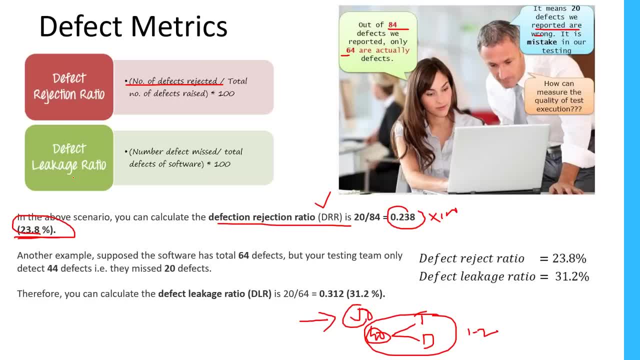 right, the customer is started using it. if you miss the defect in testing, So obviously the test customer will get the same difference. So that's comes under defect leakage. So defect leakage in the sense the tester, He will not identify those defects, So he could not identify those defects. 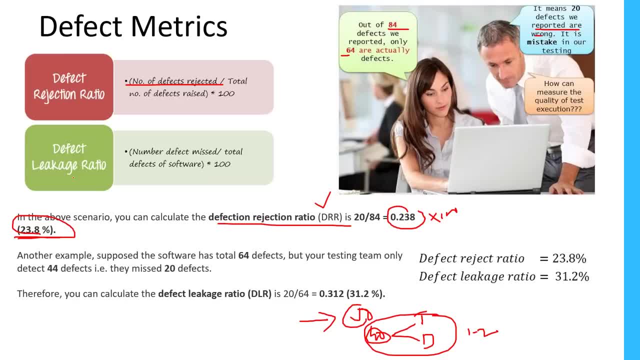 So those defects are reported by the customer. They are called as a defect leakage. So what does the defect leakage ratio is number of defects missed by the tester divided by total number of defects in the software into 100. So let us say 20 defects are wrong defects and 64 are actually defects. 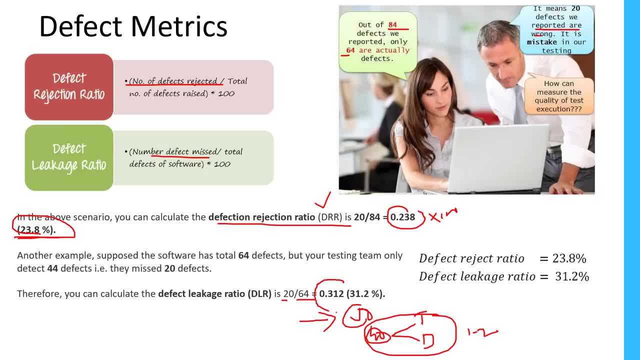 So 20 divided by 64. This will give you this number. So this is a defect leakage ratio 31.2%. is it defect leakage ratio? defect leakage ratio: number of defect missed by the tester divided by total defects in the software. So how many total defects in the software? only 64?. 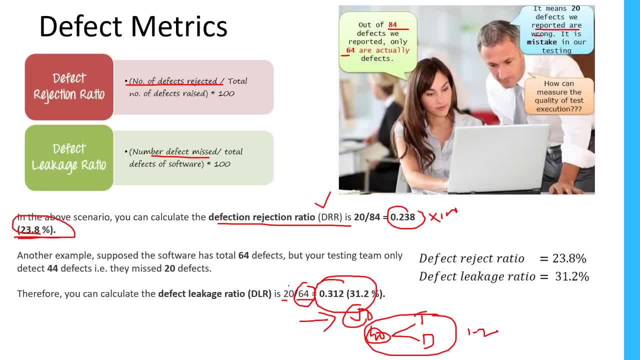 These are actual defects. but how many defects we reported and miss 20 defects? Let us assume 20 defects be missed, So 20 by 64 is equal to this much percentage comes under defect Leakage ratio. Okay, So this is how we need to calculate two different methods. 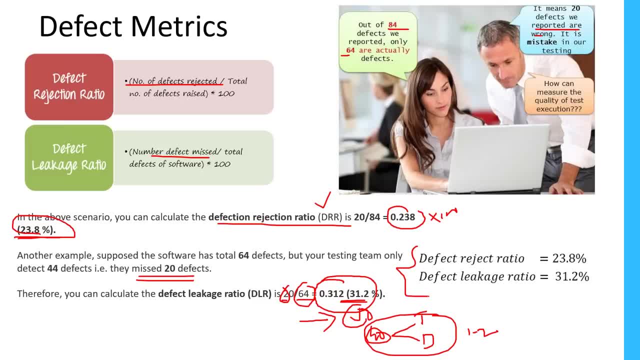 This is truly related to the defect matrix. So these metrics will give the management a clear picture how effectively we have done testing, how well we perform the testing. Have you done the poor testing or will that the good kind of testing will be decided by this Matrix. 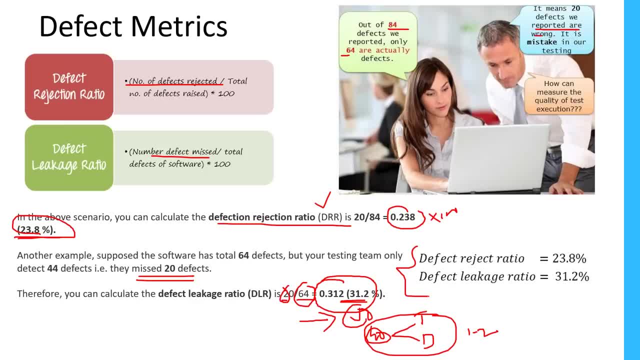 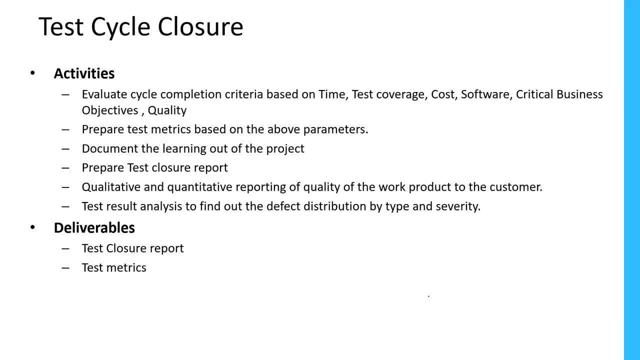 Okay, So management is always need these Matrix to calculate our performance. And the last basis test closure. So once we have done the test cases, we have executed, we have found the defect, we reported them again, retested the pixel defects and everything is done. 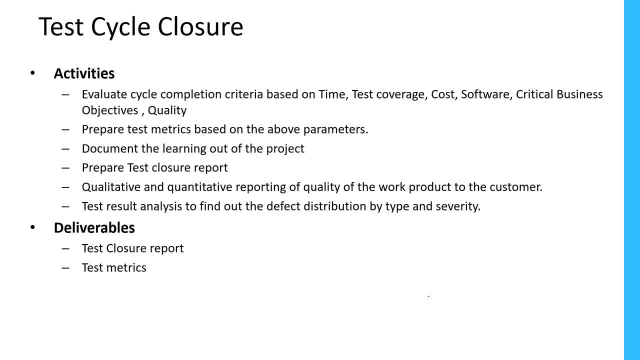 Finally, all test cases have been executed, completed. all the defects have been closed. The next final step is we have to stop our testing at some point of time. We have to certify our build. So once we have, when we need to certify our build, once you are, all test cases are completed. 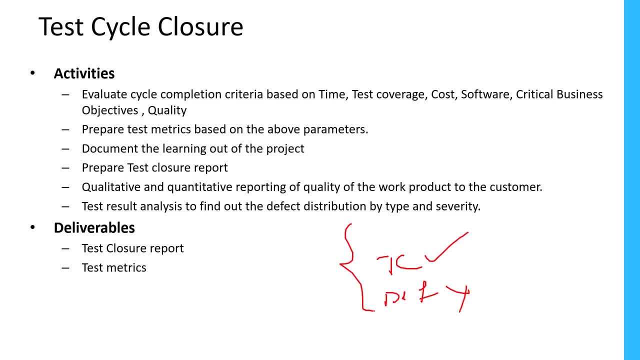 There are no Defects, and then we have to certify our build. So there will be some criteria and this is taking this decision, taken care by the management leaves and managers. So they will analyze the test closer, report and test matrix and then, based on that, they will decide whether we need to stop the testing here. 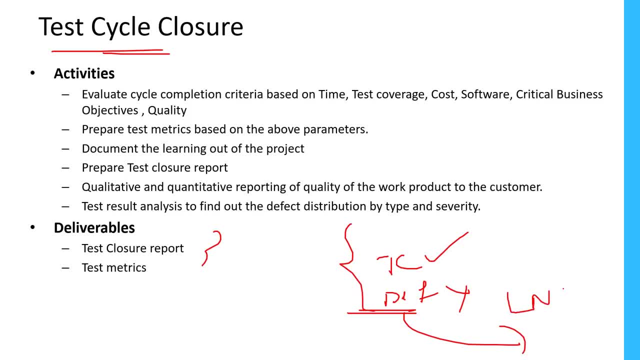 Can we certify the build? should we go or no go? So, go or no go. So this will be decided by the management team. Okay, This is a test cycle closure. This is the last Phase of testing. So test planning, test designing, test execution, defect reporting and test cycle close. 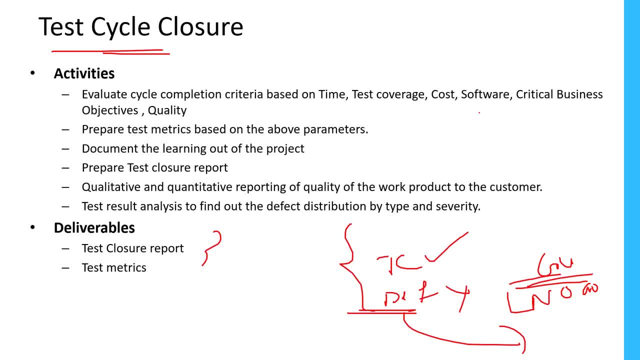 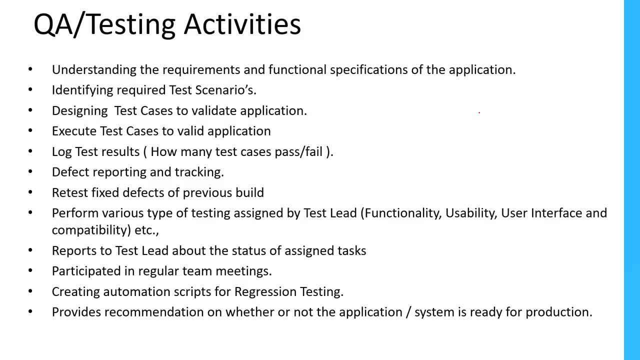 This is all about STLC process, complete end-to-end the process of STLC or testing process, which will happen in the real time, So normally the day-to-day basis. as a tester, we will perform these activities like we need to understand the requirements and functional testing specifications, identifying the required test scenarios. 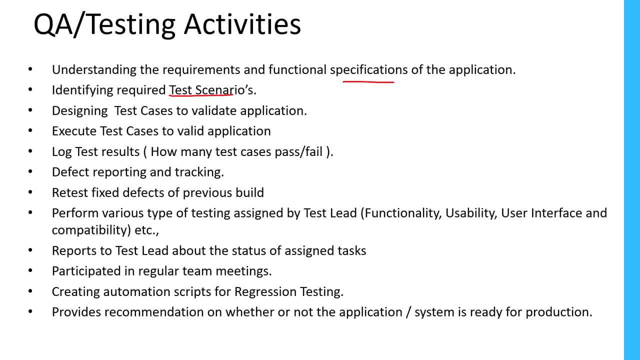 This is the roles and responsibilities of the testing in here. Okay, So even in interview, somebody asked you: what is your role in your project? What do what to do on a day-to-day basis, Like, what are your activities on a day-to-day basis as part of testing? 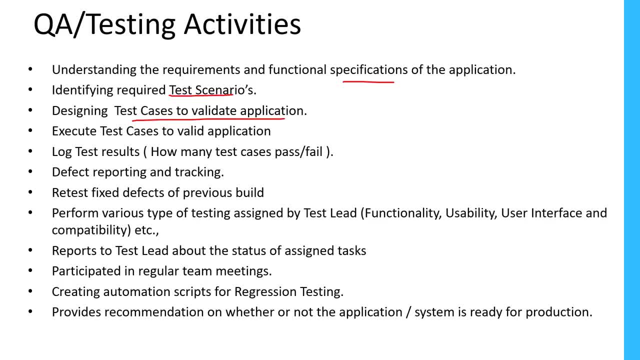 Then you have to say all these things, So designing test cases to validate application, execute your test cases, logging test results- How many are passed or how many are failed- and defect reporting and tracking and retesting the fixed defects. Okay, And the performance? 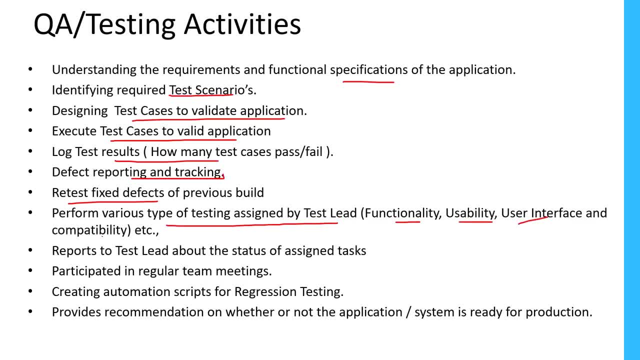 Various type of testings, like functional testing, usability, user interface, compatibility and Etc, and we need to report the leads how much status we have done. and we need to also participate in the regular team meetings and creating automation script for regression test cases and provide some recommendations on whether or not the application system is ready to production or not. 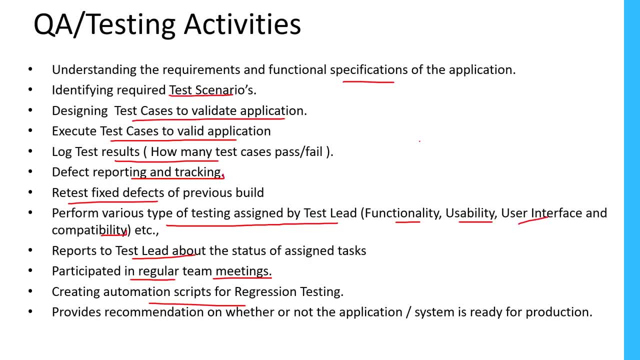 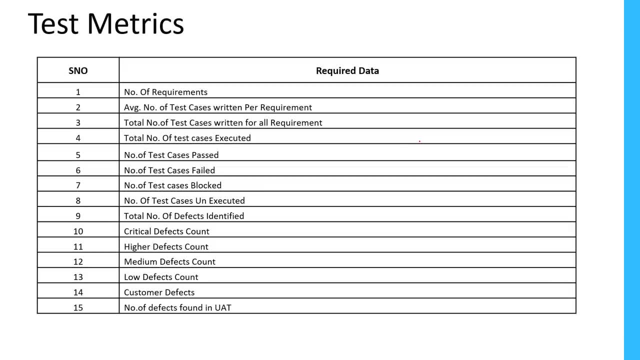 So these are all the things we need to do as part of the tester. as a testing year, We have to do all these kinds of activities, Okay, So here these are all testing metrics, because this is all, again, management level activity. So these test metrics will be calculated once we completed the complete cycle. STLC cycle. 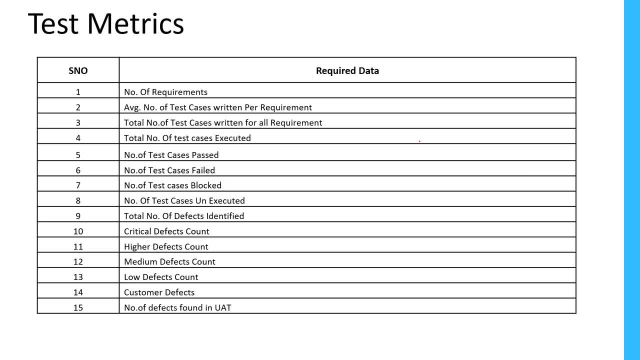 So test planning, designing, exclusion, different reporting, closure. once everything is done, Finally, we will have a matrix, because the matrix will give you the clear picture how we have done well or we have done a poor testing, or we have done Well testing or good kind of testing. 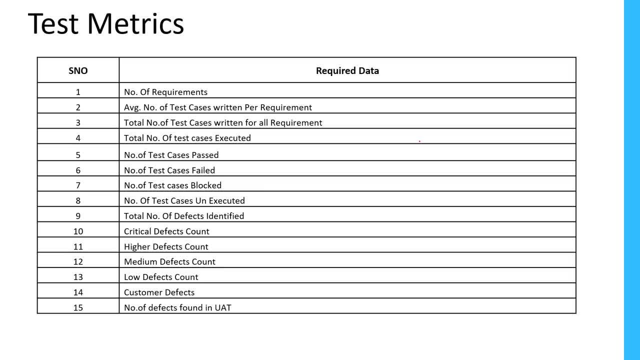 So that will be decided by using metrics itself, or if there are any improvements needed in future projects, that is, also give the clear picture by using this test methods. Now, normally, if you want to calculate these metrics, we need certain input data. Okay, so like number of requirements we have. 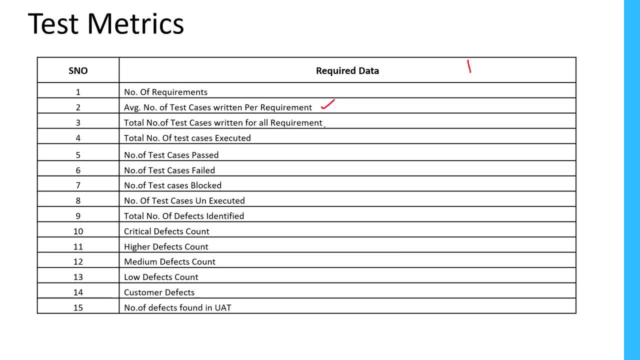 and average number of test cases written per requirement. total number of test cases are written for all the requirements. total number of test cases is executed. total number of test cases Passed, test cases failed, blocked and number of test cases un-executed. total number of defects identified. critical defects down. higher defects. 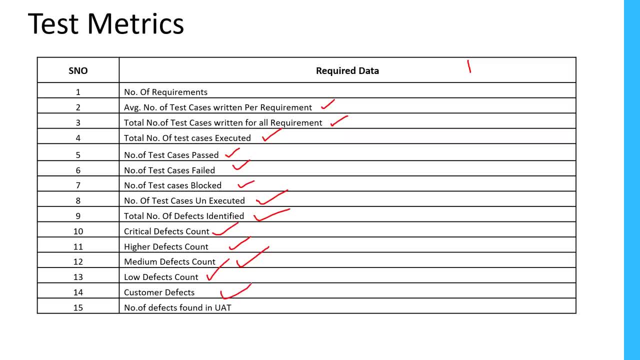 found medium defects down. low defects down. customer defects means customer found some defects after releasing the product and number of defects found in UIT testing. So if you have this data and based upon this data we can calculate certain metrics. So normally management team will collect this data from the test engineers, customers. 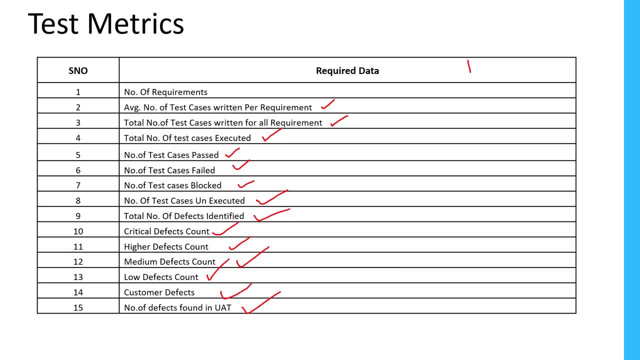 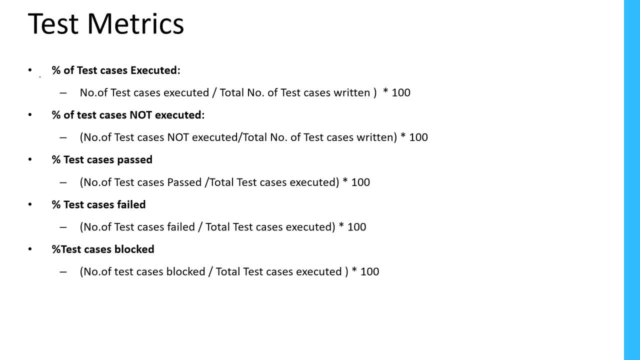 and developers, From everybody, and based upon this data, they will calculate certain metrics. Okay, So let's see what are those metrics. So percentage of test cases executed, how we can calculate so number of test cases are executed divided by total number of test cases. 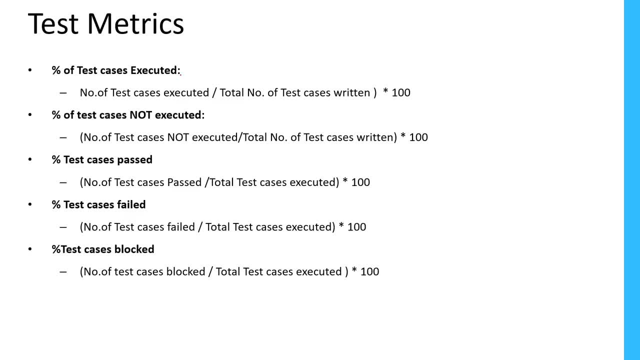 We have written into 100. So this will give you percentage of test cases executed and percentage of test cases not executed. So number of test cases are not executed divided by total number of test cases written into 100. This will give you percentage. because always management you lack. don't see the numbers. 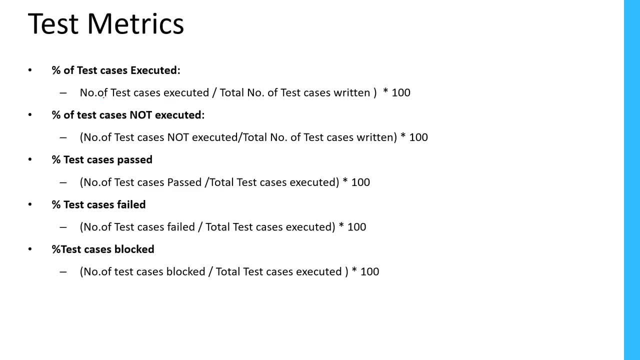 They will see only percentage. Okay, So that's the reason we need to give the numbers. We don't give the numbers directly. Let's say, 100 test cases. I have 50 test cases I have executed, so we don't give this number. 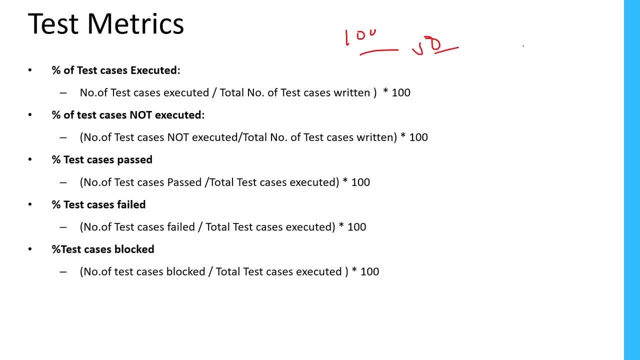 So they will just ask the percentage. Okay, So a hundred percent. I have executed 60% of the test case and 30% of the test is still pending, So we can give a number like this in percentage form. So number of test cases passed. 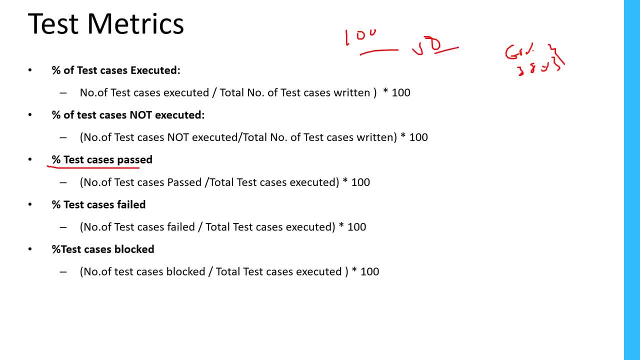 So let's number of test cases passed, divided by total test cases are excluded in hundred, and number of test cases are failed divided by total test cases executed in hundred, that will give you percentage of test cases failed. percentage of test cases are blocked. Okay, These are day-to-day basis. 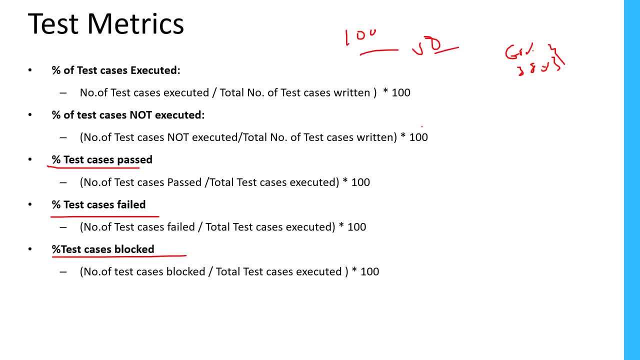 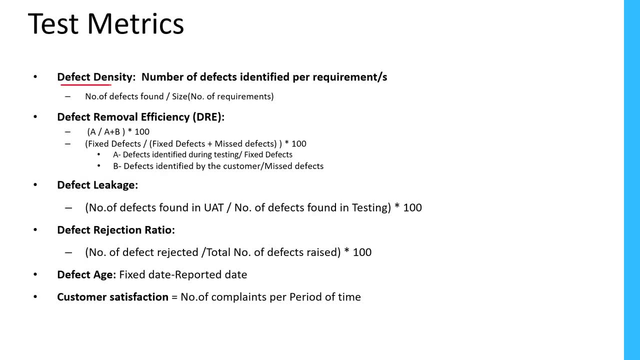 We will calculate and testing metrics, But along with this there are some more metrics We have to calculate by the management team. and defect density means number of defects. identify per requirement. for one requirement, how many defects we identified as by the tester. So that is a defect density: number of requirements: number of defects found. 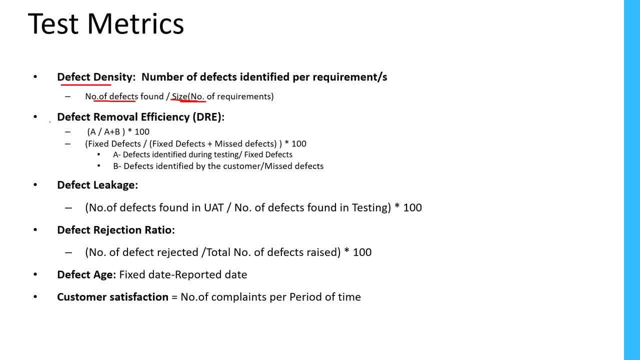 Divided by number of requirements and for more very important metrics is different removal efficiency. So defect removal efficiency DRE is calculated after post-production, means after delivering the product to the customer. We will calculate this. So this will give you the clear picture how much quality product we have delivered to the customer. 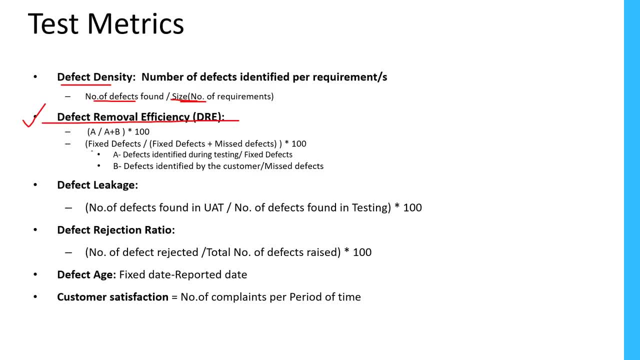 So the farmer is A by A plus B into hundred. that means fixed defects divided by fixed defects minus plus missed defects into hundred. What does it mean is fixed defect? means tester is identified those defects and developer fix it. So they are the fixed defects. 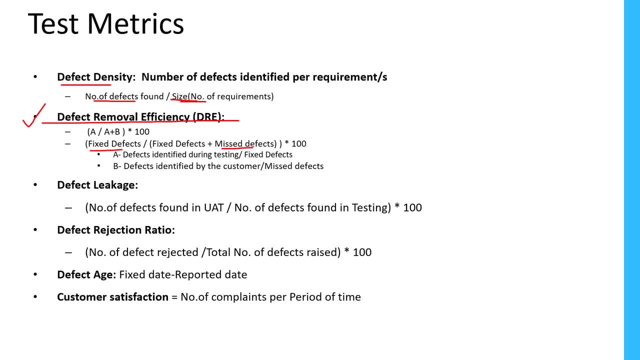 And missed defect means the customer is identified those defects. tester has missed those defects. tester is not able to identify those defects, But customer found these issues and in their environment by using the product. So he will report the defect also. right, So we will calculate defect removal efficiency like this: 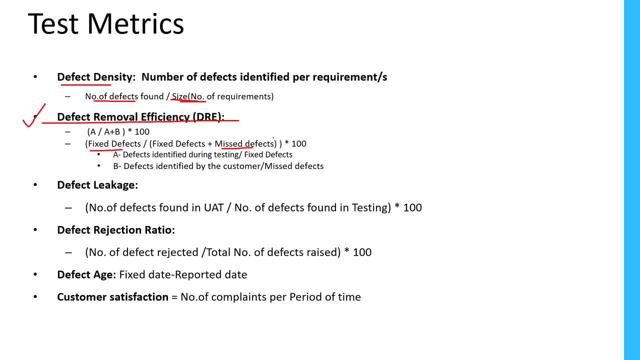 Fixed defects divided by fixed defects plus missed defects into hundred, So this will give you defect removal efficiency And then defect leakage. So, as I said earlier, defect leakage means how many number of defects we leaked means we haven't identified. So that is defect leakage. 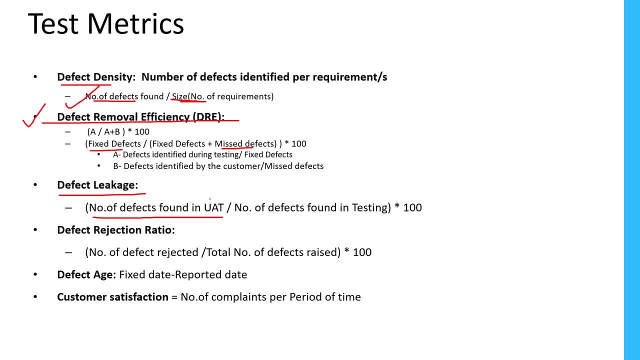 So number of defects found in uat. uat is the next phase of our testing, divided by number of defects found in testing. So uat is the next phase after system testing. There is a uat testing. user users or customers will do this testing right. 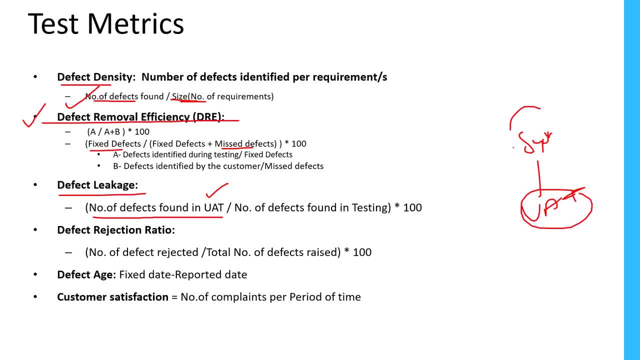 So number of defects found in uat divided by number of defects found in testing into hundred, that comes out the defect leakage And defect rejection ratio. Okay, We already calculated this. So number of defects rejected by the developer developed divided by total number of defects, We raised into hundred, that will give you defect rejection ratio. and defect age means: suppose today we have raised defect and after two or three days the developer fix the defect. So what is the duration of this that comes out? the defect age means fixed date minus reported date that comes. 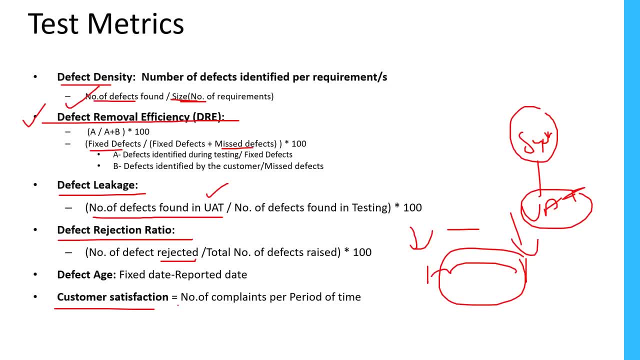 out the defect age and how we can calculate customer satisfaction. How we will know whether the customer is satisfied or not, that again depends on the customer mindset. So, number of complaints per period of time, So we will just say one to first quarter, one to three months. How many complaints the customer has given and, one to six months, How many issues or how many complaints the customer has given. So based on that we will easily identify, or we will get to know, whether we deliver the quality product to the customer or not, customer satisfied or not. 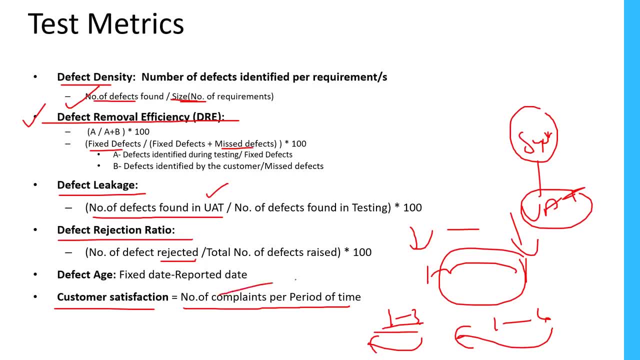 So we don't have specific method for this. this because this is just human mindset, right? So the number of complaints based upon the number of companies, Suppose. normally the customer reported more complaints within one month or three months. That means the customer is not happy with that, our product. 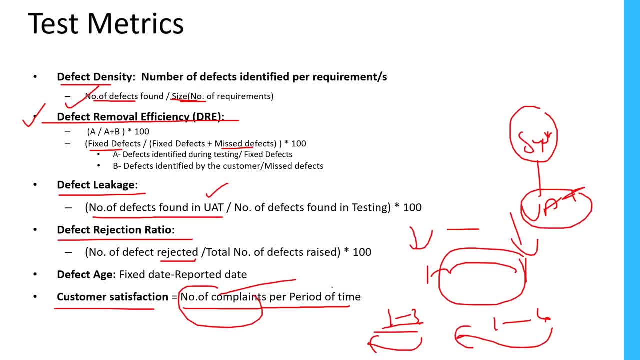 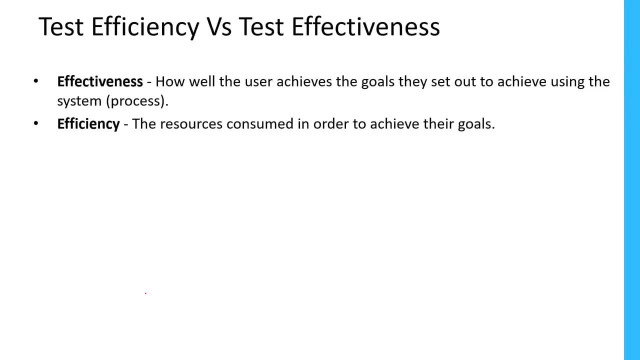 There's a common nature, right if we didn't get any more complaints? So that means the customer is happy. So that's how we need to calculate the customer satisfaction. These are all the few test metrics. along with this, We have effective Yes and efficient. 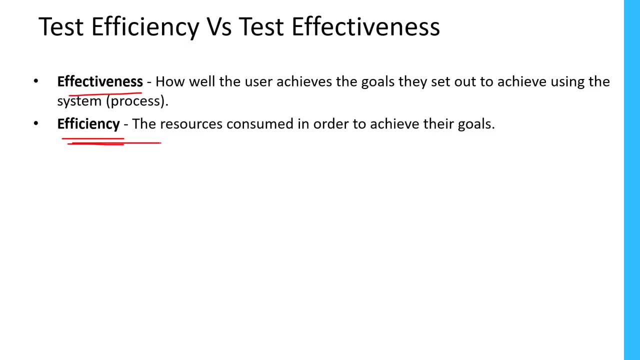 These are the two last metrics. We have effectiveness. effectiveness and efficiency very important, but both seems very similar, but not exactly the signal. Effectiveness means how well the user achieves the goal The set out to achieve using the system process. efficiency means the resources consumed in order to achieve their goals. 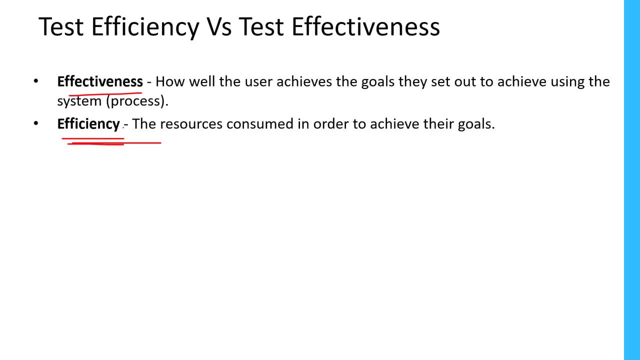 So let me just clarify these difference between effectiveness and efficiency. Suppose there will be some goal: How well the user achieves the goals the set out to achieve using the system. So if you want to reach that goal, whatever things we have, we need a resources. that means resources means either hardware resources- 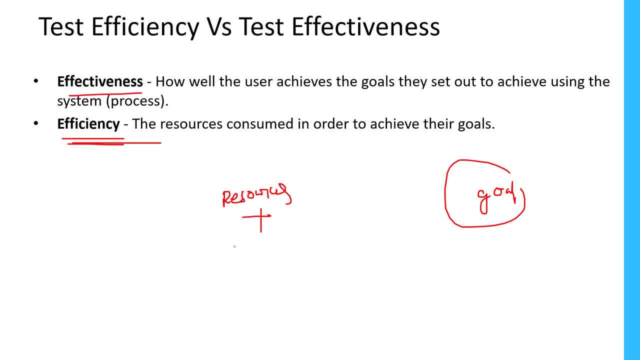 or human resource or team plus process. We have to follow certain process right. if these two things are well and then we can easily achieve the goal. So if you want to achieve the goal, we need to have skilled resources, proper resources and good resources, and also we should follow process effectively. 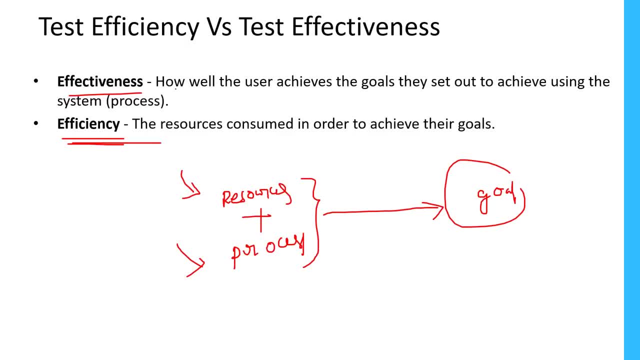 Right, then we can achieve the goal. So effectiveness says how well the user achieves the goal They set out to achieve using the system. So by using this process, by using this process, how well the user achieves the goal, That means how well they have utilized this process to achieve this particular goal. 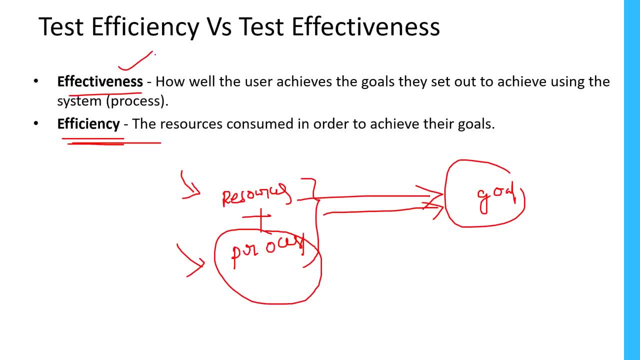 That is called as an effectiveness. So here, effectiveness is talking about the process. Remember this. Okay, effectiveness is a talking about the process: How effectively we use this process to achieve our goal. How effectively we use this process to achieve our goal, that is called as an effectiveness. 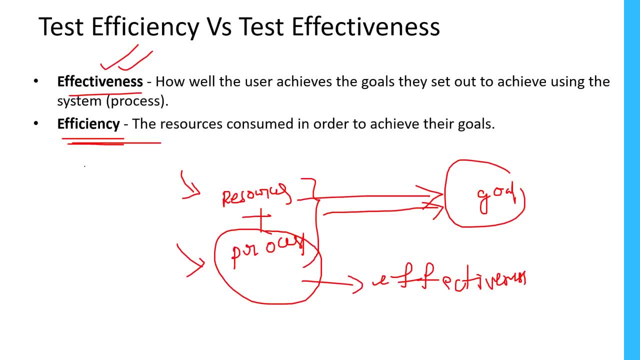 It is talking about the process we follow, And process means, again, test planning, test designing, execution- These are all comes under the process. So how effectively we use of this process. We followed this process to reach this goal, that is effectiveness. and efficiency means the resources consumed in order to achieve their goals. 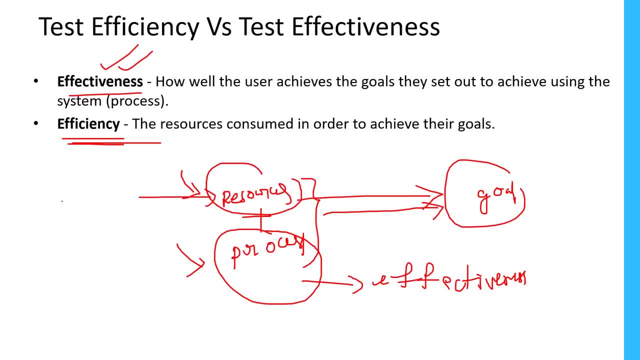 Efficiency. talk about the resources, not the process. So how well we utilize These resources to achieve this goal- A small difference, Okay. how well we use this process to achieve the goal is called effectiveness. How well we use these resources to achieve this goal is called efficiency. 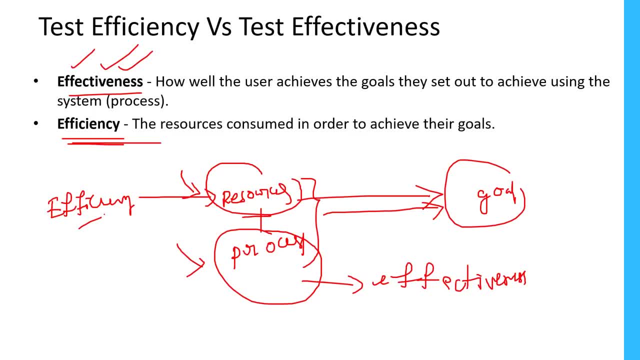 That's it, simple: differentiation, effectiveness and efficiency. effectiveness is talking about the process. efficiency is talking about the resources. Suppose I have five resources. Let us say I have five resources, I have 15 days of duration and five resources. almost the task is completed within 10 days and rest of three resources are completely free. 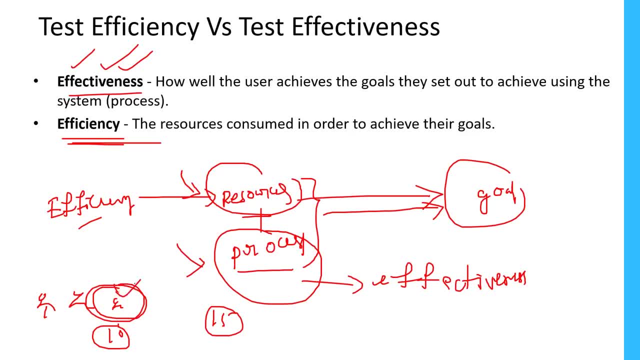 So what does it mean is I haven't effectively used these two resources to complete my project, So that is not comes under the proper effectiveness. So I have to utilize the resources- means hardware, software, human resources, everybody- effectively. That means I have to use the 10th effectively without wasting any time. 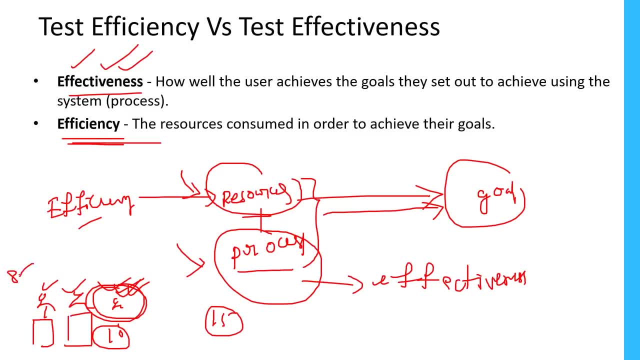 So per day, if they spend eight hours, we have to utilize, we have to get the deliverables or we have to get work on eight hours every day till the entire duration. That is the main thing. So efficiency means how well we have used the resources to reach that goal. 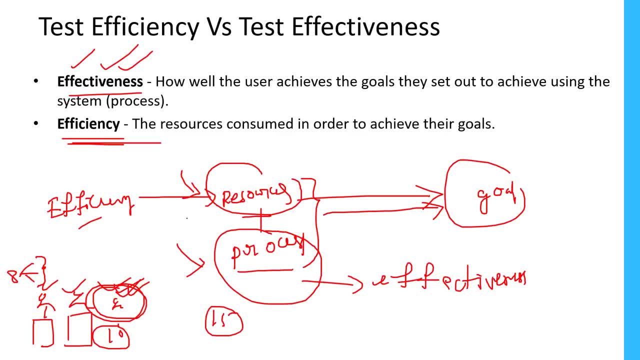 and how well we have used this process to reach the goal that is called as a effectiveness Efficiency, and so these are the two important metrics we have, So I'll interview these. questions will be asked. So these are all related to the matrix. Okay, 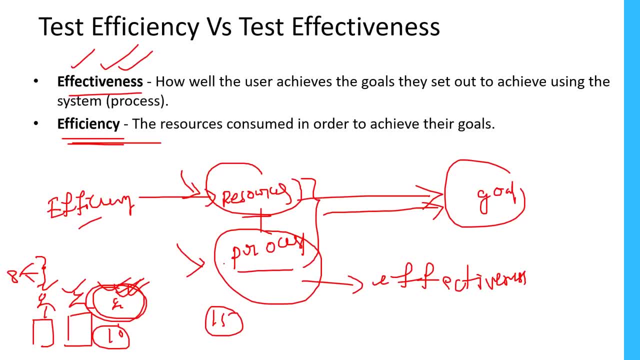 So with this we have done the complete STLC process in the real time: how we have to start, where we need to start, What are the testing activities we do, What are the input documents they required, What are the different duty we need to do every day today? 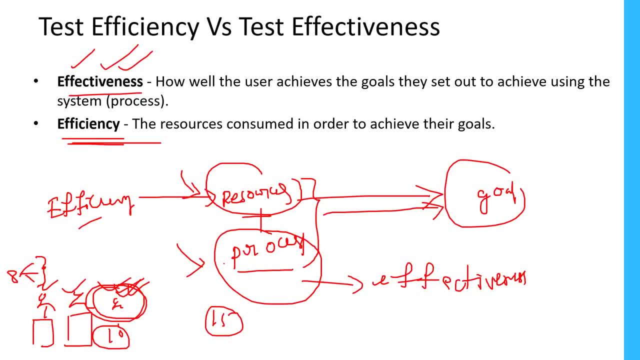 What are the activities we do? Okay, So what are the different meetings We'll conduct? how to get the bill, how to install the bill, how to test the bill, How many cycles CBRT, priority, defect reporting- These are all comes under the STLC process. 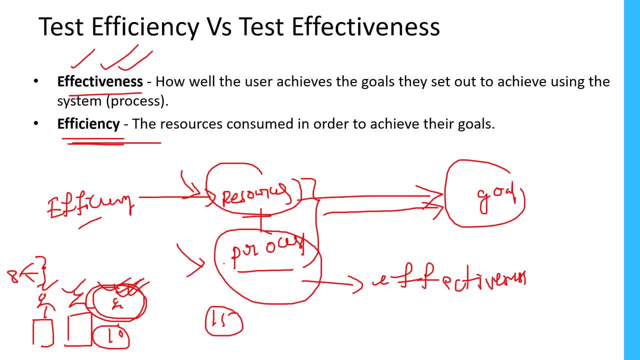 So once we are clear with this, then we can enter into the project. So any questions so far. So I have done with this. So STLC process now. if you have any questions now you can.